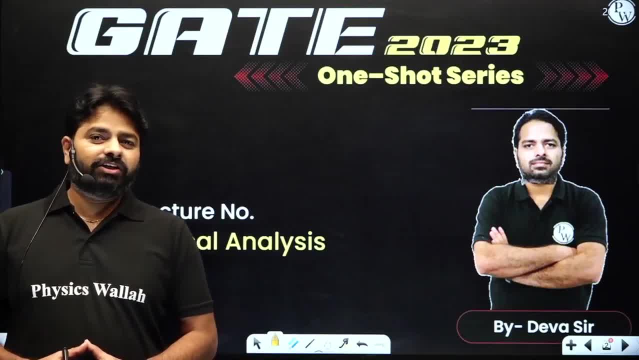 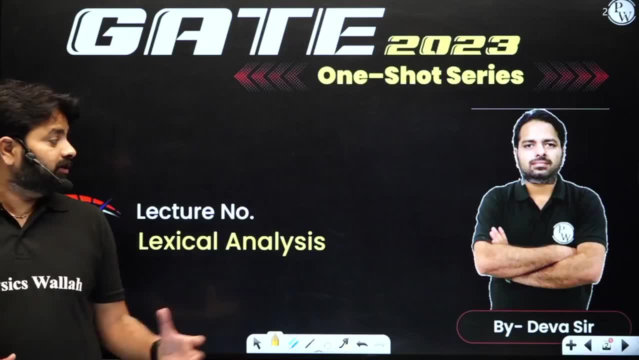 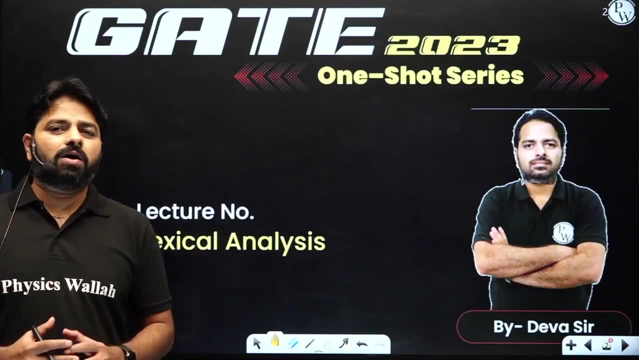 hello friends, we are going to start the compiler design, in which the first lecture, which is lexical analysis, the weightage of the gate exam is very less, but which will give you insight into the compiler design, how we begin the whole program while scanning, how the tokens are recognized in 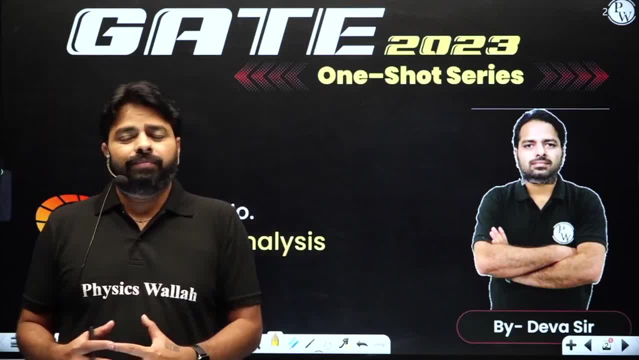 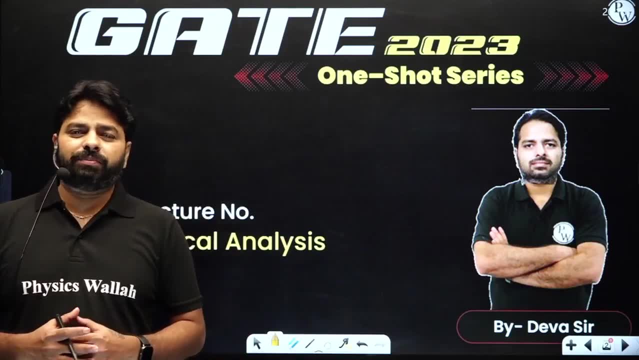 the lexical analysis, if you look at the weightage of the compiler design in the gate, which will be varying from four to seven marks in between. so average of five to six marks you can predict from the compiler design, but sometimes seven marks, sometimes even four marks we can, you know, predict. 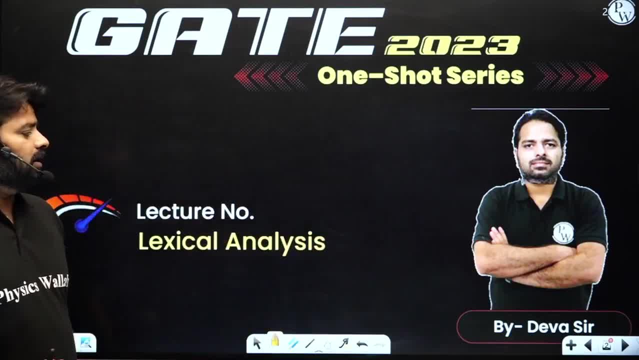 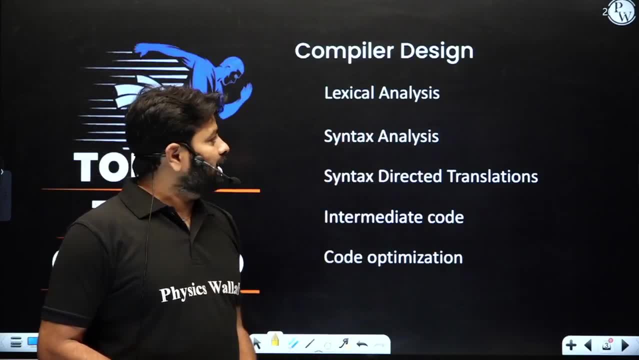 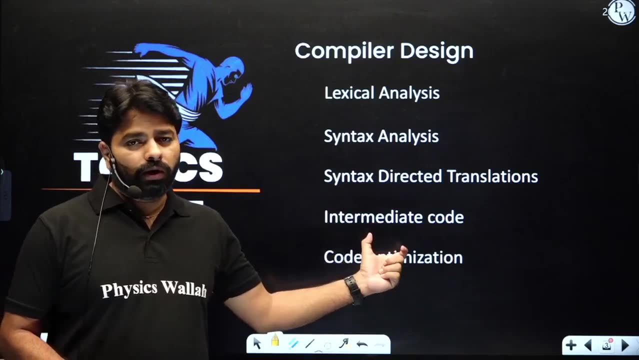 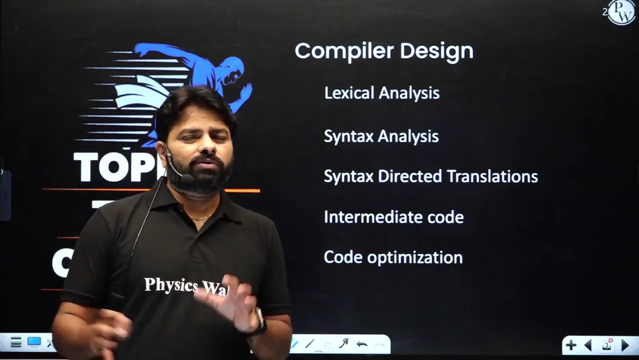 from the compiler design. okay, in this compiler design, we will be learning lexical analysis and i will help you to learn syntax analysis, then syntax directed translations, then intermediate code representations, then code optimization. okay, so, which will be covering the overall, the weightage around four to seven marks which will be predicted in the exam. 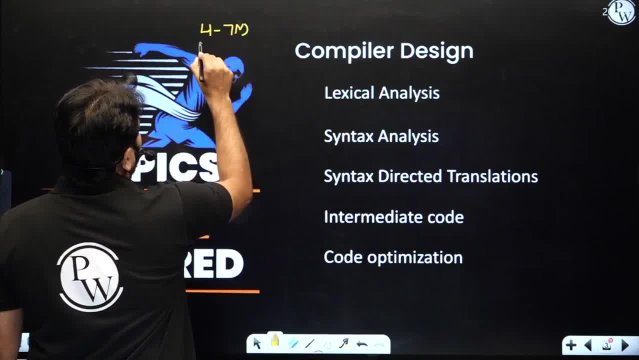 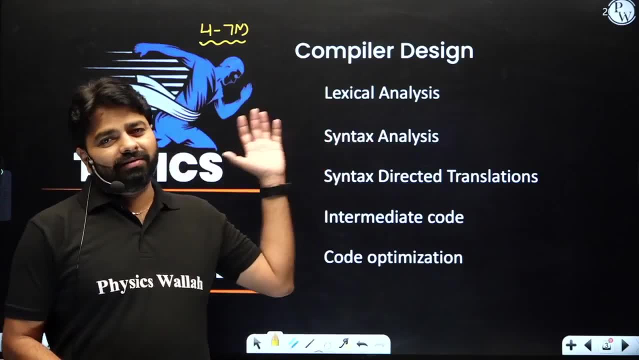 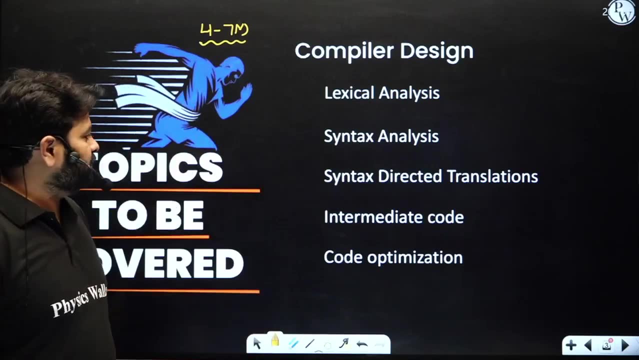 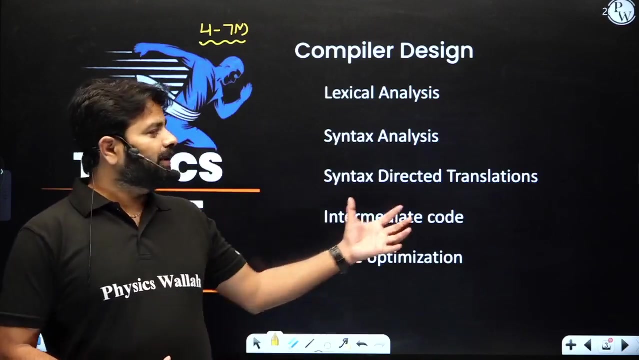 four to seven mark. in some of the years you will see five, six. the most of the years you will see five or six marks. you know unpredictable marks, like you know, sometimes four and seven. they are unpredictable but still we can guess it may happen in future. okay, let's start with the lexical analysis. but you know, as we are beginning the compiler design. 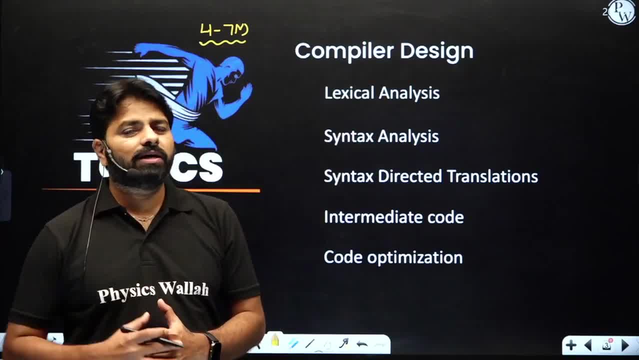 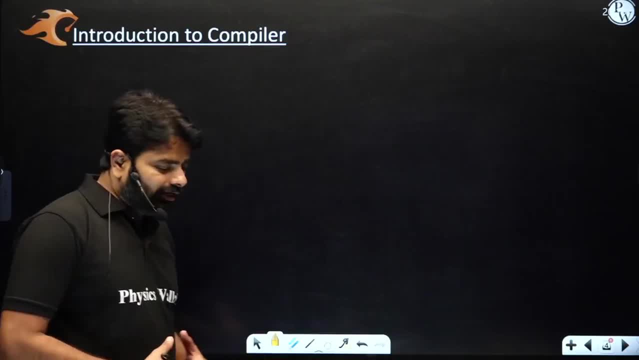 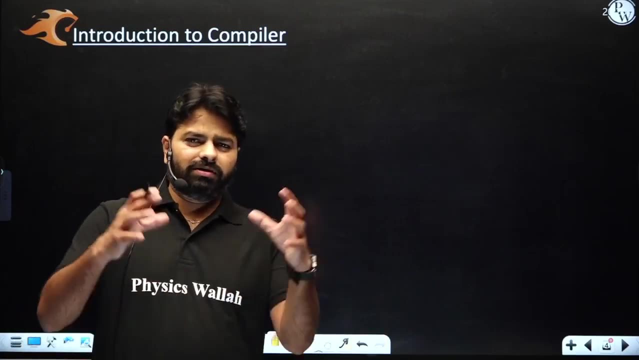 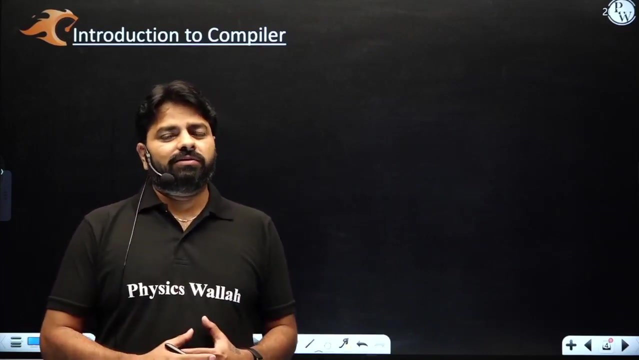 first you should learn the introduction to the compiler design. then we will move to the lexical analysis. what is the introduction? what we are going to learn in this introduction? you know the compiler is the collection of phases right, how these bases are going to work in compiler. before that, first let me help you some of the few concepts. 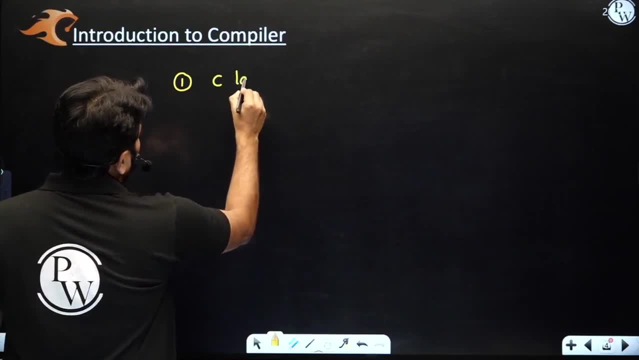 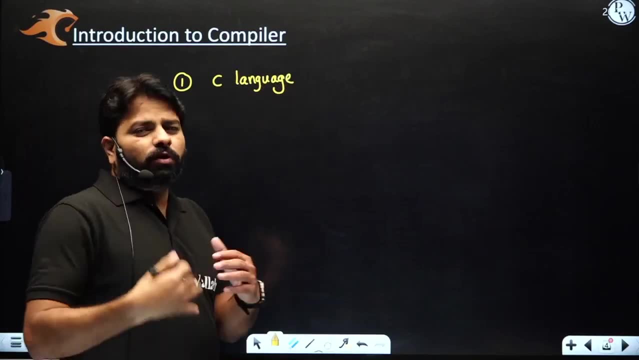 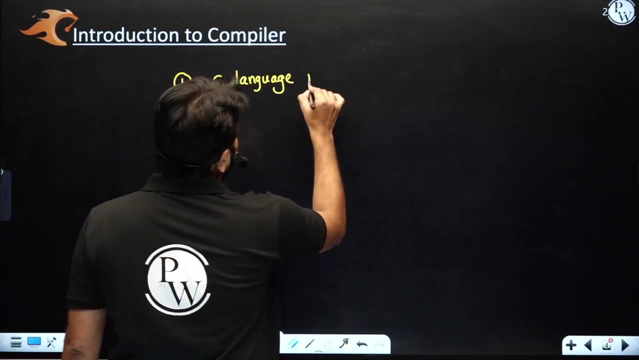 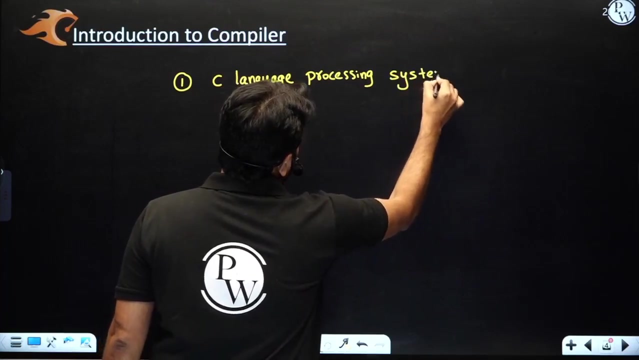 mainly, if you are going to give a c language or c program, you are going to use c language, right how this c language or c program is going to process from high level to low level. so the c language, the processing system, we will be learning first. then we will move to the main topic, which is the phases of compiler. 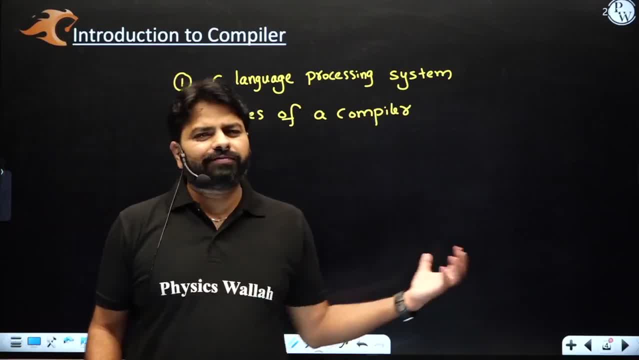 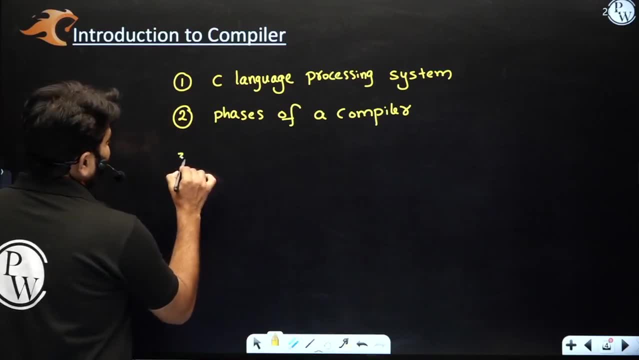 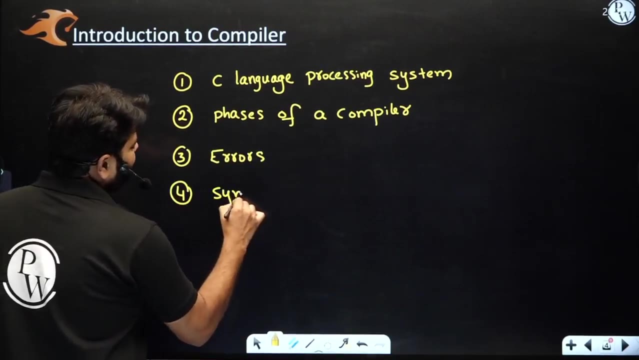 in this we will be learning, like lexical, syntax, semantic, various phases. we are going to learn in the phases of compiler. then, if you are interested, we can also look at some of the errors and also symbol table. many things are there. then we will move to lexical analysis. let's begin. 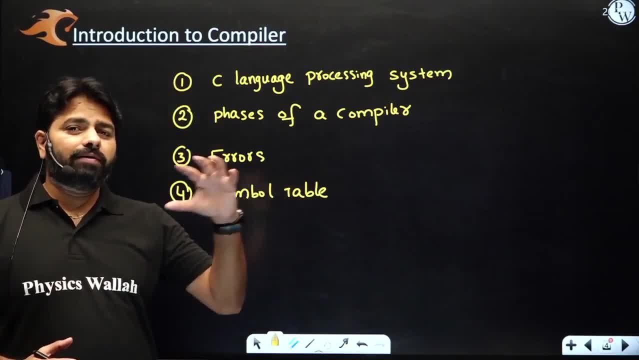 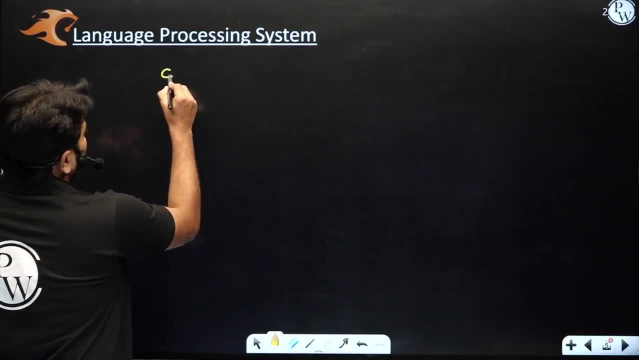 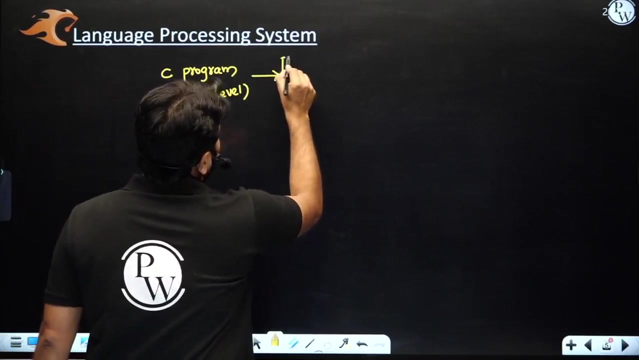 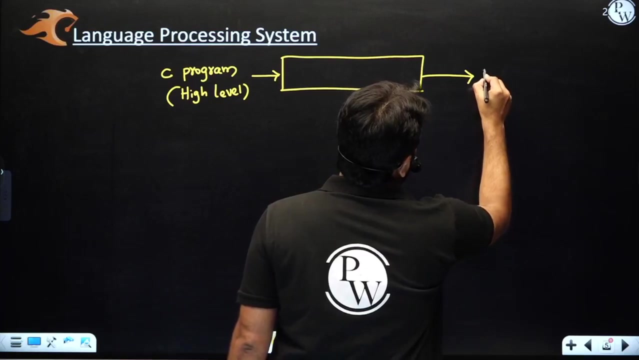 at the first how c language is converted from high level to low level. very simple. you give a c program which is high level language. this is high level, right, high level code. where do you give you give to? let's say you do something here. it will convert to the machine code, low level code, basically. 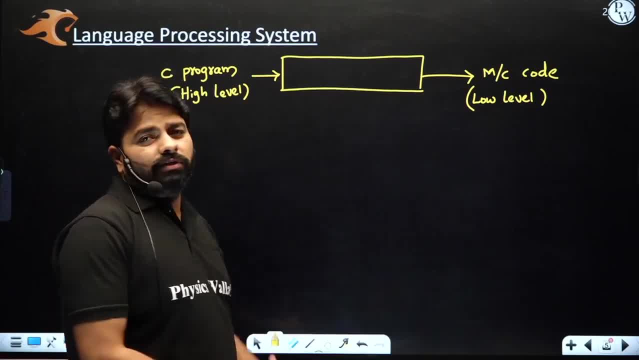 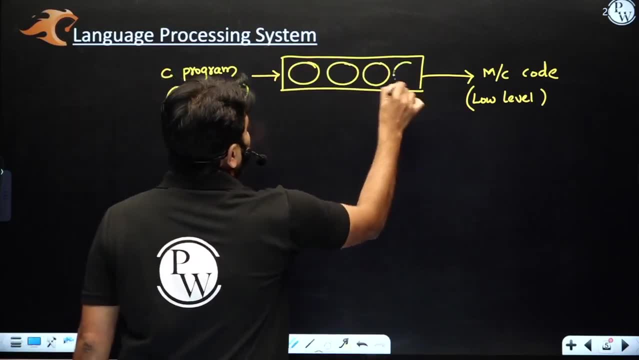 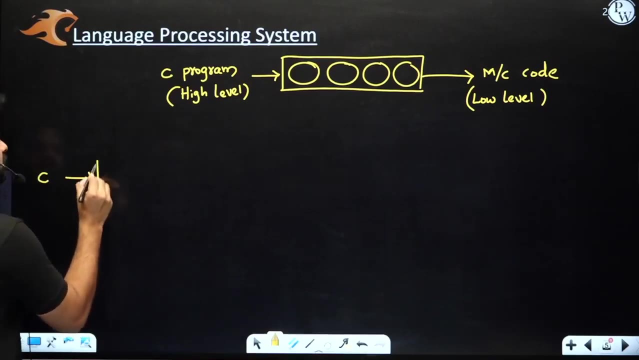 maybe you can say executable machine code that you want to convert. then how many components are involved here? the various components are going to be involved here, various components. we are going to learn some of them here. so let me help you again. you give c program the first component, which will be involving editor. 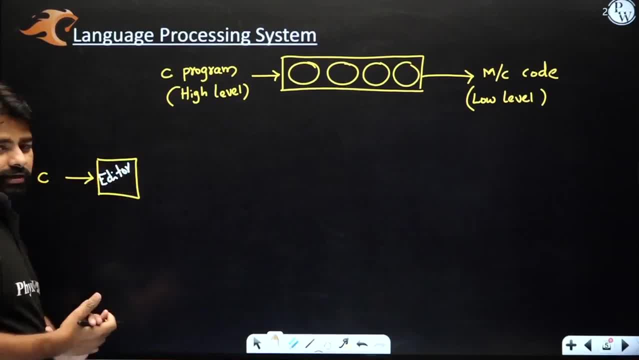 where you write a program, so c program. you are going to write on editor, right? so once you write or edit the c program you will compile. so while compiling what happens here, i'll put a boxes. you try to understand what's going to come into the picture. 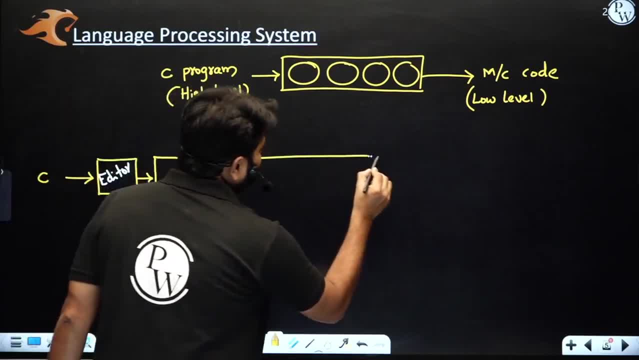 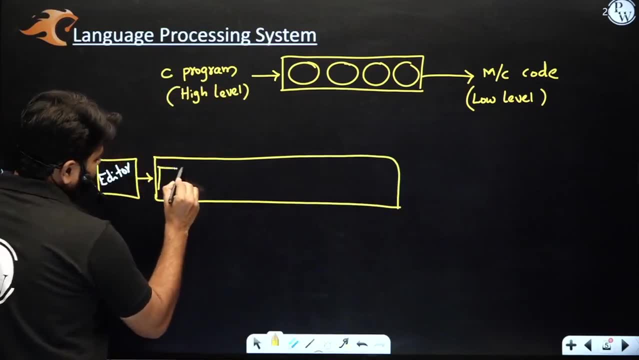 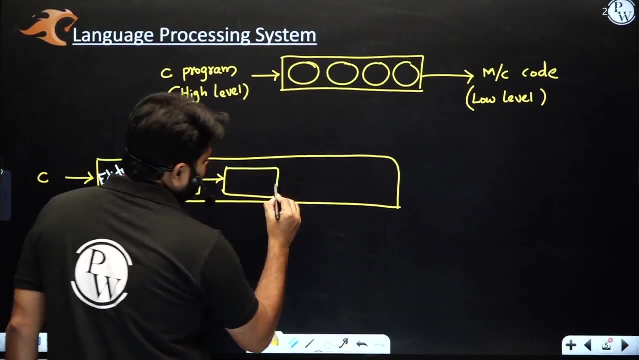 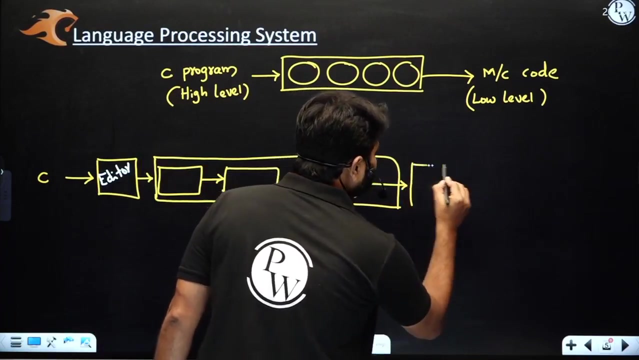 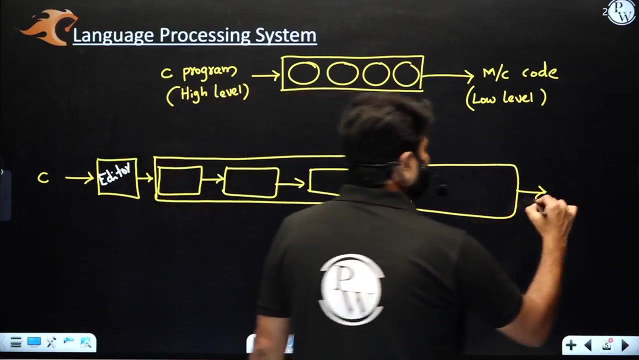 there are many things. i'll put one box- actually it may not be one box, okay- here- pre-processor, then compiler, then assembler, then the output will be produced somehow. and again here the two things might come here, and then you will see the actual executable code here, executable machine code. 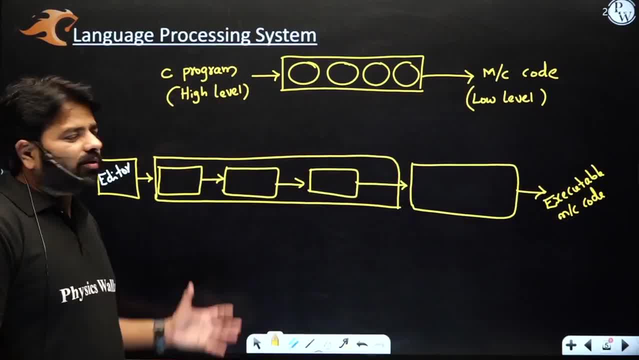 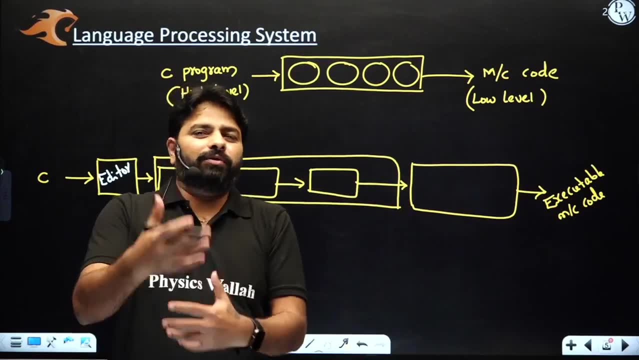 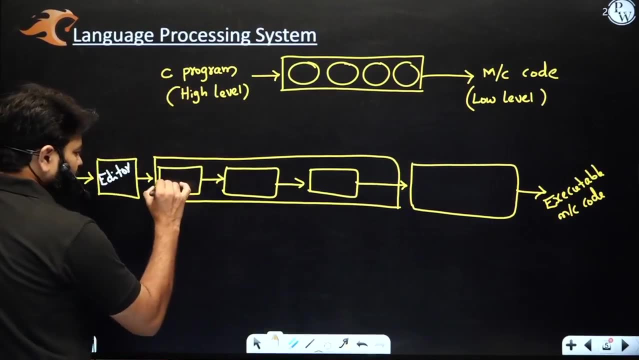 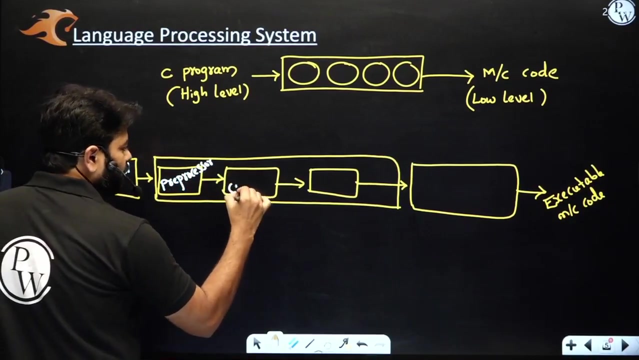 very interesting, right? so many things are happening, but we don't worry about all these things. just write a c program and do build and run, or compile and run, you will see the output, or you will give an input, you will see an output. okay, let me write some of them here. the first thing is pre-processor: right, pre-processor, then compiler. 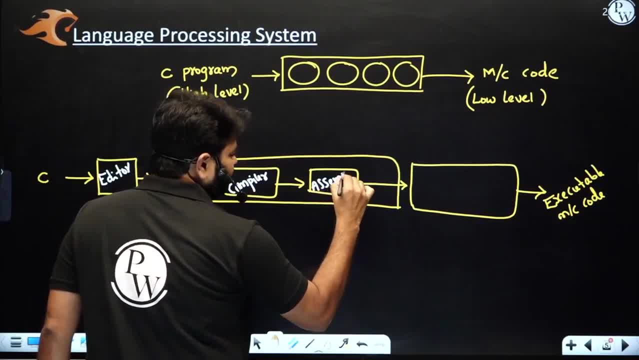 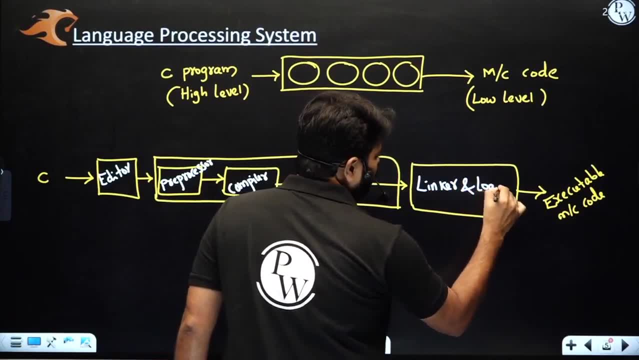 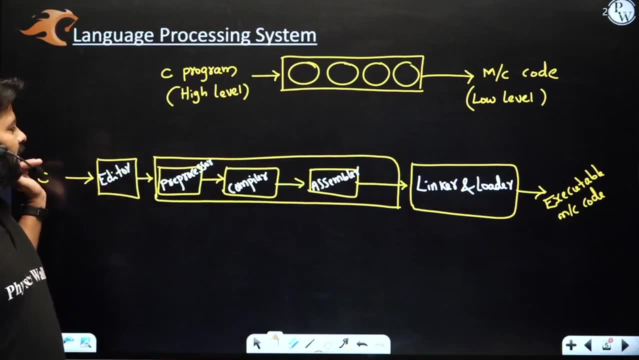 hear assembler here, linker and also loader, linking and loading purposes. now what is happening here? the you give high level c appropriate. let's say you are writing some program here. you're writing some program which might be having one declaration and you might be having some assignment. you might 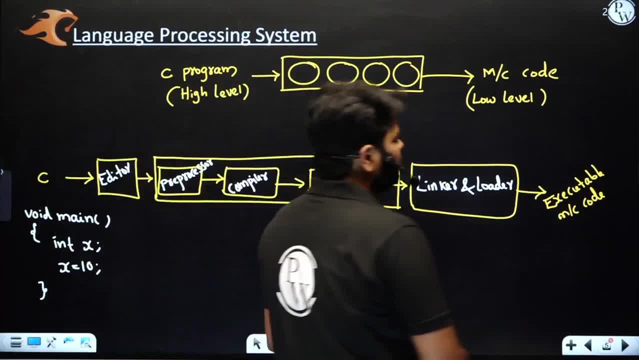 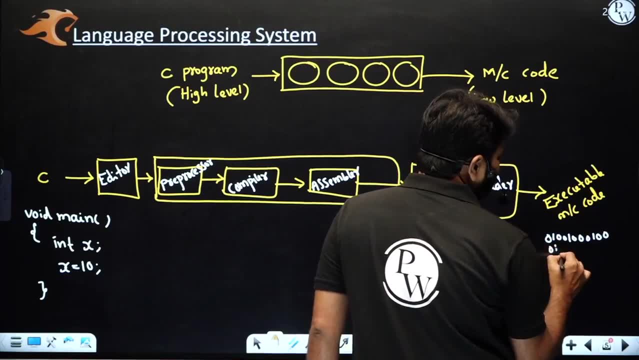 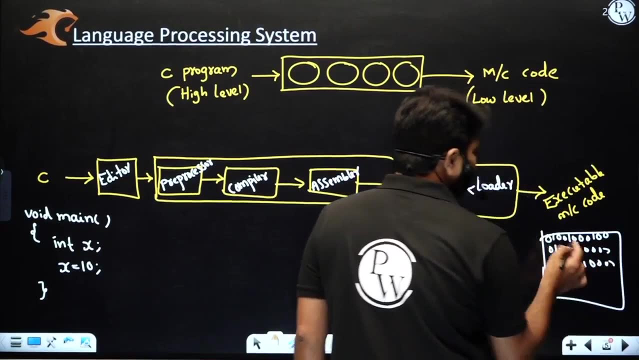 be printing or something else and somehow here executable machine code you don't see. you see just zeros and ones. don't know what actually it is here. but it is going to run something, this is going to be your file. so somehow it's converts right and during this conversion so many components are. 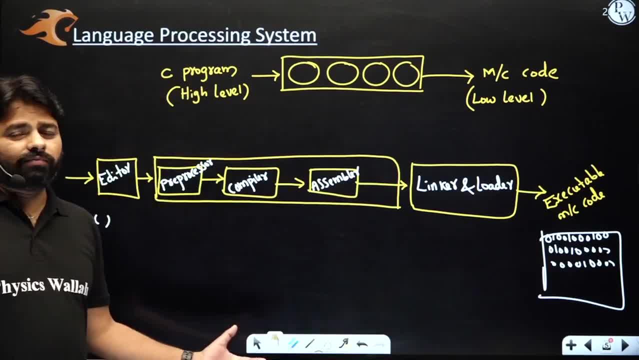 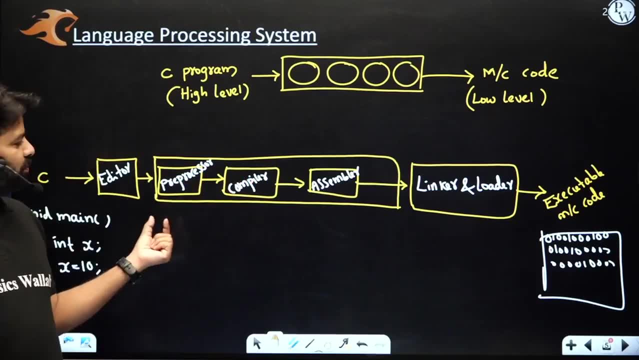 involving here how they are going to convert out into various. you can see various outputs, like you know pre-processed output and you know assembly code and then relocatable machine code, and so many things are happening here when you look at the editor, when, once you edit your code, then 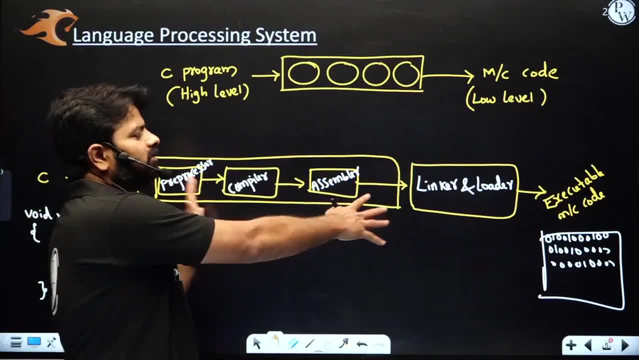 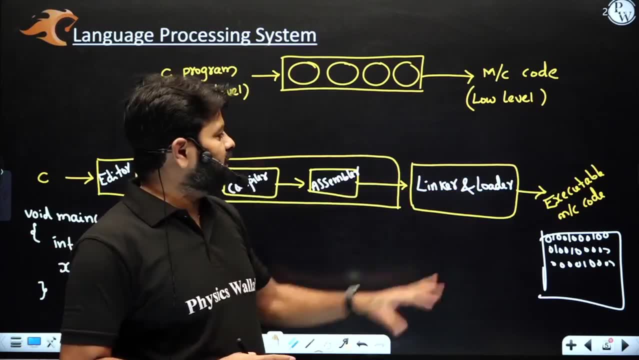 you start compiling this, this whole stage of compiling, right, this is a complete stage of compiling, and this linker and loader, it might be part of, you know, compiling and also in the part of execution. so the this thing is a static and dynamic. it's a hybrid model, right, but this stages are, you know, 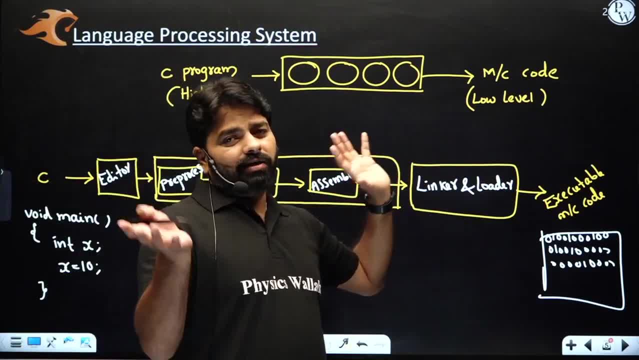 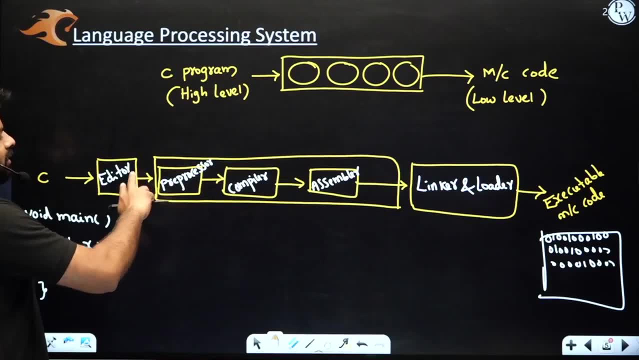 static stages. these stages are compilation stage as well as runtime stage. now there are many things, as I said. so what's this? pre processor will be learning one by one, right as we are not a hurry about you know understanding code, the conversion from C to executable code. will learn one by one and remember. 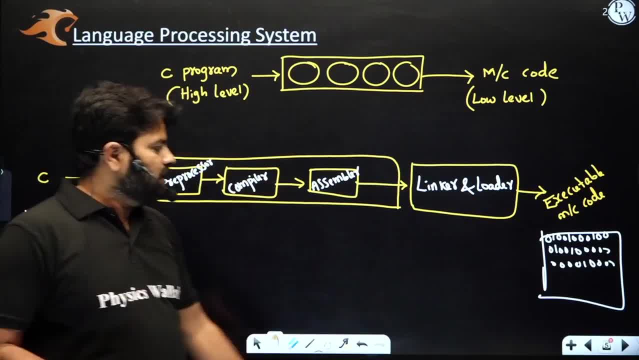 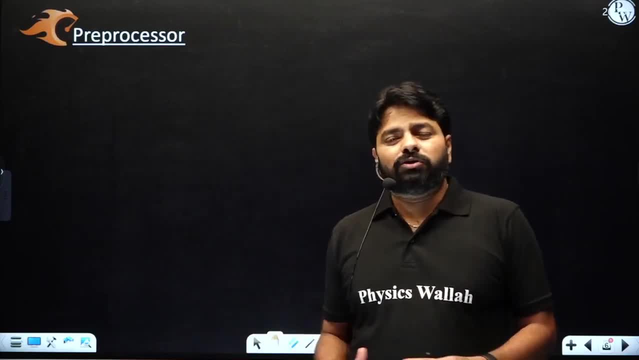 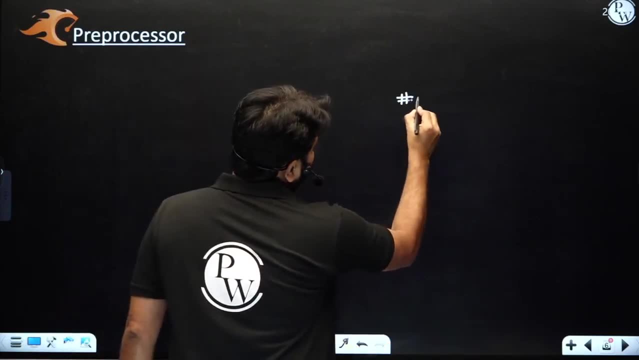 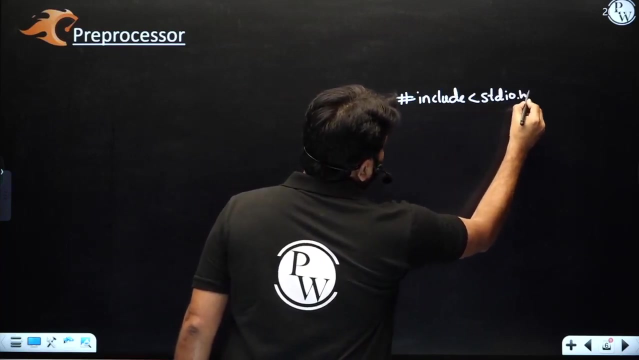 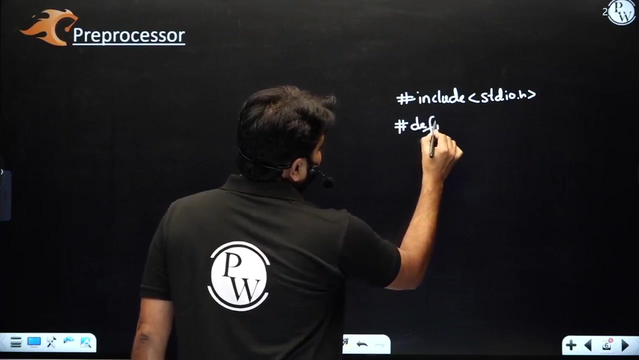 you know simple definition for each component, which is here: what is the pre processor? okay, you see there are many statements in pre processor. then what are they basically? you have come across ash include. right, this is called as pre processor statement. it's a directive statement. basically, sometimes you have seen ash define you. 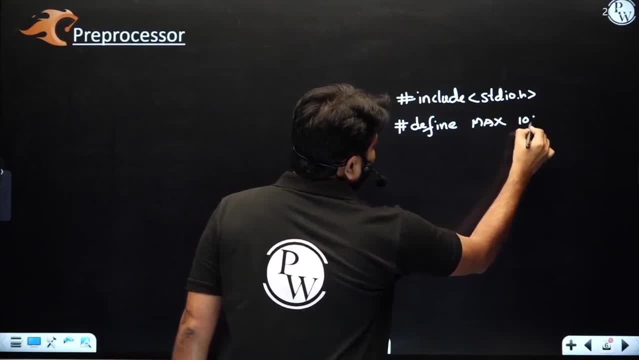 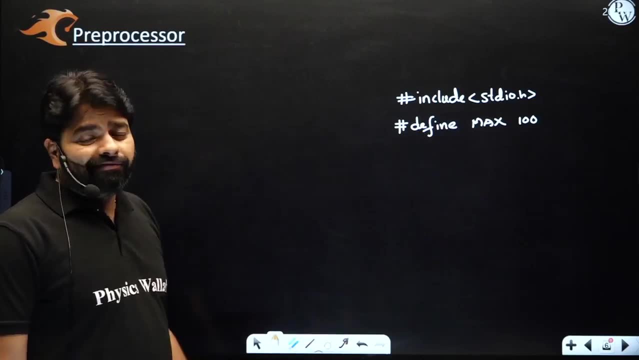 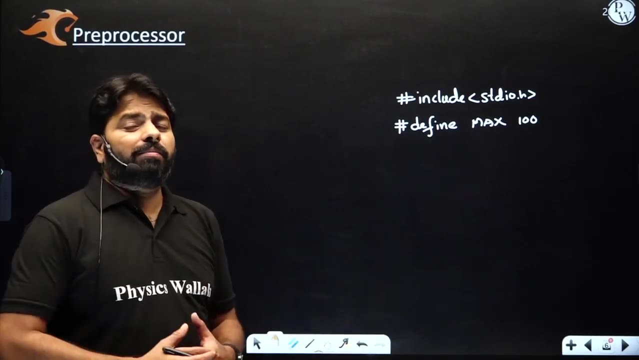 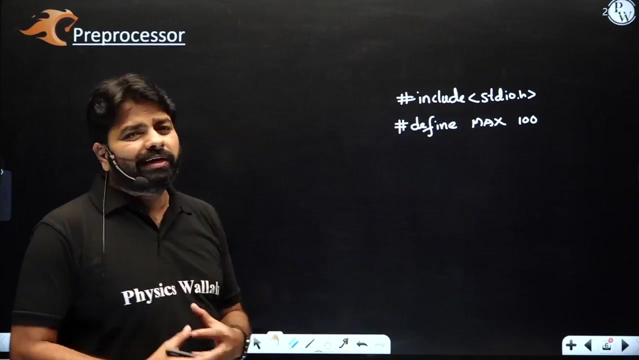 know max 100, something like that. okay, there are various pre processor statements. even you have ash if, if defined, if not defined, ash else. and if there are so many pre processor statements, are there right? I'm just taking two examples. what is the specialty of these statements? these statements begin: 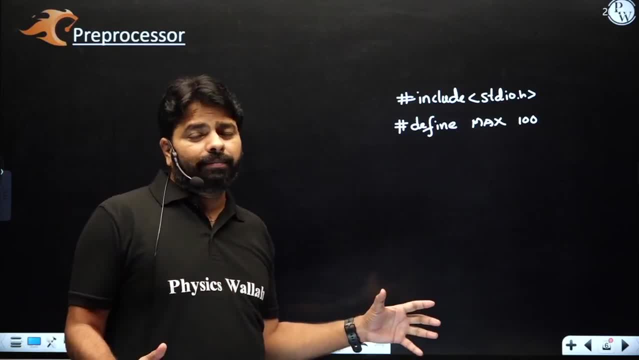 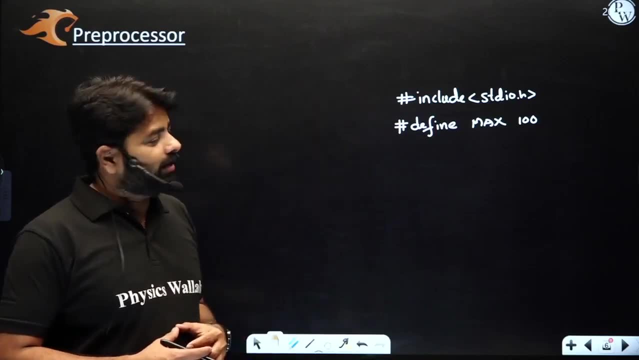 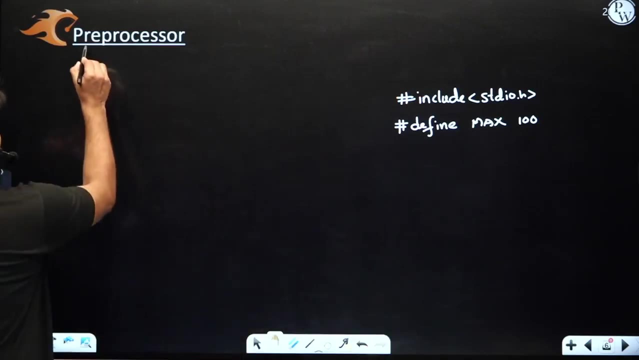 with ash and this can be written anywhere in the C program, anywhere in the C program, in but- but we do always mentioned in the beginning of the program: okay, but any statement which begins with the ash, a call as pre processor statement. here this pre processor is going to do something. it. 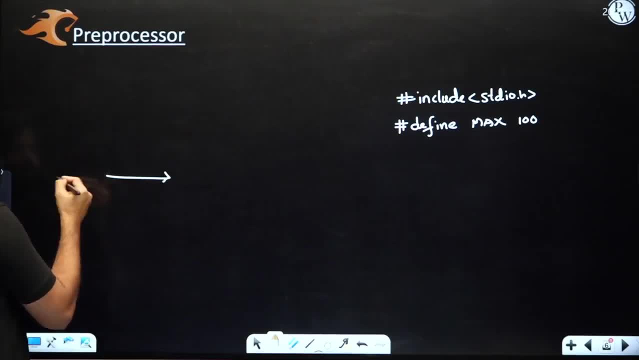 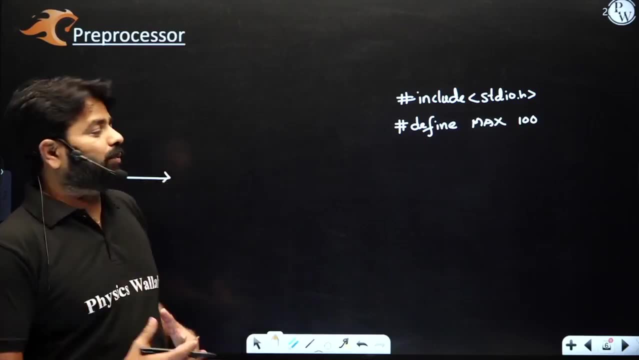 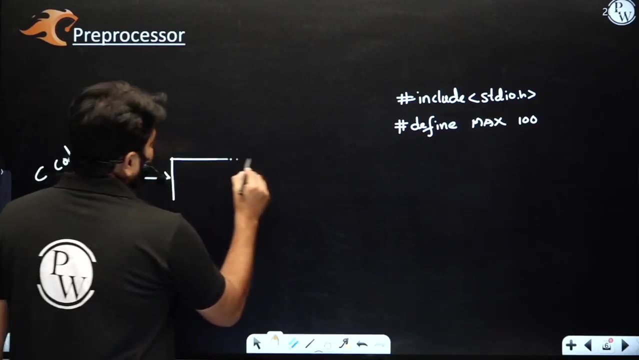 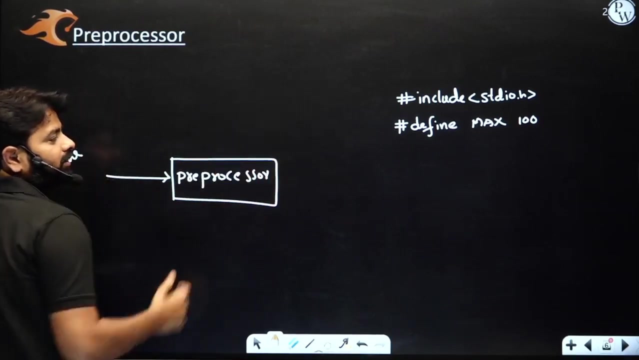 takes though C program which has the pre processor statements, then it does something to them to convert into the pure c program without the preprocessor statements. so you give c code, the preprocessor understands all the statements which are beginning with ash and it does something to them. it produces pre-processed 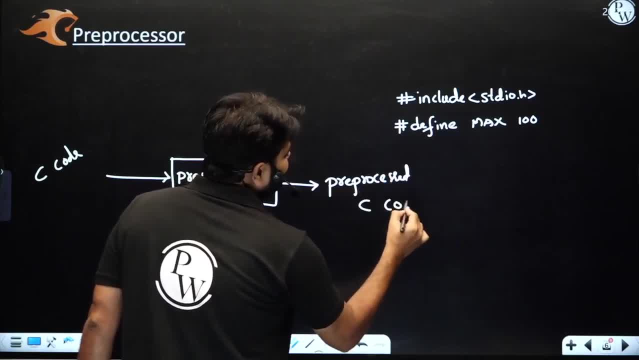 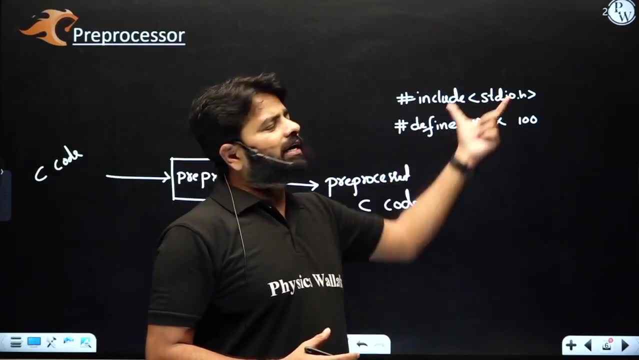 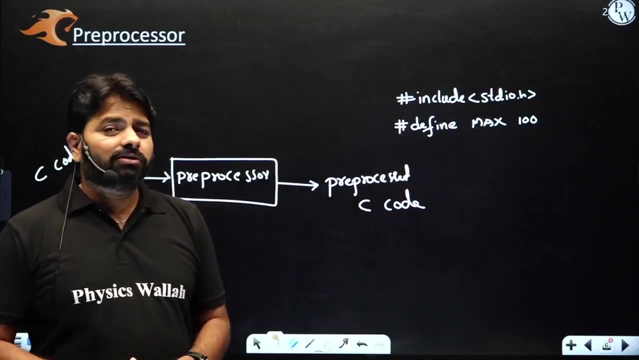 the c code. it means it's going to do something for the that pre-processor statements. okay, so this ash include sd over dot h. is another file, right? another file. it need to be linked. so it gives some information to the linker so that the linker understands. okay, there is another file, this: 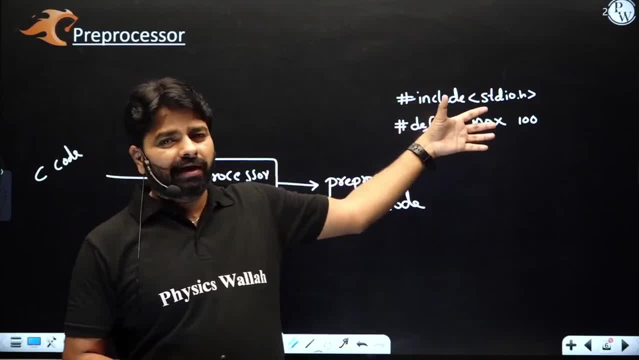 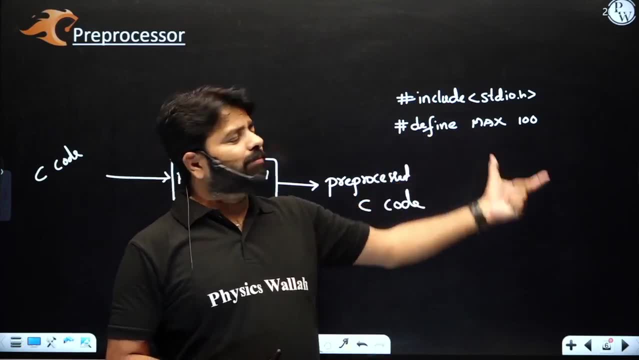 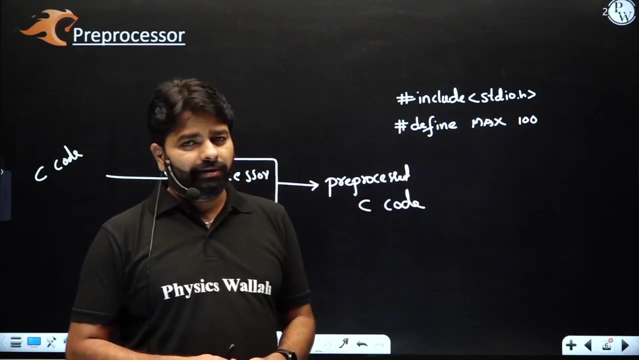 file is going to depend on so that when you use the printf and scanf it's going to look at in some library file which is already have a reference here. and this, as defined max 100 is does by pre-processor. wherever you see the max constant it's going to replace with a hundred. is it clear that max whole program it's going. 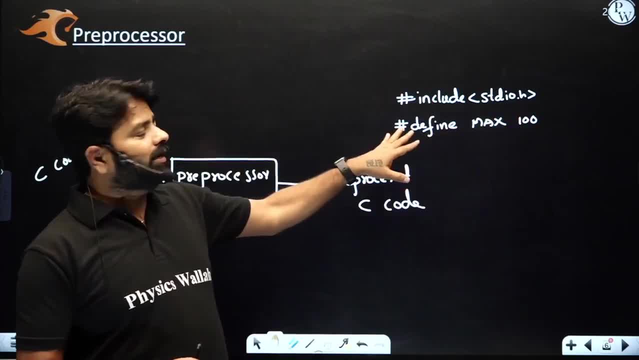 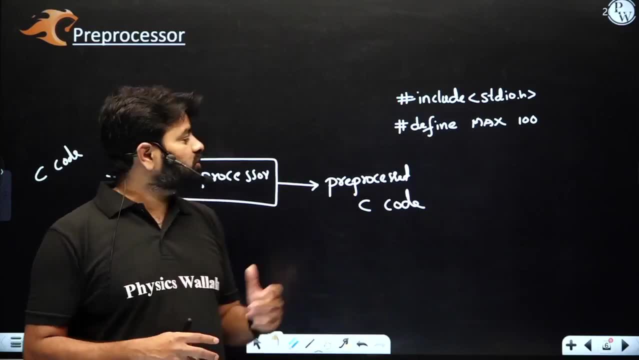 to look at and replaces with the hundred. it's very important. uh, these two statements, or any statement which begins with begins with the ash, is going to be understood by the preprocessor. it does something to that code so that when, when the compiler sees the code, there are no 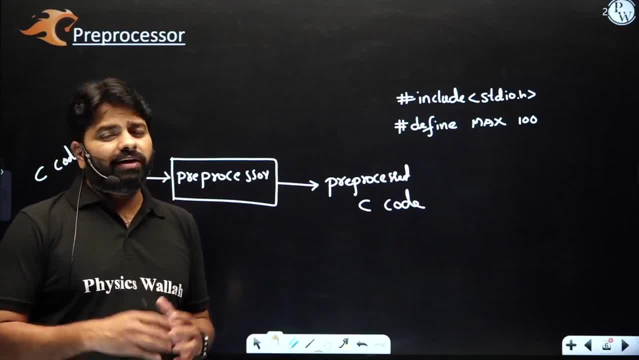 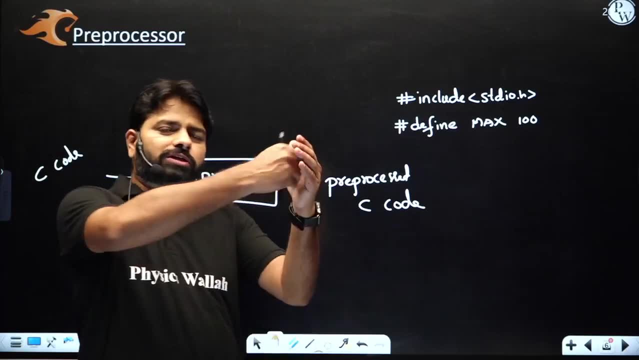 pre-processed statements so that it can analyze using the various phases of compiler. when you look at the practically, the pre-processed is also part of the compiler. so when you scan the whole program- the lexical analysis and pre-processed- both are going to come into picture. 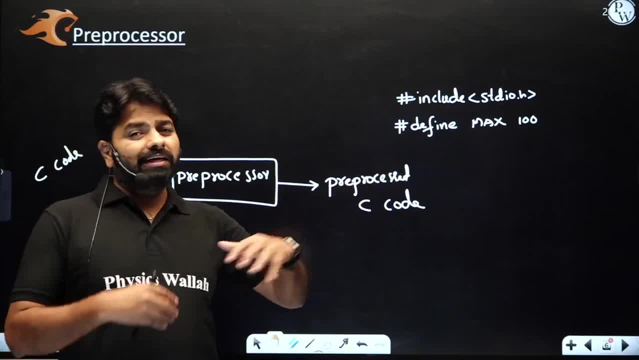 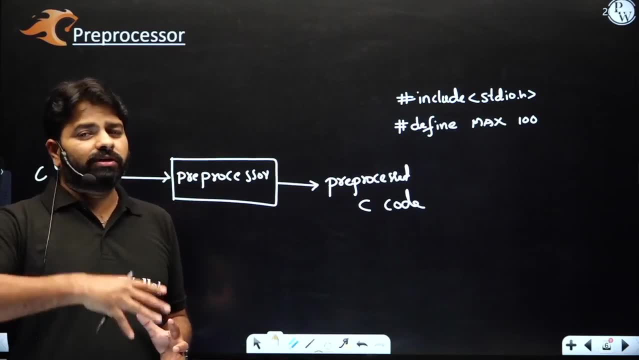 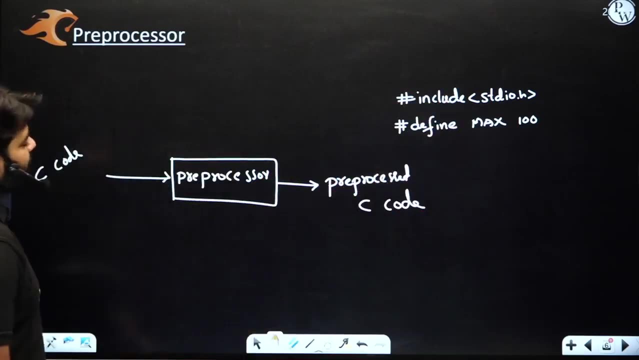 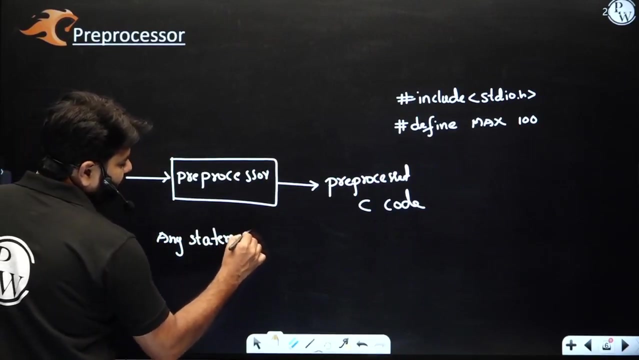 and they invoke it okay. so don't worry much about the internal implementation. but remember the pre-processed is the first stage during compilation, during compile stage, first stage during compilation, to understand all pre-processed statements. so what is the pre-processed statements? any statement which begins with the ash in c language. all the pre-processed statements begins with ash. 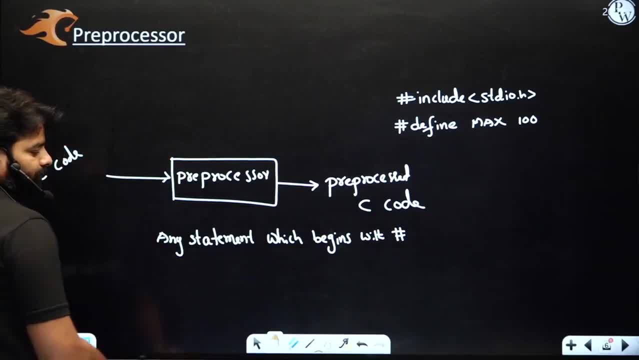 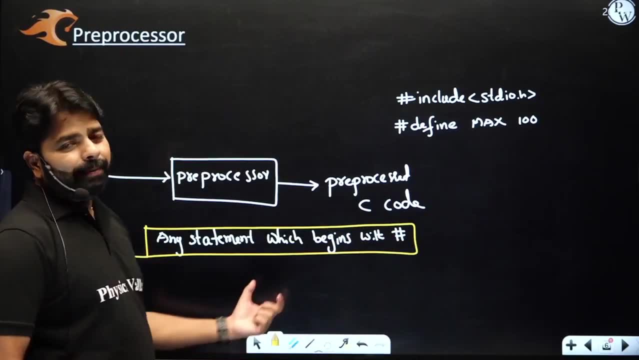 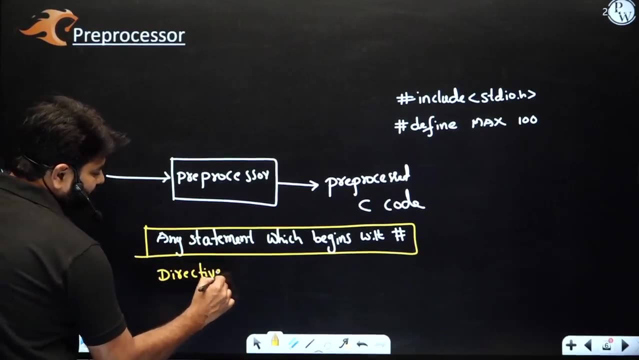 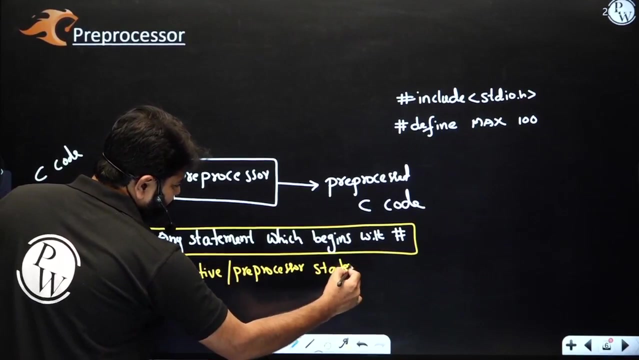 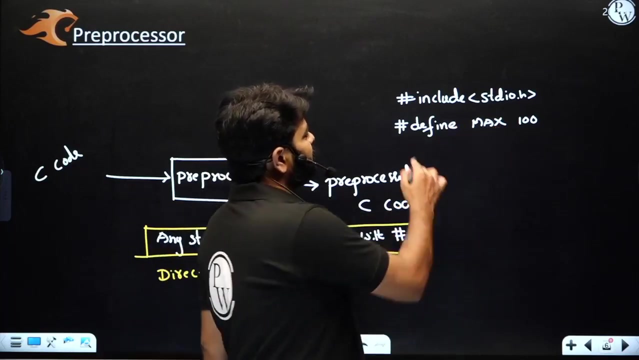 if the pre-process do not understand, it will produce an error. any statement which begins with ash is called as pre-processed statement or you can say directive statements, directive or pre-processor command or statements. this is called as a macro. this we defined a macro max, so this is called as macro definition. 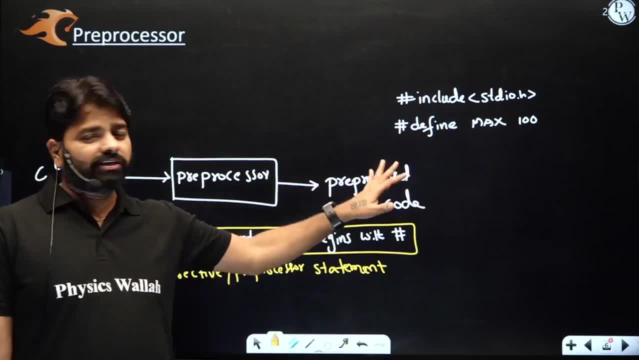 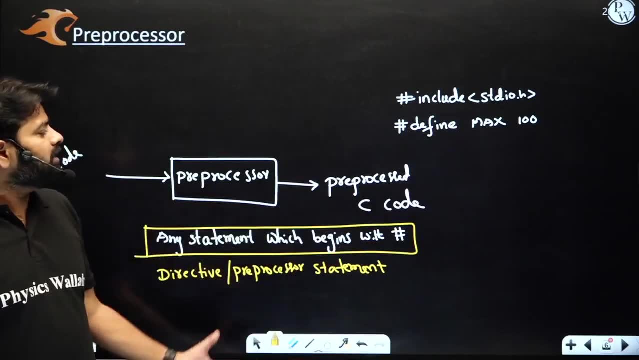 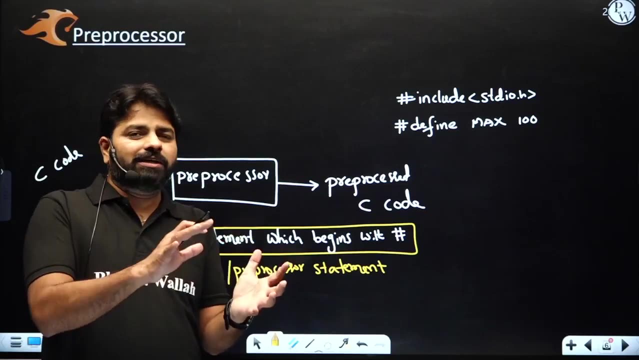 fine conditional macros also. we have, like ash, f ash in and if ash else, like you have so many many macros in conditional macros in C language. so this is about all pre processor: when you give, when you write a C program, first you understand. you means the system understands, compiler understands the pre process statements. 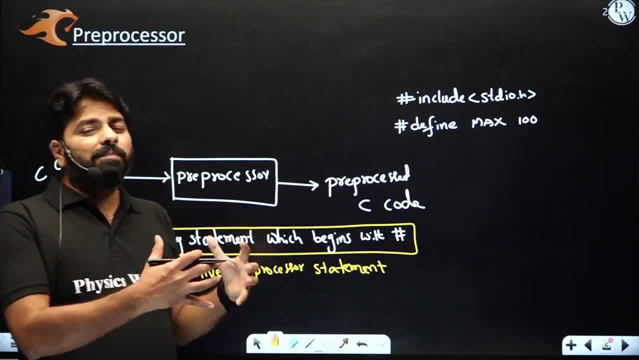 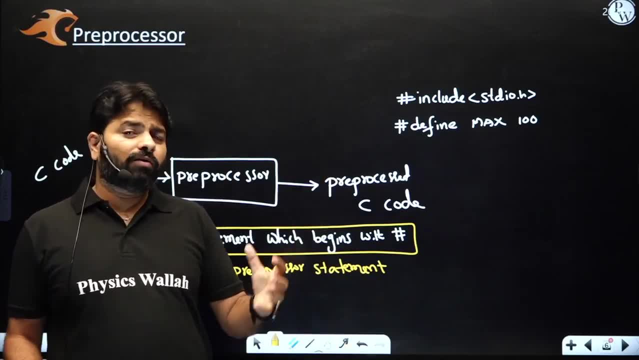 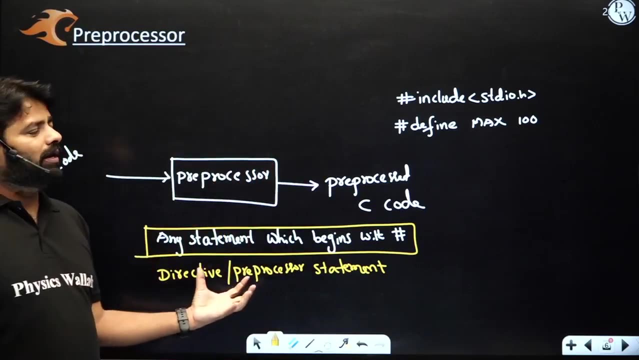 during pre processing stage. then it comes to the compiler phases. as we are talking about compiler design subject, there we don't involve much about pre processor. we involve from lexical analysis to code generation, all the phases right. but this we process. understand the definition. what is happening here? we can include the files, we can define new macros and we can have 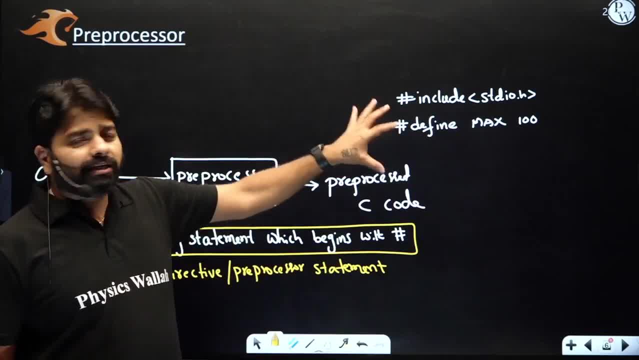 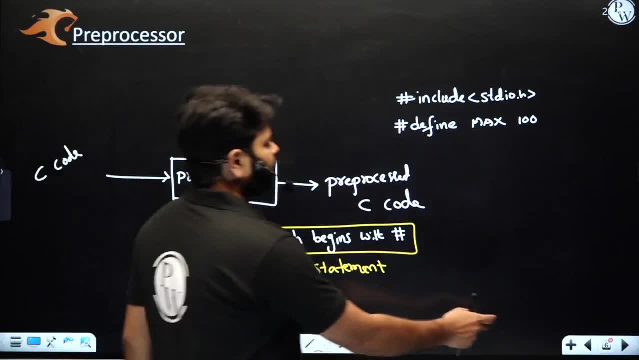 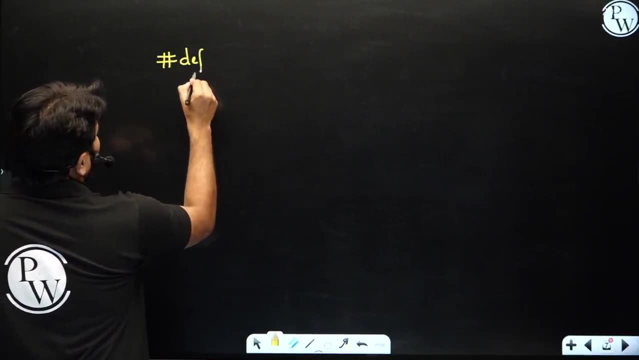 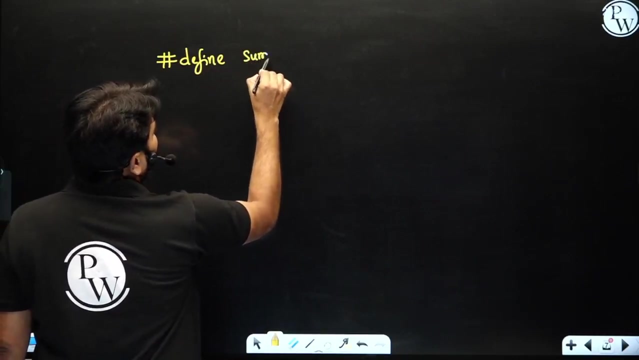 conditional macros to check the whether the macro is defined or not, that things can be done with the help of pre processor. okay, so now a very simple program for you. like I have, ash define, I'll just write sum of. of course looks like a function, but it is not a function. 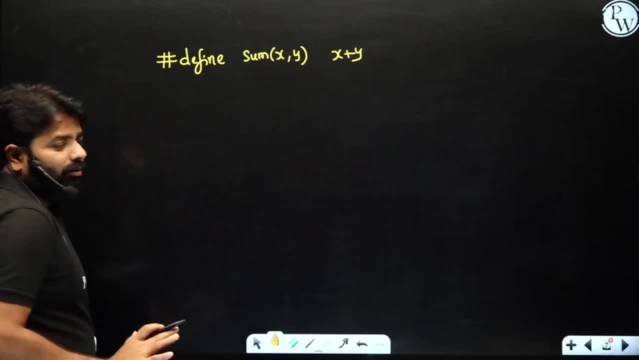 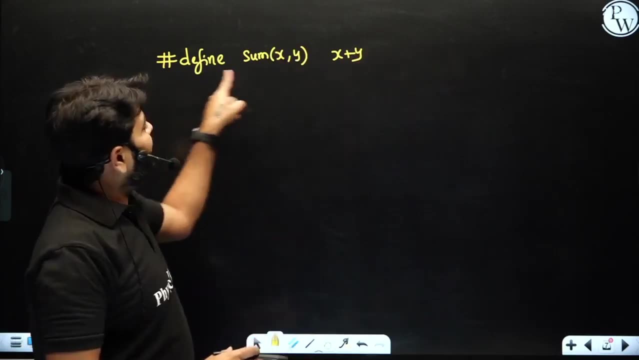 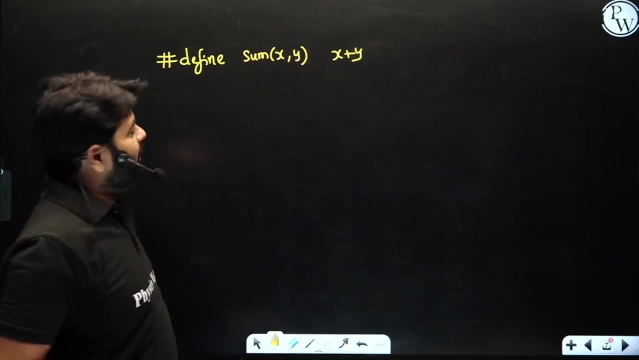 okay, X plus Y. do not write semicolon at the end of the statement. this is not a C statement, it is a pre process statement. normally C statements ends with the semicolon, but directive statements do not end with any such semicolon. so do not use semicolon at the end of this pre process statement and spaces everything. 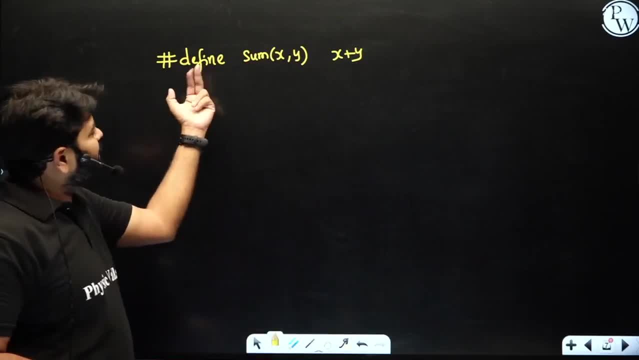 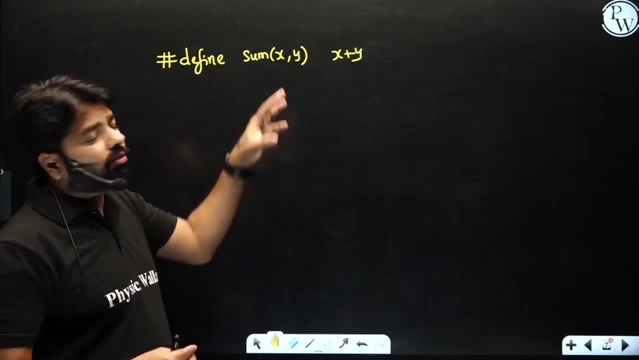 that you do here is very important. if you are going to include the spaces anywhere, it's going to produce the error, remember it will not allow to compile because preprocessor is not going to understand it. so do not include the spaces anywhere you like it. so, as per the 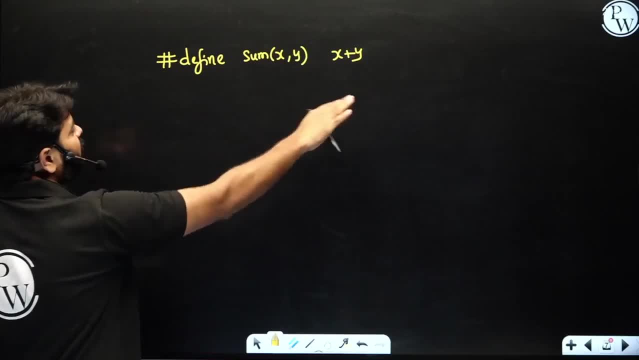 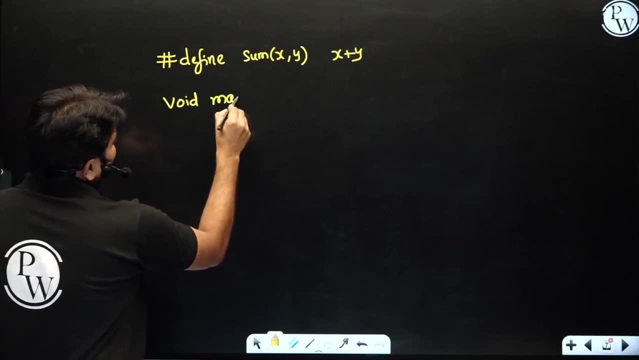 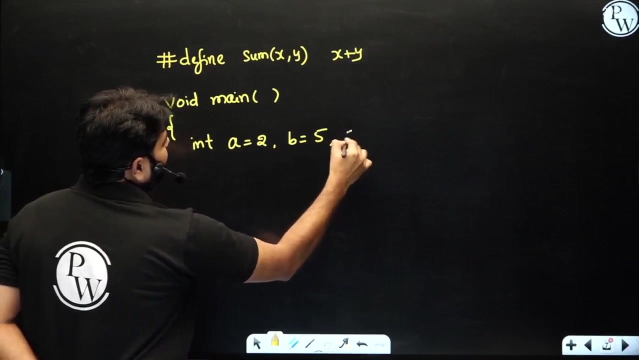 system or, as per the preprocessor syntax, just follow it. okay, now i am going to do something here. let's write, let's think about this statement. i'm going to do here some expression: a is equal to b is equal to 5 and c is equal 0. okay, don't worry much about it. c is equal. 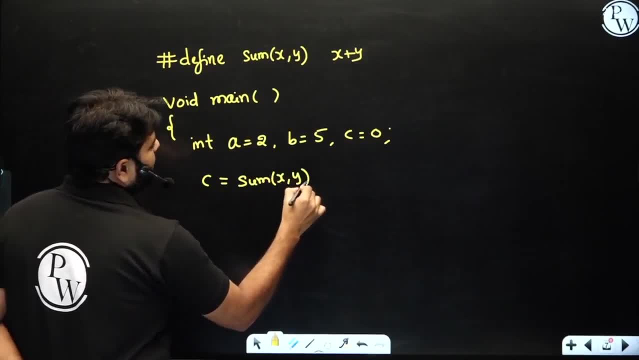 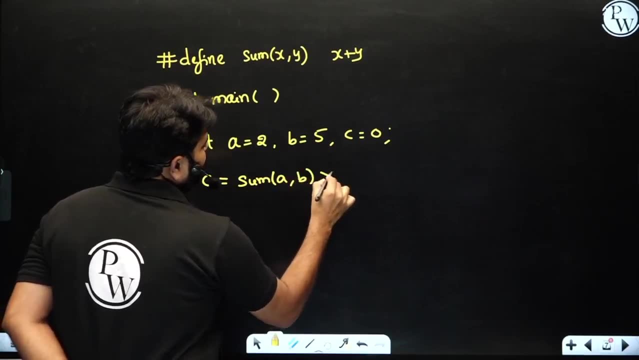 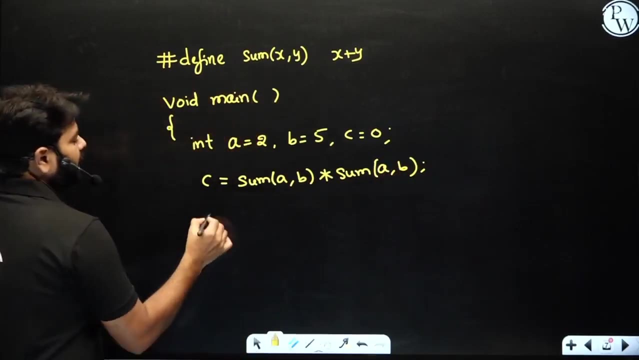 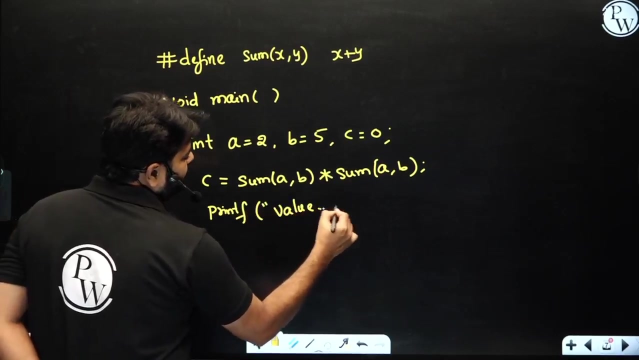 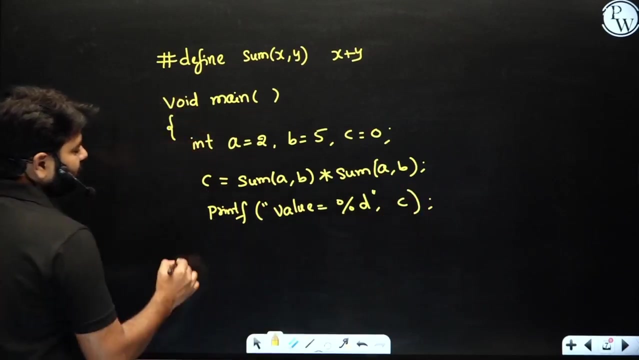 sum of x comma y multiply with- oh sorry, x is not there right here here- a comma b, a comma b multiply with sum of a comma b. okay, and then i may print the value of the result. the result is, let's say, decimal integer, decimal value present in c. okay, now try to understand the output of this program. 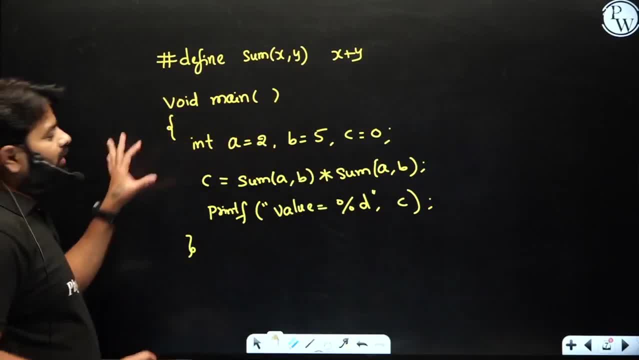 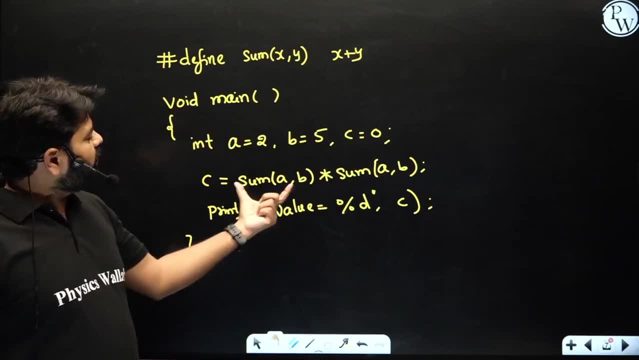 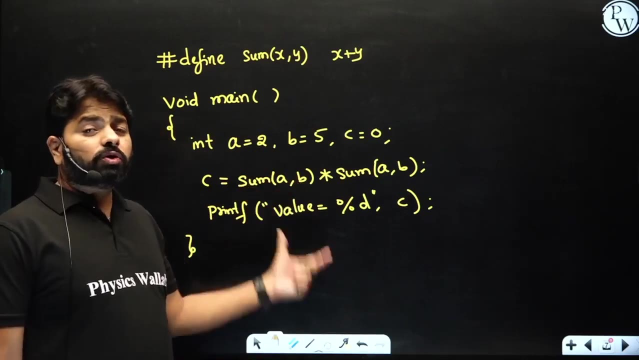 okay, this is the input that you have given. nothing already. the data is available within the program, so there is no input. input is already taken within the program. now, uh, what is sum of a comma b? a is 2, b is 5. will it be returning? uh, 7 or 2 plus 5? 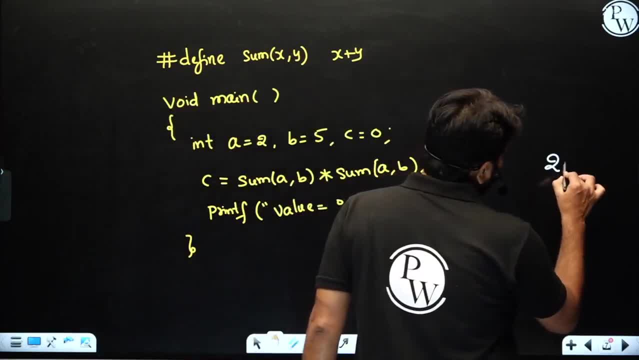 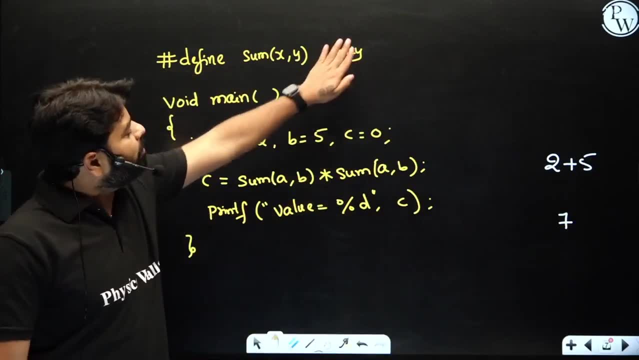 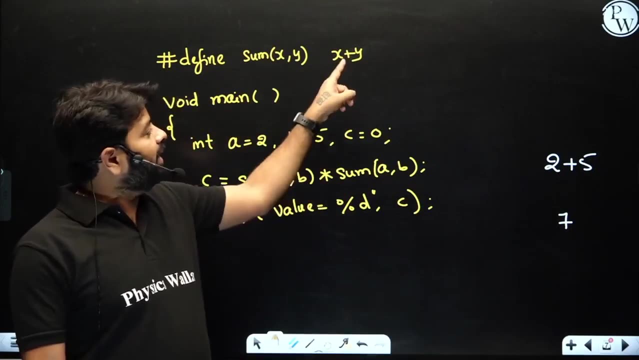 both are different. remember: replacing with 2 plus 5 is different from 7.. what is the difference? if i am replacing 2 plus 5, that means i am doing copy paste simply without evaluating. but if i am replacing with the seven, that means i am taking two plus five and evaluating. 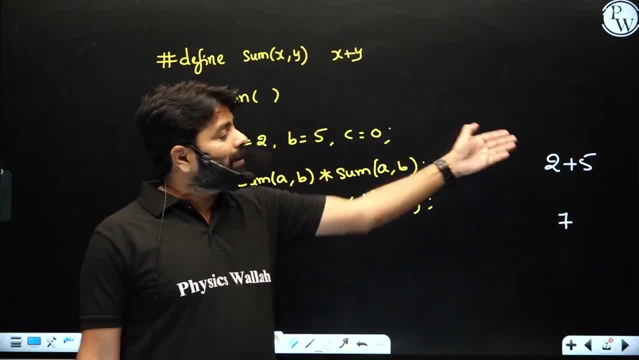 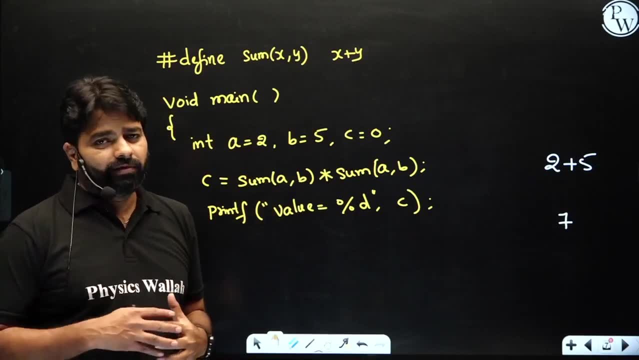 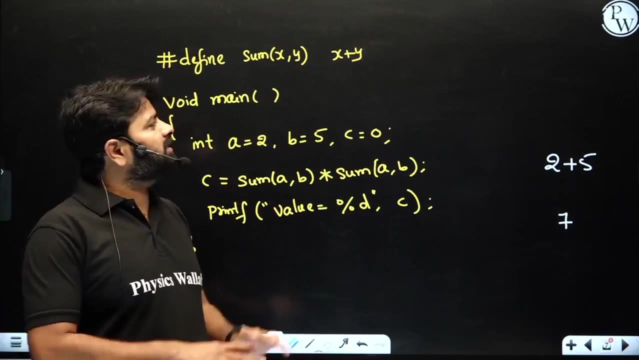 then seven. i am putting here. so what should i put? two plus five or seven? so what preprocessor does? it does not evaluate any expression that you have here. this is an expression. it's not going to be evaluated. that is just text. it assumes it's some text. it's going to replace it simply. so x plus y. 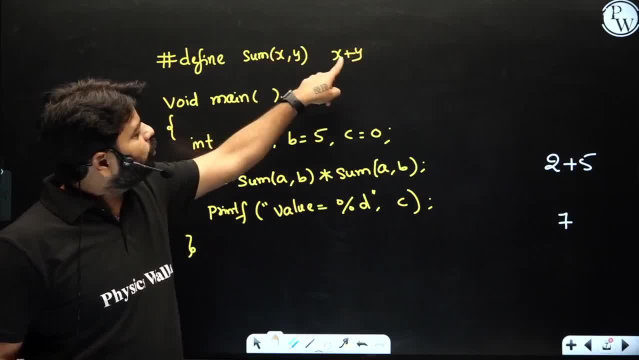 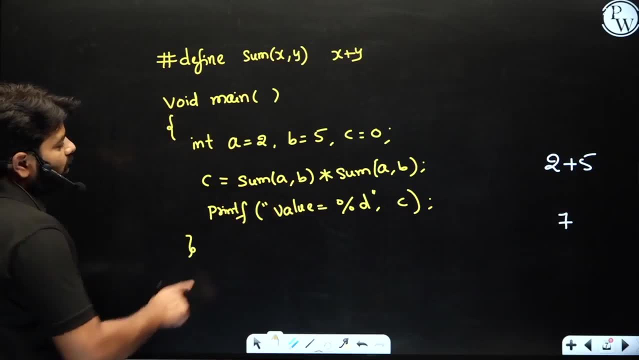 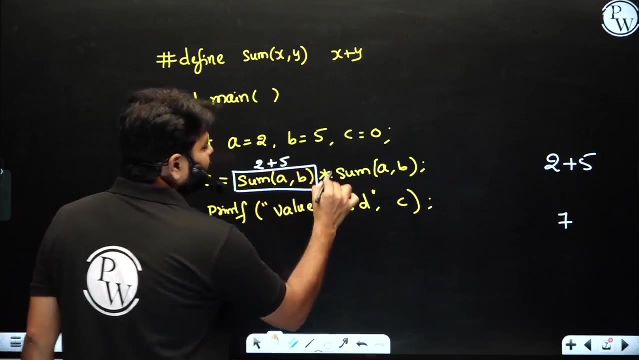 that is, you pass two comma y, two comma five. two plus five is going to be replaced in sum of x comma y, that is a comma b. now here, what happens here, especially what happens? it's going to be replaced with two plus five. that's it, and this will be replaced with two plus five. so this: 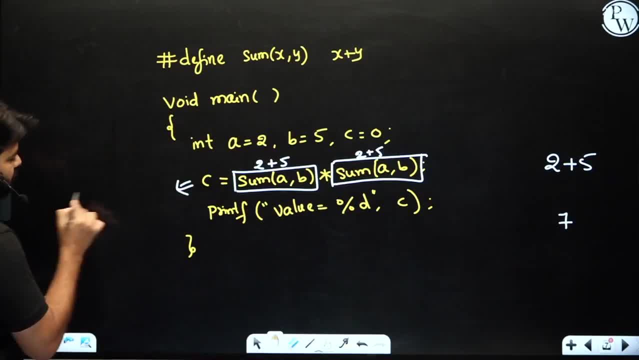 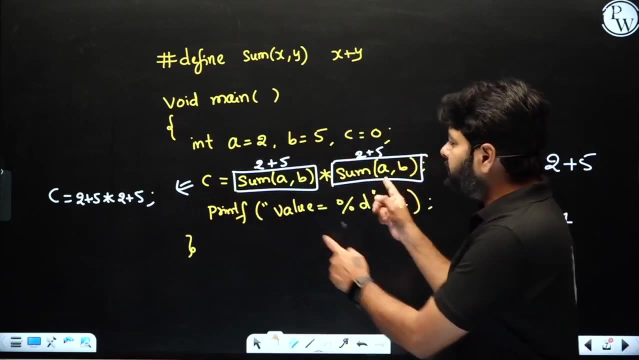 expression, especially this one. what happens here is: c is equal to two plus five. multiply with two plus five 5. this is an expression seen by compiler. the compiler is compiler is going to see this statement, but preprocessor is going to see this statement. it's going to replace with 2 plus 5. 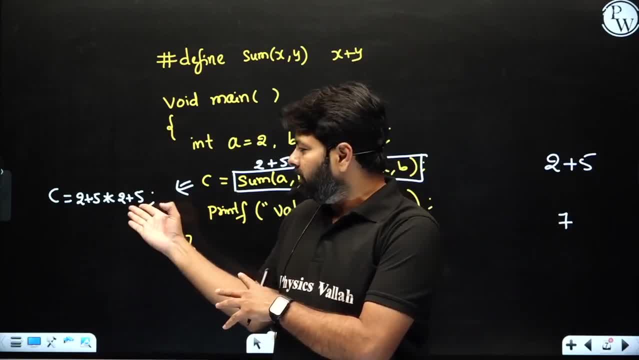 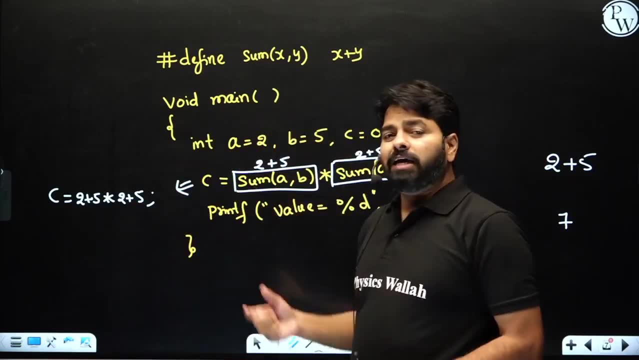 so when it comes to compiler, the compiler knows that only 2 plus 5 multiply with 2 plus 5. now compiler can decide what to do. right, if the preprocessor doesn't come here. the sum is actually not a function. the sum is the macro. here you can see that. so it looks like a function. arguments: 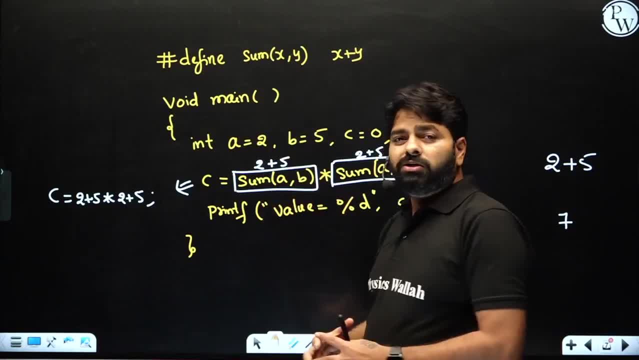 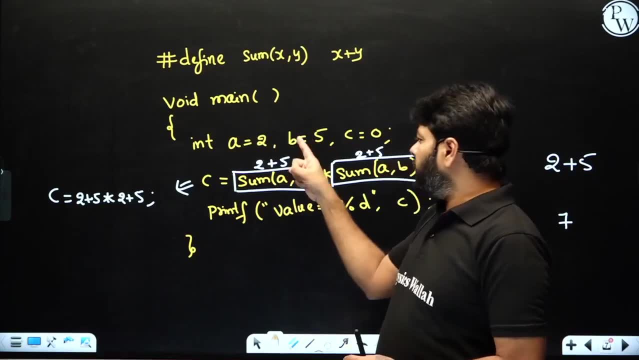 but it's not a function at all. so the preprocessor is going to come here and replace the sum of the 2 comma 5 with a comma b, with 2 plus 5. a and a is to b is 5 already. so it's going to take care. 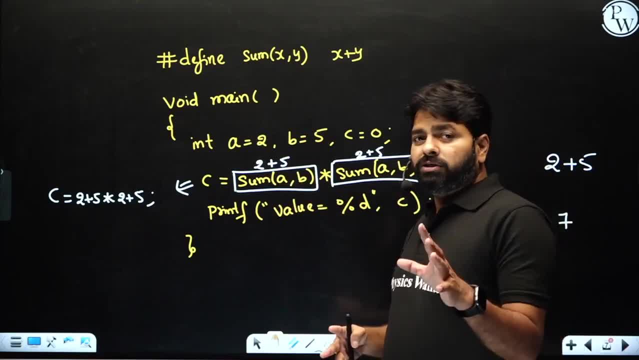 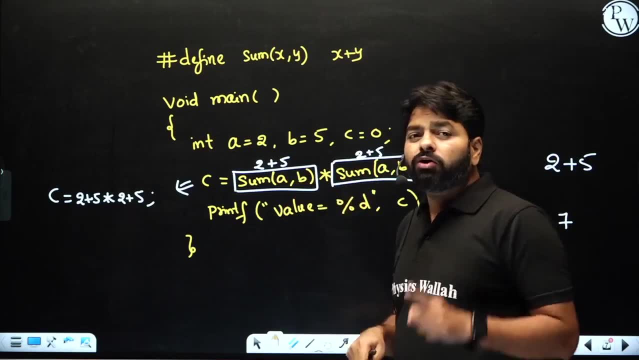 of that, fine, so this is the job of a preprocessor. this is a job of preprocessor, so what it's going to do, sum of a comma b- will it replace a plus b or 2 plus 5? that is also important when you look at here. i'm just going forward and i'm explaining the values. 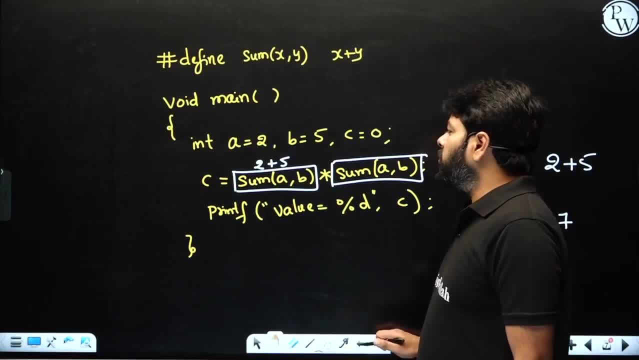 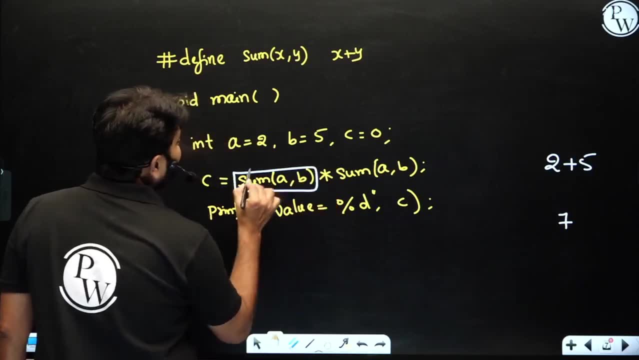 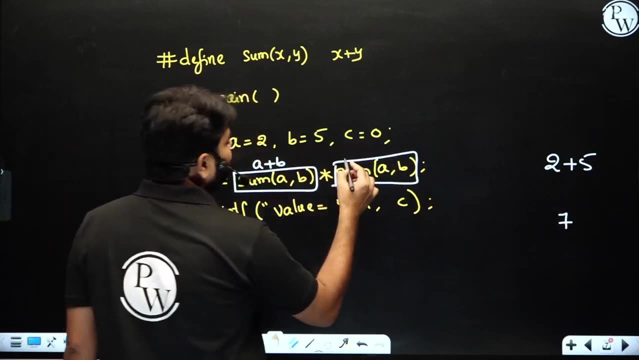 but in between, if the values changes, it will also change. so instead of these two plus five, the sum of a comma b, it's going to replace with a plus b. that's it. if you pass 2 comma 5, then only it takes 2 plus 5. 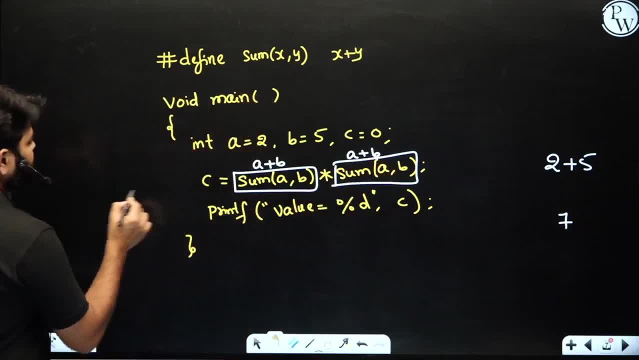 otherwise simply a plus b. so this actual replacement of the preprocessor c is called a plus b. multiply with a plus b, then when it replaces with the 2 Allen coefficient. so now, when, when the clock changes, it is not an, a con辛苦, but the 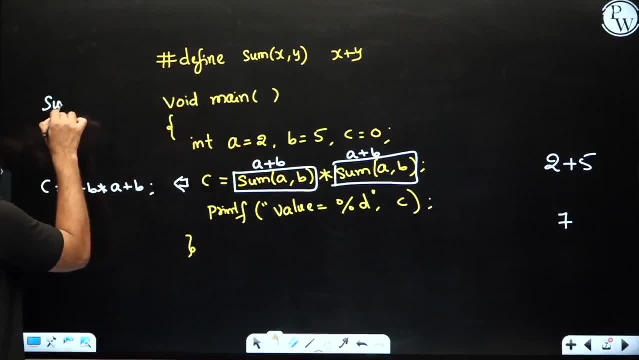 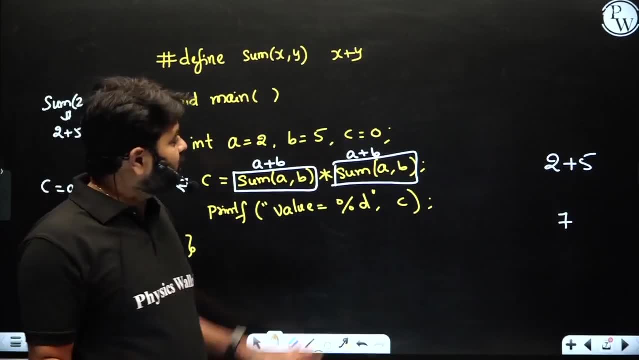 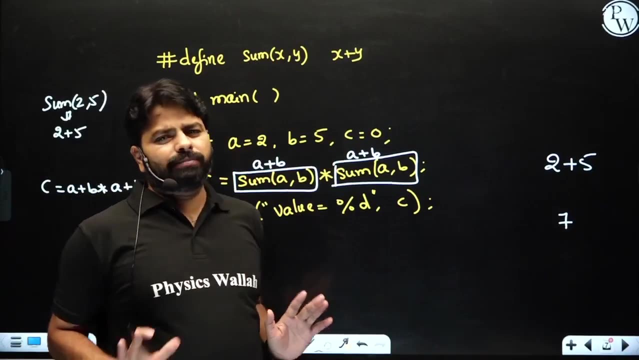 plus five. if you call, if you write a macro sum of two comma five, then it will replace with two plus five. here i'm not doing it. any evolution. i pre-processor will not understand what is the value of a? what is the value of p? it just does you have given a comma b, does a plus b, you have. 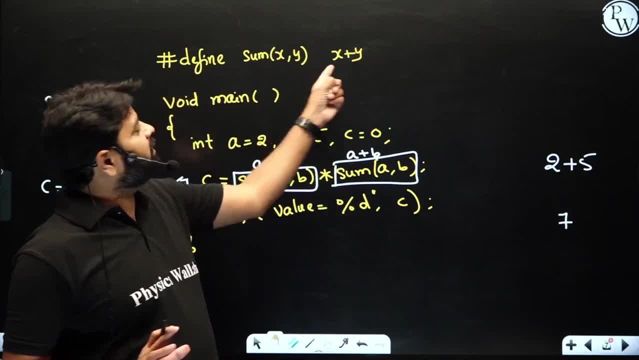 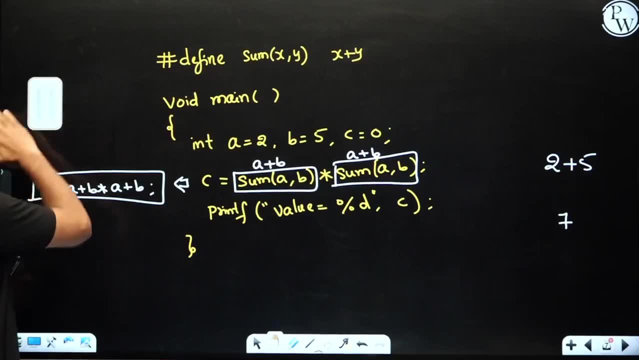 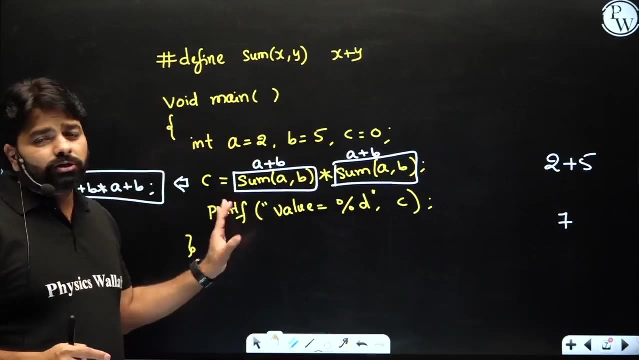 given hundred comma, thousand, hundred plus thousand. that's it, the job of this macro. okay, so that that is all you know the what pre-processor does here. it's not going to understand more in detail like a compiler. compiler does something to understand, like syntax check, semantic check, but pre-processor 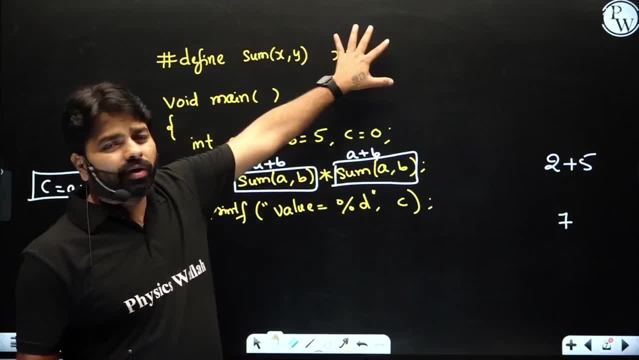 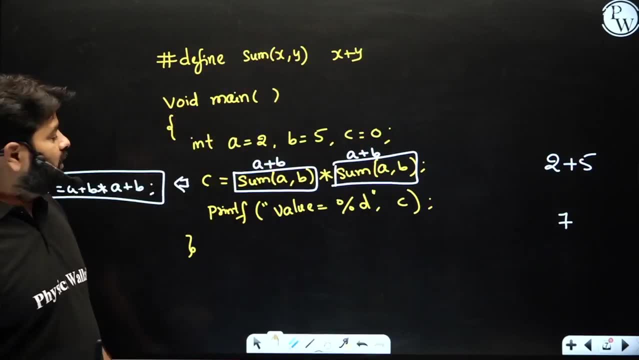 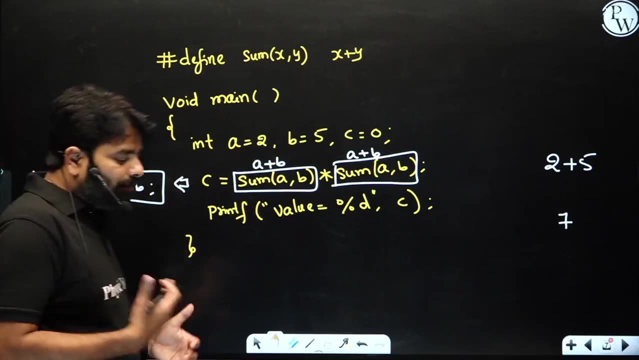 don't do that, because just replaces what is here and what is going to be replaced. so this is called as a constant and this is called as expression. okay, it's a macro definition. now you tell me what's going to be the result: a is two, b is five. the compiler: uh, once you compile, then at run time, 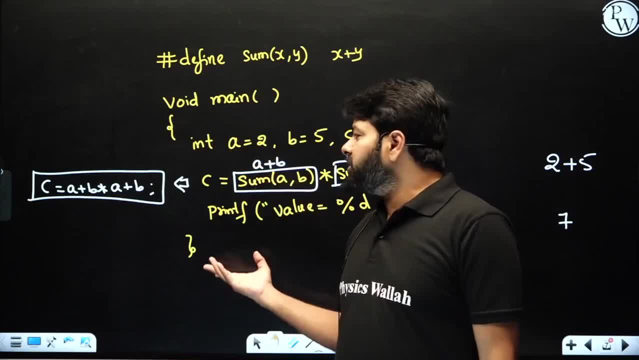 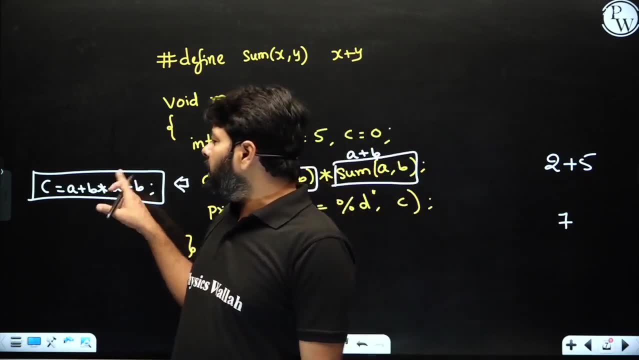 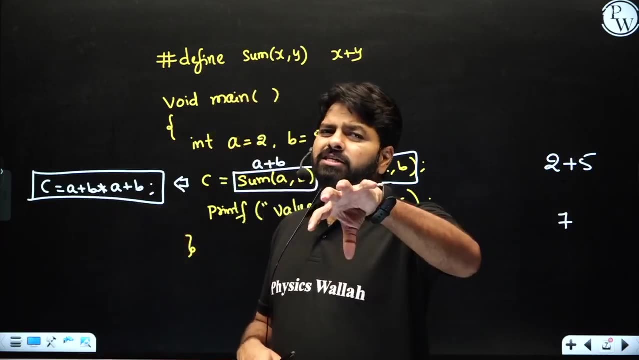 the a value is two, b value is five. the system understands how to um, um evaluate, because compiler already disclosed how to understand. so, compiler, what he does is: there are arguments, there are, you know, precedence rules. using those precedence rules, there is addition, there is a multiplication. so it takes a priority for multiplication, so it does first. 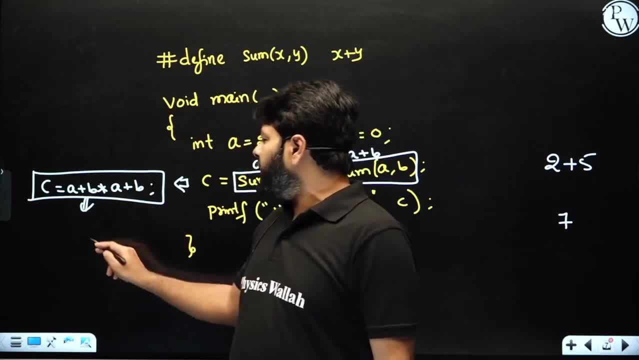 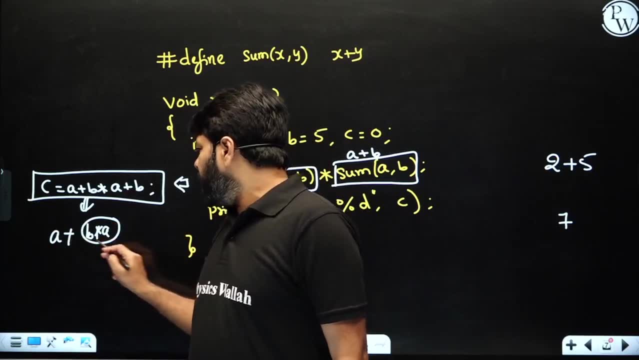 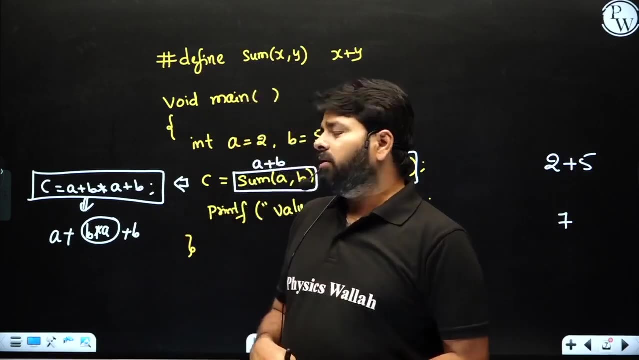 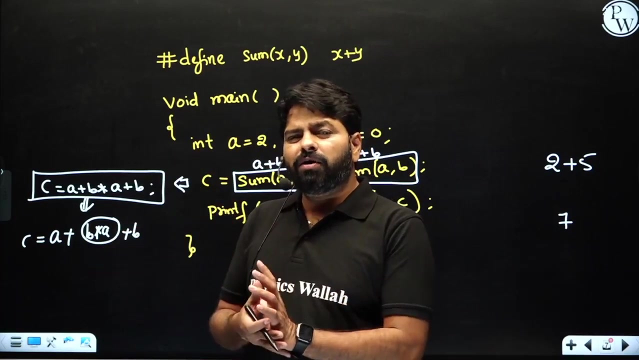 multiplication. the. what compiler does is first b, multiply with a, does once it does, then you have a plus a, result plus b, and now there are two additions. after doing multiplication, there are two additions and also there is assignment. assignment will be done at the end anyhow. so now two additions are there? how these additions performed? which? 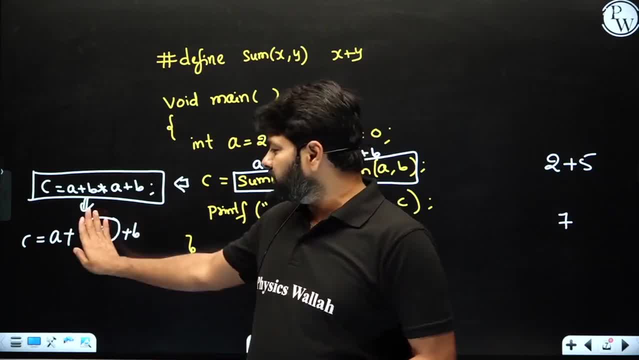 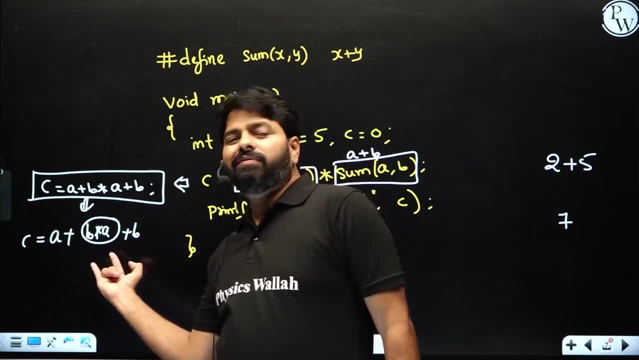 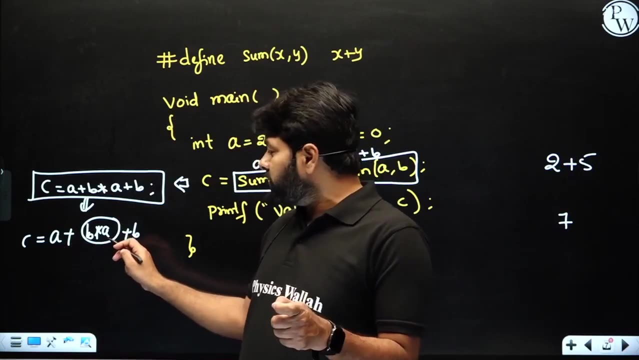 addition should be done first c plus some result, or that result plus b. what is going to be done? the in c language, the two plus are actually having equal precedence. so it follows left right. it follows left right. so now the who is having, uh, the who is the left plus. that's going to be evaluated first. 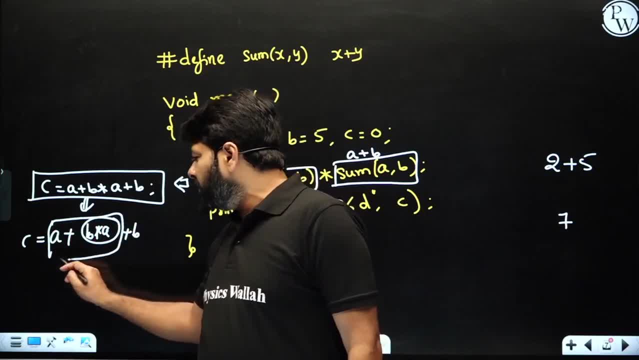 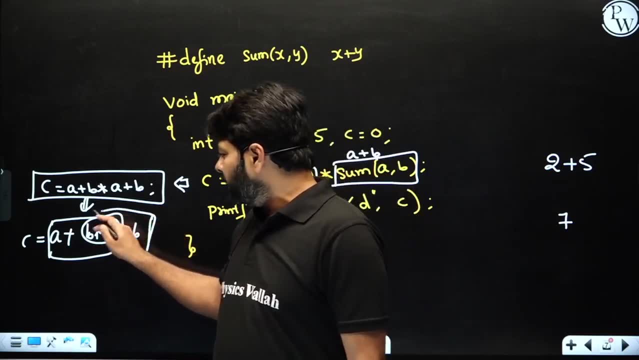 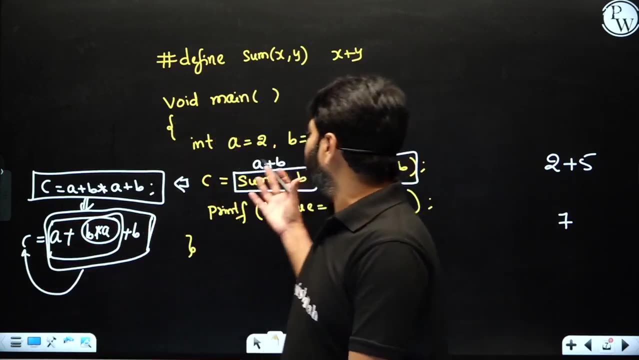 then this: a plus. the result is going to be evaluated then with that, the another plus, because equal plus only the next two operators. so this plus is going to be done next, then after that the result will be assigned to C. this is how going to be evaluated. now, if you look at the result 2 and 5, so to multiply, sorry, 5. 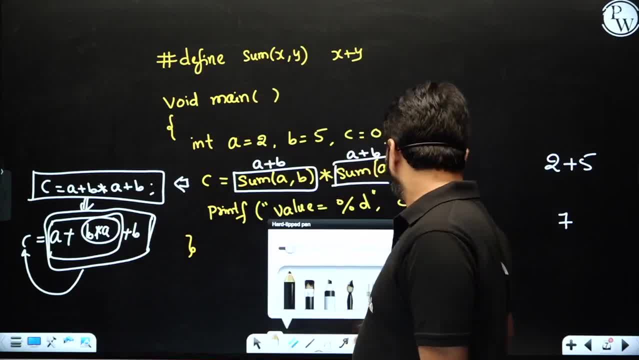 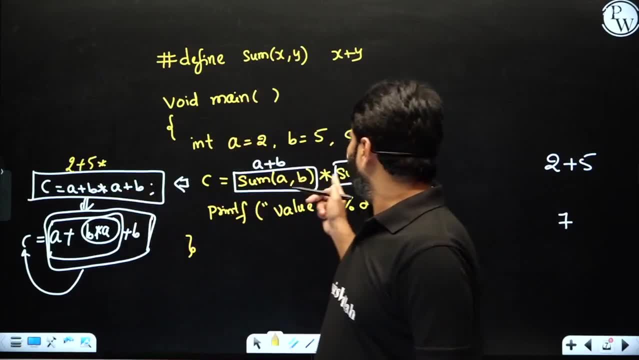 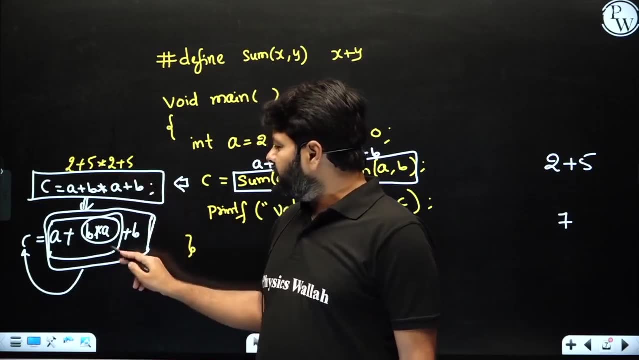 here. this is a 2. let me write that a is 2, B is 5 and multiply with a is a 2 base 5. this is going to happen, right? so what is B? multiply with a? this is going to return 10, and then, after that, a plus. 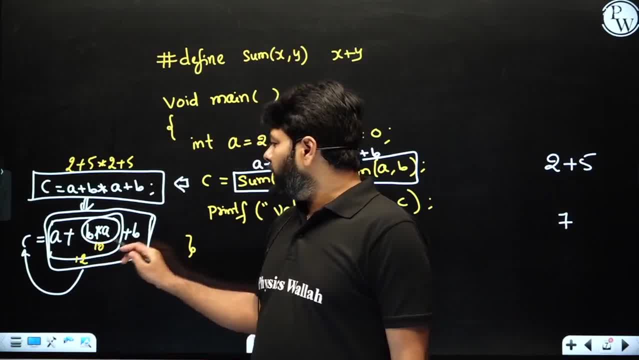 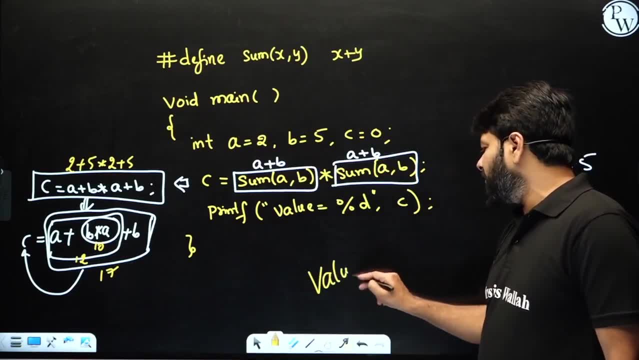 that's 2 plus 10, that's a 12. then 12 plus 5, that's a 17. so C value is 17. so here the output comes as value is equal 17. okay, then where is the problem? problem is what you. 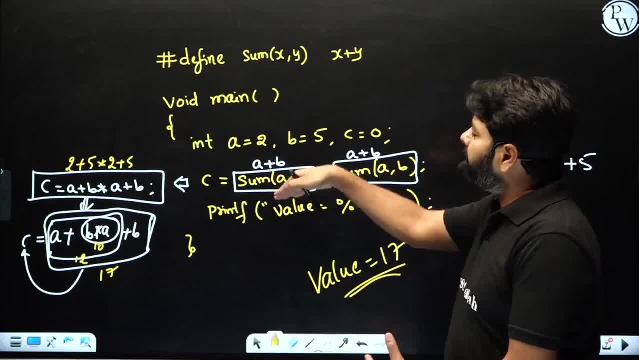 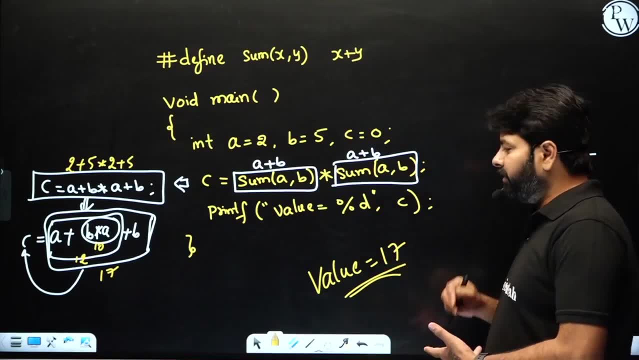 might predict. that's 2 plus 5. the 7 might be returning. what happens if 7 is returning? 7 multiplied 7, which will be 49, but where is the 14 and where is the 17? so huge difference, right, and when will be returning? when will be? 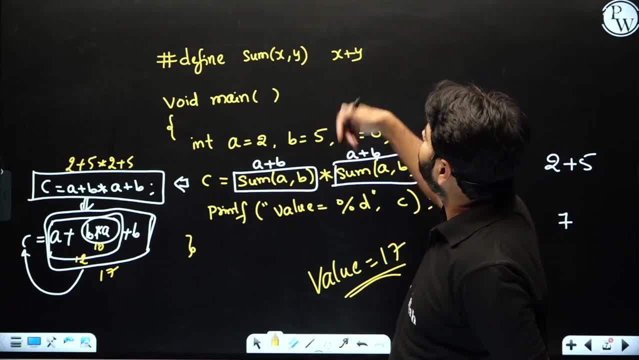 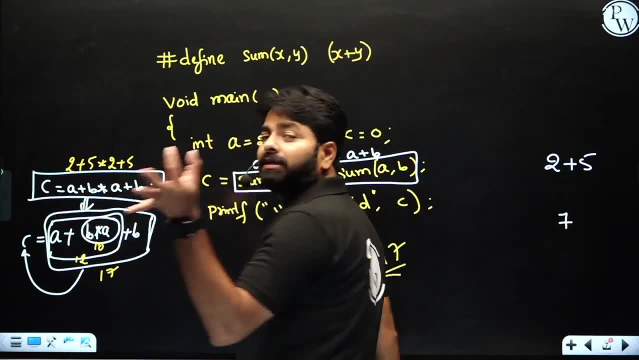 happening that in place of this x plus 5- if you give this parenthesis, then definitely we will not get in place of this x plus 5- if you give this parenthesis, then definitely the same parents will be put. then a plus b, the 2 plus 5 is evaluated first because parents is. 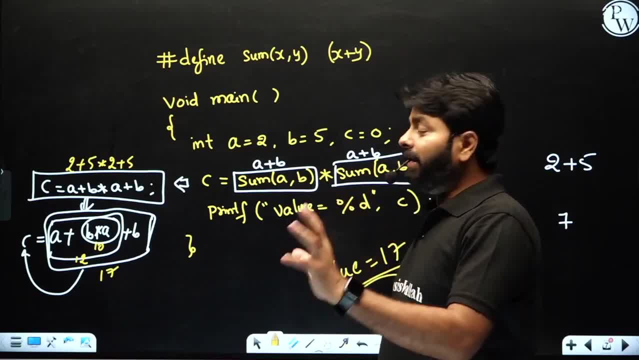 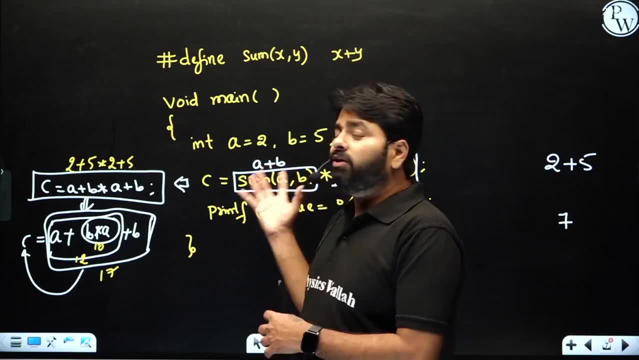 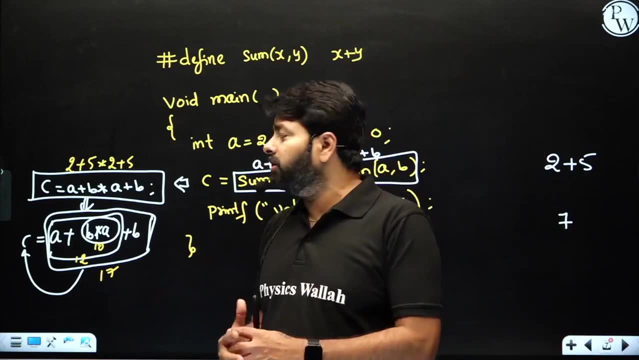 having more precedence before applying any. you know other operators. it's very important if you have certain things the you might be evaluating 2 plus 5 first, so you should know that's what the compiler required for you. somebody writes an expression. the compiler takes a decision where. 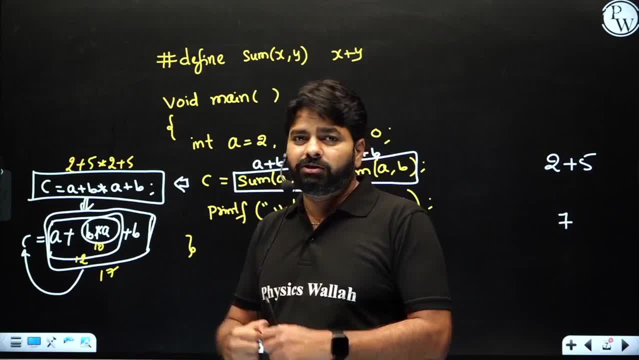 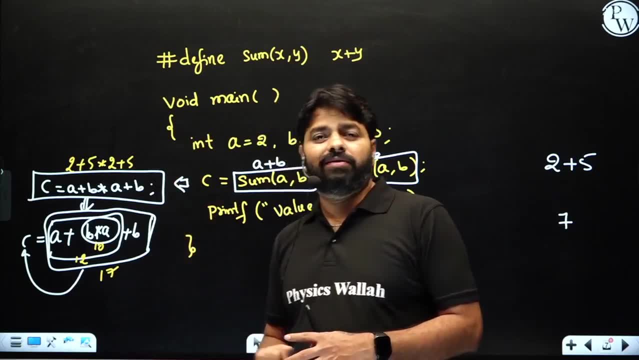 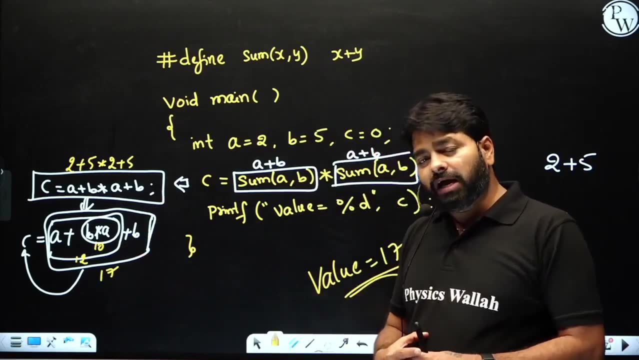 the precedence is considered because already the compiler has some precedence rules and are following those precedence rules. the expressions are going to be evaluated at runtime. so before runtime, only compiler gives all information to the motion of which operators should be considered first, which else is considered next. ok, this is about the preprocessor now. I hope you understood. 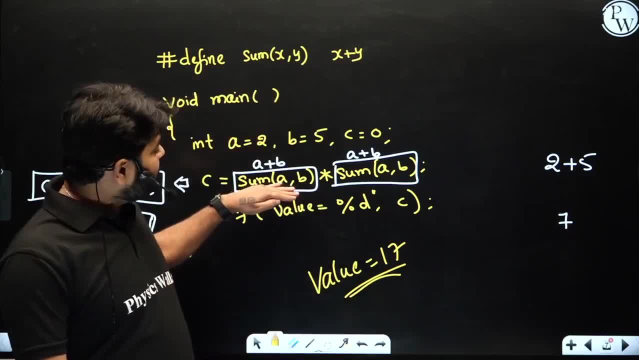 preprocessor is not going to execute. it is going to replace this statement with a plus b and this is going to improve the performance of the machine. so I hope you understood. the preprocessor is not going to execute, but it's going to replace this statement with a plus b and this is going to improve. 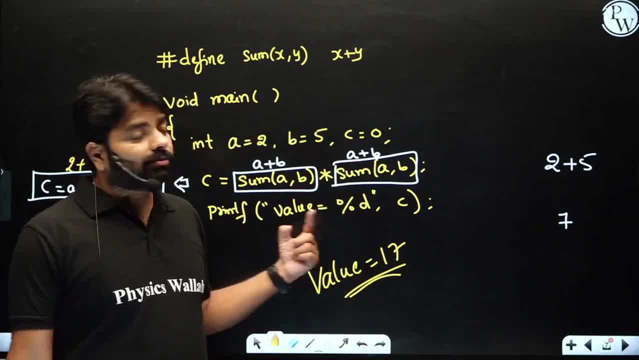 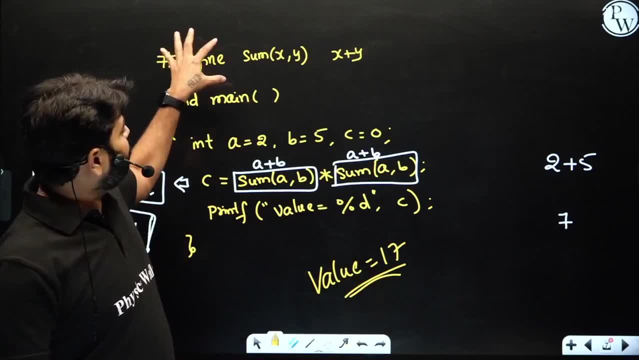 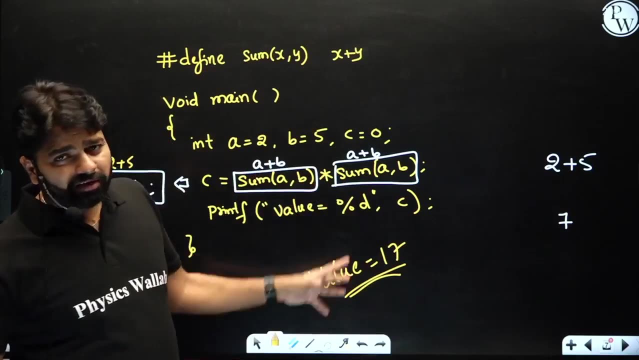 the output that you see at the end, that value is going to be 17 once you compile and run this code. and this is going to be 17. okay, but this job of the pre-processed job is to replace this constant with the expression as it is, without evaluating an expression. okay, without evaluating. 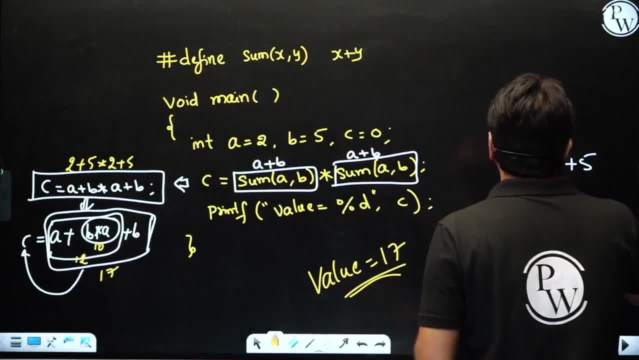 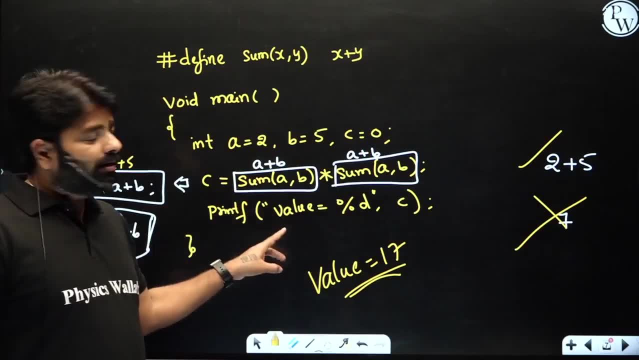 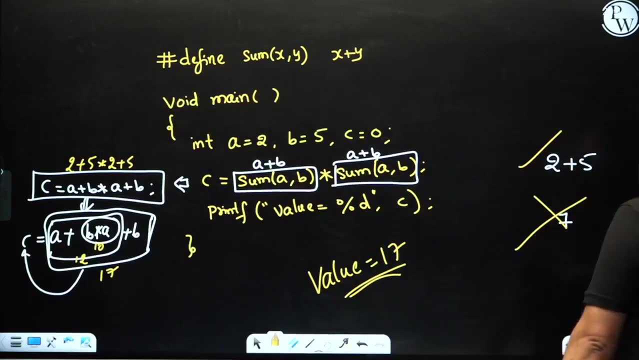 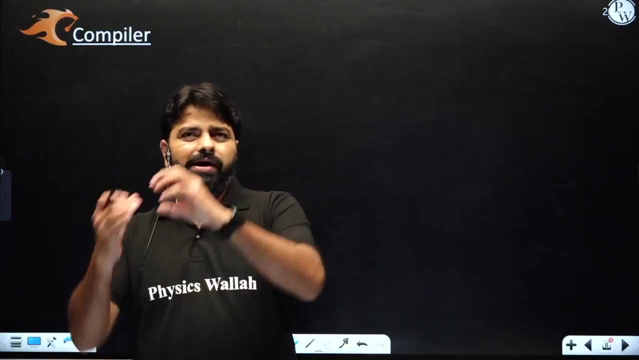 an expression. right, this is very important. it's going to be placing 2 plus 5, not 7, okay, so both are going to be different: putting a plus b, putting the result of a plus b. both are different here. okay, now you got to know. pre-processor: it takes the c code and it analyzes all the directive. 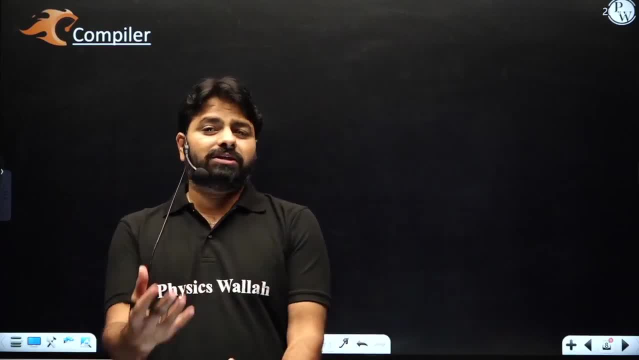 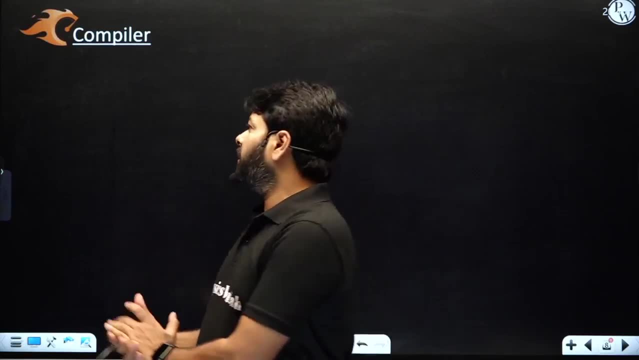 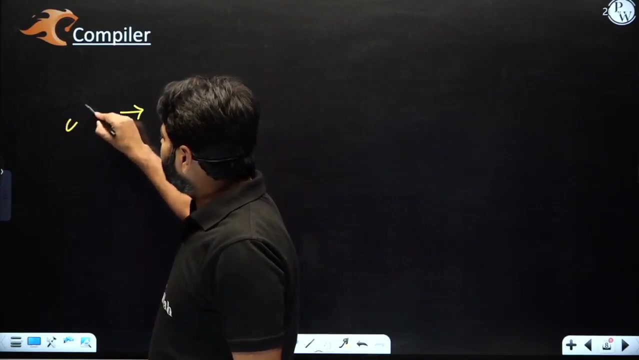 statements. then it gives you the pre-processed c code. so you don't see any pre-processed statements now, so that the c code can be understood by the compiler. so so, so what's this compiler? compiler has many phases. we will be learning them. do not focus much on that. it is also c code, but you know that it's already pre-processed one. 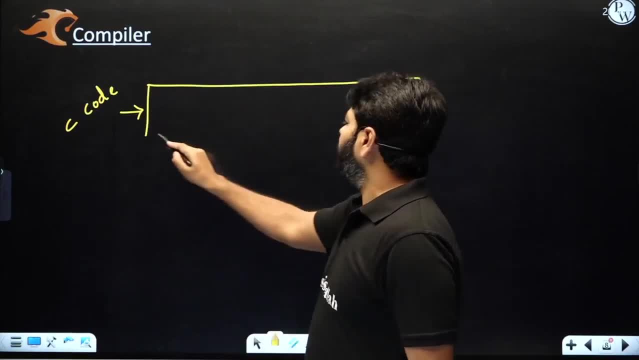 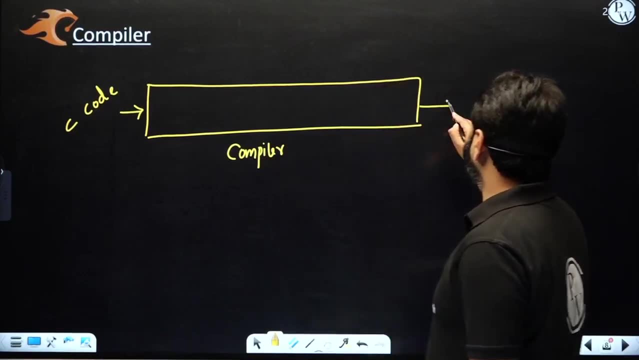 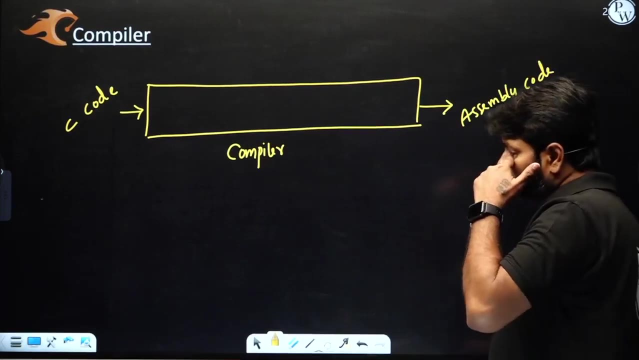 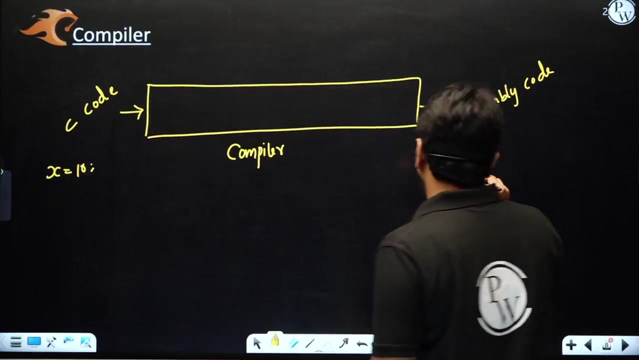 and this c code is given to compiler. it's a compiler and it produces, let's say, assembly code. do not include assembler inside, just say assembly code. example: if you have something like this: like x is equal 10, here it might be happening something. if you are aware of it, okay, not then. 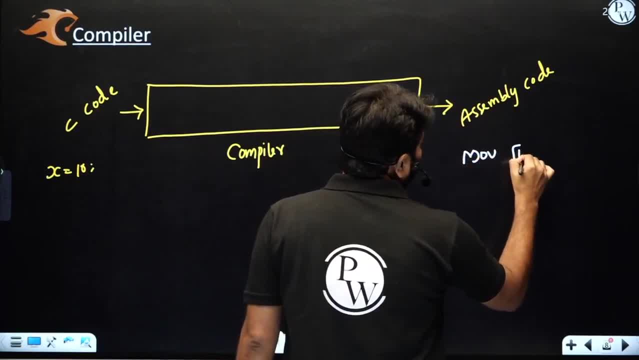 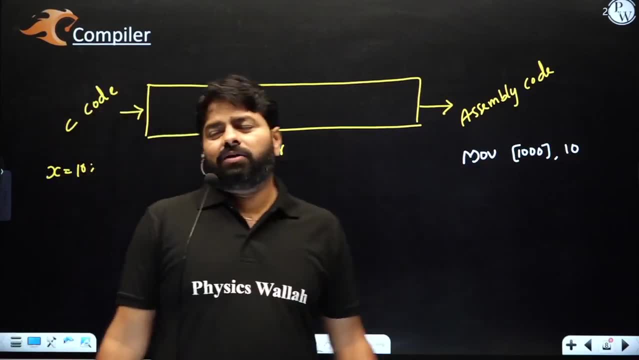 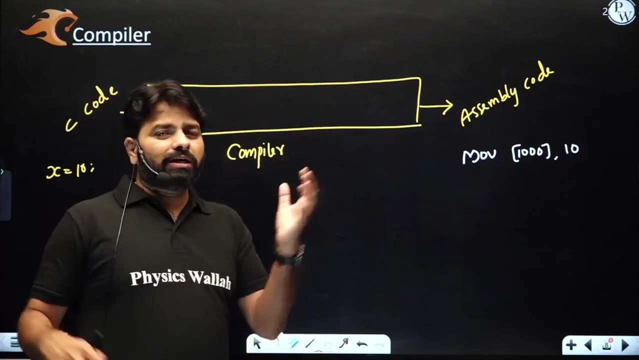 just ignore it like move. maybe you know some location. it's going to put that data 10. this is assembly instruction. right? every you know the whole c program will be converted into the assembly program. what is the compiler job? compiler job is to understand the c program and convert into. 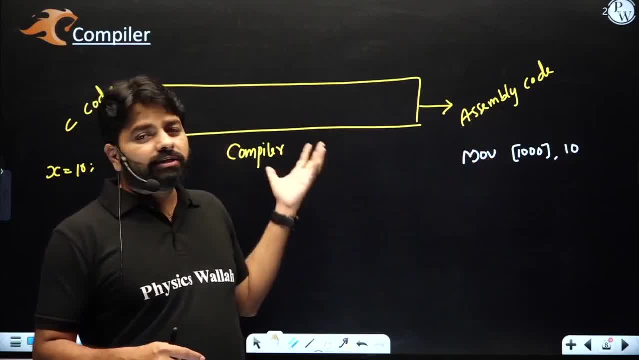 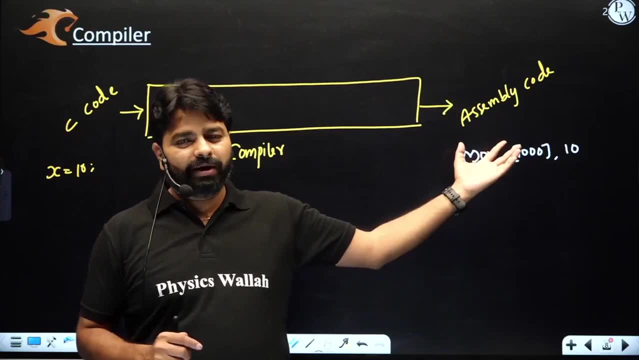 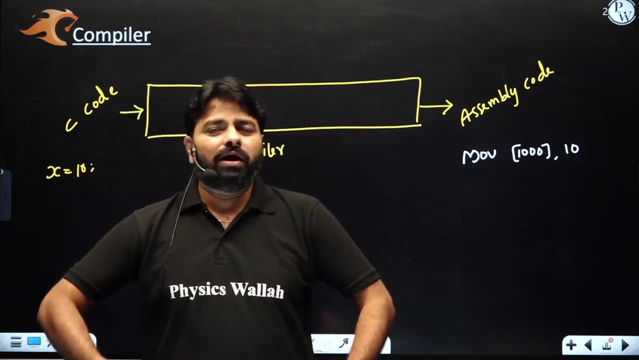 assembly program. but you also know the c program is going to be converted into the assembly program. than also the compiler is executing its own program. so 6 it's. it's a program that takes a program and converts it to another program. how beautiful it. but this is the beauty of compiler: it is executing some program because it has own power and it takes somebody which. 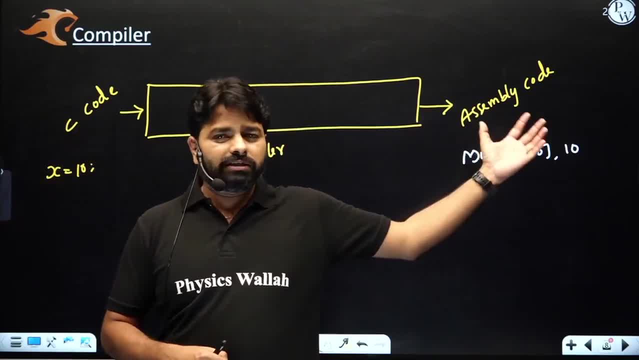 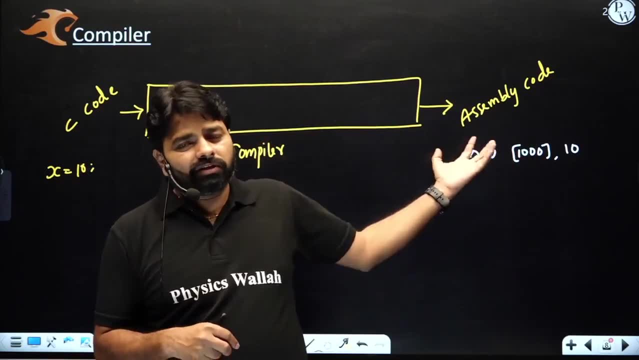 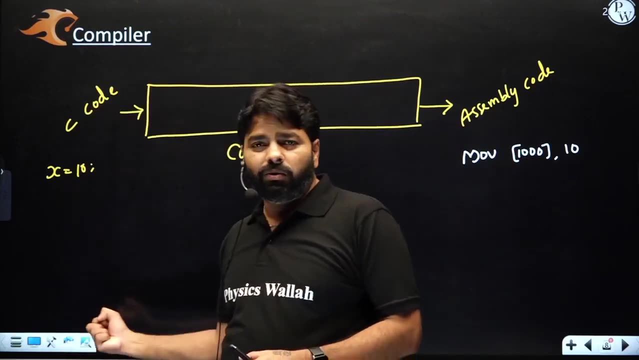 want to convert into which. you want to convert into machine code, assembly code, so it understands all c code and process something and gives to the. it converts into assembly code. so dashing, okay, so do to do that how this compiler actually understands the c code. let's see code you write. 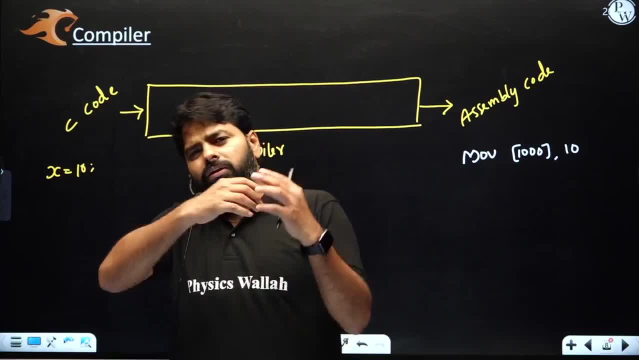 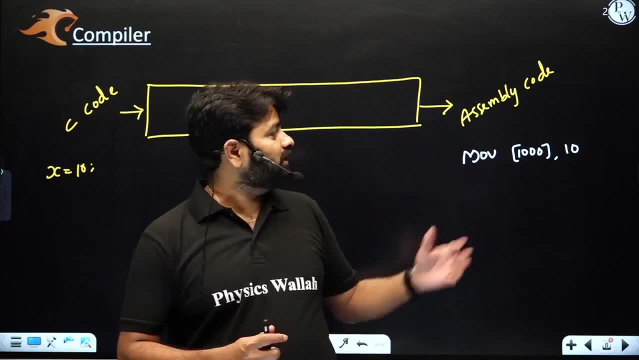 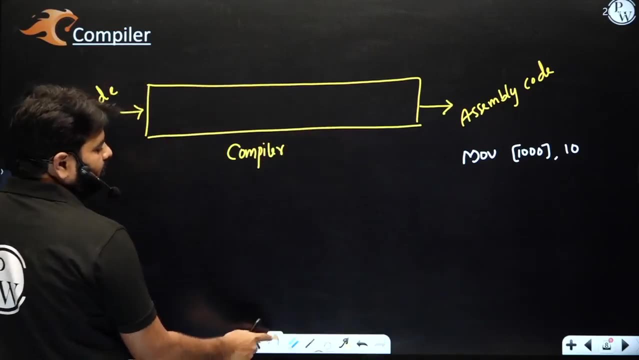 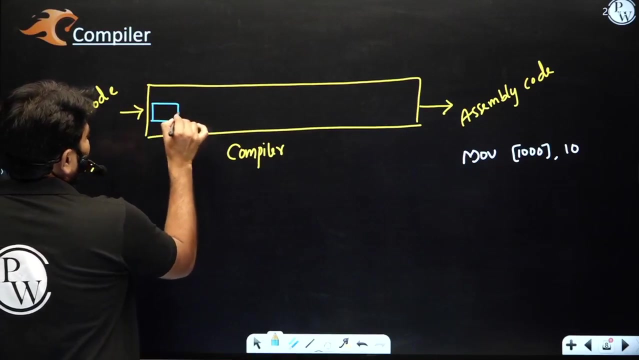 functions, variables, if statements for statements, all the statements it understands. it understands, uh, its syntax, it understands the semantic and it converts into the corresponding assembly code. correct, so to do that. it has various phases. we'll be seeing soon, but let me write some of them here here. there are many phases, like you have lexical analysis, then syntax analysis, then syntax direct. 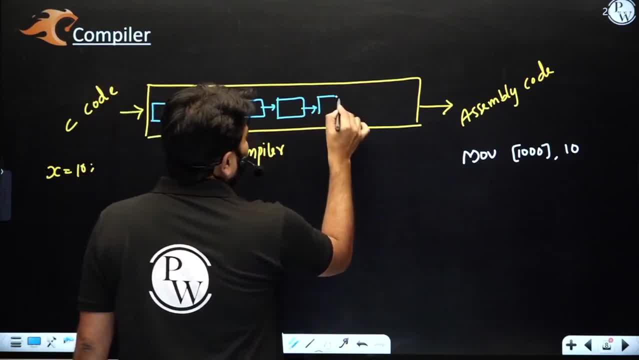 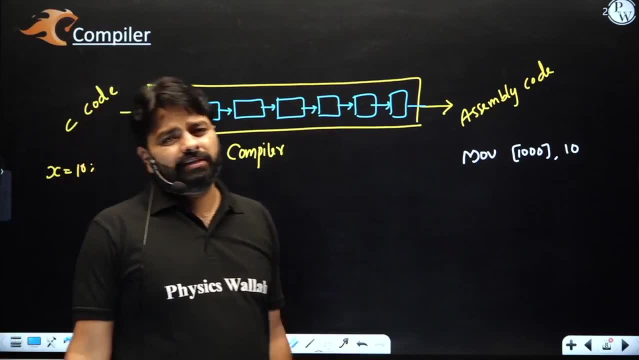 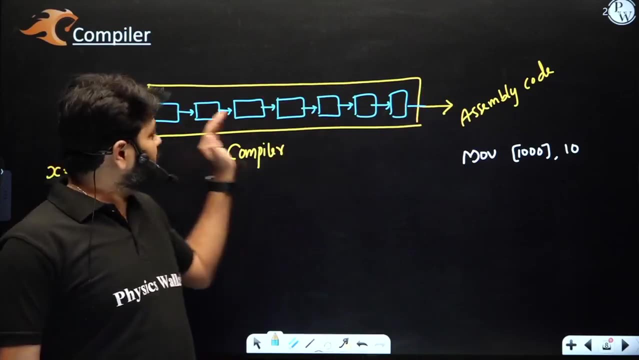 semantic analysis, then intermediate code generation, then code optimization, then code generation, then code optimization and that's it total. you will see seven phases to convert the high level code to the low level code, high level code to low level code. this boxes i'll be disclosing once we see the introduction. in the introduction you do not require right, so at the 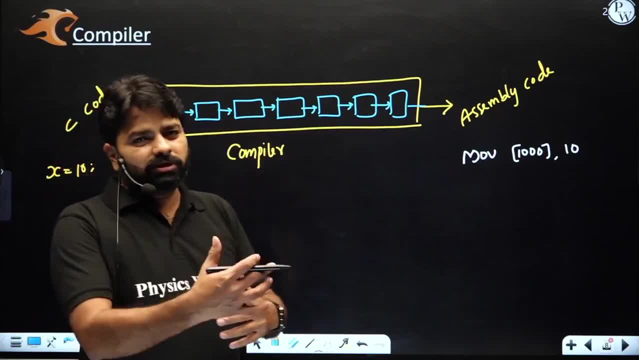 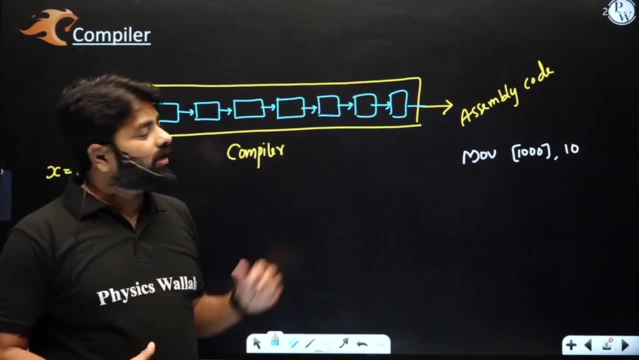 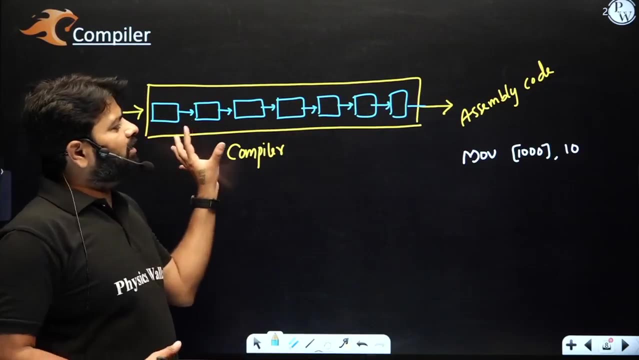 end of the introduction we will be seeing after this c language processing system. we'll talk about the compiler, what are the phases and how it produces an error and what other things required to understand or to analyze this code and produce the assembly code. fine, so this are the you know. 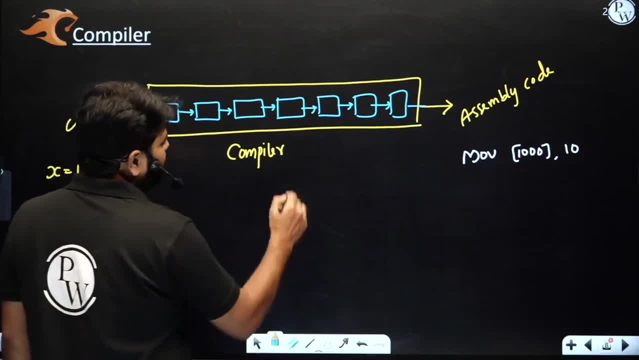 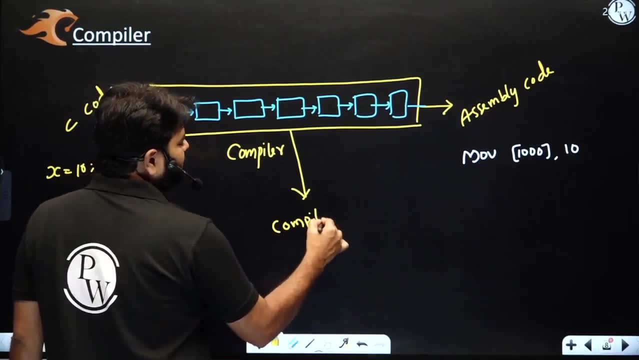 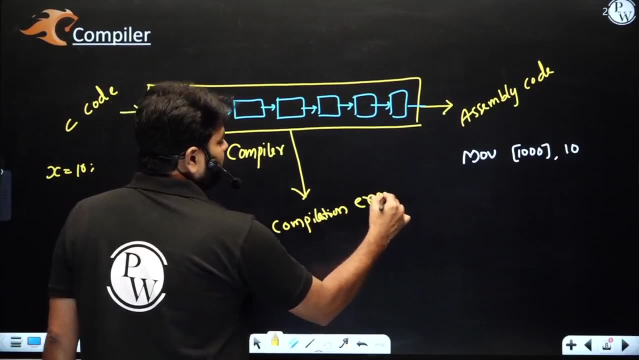 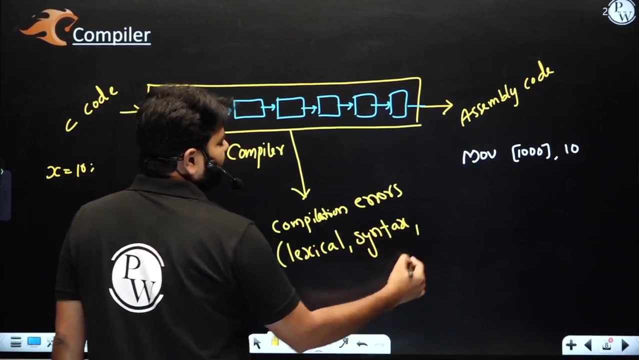 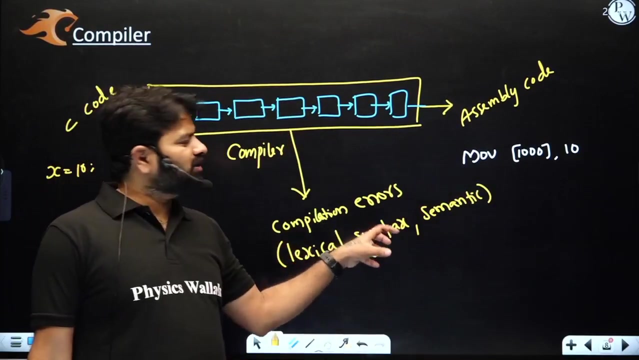 this is the thing that we are going to do, and compiler produces a syntax error whenever it doesn't. whenever it has seen some errors, it also produces special errors. there's a compilation errors. compilation errors like lexical syntax, mostly the syntax or favorite here remaining. compiler decides how to produce right. mostly we will focus on syntax and some are semantic. 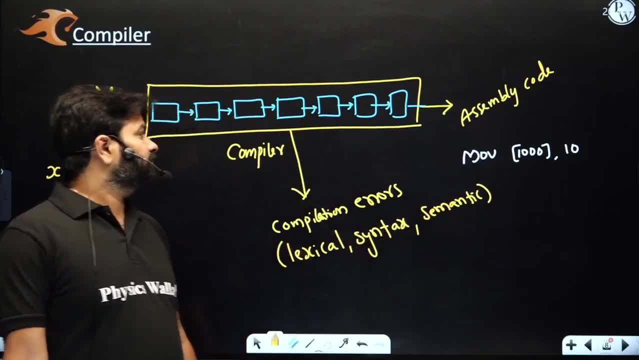 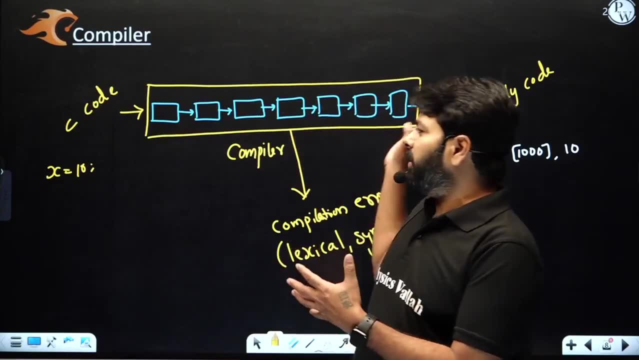 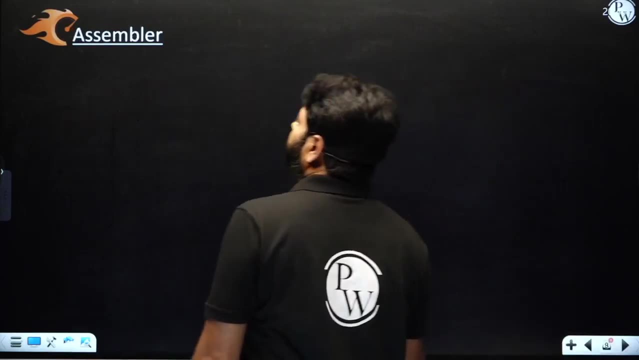 lexical is very special here. we will be saying in the first chapter: okay, this is all about compiler, the whole subject we are going to just look at inside this compiler and different phases of the compiler- okay, we'll come back, don't very much about it, we'll come back next. assembler: okay, we don't deal much about assembler, as you. 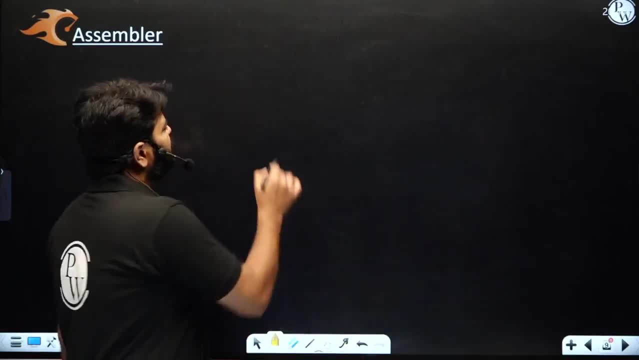 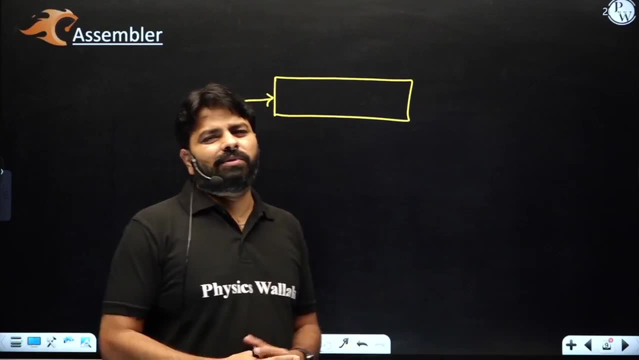 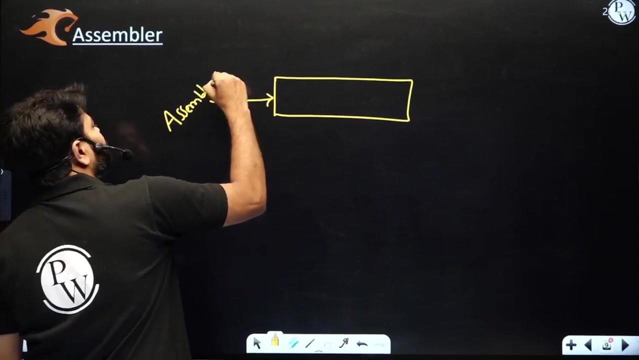 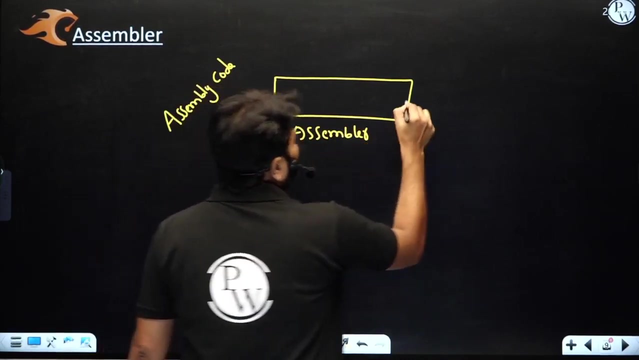 know we are talking about compiler. just we'll talk about, you know, simple assembler definition. we don't go in detail about assembler like one pass assembler, two pass assembler, the various things right, we'll just look at. we give assembly code or assembly program, this assembler analyzes this assembly code and produces machine code. of course, to do that the assembler should have the 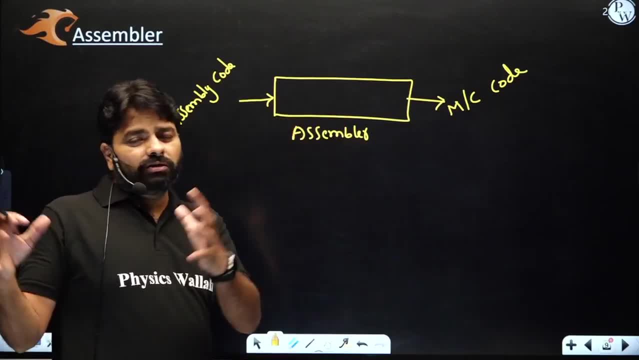 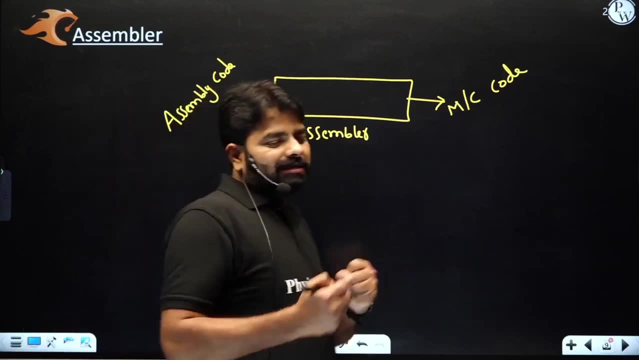 knowledge of many things, because this purely depends on the machine, and every machine the assembly assembler is going to be different. so you don't, you know, remember customers to call you should make these assembler. thank you guys, thank you the assembler. and you don't install that way. assemble is fixed once you buy the system right. 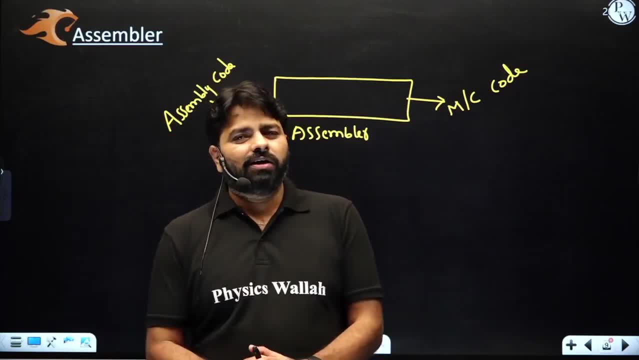 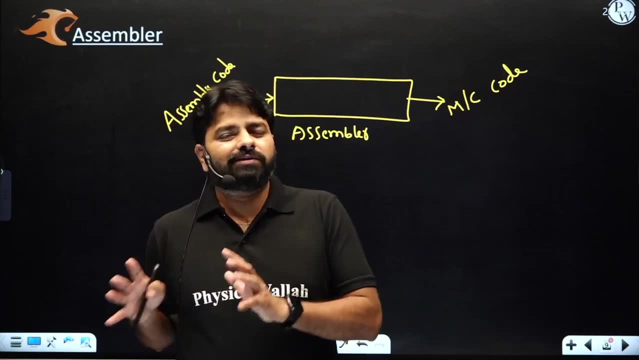 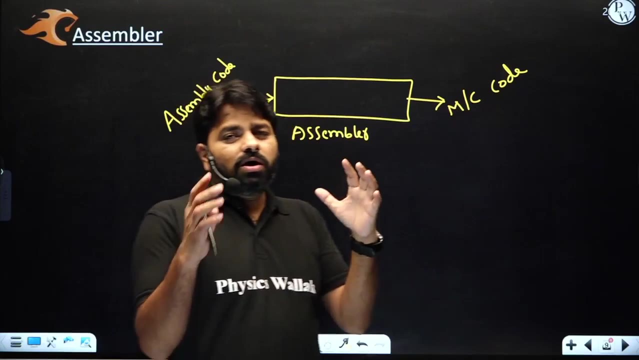 because once you design the architecture, once you have the architecture of the system, then this are similar, already fixed, because you can't change the assembler to the machine. every machine has a fixed assembler to understand its own assembly language, because it purely depends on the machine. okay, but compiler you can install whenever you require it, and but compiler also. 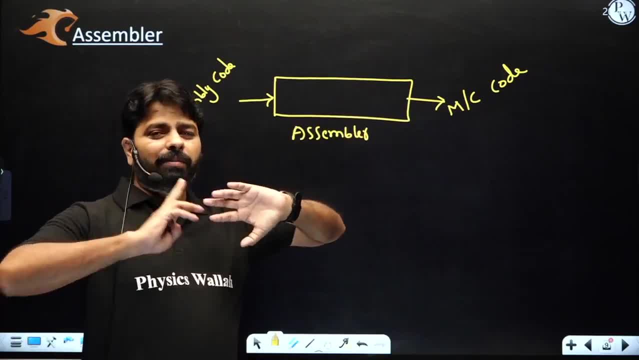 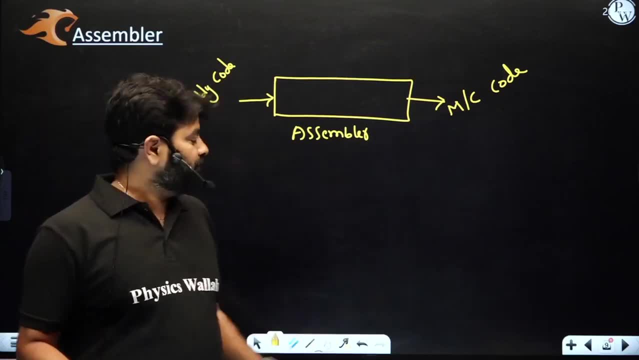 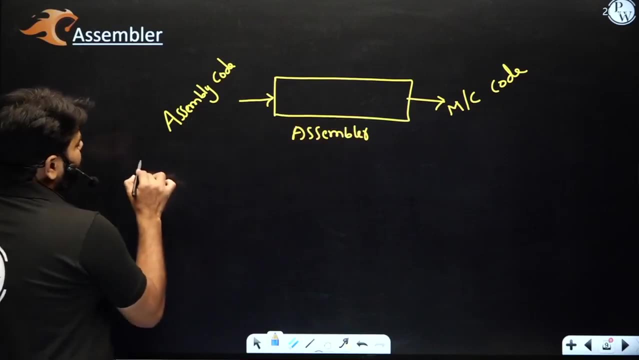 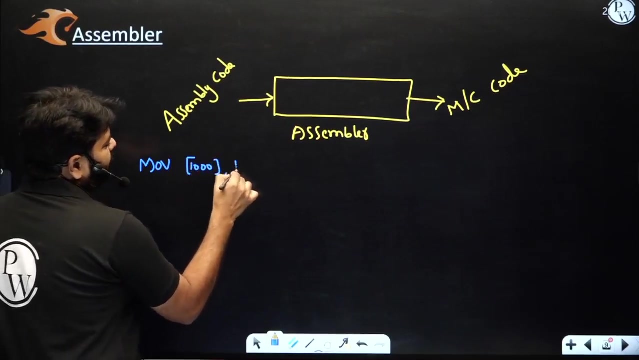 depends on assembler, assembler depends on the machine. indirectly, compiler depends on the machine. this compiler has to produce assembly, assembly code, and assembly code varies a machine to machine. okay, now what's happening here? let's say move, uh, previously i was writing something like right thousand comma ten. then what this assembler has to do, it has to convert the whole. 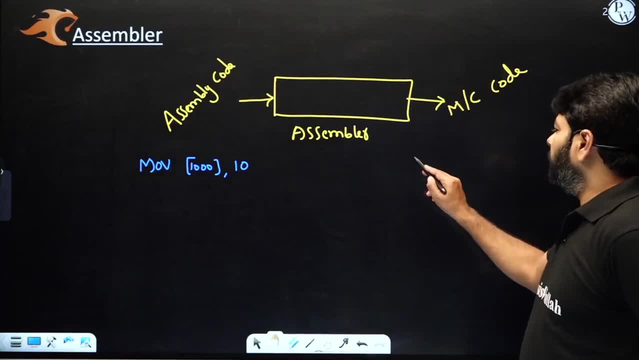 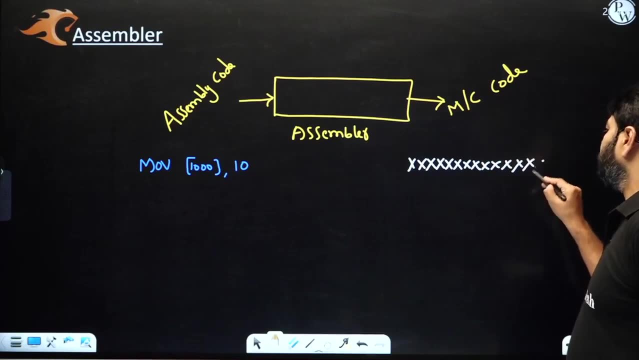 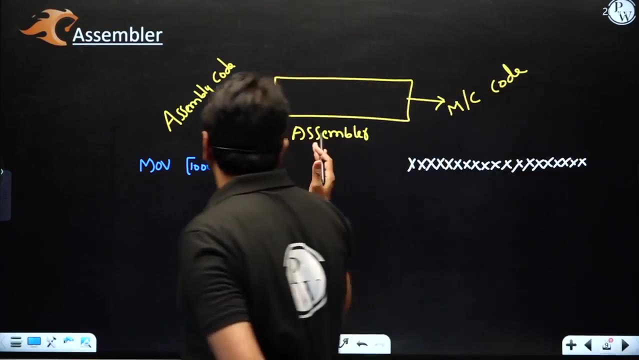 uh, instruction into zeros and ones like: i'm just writing x, x, but this x is nothing but either 0 or 1.. it's going to convert into something like this: the x is either 0 or 1. okay, what might be happening here? it has to understand. assembler. 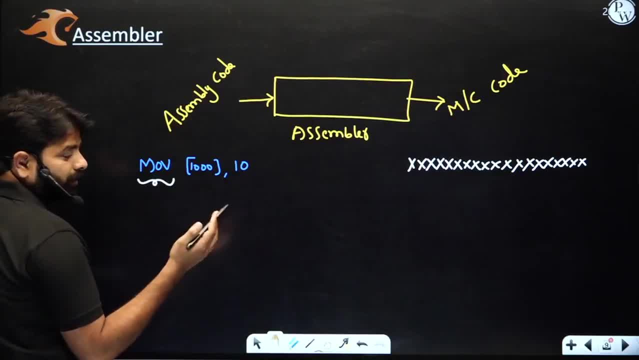 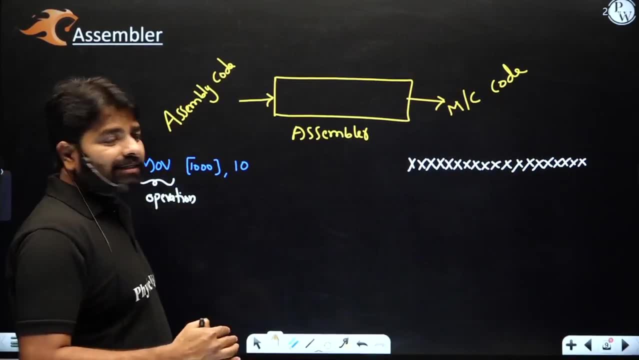 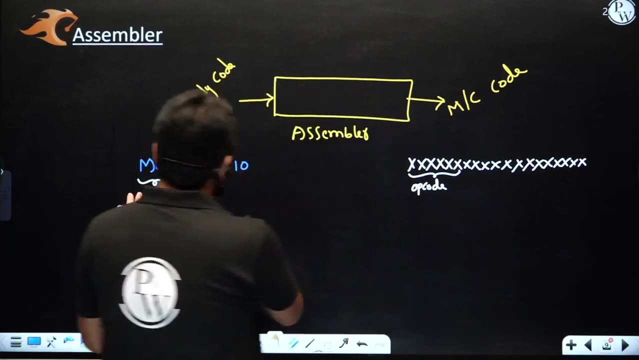 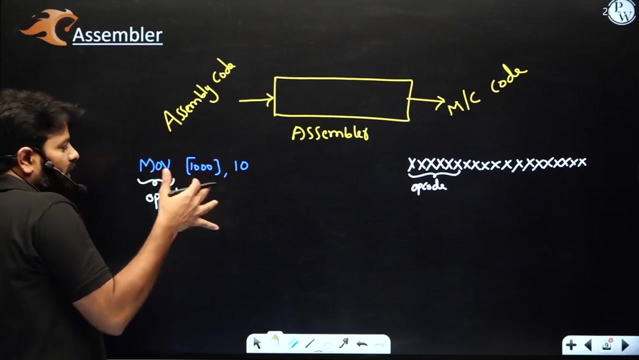 is going to understand. what is this opcode, corresponding mnemonic code, and it's going to be operation. right, what operation it is? what is the corresponding binary sequence for this? it might be some sequence for this opcode, corresponding opcode. this operation has some mnemonic code. it's going to replace with that and here and this whole instruction. right, it's an instruction. 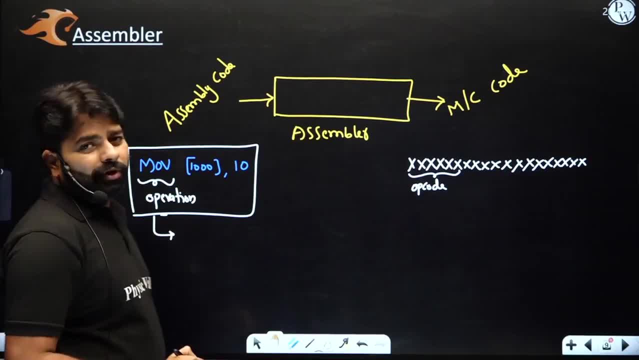 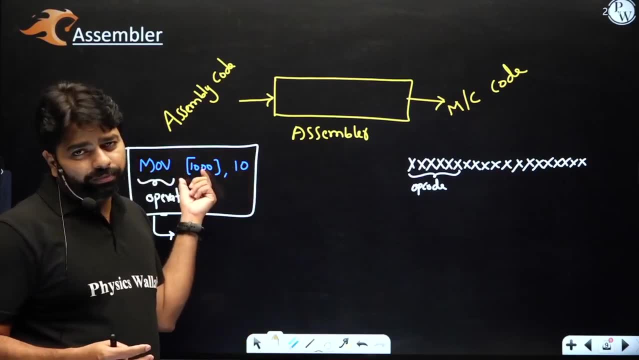 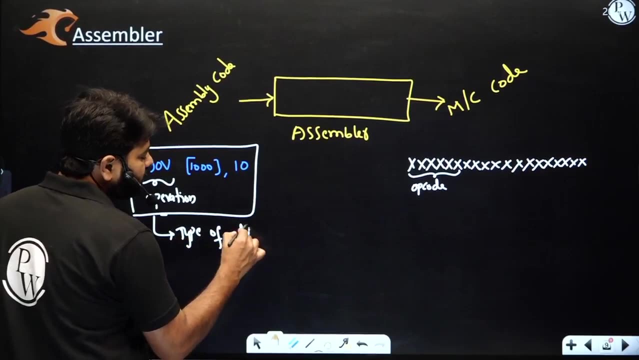 this instruction is. what type is it? memory direct memory, indirect register, direct register: indirect. so it's kind of the immediate instruction where data is you are going to place in some of the memory location. so what is the type of addressing mode? type of addressing mode: if you study computer organization, definitely you will learn. 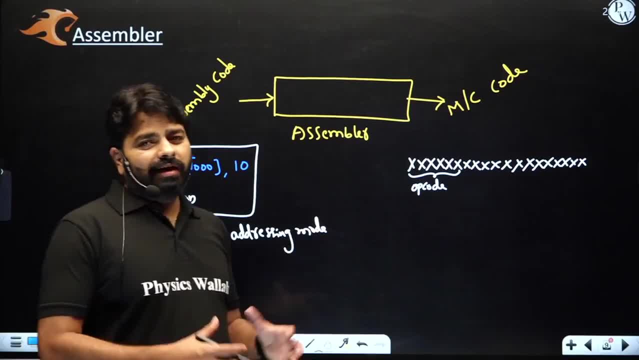 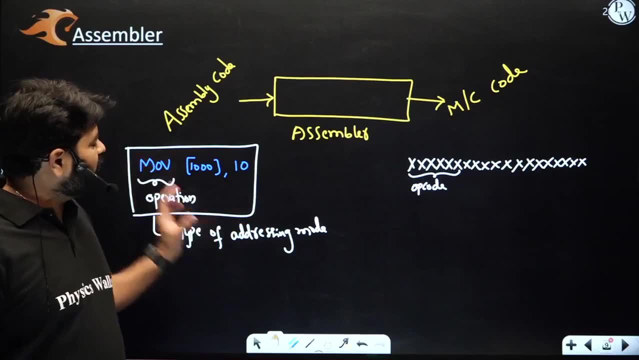 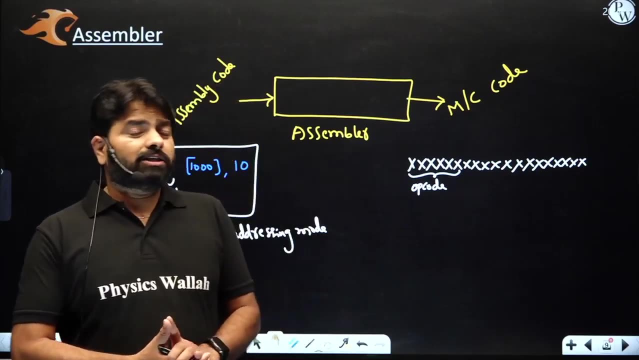 addressing modes. there you will see, uh, the immediate instruction, or you know, one byte instructions, two by three byte instructions. you will study different types of instructions. right there you will see types of addressing modes and type of addressing modes if the machine supports, let's say, 16 addressing modes. for the 16 addressing modes you require four bits, so the 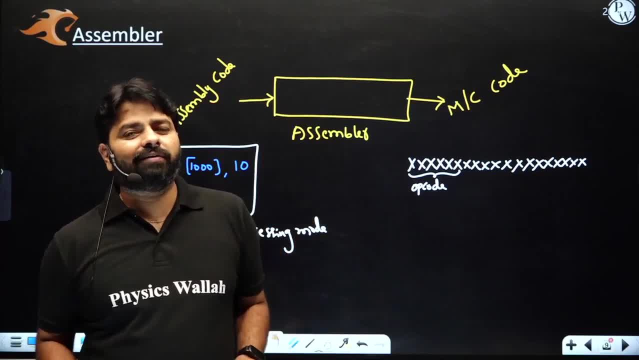 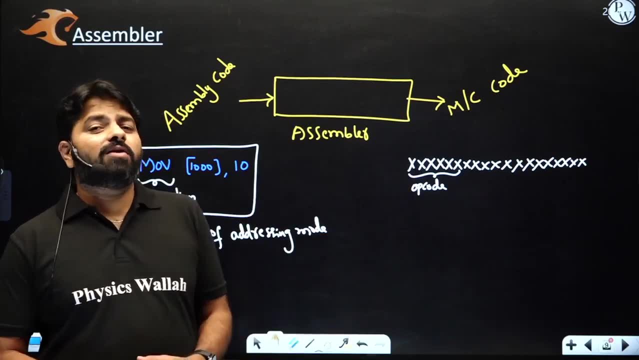 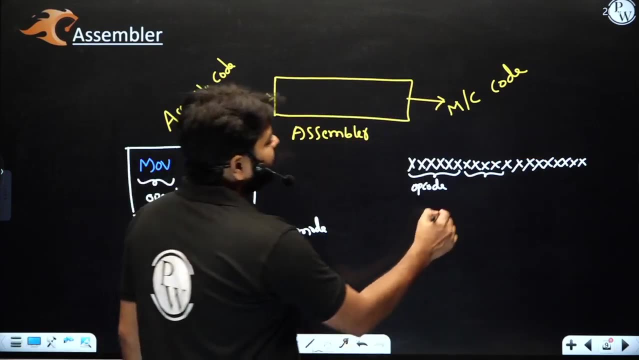 difference between the two is that, using four bits, i can, uh, uniquely identify the 16 different addressing modes. so let's say my system is supporting 32 addressing modes, then you require 5 bits. so how many bits required that depends on your system. okay, let me say that four or five. 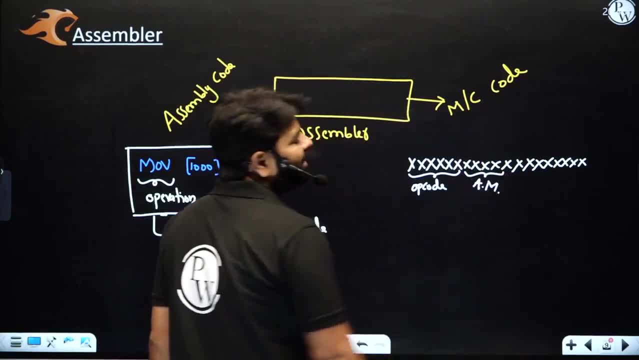 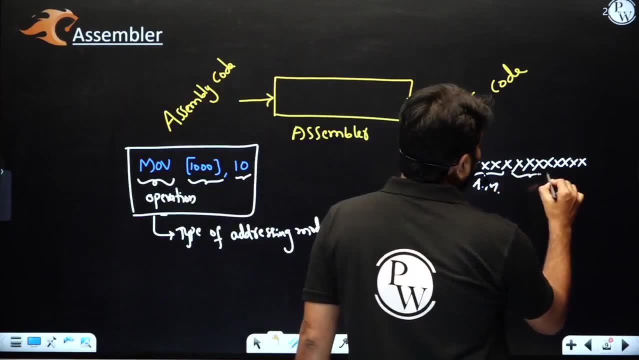 this might represent. what is the addressing mode? a dot m represent addressing mode and then maybe you know you have operand one, operand two. similarly, you require, you know operand one, operand one, something else, operand two. if you have any other, just include it. but this is how the assembler understands. 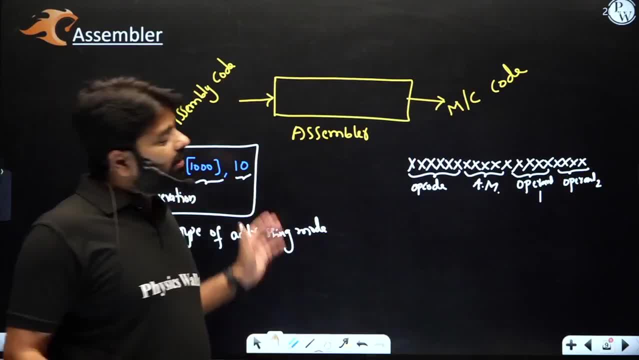 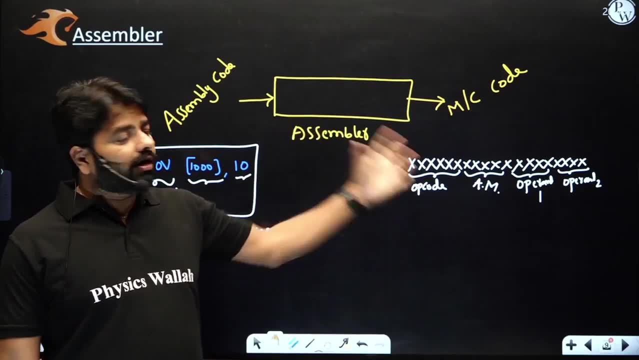 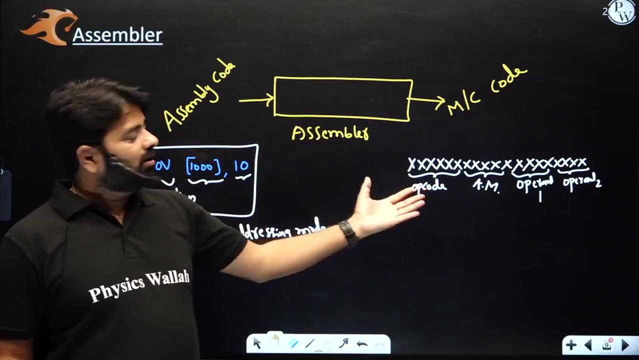 the old assembly instruction and it has a mappings inside and it converts to the equivalent machine code. equivalent machine code. but whatever it does is already done by the compiler. it's just converting. assembler is not having its own knowledge. right, it's just depending on the motion. but this is. 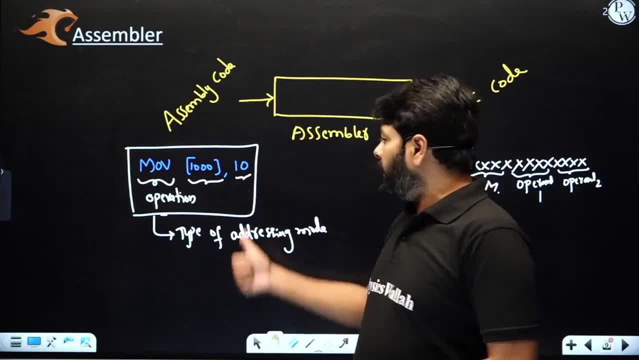 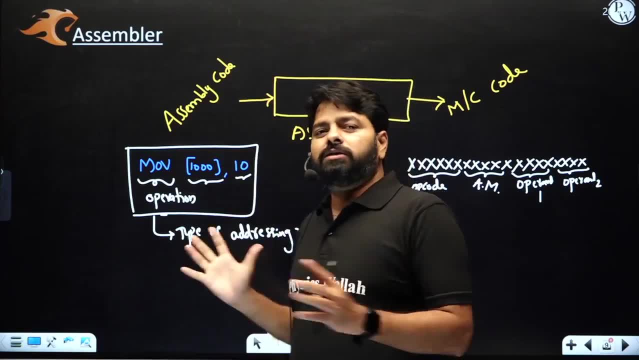 already done by the compiler. take some address 1000 and i have the data 10 and it is the move instruction. the compiler already instructed the assembler to do this. so assembler is going to do by looking its own mapping, because that mapping known to the assembler, because what system is? 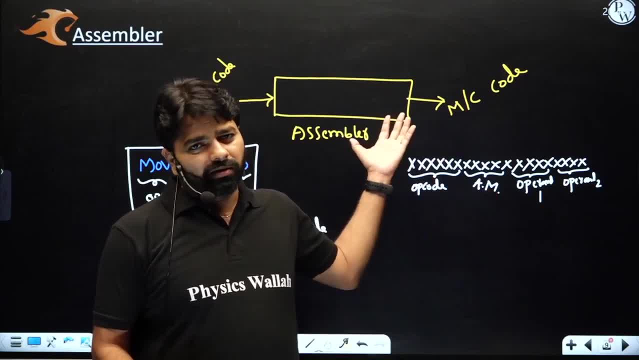 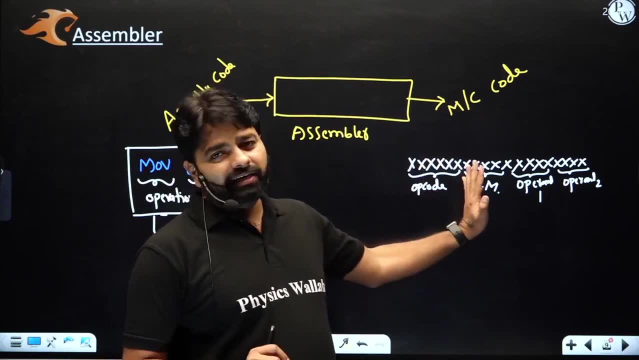 uh, actually, you know, having that's known only to the assembler. if compiler knows that, that compiler has to be fixed to the system, right, we can't uninstall and install. that's why we need the assembler support. then after that, here we are going to look at the assembly of the assembler. 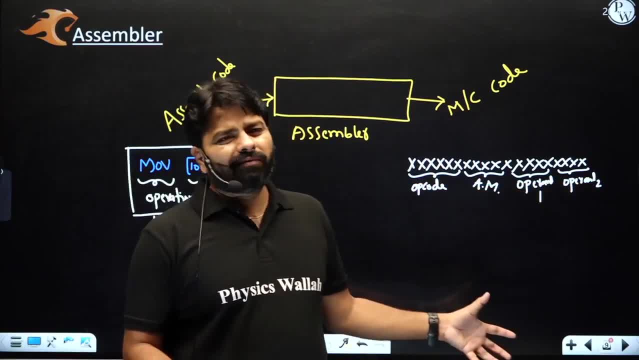 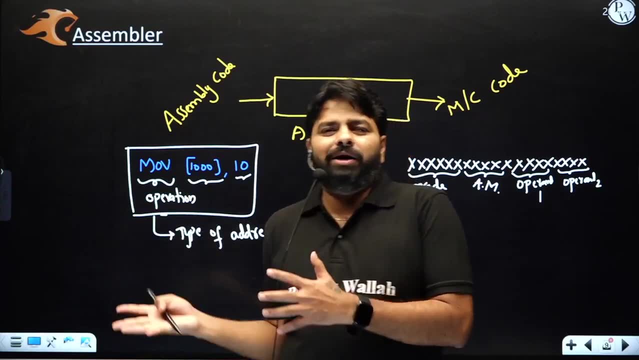 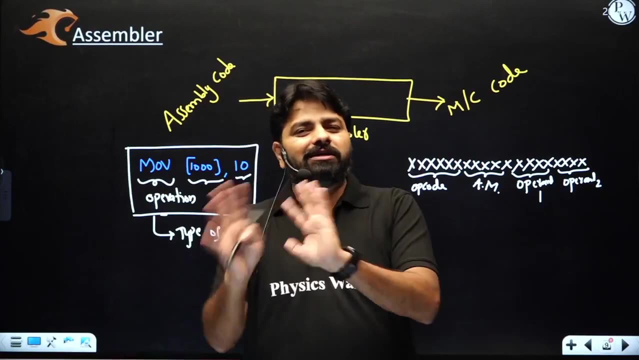 what you have done is: uh, you know, may not be available. sometimes you want thousand address here, but the thousand may not be available in the uh main memory. somebody might be occupied there. then you require some support of loader. the loader comes into picture. it can alter the addresses of. 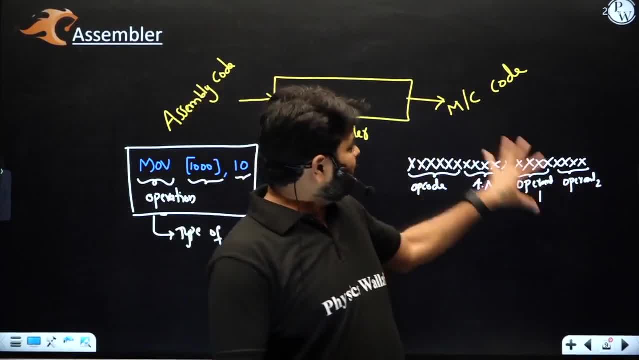 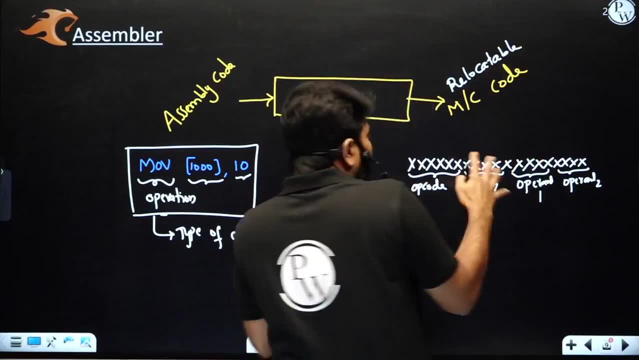 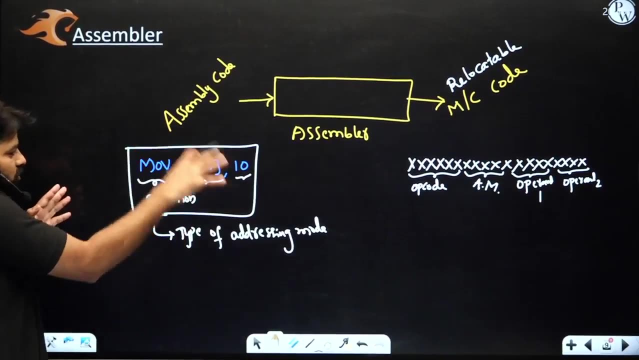 the instruction or data. that is the next part. so whatever the address is produced, it's going to be relocatable means it can be changed whatever the assembler does. it's not fixed everything here. what the 10 is fixed, the operation is fixed, but this thousand and it might be stored somewhere right. 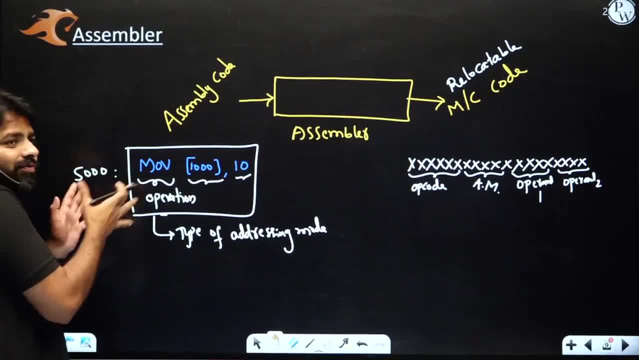 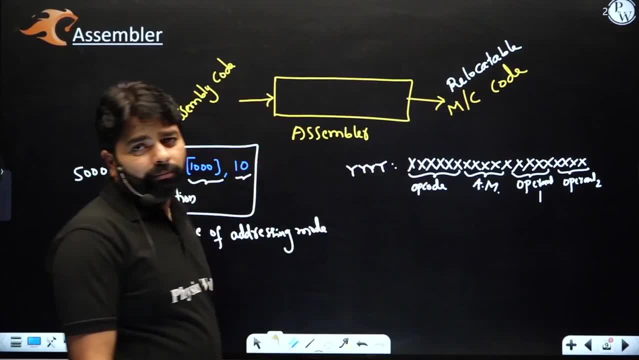 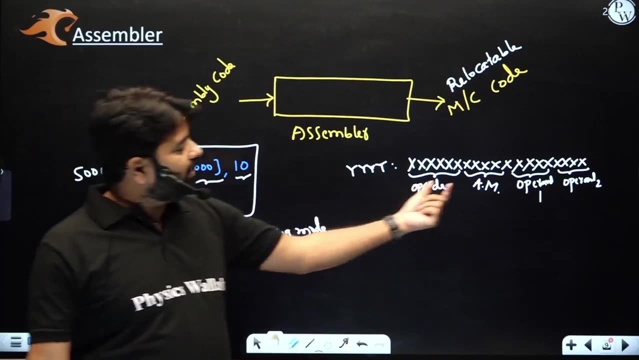 let's say 5000, because 5000 is an address where this instruction is stored and that 5000 may be changed later. it could be moved to 6000 if the 5000 is already occupied. the loader decides here two things. i am talking about this thousand, maybe that operand one, and this address of an. 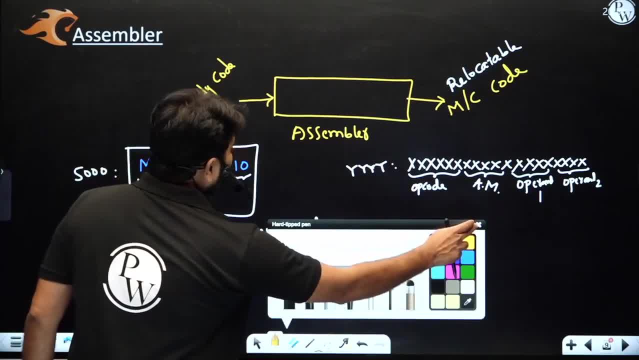 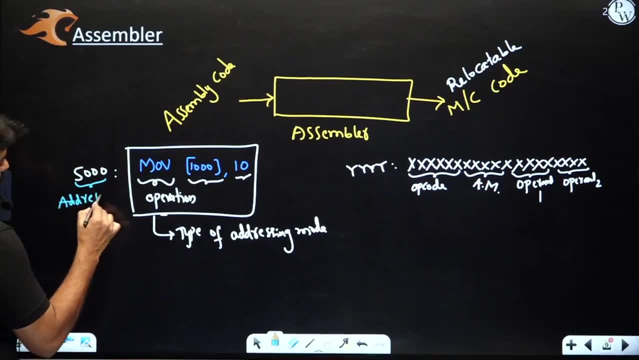 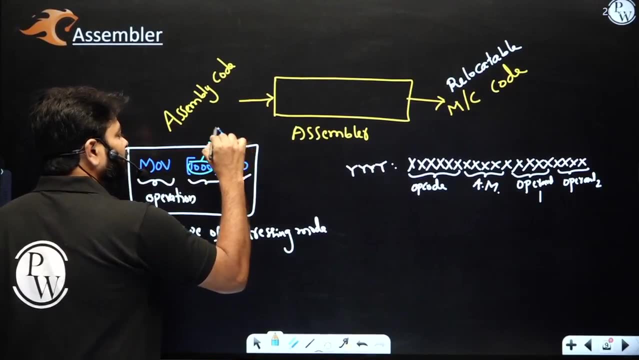 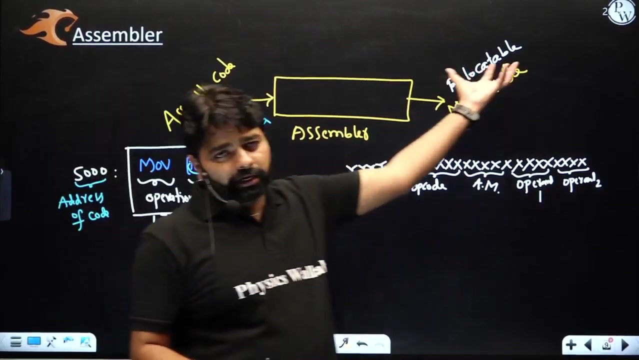 instruction. there are two addresses that you are dealing here. right, many are, how many are dealing here two addresses. this is address of instruction, or you can say address of code. and what is this? this thousand, especially this thousand, is address of data, address of data, and these two addresses are actually relocatable. so what assembler produces? 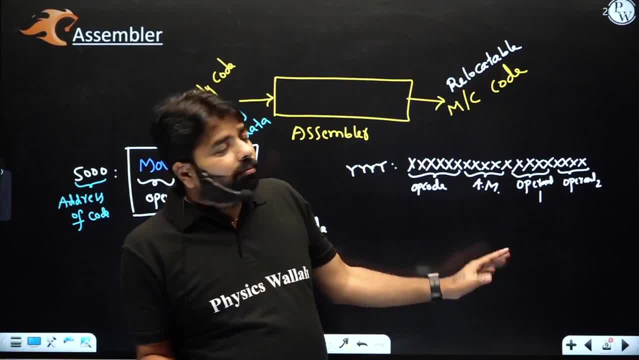 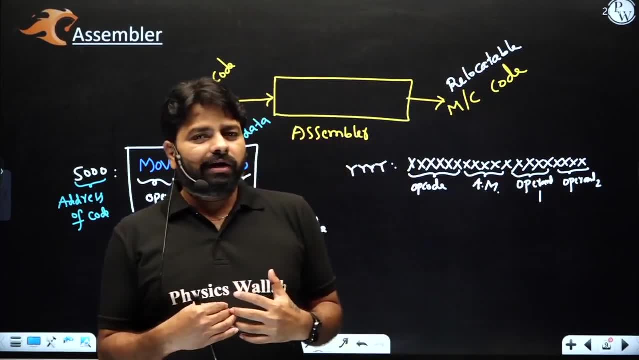 it's not knowing about it. it will directly produce a machine code. but whatever the addresses it has, the loader understands it. okay, some are at some addresses which you are asking me right now. they are not available, so i will change them and but the logic will be same. there is no difference in the logic you 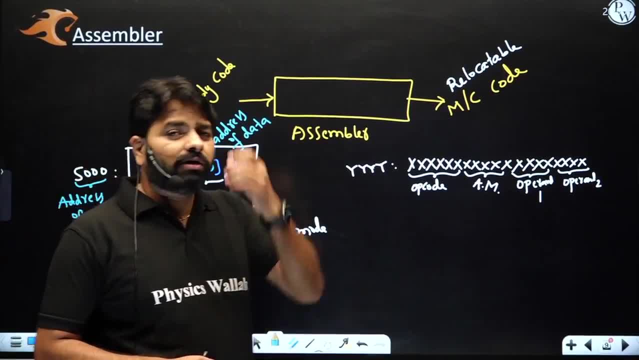 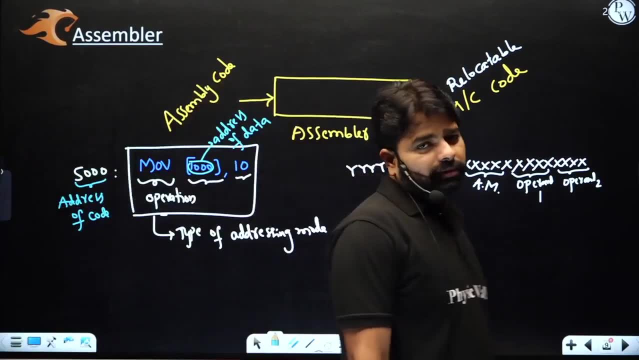 want to perform the 10 to be stored into the some memory location, it will do the same, but not exactly the address given by the compiler or assembler. fine, this is about assembler and really you want to know about assembler. okay, the whole thing, whole thing can be done. 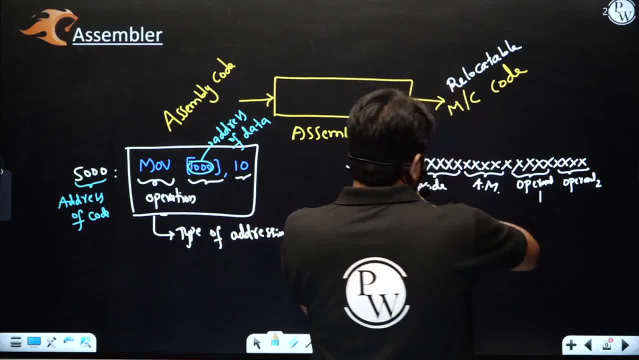 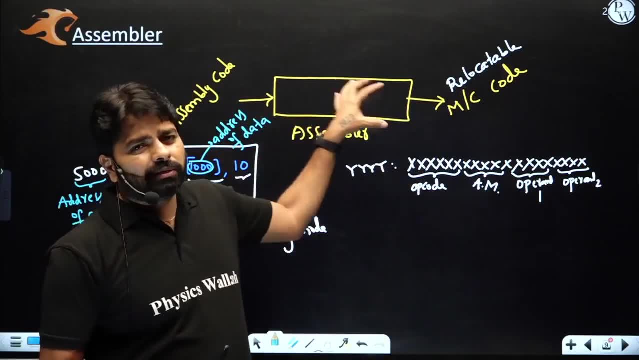 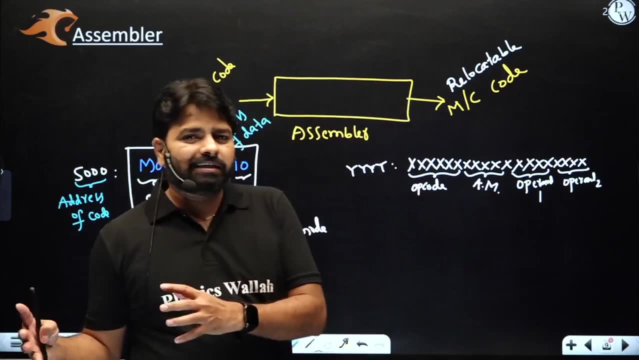 in one pass or two passes right to to convert into the uh, the assembly to the machine code. the whole process can be done in either one pass or two passes. that depends on how the assembler is implemented. fine, we are not going into that details, but anybody want to learn. yes, you can go for the assembler implementation and check that. 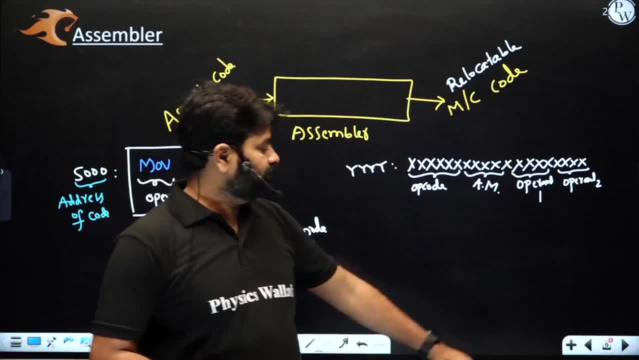 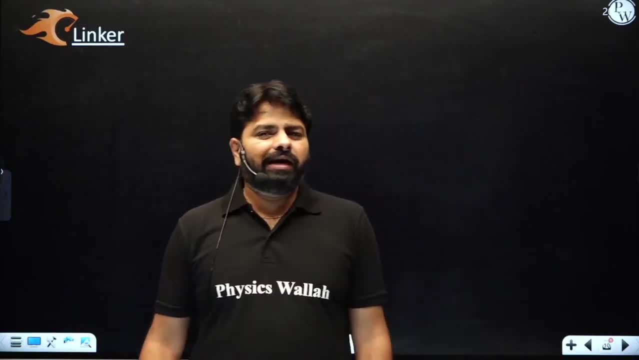 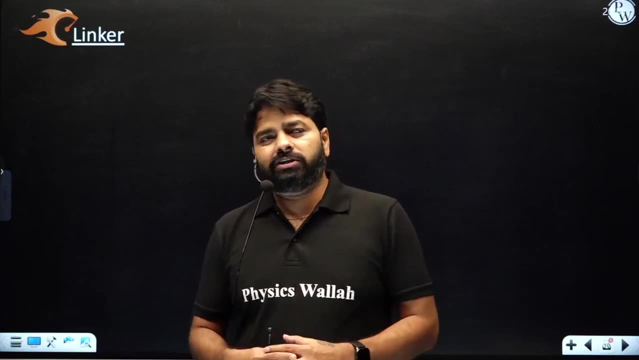 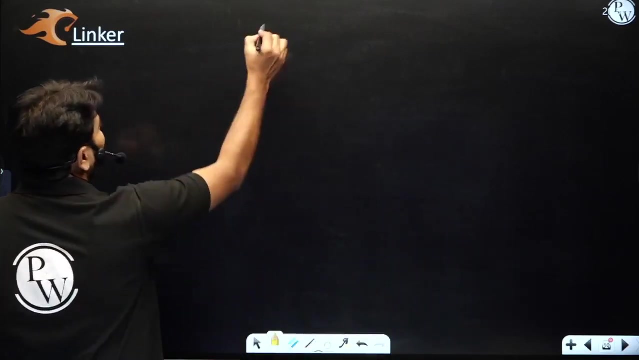 how the assembler does different passes like compiler. now we are almost near linker. as you know, the linker is going to help you when you are referring x nulls, x null or references or external files or external variables. the linker main purpose is here. you have many things right. let's say: this is your file, program file. this is, let's say, file one. 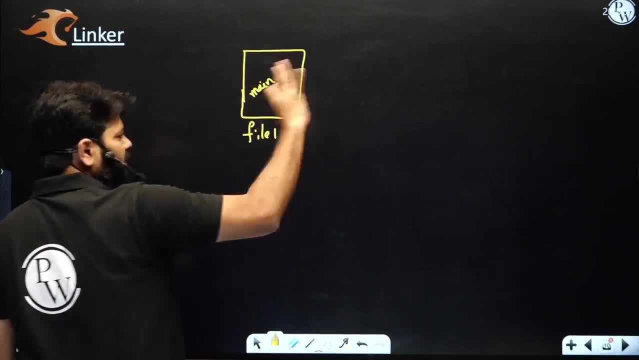 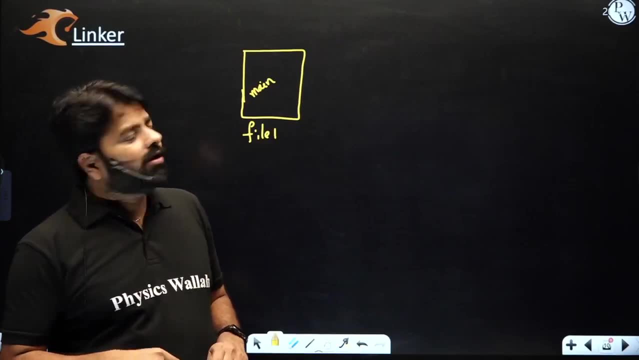 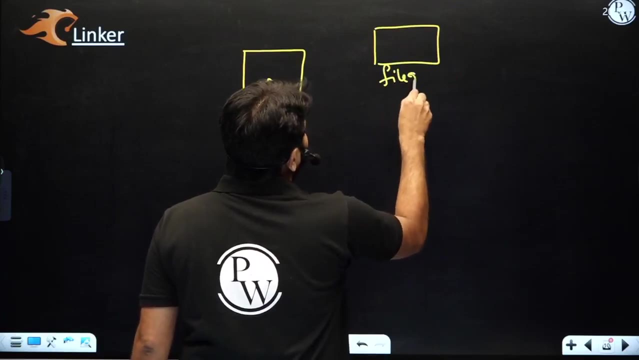 you have main function here, let's say the main main file for you, that is the first program need to be executed there. you have written the main function, but this not only the file right, there are many other files actually needed to refer. let's say this is a file 2. you require to link this somehow. 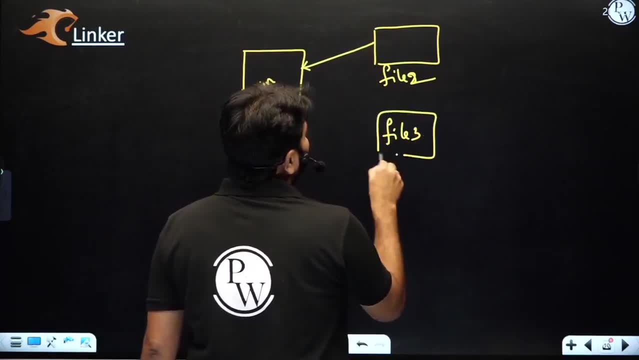 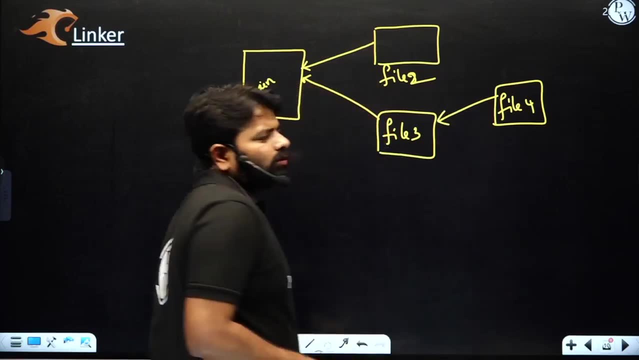 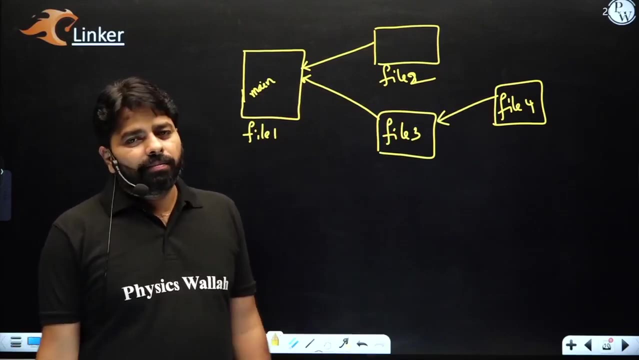 and there could be another file 3 you might require to link here, or there might be file 4 it might be linked to here, and how this is going to be resolved. who is going to resolve? is it pre-processor or linker? going to be resolved by the linker, but why do you want to refer external files? 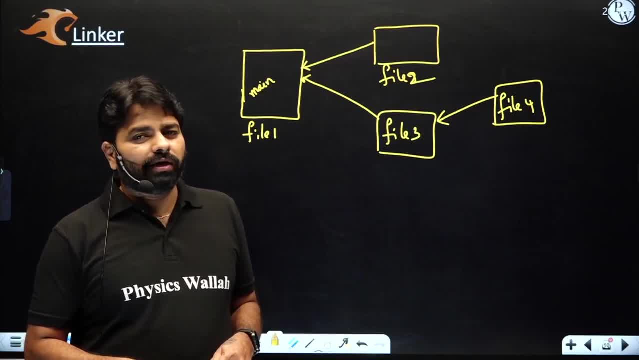 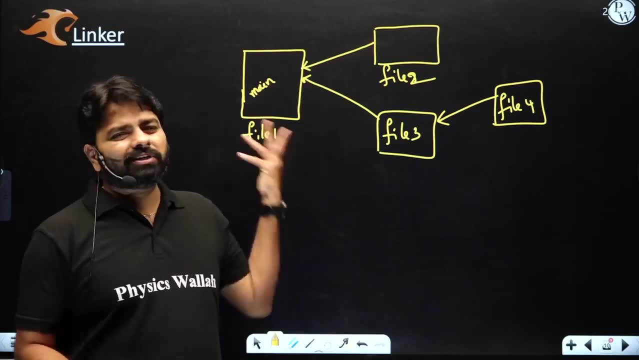 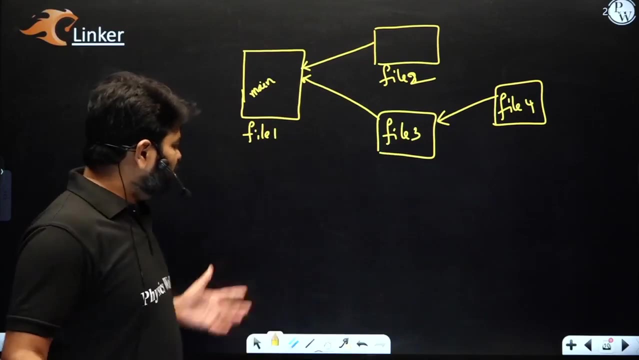 because you might be using, or you might be calling the functions or you might be using variables. what is this? functions and variables. sir, i already have the functions of variables inside the main. why do i want the functions and variables from other files? yes, you should. you know very simple. 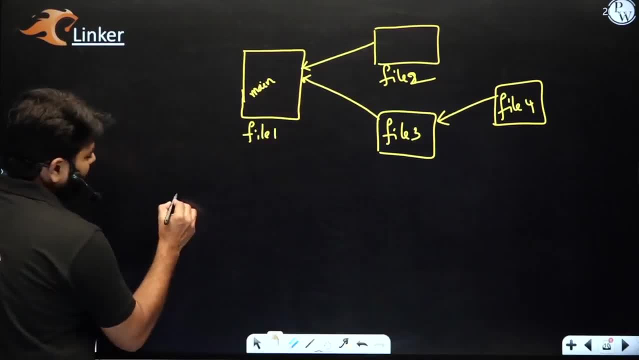 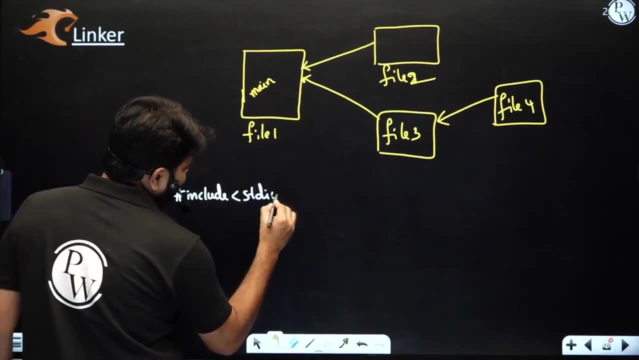 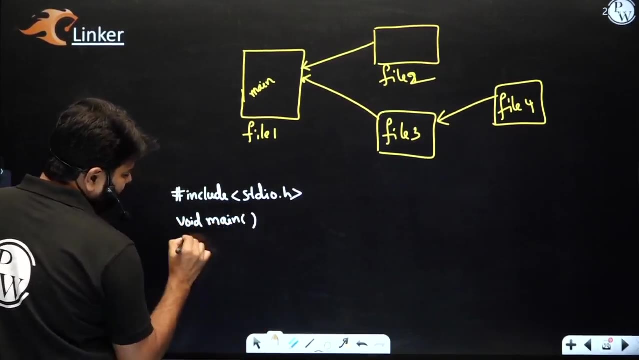 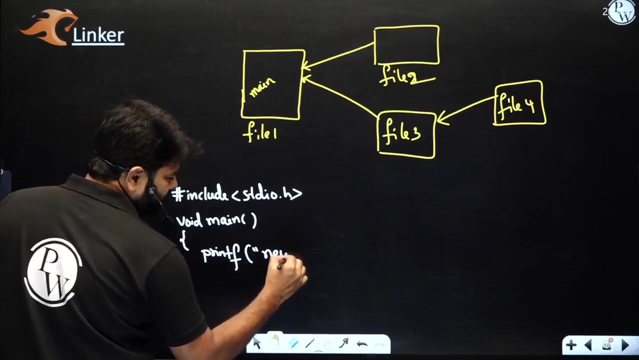 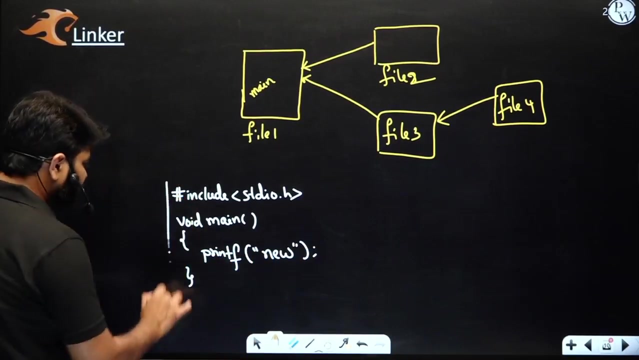 program that you are writing every time. let's see that what's actually happening: ash include. let's say stdio dot h, very famous, right. then you write something here wide main, and then you write printer. let's say the first program, let's say new. now look at, is this one file? no, it's actually the file do you want? you want to execute but this? 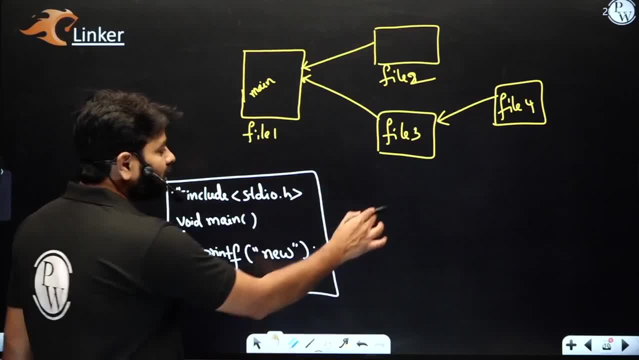 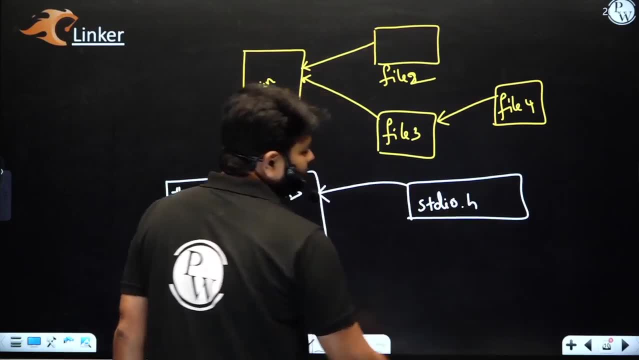 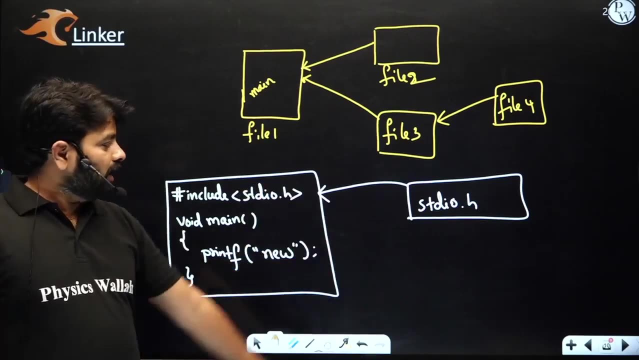 cannot be executed without std over dot h. that means there is another file which is linked here. file is linked which is stdio dot h and there is a corresponding library file where the printf definition already converted into a binary code and this file, without this file linking this file, cannot execute that. who? 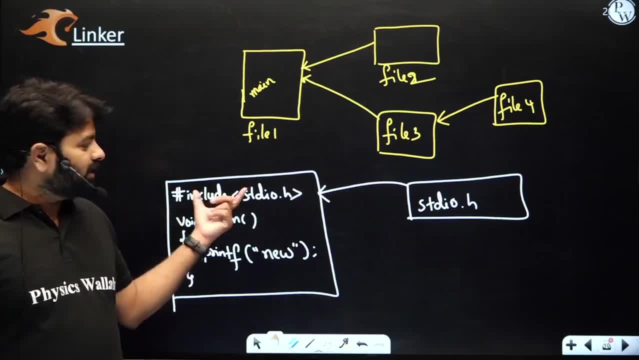 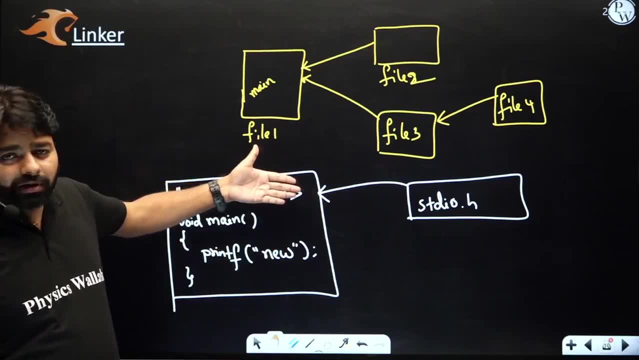 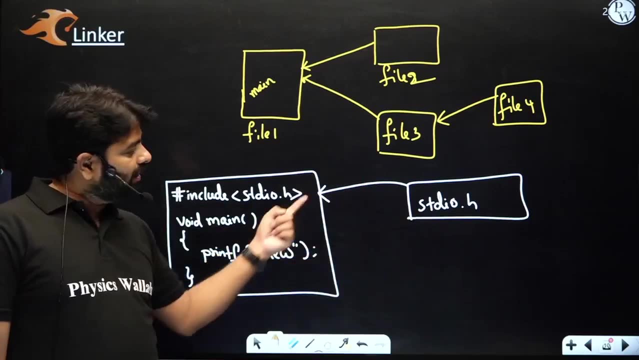 is going to come into picture here. right here, linker support is needed. first, pre-process: understand the statement and it. it. it informs the compiler: don't look at this code. linker is going to look at this code. somehow the printf is going to be resolved by the linker. 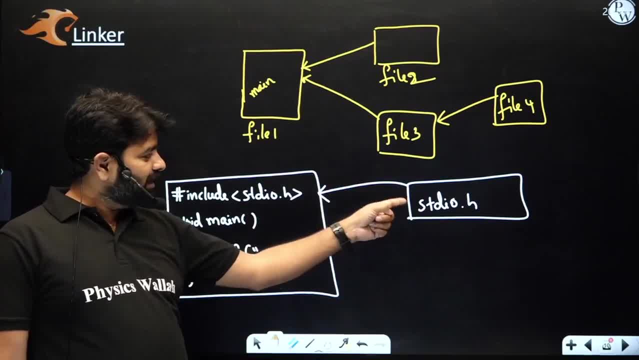 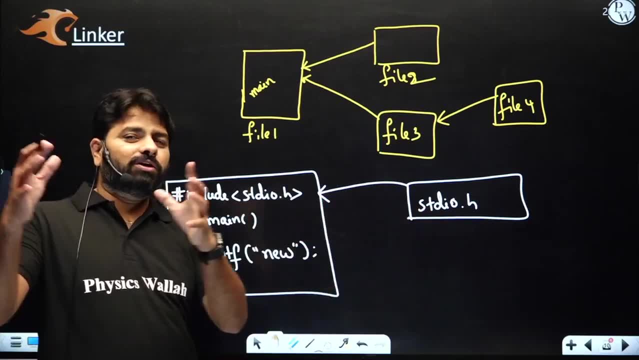 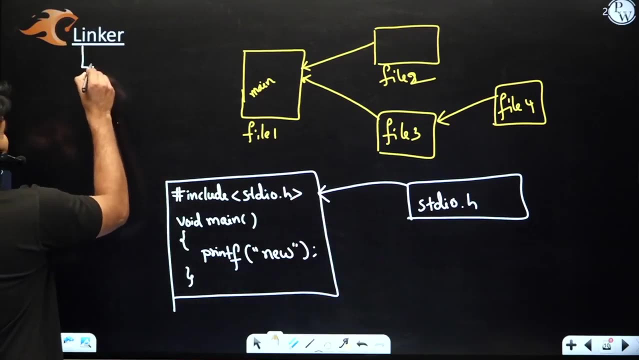 by looking at this reference, by looking at this reference, stdio dot h is linked to this file, so somehow the printf is going to look here. so the definition exists. it's going to be executed at runtime because result it resolved. so linker helps us, linker helps us it. 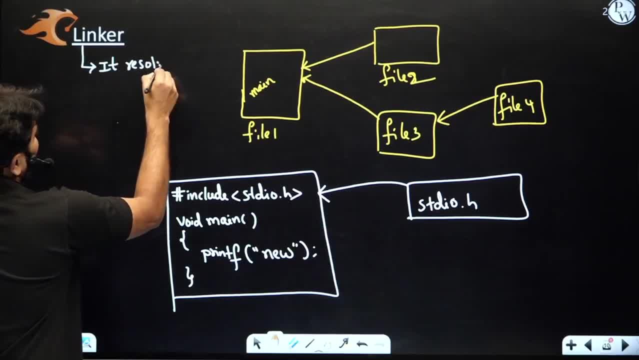 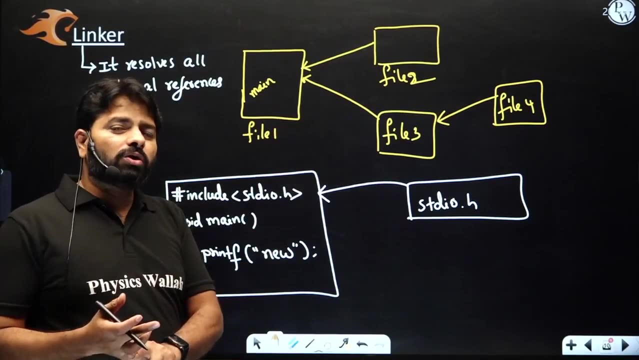 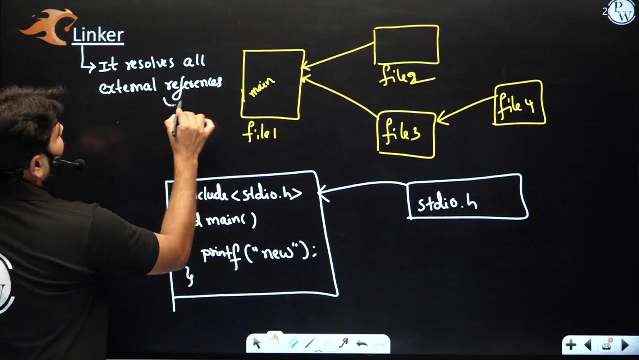 resolves all external references. all external references? what kind of references? mainly files. but why do you want files? because within the files you have the two things: either variables or functions. sometimes you refer external variables, then also you need a linker. so this references depends. it's files actually, but it 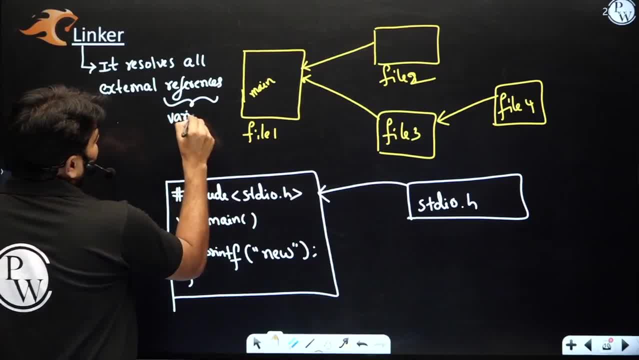 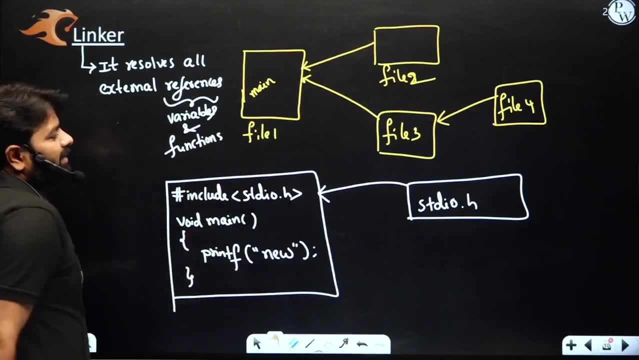 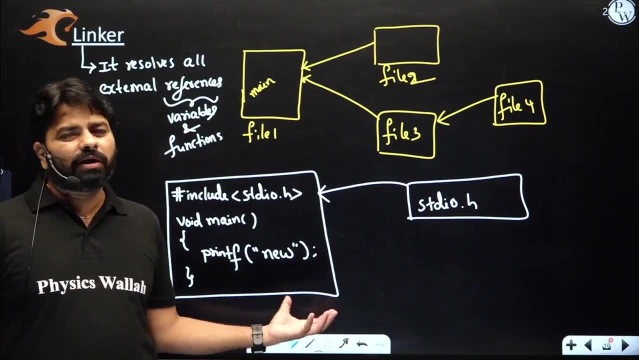 depends on variables and functions. both are going to be resolved by the linker. by the linker you can try your own program. basically, you know, as a beginner you always write a single program, but actually you can write many programs. you don't need to write a stdio dot h. you can write your own c program, you can. 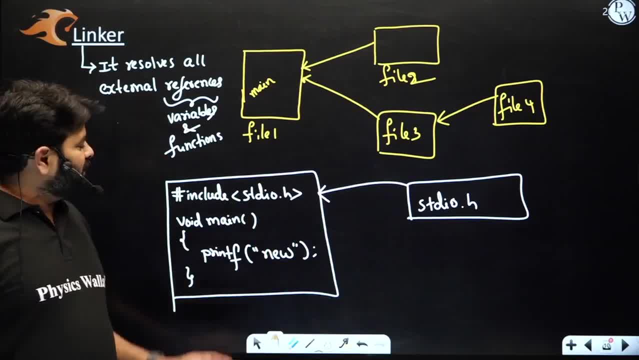 include here so that the linker is going to link that file and during execution, somehow it's going to be called because of the linker helps to understand where the printf exists or where your own user defined function exists. okay, so the linker is going to be linked to that file and during execution 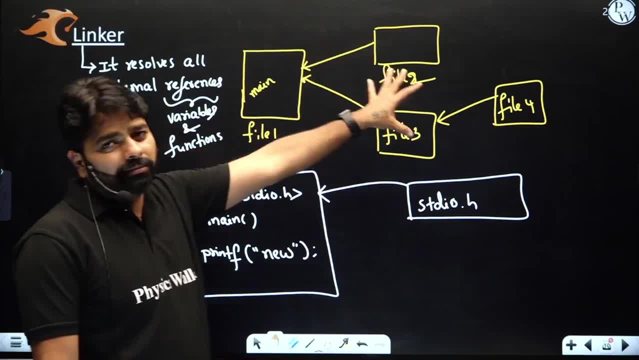 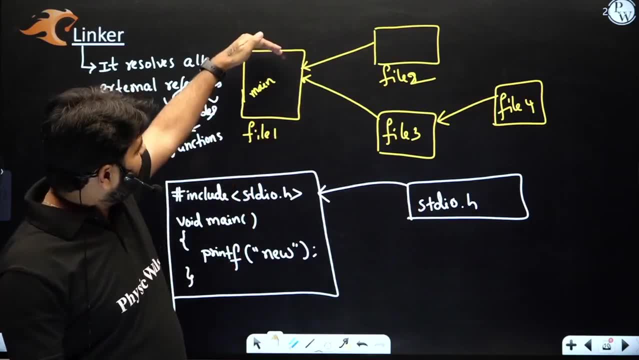 that file is going to be linked to that file. okay, so i will recommend to write many file, many programs, many c programs, and keep the main only in the main program where you want to start execution of the program. so while you're executing this program, many files are going to be. 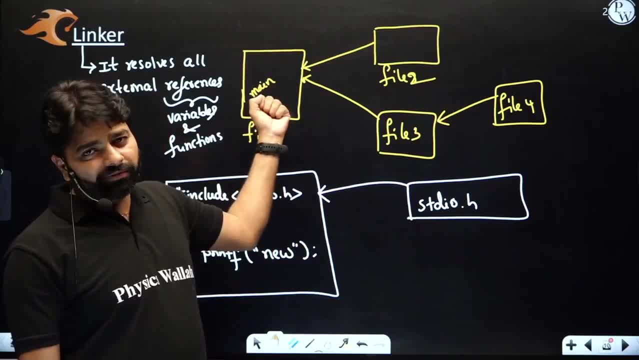 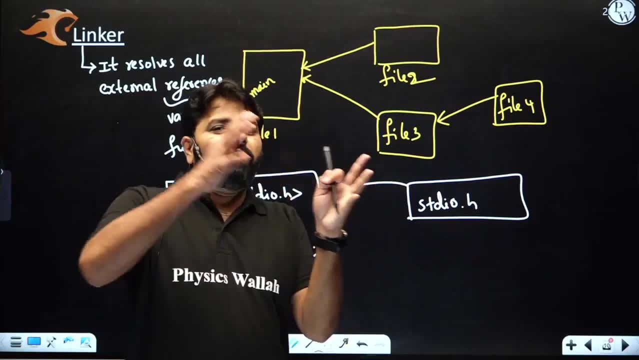 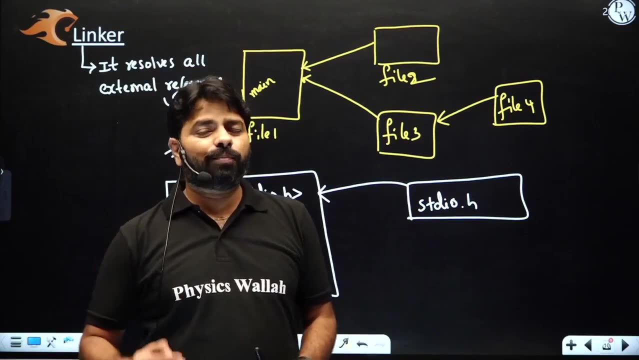 resolved or linked to this file. to understand the code that you have written in this file. okay, this is about the linker. linker. actually, what does? even though you have different programs? it will make the all the links flow as a single flow program so that when the operating sub starts executing, it looks like sequentially it is. 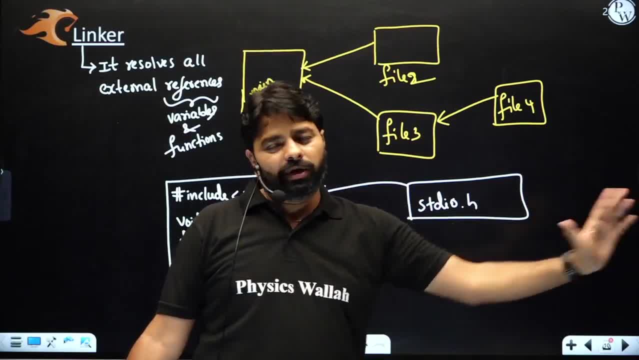 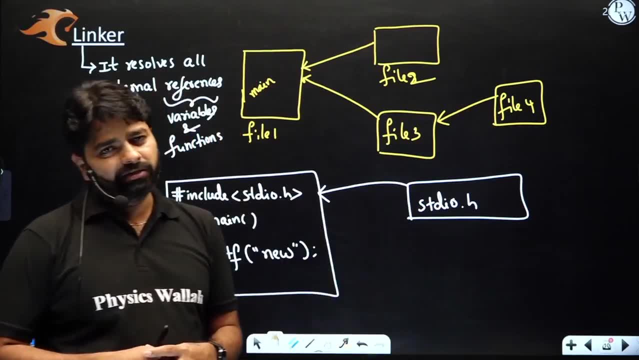 executing like it's starting. it just executing like one program. it will not execute like a different programs. as the linker already resolved all the external references okay. so instead of printf, it goes to somewhere, because you it might be providing the address here. it goes there and executes and comebacks this. 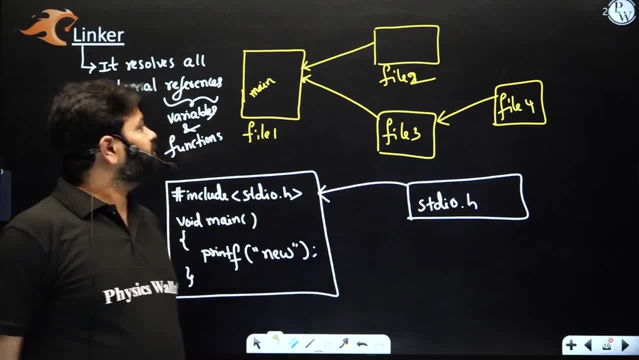 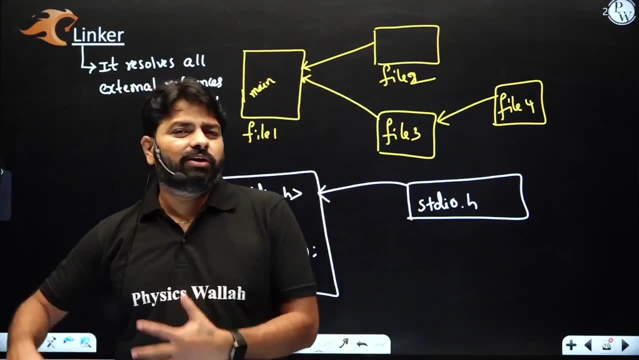 looks like simple function, jump and coming back. okay, it's about the linker. it's about the linker, but i'm not talking about the linker- all the places that we use in reality in operating system. okay, a linker is might be used in various places, but i'm only talking. 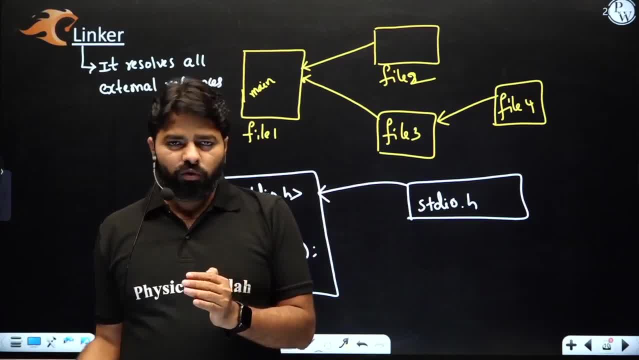 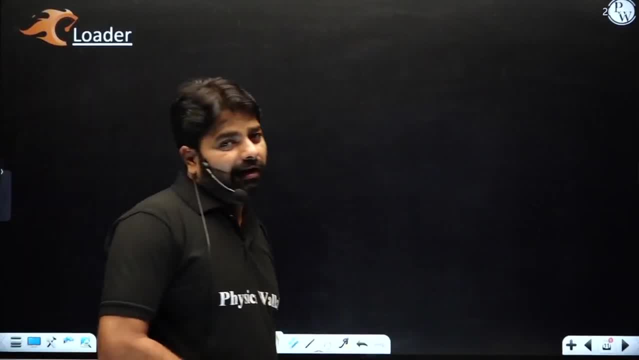 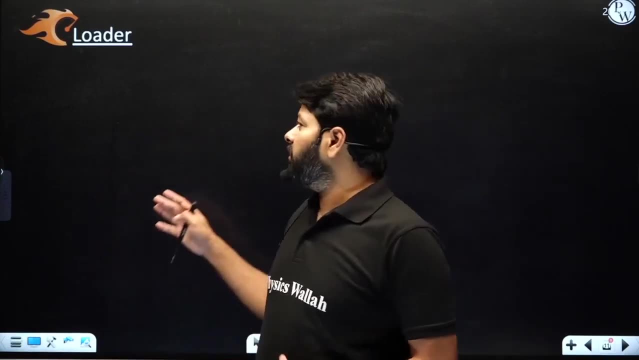 about in c program how the linker is invoked. okay. when it comes to implementation, you have again two types: static linker, dynamic linker. static loader- dynamic loader: okay, that you may learn in operating system or in some other subjects- really not much required in today's. a modern compiled design for the gate exam. 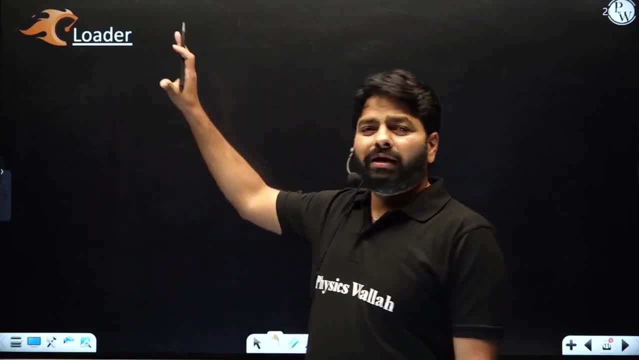 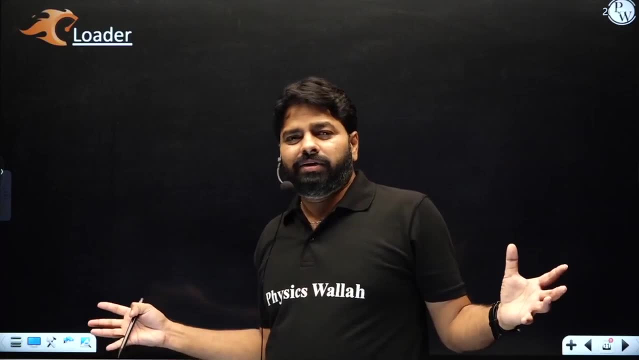 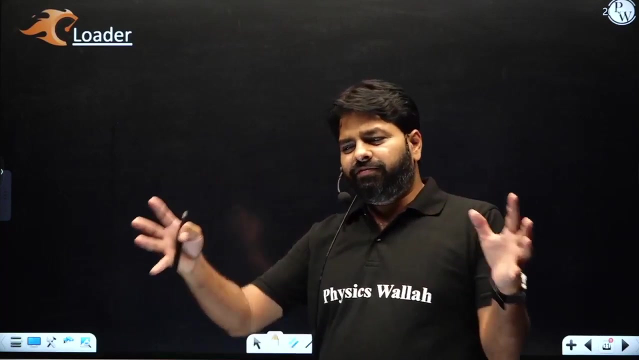 loader again. uh, you know the loader as a very big is. it's a very big topic in operating system and we are not talking about all types of loaders, right, we are talking about how the c program takes the help of loader. okay, here you have different files. 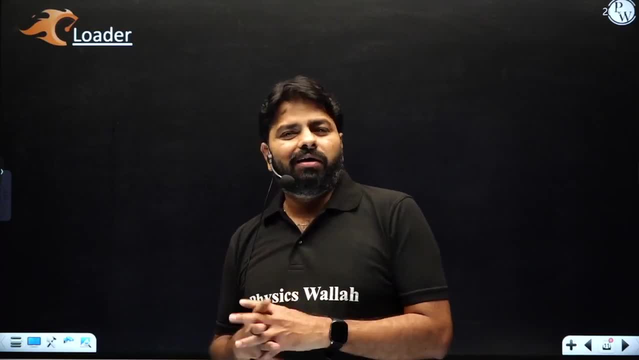 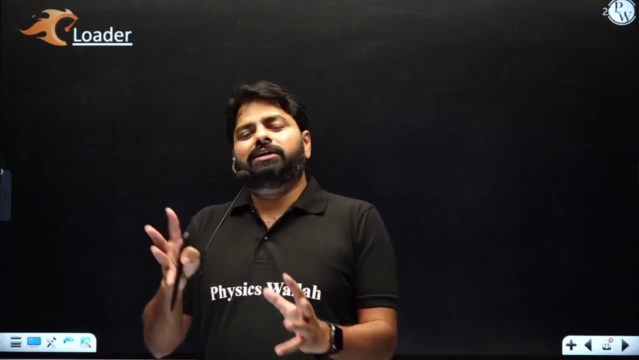 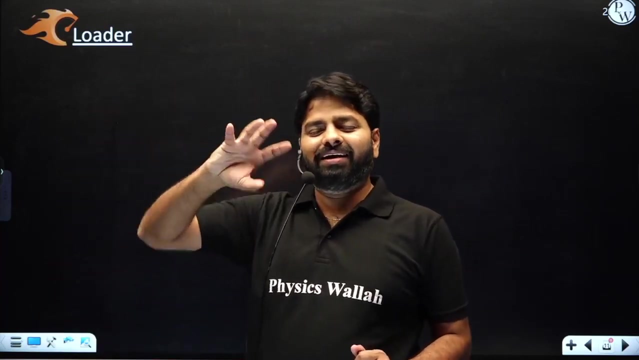 it need to be loaded right to link. so linker and loader need to be communicated somehow. so that is it- statically should be done or dynamically should be done- is going to be implemented according to the requirement. so both linker and leader, uh, so linker and loader, linker and loader need to be communicated together. 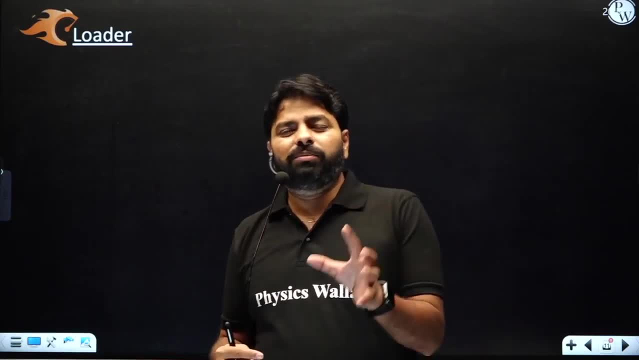 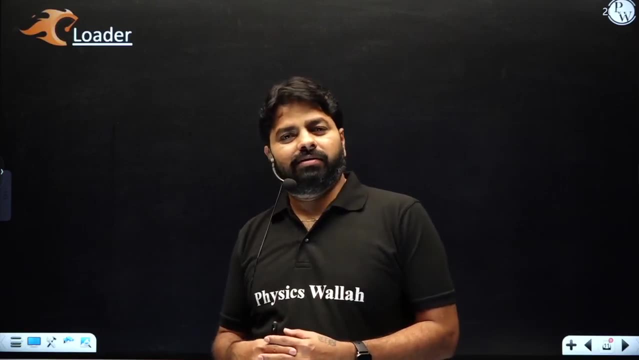 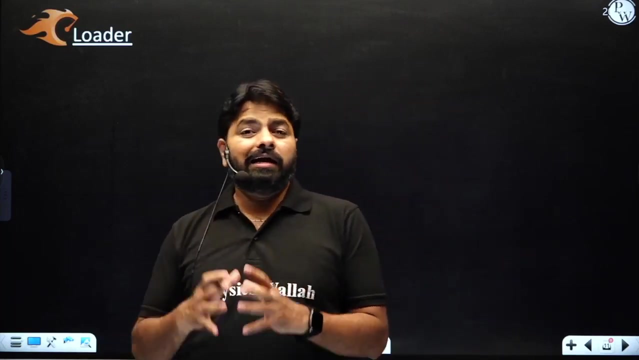 or need to be involved together to understand: do you want to implement static loader or dynamic loader? if the loader is static, then linker. you can implement very simple: either statically or dynamically, because that is already known right. and suppose a linker linker want to be static, then loader has to be static. why? because linker is static means it need. 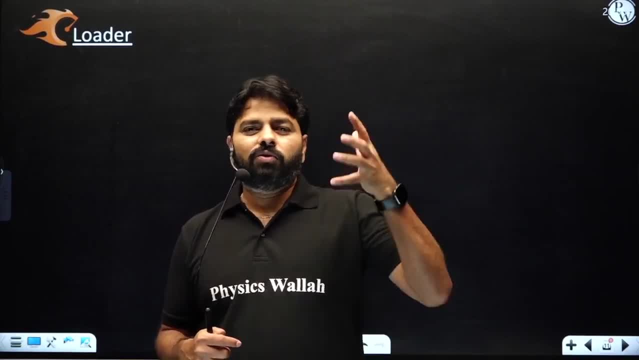 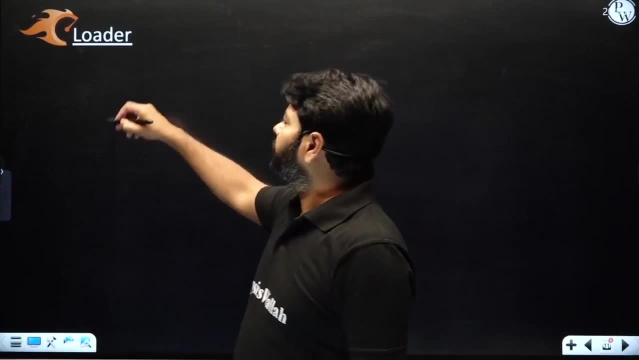 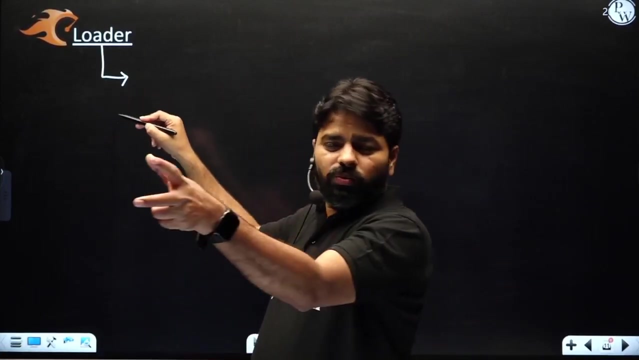 to resolve before execution. if you want resolve, you need addresses. if you want addresses, loader has to come into picture. so many many uh relations are there. okay, now loader. what do you mean by loader here? i told you its main purpose in the conversion of c program high level to low level. 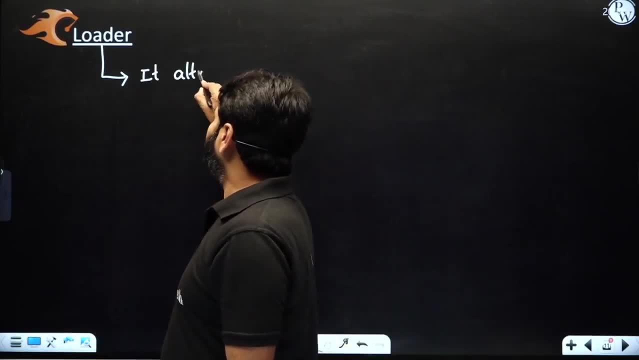 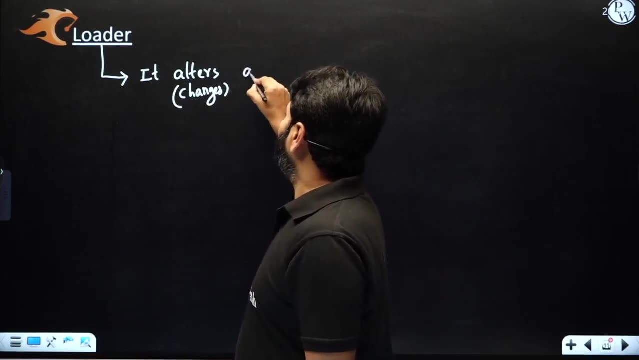 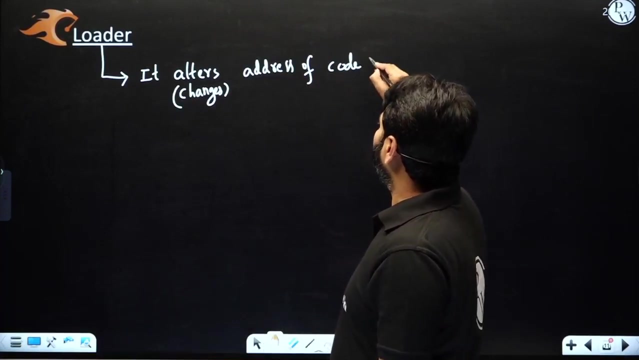 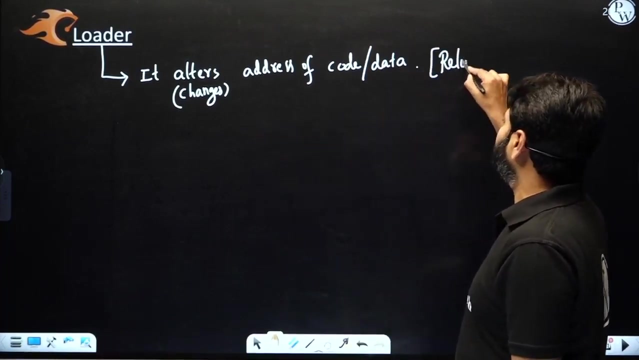 it's going to alter. it alters or changes. it's going to alter. it, alters or changes. it's going to alter. it alters or changes address of code or data whenever necessary. address of code or address of data or data. this is called as relocation. what is this called as relocation? it means 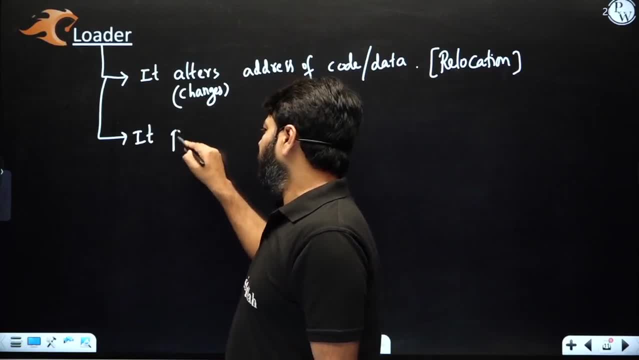 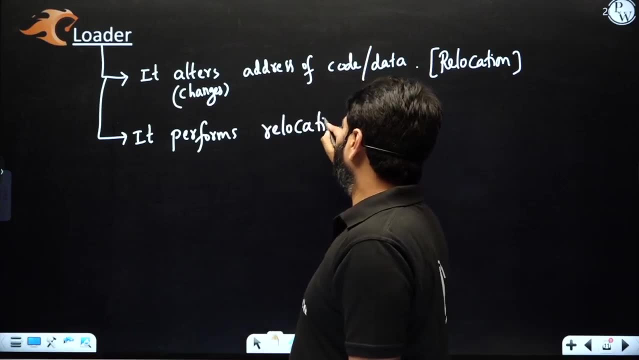 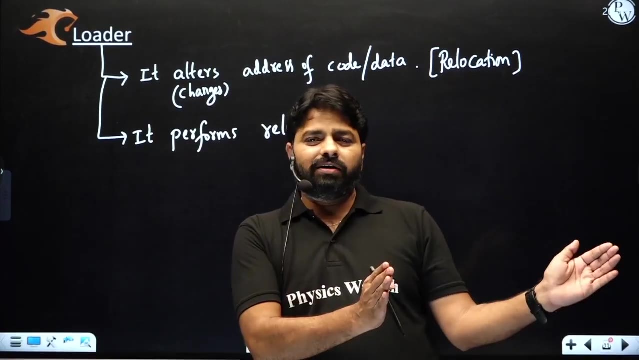 it performs simply. you can write the same line another way: it performs relocation. it does relocation. what is relocation? nothing but altering the addresses of the code or data. that's why i told the instruction should be stored somewhere and the data should be stored in somewhere in the main memory. so for both of them you need memory locations. 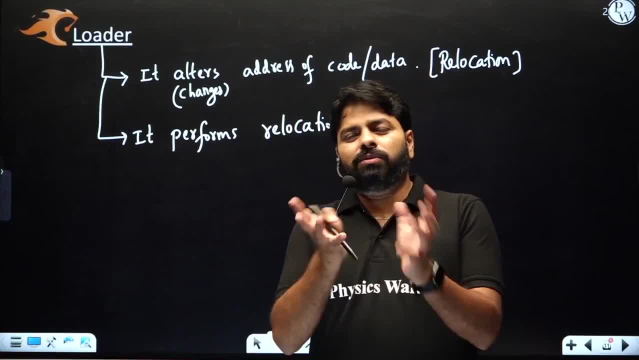 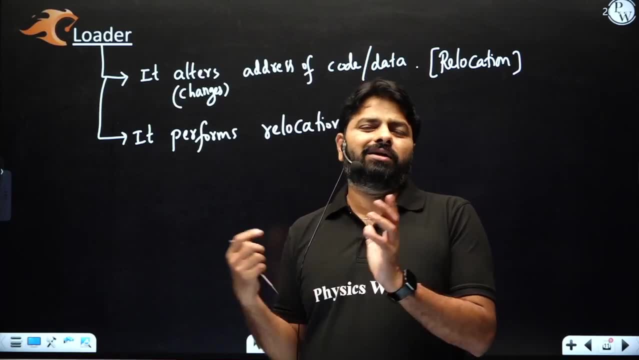 but what the compiler and assembler did is assume some address and converted, but that may not be available at runtime. right, the compiled code may be run. maybe you may run on the same time day or maybe another day even on the same day. it may not be at the same time. right, you may run. 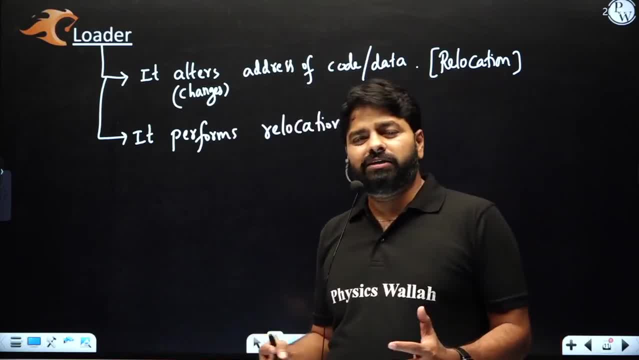 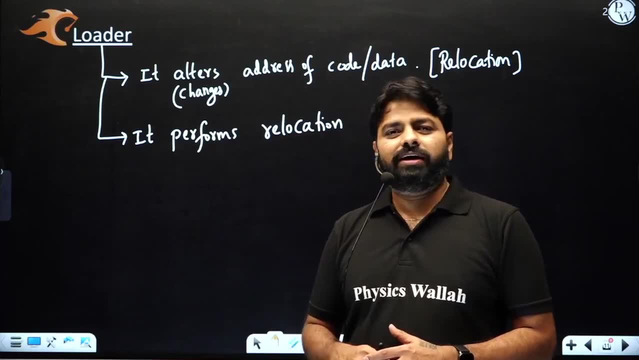 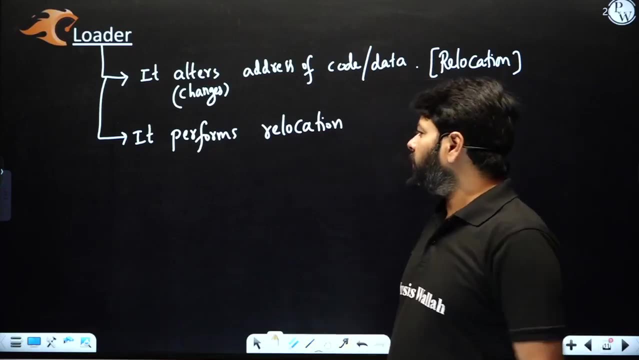 after a few seconds, but every second or every few seconds the snapshot of the main memory could be changed because of you exit and start many programs right. so that's why the loader and linker really needed to compile and run the code. so this is about the loader and it's about all uh components. 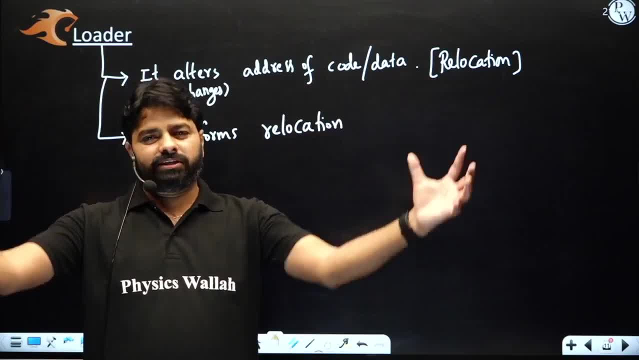 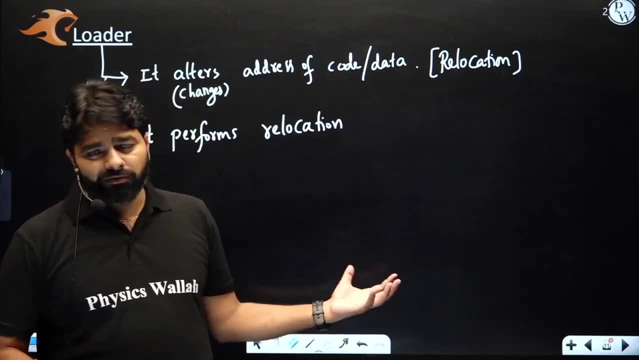 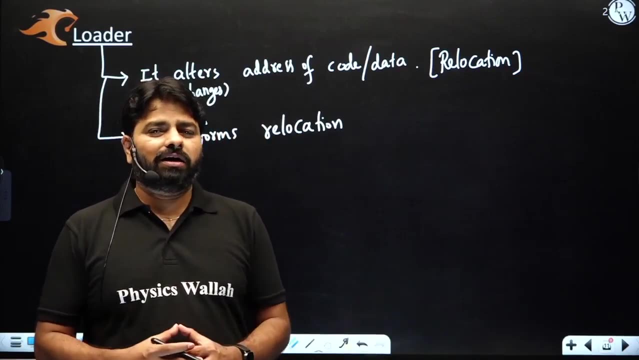 that we have seen within the language processing system, from how high level, from high level to low level, how the program is converted and what are the components are involved: pre-processor, compiler, assembler, linker, loader- all comes into picture, but all these things are just treated like a 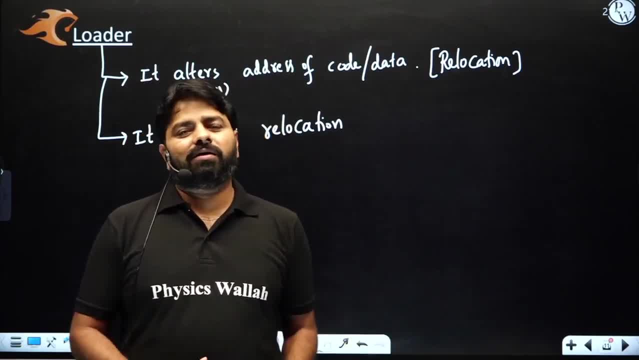 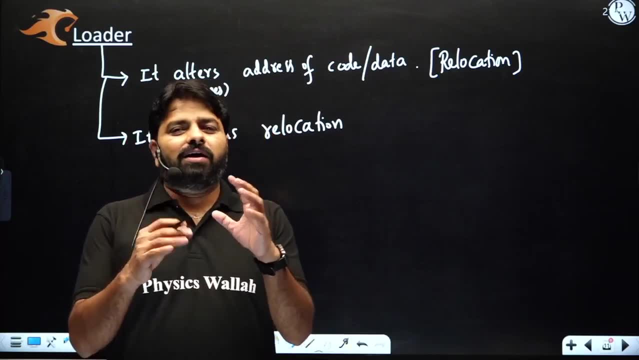 single program that you are not aware of it. just you type or click on build and run button, it's going to happen all the things. okay, you will only see how to enter an input and how to get an output. that's it. uh, the whole logic is going to be executed. 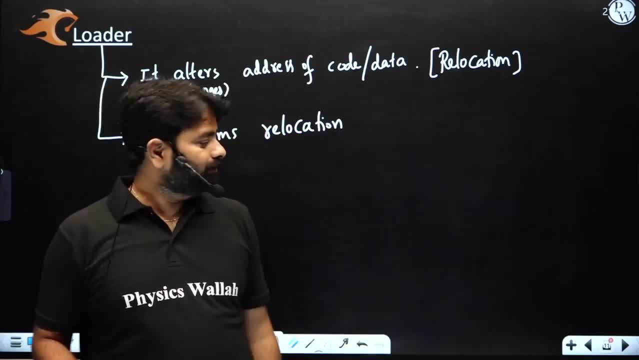 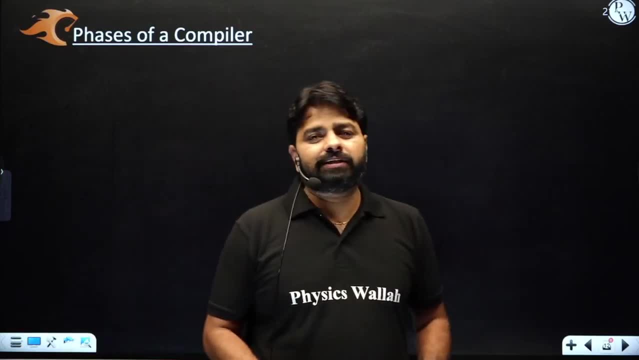 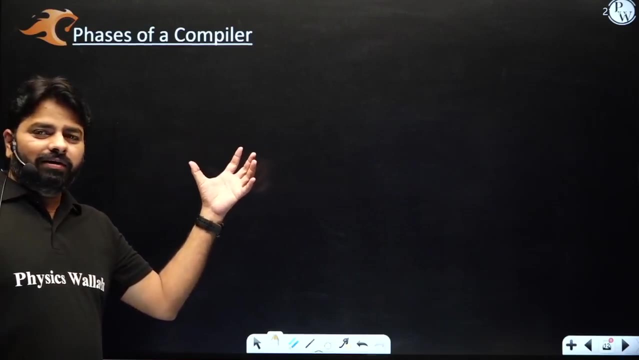 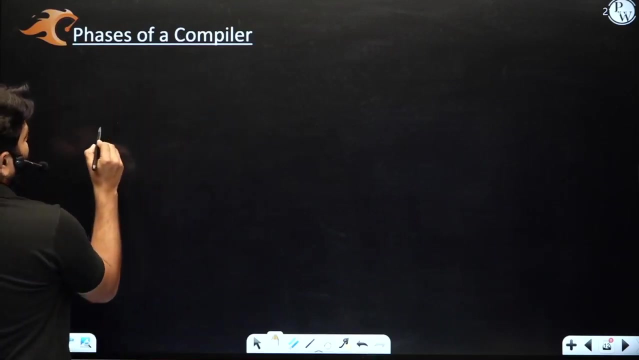 because this translation done in background. okay, now we'll move to the phases of a compiler. phases of a compiler. i've already disclosed that. how many phases are there? let me show them in sequence. you know, when you give a c program to the compiler, the first phase which comes into the picture is: 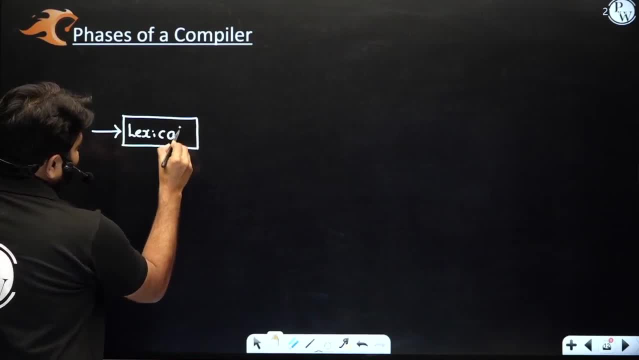 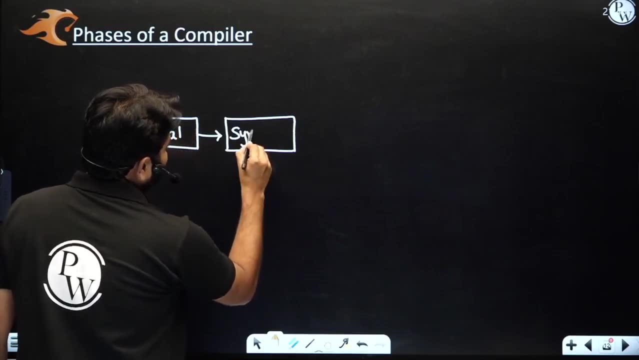 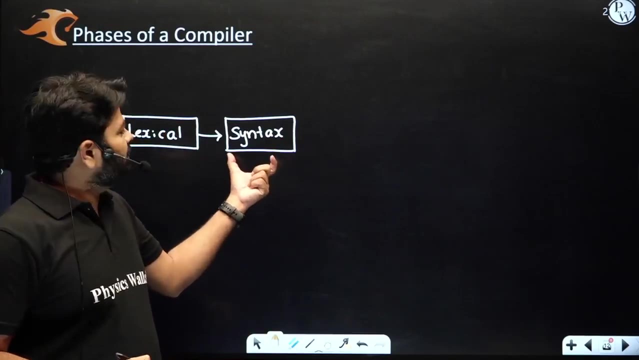 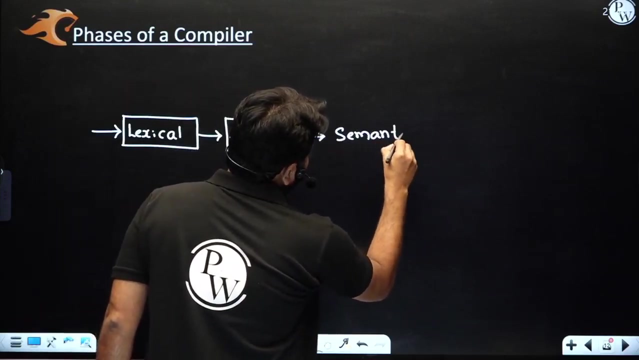 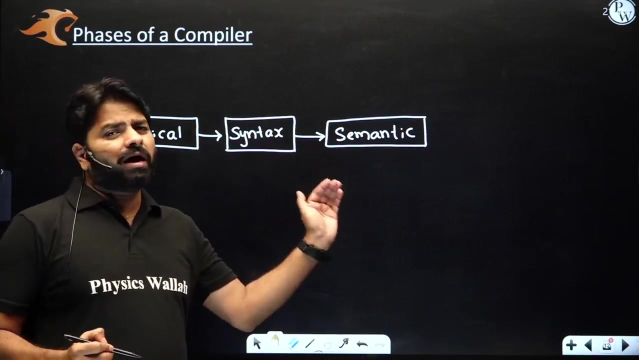 lexical phase, also called as lexical analysis. then you have syntax. this phase is very, very important for the exam point of view. we spend a lot of time here than any other phase. then you will have semantic analysis or semantic phase. these three phases are our analysis phases. then you have 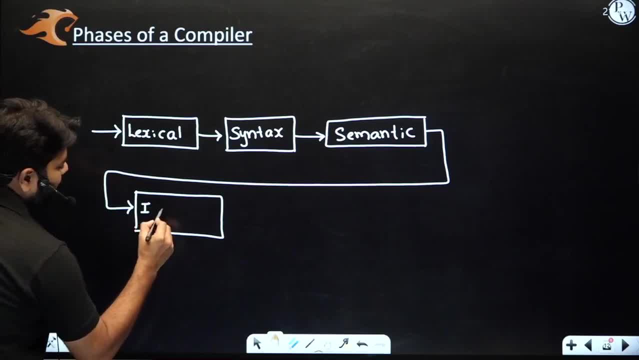 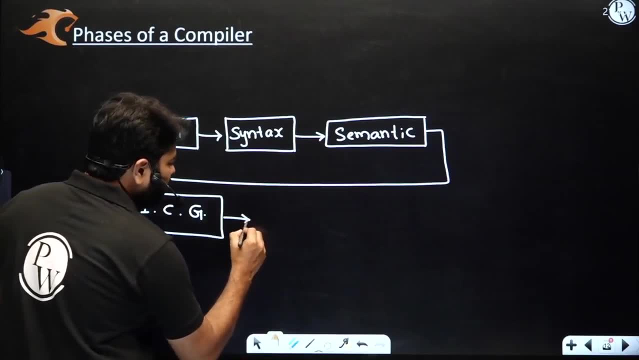 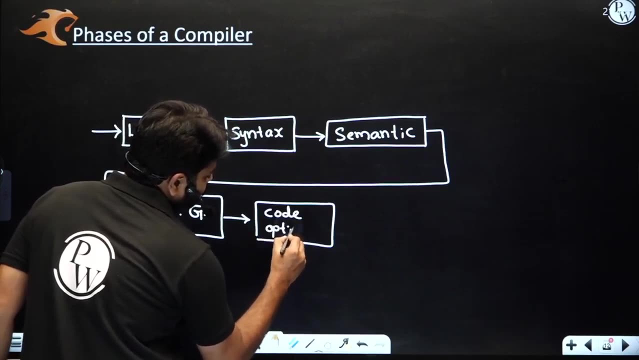 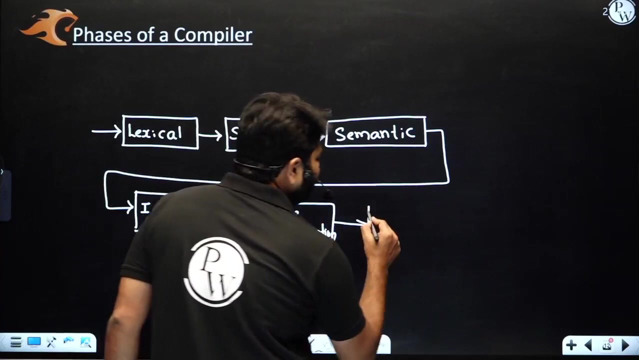 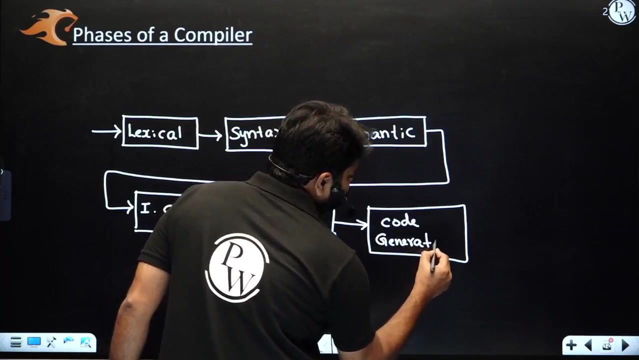 intermediate code generation. you can call it as icg, intermediate code generation or generator. then the output will be given to the code optimizer. or you can say code optimization, code optimization. then you will be having very important phase at the end. that's a code generator. this code generator is going to produce the assembly code. 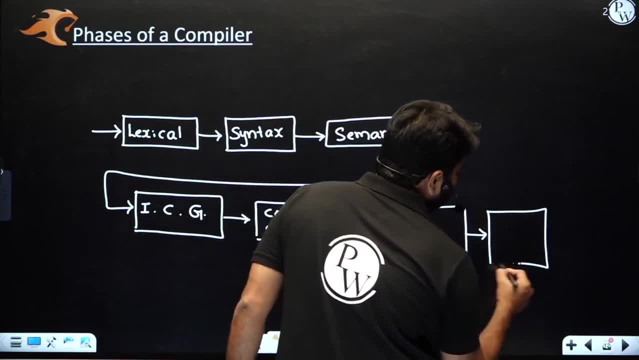 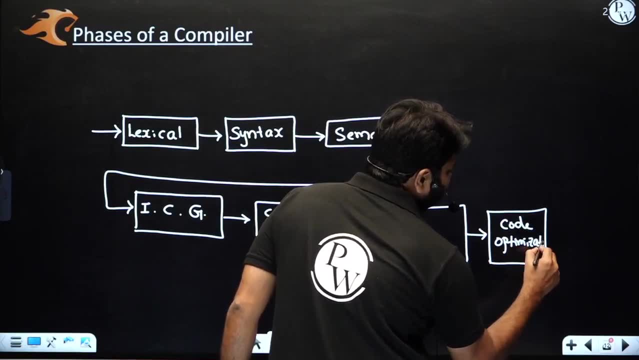 at the end. then, after the producing assembly code, in case, if you want to optimize the code, still have a browser code generator, solutions, code code generator, similarity accelerator, code ability, code, queda, all efendim code, still- you can apply this code optimization at assembly level. then finally we will get the optimized assembly code. now you can see the first. 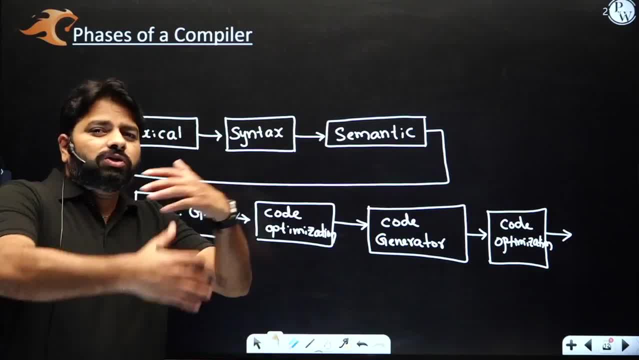 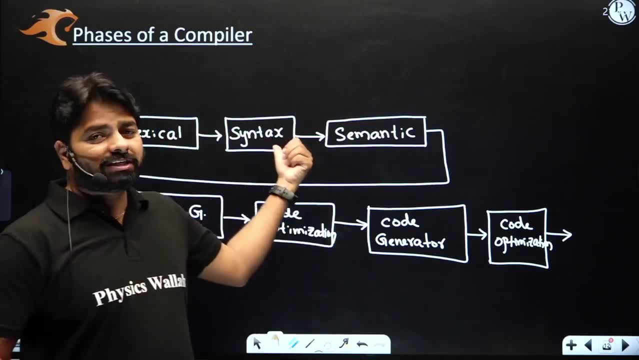 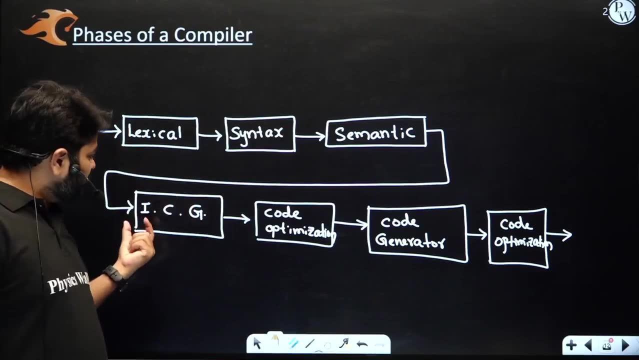 three phases are actually analyzers, that is, they are going to analyze the program rather than converting into another form. the whole C code is analyzed lexically, syntax, syntactically and semantically. here then the analyze, the C code, will be converted first time into intermediate code. then you can further optimize that. 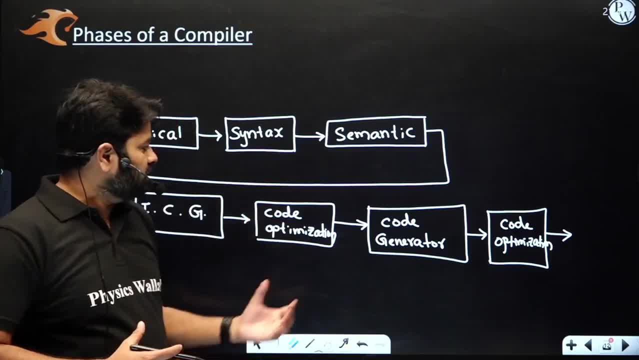 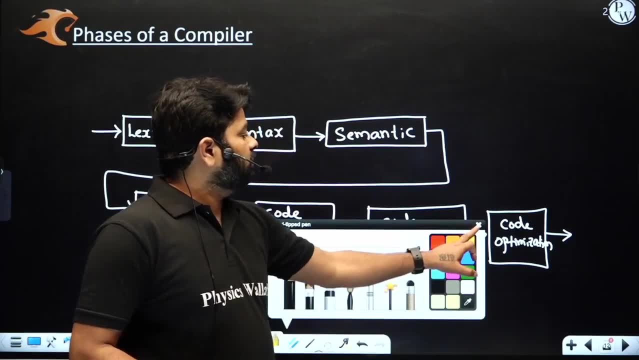 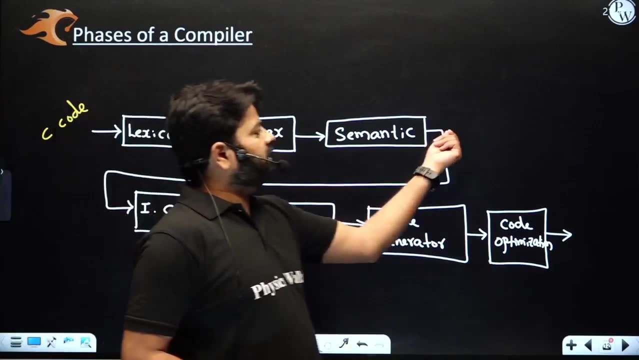 intermediate code to our to save your time and space. then later you convert into assembly code with the help of code generator. let me put all those conversions here. here you give C code and here it's important the analyze the C code. I can say: but rather than saying analyze C code, let me produce the. 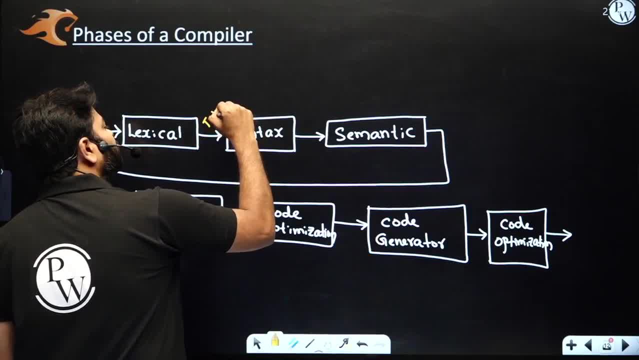 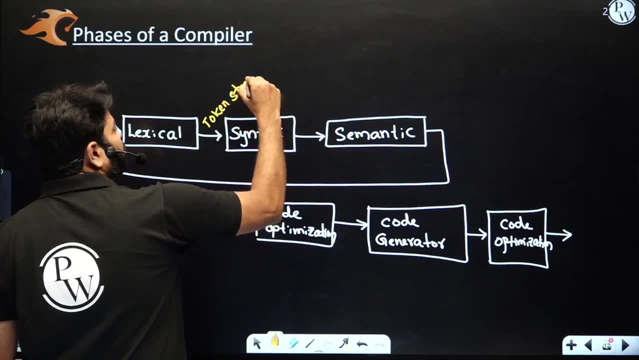 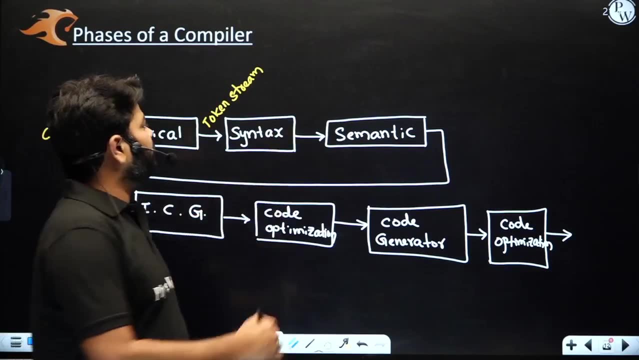 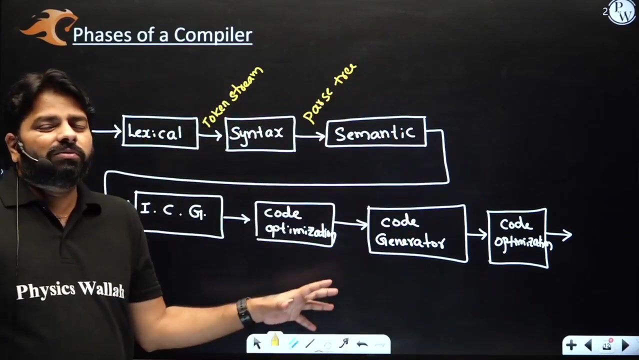 uh, sequence of you know the conversions here: token stream or sequence of tokens. token stream or sequence of tokens, the whole program will be converted into a tokens sequence of tokens. then here let me say parse tree, the whole program, just it. we convert into simple parse tree, which which will help verify the syntax. 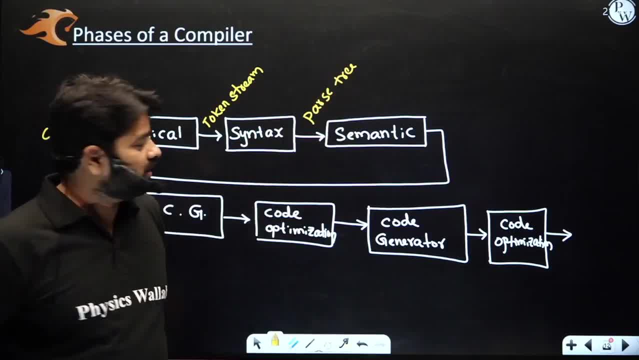 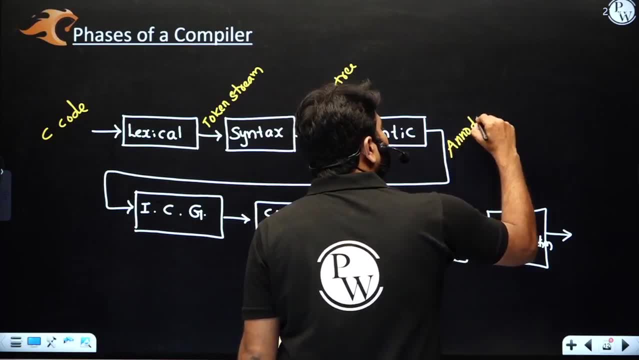 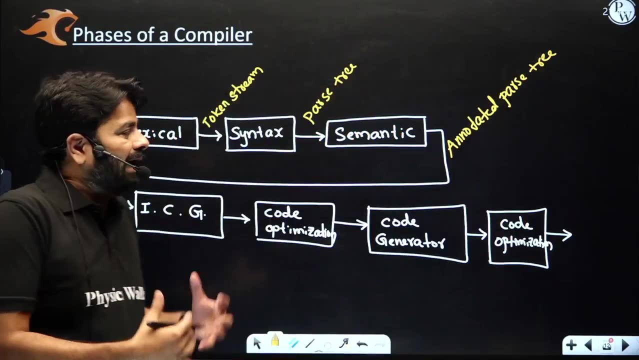 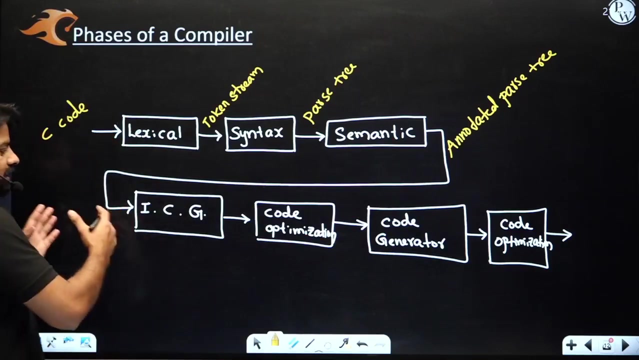 there is. there is no syntax error. it will produce the pass tree, then semantic. what is the semantic? it's going to produce something like annotated parse tree, annotated parse tree. this annotated parse tree will have the semantics or translations or actions within that parse tree, which is decorated parse tree, and the intermediate code generator is going to produce in. 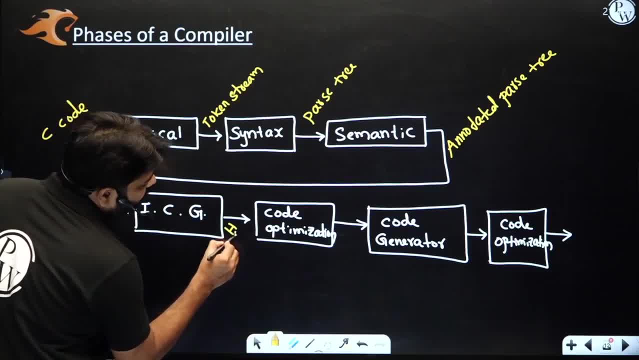 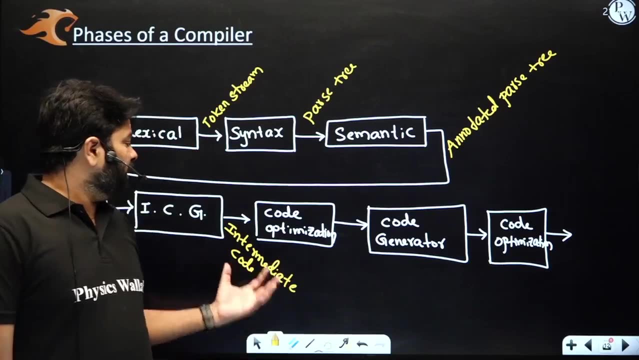 intermediate form. here this intermediate form could be represented. I'm just saying intermediate code, but this intermediate code can be syntax tree or could be three address code, could be ssa code and could be directed a cyclic graph. there are many intermediate code representations we'll be learning there. 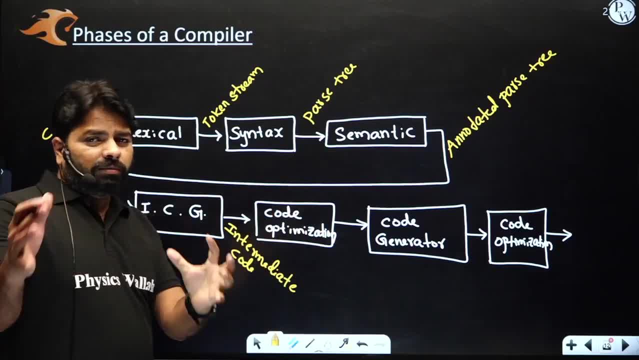 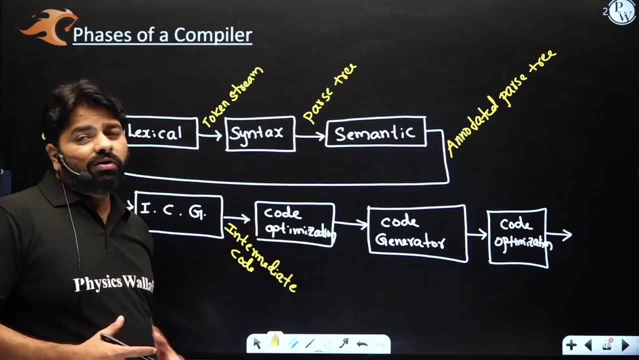 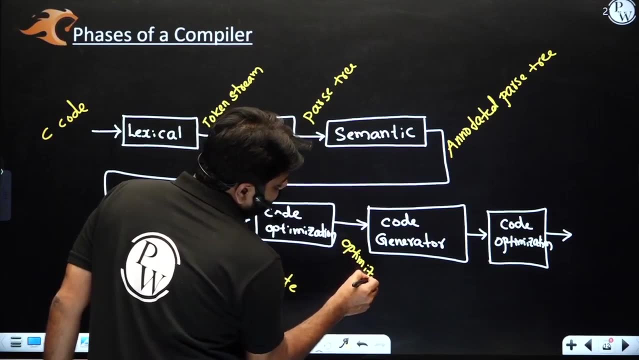 by taking this intermediate code we can further optimize and you may reduce the number of lines, or you may reduce, or you may produce another intermediate code which can save your time or space. so this one is again intermediate code but if possible it will produce optimized version of the. 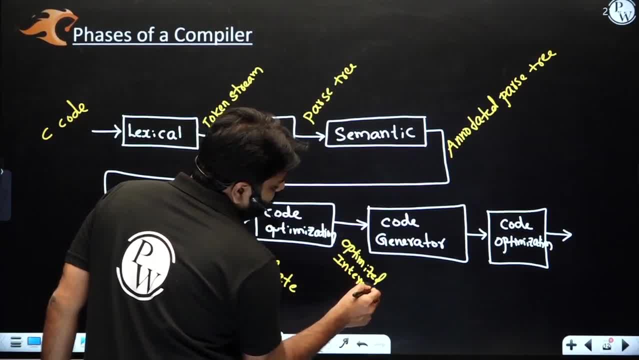 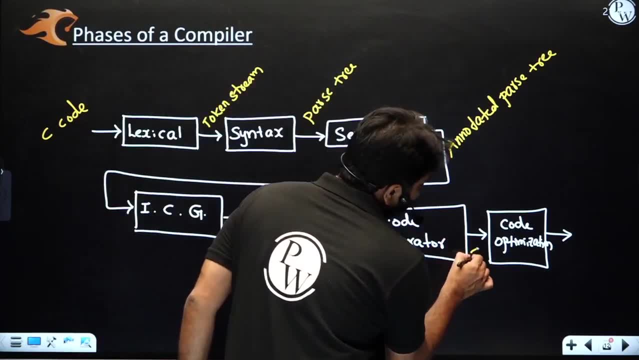 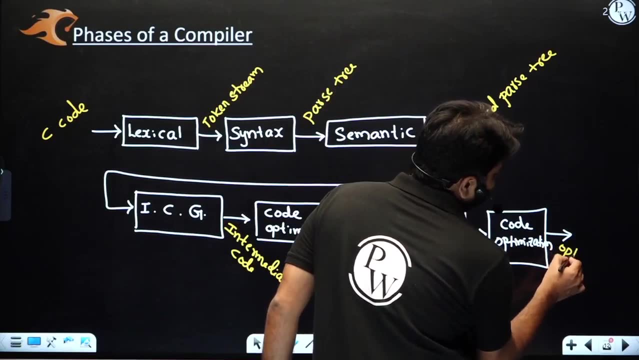 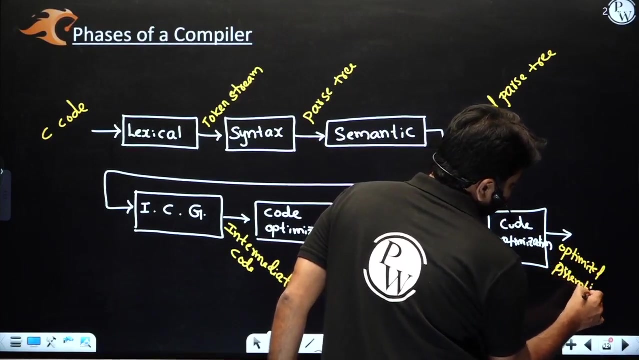 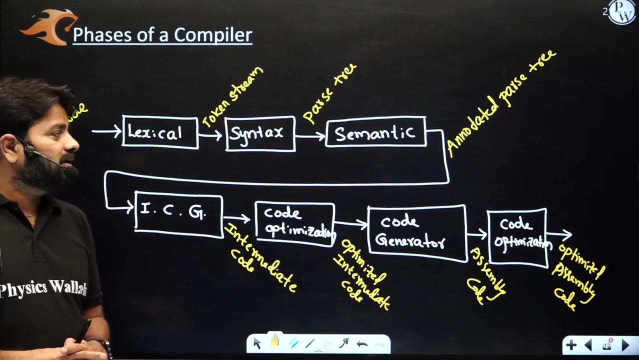 intermediate code. if it is not possible, it will produce the same intermediate code and this intermediate code will be converted into assembly code. first time here: assembly code and this assembly code. if possible, it will convert into the better version of the assembly code. this is how all the phases of the compiler are going to help us here, and let me help you. 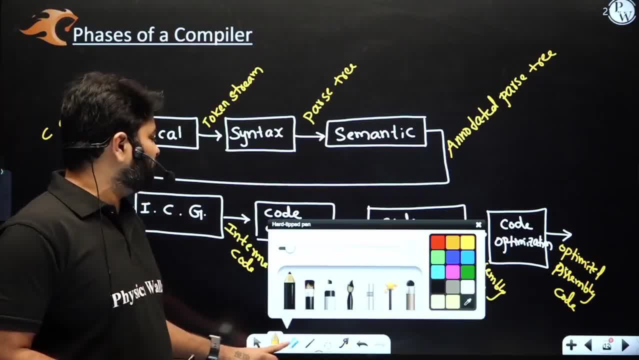 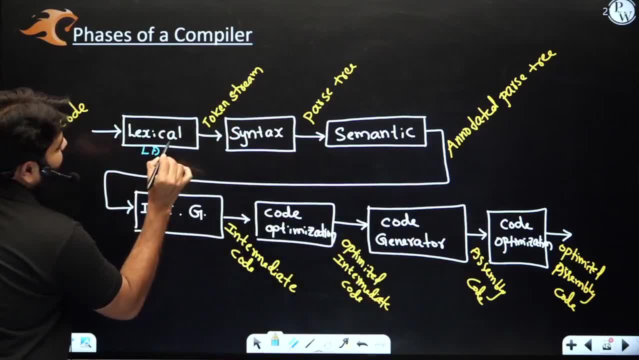 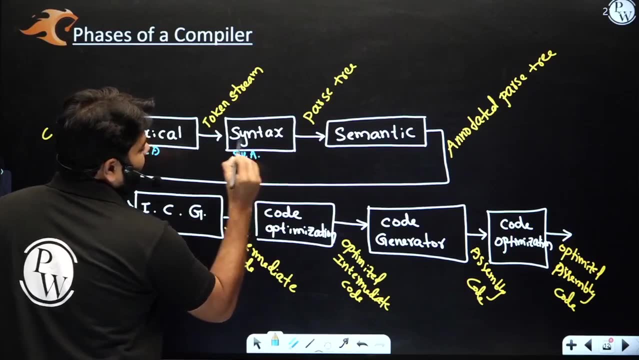 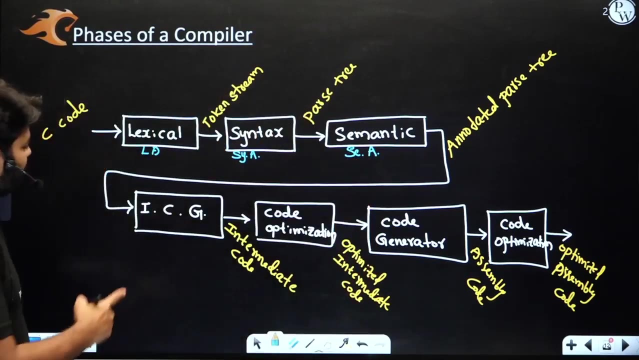 the six phases. okay, i'm going to use some short names, because every time writing the old name is difficult. right, the lexical analysis. i will use, let's say, l a lexical analysis. okay, syntax analysis. i'll just write s y a syntax analysis. semantic analysis. let me write s e a. that's a semantic analysis. then icg: intermediate code generator and code. 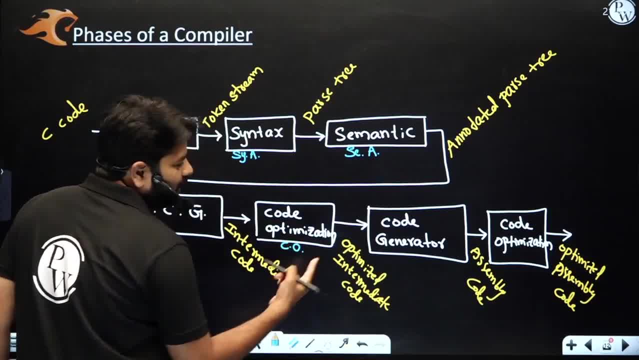 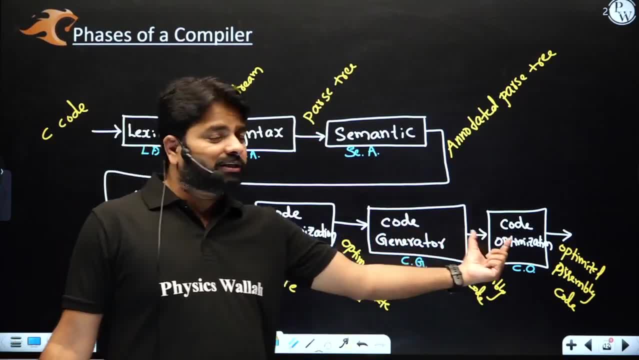 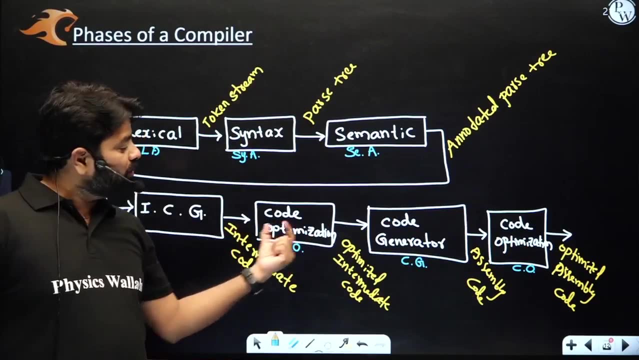 optimization. it's a ceo and it is code generator and it's another ceo. but these two different code optimizers, optimizations, even though theoretically you will have the same similar concepts. but this code optimization takes intermediate code, produces intermediate code. but this core optimization takes assembly code and produces assembly code. that means both code processes and code optimization. 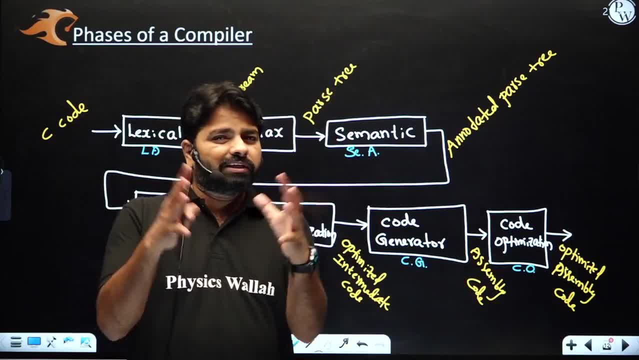 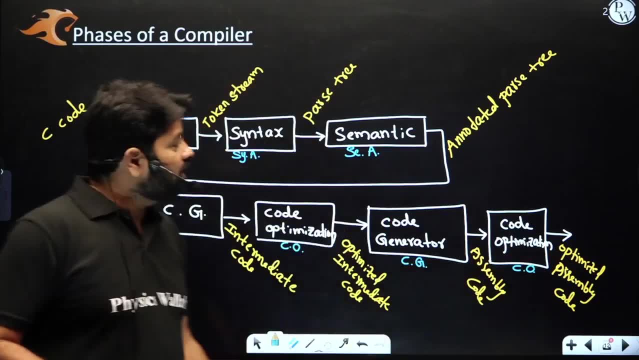 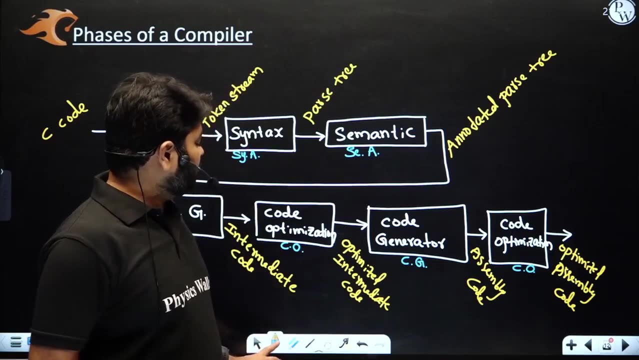 programs are different, even these two programs having the same name: code optimization. code optimization, but code optimization on intermediate code, this code optimization on assembly code. okay, so this phases I am going to put into another way or another form so that you will be having some other introduction. 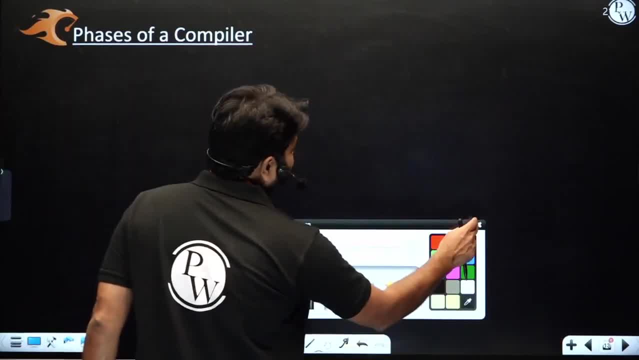 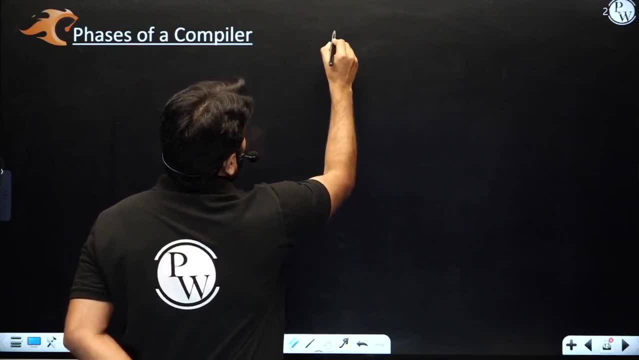 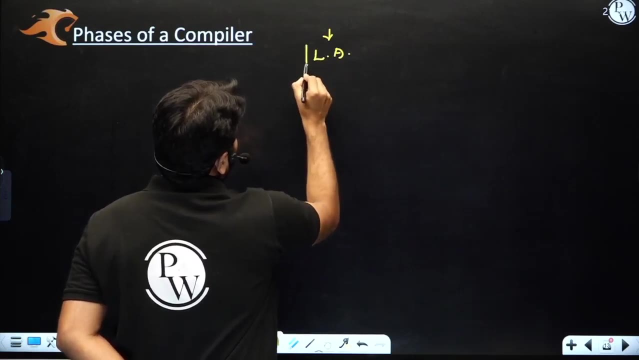 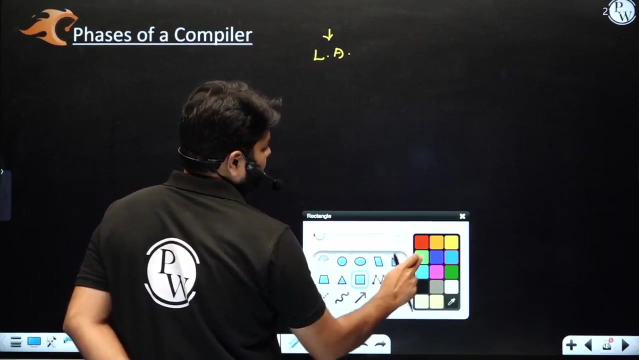 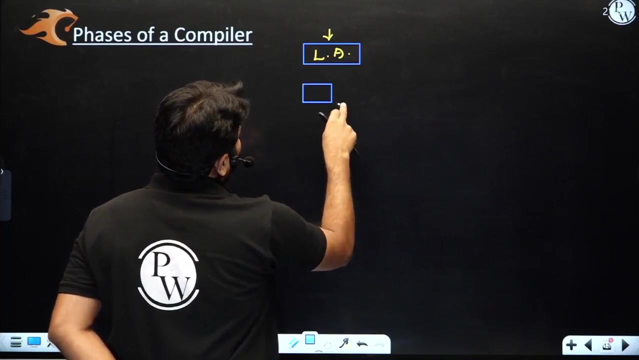 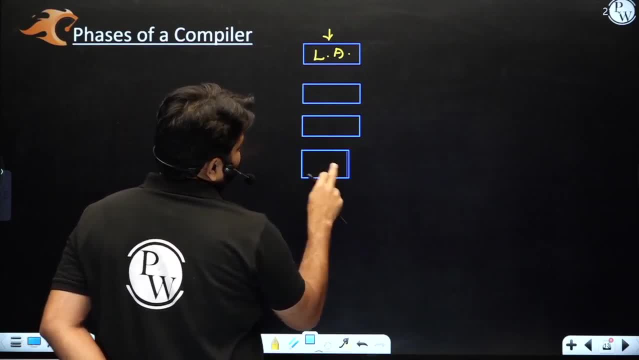 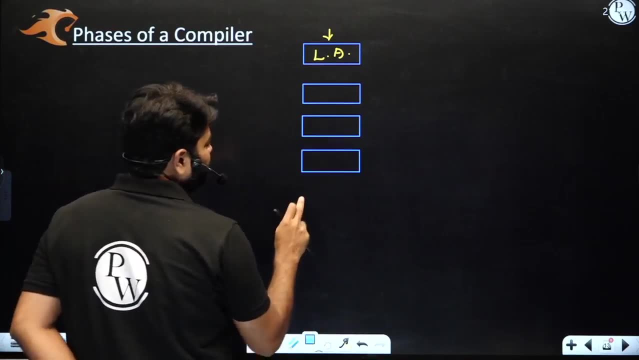 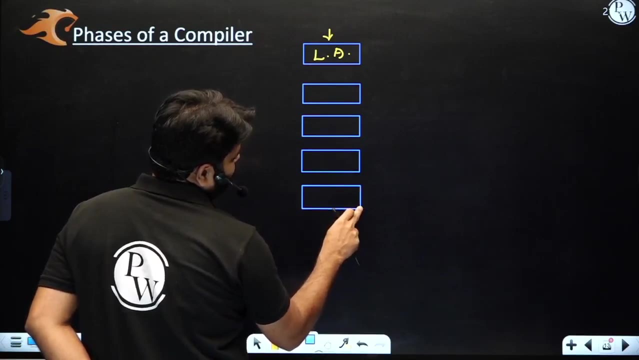 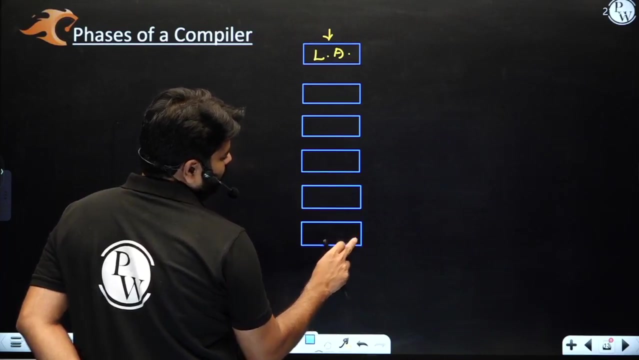 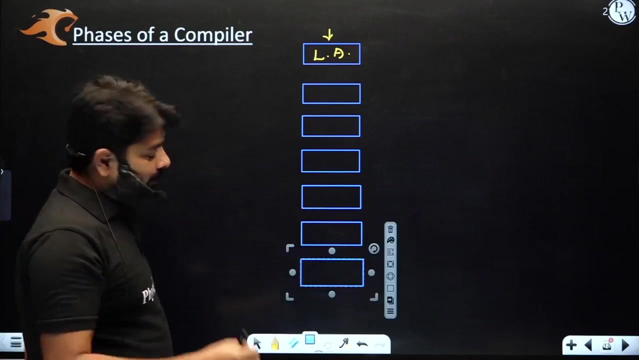 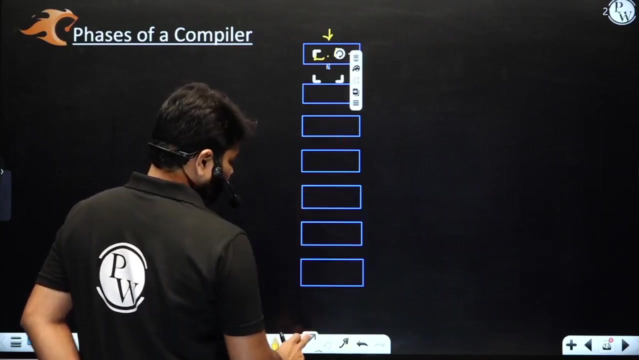 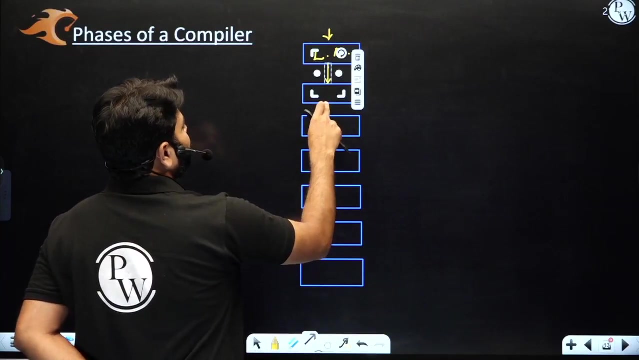 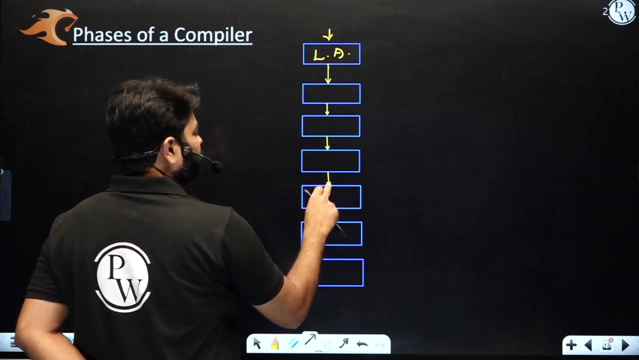 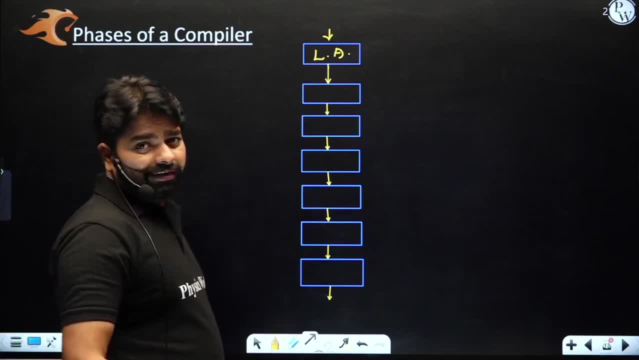 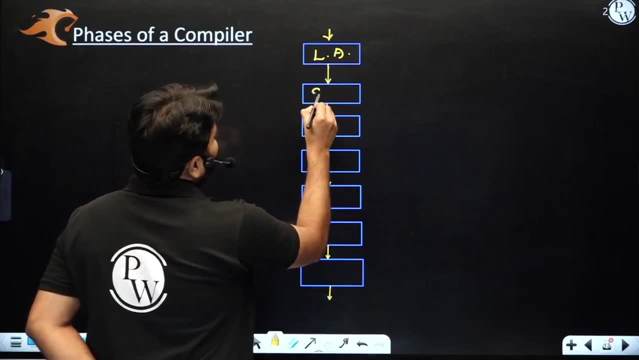 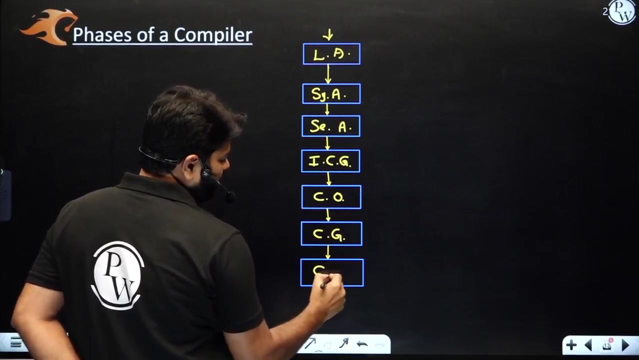 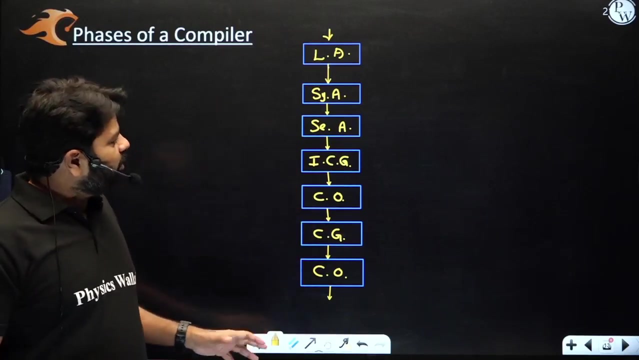 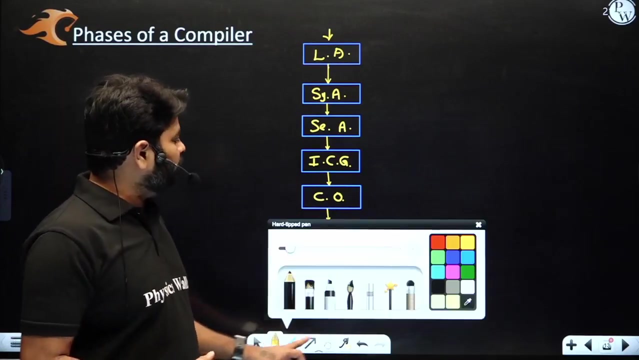 the final outcomes: atur, special code. here what you have: syntax analysis and semantic analysis, intermediate code generator or generation, code optimization, code generator and code optimization. sorry, now there are, right, different phases. there are different phases. we are going to use in our two ways, two ways here: analyzers and 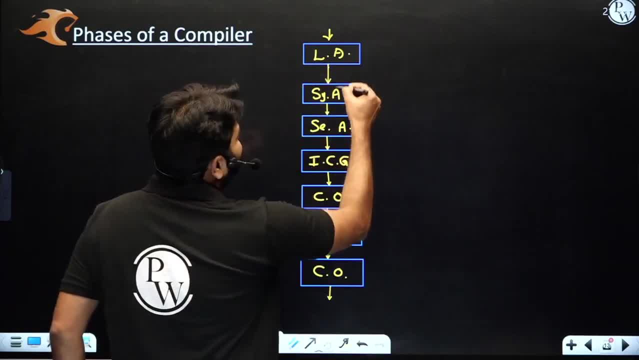 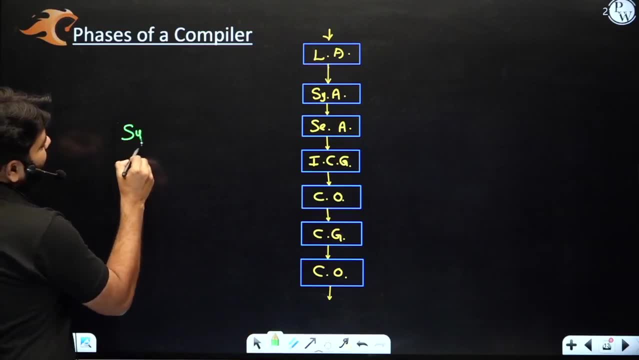 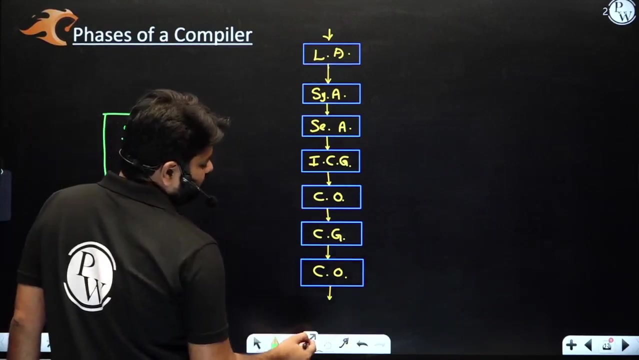 synthesizers. what we call the first three are analyzers, but when you look at the whole compiler, whether it is analyzer or synthesizer, all of them are going to interact with one special data structure to understand the program. to understand the program, if you look at lexical analysis, has to interact with the symbol table and 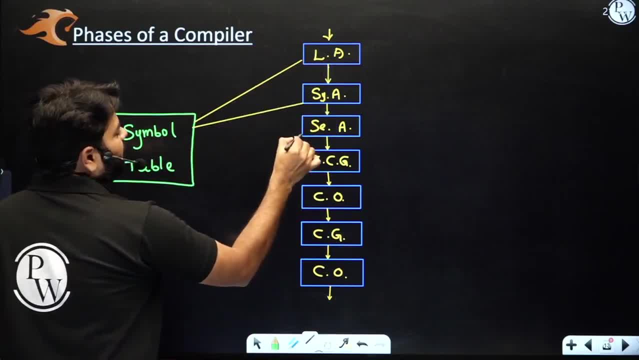 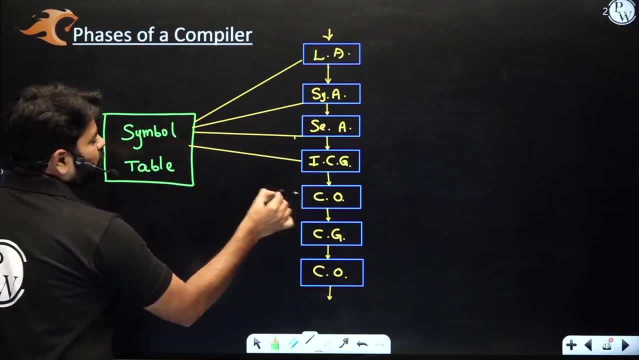 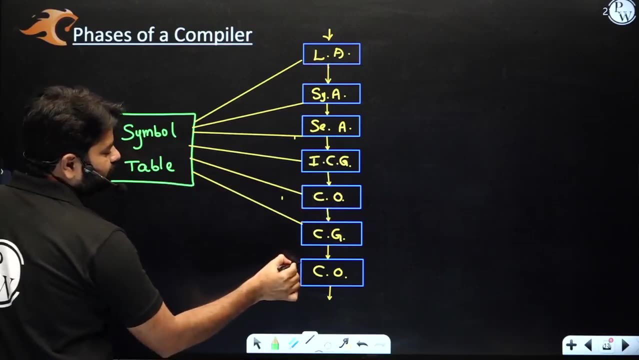 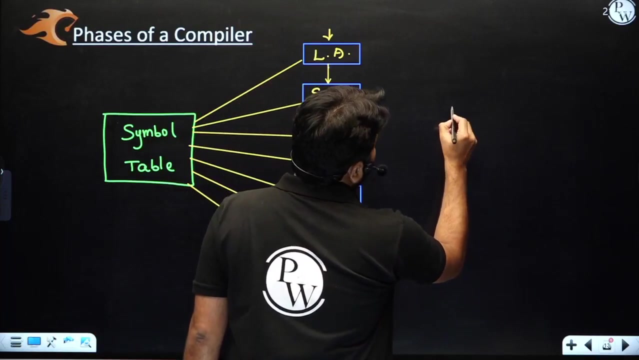 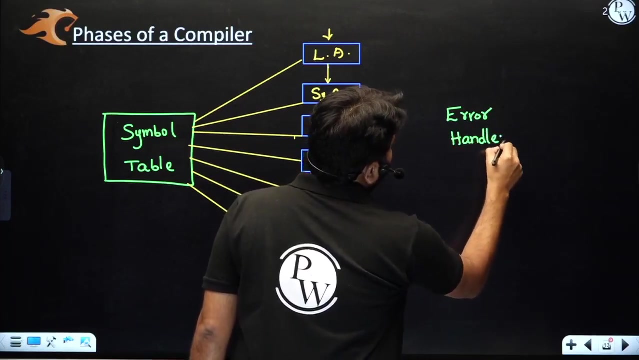 syntax analysis and then semantic analysis, intermediate, code generator, code optimization, code generator and code optimization. all the phases are going to be the same. to interact with the symbol table, we have the another one, which is error handler. this error might be produced at any stage or any phase of the compiler. all the phases are going to interact with. 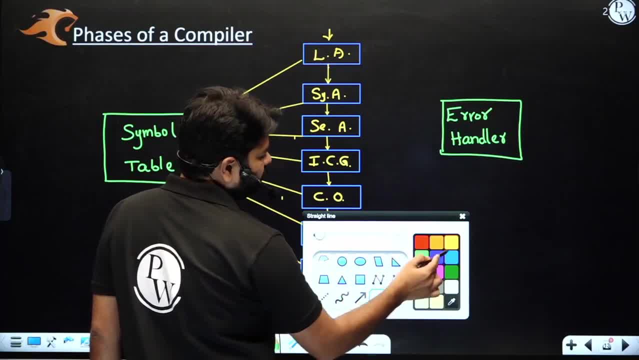 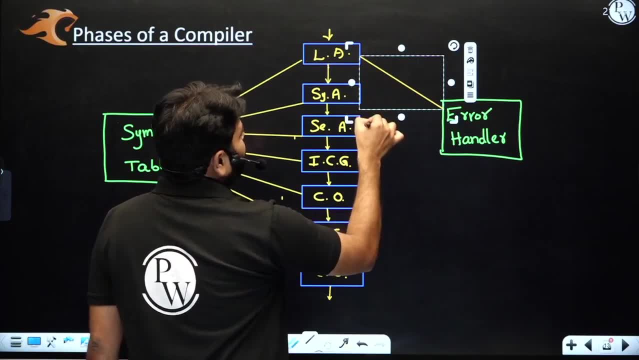 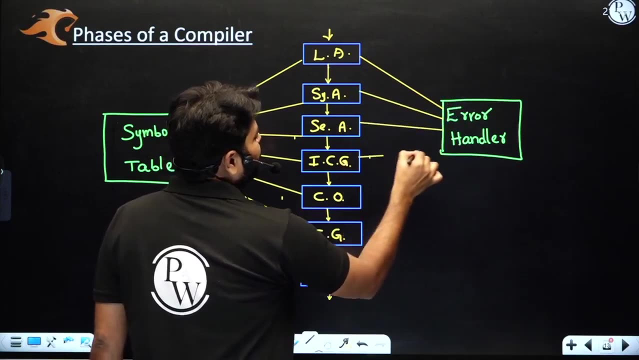 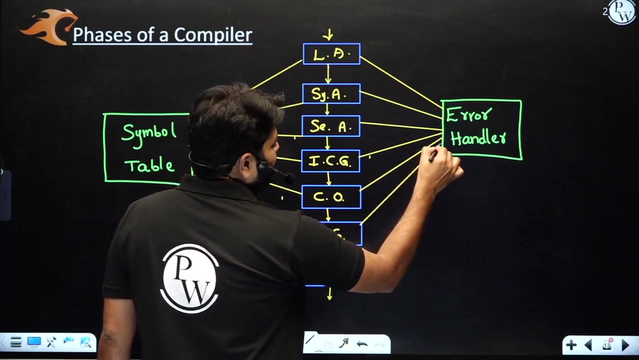 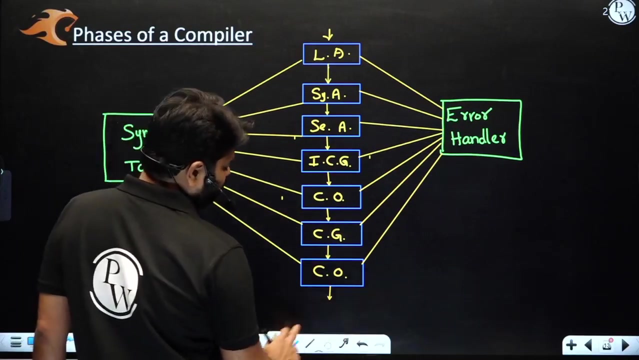 the error handler. comentarios from other fields are the same. so we are not going to get into state block signs in the next four yearіл in this kennel … … …. … here it might be possible some kind of lexical: сначала andнач pär dreams e options. here …. other phases: mainly the compiler is errors depends on the analyzers. and let me put in to here: here it might be possible some kind of a lexical: forbidden least compilations under our enormously clear example, if you apply to me. here it might be possible some kind of放 logically a condensed lexical. here it is like saying: we can you solve the problem with là, or let us do a simple gry by doing it instantly. 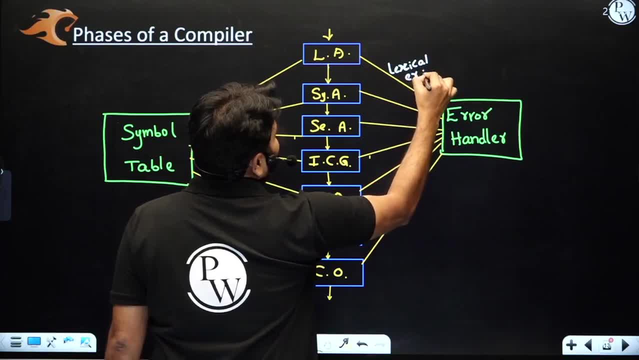 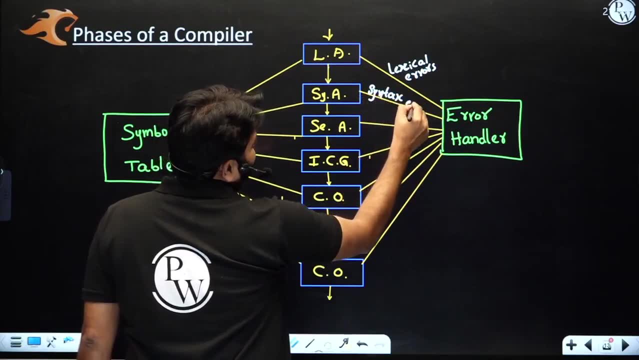 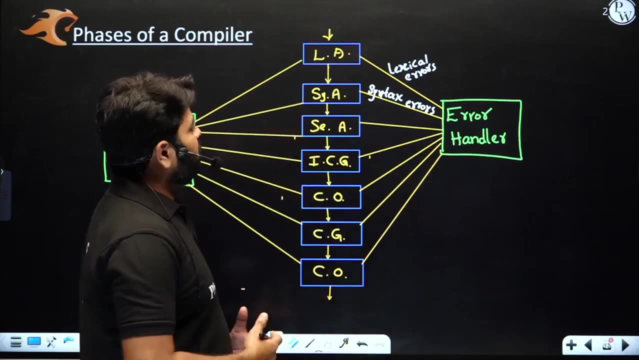 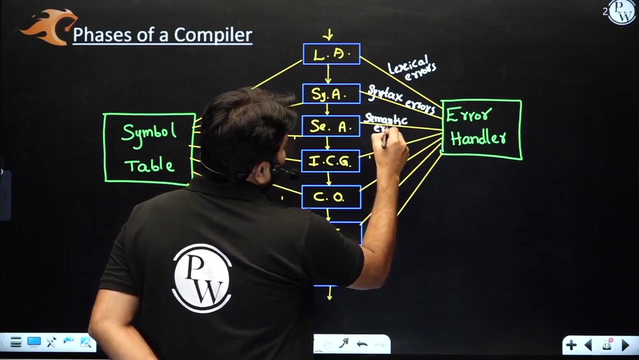 or token related errors. okay, here you might have some syntax errors. you will report to the error handler so that error handler takes the responsibility to produce the error to the user or programmer. and semantic analysis- some type checking related errors. so i'm just writing: semantic errors and other errors are basically fatal errors. 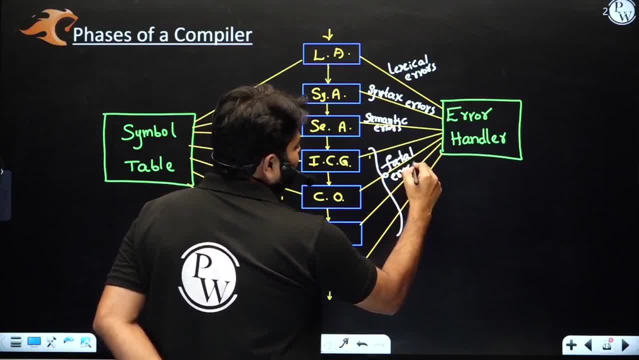 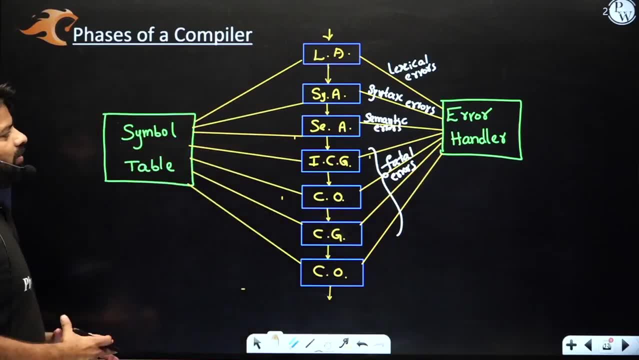 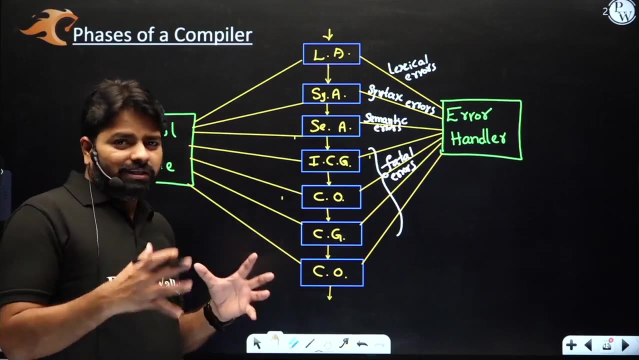 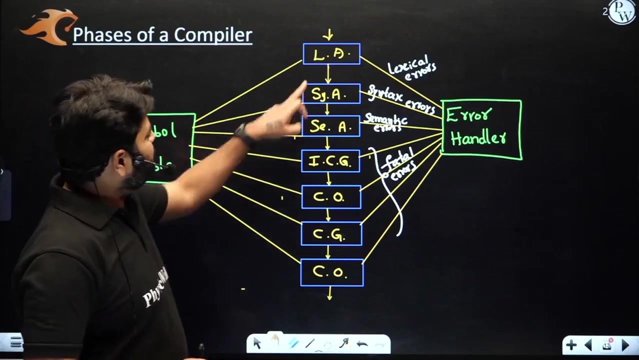 they are unavoidable system errors, basically due to insufficient resources. it could happen. now, as i told here, there are few phases which are part of the analysis. other few phases are part of the synthesis, so which are the part of the analysis? the first three, the lexical, syntax, semantic, are going to analyze the code, so these three are called as analyzers. 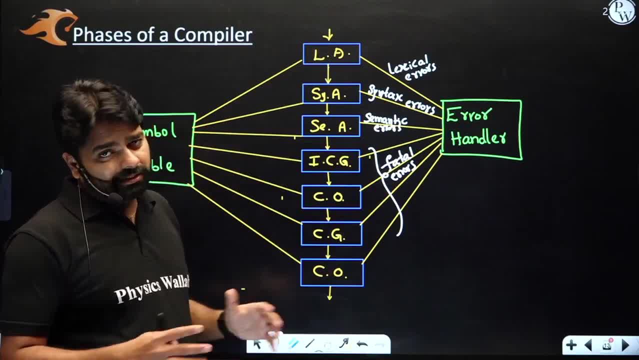 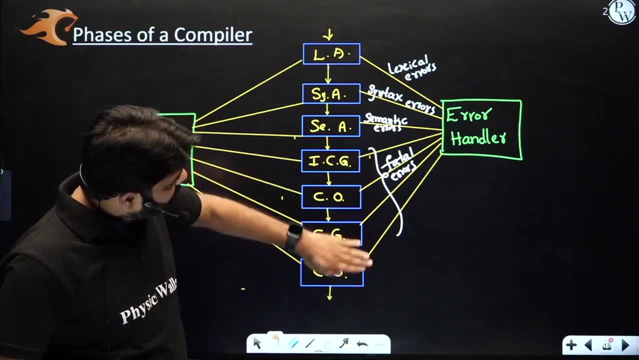 so these three are called as analyzers. the remaining part is called as the synthesizers, the. everybody is going to convert one form to other form, so these are the synthesizers among these four. the code optimization actually need not be. it's a separate phase you can also implement, is a part of the intermediate code. 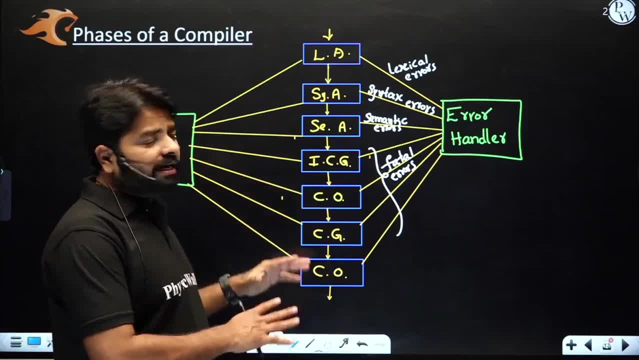 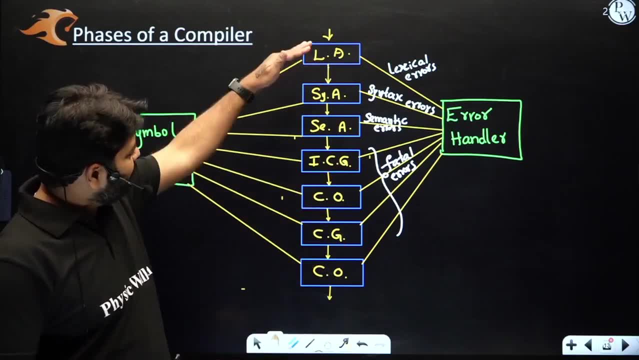 generation here is a part of the code generator but to understand it's a very special in this compiler. that's why we need a different way to implement so we can separate that too. the total seven phases, if you look at, and the four three phases are analyzers remaining or synthesizers. 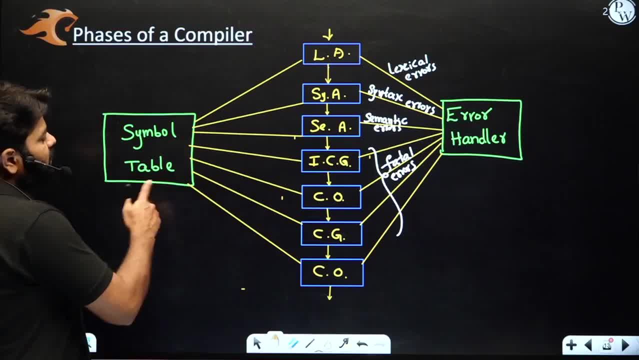 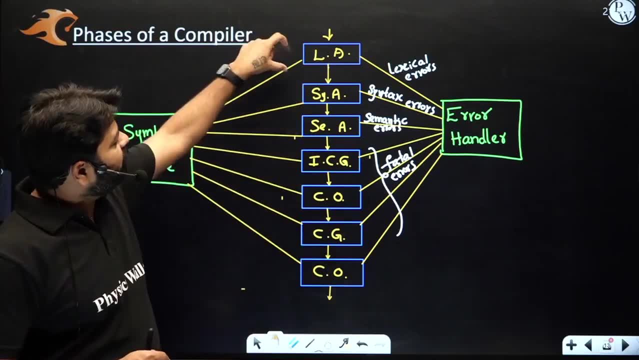 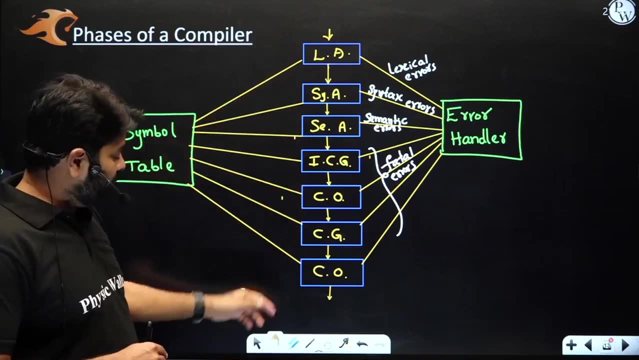 fine, now, what is symbol table? what is symbol table? will look into the symbol table once we complete all the phases, right, so we will focus on each phase. what is this? lexical analysis, syntax, semantic, ICG, you know, code optimization, code generator and code up the optimization. let me 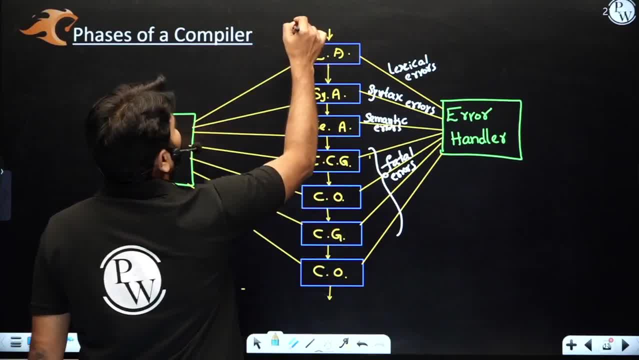 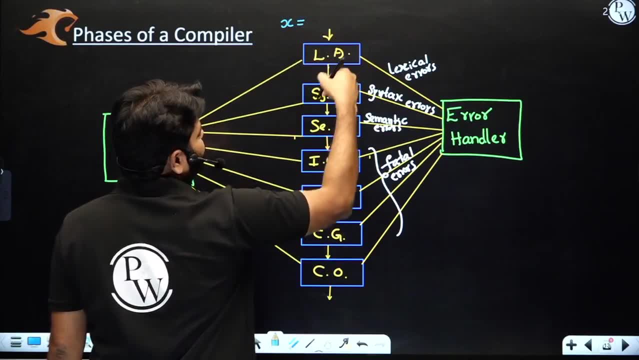 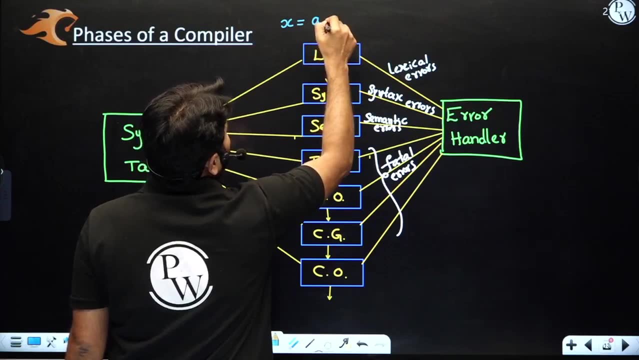 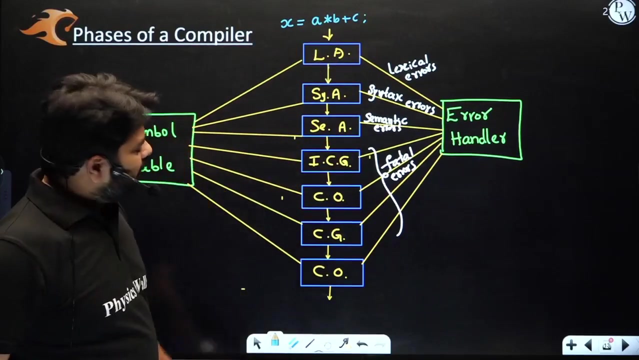 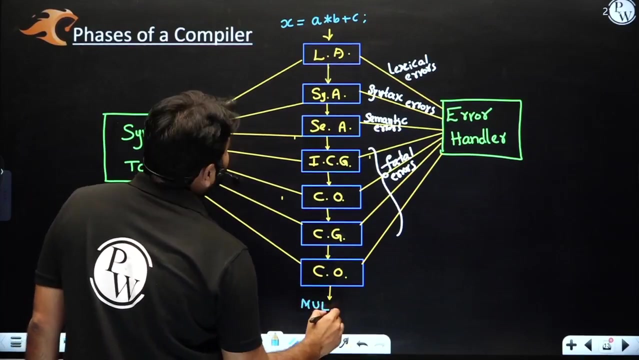 take some example to help you. that is, you know, I take a very simple idea example to understand here. let me write here: X is equal a multiply B plus C. this is my high level code and assembly code could be different, you know, I it might be possible that multiplication. let me write here: 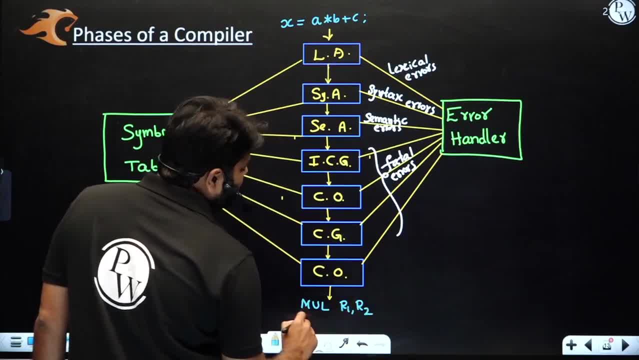 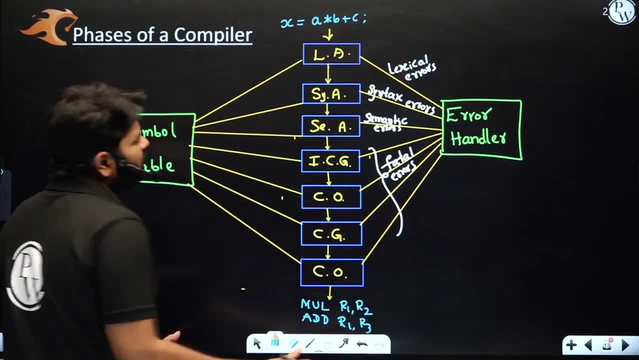 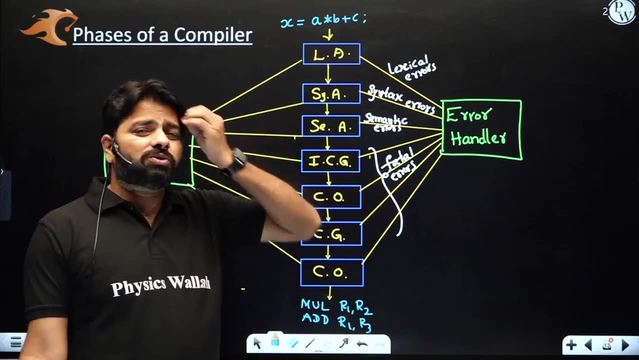 okay, R1, comma R2, and then addition that R1 with, let's say, R3 could be. you know some output- this I'm saying it. you know it could be one of the possible output if ABC might be. so if they are stored in registers, this could be possible output predictable from the compiler. so it need. 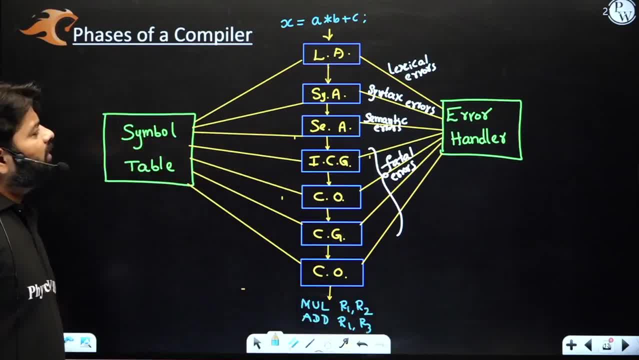 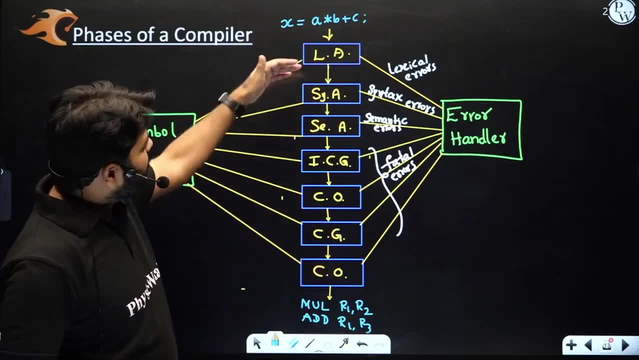 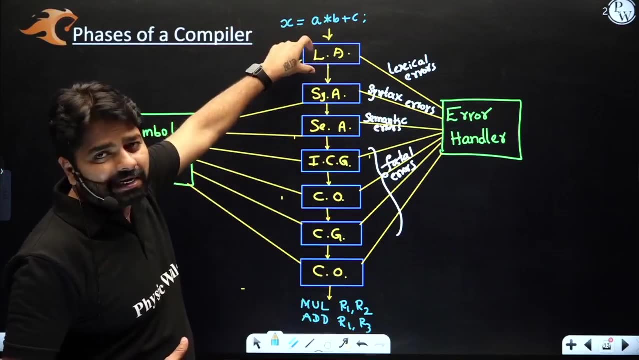 not be exactly, but you know similar one. or now let's focus on the each phase of the compiler, how the each phase going to take an input and produce an output. then we'll start one topic here, you know, in the compiler, the first topic is lecture analysis. we will spend 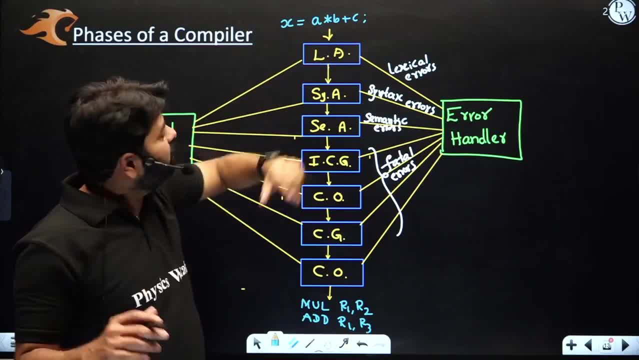 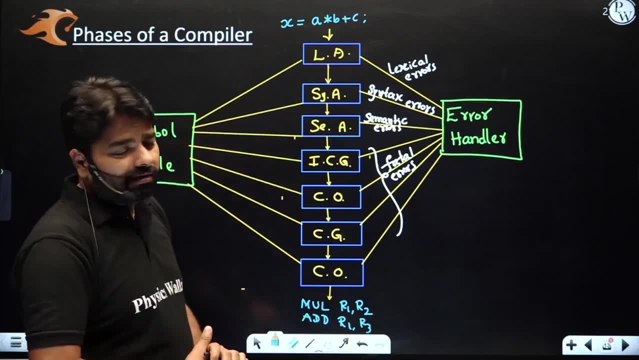 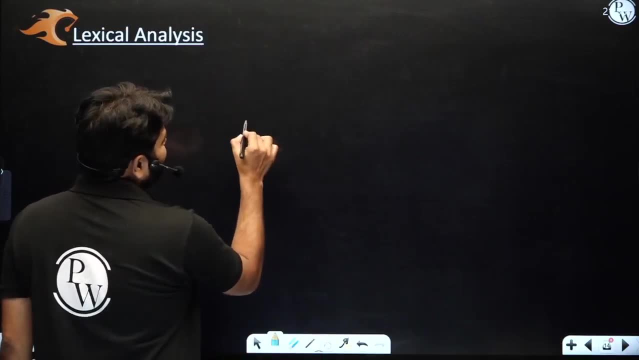 a lot of time to understand how this is going to be scanned, but right now, just see the input and output to learn. so, as I told, it has a lot of meaning like analyzers, synthesizers, and we'll see. overall too. okay, the first phase is lexical analysis, right, so what is the lexical analysis here? 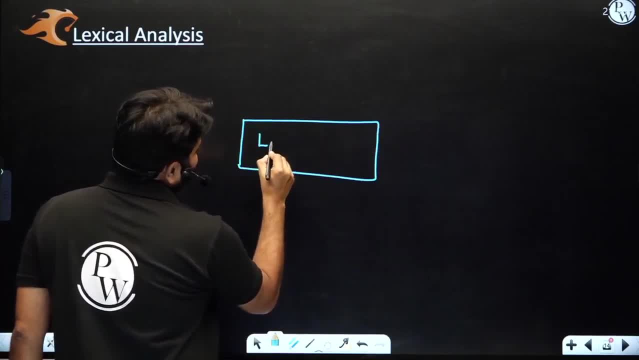 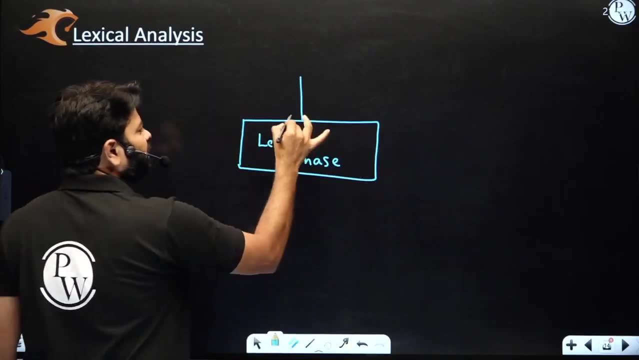 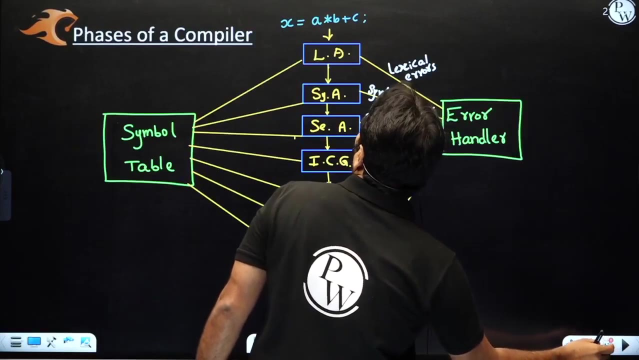 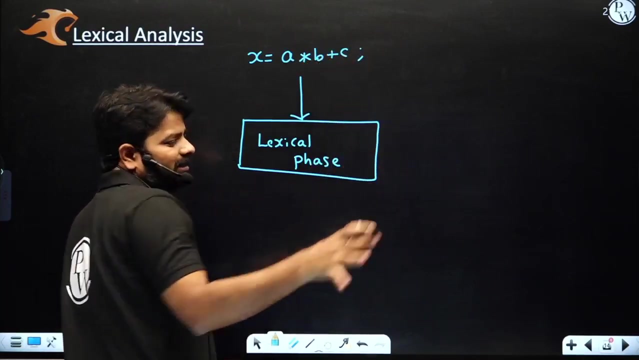 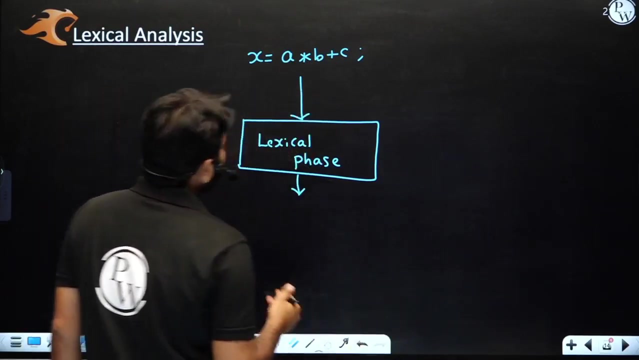 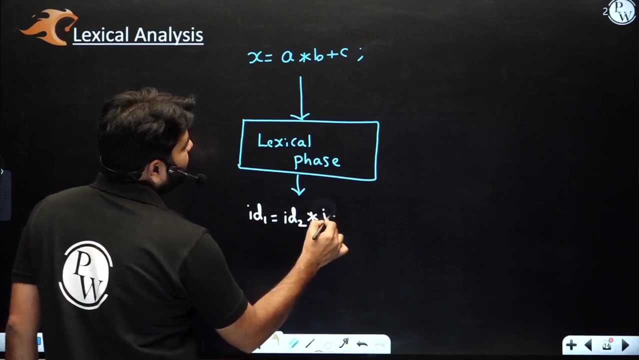 lexical phase. lexical analysis, phase analysis. both are same here. so you give input something like: x is equal to a. what was it? multiply with the b plus c? this is some high level c code. now what is expected here? expected something is- you know- don't worry what i write- but something like: id1 is equal id2 multiply with id3 plus c. 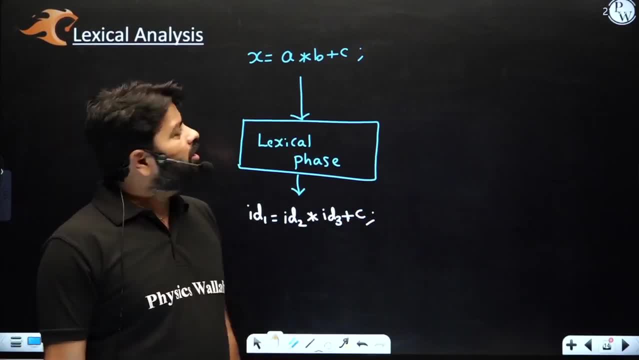 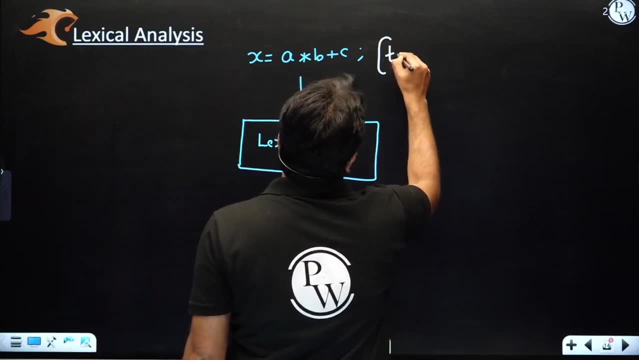 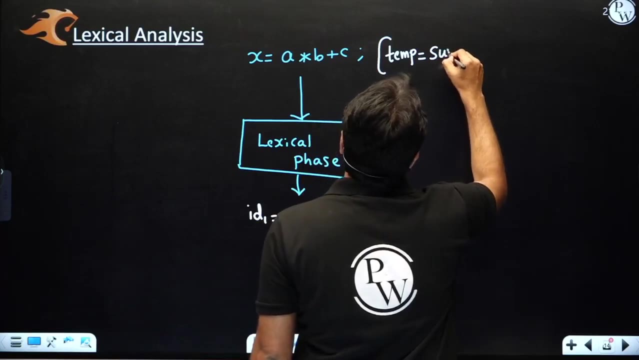 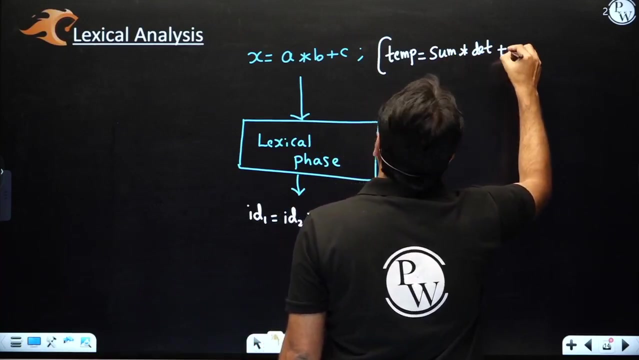 like this: it converts everything into tokens. maybe you know need not be: x is equal to a, a star b plus c. you just give any other something like this. you know temp is equal. you know some multiply with: uh, det, something determinant plus, and i just want to say some other count. 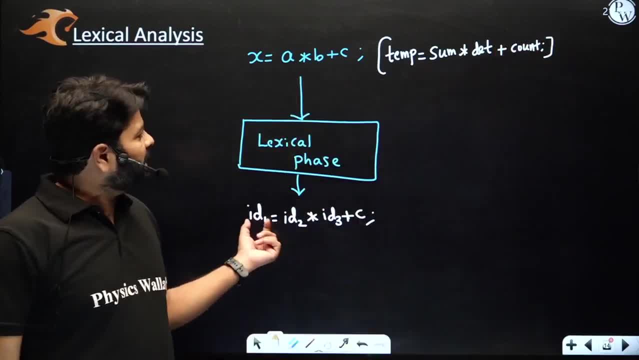 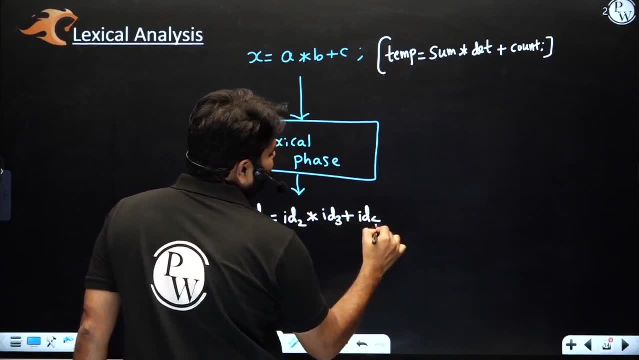 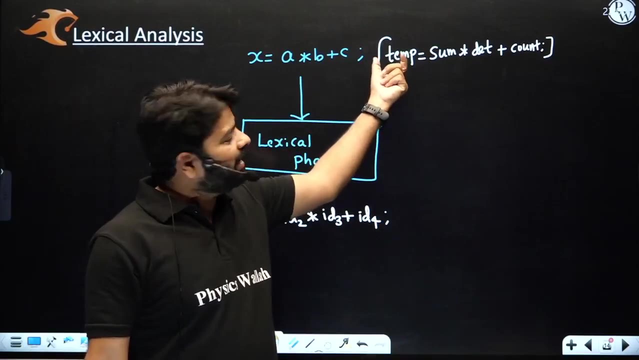 you could give anything like this also. it converts something like: id1 is equal to id2, multiply with id3 plus. sorry, last one, not the uh, some id, id4 need not be exact same subscripts, but similar to this. now it's produced. as it collects, you know, it groups the characters into tokens and produce the corresponding token. 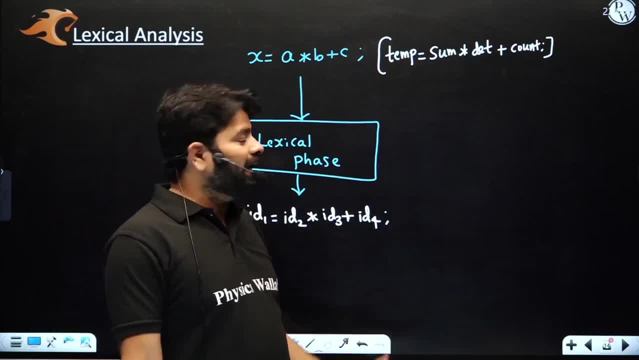 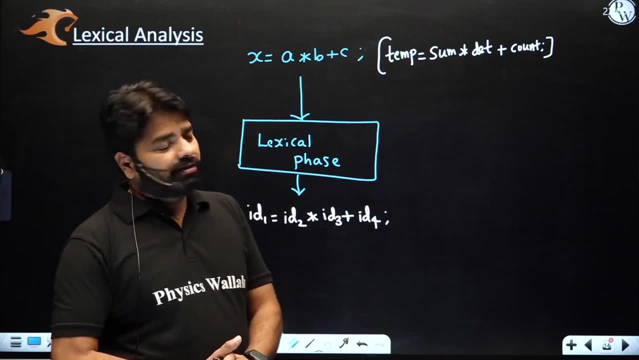 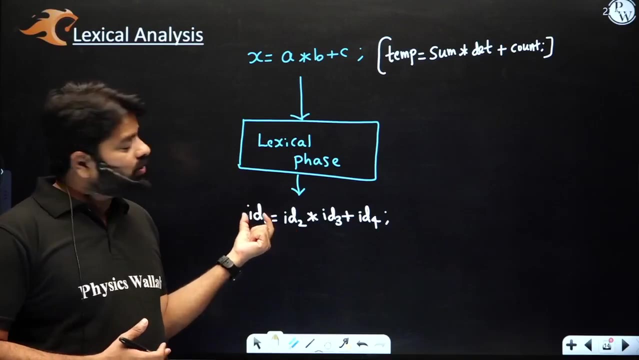 it may be. id1 is equal to id1. multiply with id1 plus id1. if all are same variables, okay, so this is the expected output from a lexical phase. is it exactly the same way? yes, it's, it's exactly the similar way, but it's going to group. it's going to group. it's going to group. 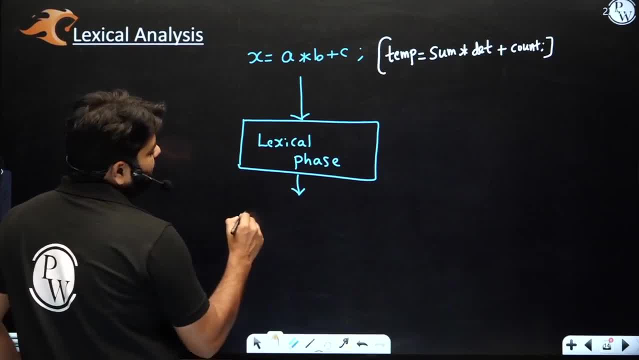 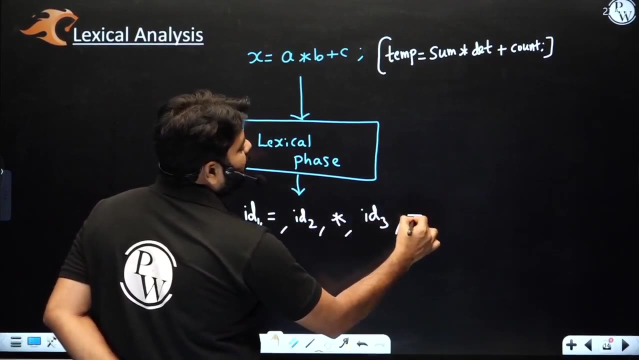 how it groups. basically it's a statement only. but first id1, that's for x, uh x, then equal to maybe some other uh token name, or it could be equal, or next id2, next multiplication, next id3, next addition, next id4, next semicolon, it's going to inform to. 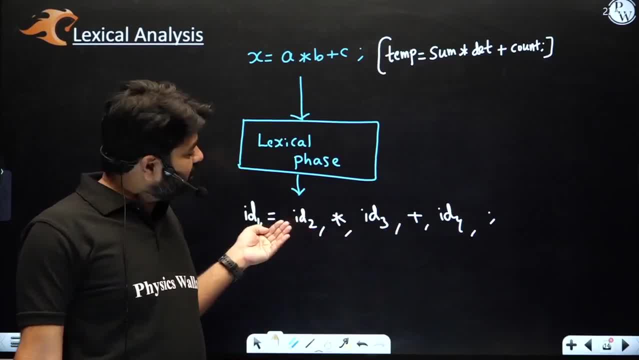 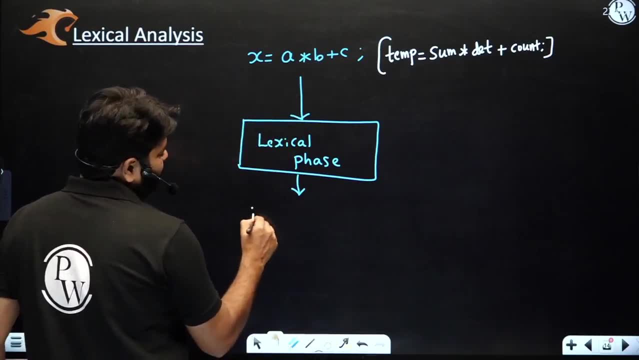 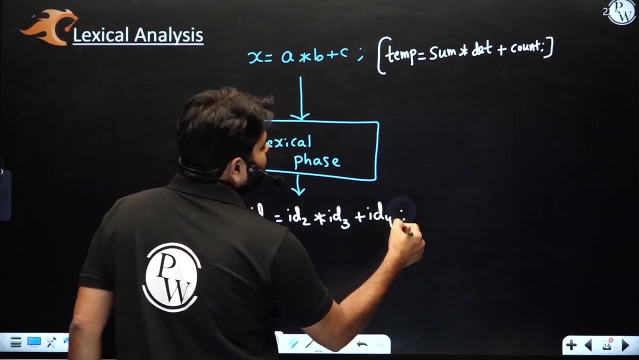 the syntax analyzer. who is the next token in this? uh, in this program, it's going to produce the sequence of tokens. that's why we call- we call token stream what we call token stream. this will be visible to the syntax analyzer. so now, when syntax phase comes, it will be taken as: 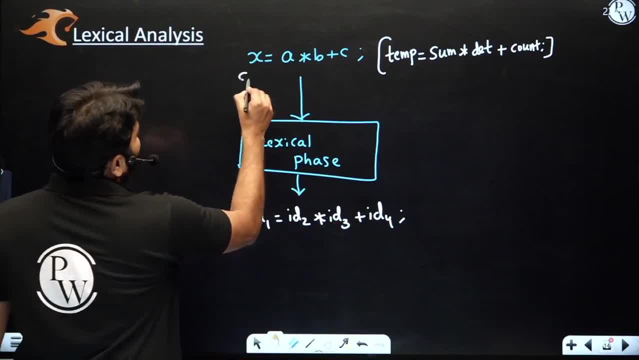 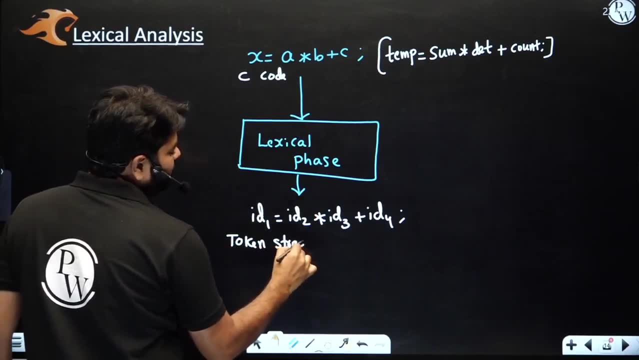 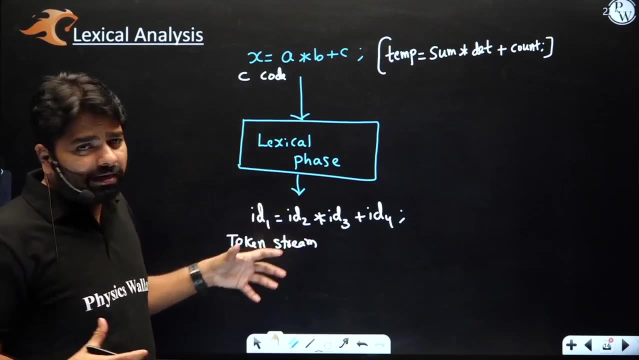 an input. so what is the input of this one? is a c code, right, high level code. what is the output of this one token sequence or token stream or sequence of tokens. this will be produced and if in if, if it finds any token error, it will produce some error, or you can say it uses a symbol. 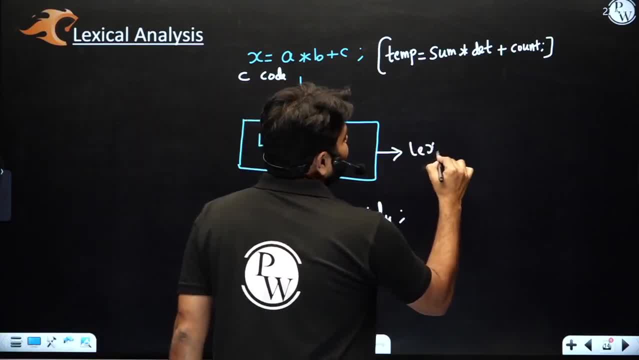 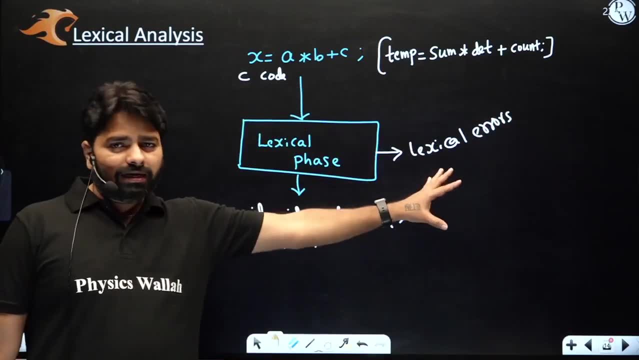 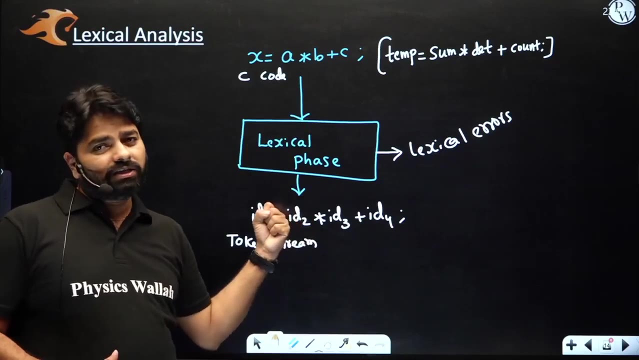 somehow it produces error. if there is any lexical error, what are the lexical errors? we will see in the lexical analysis. okay, right now, don't focus on what are the errors. okay, this is about the first phase of the compiler. it simply does a scanning of the code and produces the token stream and this: 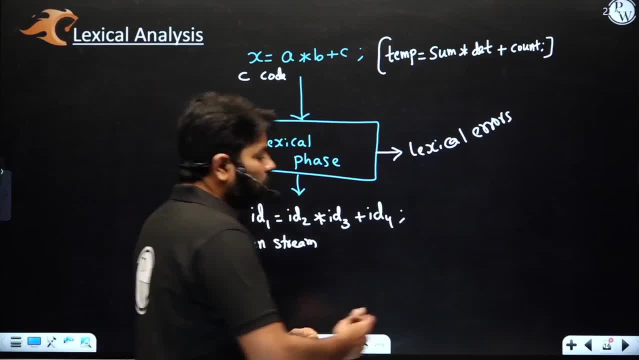 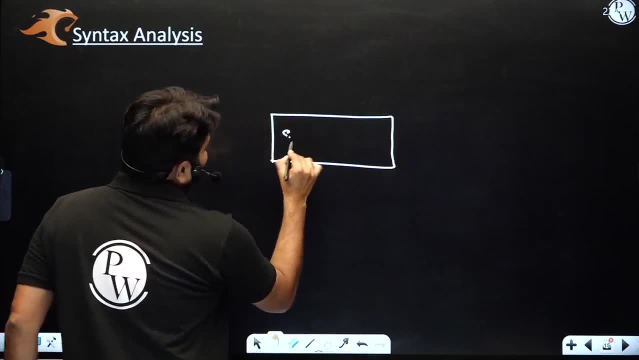 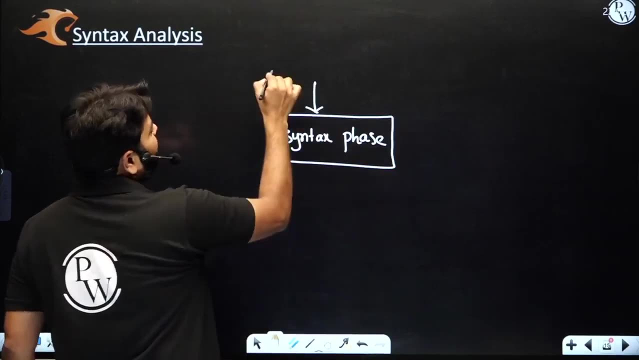 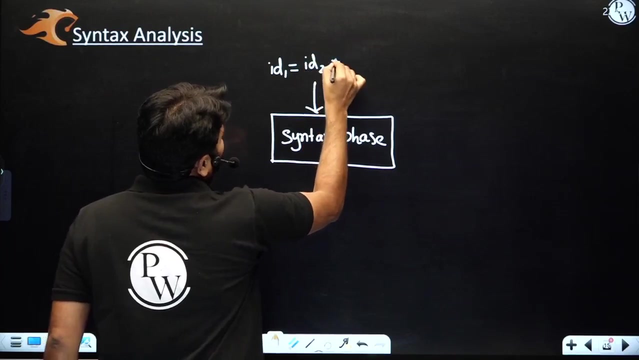 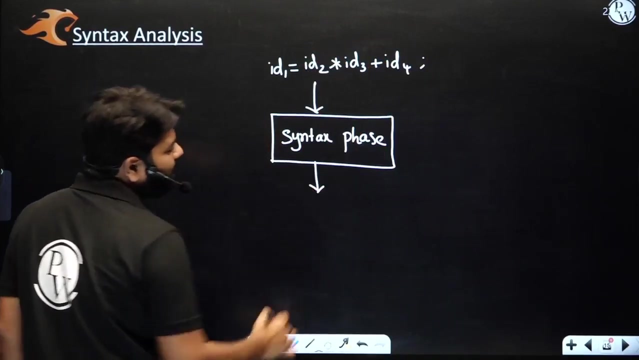 token stream will be taken by the syntax analyzer. so what is the syntax analyzer job, the syntax analysis, syntax analysis or syntax space? it takes the program that you have, uh, the token stream. the output of the lexical analyzer, id1, is called id2. multiply with id3 plus id4 and this will be taken and will produce a pass string. 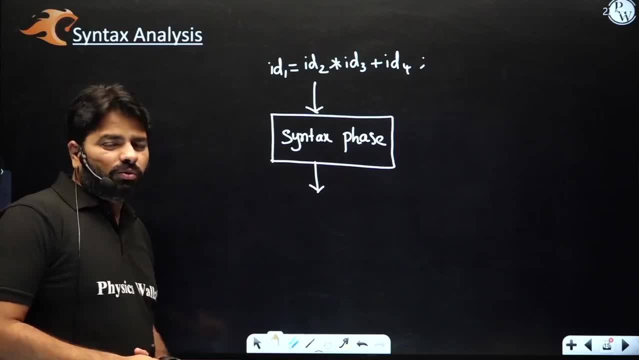 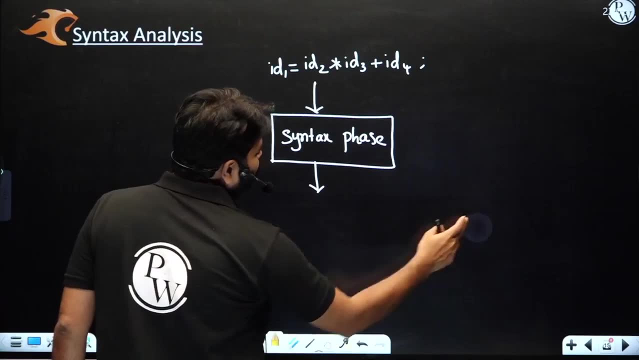 okay, what is a pass tree that uses a context grammar to derive the string? okay, don't very much about it, i'll generate my own pass free. i'll generate my own pass to here. don't worry how it is, because it might be my own compiler or my own context free grammar. there will be root. 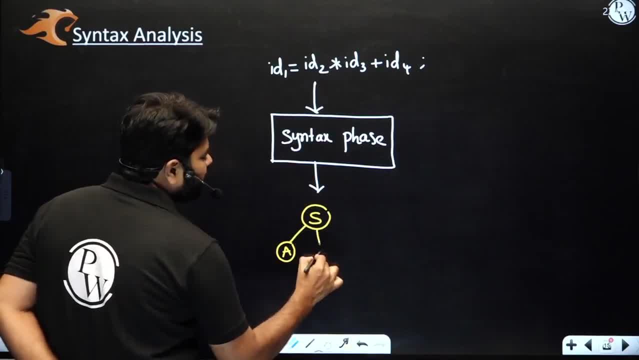 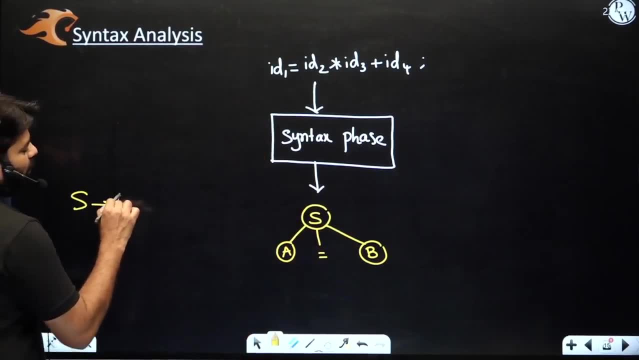 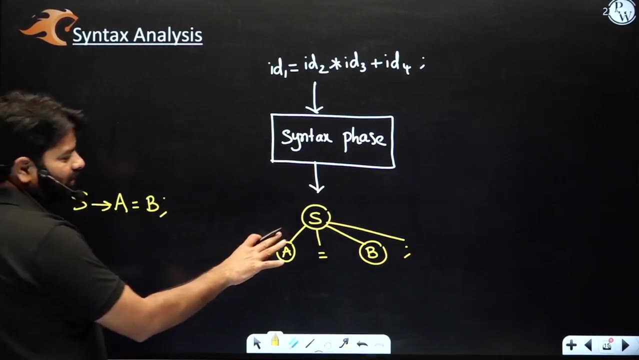 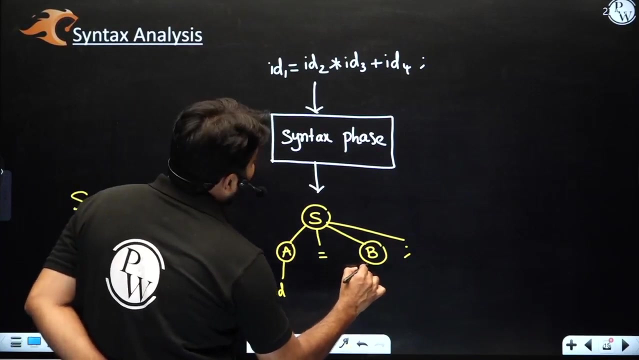 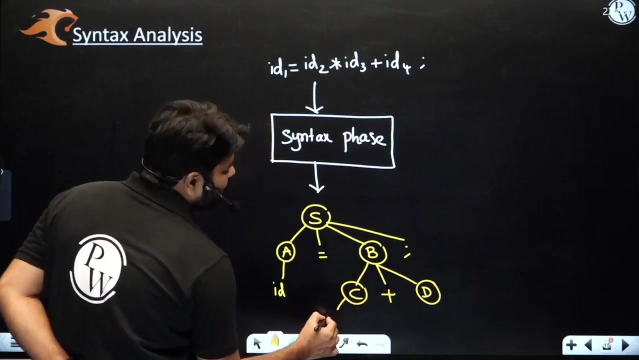 and there is some how to produce. there are variables, productions. basically you have a production, something like inside s arrow, a is equal to b, semicolon, maybe you have here, then this is off of the pass tree, a part of the pass tree, and a will have something like id and b will have something like c plus d, and what c does here, the id? 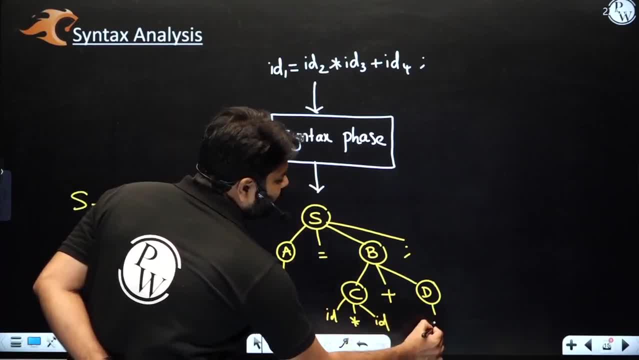 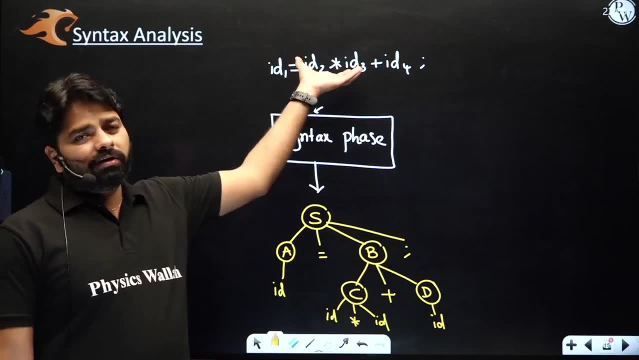 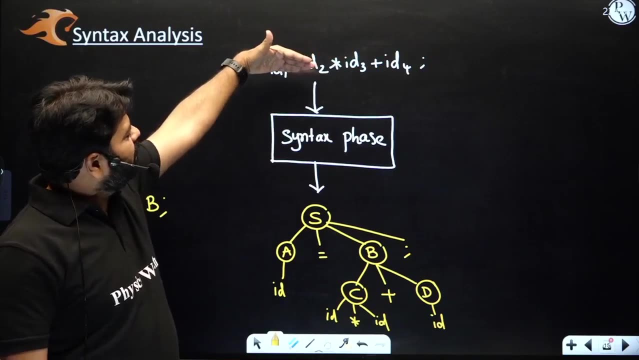 multiply with id and d derives id. this could be, you know, uh, one of the possible pass tree for the this string. it could be, as it's called as an out string. this is the string which is actually the sequence of having sequence of tokens and for this string you have the corresponding pass string. 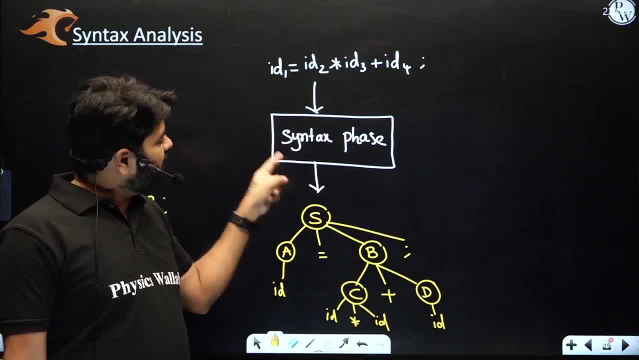 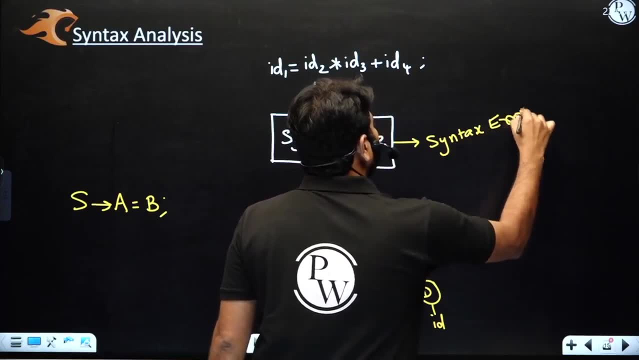 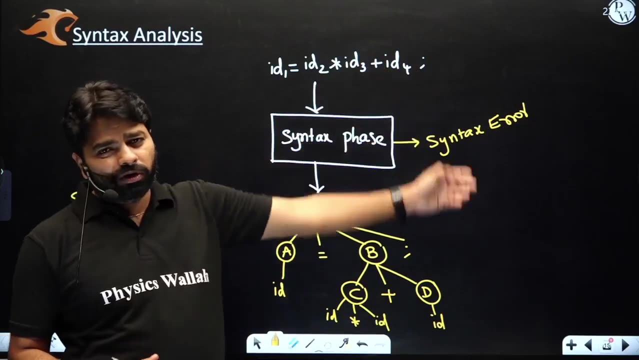 in case, if there is any syntax issue, this syntax phase will produce syntax error, mentioning the reason you see a lot of syntax errors right in the program when you have some syntax issues while you write the code. okay, if you miss the semicolon or if you don't write all the operands properly. 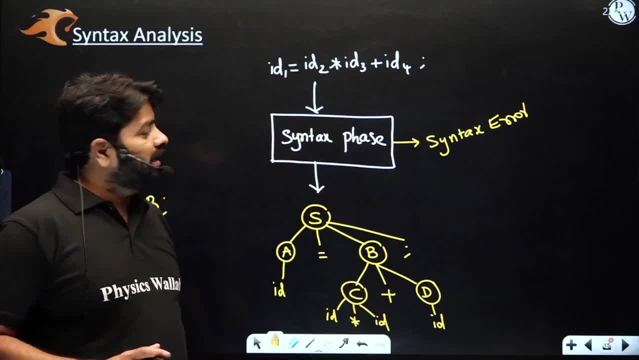 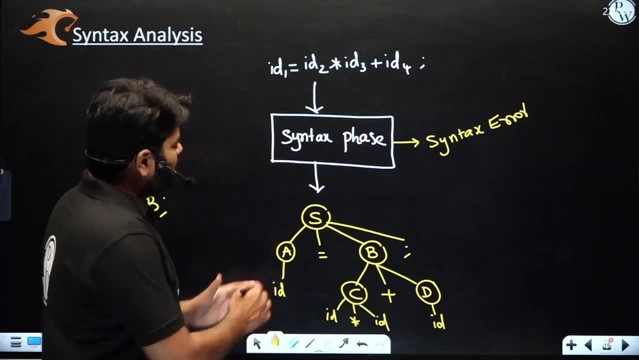 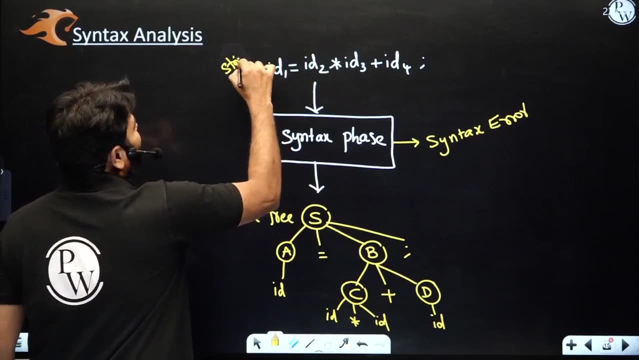 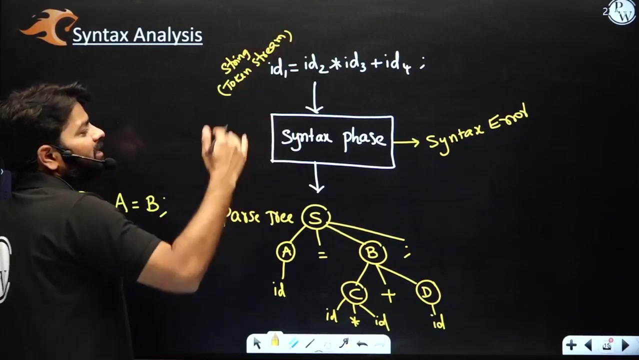 you might get some syntax error. that will be displayed by the compiler in which line which place a possible syntax error exists. this is called as a parsing. what is the output here? power spring. what is the input here? this is considered as a string here, but actually this string is nothing but token. frame is output of the lexical analyzer, but it is input to the 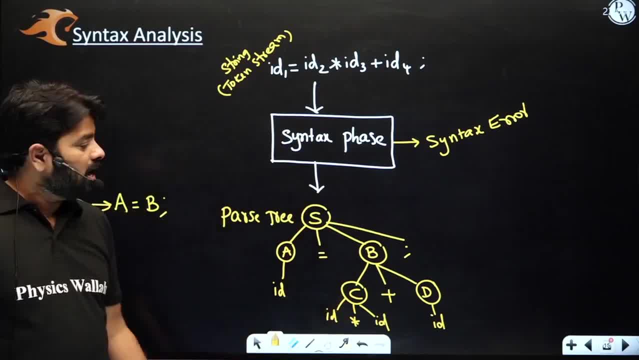 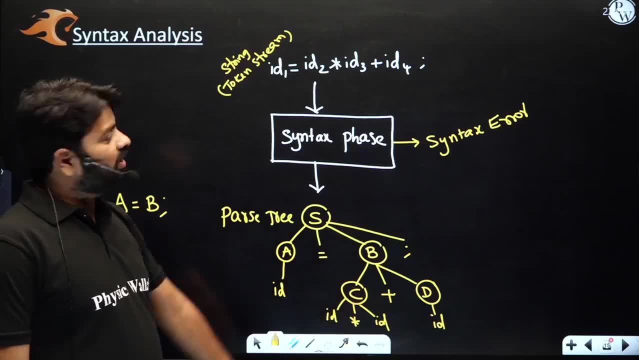 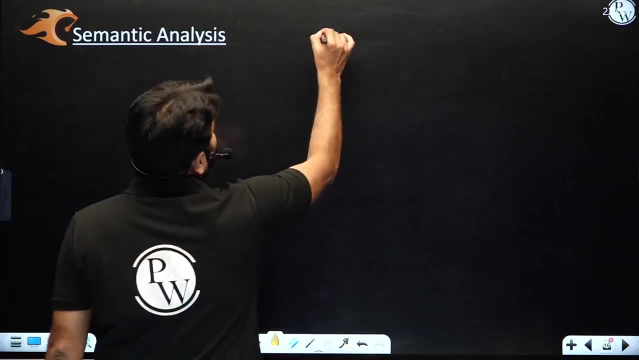 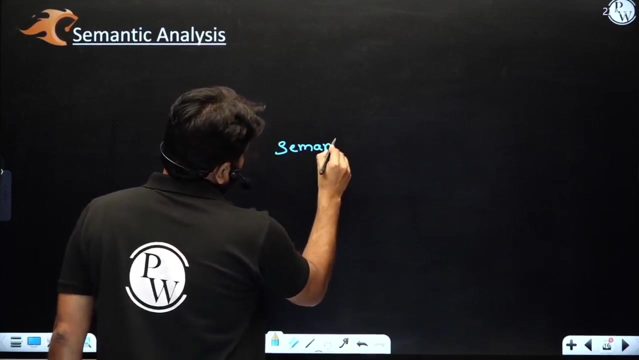 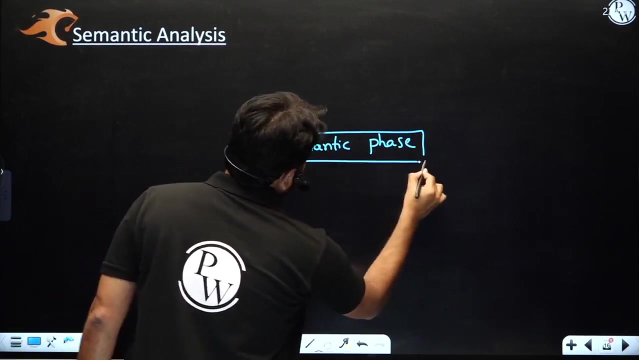 syntax, space and syntax. this produces the power string and this posture is input to the semantic analyzer. so, okay, the same one. okay, i uh copy the same one to this semantic analysis. here in the semantic analysis, the parse tree semantic phase or semantic analysis analyzer, the input is the r3. output is: 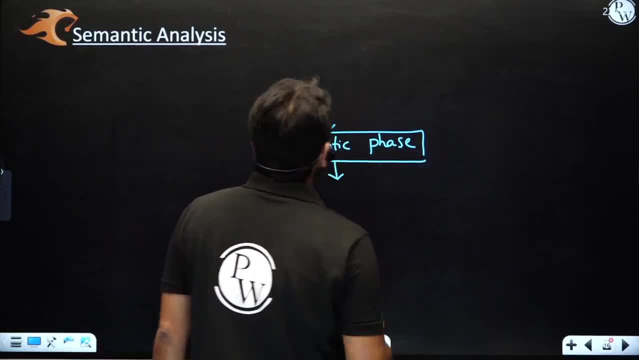 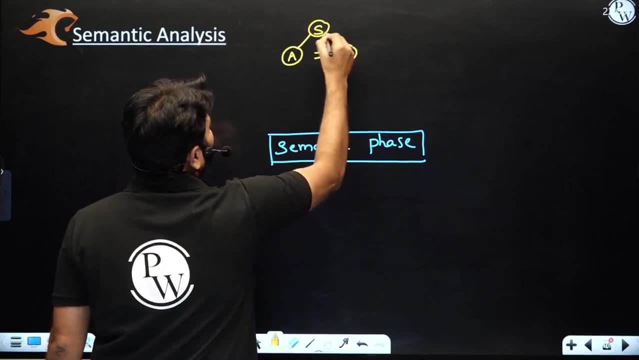 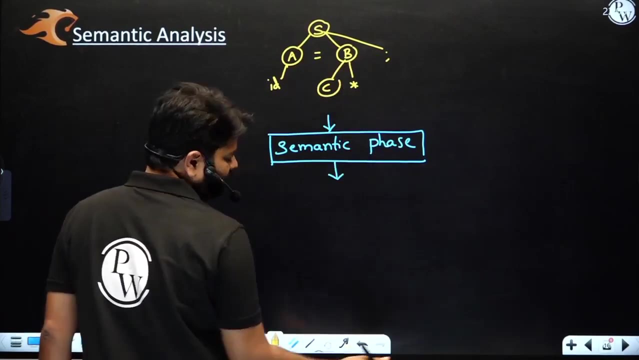 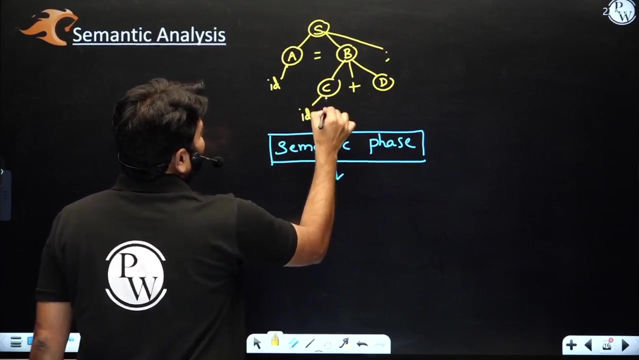 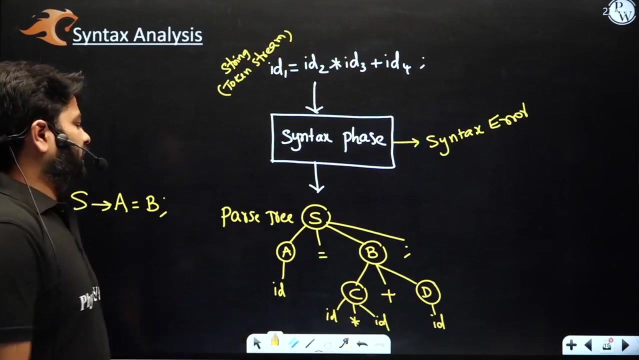 the annotated parsing. there is some tree right s. okay, a is equal to b, semicolon a to id and i said c multiply. sorry, addition d and c has some id, star id, d2, id, same. yeah, perfect now. this is the input to the semantic phase. now what is the output? 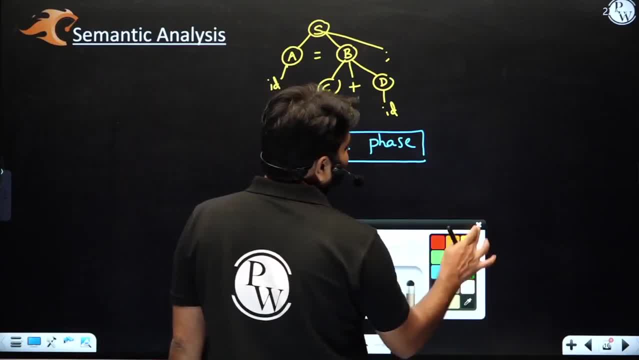 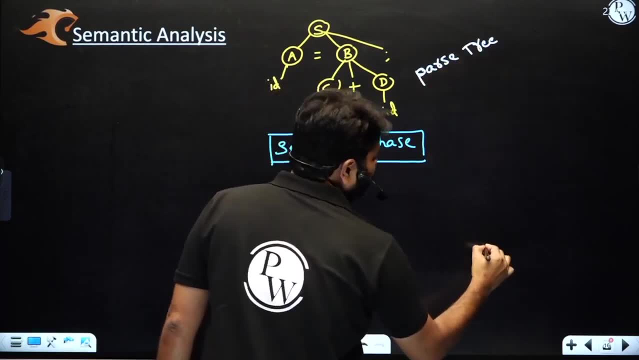 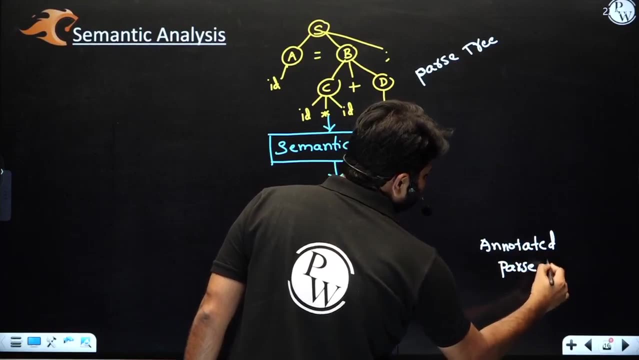 okay, it looks weird as you are not aware of the compiler if you are beginner, but still you should look at. this is the parse tree and what we are going to produce here, annotated parse tree that we are going to decorate. with some translations i might have some meaning inside. so what i do here. 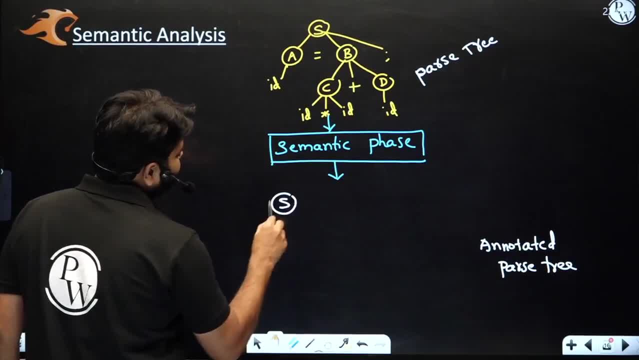 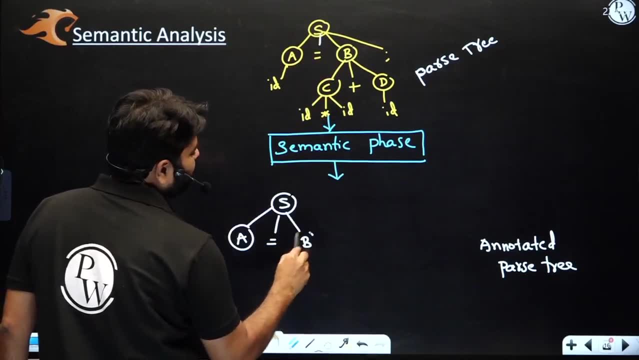 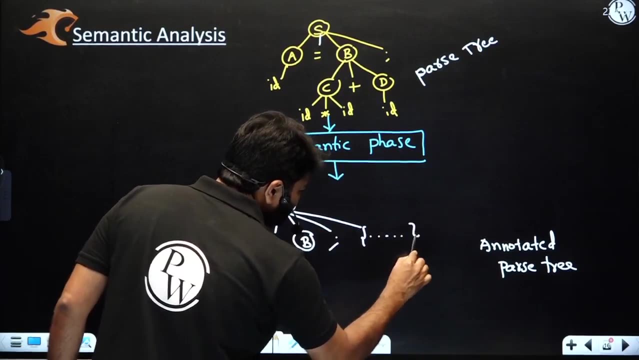 i produce the same code here, that same thing i produce here equal to b, and i might have some rules here inside. don't worry what are those rules, but here there is a meaning here i'll write something here to check the types: is that a and b are having the same types if a dot type is equal. 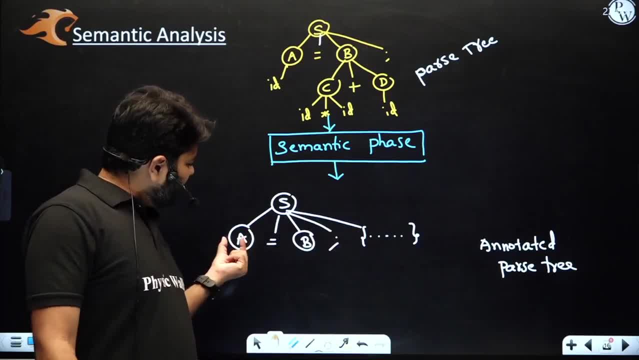 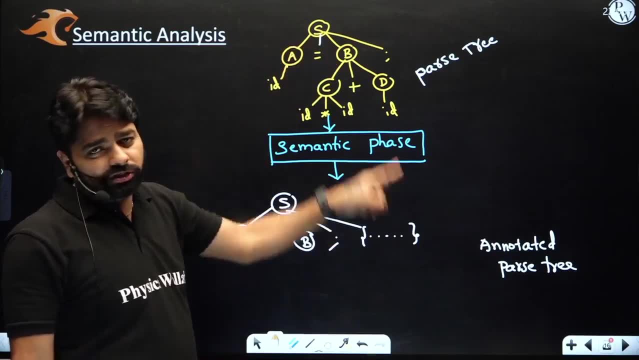 b dot type. there is no syntax error. in case, if you see here, if a dot type is not a same as b dot type, it will produce a semantic error because its expression this type should match. okay, if you. if it, if it is not going to support implicit conversions directly, it will produce an error okay. 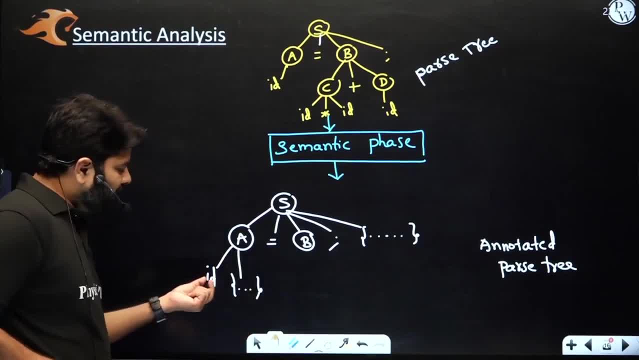 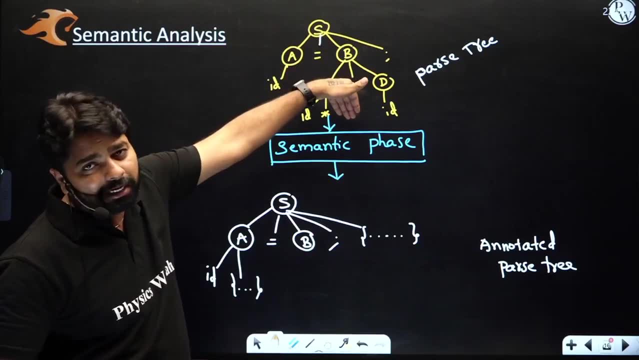 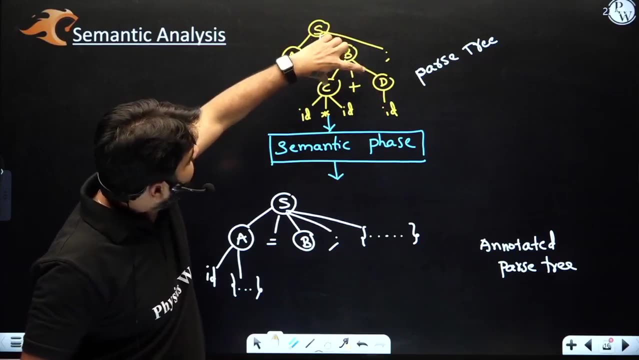 id and u. it will assign somehow this id dot type to a dot type and b gets the types from the uh, c and d but c gets the type from id multiplication with id. these two types are matched. then c dot type is same and d dot type is same as id dot type and c dot type d dot type. if they are same. 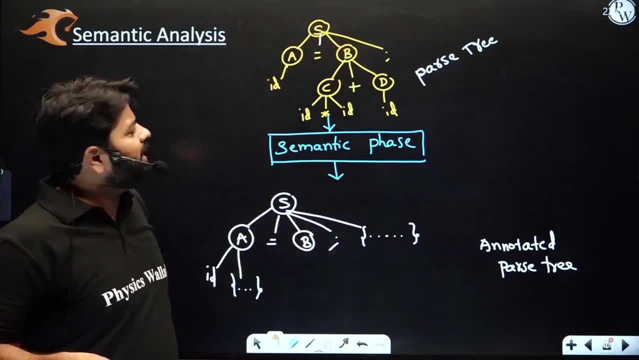 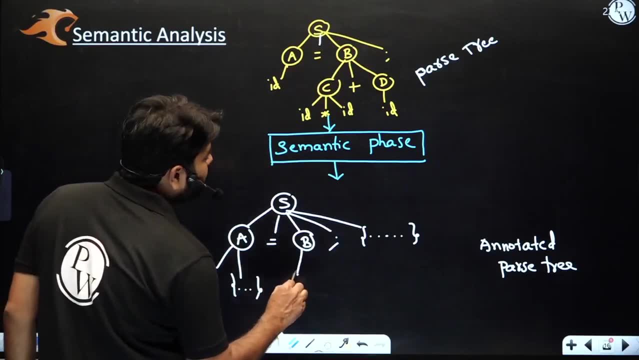 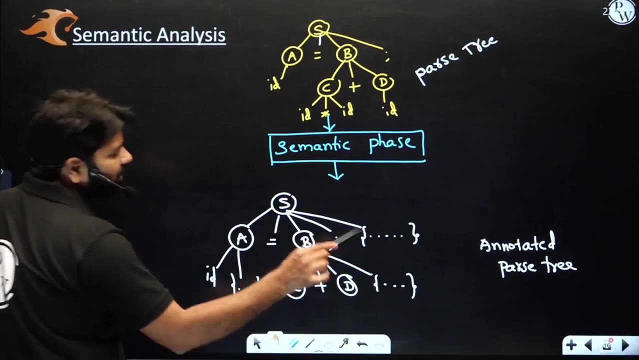 then we will get the same type in case. if it any any mismatch in at any uh sub tree, then it will produce the semantic error. so here, each place, it's going to check the types. even here also there is a type checking. okay, i'm just putting the dots, but 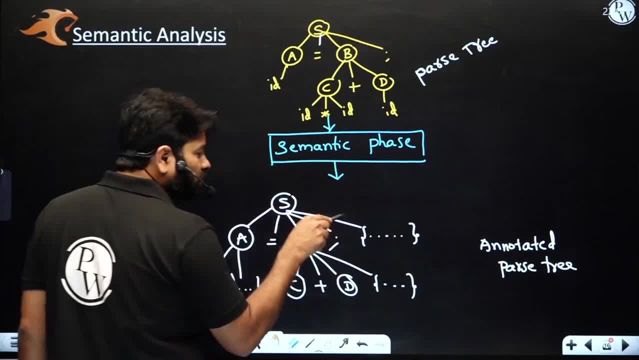 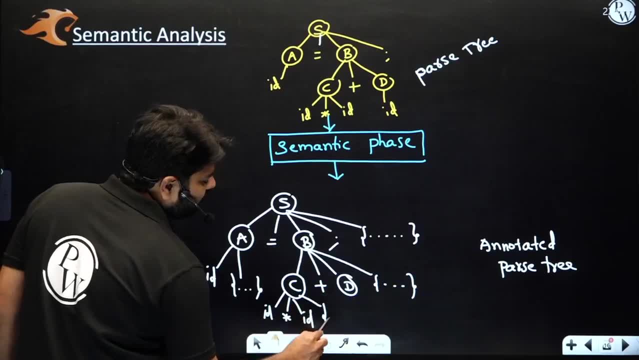 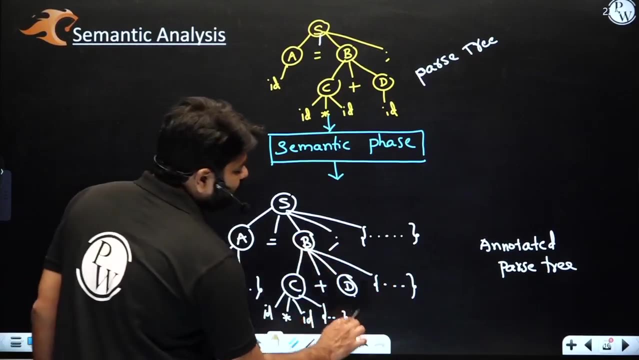 assume that they are the annotations here. they are going to have some translations now. id multiplication with id, the translation no need to be at the end, it depends on you know what kind of translation you need it. and d id and that type will be decided here. id dot type. 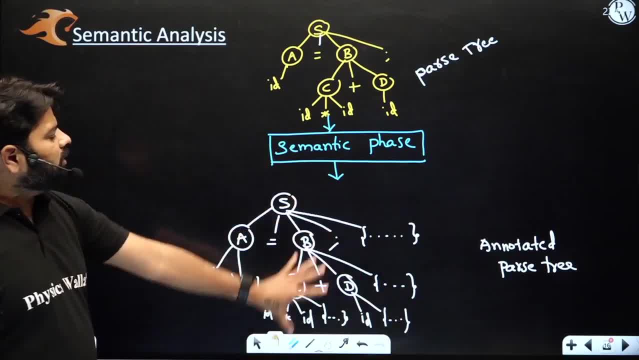 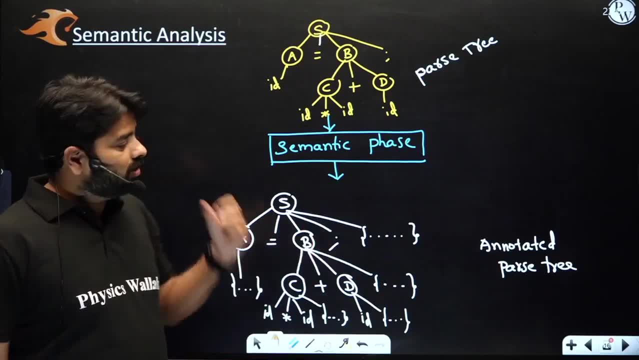 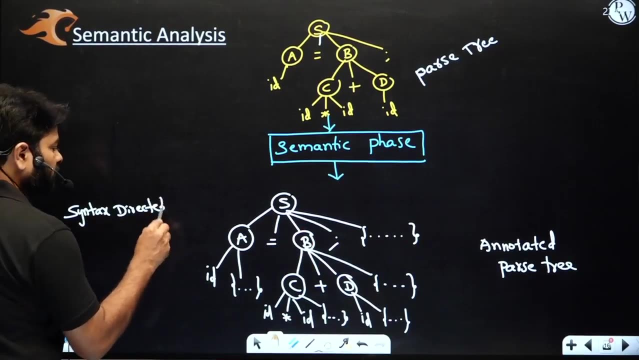 will be assigned to d dot type. okay, so all the things are actually, uh, done by the sdts are going to help us to do this semantic analysis. so we are going to use syntax directed translations, which are going to help us to perform the semantic analysis. okay, you will be writing. 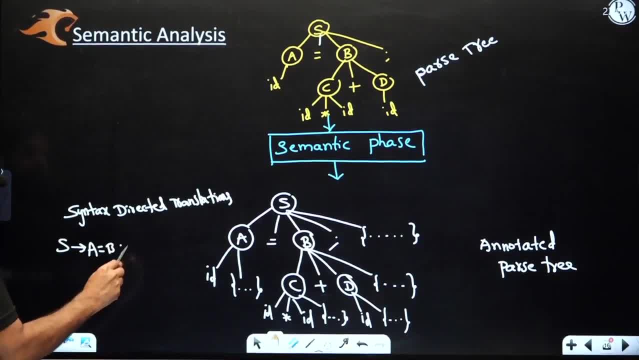 something like s arrow: a is equal b semicolon. you will be writing the production like this, along with some translation. similarly, you are going to have the grammar. actually, your grammar might be used simply a is equal b semicolon, but there is a translation added to that context-free. 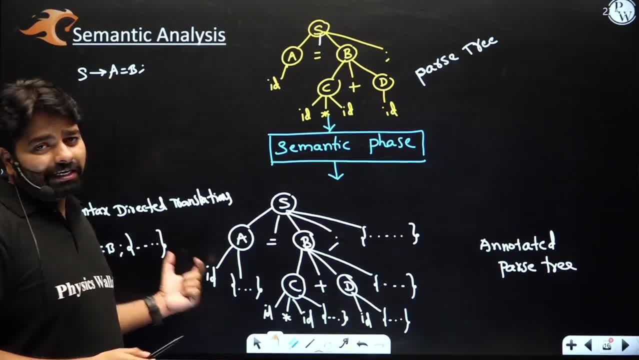 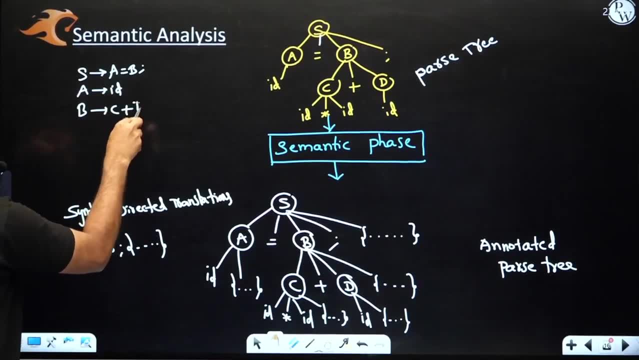 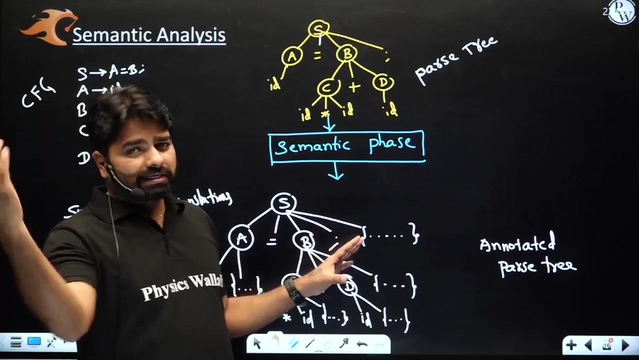 grammar, so that we call it as syntax directed translation, translation here. when you look at the grammar, your grammar might be looking like this: b is equal to c plus d, and c derives id, star id, d derives id, but here the translations are added. this is the context-free grammar, but here the context-free grammar along with the translations. 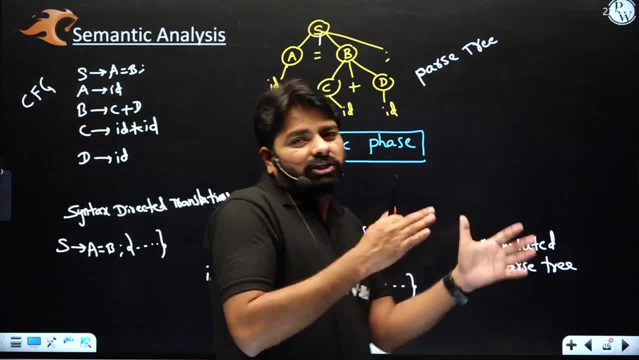 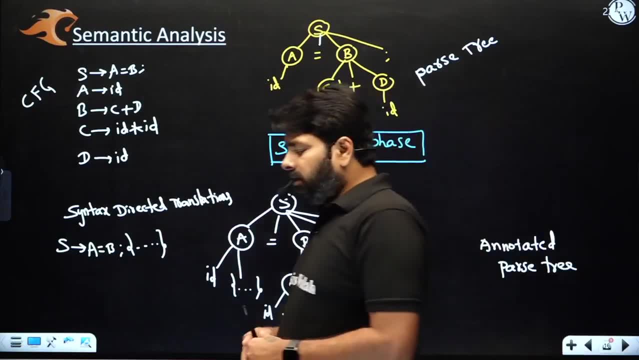 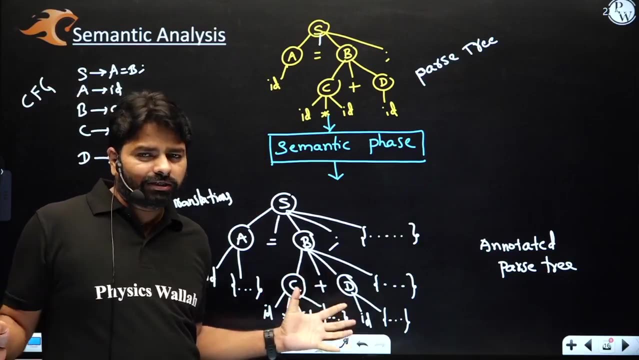 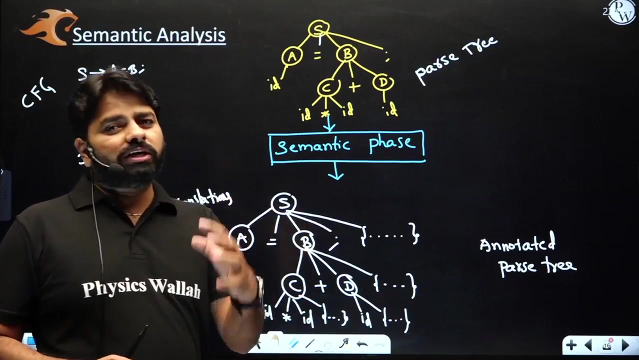 called as syntax directed translations that syntax are actually directed to the some meaning. so we call sdt syntax directed translations. fine, this is about this semantic analysis. now this one: once lexically, syntactically, semantically correct, then this code will be converted into the intermediate code: intermediate code. so intermediate code generator is going to: 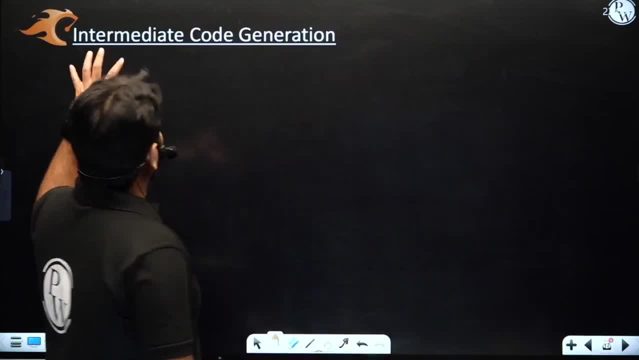 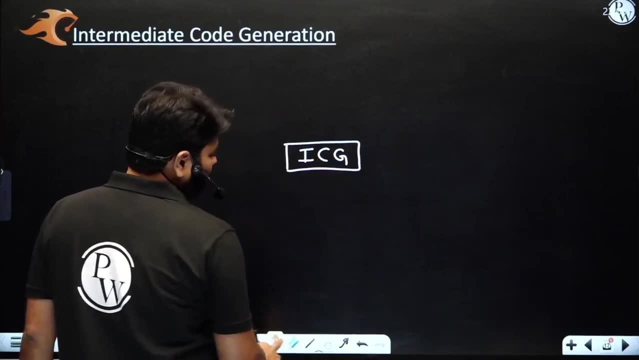 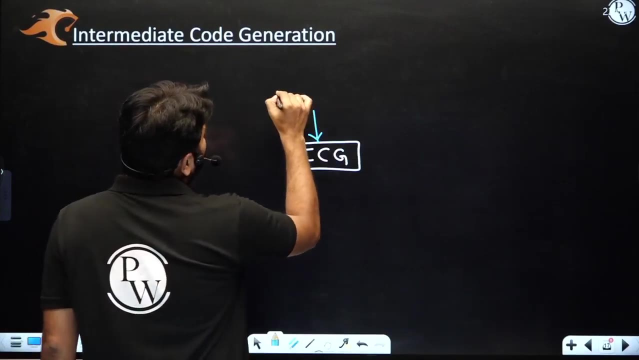 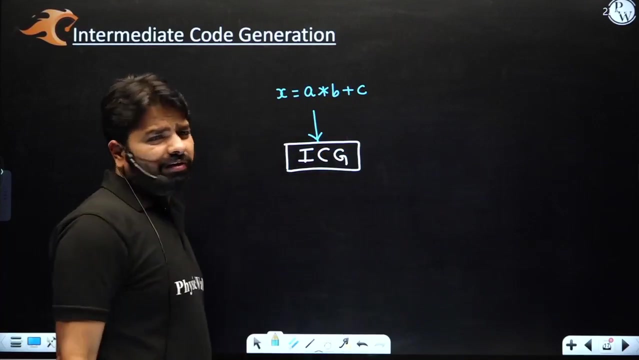 help us. when you look at this code, the intermediate code generator or generation icg, what it is going to do here, no doubt the analyzed code comes out here. comes here that analyzed code. what was that analyzed code here? something like right x is equal to a multiply b plus c. after verifying of verifying: 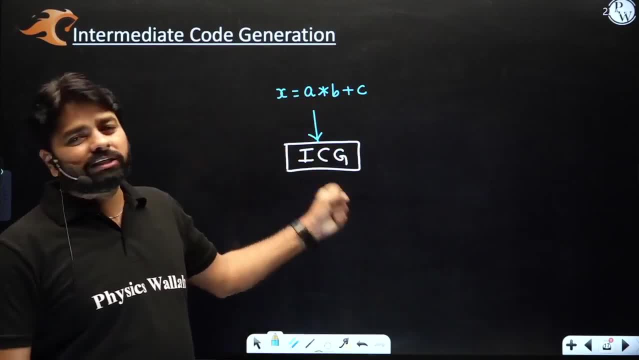 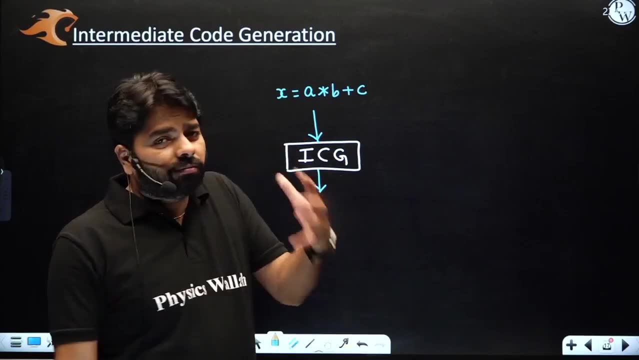 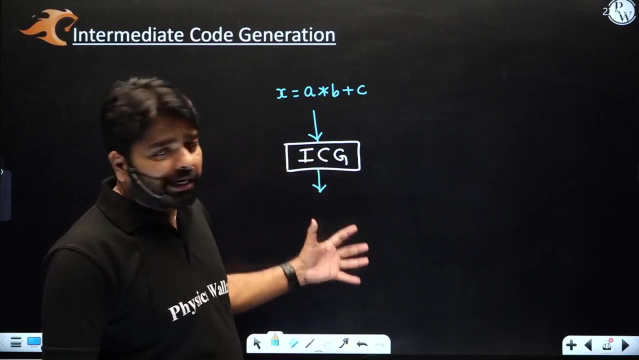 lexically, syntactically, semantically, that code is taken by icg and it produces some form of intermediate code. there are many forms for intermediate code, like syntax tree, directed acyclic graph, 3rd order address code and control flow graph. there are many things. i'll take one of the best form. 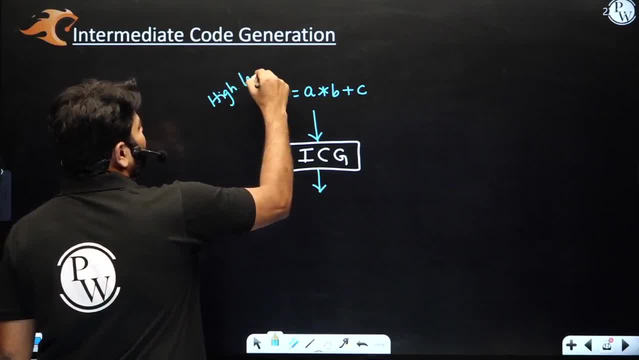 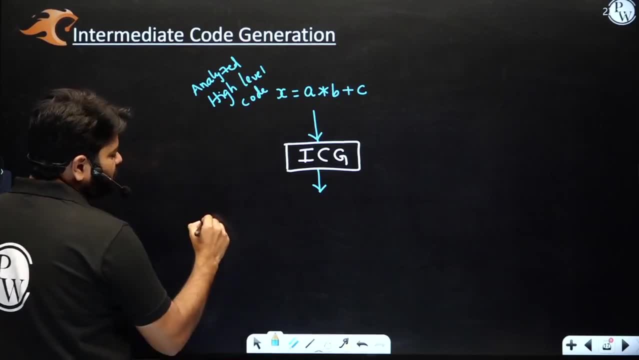 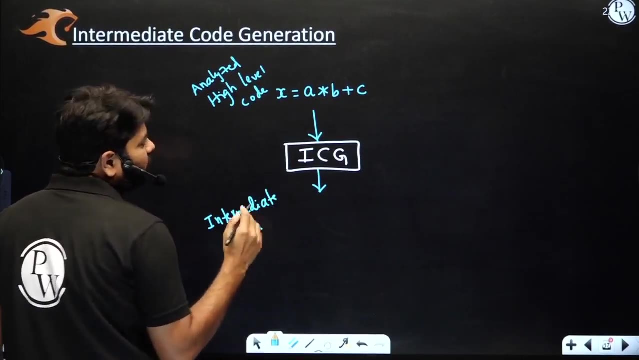 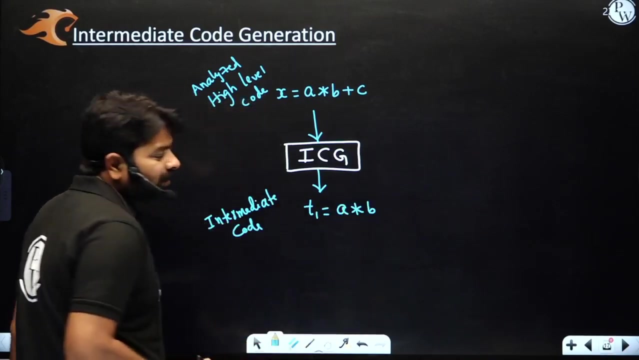 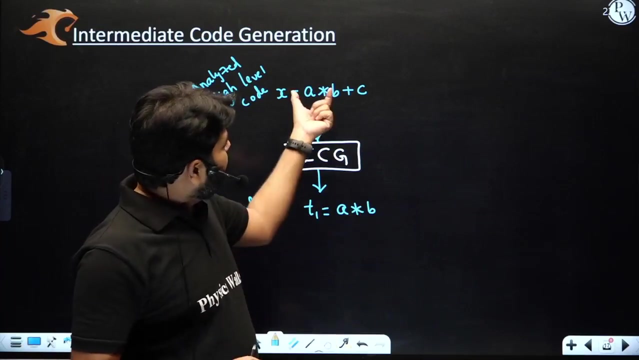 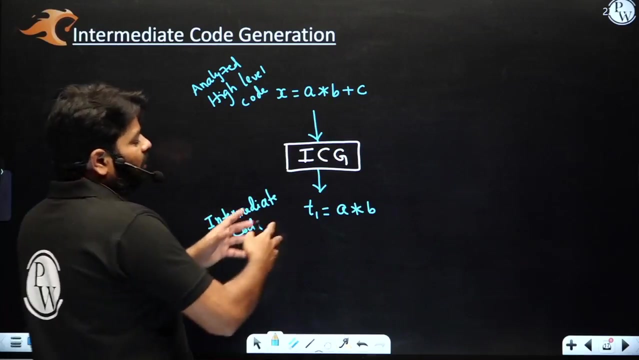 this is high level code. i'm just saying analyzed, analyzed, high level code, and now it produces the intermediate code. what is this intermediate code? it's something like Main System, St擊prinzip, Stżejprogram, Stregprogram, St Rachr, Stregprogram. 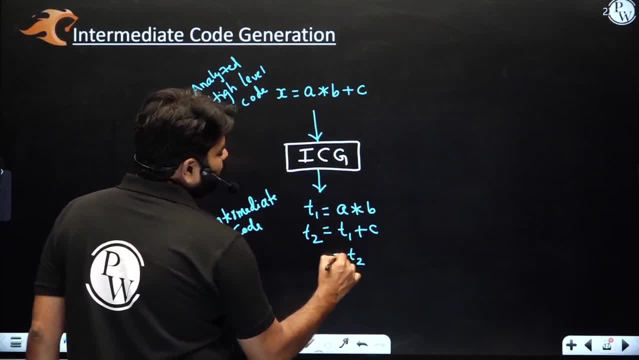 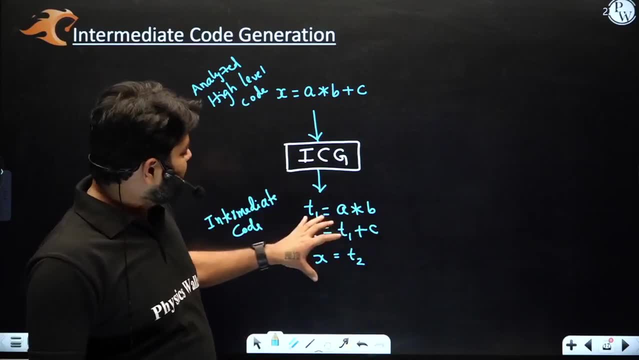 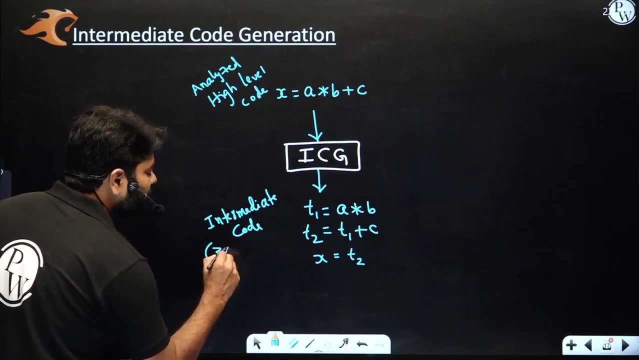 stregprogram, stregogram, ody, of some three address intermediate code and this output is example i have taken. here is three address code. three address code is also called as 3ac or you can say tac. okay, i've just taken one example here. okay, but no need to be this three address code, you can also draw a syntax. 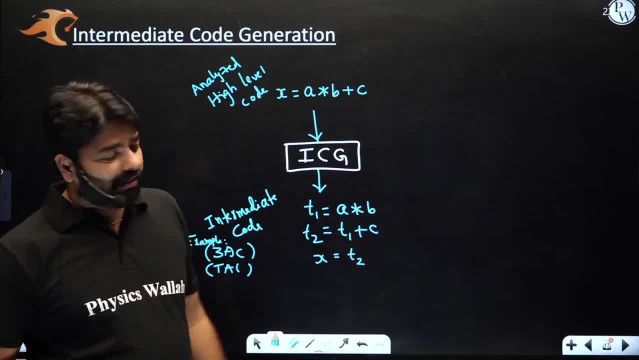 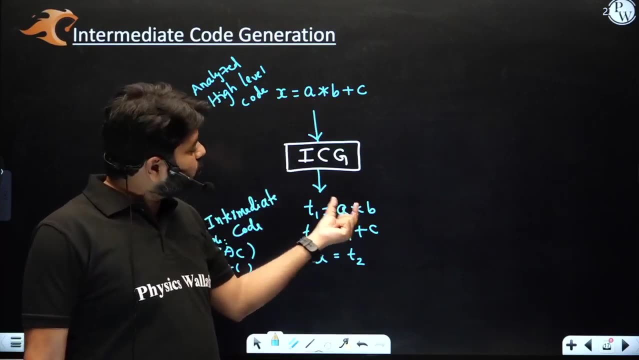 tree here. you can also do some other graphs here, control for graph, something like that. now this code can be further optimized. how see, instead of storing in t1 if really a is not used in the future, you can also store the result in a. or you can also store the result in b if a and b 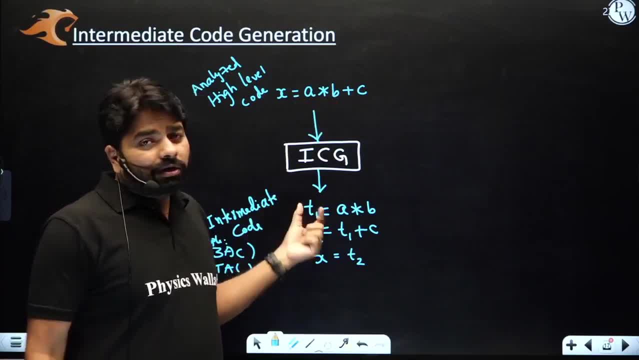 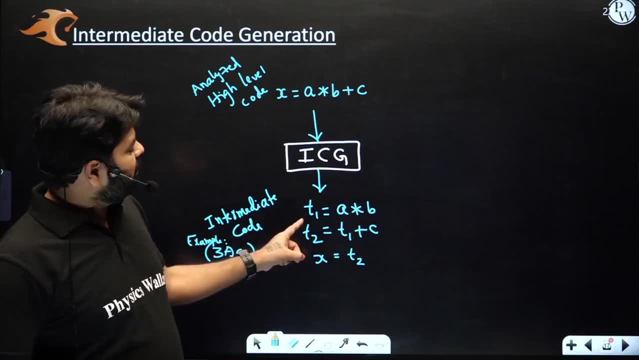 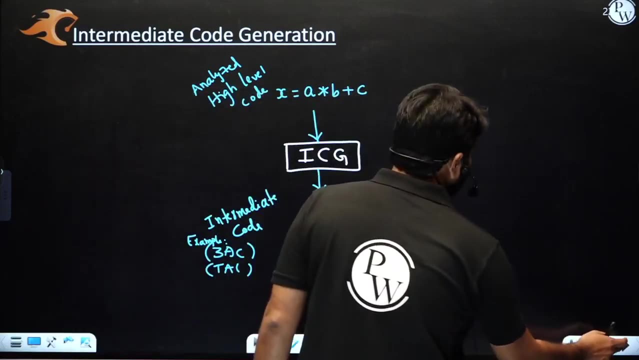 are not used. after multiplication of a and b, then you can reuse the variables. that is done by optimizer code optimizer. so i will take this code: t1 is equal to a, multiply with b and t2 is equal. t1 plus c and x is equal to t2. these three lines i'll check. 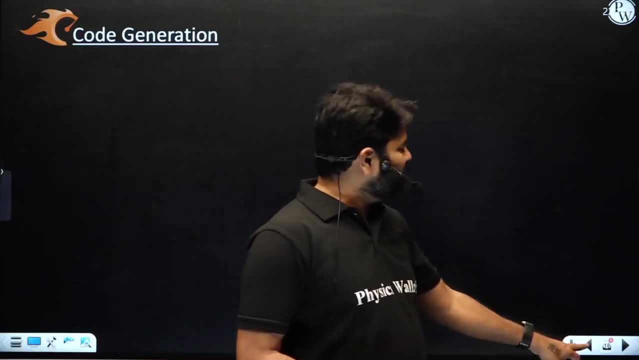 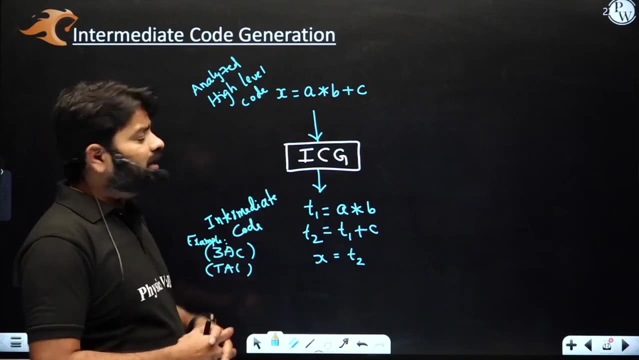 i'll- uh. sorry, code optimization i have not taken here, but let me help you here itself, because i have taken a separate topic. in case, if you want to optimize further, yes, this can be optimized. this may be optimized further, right? so i'm just dealing this as at the end. 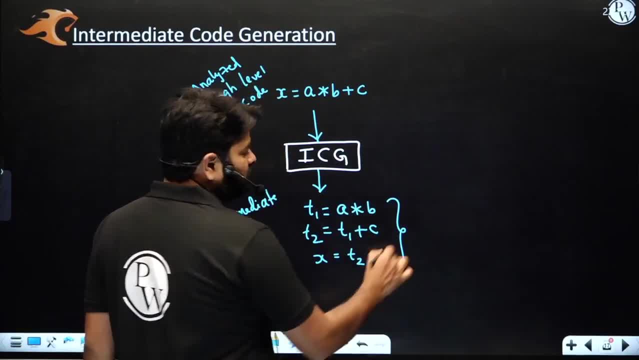 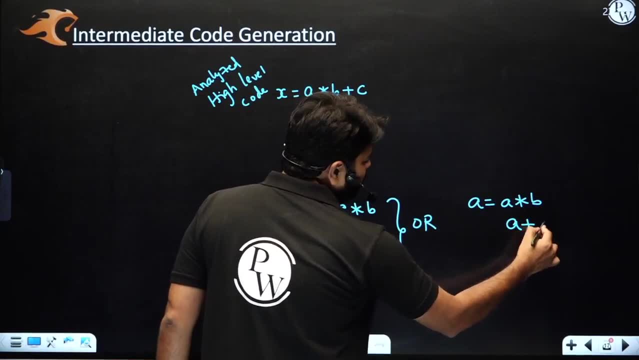 but assume in case, if you want to optimize, then how do you write something like: a is equal to a multiply with b, and then this a plus c again you may store in a in case a is not useful in the future, and that would be fine. x is now. 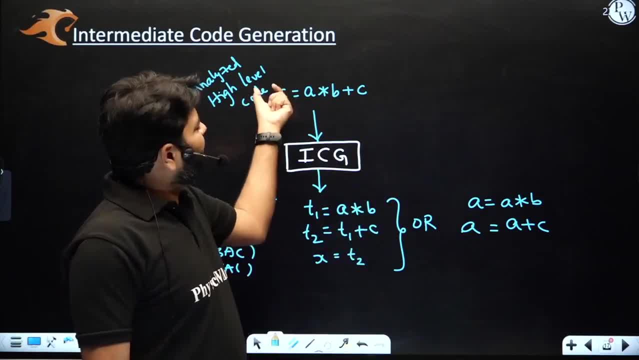 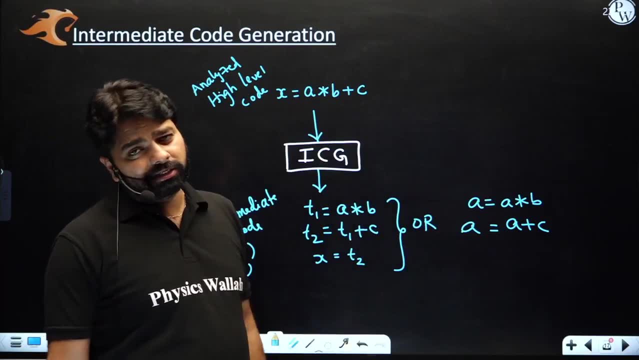 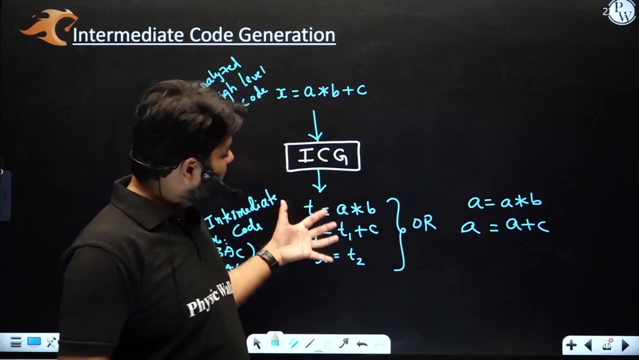 a in future, that a is, uh, not there, then wherever you want x, that that place you can use a. see just a, b, c. three variables are enough, but here you require four addresses. you are saving the space and here three instructions. here two instructions. see, the space is saved and the calculations are also. 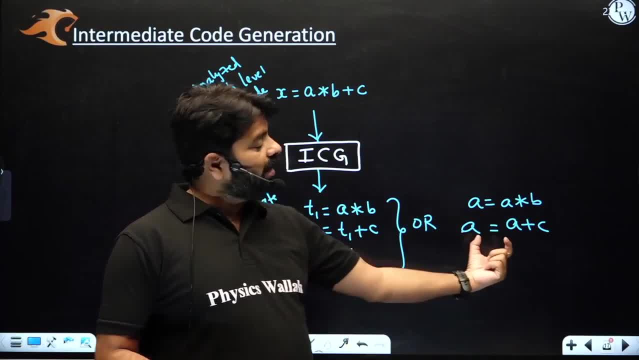 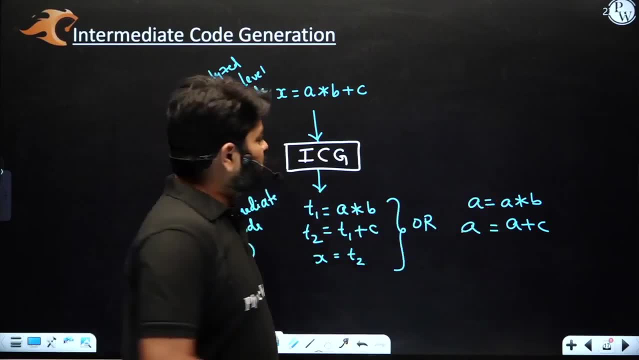 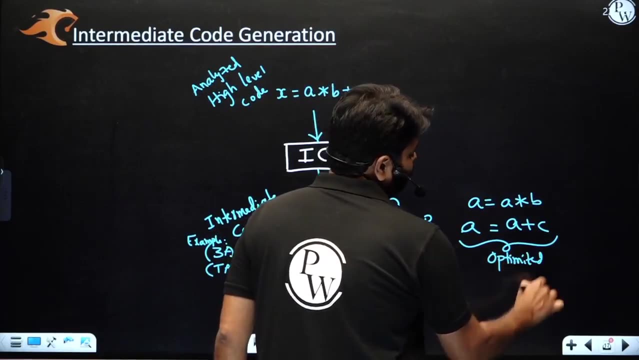 here. this is additional cost you needed moving here. you don't have extra move, so that's that's optimized version of the three address code optimized version. so in case, if you want to optimize further, so you may be considered this one optimized version. okay, that will take care of. uh, by that will be taken care by the code. 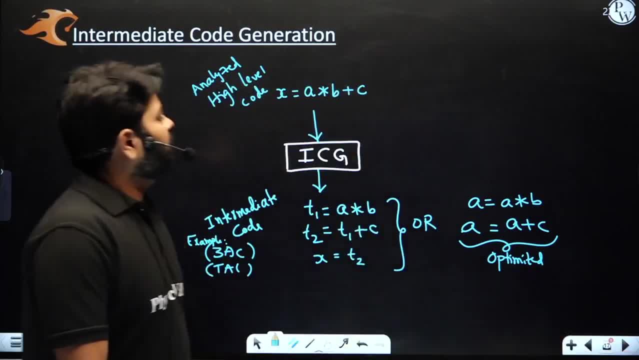 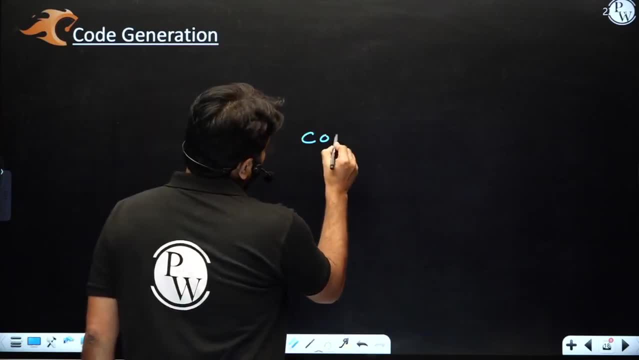 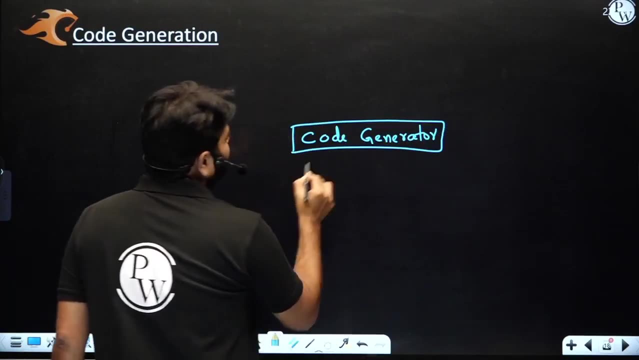 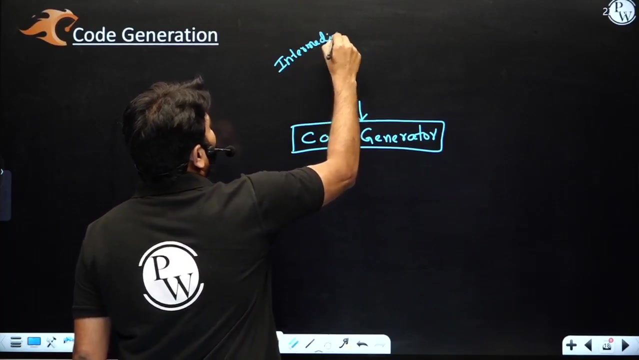 optimizer. now the code generation. when the code generation sees you got a three address code as an input, code generator or code generation, okay, what it does? it takes the input as some intermediate code, right, some intermediate code, intermediate code. so one example i have taken as three address code: 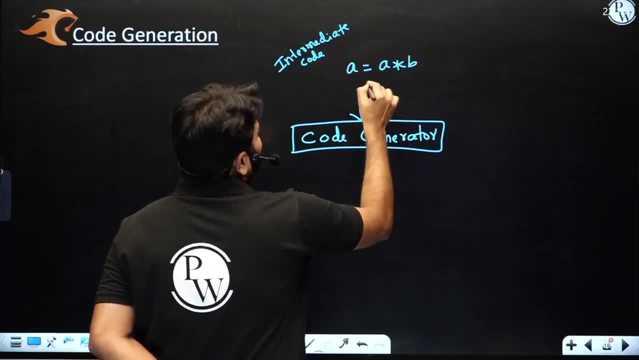 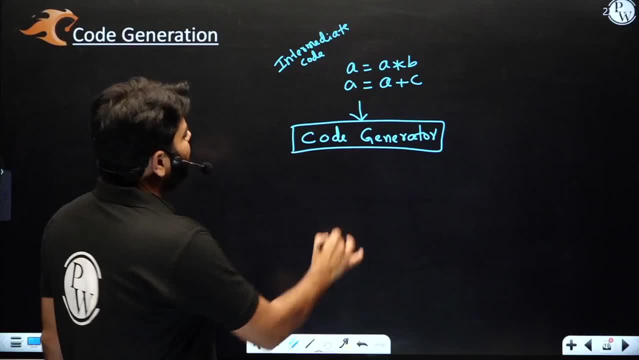 which is having something like: a is equal to a multiply with b, and then that result will be added with the c and stored in a. this is one of the possible ways to applymm指数 sendo 안에 3 number code as an input possible three address code. now, correspondingly, it will produce. i told in the beginning that it. 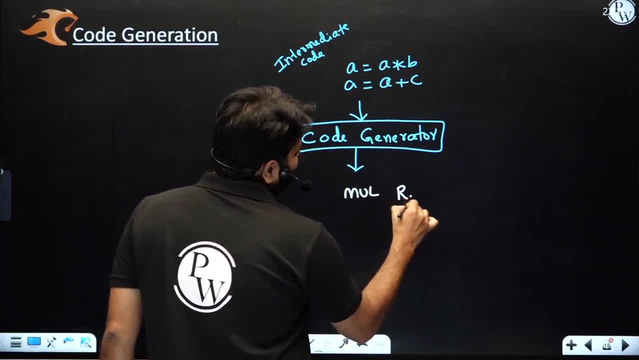 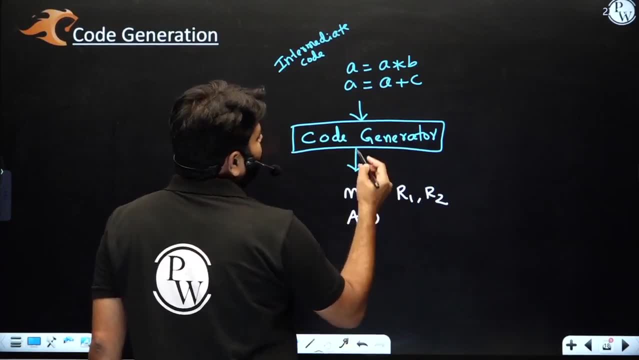 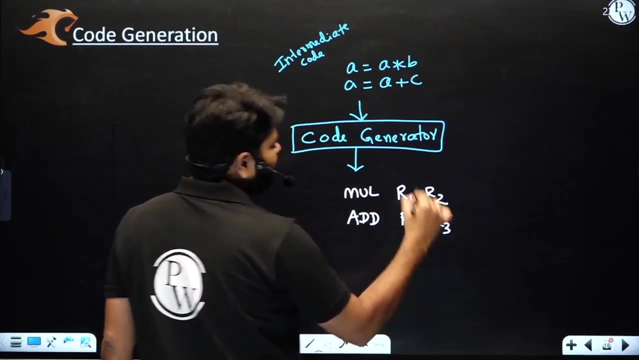 may produce something, multiplication like r1, comma, r2, this corresponding multiplication, and then you know your addition: uh, what is that? r1, the result, right, r1, with some r3, the c might be an r3. it's a corresponding a result and this is a possible uh assembly code, in case if it. 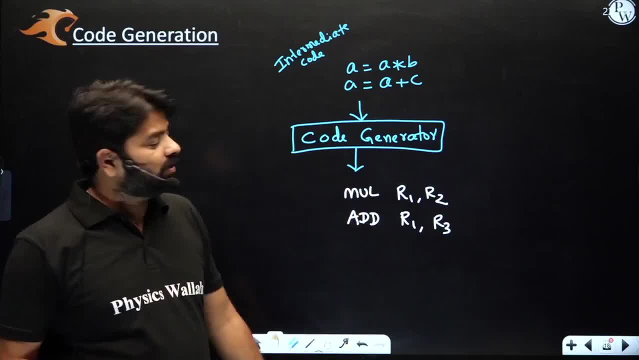 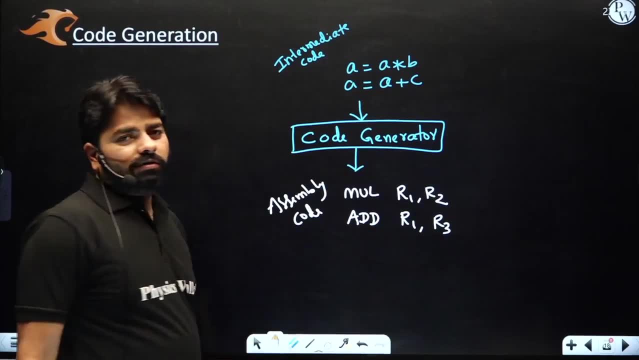 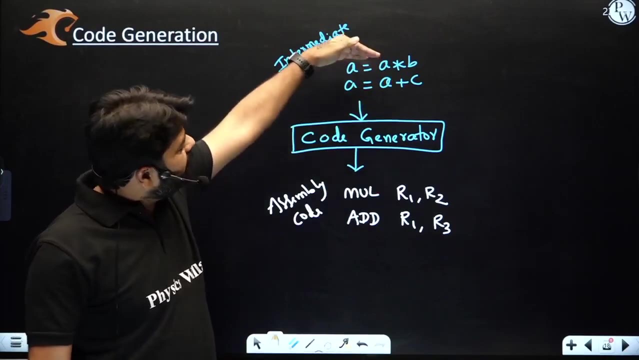 is possible to optimize, it will. otherwise it will produce the same assembly code. so this is assembly code right to do this. you know, every three address code instruction or every intermediate code instruction need to be understood by the code generator. okay, here the multiplication is there. that's why it's producing mul. 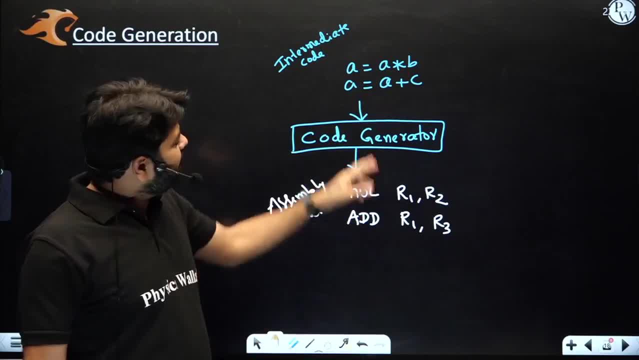 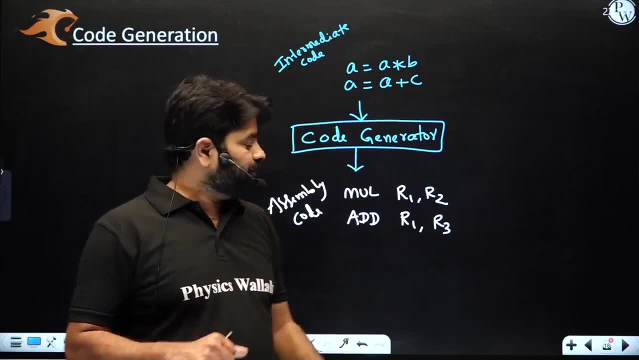 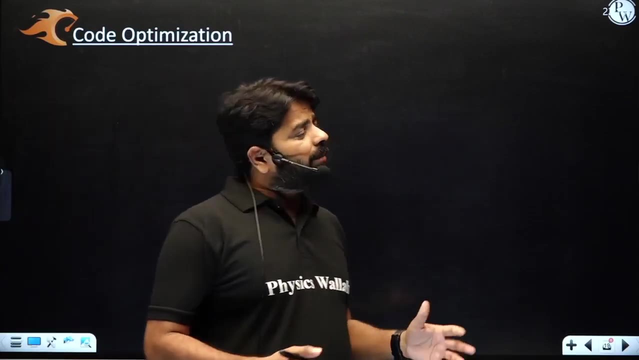 instruction here. addition is there, so it's the add in case you require extra assignment. you require a move here. so it's all understood by the code generator. okay now code optimization. that's why i told this can be used in two places: a code optimization on intermediate code, code optimization on assembly code. that can be dealt with a lot. 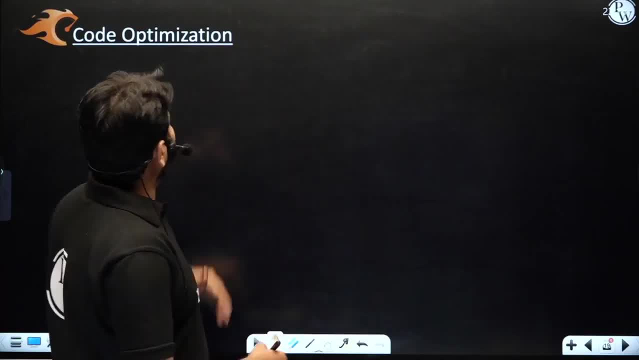 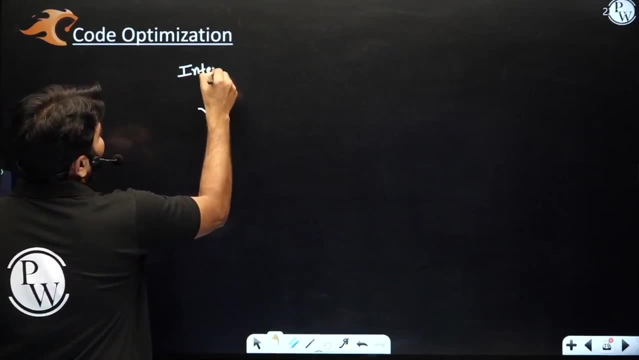 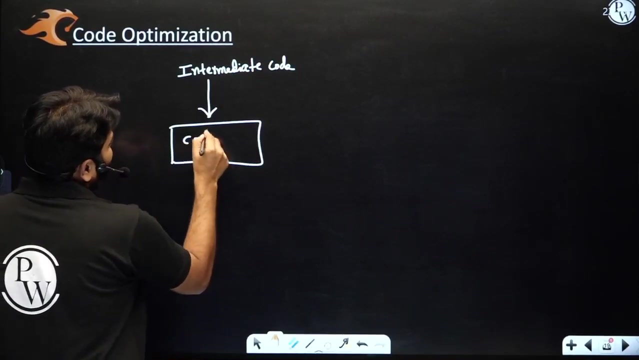 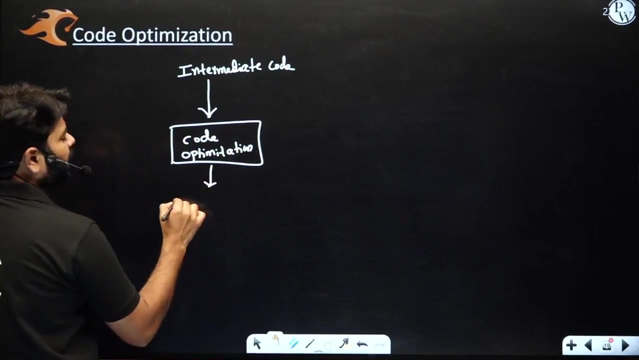 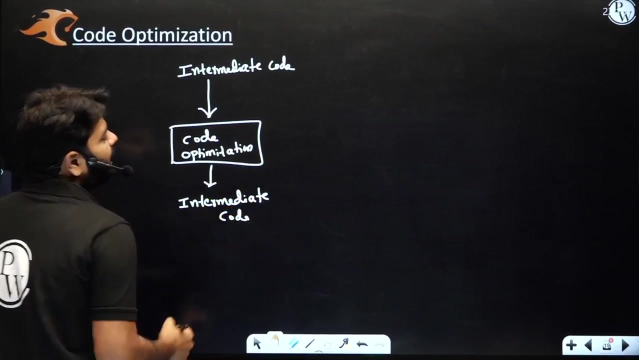 of different code optimization techniques and that we will see at the end. but there are two kinds of code optimizations: right one, you have the intermediate code level. this intermediate code will be given to code optimizer and it will produce again intermediate code if possible it will optimize right. another kind of code optimizer is: 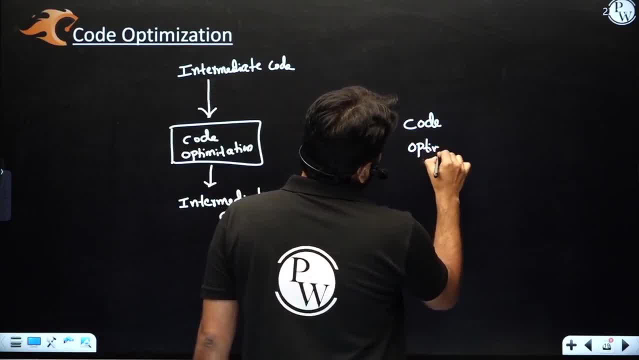 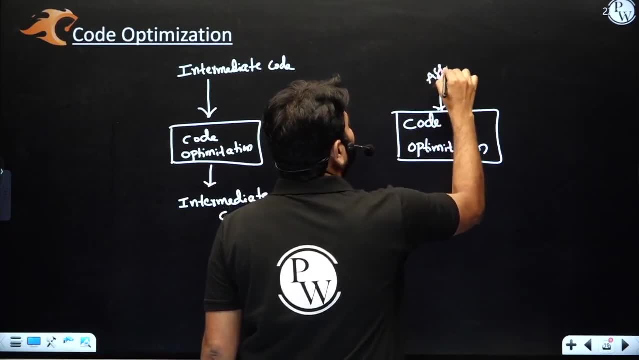 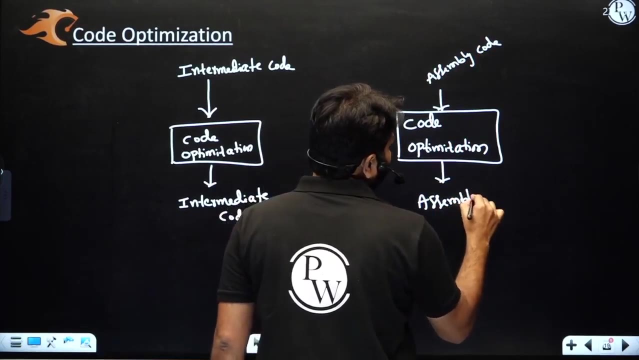 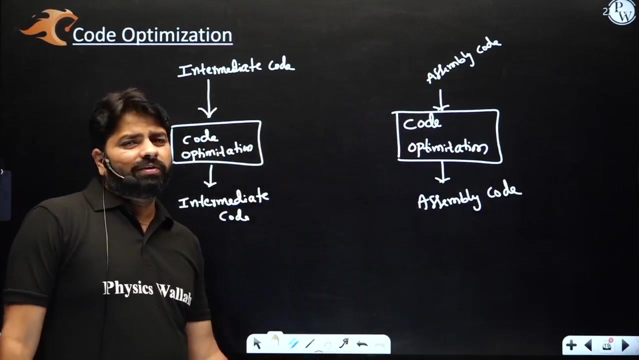 an assembly code but both code optimizations are different at the executed at different places. this will take assembly code. if possible it will produce optimized assembly code. the output is also again assembly code. fine, this is about code optimization. that will be the last chapter for us and in the last day lecture we will be dealing- we are going to deal- the different optimization. 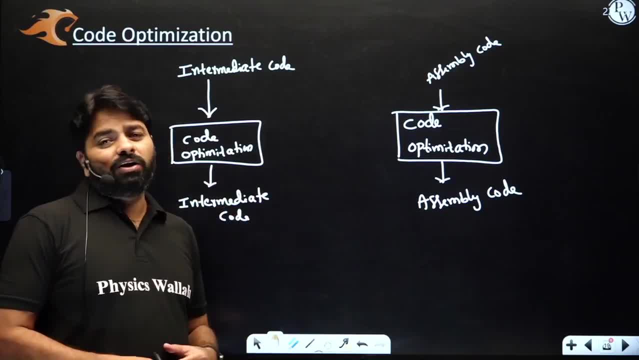 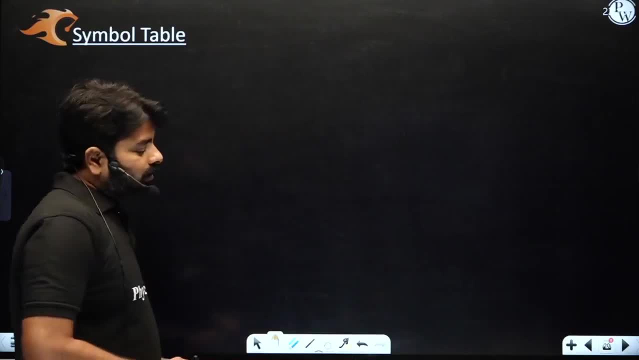 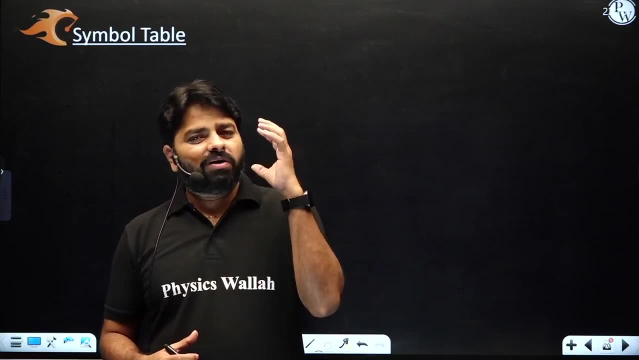 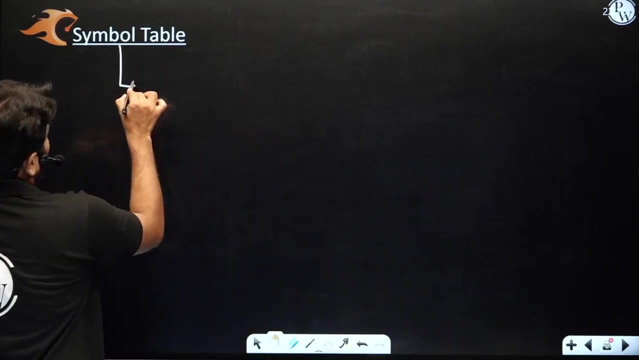 techniques at high level, at intermediate level and at a low level. we are going to see. all okay, now we have seen we have seven phases in the compiler and all the phases are going to interact with the symbol table. now, what is the symbol table? basically, it is a data structure. what is it? 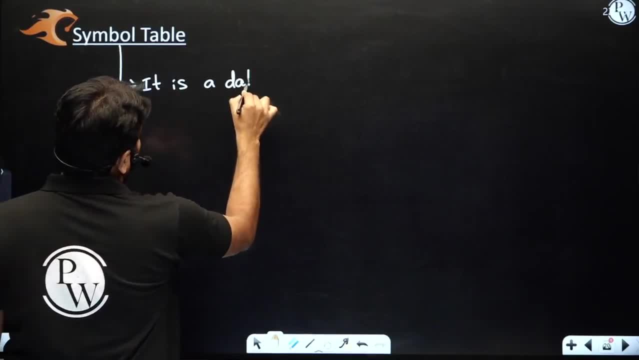 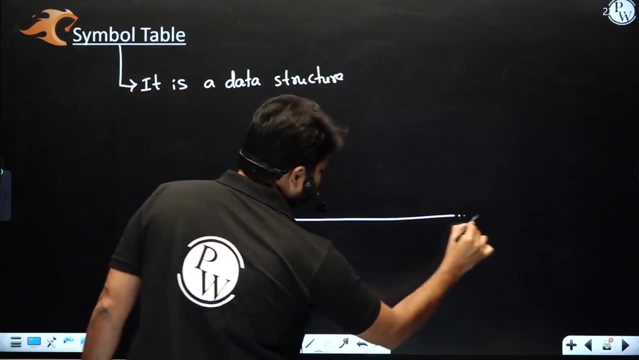 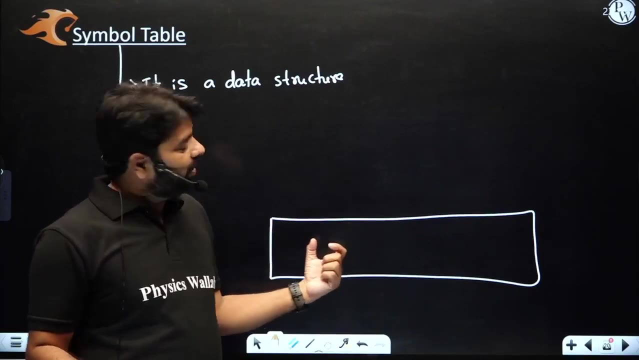 it is a data structure, only table. right, it is a data structure, it's table. okay, of course, uh, table may not look like exactly the same. it depends on the compiler: how it was um designed, like using array or using array of pointers. it might be mixed of many things. 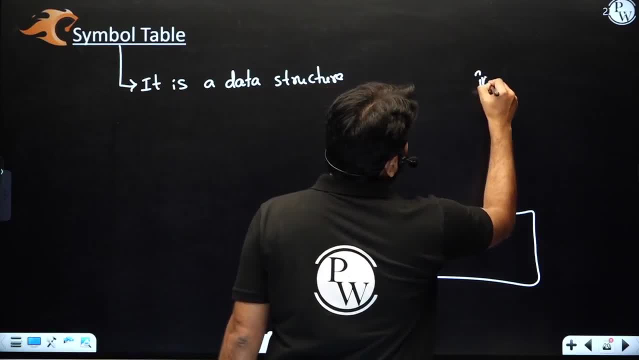 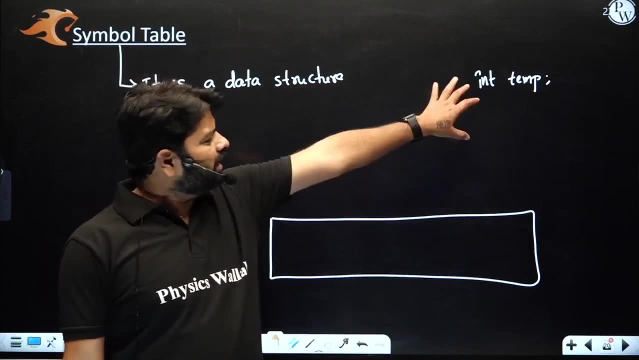 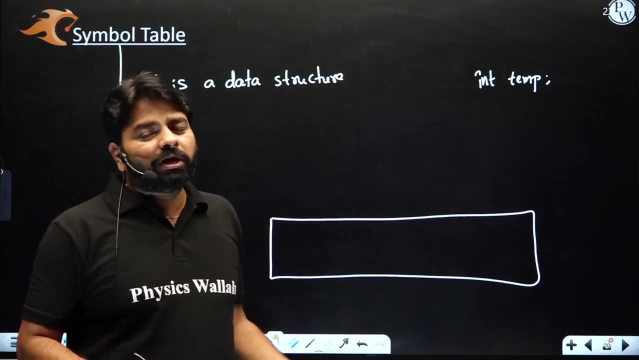 okay, when you write a program, basically, like you know, int, temp, something like that, int uh can be understood by the compiler. saying like this: one is Angular. it is int understood by the compiler, but temp also understood by the compiler. but temp is the name given by you, right? int is not given by you, it is a reserved word, so that compiler knows it. int means 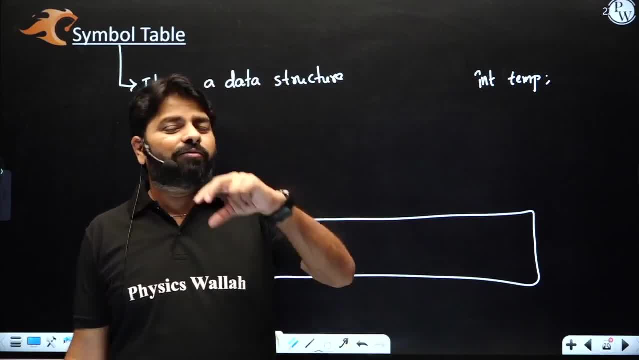 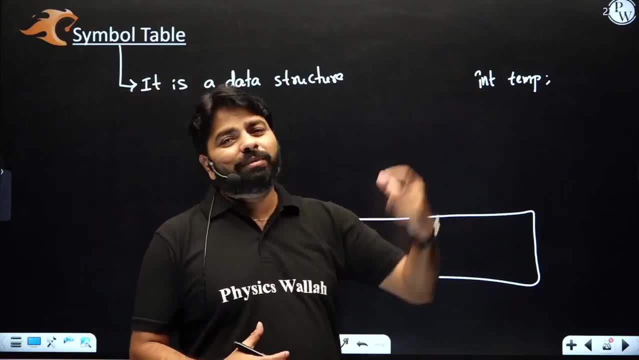 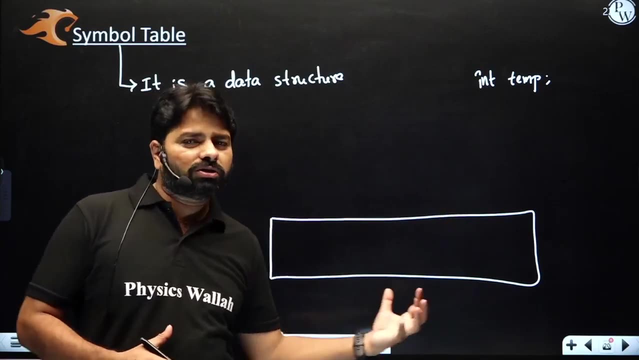 okay, int is going to mention temp is going to hold an integer with the size, either two or four byte. the type and size are, you know, decided by the compiler by looking at the int. but temp is the name, right name. you might be giving x or temp or count. you can change the name as you want. but 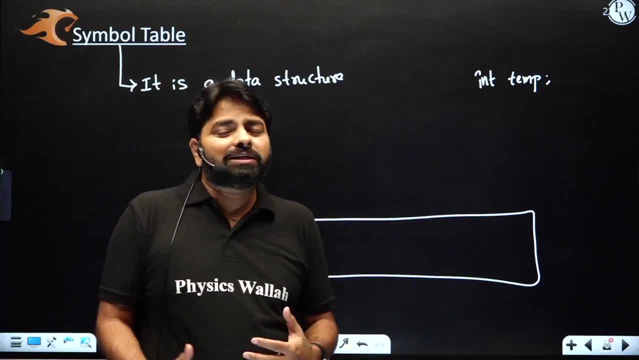 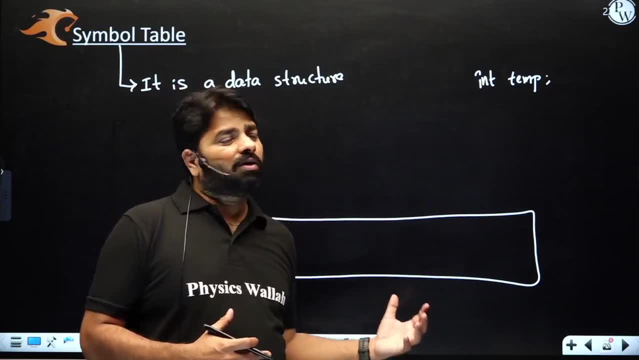 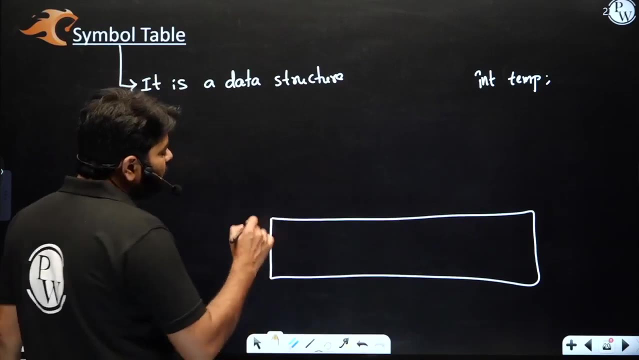 program. in the program you might be using many places this temp right. so compiler is going to analyze this temp and how many lines it has occurred and how you are using it, how long it will be useful in the future. you might be needed to optimize this variable further. it's going to. 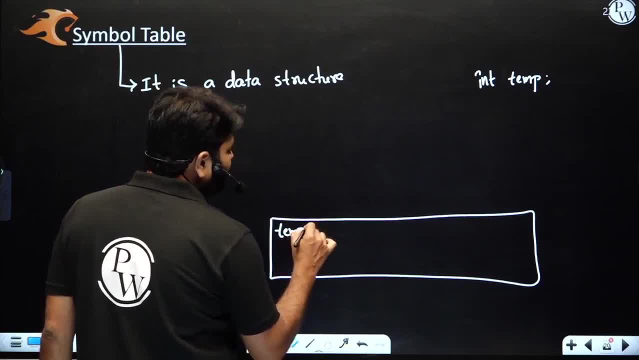 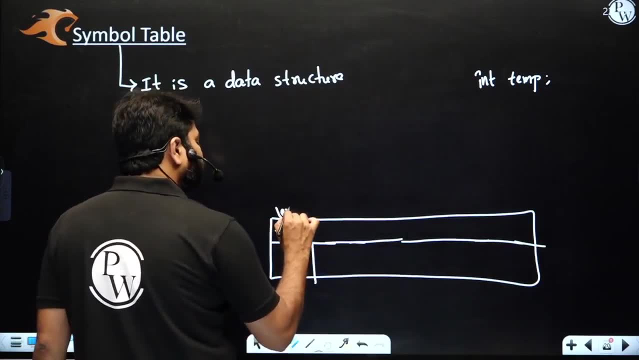 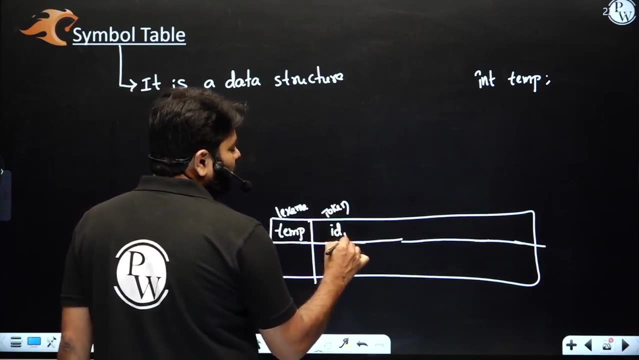 maintain: right, the temp is going to stored in the symbol table. somehow, you, it's going to store in the symbol table. the temp is actually lexin internally. it will give a different name, or let's say id 1, and it's going to maintain what line it. 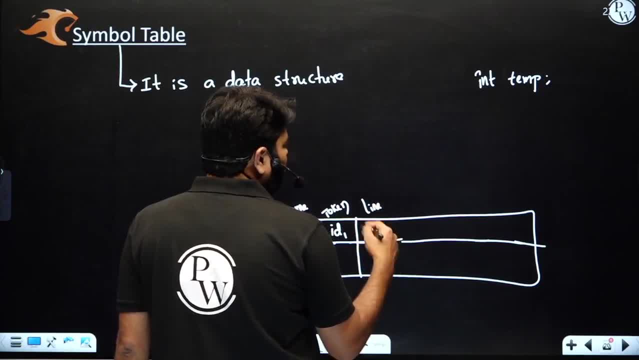 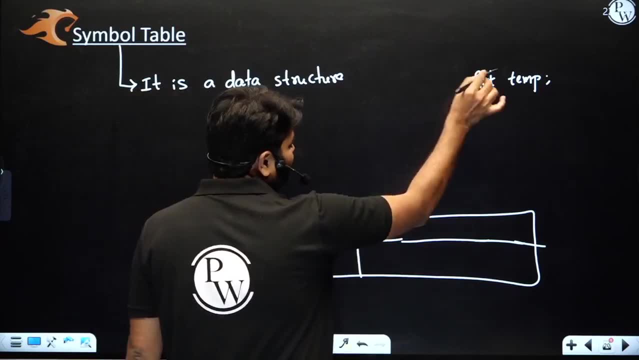 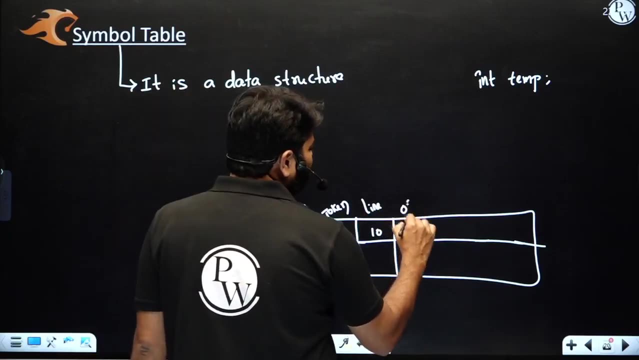 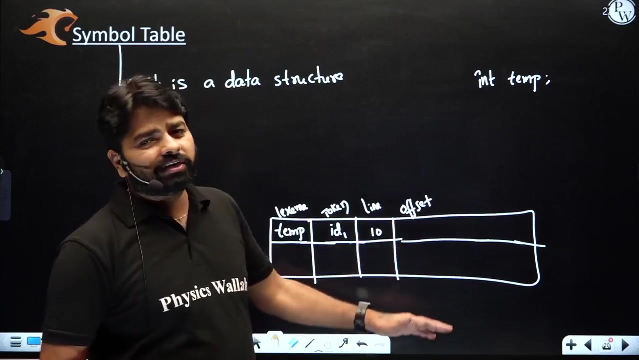 is maybe, let's say, line 10 or, you know, in future you might be getting different lines, but assume that if line maintained that line 10, let's say that number 10, it might be the instruction. this may be a maybe in future it might be using offset, this temp variable created at some offset from the function. 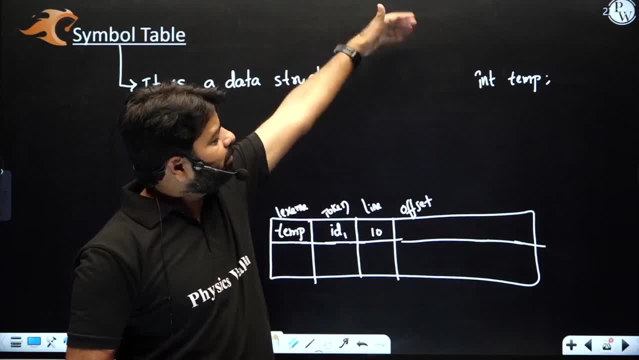 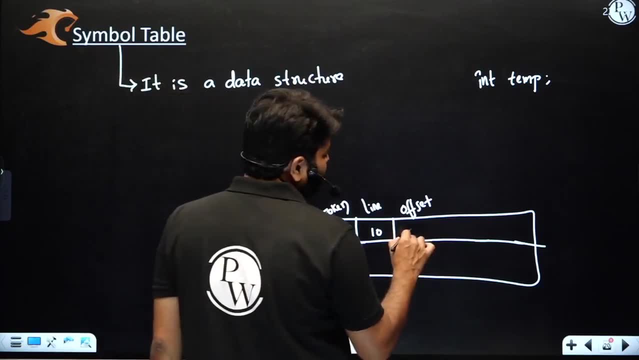 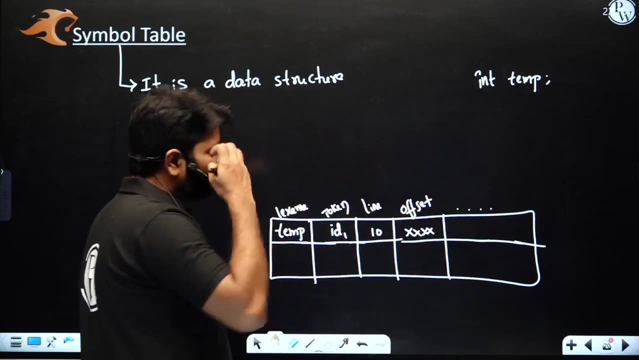 because function also stored at particular location and from that location of for this temp is declared. our temp is assigned to the particular memory location, let's say x, some location, some offset it is, and so on. there are many things to optimize further. and what is symbol table? 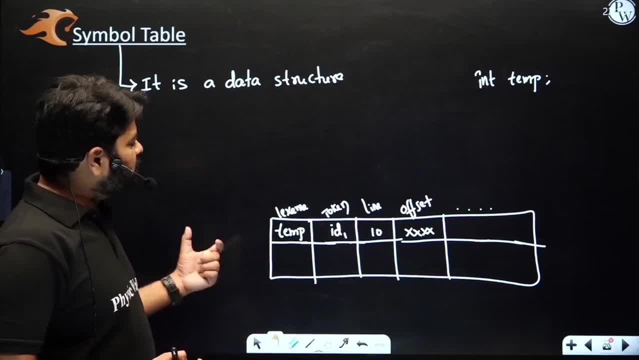 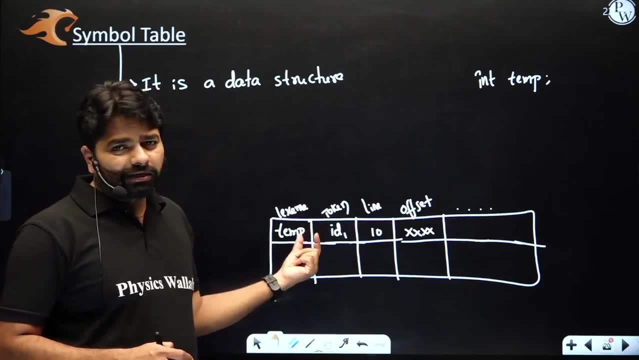 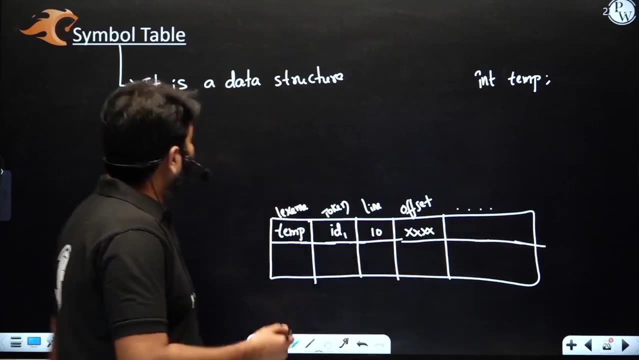 basically it's a data structure. it's going to store the attribute information of the token. so if there is a particular token, right our identifier, you can say this identifier even for the function name also you might have an entry here. so it's basically the symbol table, those. 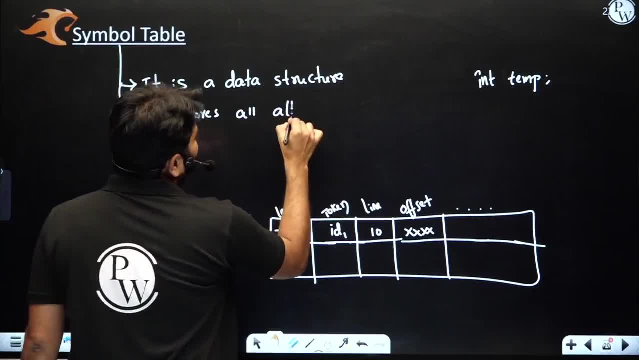 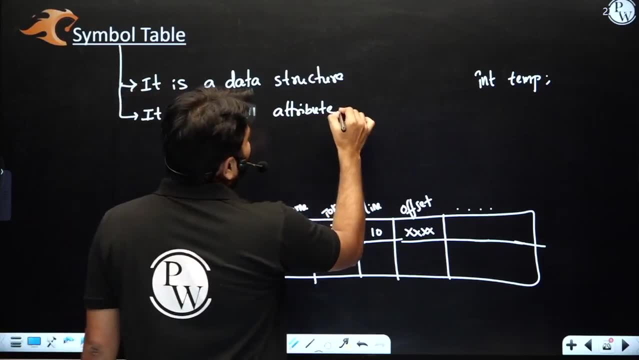 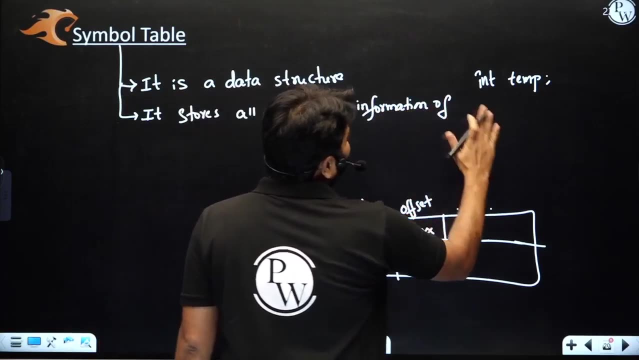 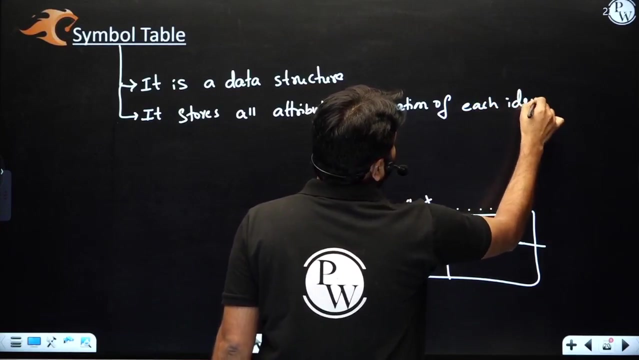 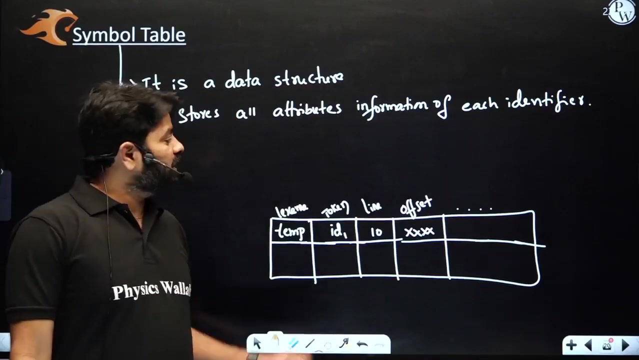 all required: the attribute, information attribute- basically we say column, right, so every column has the different name that we call as attribute. all attributes information of an identifier, of each identifier, let's say in the program, is the main purpose you require, the main purpose you require, so that the lecture analysis, it will throw the token in syntax analysis, may be line. 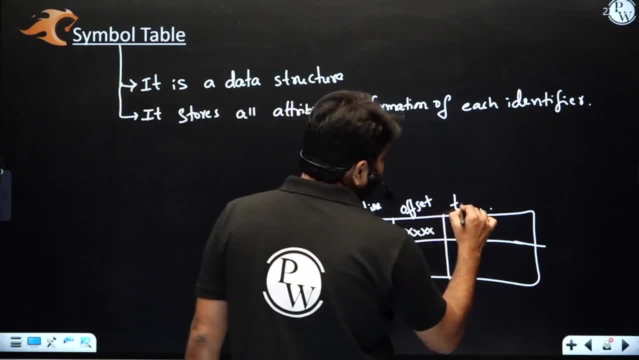 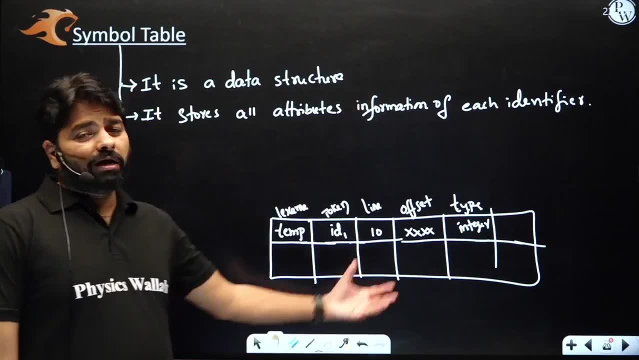 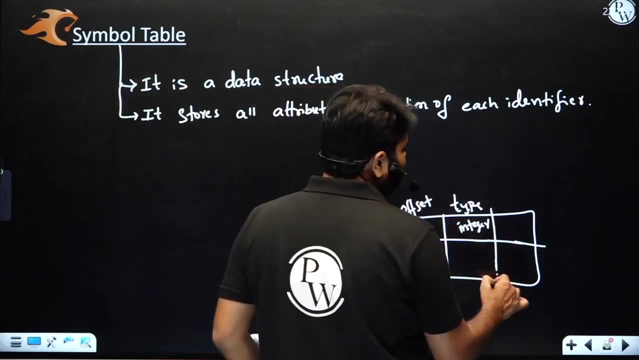 number in semantic analysis may be type, what type it is, let's say integer. in intermediate code generation may be offset in code generation may be address or register location. that's exactly where do you assign it. many things right, every phase you require, like in code optimizer, maybe this temp: 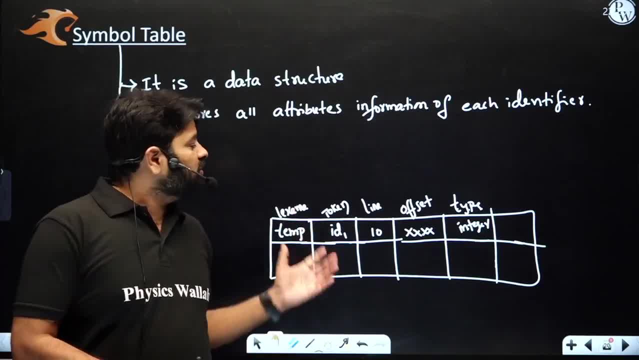 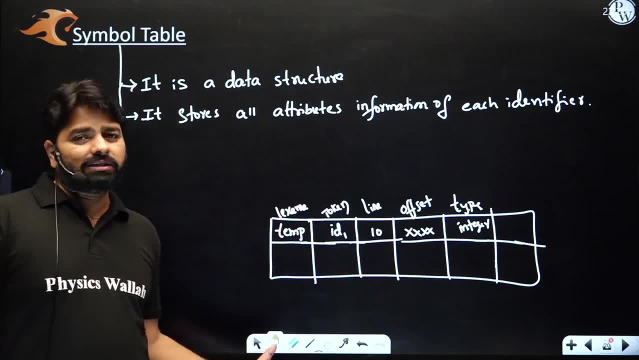 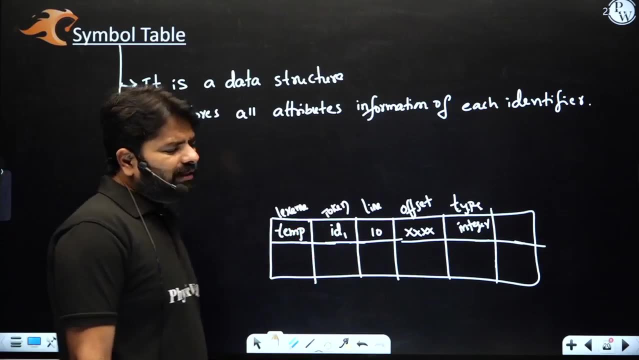 could be replaced with some other variable or other addresses, so it's going to be maintained in the symbol table. okay, the symbol table is going to help to analyze the code in various phases in the main purpose of the symbol table. in the in the previous gate exams it was asked like what data structure is. 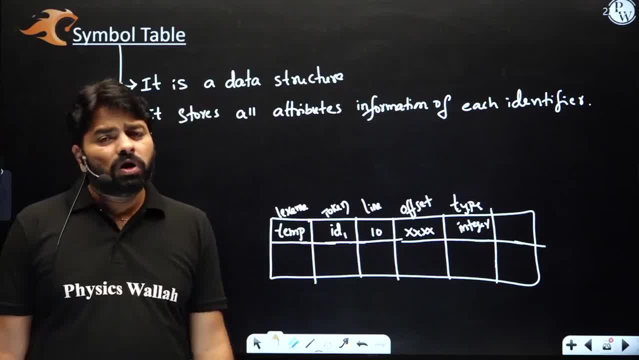 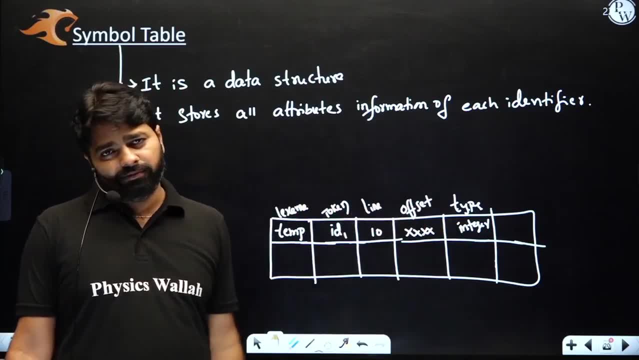 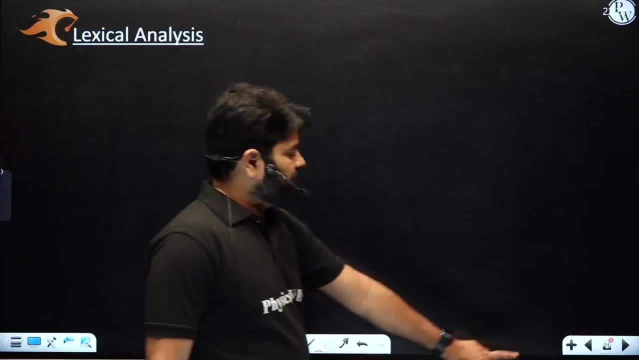 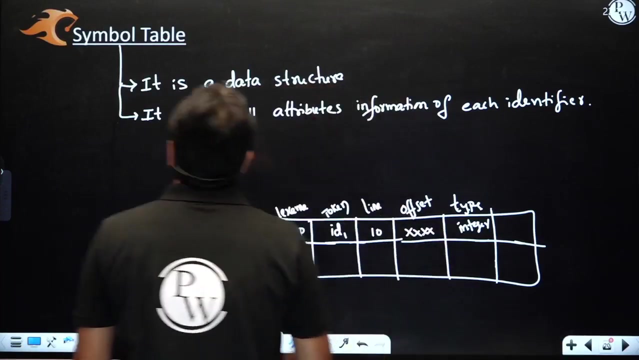 used in compiler. they have given one of the options: symbol table. so what is a symbol table? right, it is a data structure that stores all attribute information of identifier. okay, now, before going to the next topic- right, the first topic, let's analysis. let me tell you errors, because you have error handlers right in the errors. we have the. 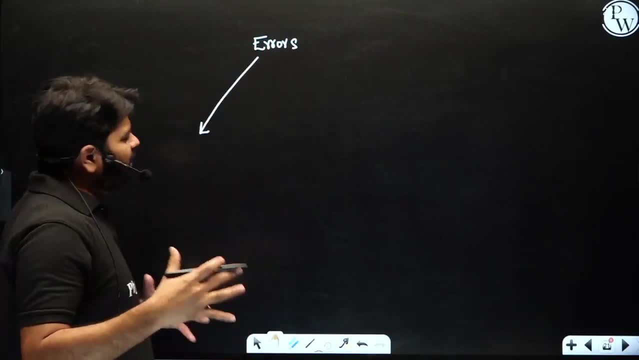 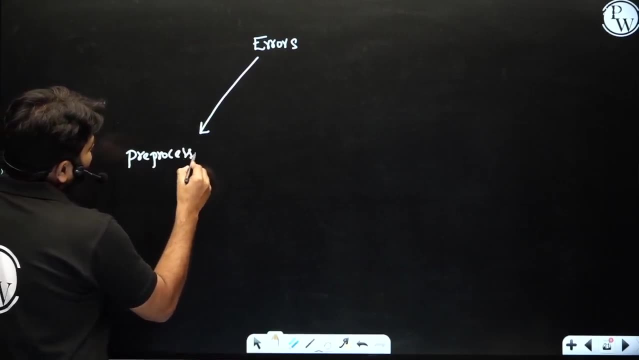 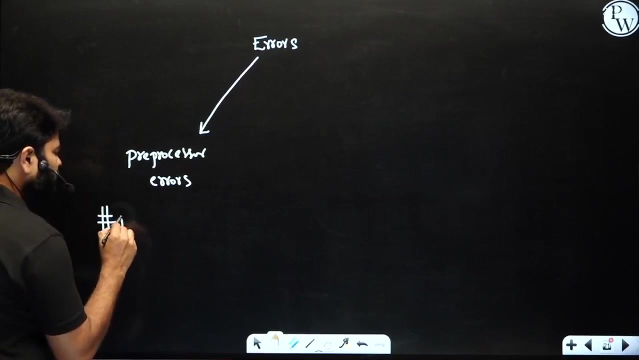 lot of errors. it means at every stage you may get a different kind of error. one kind of error is a pre-processor error. pre-processor can also produce errors when, when it produces, you have written Ash, you have written something like include and you have given space as much. or you have written something like 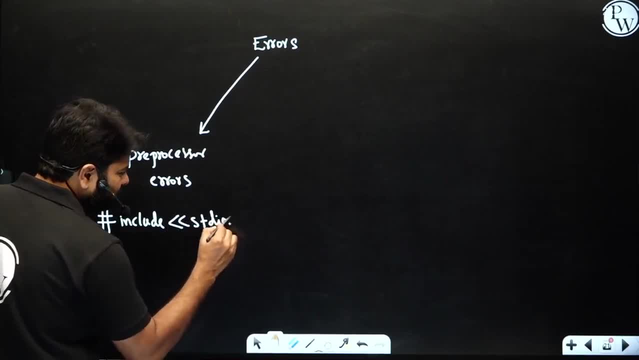 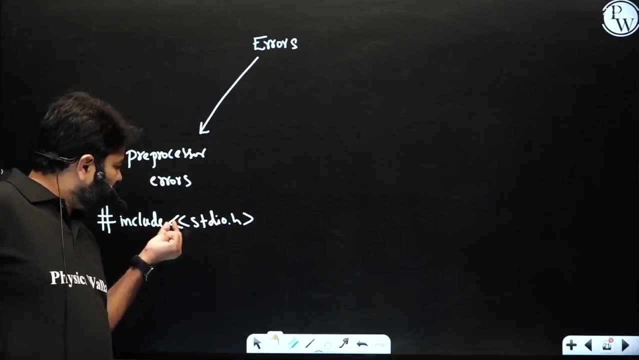 STD. ioh, see, it's not the actual right, actual come. it's not the command. if it is pre-processer command, here should be one here less than symbol, here greater than symbol. do you have written here two less than symbols? here preprocessor will produce an error. it's not the preprocessor right command. actually, ash tells us, tells the compiler. 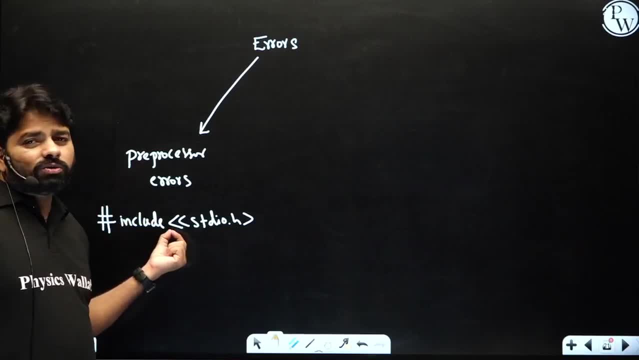 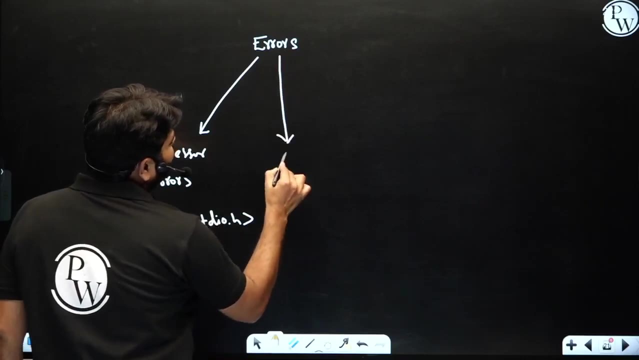 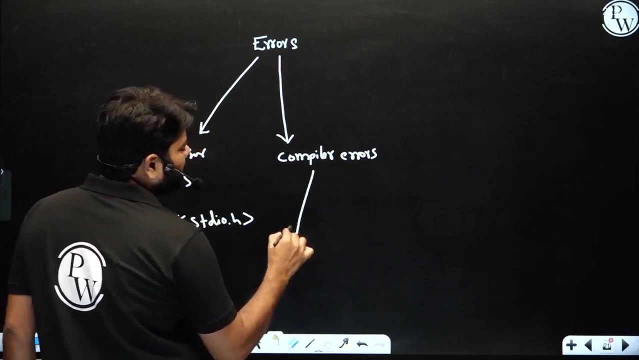 that it is your command when the preprocessor trying to analyze it shows that there is something wrong with this command. so you have to verify what mistake it is. so even include the spaces, many here, it will produce the preprocessor error. other errors are some compiler errors specific to compiler phases. they are maybe lexical errors. will see in the 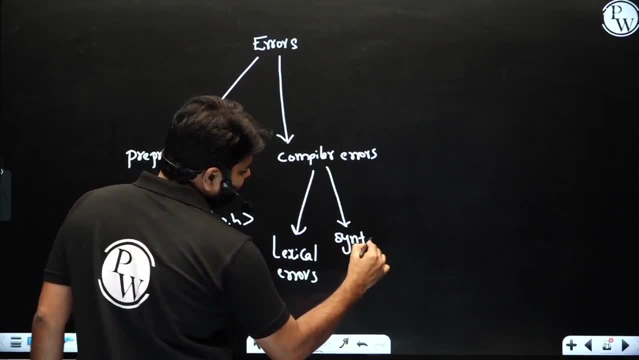 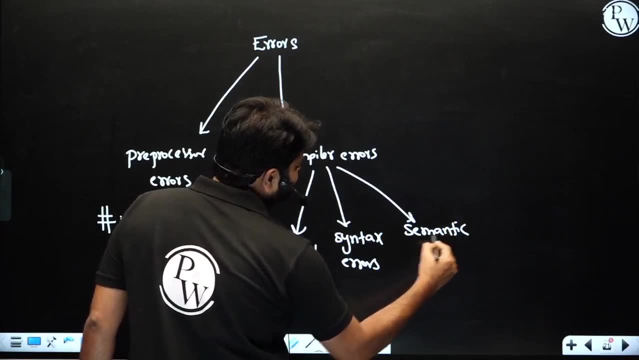 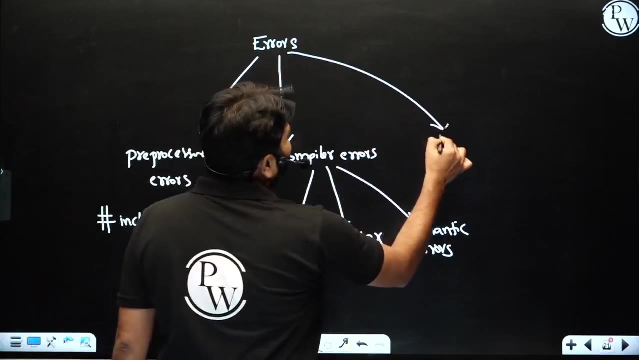 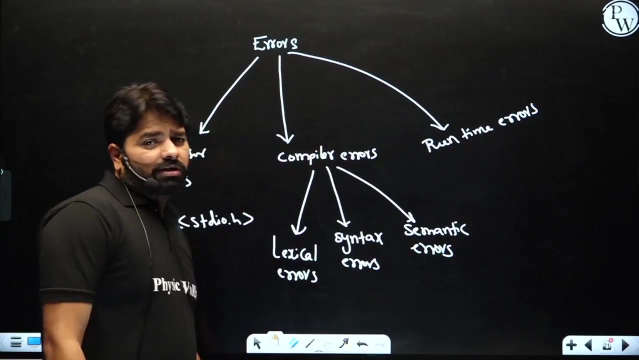 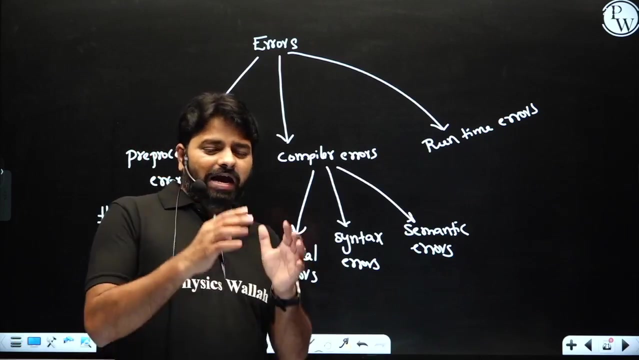 lexical analysis may be syntax errors will see in syntax analysis there could be semantic type related errors. type mismatch errors mean compiler errors. some errors are runtime errors. during execution you may face a runtime runtime errors like divide by zero error. or you are accessing an element which is outside the array declaration, like you declared as a of 10, but the 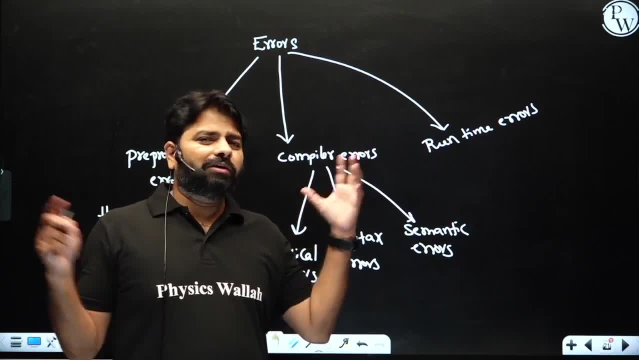 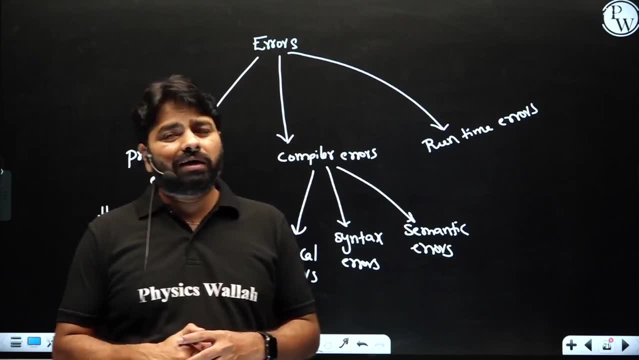 even you declare a of 10: 0 to 9 only accessible but you're trying to access out of bond, then you may face runtime error. or you are dealing with the pointers and you are trying to deal with the wrong addresses. then you may see the runtime errors. 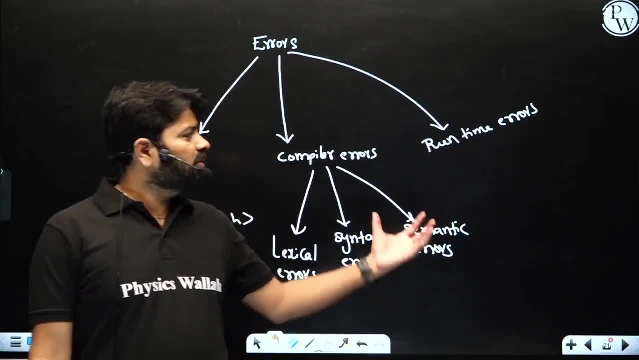 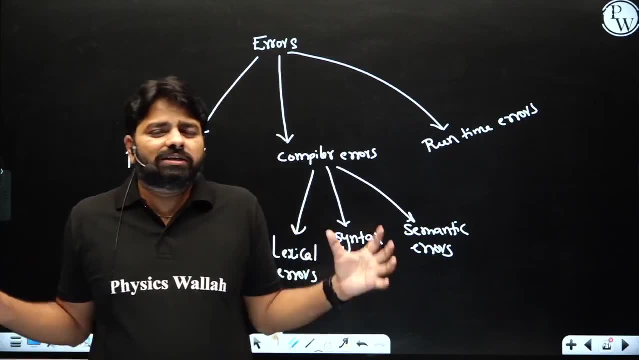 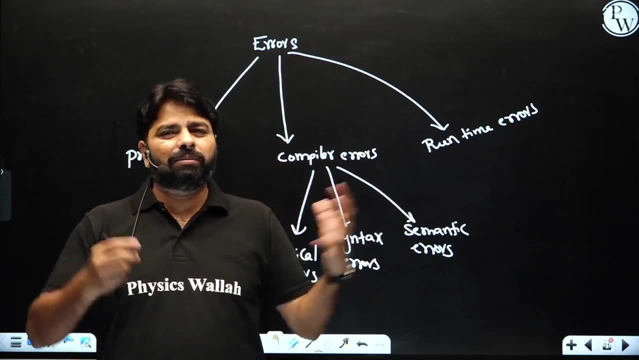 okay, that many runtime errors? definitely we're going to see them at the end. now, uh, with this we have uh understood just what is a compiler, what is there inside the compiler and how many phases are there in the compiler and how they are going to interact with the symbol table and error handler. 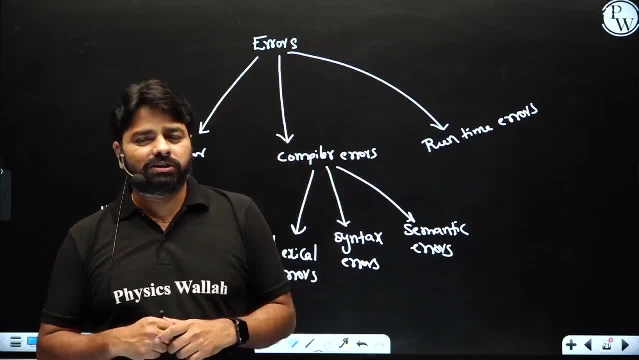 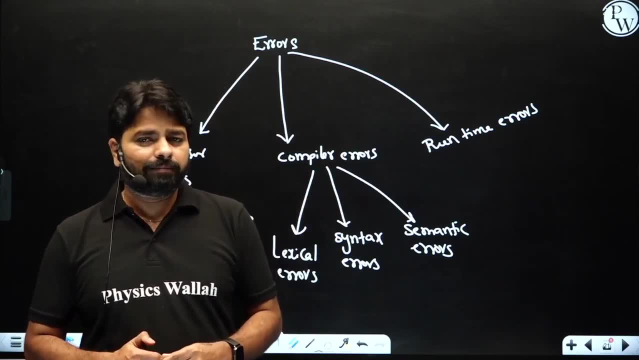 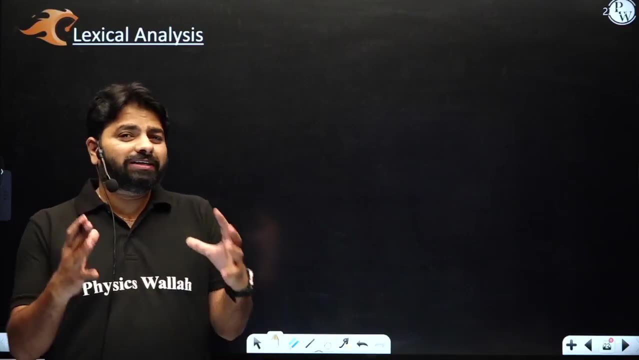 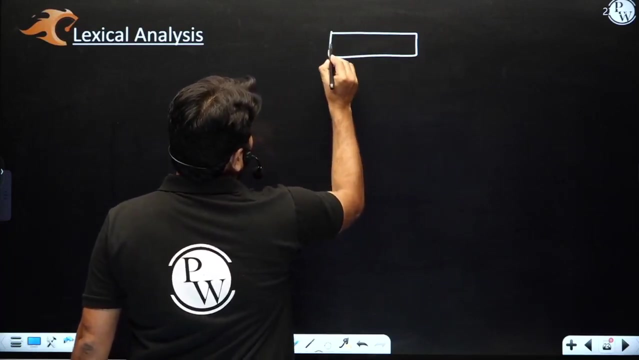 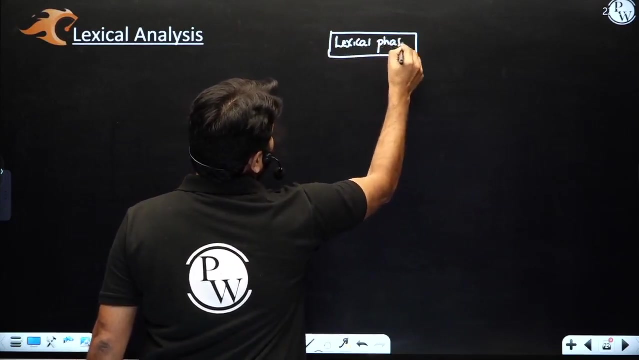 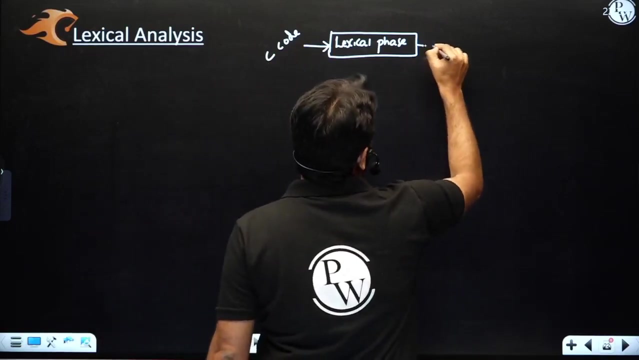 to do the compilation process, and now the first phase of the compiler is the lexical analyzer. right, let's begin the lexical analyzer. we have already know what is lexical analysis. what is lexical analysis, lexical analysis, what is the lexical analysis? it takes the C code or high level code and it produces the sequence of tokens. 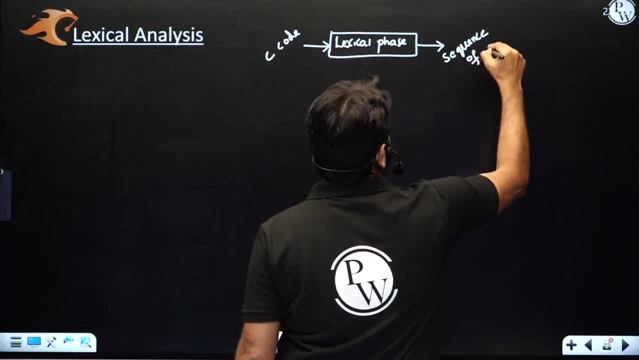 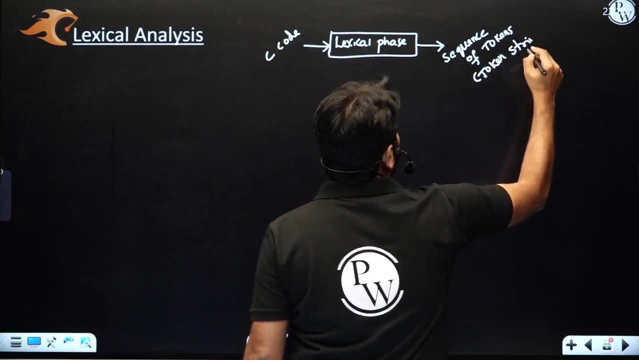 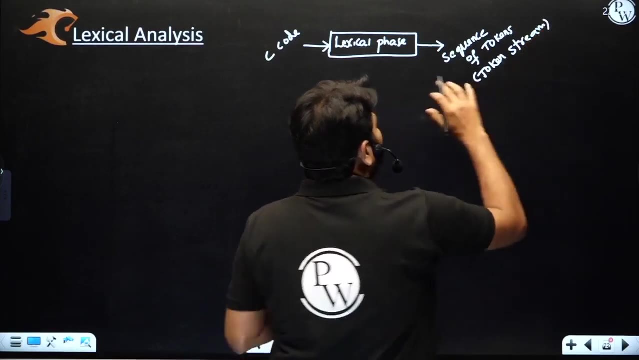 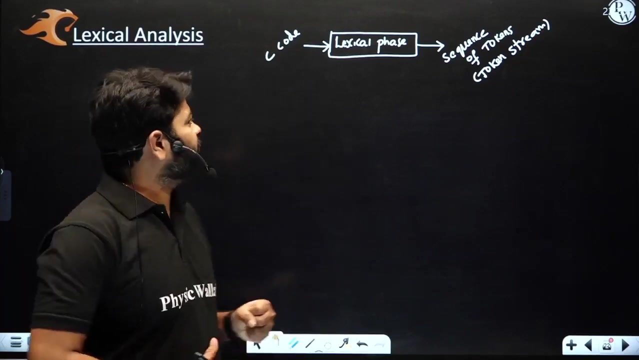 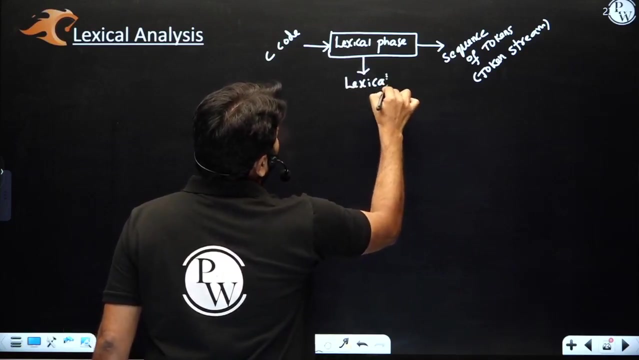 and stream, basically sequence of tokens, also called as token stream, or simply just a string of token stream. just it looks like a string, whole program converted into one small string right by introducing the tokens. if there is any error by this, it will produce lexical error, it will report the error handler and error handler A main until the errors, or it will report to the 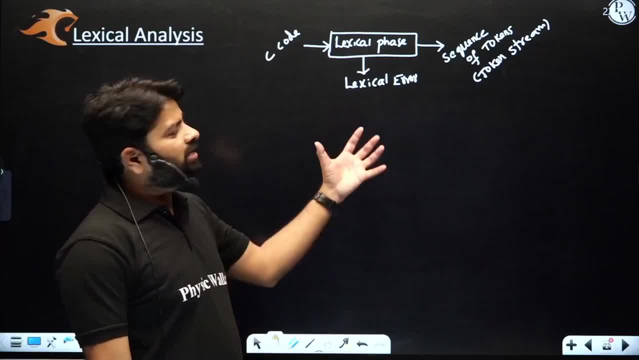 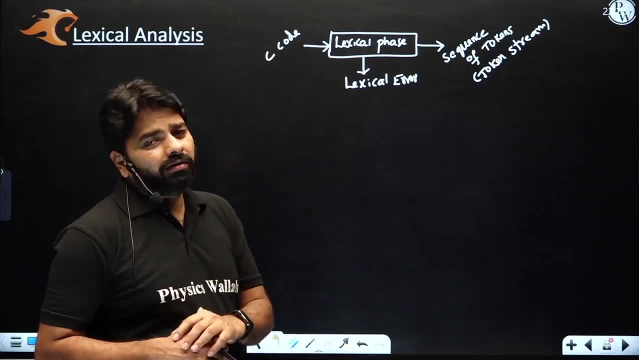 programmer. these are the errors happen. you give the facility to the error handler. it really you wanted to correct the errors through the program. you can also do certain uh errors handling with the help of error handling programmer, a program, and also you have a symbol table whenever you. 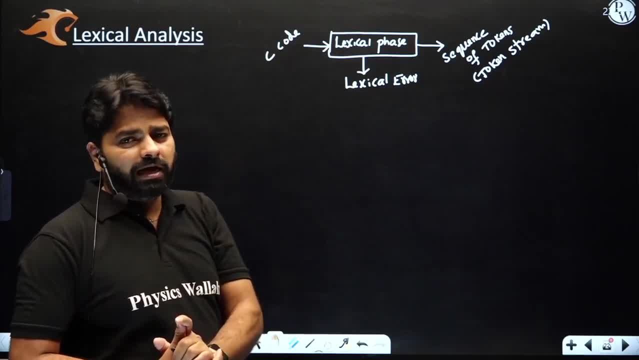 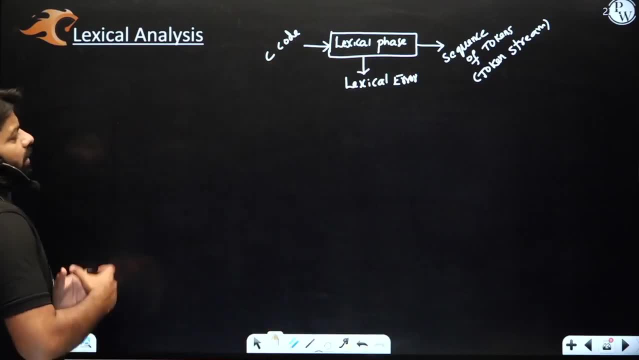 detect or whenever you see any identifier which is first time appeared, then you can put in the symbol on. you refer it whenever needed. okay now, uh, this is the main part of the lexical phase. what it does right it. the first thing is, when it sees the c code, it's going to group the characters and 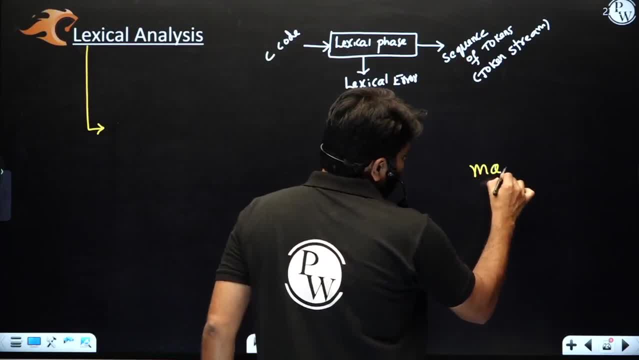 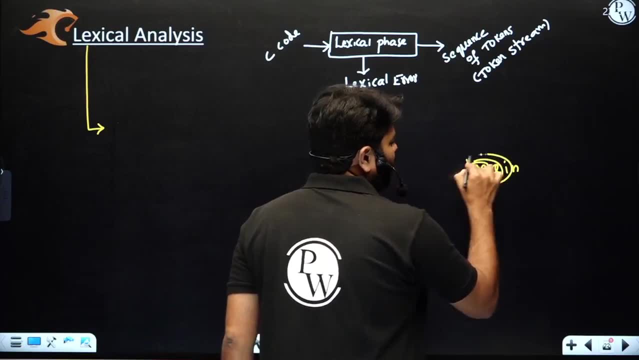 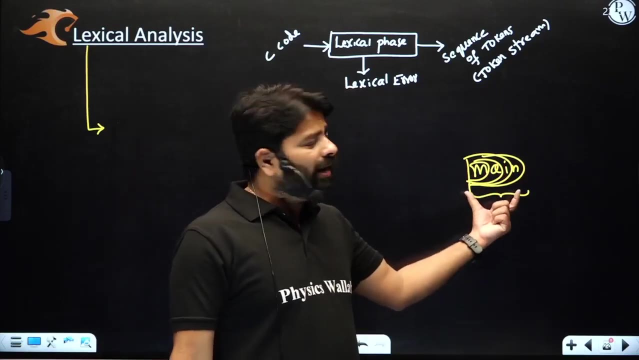 converts into token, like whenever it sees m, a, i, n, the four characters, right, it's going to group, like it starts somehow. it groups m, then a, then i, then n. okay, it knows somehow, using with the help of finite automata or regular expression, with the help of patterns, the main is one token, which is: 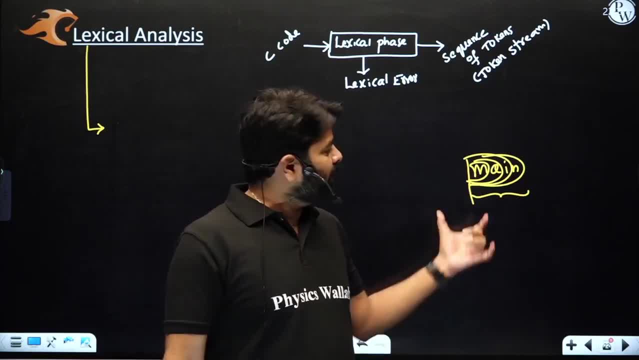 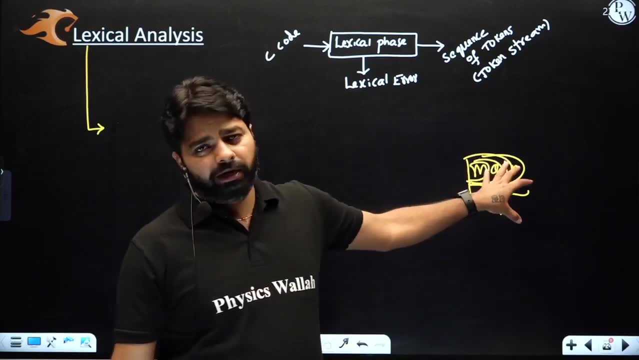 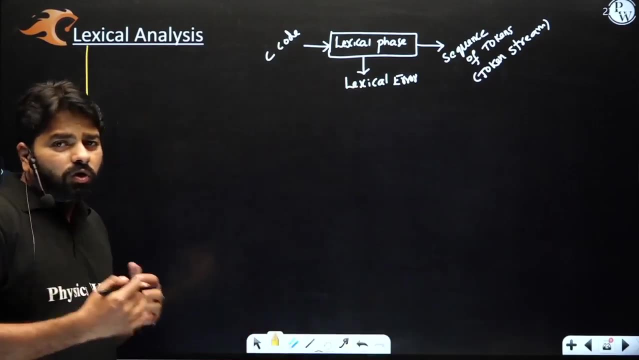 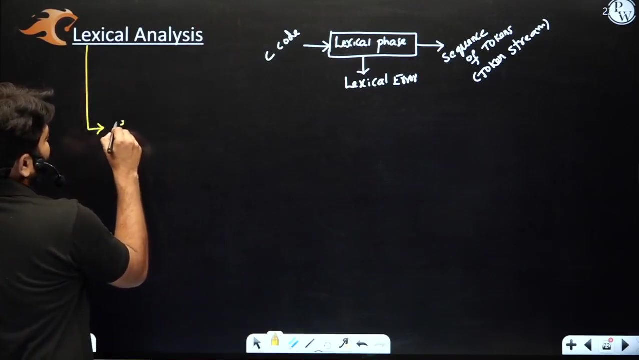 identifier type. so id1 might be generated for the main, because it's not a keyword, it's identifier. so maybe id1 is a corresponding token name for the main. so this will be a produced by the lexical analyzer. so it's going to you group the characters into a token. so the job of lexical analyzer is, uh, scans. it scans. 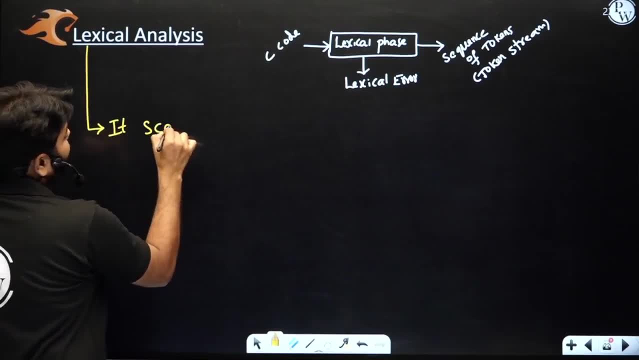 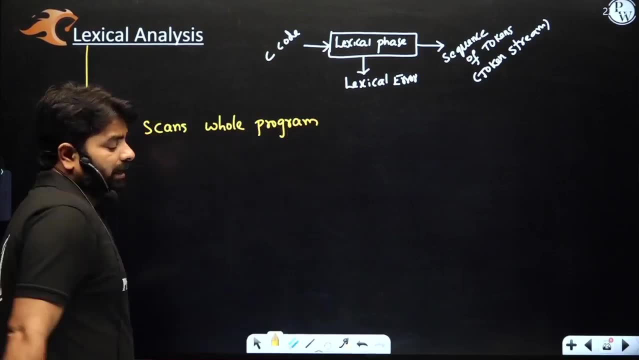 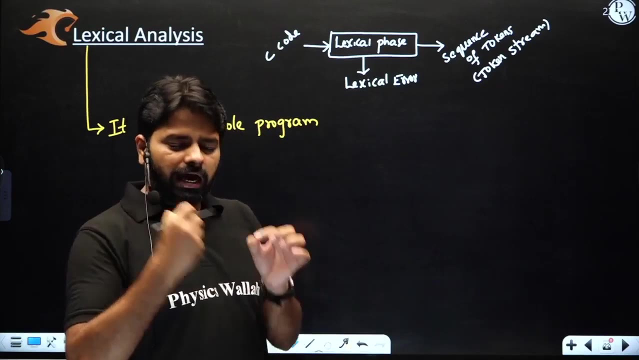 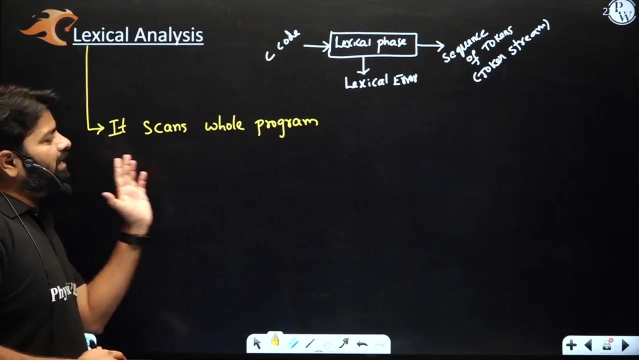 whole program without leaving any character. it scans all program. remember, it scans all program. it can't ignore even single character. of course, to generate it may ignore, to scan it will not. it has to reach every character of the file, from first character to last character, without ignoring. it scans old program and what it does. 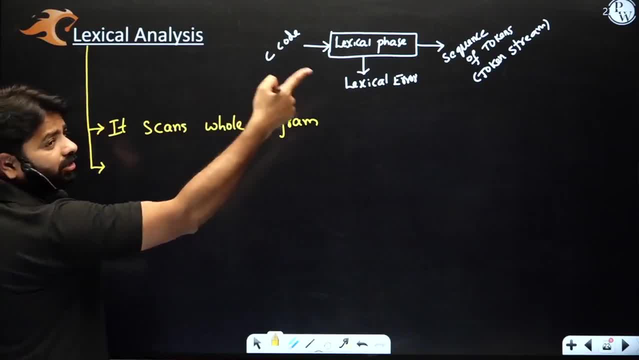 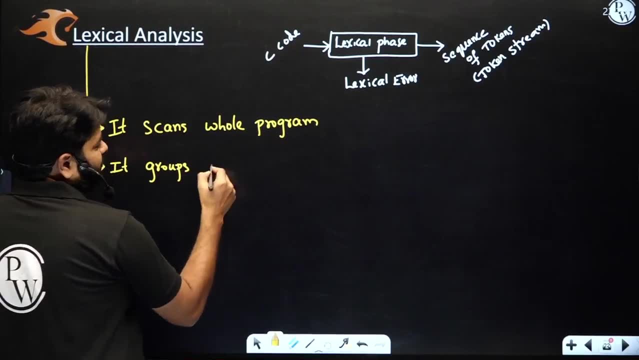 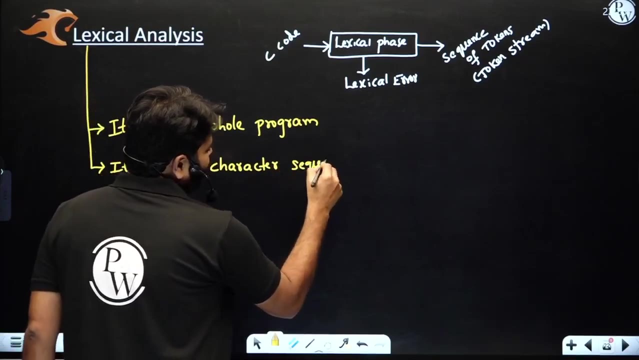 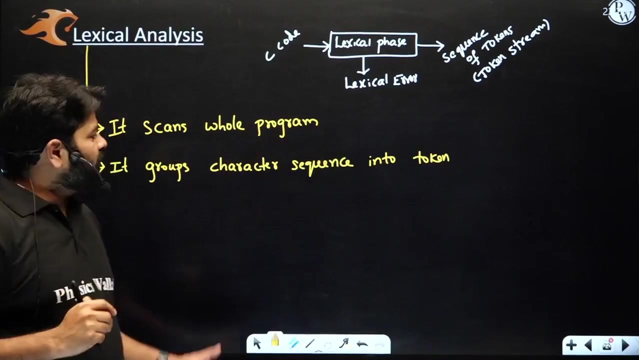 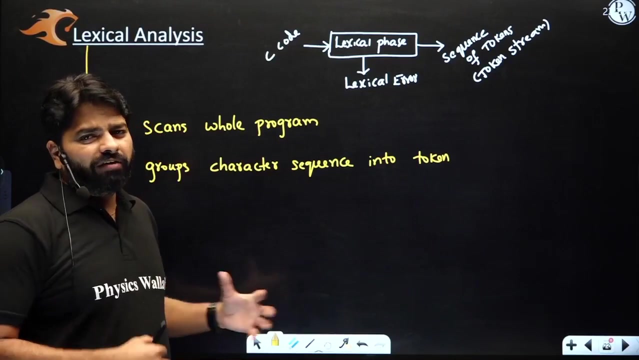 it converts right, it is going to group the characters into token. it groups characters sequence. it groups a character sequence, one or more character sequence, into token or tokens. okay, whenever it detects some a meaningful character sequence, it produces a token. so it's going to do every time it finds a character sequence and produces token. so every time it's. 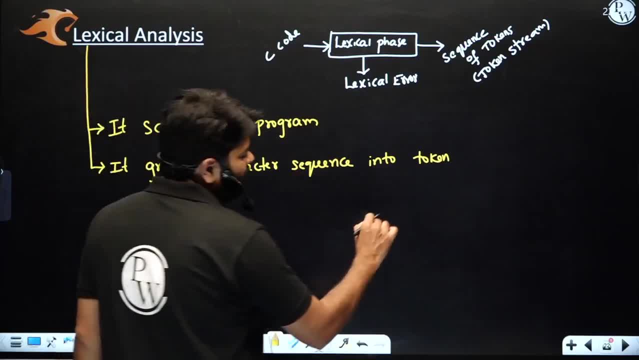 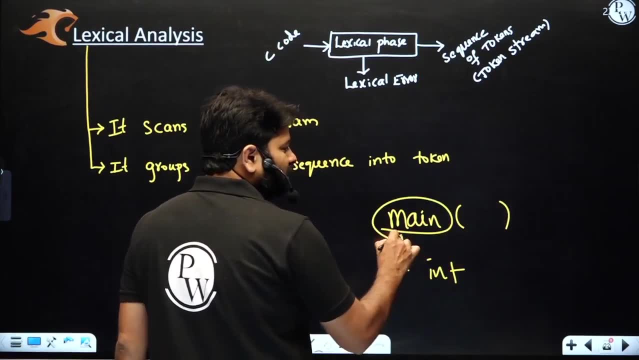 going to do the job till the end of the program. example: if you do, if you write this program main, something like this, and and so on, if you are writing this, it detects this one, then it detects the open and then closed, and then open and then int, going to group the characters and 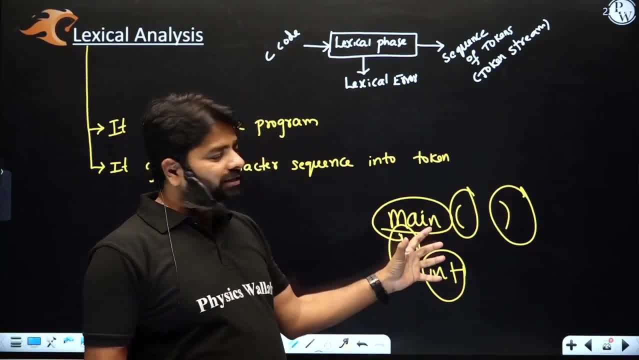 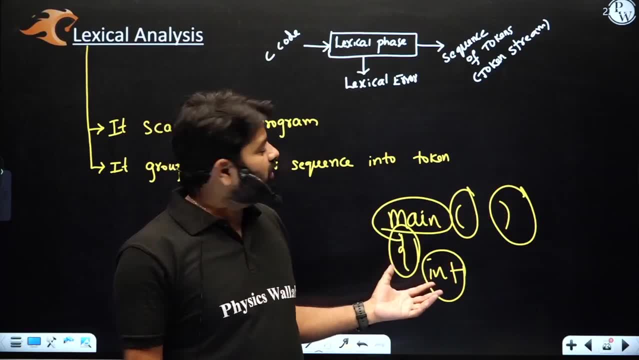 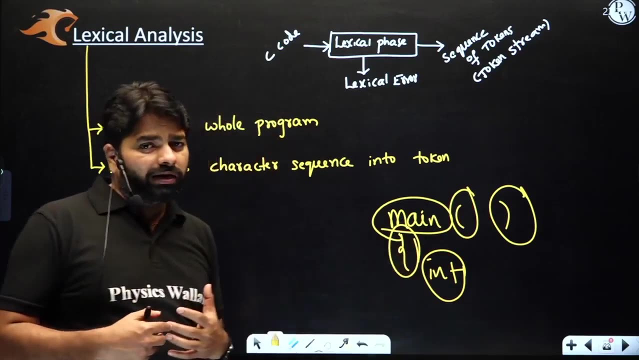 identifies the tokens and produces. so. when it does it, it's just one, two, three, four, five. it produces corresponding five tokens in a sequence. you don't need a spaces, because the spaces are only for, uh you know, identifying the tokens. here the spaces are basically required here. 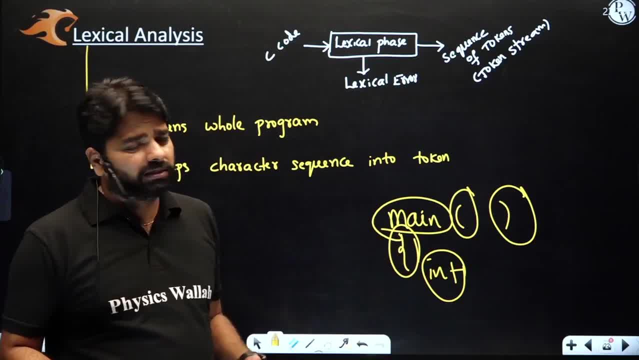 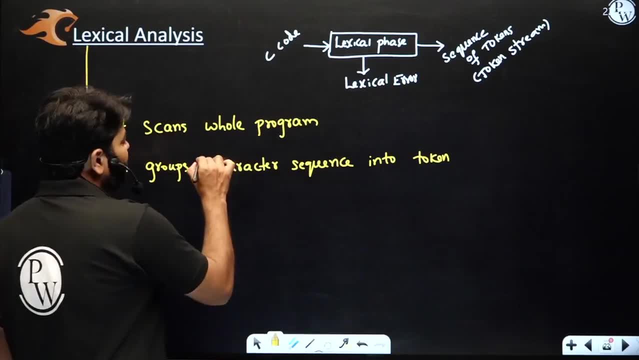 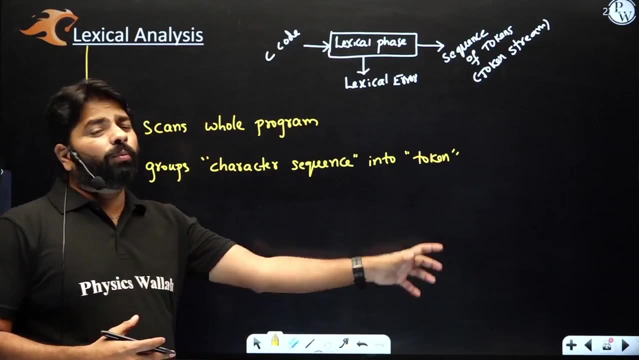 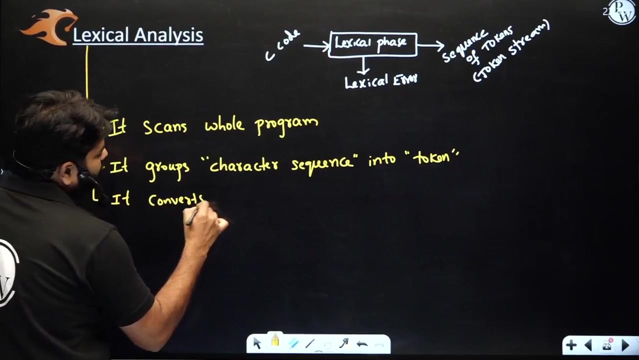 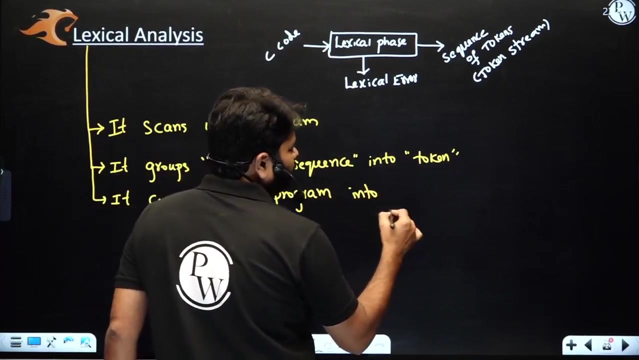 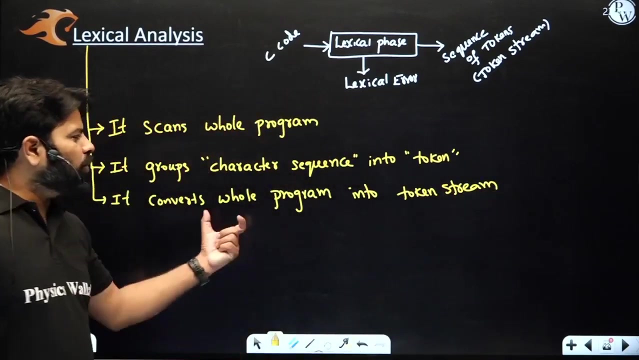 uh to separate the tokens. apart from that, you don't need spaces here at all. okay, it groups the character sequence uh into character sequence into token. so it produces a sequence of tokens by uh scanning whole program. it converts whole program into token stream. it converts all program into just one token stream. it's simply a string. 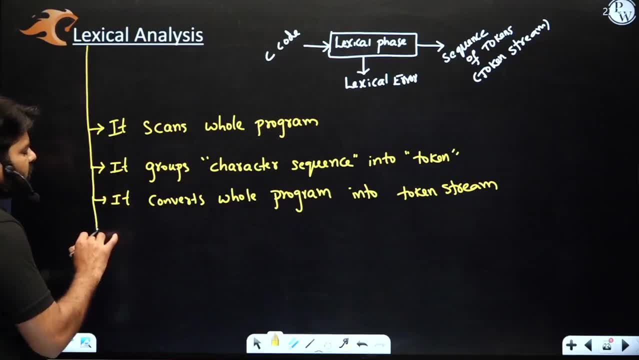 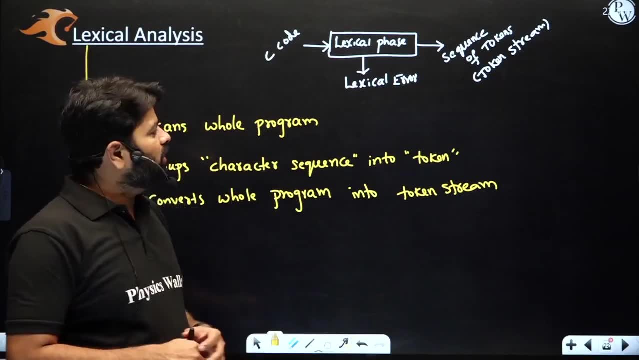 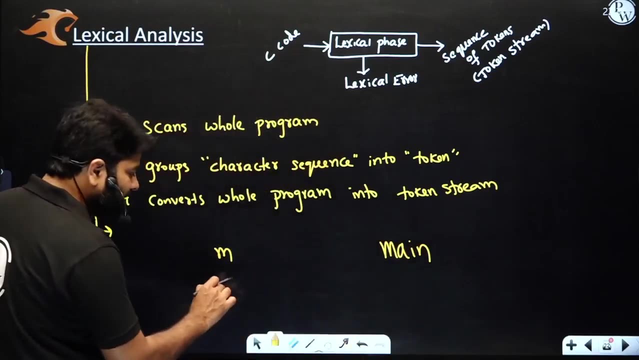 looks like okay, but how this is going to convert. it needs to group this characters, right. how it's going to group the character sequence? there is a rule. suppose you have something like m a i n right, but m is a valid token. even a is a valid token. i is a valid token. n is a valid token. 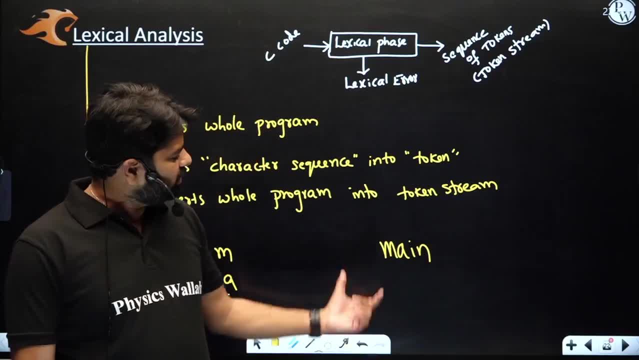 but it's not going to detect four tokens here. it knows that it is a one token. how it's going to start here? it's going to say, because this is the target token, it's going to clone a token and analyze it. c krit part two. there is also the 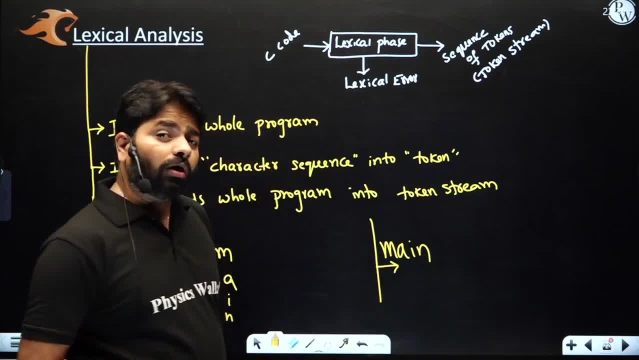 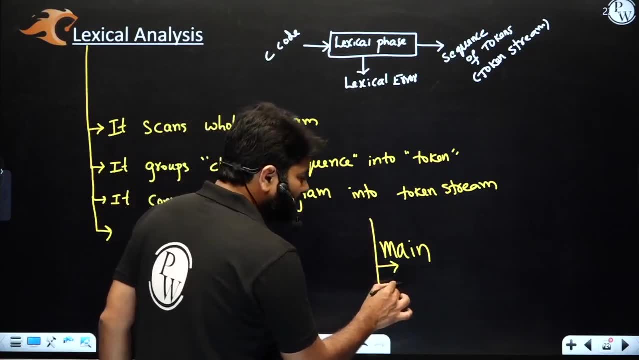 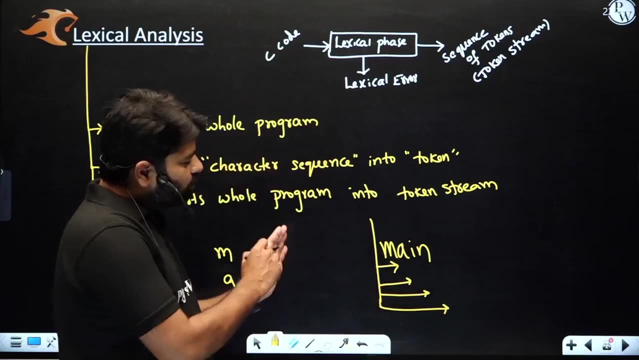 follow maximal munch rule. it's going to follow longest prefix rule. it starts. it's trying to detect the. what is the longest prefix? o, m valid, m a valid, even including i, m a i is valid, m a i n is valid. so it's going to group m m a i n. so each character is going to group with the previous. 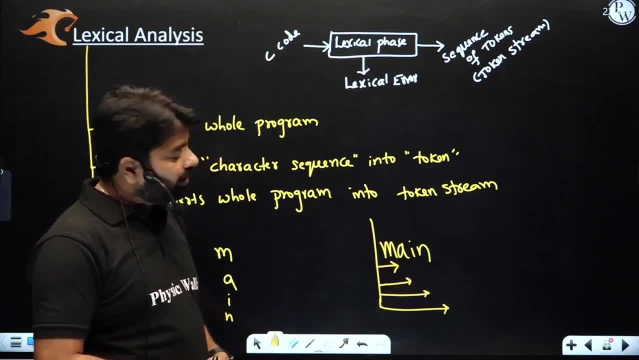 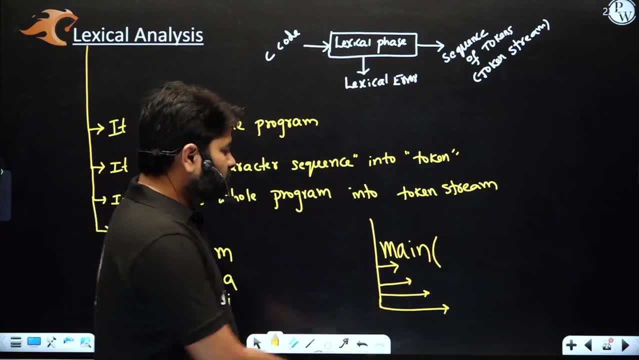 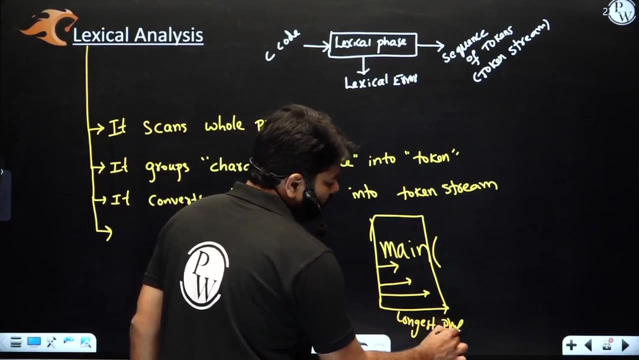 group, then it's going to find which is the longest prefix. when you have the open parentheses, then it knows that that open parentheses cannot be part of the identifier, so it detects the longest one till here. so this is called as longest prefix match. it's called as maximal munch rule. 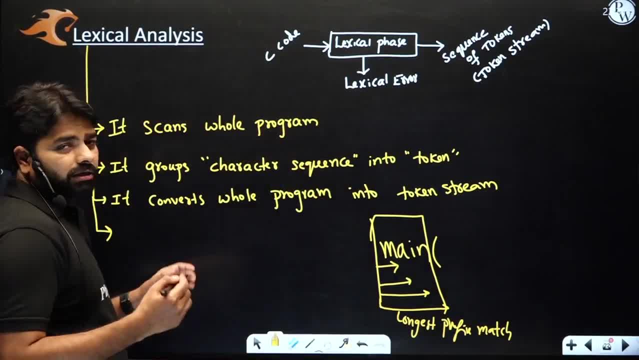 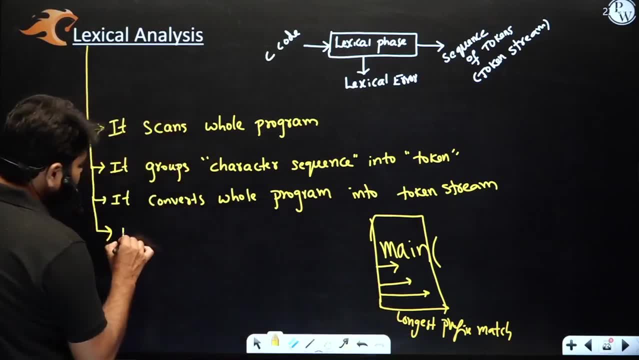 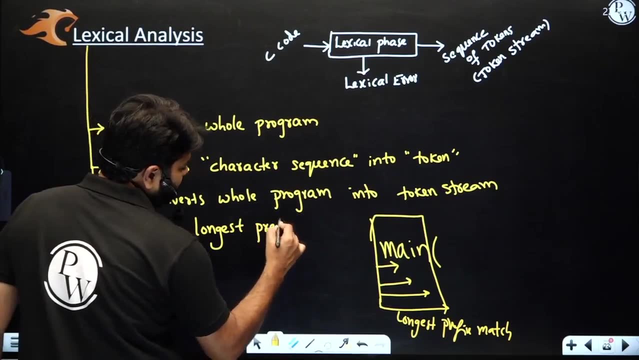 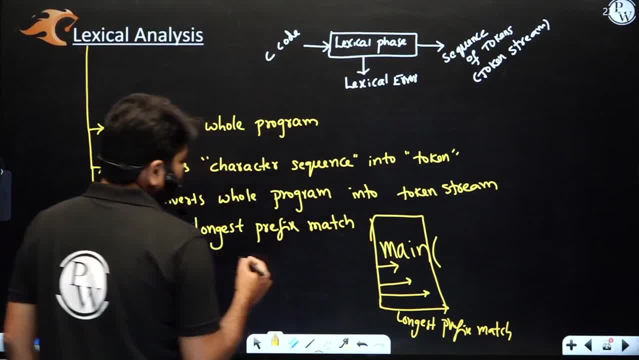 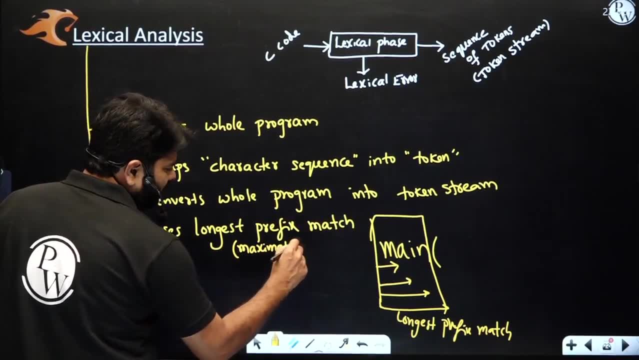 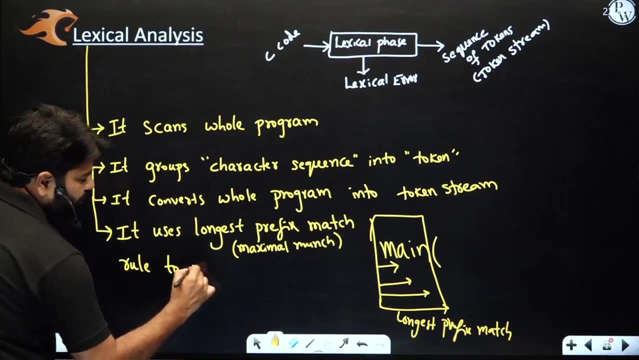 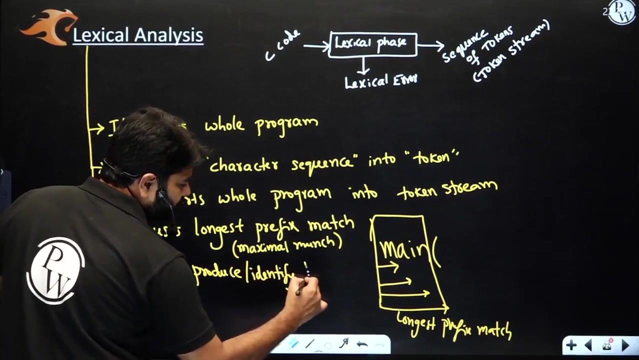 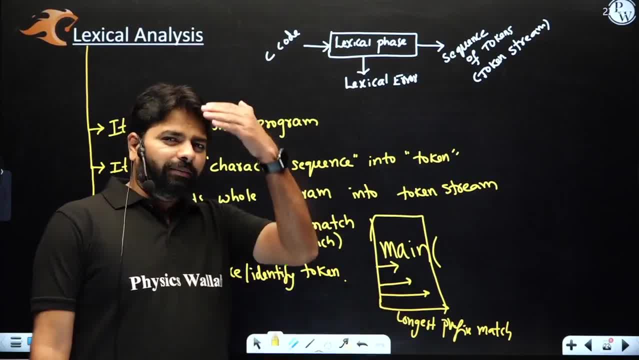 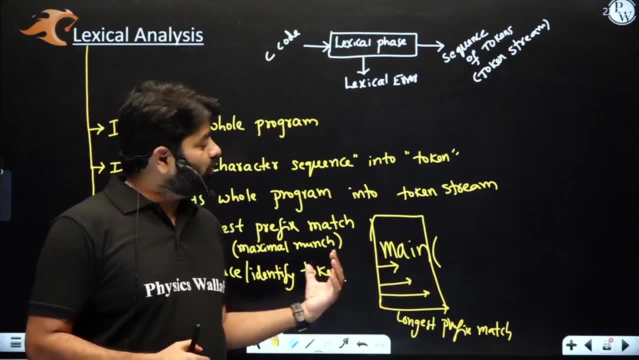 while scanning. this is a very important point. each time it detects a token, it will start again grouping the characters with the help of the syntax analyzer. it always communicates with the syntax analyzer to do this thing: to detect or to separate the tokens. if you get the space, 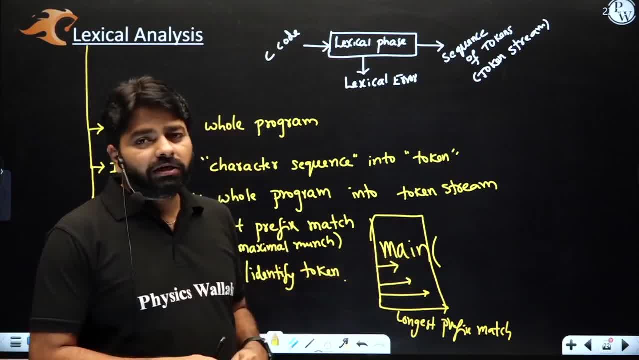 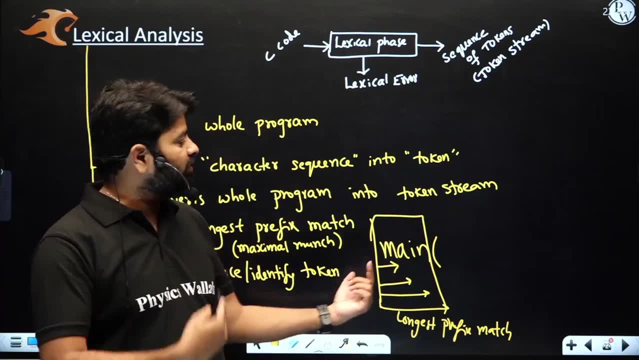 then lexicon job is so easy. if you don't get the space, then it has to separate the token here. but that cannot do alone, so it takes a little bit help from the syntax analyzer. okay, anyhow, if you want to think about lexicon analyzer separately. these are the main points which 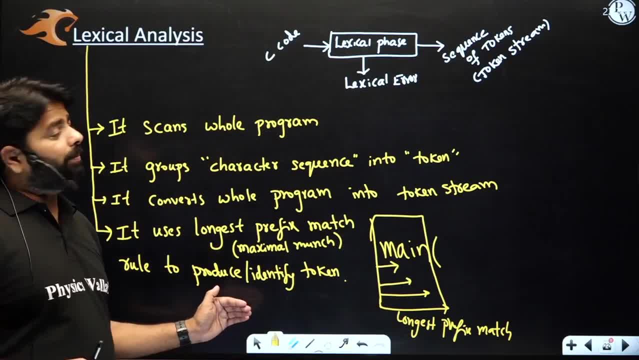 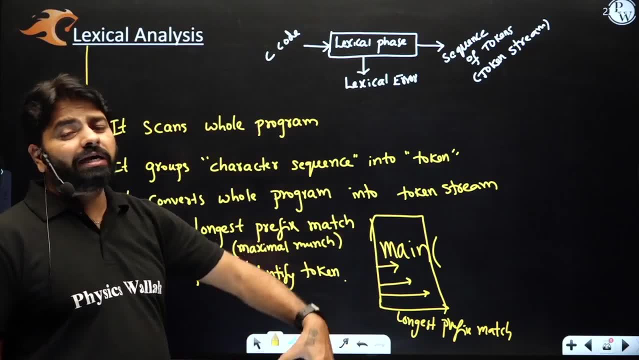 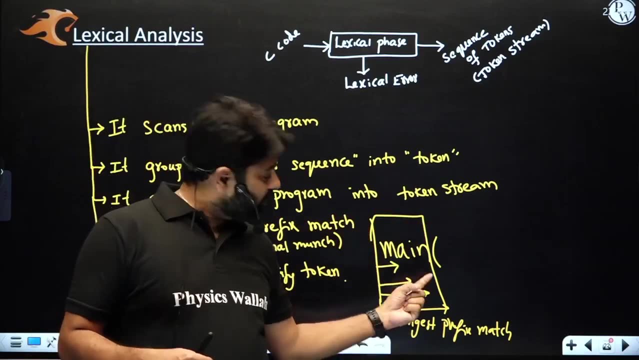 are needed and during the scanning, many things are going to happen. what are the other things are going to happen, like spaces here will be ignored by lexicon analyzer intentionally because they are no meaning later on. they are having no meaning later on. so spaces that you see white. 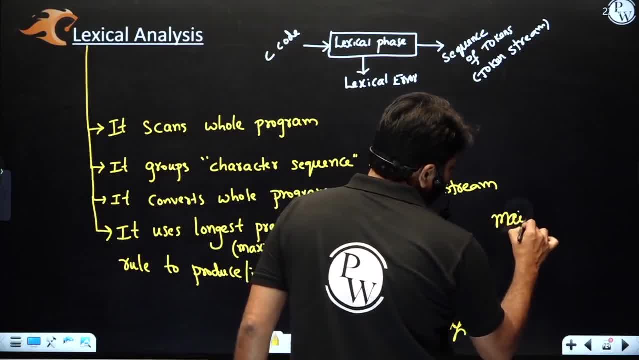 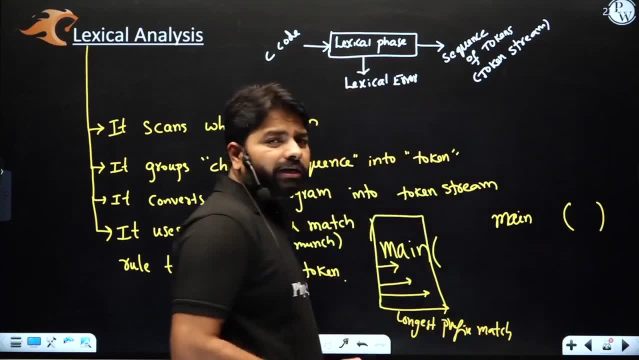 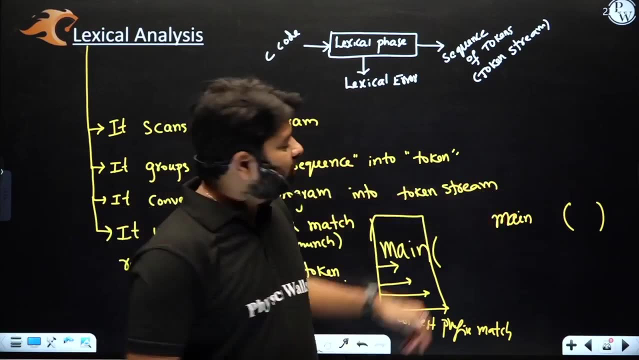 spaces, right, when you write your main, you have lot of spaces, a lot of spaces. and these spaces you see here, right, lot of spaces, they are ignored. they are intentionally ignored by the lexical analyzer because already it's a token separated, this token separated from here. so here what it: 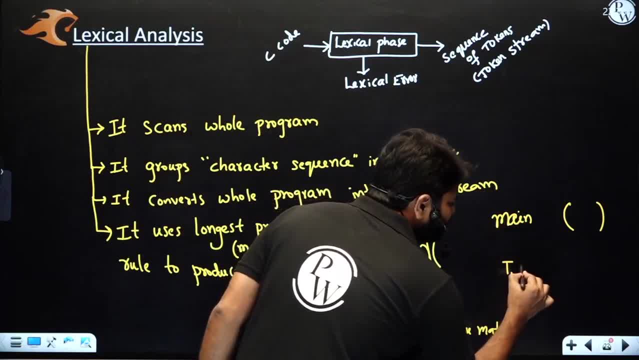 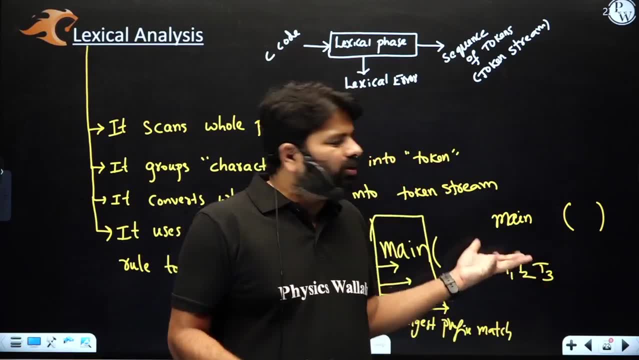 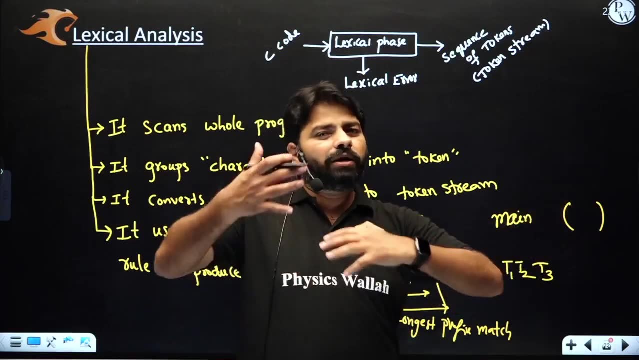 produces like t1 for this, for this, t2 for this, t3 and to. to specify t1, t2, t3, you don't need spaces, because t1 means main, t2 means open, t3 means closed panthers, so these spaces are only to identify. 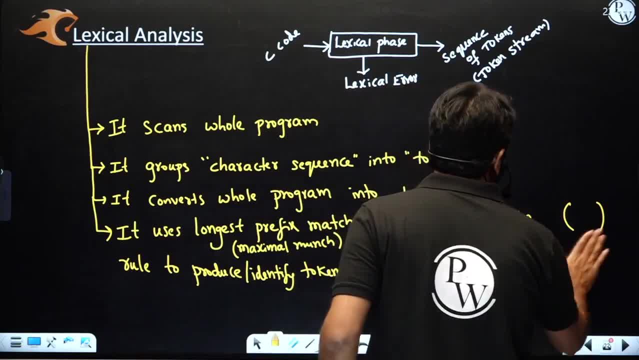 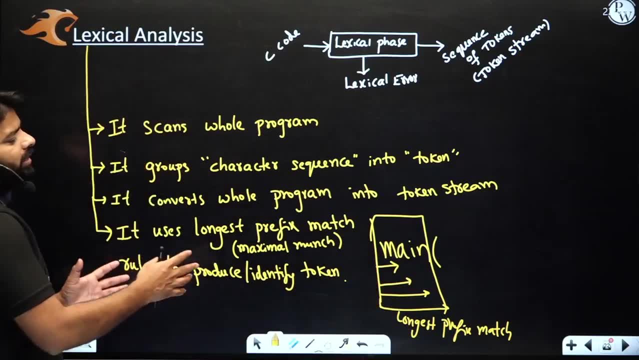 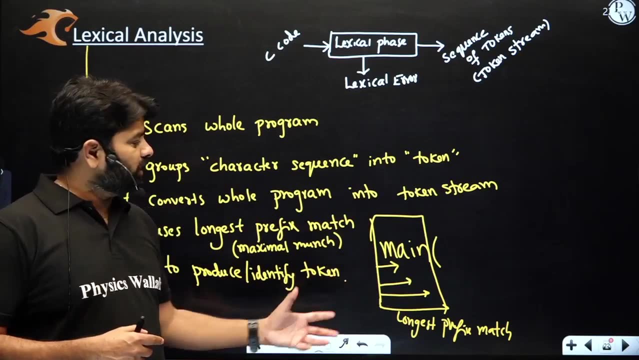 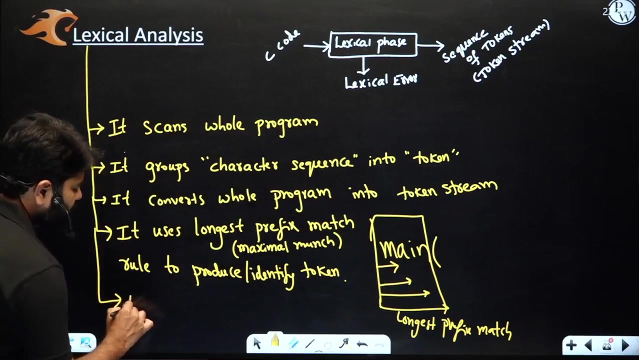 the tokens. basically, if, even though you don't have the spaces, the lecture analyzer does that- identifying the tokens. now what i told here: it's going to use the longest prefix match tool to produce the tokens, to produce the tokens while scanning the whole program i have just discussed. it ignores few things. it um identifies, basically. 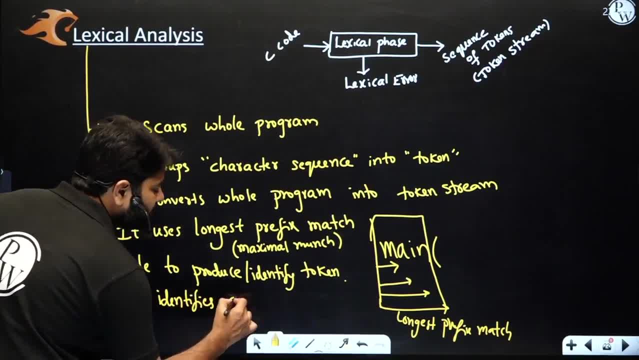 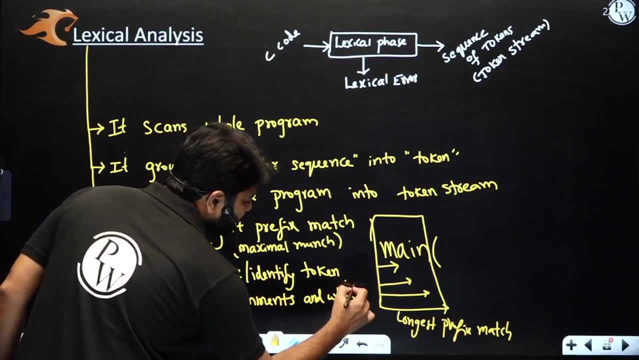 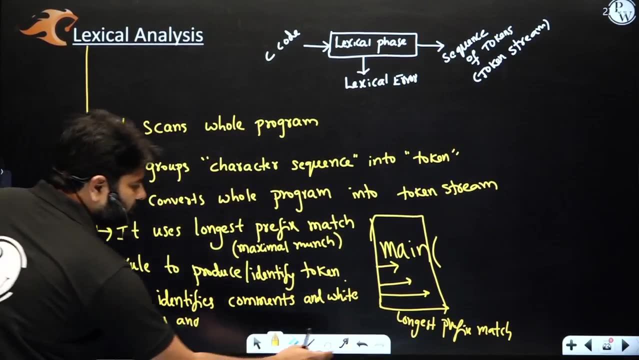 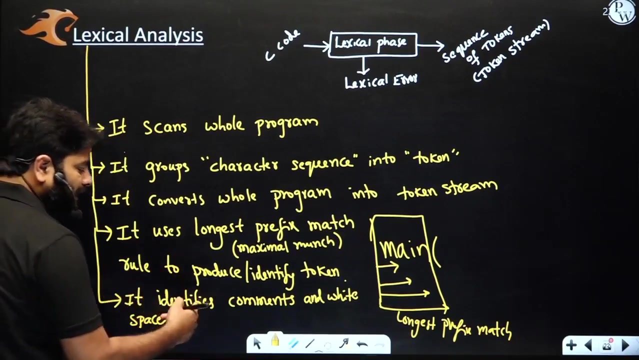 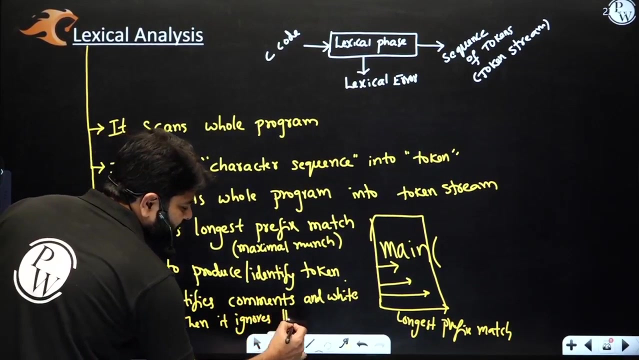 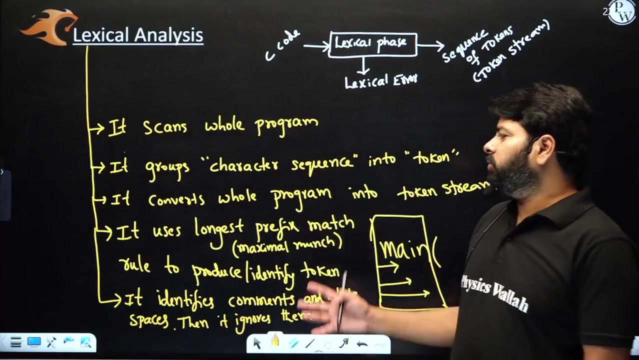 not only tokens, it also identifies comments, white spaces and white spaces and spaces. and the job of lexical analyzer to ignore them. it identifies, then it ignores, it ignores them. it is also the job of the lexical analyzer. and when you look at the lexical analyzer, you need to understand: are these points also when every time the identity? 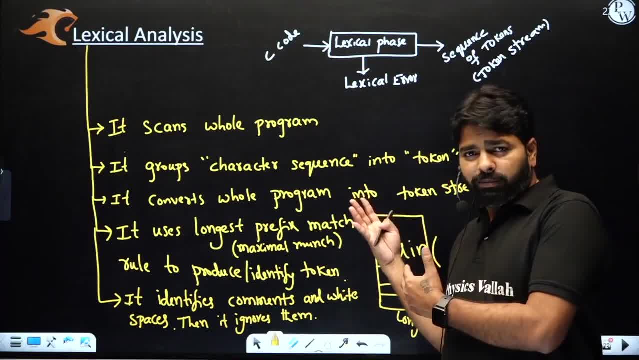 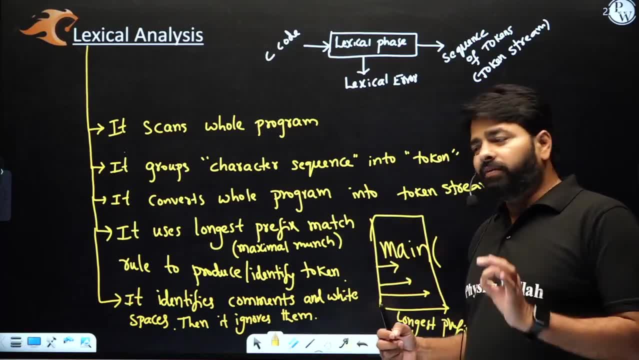 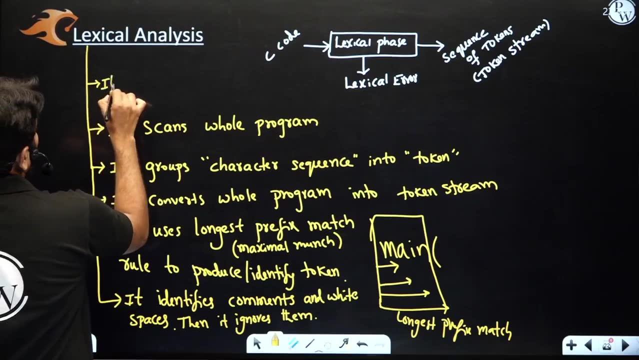 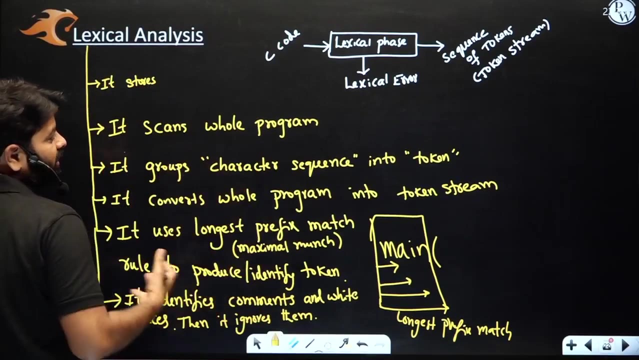 fire appears newly, it's going to store in the symbol table. so it is also having another responsibility. it stores the identifiers in the symbol table whenever they occur first time. so let me write somewhere here at this point: it also it stores or it creates the symbol table, because the first time the symbol table is needed here it stores. 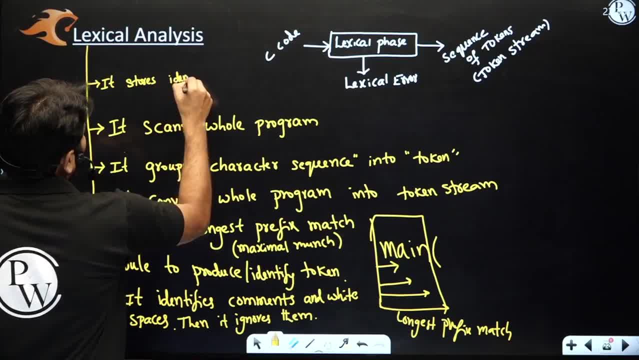 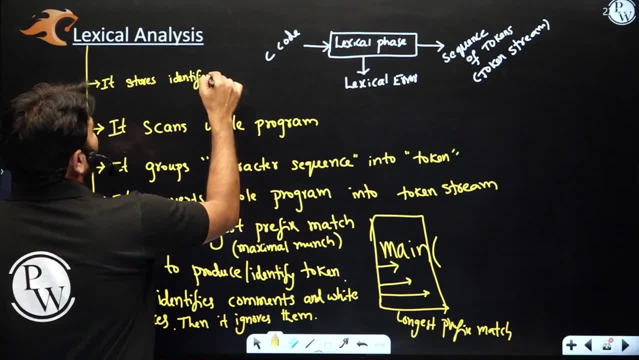 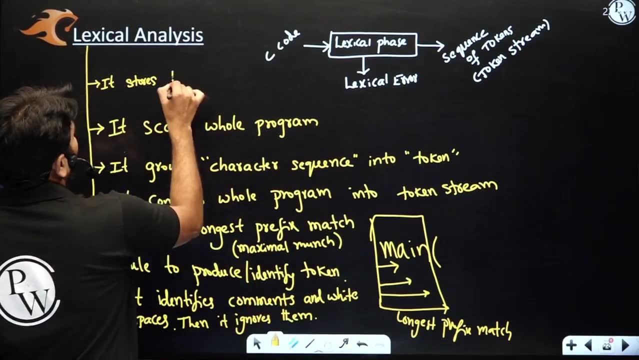 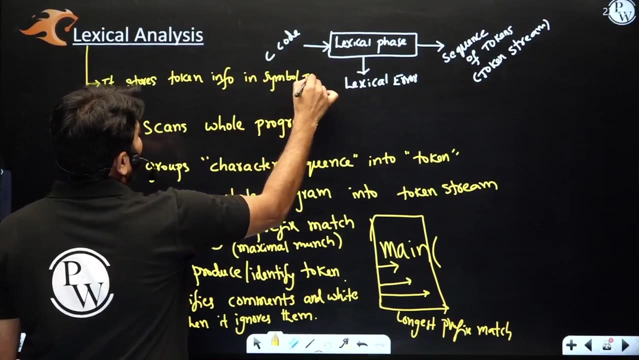 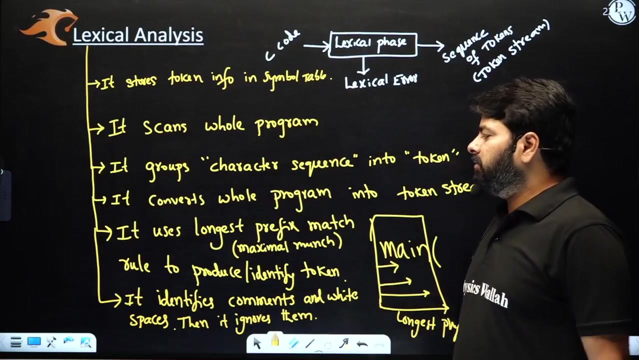 identifier. what information needed here? basically, token information. it stores identifier or token information. you can also say it stores token information in symbol table whenever you see the identifier. fine, these are the things needed for the lexical analysis right now. you might, uh, raise one question, but you also explained about lexical. 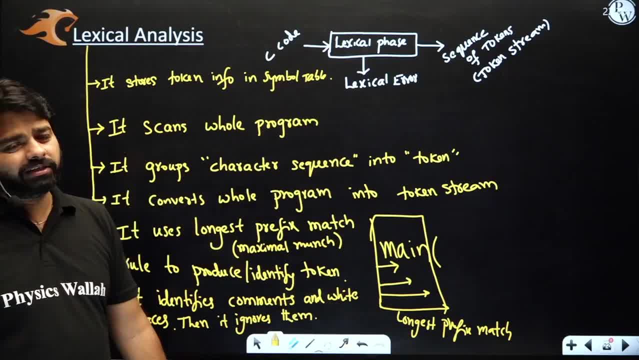 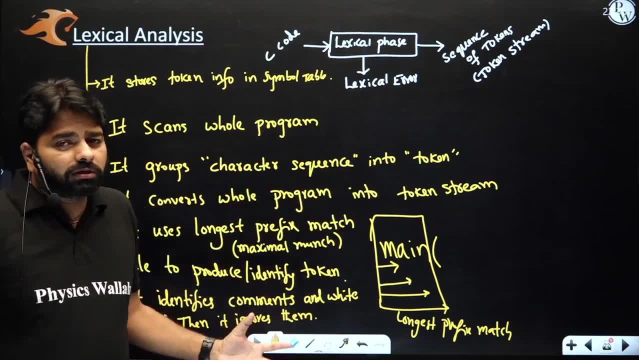 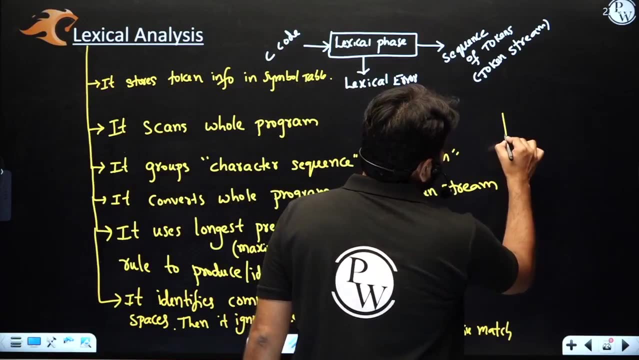 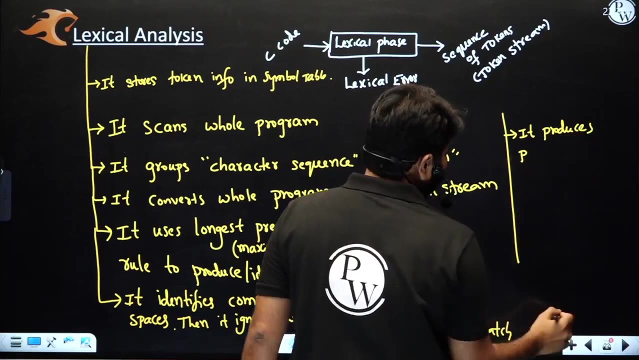 error. who is going to produce a lexical error, lexical case? so if you want to understand them, whenever you are trying to group the character sequence into token, if not possible to group, then what happens immediately? it produces. it is also responsible. it is also responsible, it produces a lexical error. 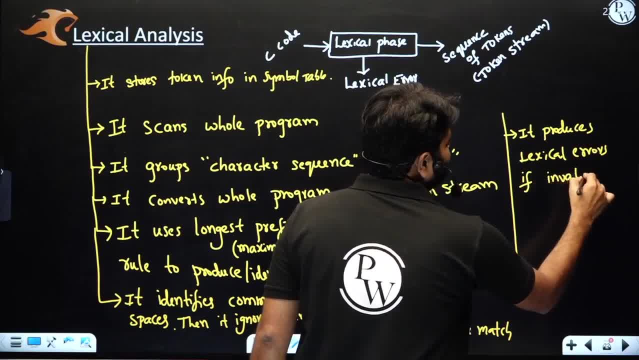 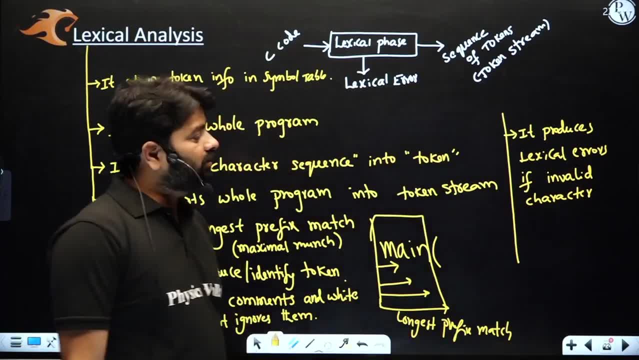 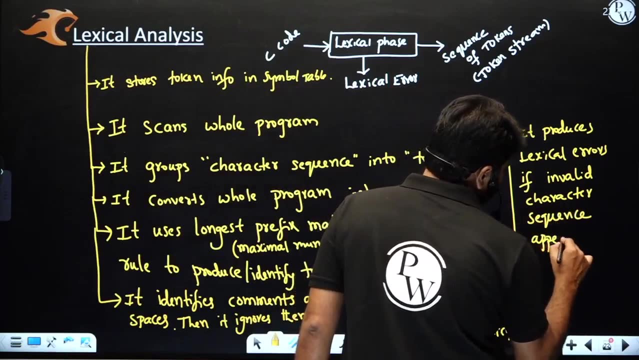 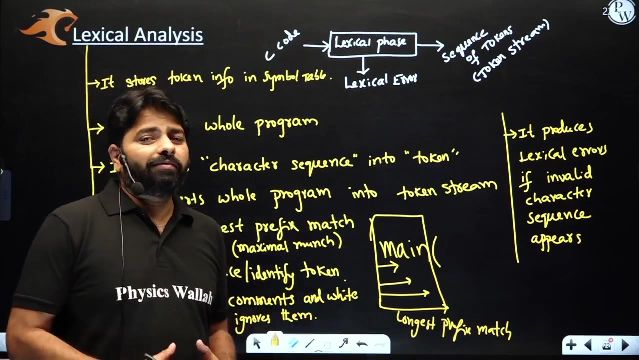 if invalid character appears in a sequence: invalid character, scene, invalid character or characters. if invalid character sequence appears, it is not able to group into token. it means there is the wrong, there is wrong, there is wrong. so there is something wrong with the program. you have not written a valid. 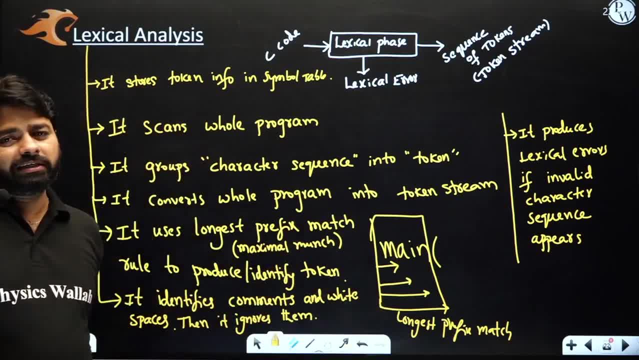 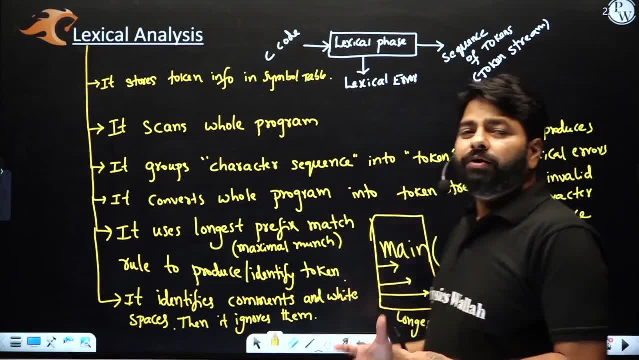 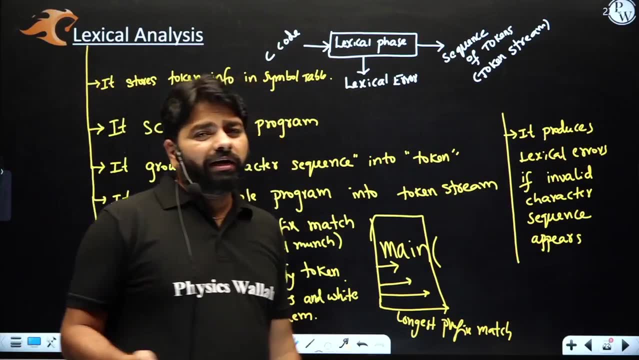 tokens. when will it happen? we have to see in this lexical analysis. with this, almost all theoretical points are covered. now your job is how to perform the lexical analysis. you got all theoretical points. now let's look at this. examples before the examples: if you want to relate with the 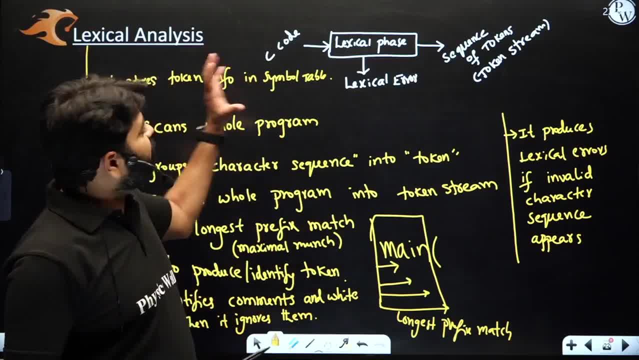 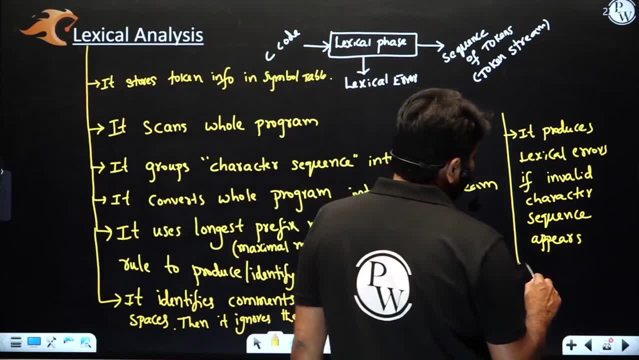 theoretical, uh theory of computation or automata theory. to perform this lexical analysis, you may use either a regular expression or regular expression. you may use either a regular expression or finite automata. if you want to design this, you may use either a regular expression- is a very special topic- or you can use a finite automata. 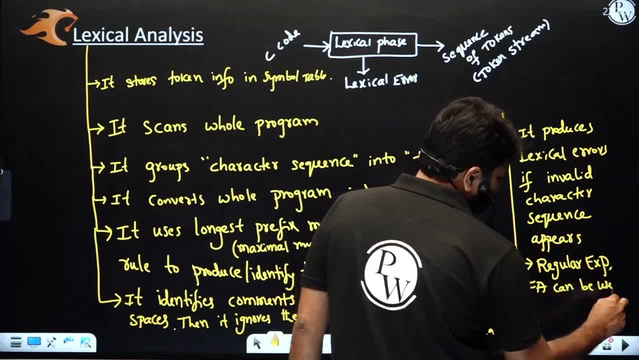 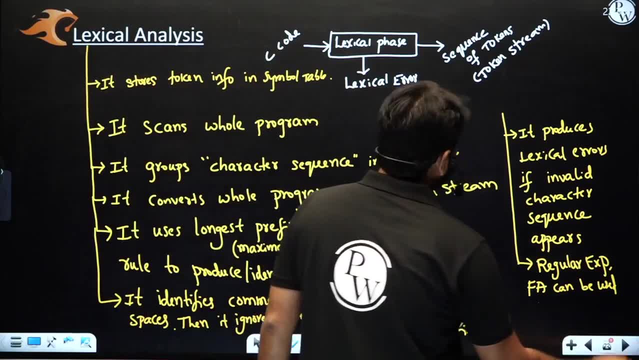 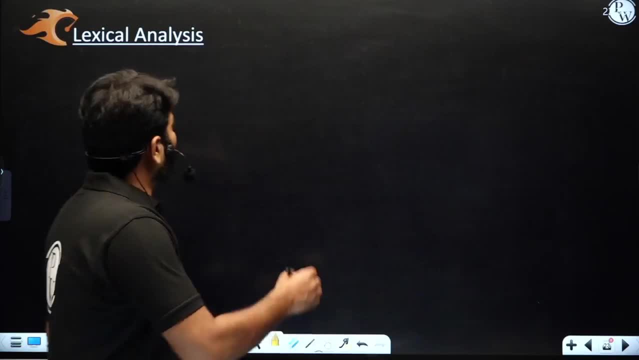 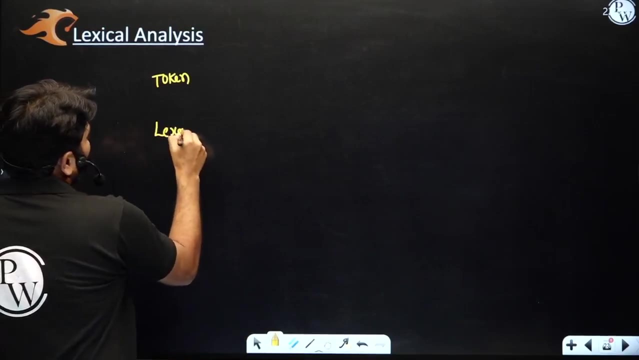 can be used to design. this can be used to design lexical analysis, theoretically. okay, let's start with this lexical analysis. let me start with a few examples. now i told you need tokens- right, always important. what is token, token? and also there is a word called as lexin. basically, lexin is what you write, what you 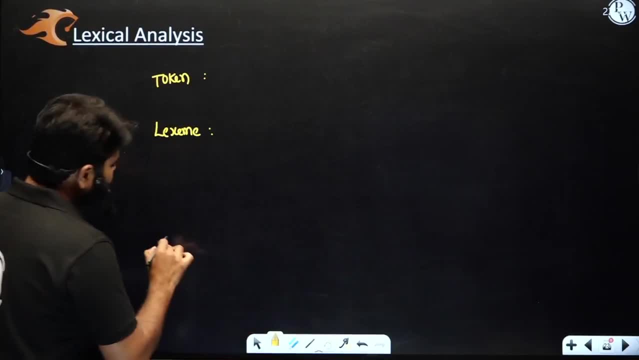 write in actual uh logic or actual program. suppose i'm writing a program like main right- it's not always like this. just for you know understanding these words. otherwise you don't need the difference between local token and lxada. i'll show it to you in the top judges. 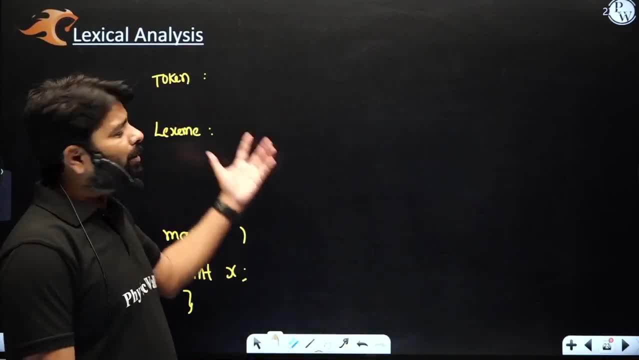 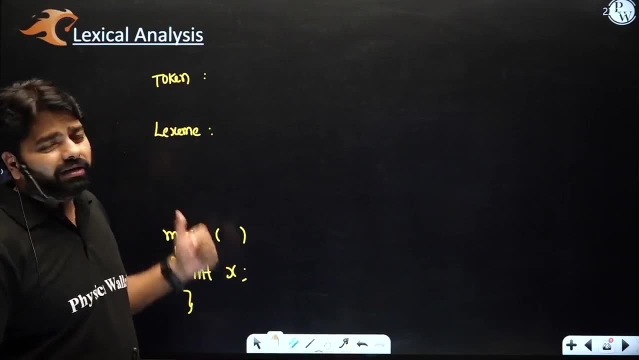 lexem. do you think they are different? no, not at all. for the programmer both are same, only the compiler side, because as the compiler sees, as the you know, a different. that's why i'm talking about compiler side, not your side, programmer. there is no difference. token and lexem. they are same actually. 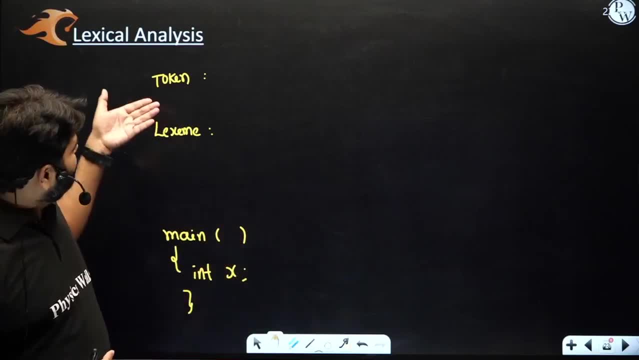 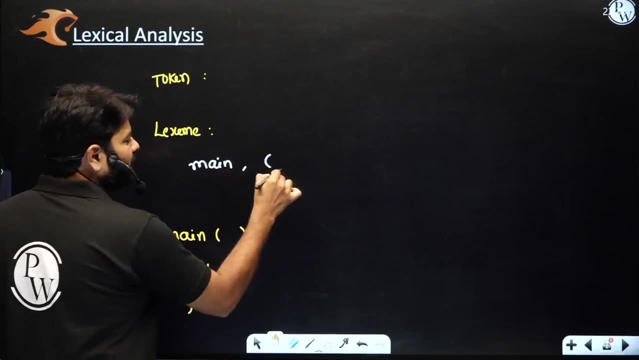 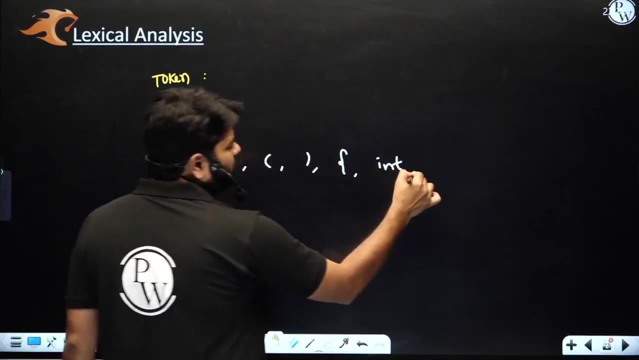 but for the compiler side, what happens? the lexem means what you're writing here, the main. these are the lexems, basically main and open parenthesis, closed parenthesis, then bracket this int. these are actually lexems it's going to do like this lexems it's trying to treat. 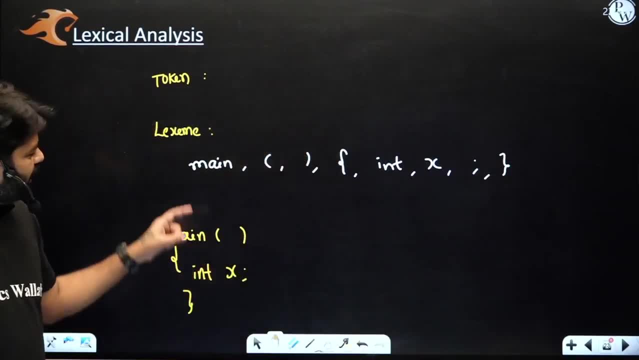 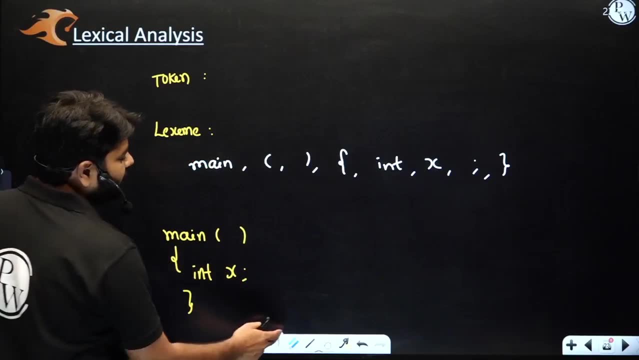 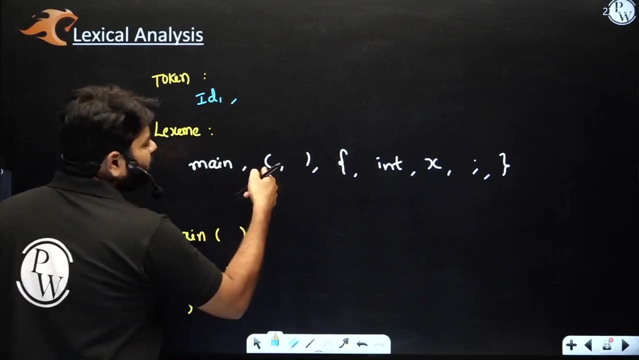 a different lexems here. for each lexem we might write a different token inside the compiler. once it sees the main, it does something. it will relate some other way, like id1. this main might be id1 and this might be. you know, if it is operator it could be having some different name here. 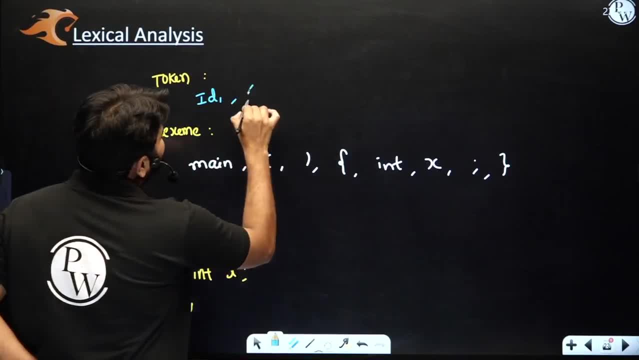 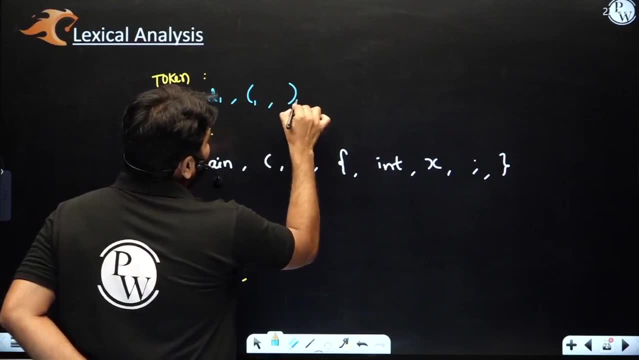 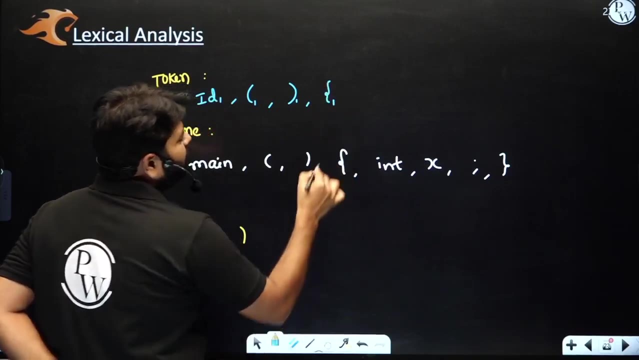 if there are many open parenthesis are coming, maybe it will give some name like open parenthesis 1 or op1, something like that, and this one, the first one coming, let's say closed one, or if it is another. you know this open brace is coming here. int is the keyword, so it might mention like int might be. let's say, a compiler has already, you know. 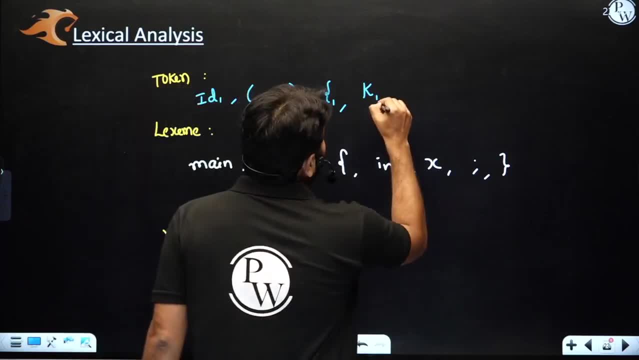 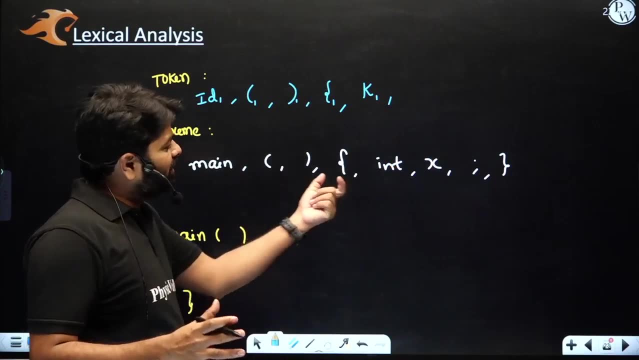 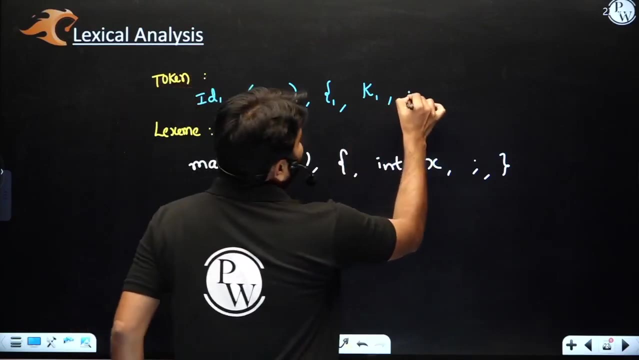 uh mappings for each keyword. let's say int might be k1 or k10, k100, whatever. it is maximum 32 keywords, right? so give some uh subscription between subscribe. uh, that uh subscript in between 1 to 32 and x is identifier not appeared at. so it might be the first identifier, but already one identifier. 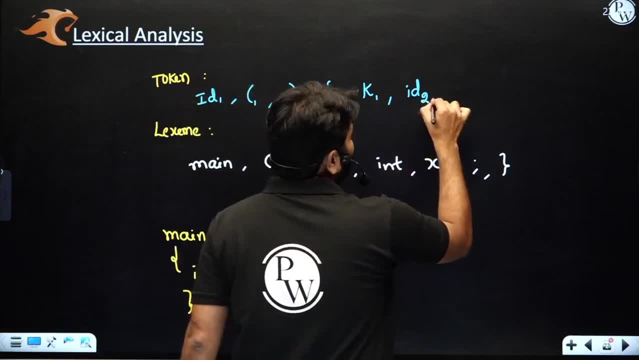 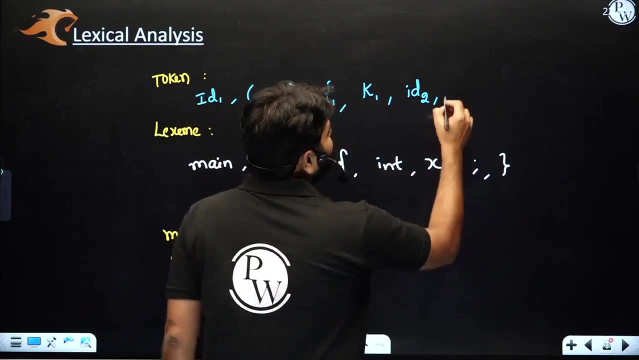 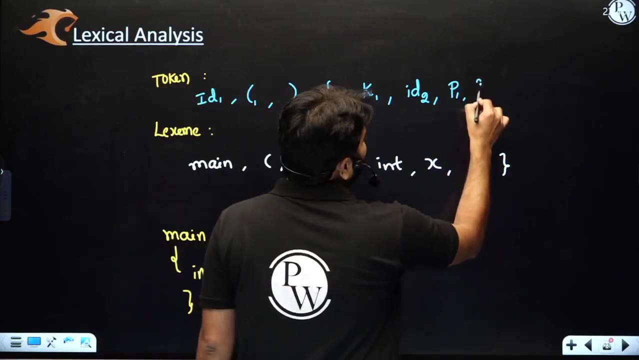 appeared as a function name. this is a variable name, so id2, but first variable, but second identifier, and semicolon is a very punctuate special right. so i might have, let's say, uh, p1. p1 means a punctuation symbol and this one is the first one. so i can keep like this. it's your choice, it's a compiler choice. it's a compiler choice. 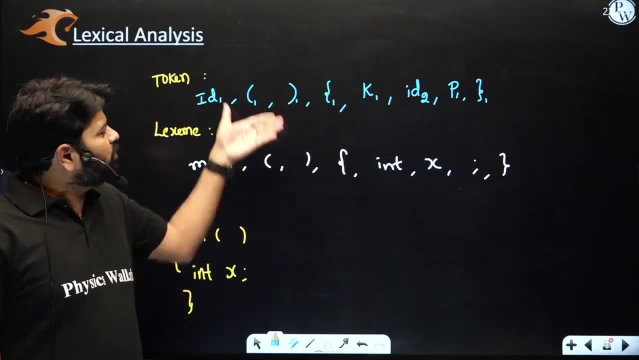 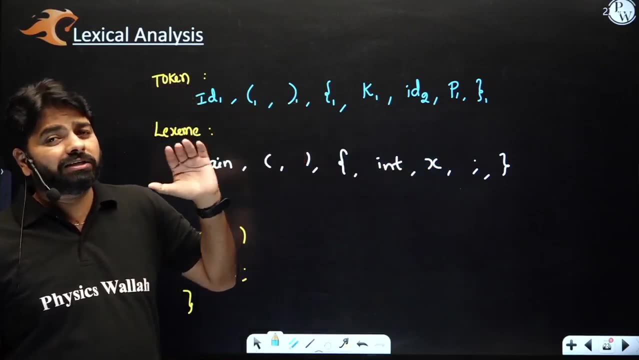 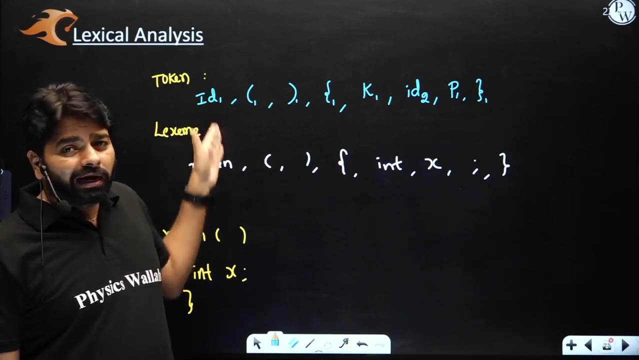 whether these two are same or different. is that clear? sometimes you may see same, sometimes you may have a different mappings. that's fine, the legacy, what you write token, what compiler analyzes or understands. okay, compiler sees this one and might be storing this one, but still, the each token uniquely identifies the lexium. right for this. you might have the table for them, like: 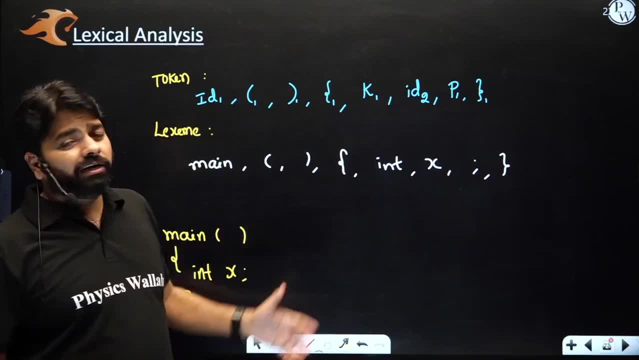 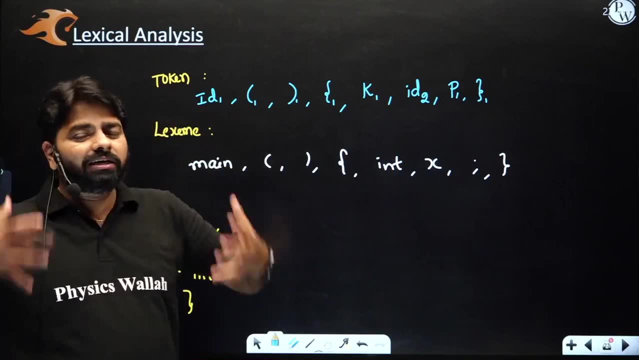 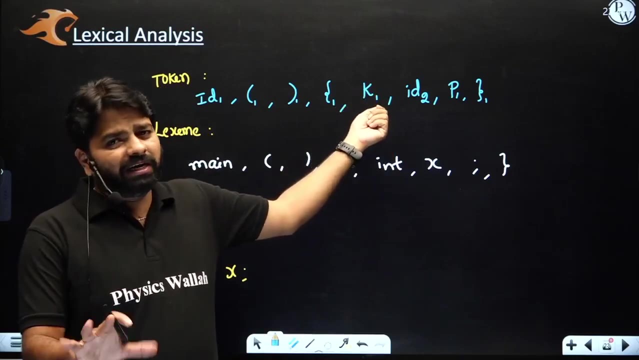 constants it might you maintain literal table and for identifiers it might maintain the symbol table and others already. compiler has int, already has internally the meaning for the int. so int might be int only if you do, if it, if it uh do not want to replace with any other, so int also is the right. 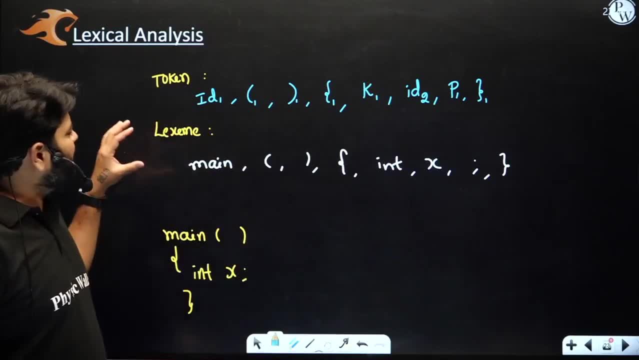 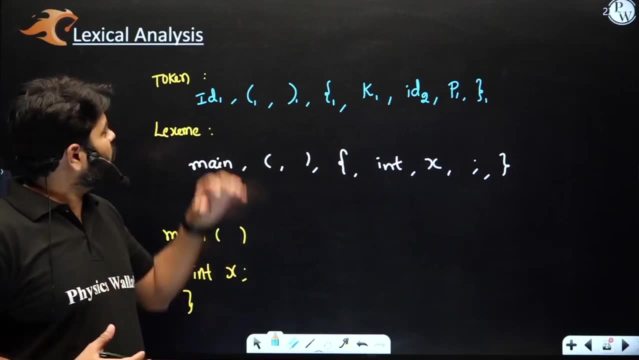 word to put in the token. okay, so this is what difference? let's name what. you are right: token, what is understood by the compiler. but lexium is nothing but group of characters only. token is also group of characters, but replaced with some token name. okay, so each token uniquely. 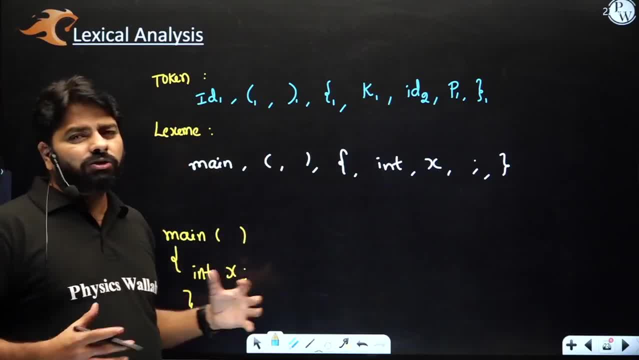 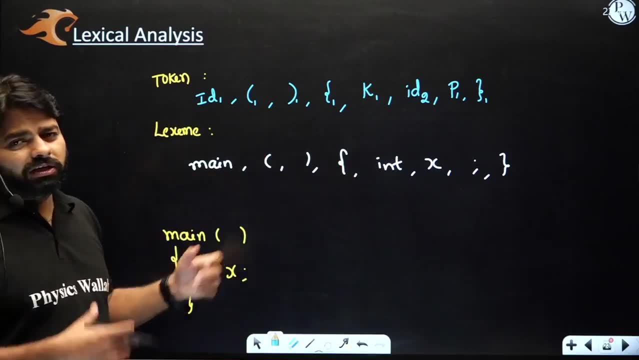 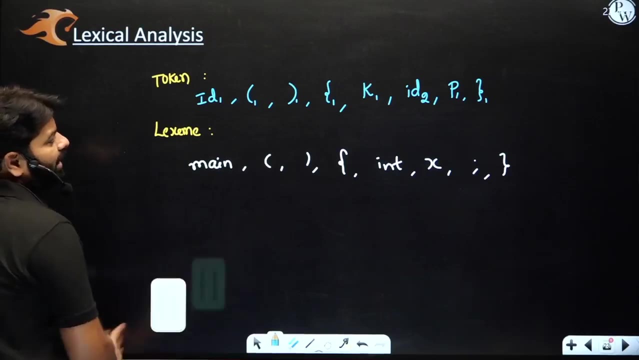 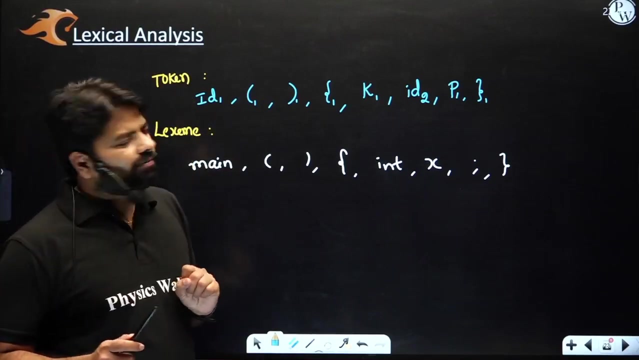 represents the lexium here. whenever i say id2, it's x. whenever i say k1, it's int. whenever i say id1, it's the main, it's uniquely represents it uniquely represents a lexium of the program. this is the lexium and token. lexium and token. as i told, we are going to begin the types of tokens when you. 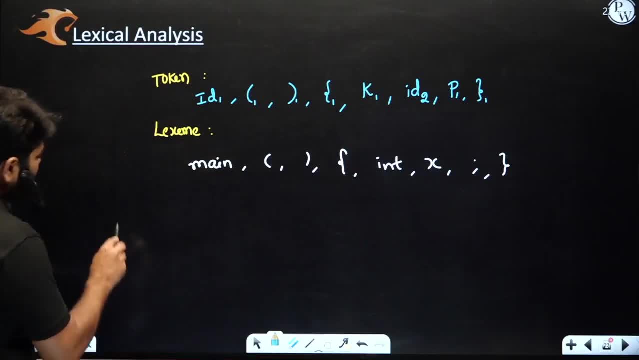 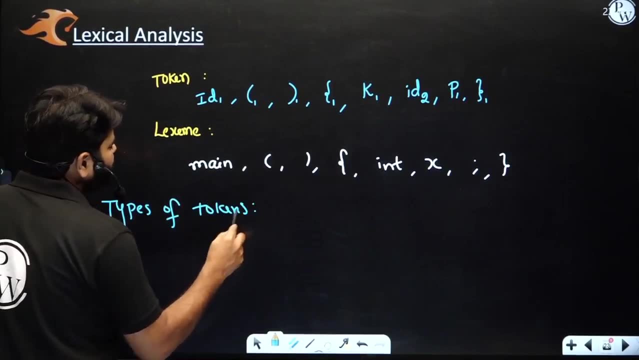 are doing this many things? how many types of tokens are there? how many types of tokens? do you have any idea of this? the five, six: okay, depends on how you analyze, but i just converted all of them into five. but some books they say four. some books they say six. it's fine. 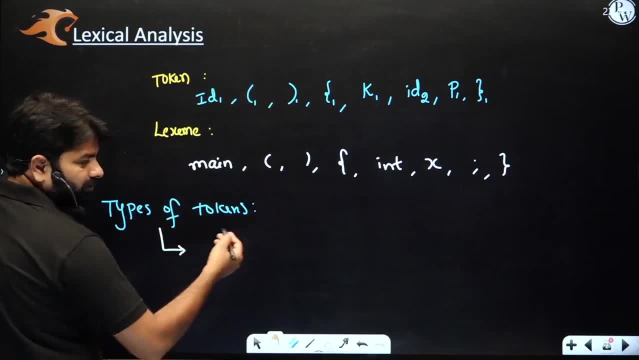 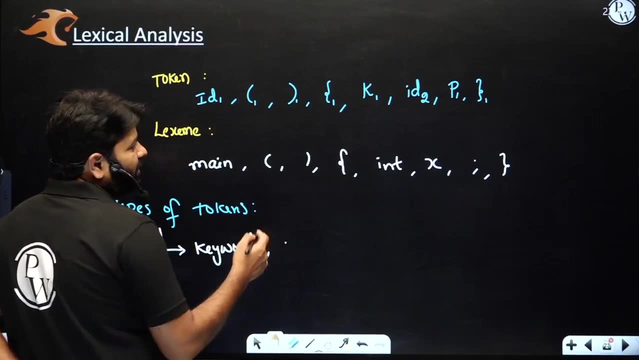 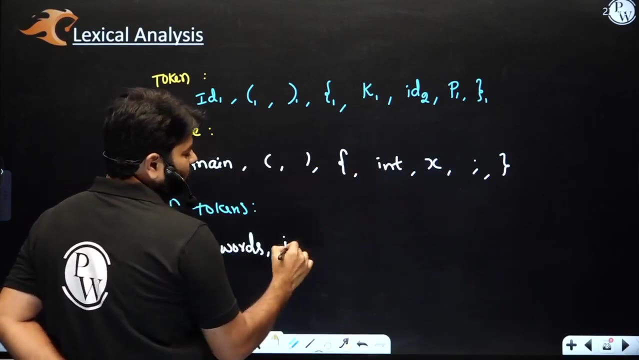 okay, how many types of tokens are there here? i'm just saying, uh, the five. they are keywords. what else you have? if you look at here, keywords and what else you have, sometimes you have identifiers that mean x. what are they? identifiers? whether it's variable name or function name, a structure tag, they're all. 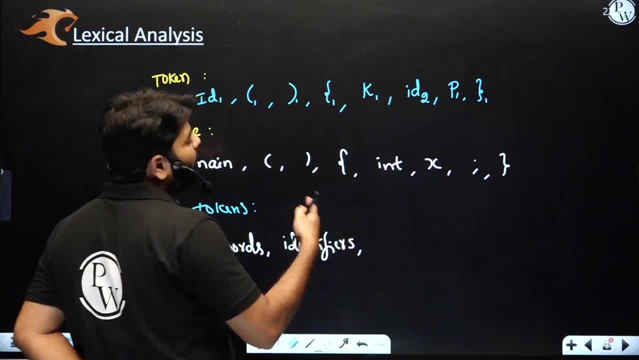 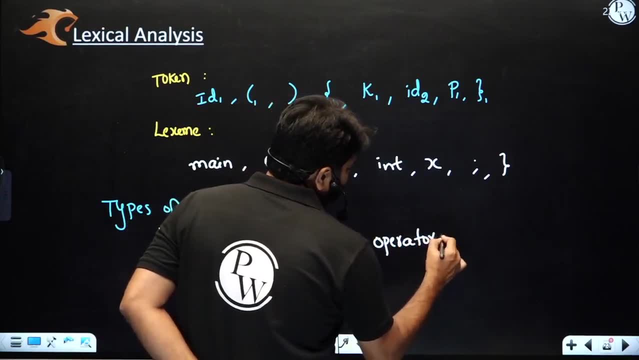 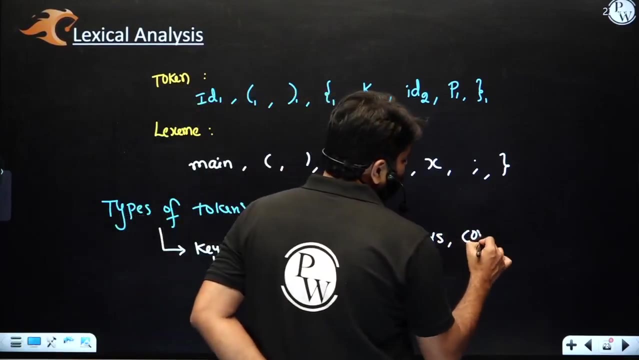 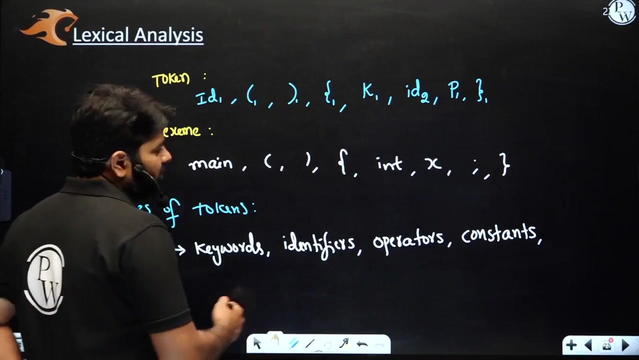 identifiers. what else you have? sometimes you will have operators like equal, plus minus. they are operators. sometimes you may write constants, maybe integer or character string. you may have literals or constants here and, apart from this, special symbols you may call special or punctuations. okay, so constants. and finally you will be having 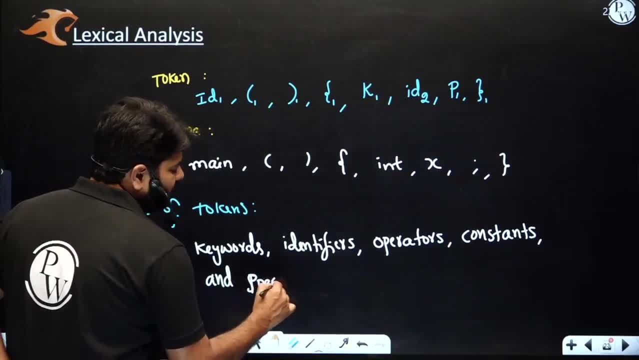 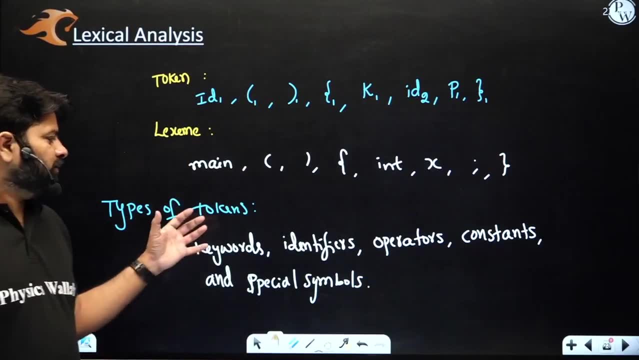 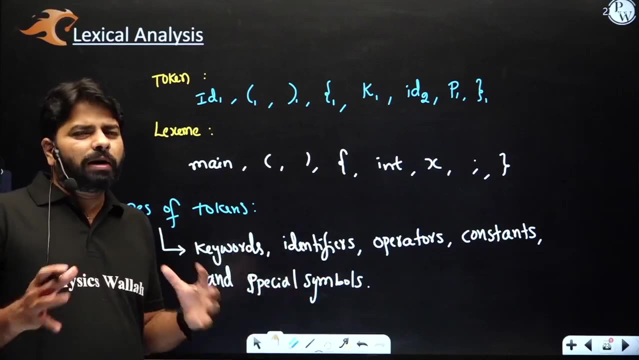 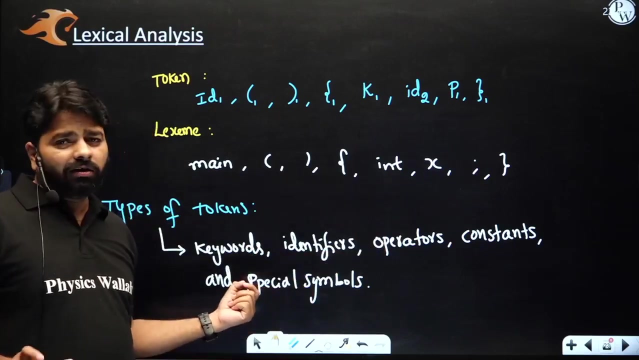 uh, punctuations or special symbols. let me call as a special symbols, including punctuations, soension. so i have divided all of them into just five types of tokens. we just remember them, this five types, the old programm, actually the sequence of tokens, and every time you detect. 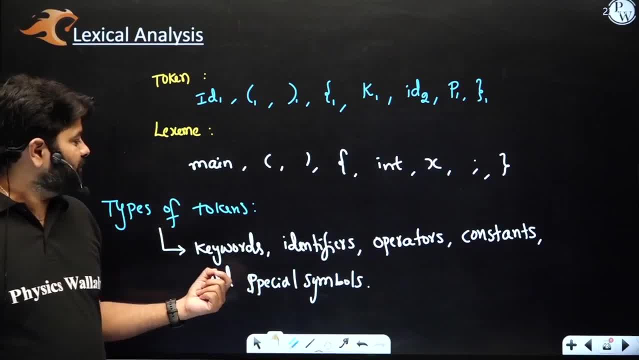 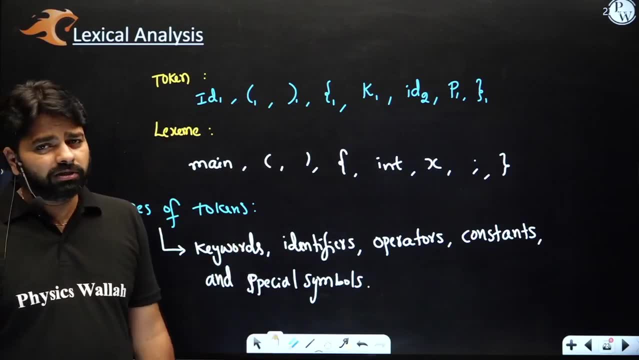 the token that should be belong to one of them. if not, then it will produce lexical error. if not, it will produce lexical error. okay, i hope you have uh clarity of the tokens now. i am going to start with examples, but it's in the description of this video, so please forget to enter your senior letters if you hope to check them out. maybe next time you complete a whole learning session of picking all the tokens and wish you success in this video. you will get awesome learning, better knowledge. then i am starting with my have more points? okay, so let me conclude our session. our word, these tokens. iam going to divide all them into twoASCP tokens, all expression, one, two dre x, two yido, n, uh, five types of tokens. you just be sure that all of these tokens, our code, is divided by the sequence of token. 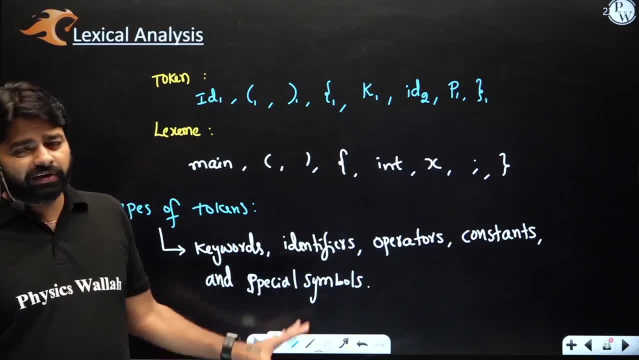 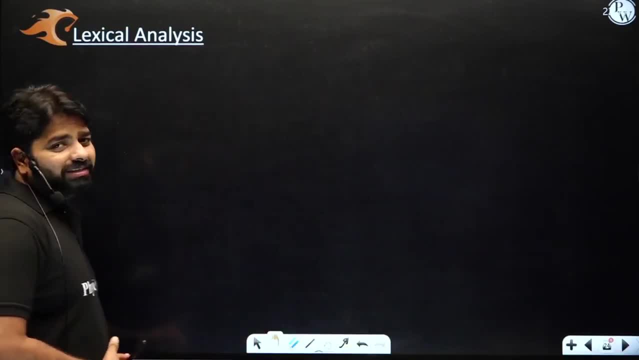 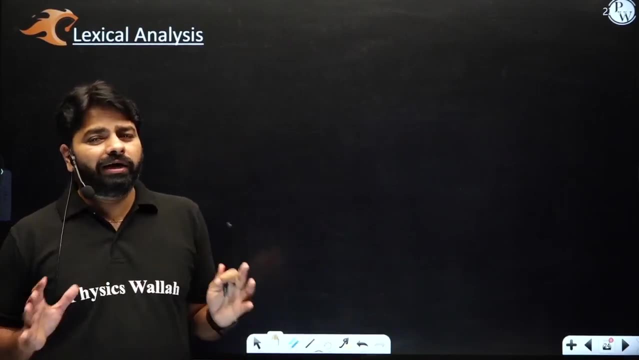 time I analyze the example, I do with a different example, so you need to practice, in case if you are not aware of the tokens like keywords. what are the keywords? what are the operators? you must learn before practicing this example. I believe that you are good at C program, in case if you are not learning C. 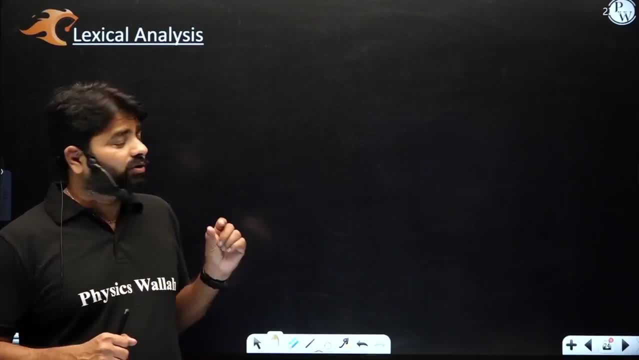 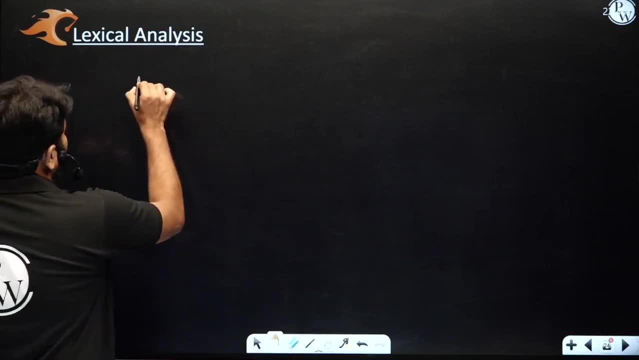 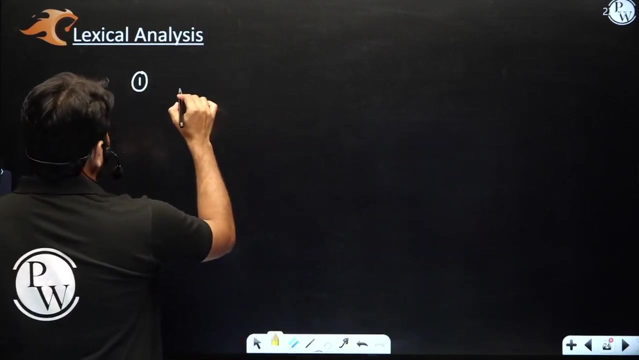 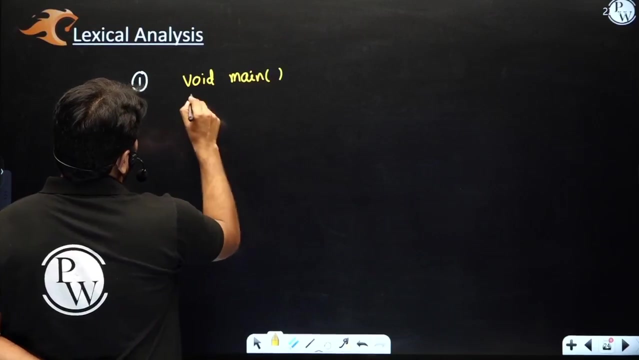 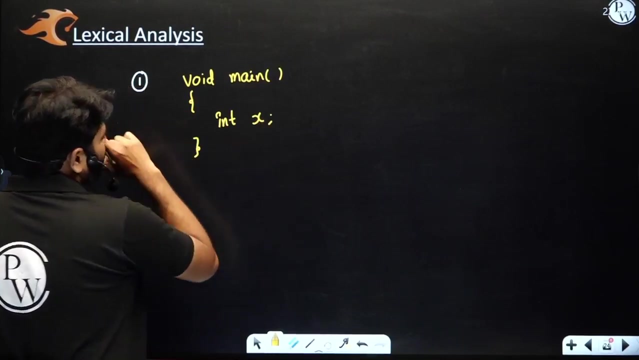 program. it's better to learn little bit of how- you should have little bit of programming knowledge before analyzing this- that you will know how compiler works. okay, first example. it's a very simple one, just to find: do you have any lexical error? if no lexical error, how many tokens are there? is a clear? do you have any? 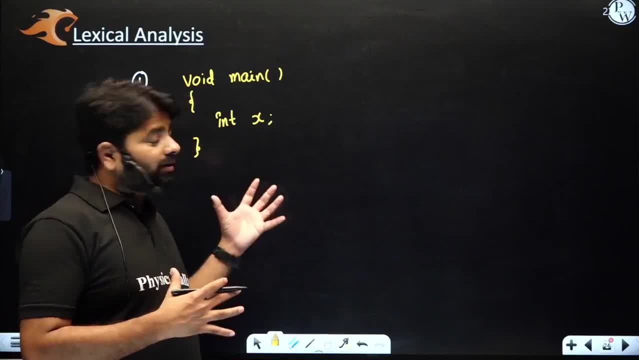 lexical error? how many tokens are there? is a clear? do you have any lexical error error? how many tokens are there? is a clear? do you have any lexical error? for that only you error, for that only you should know, for that you know to find. do you have any? 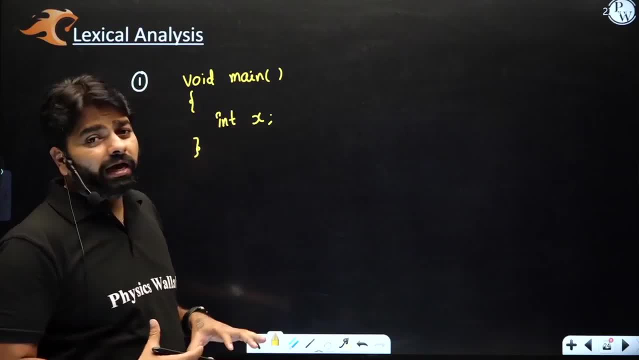 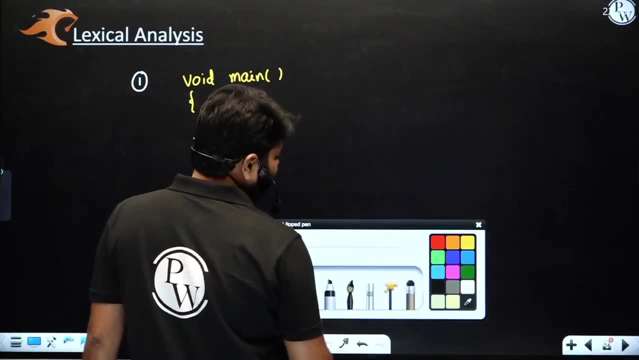 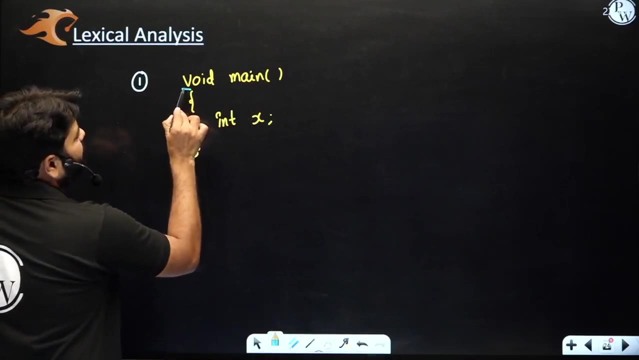 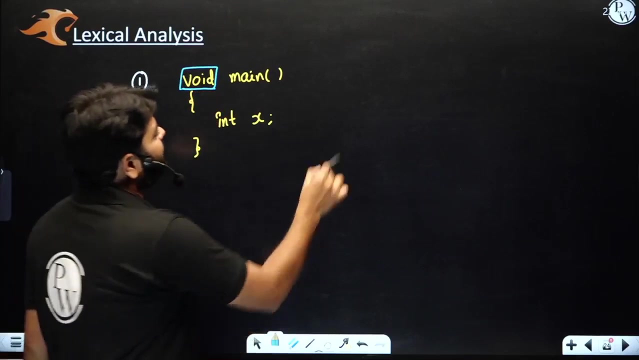 lexical error. first you should analyze: is it producing? is it producing any lexical error in the beginning? so I may not give lexical error. it does like this: it starts scanning here and it's does first character, second, third, fourth. we've got a space so it detected as one token. so I'm just writing. 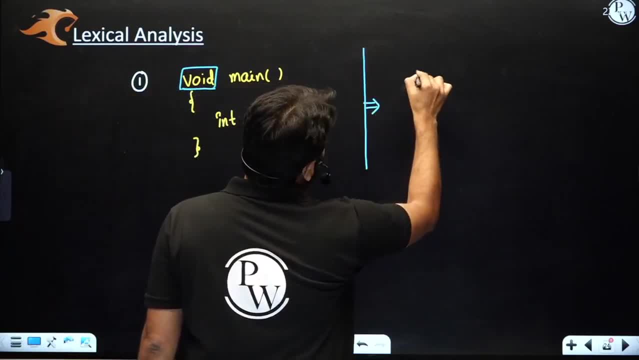 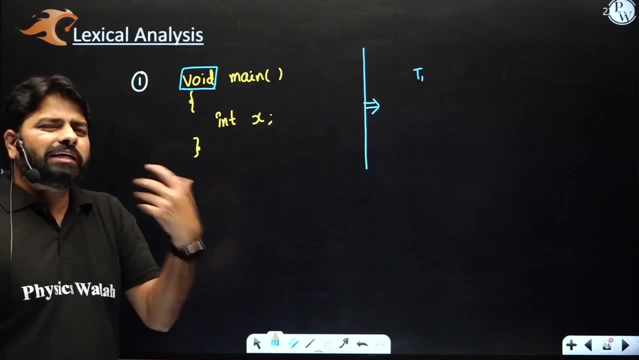 that the corresponding the token here. okay, first token, let's say t1. don't worry what is p1? okay, that wide, wide is a keyword, maybe it is a k1, but I just want to say t1, t2, t3, that's how that's. 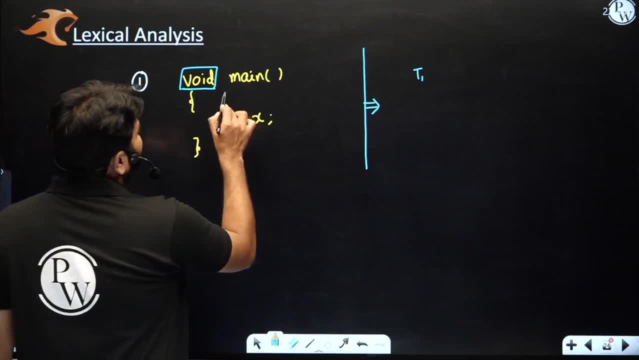 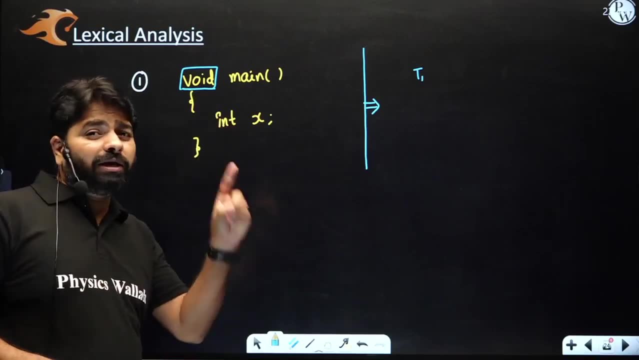 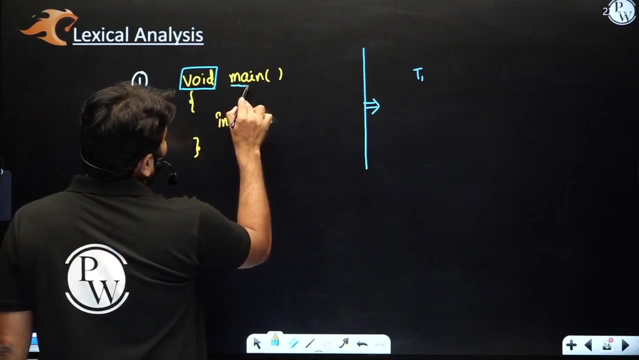 one to maintain the count and then space. what happens to the space face is ignored. it will not be counted as a token, but it is identified by the lexical analyzer. it is identified, so it is ignored. then it starts scanning from hereiß in. then after that open parenthesis is the different token belongs to. it is not the part. 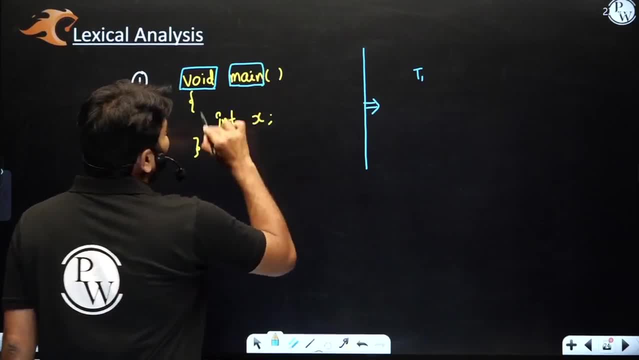 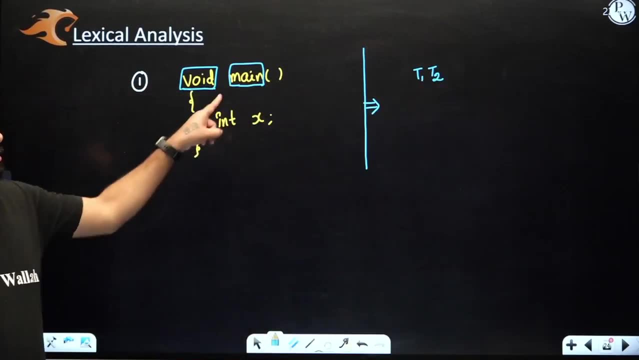 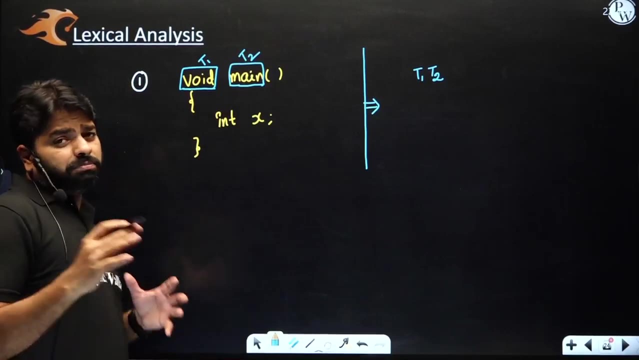 of the identifier and somehow it has a rule, identifier rule, so it knows that main is another token which is identifier, which is t2. let's say, okay, the t2, so t1, t2. i'm just writing this is t1, t2 and then open parenthesis, then space, without space. also it does it's as a separate token, which 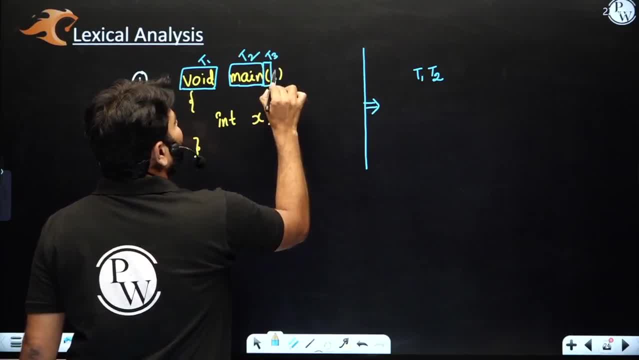 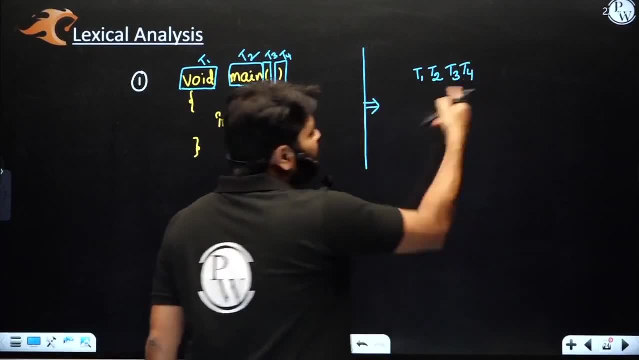 is t3, then if you have the space, fine. if, even though you don't have the space, it will detect as t4. so now t2, t3, t4. see when i am producing. i don't care the space, i don't have the space at all. 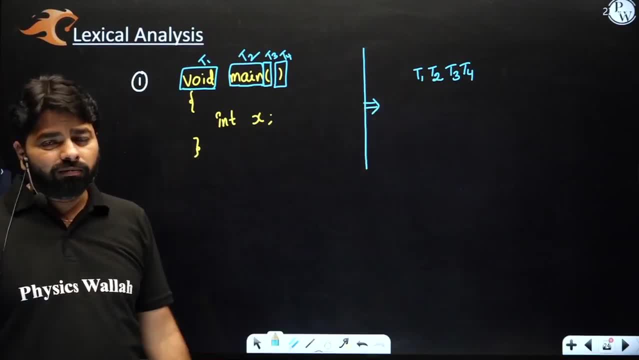 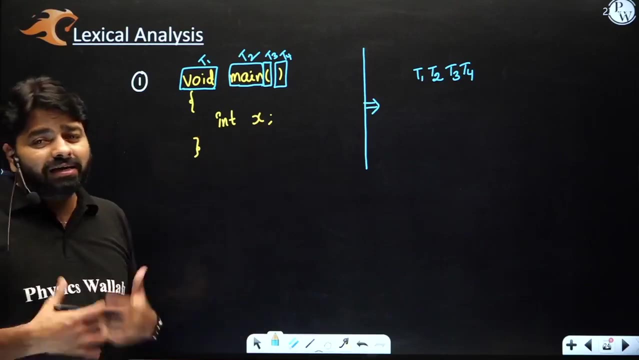 now t5 is. i'm going to write immediately after t4 because the spaces are only to understand how to group the tokens. only right, once you have the tokens with you, you don't need the spaces. in fact, later we also delete the semicolons. in fact, we also delete the declarations, because compiler going to learn a lot from this code. 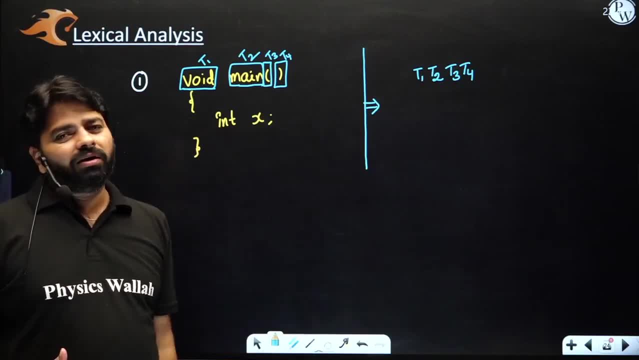 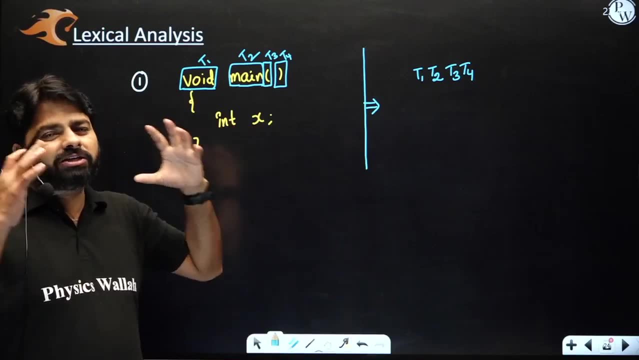 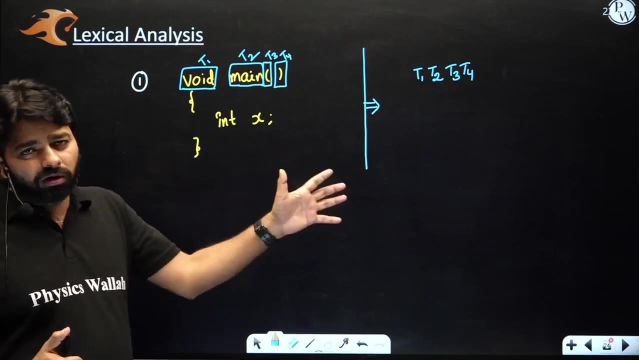 okay, when you convert this code into the machine code, you don't have anything here. it's mapped. this index also it's not there. x is the two bytes or four bytes. it's going to remember the x mapping somehow, so it's. it's something different. when you see the machine code, you can't see the everything. 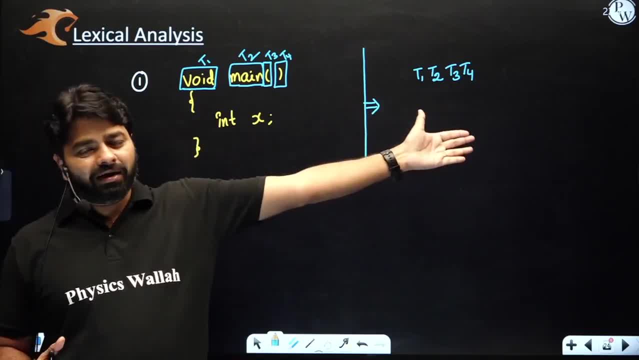 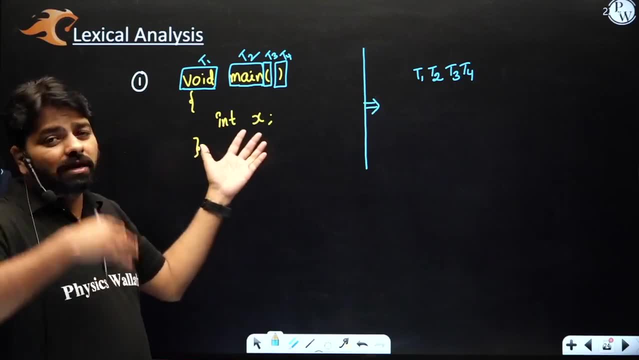 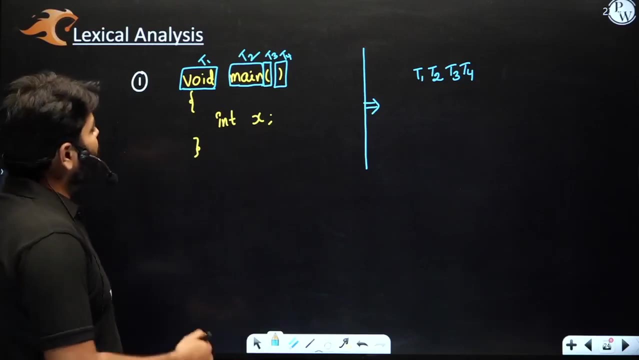 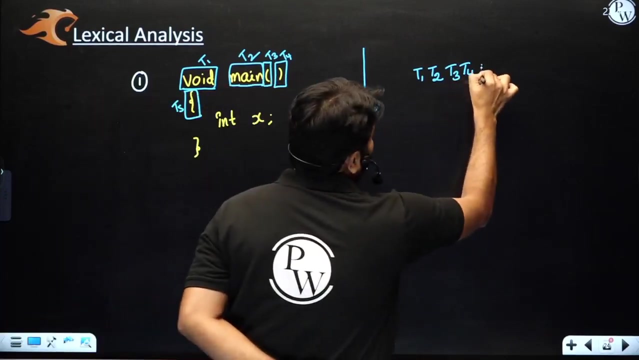 in terms of lines only. this line may not have the line there. it might have the layout and stores this information somewhere. okay, some statements. you will see the conversion. some statements: the compiler does the mapping into some layouts or some other files, data files. okay, now this one is the next one. right, this one will be t5. okay, t5 here, and then a space. 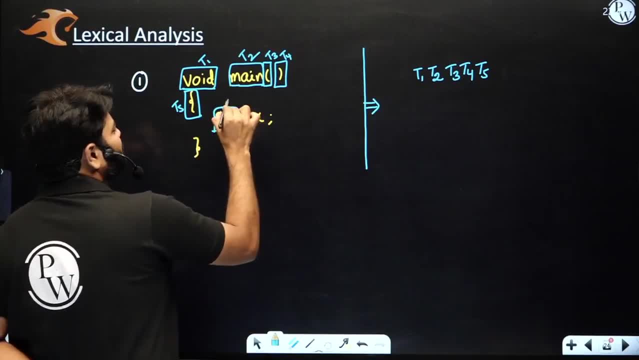 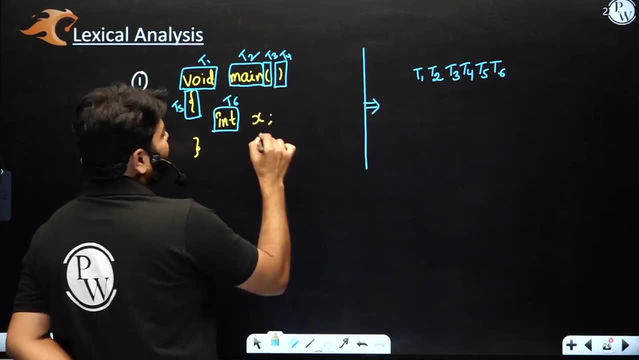 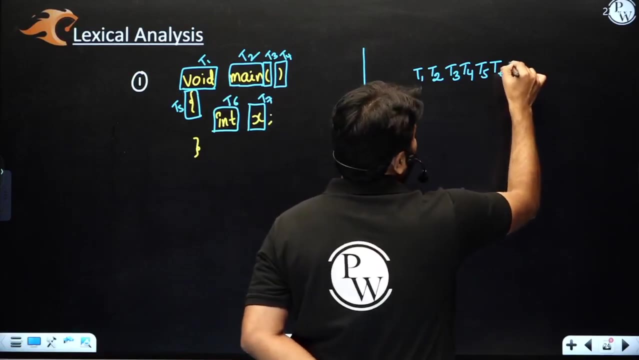 white spaces ignored. and then this one is a t6. see, this is going to be a the token string or token spring, then space. this int is the keyword, x is identifier, this is a t7, and next semicolon, that's a t8. token 8: 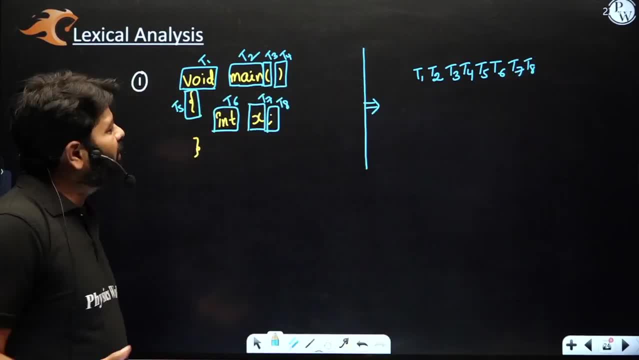 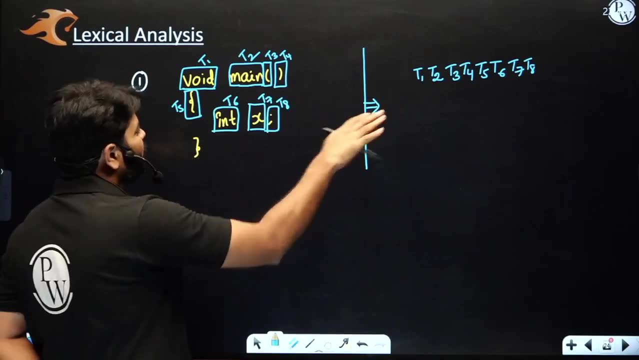 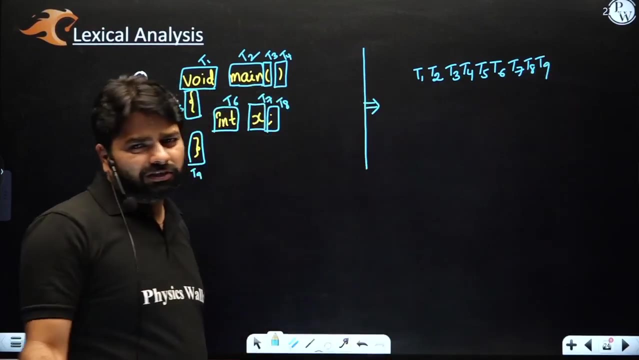 okay, some tokens might be same, like semicolon might be appeared many times. oh, you may give a different token name or same, but total how many tokens total? so far eight, and the last one is nine. total nine tokens. some tokens might be repeated, that's fine, we don't care, but total tokens. 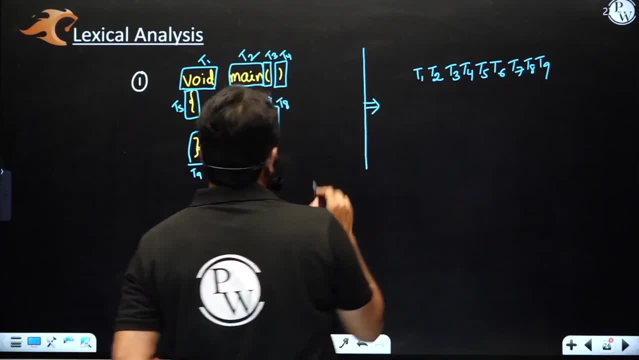 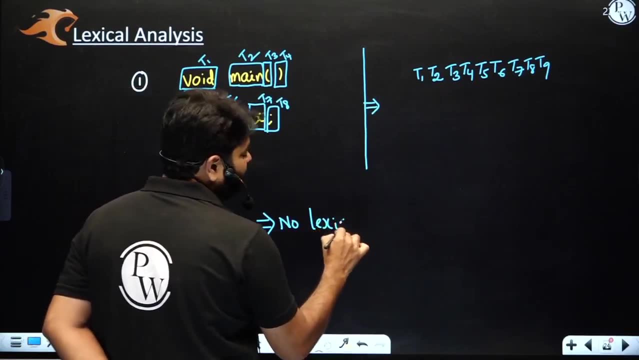 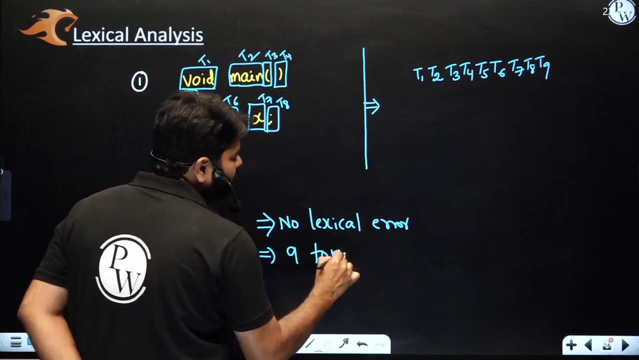 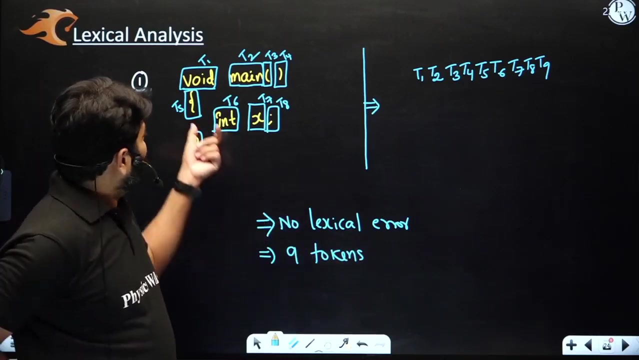 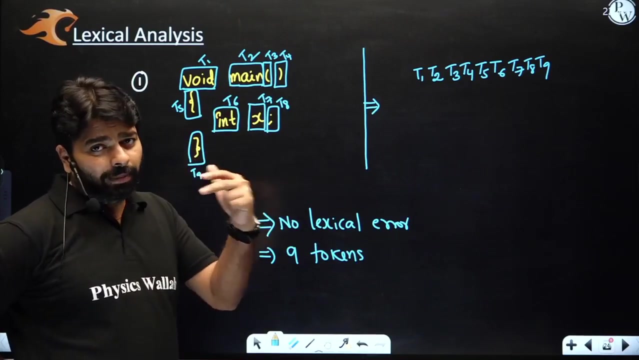 recognized nine. so i can say here: no lexical error, as i'm able to detect the token for every group that i formed- no lexical error. and how many tokens we have here total nine tokens. sometimes it could be possible. how many times identifier appeared while scanning main one identifier X, another input two times? okay, how many times? two times, how many keywords? 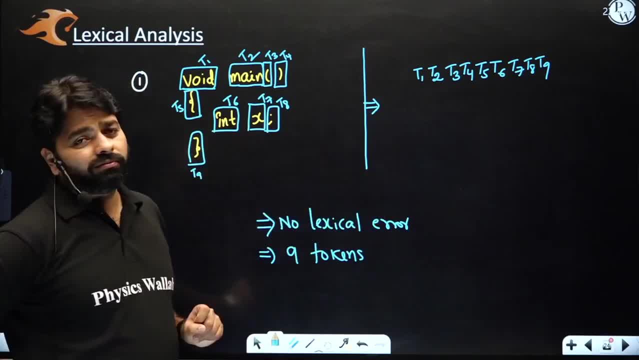 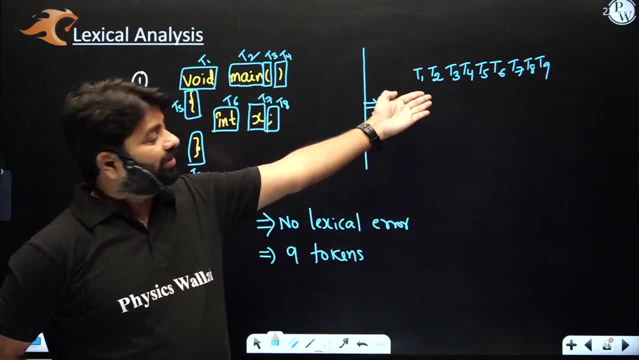 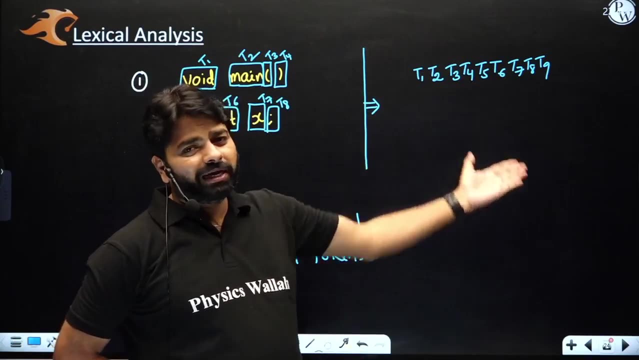 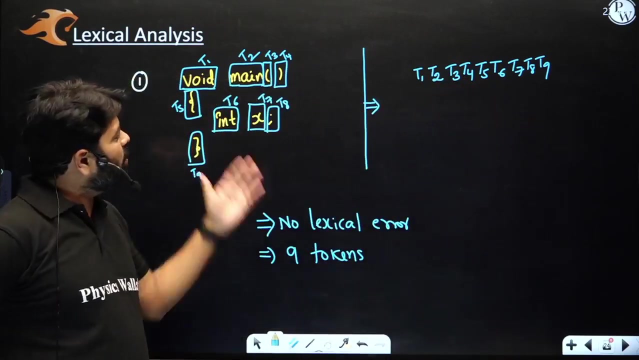 appeared while scanning white int. some interesting questions might be asked. you should be ready for them. so this is the token sequence, or token stream, or simply a string that will be given to syntax analysis. okay, this is with. this will be the input to the syntax analysis. not be exactly this way, but i told you know it's a compiler decision how it has, how it's going to. 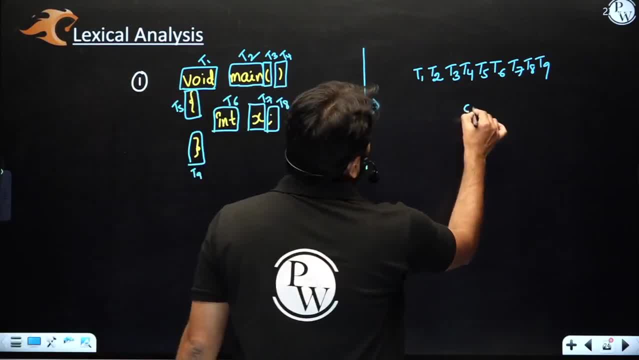 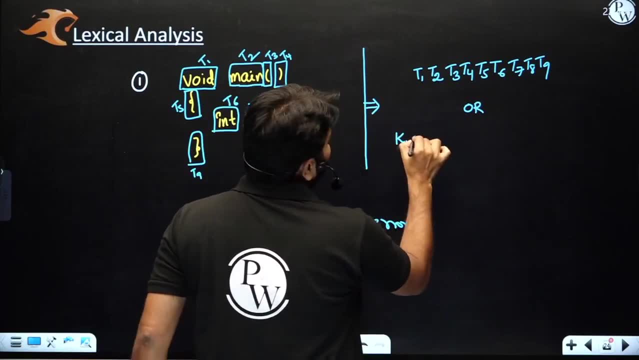 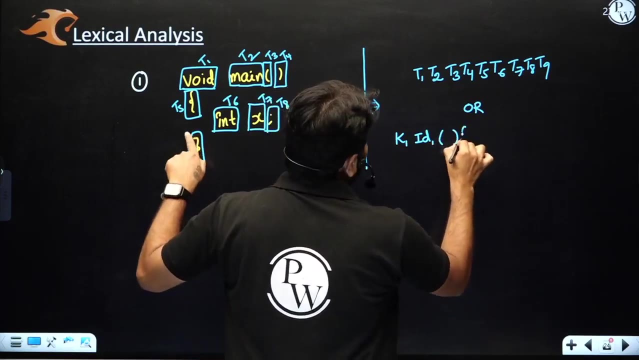 convert, maybe this one or maybe some other one. like the first one is a void, maybe keyword right, so k1 and next one is the main, maybe like id one. next, you know, open parenthesis, as it is close parenthesis, and the open bracket, the int, is another keyword. let's say k2 and id. 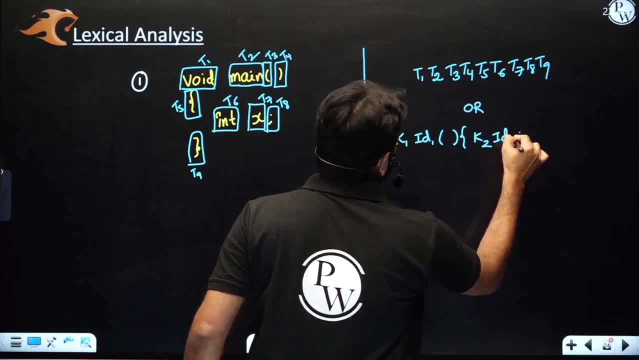 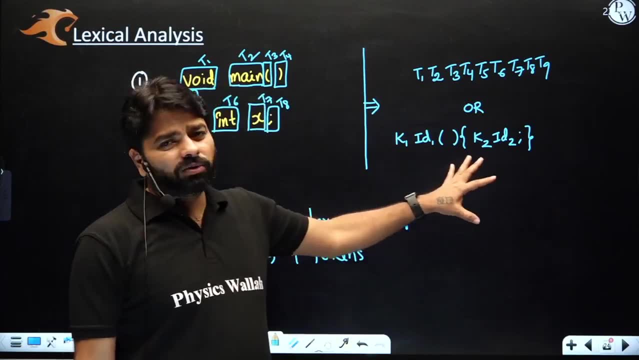 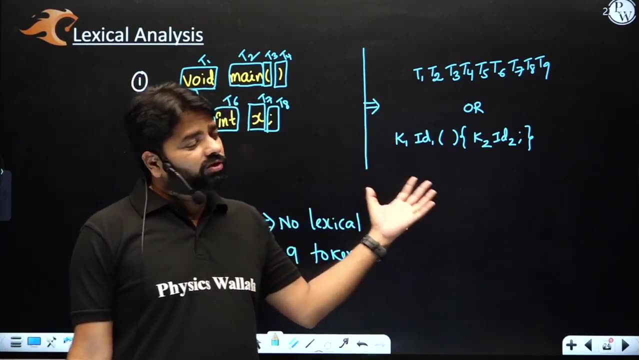 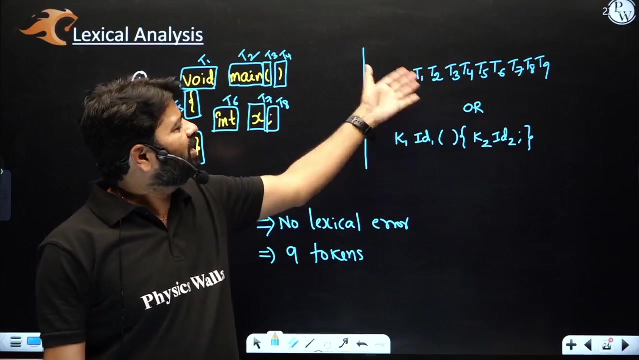 that's the second id id2 semicolon, maybe semicolon or maybe closed. this could be the another possible. the token sequence: that's fine how the compiler does its own job, right, fine, this is how the um sequence of tokens produced by the lexical analyzer. the better way is to you know, understand this one. it's, you know, generalized and everybody can. 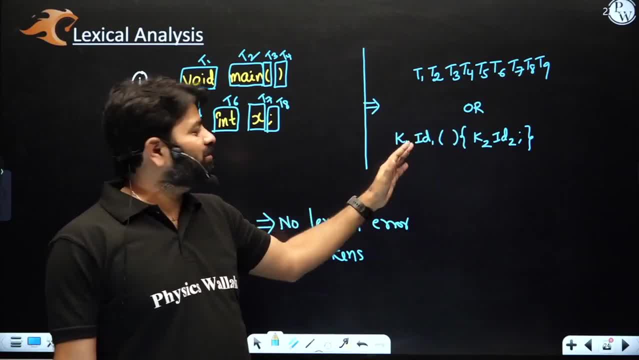 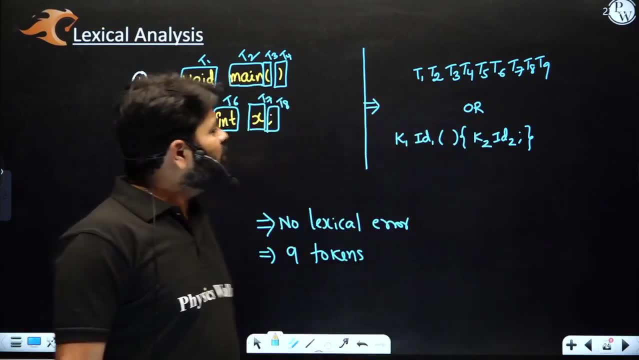 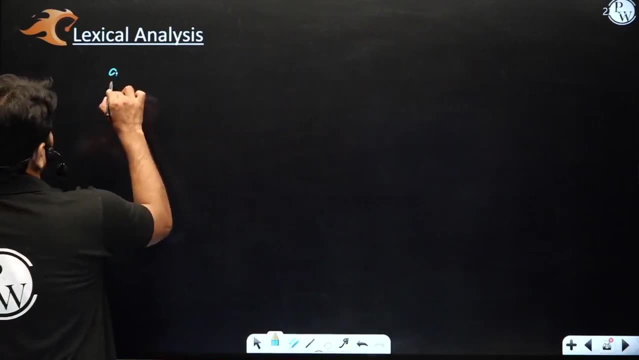 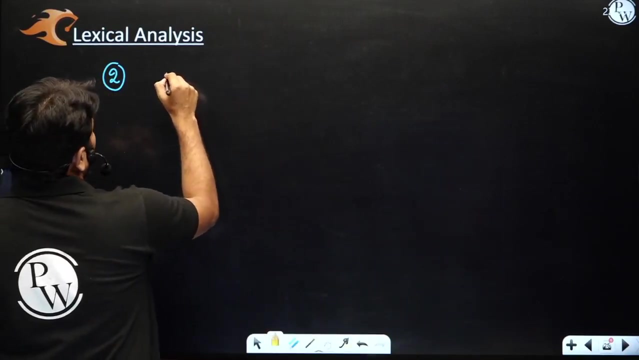 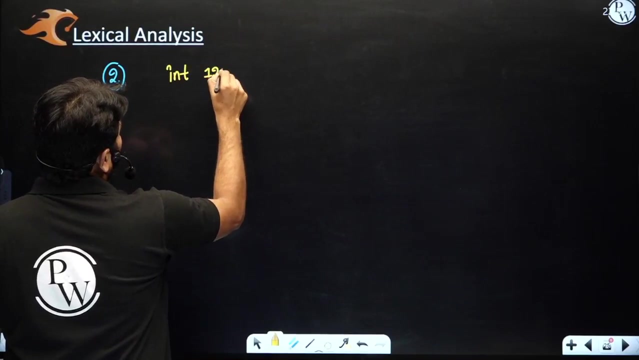 understand. but this thing is, you know, sometimes i keep the same, sometimes i convert into some other labels. you know that. okay, but this is the best practice to do. fine, and now, this is the first example. right, let's go to the second example. int. one, two, three semicolon. 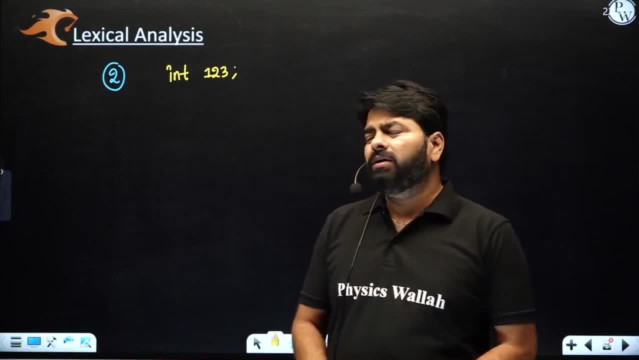 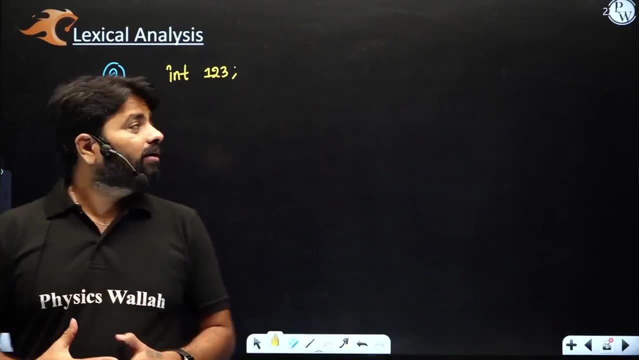 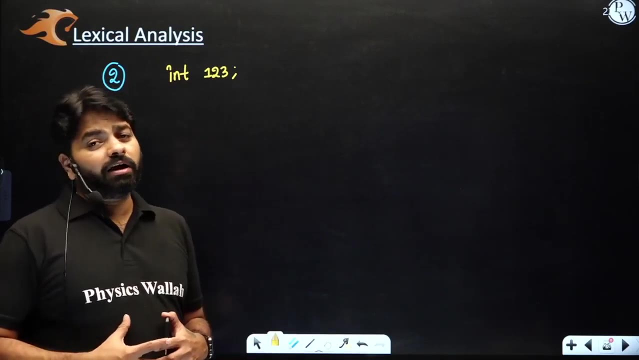 of course you may have a compiler error, but lexical analysis may not identify. sometimes other faces may identify. when it comes to lexical analyzer, yes, the lexical analyzer will not have power to recognize the error. compiler error here. why, when it is trying to group, it looks like everything is fine, you see. 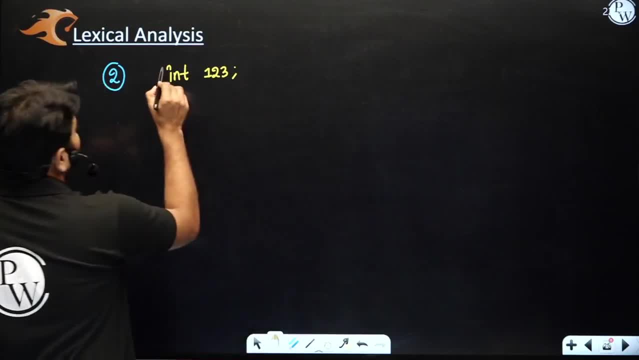 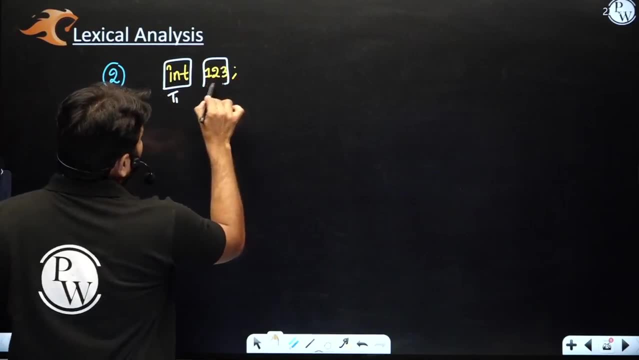 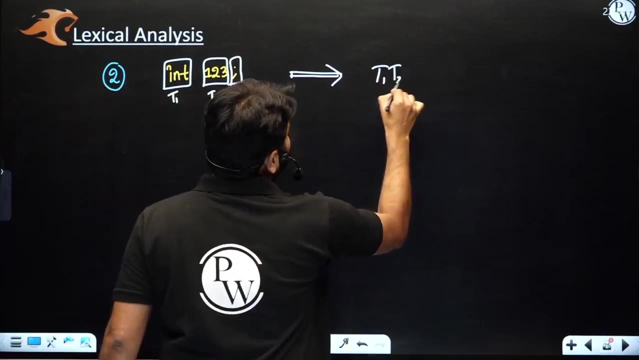 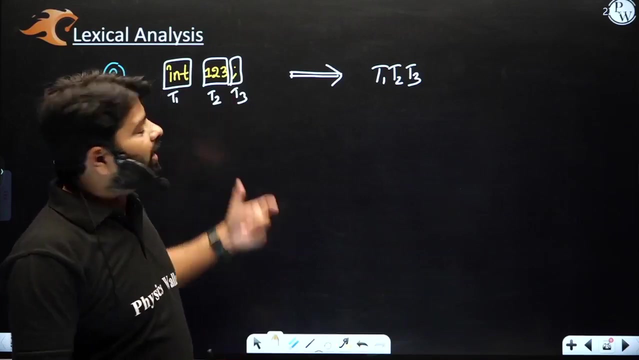 int one group, let's say t1. token, one keyword, one space ignored: one, two, three, it's t2 and semicolon t3, the corresponding output will be t1, t2, t3. that's it. but when you look at the syntax or meaning, you see that the one, two, three never be identifier name. 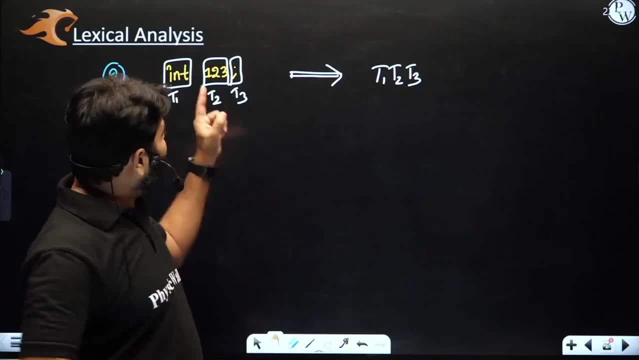 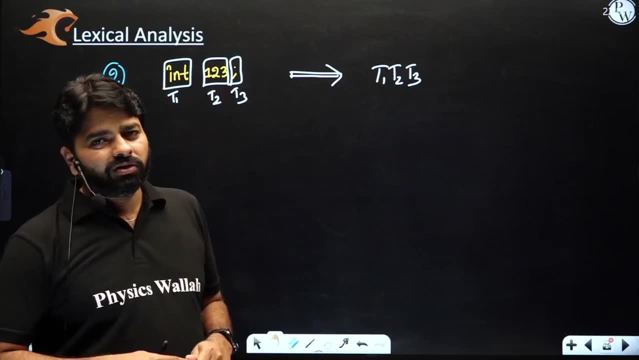 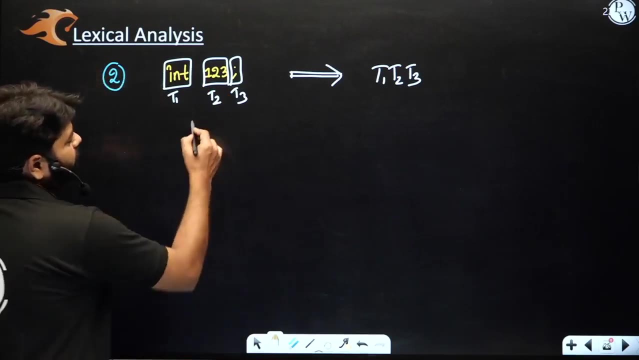 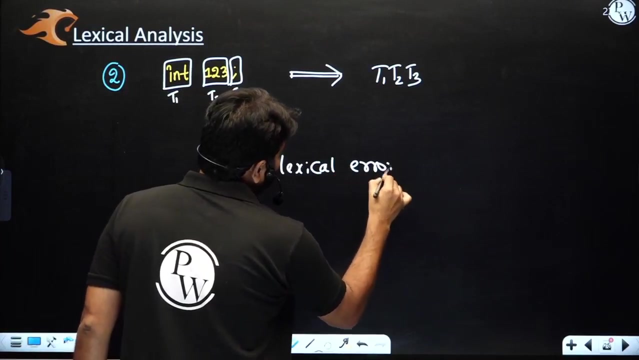 because int there should be variable name, and variable name never be constant, never start with the digit. it's already started with the digit. so syntax is not appropriate. there is definitely syntax error but not lexical error here. so here i am saying no lexical error and definitely which error you will be having. syntax error exists. 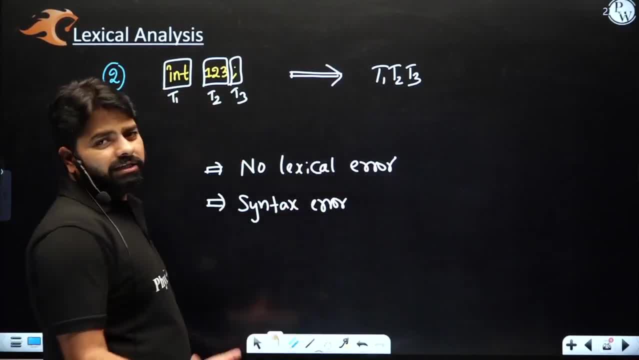 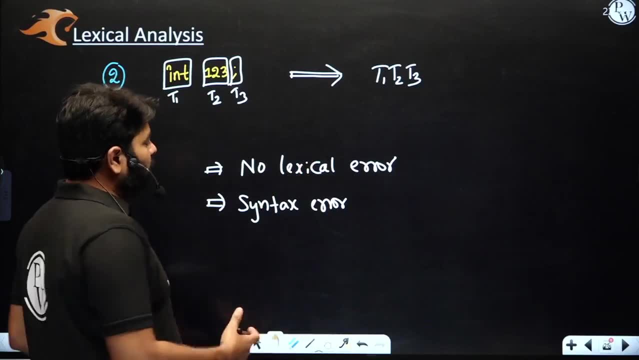 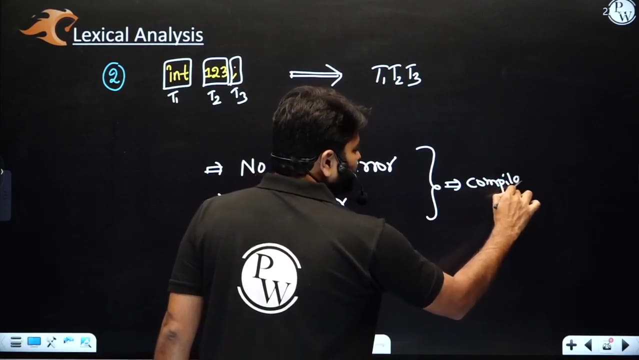 it means somehow compiler error is there. compile error means it may be lexical error, sometimes maybe syntax error or maybe semantic error. so any how, the compiler error is there somewhere. if they ask about compilation error, yes, there is a compilation error, without any doubt. that has not happened in the lexical, but it happened in some other phase. 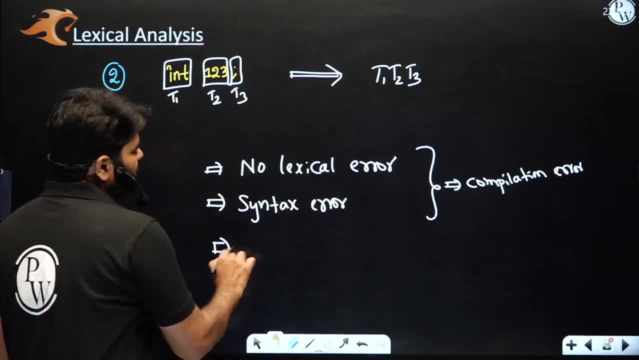 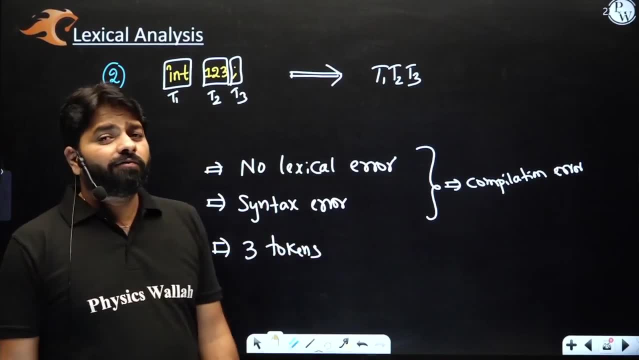 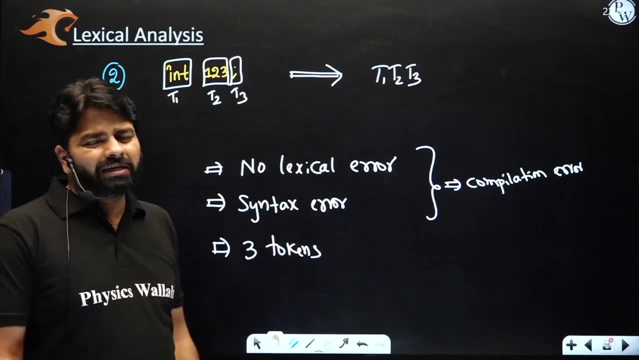 later phases. now, how many tokens? we have three tokens recognized in the program. how many tokens find the number of tokens in the following program? then if this program is given, you should produce or you should say, three tokens. don't worry about, you know, duplicates. like x is appeared 100 times. 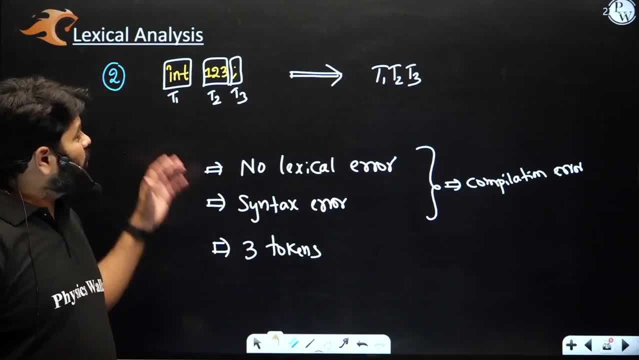 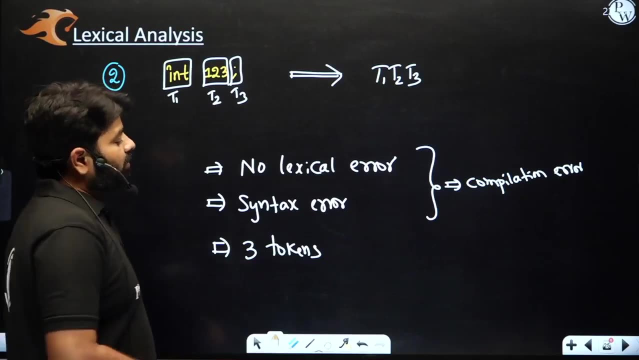 but 100 times. it has to understand that token, right? so when they ask, find the number of tokens, count every token which is appeared while scanning. okay, but compiler understands different way if the same token appears again, again. but it has to recognize somehow. okay, by looking at the symbol table or you know. it has to write. 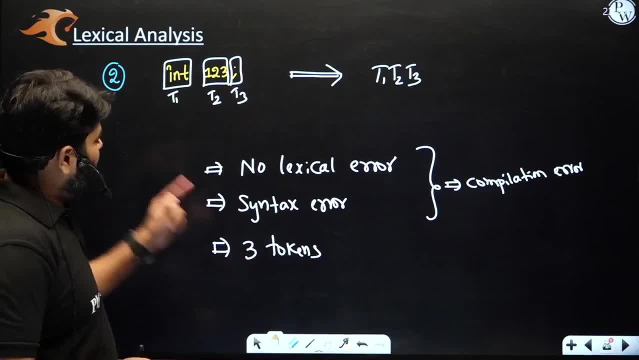 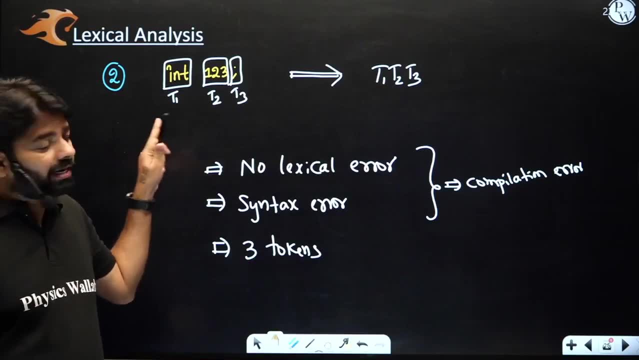 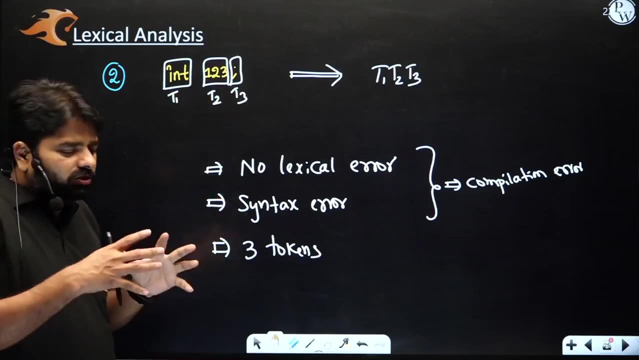 it has to implement internally. let's move to the next one. do you have a lexical error here? no, no, lexical error. do not say lexical error, as it is a syntax error, because after end it is expecting identifier. there is no production or there is no syntax rule in the compiler. uh, to write this line into space, a constant. 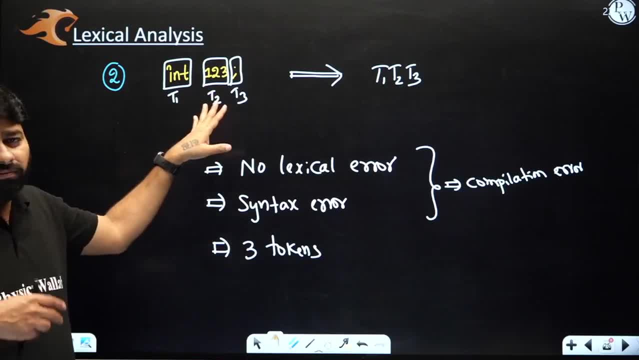 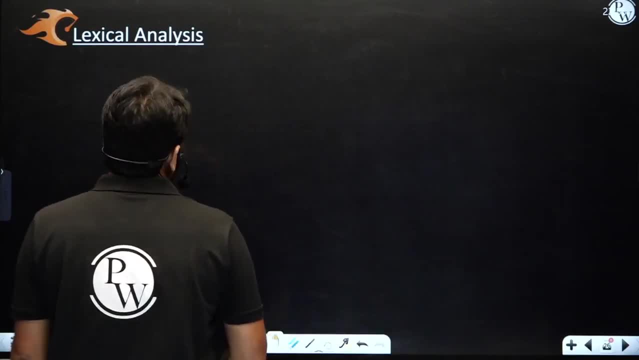 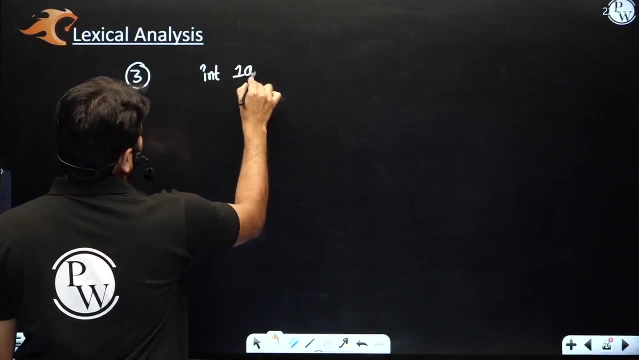 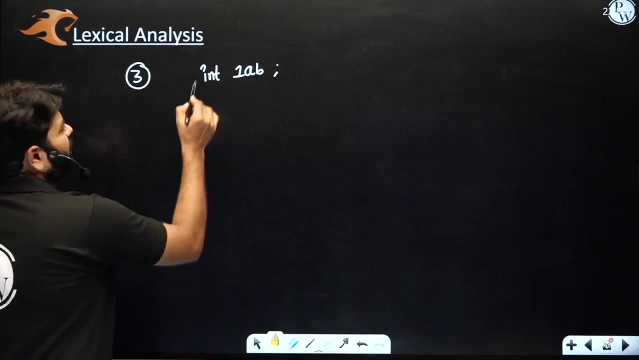 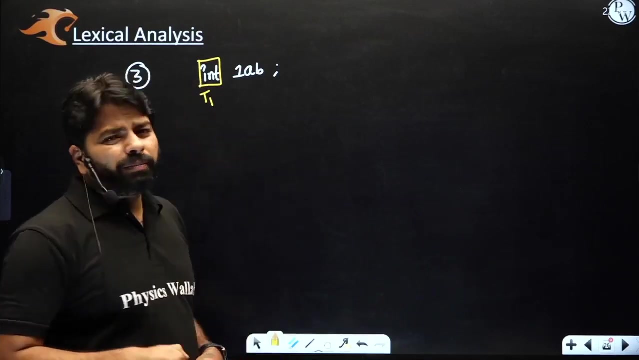 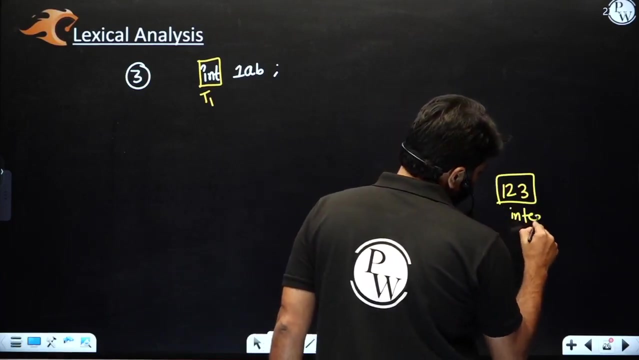 right, it's a one, two, three, and this is uh, very difficult. actually it's not the proper code in syntax. third, one now. okay, now int great token one. what happens? one previously one, two, three. what is it? one, two, three? it's actually one. what integer constant. 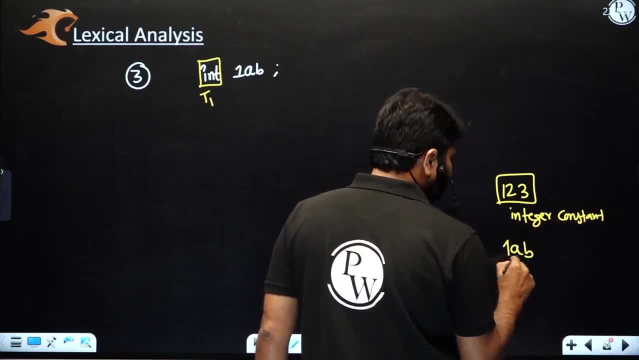 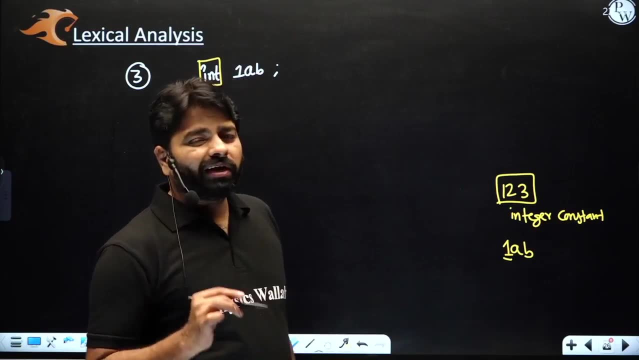 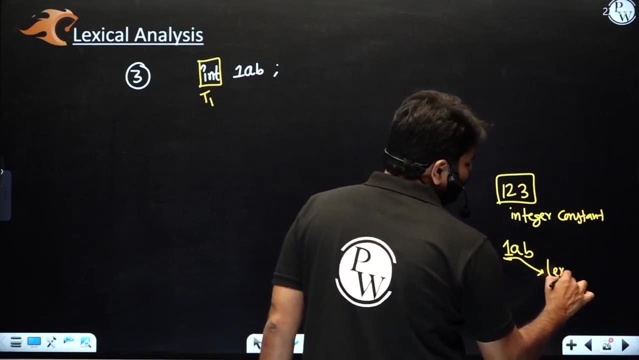 constant. but what is one a b? what is this one a b? when it started with one, it predicting the constant might be coming, but after one a came, then immediately it will produce error. this invalid sequence happened, then lexical error will happen because the a cannot be part of the. 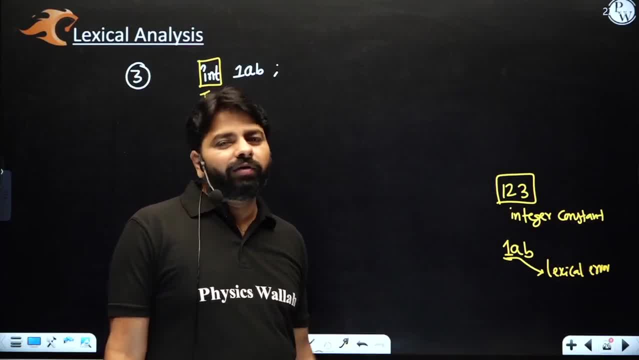 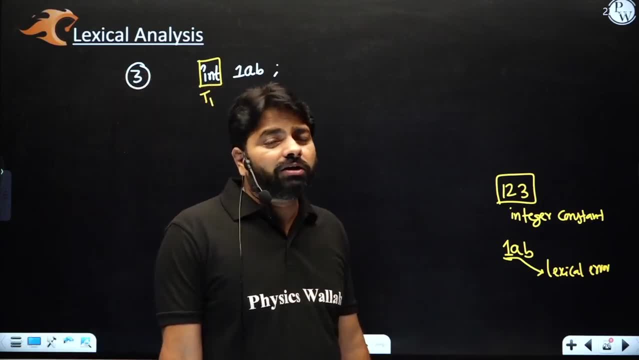 constant and it is predicting constant now because you started with one and identifier name never be starting with one. but i am not worried about is it identifier or constant. i only know that one started, then it should be a constant. that's all lexicon. else it does. it doesn't know you have something before, after, after me, it never looks at. 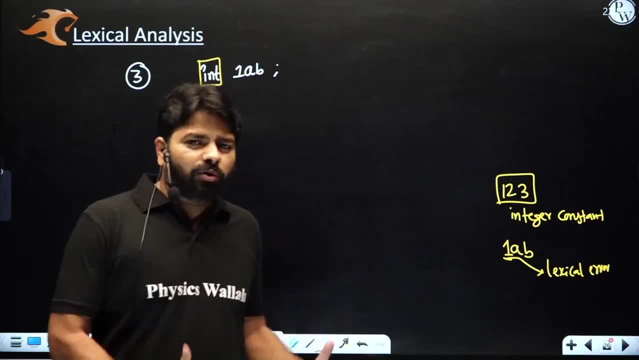 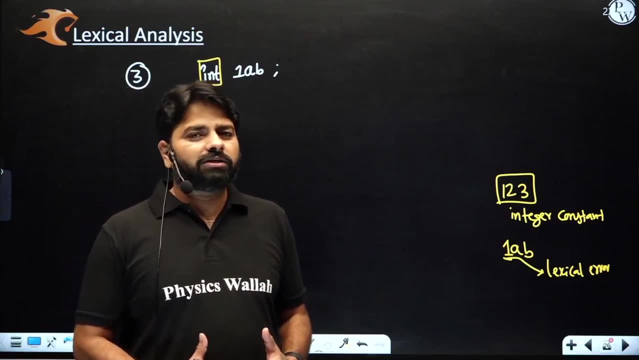 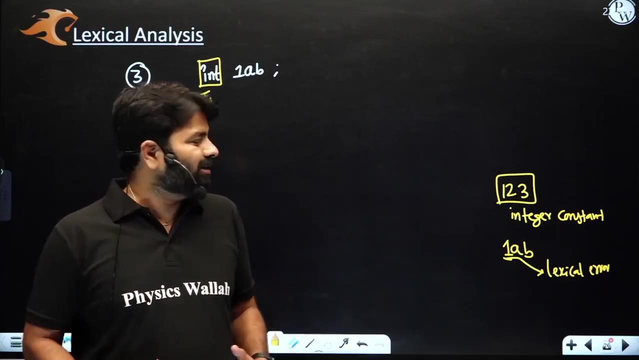 because not going to worried about syntax, it's only worried about what i am grouping. am i grouping something which is meaningful? i started with one means: i should see only the constant, because there is no one will have, will begin with the digit, except the constant, integer or real constant, something like that, right? so here one started that means in compiler, the. 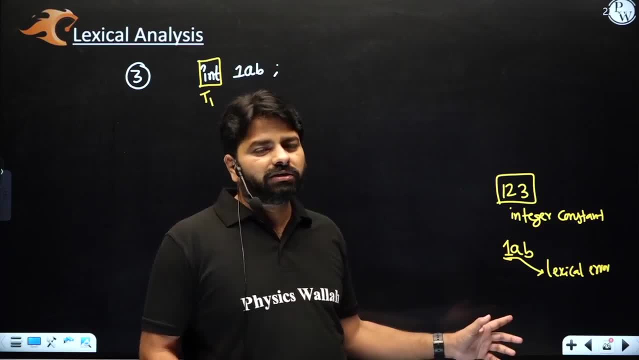 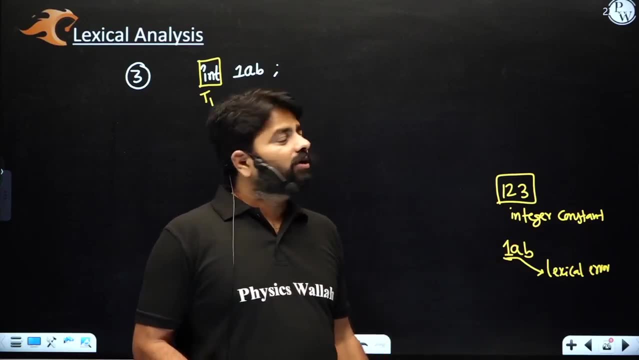 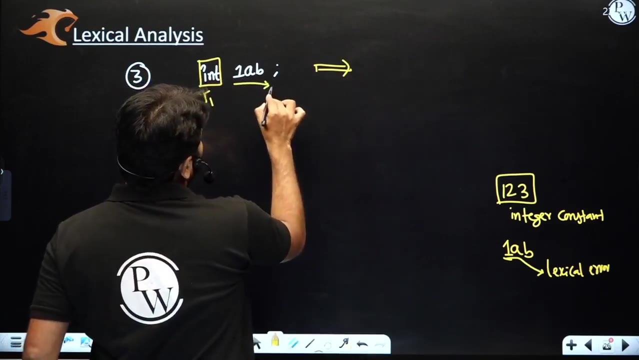 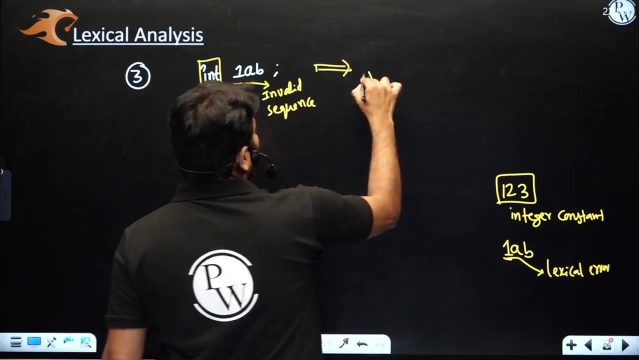 implementation after one. it only looks for the digits, or you know, decimal point, something like that. but this thing, one followed by a, has no meaning to the group. so immediately what happens? it's trying to produce t1 followed by something, but here there is a thick and invalid sequence happens. invalid character sequence immediately produces the lexical error. 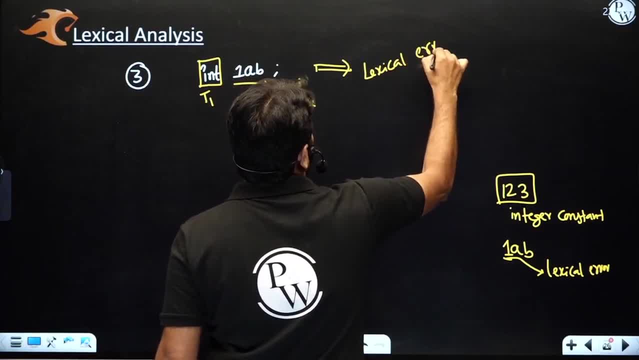 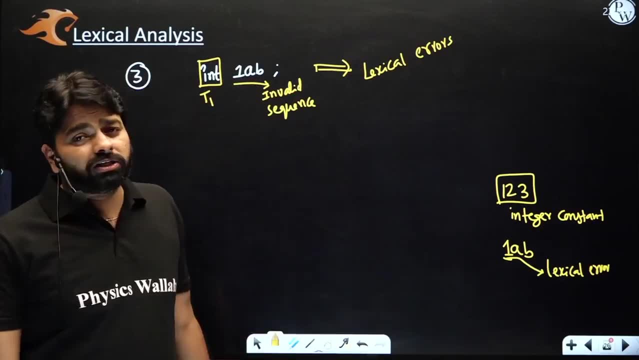 once you have a lexical error, please don't find how many tokens, as already we have, you know, done mistake here. so once we have a lexical error, maybe it will cause a lot of syntax errors. that's, that's the reason. first you keep uh, you know uh, valid tokens are valid lectures. then, 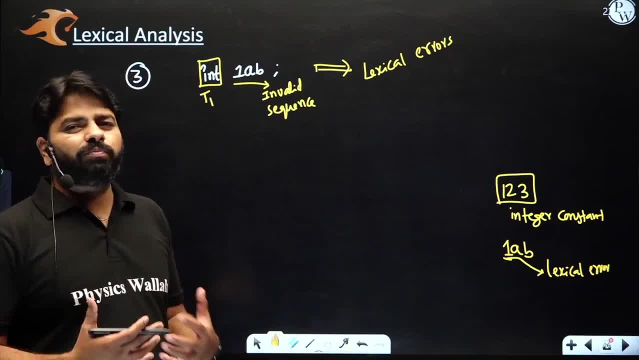 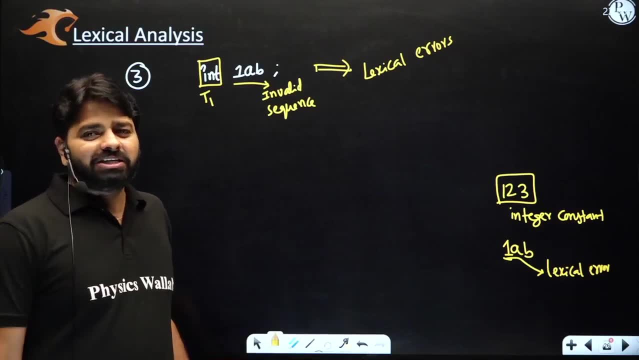 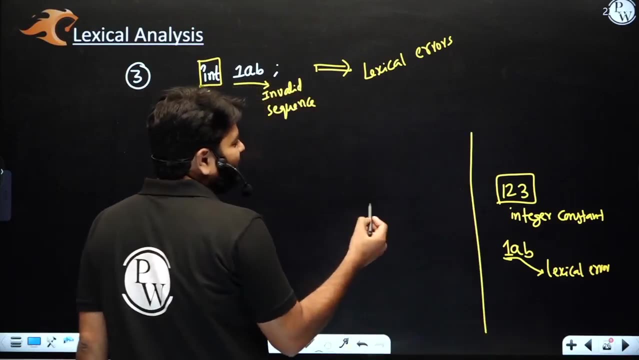 uh, right, syntax properly, then check for the proper semantic and your program may be logically correct. still, we cannot guarantee lexically, syntactically, semantically correct till you may have the logical errors. so how you know how many things you should take care right, see when you are writing a. 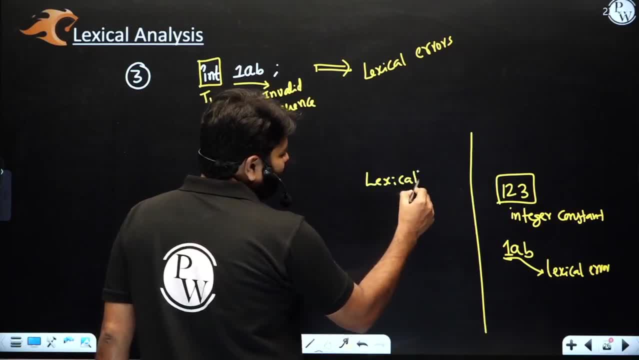 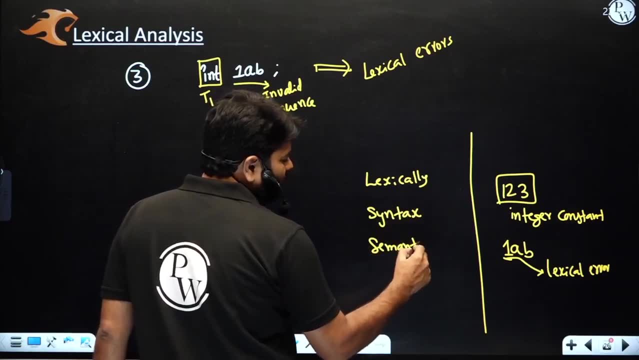 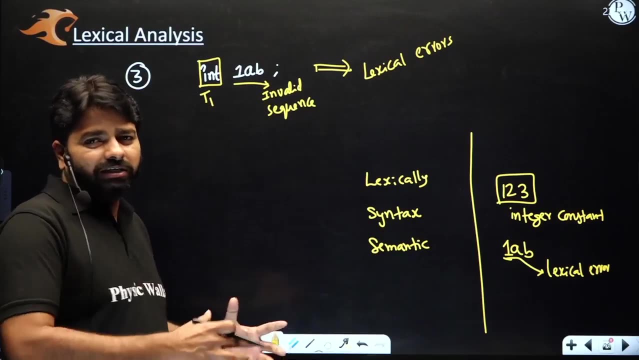 program. first ensure your program lexically valid. then syntax check properly. then semantic, all the types have you done properly, like expression, left elixir, also id for eachOH. we need an parameter outdoors for lexix to determine out: say you don't as al salut, but you cannot11. you need that. 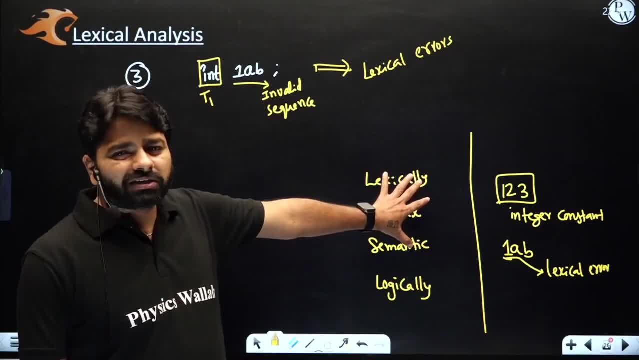 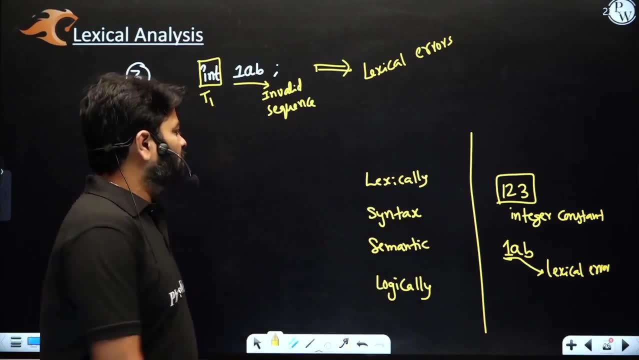 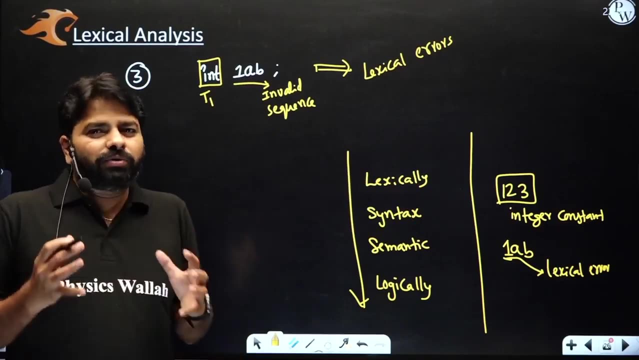 flow into your procedure if you can insert function subtれ simply, and now you will take a product from each. so let us complete the notebook. currently, the program of the program is 100, 100 prevalence, which is a program at least one of its 10 and you will get knowledge of. we need your logic: never something quickly and safely. 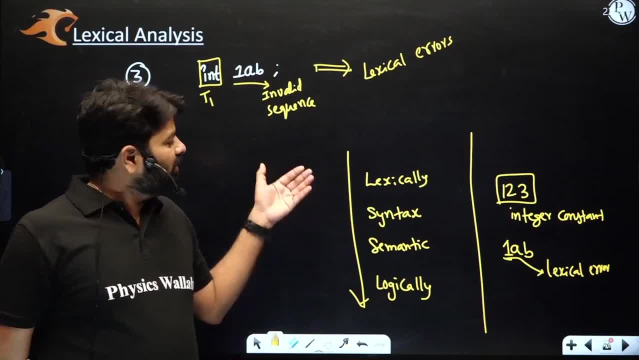 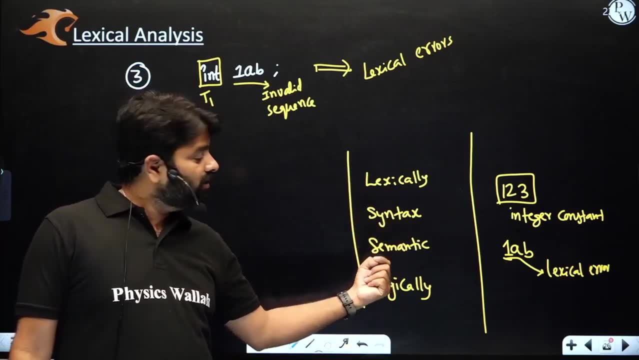 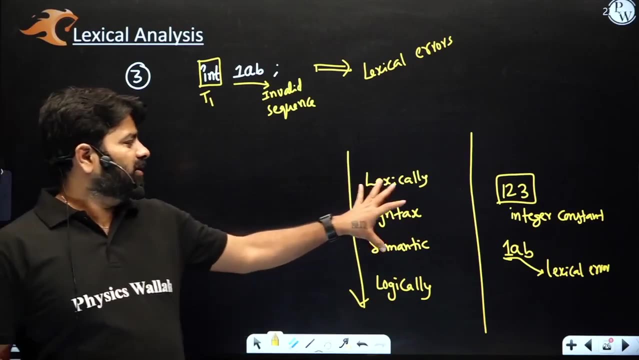 if you write invalid token, then you will have syntax, semantic. everything is possible. so ensure lexically valid, then ensure syntax is correct, then ensure semantic is correct, then at runtime you will get to know whether your logic is right or wrong. okay, you will focus on logics, but the 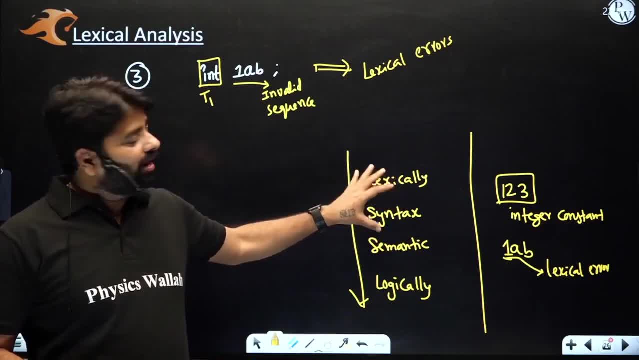 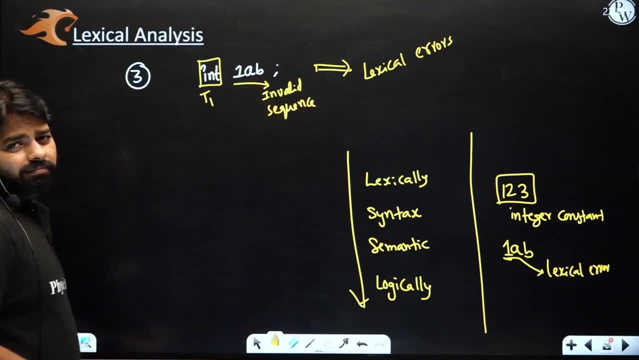 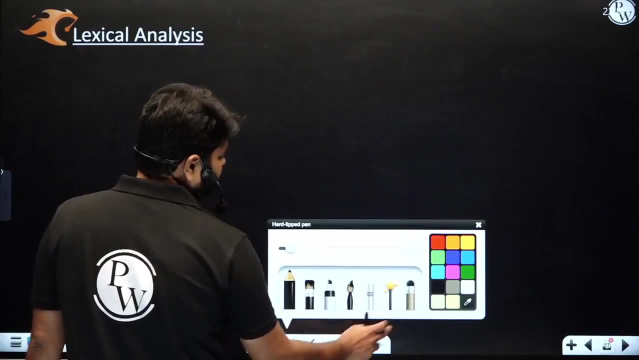 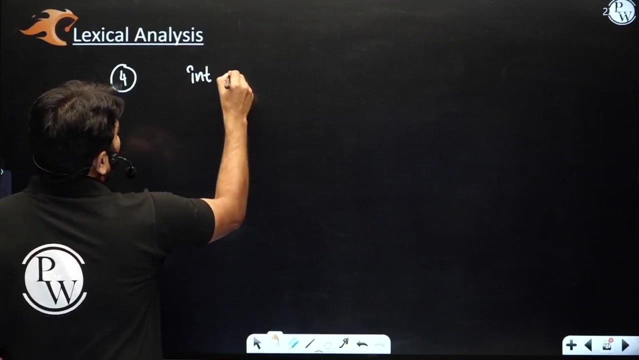 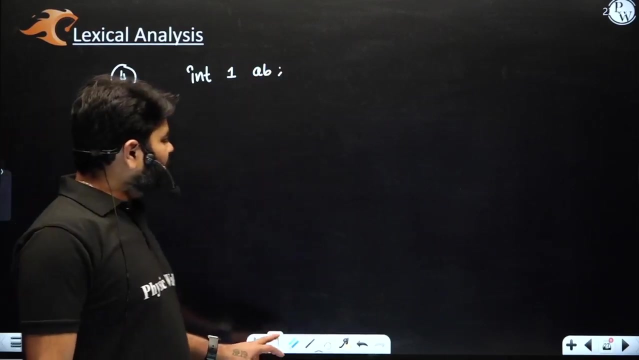 system will not understand your code unless you follow the compiler rules or language rules. fine, this is the lexical error, right? third one is a lexical error. let's go to the fourth one. the fourth one int say one space, a, b and then semicolon. now what happened when it is trying to group? 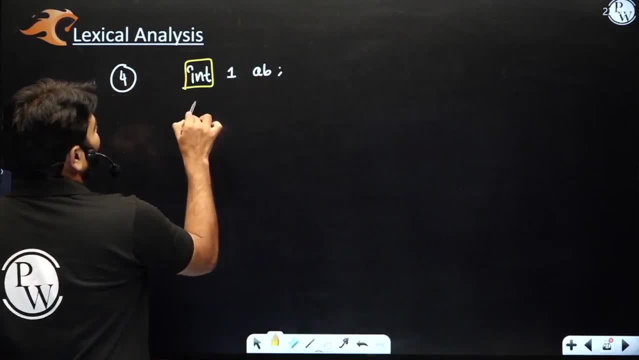 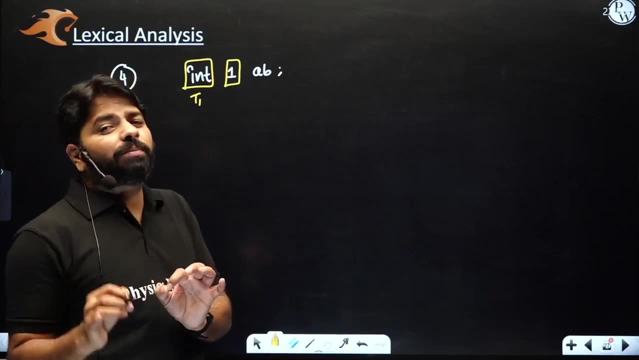 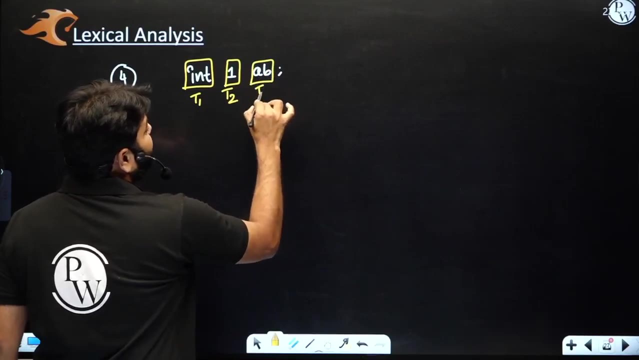 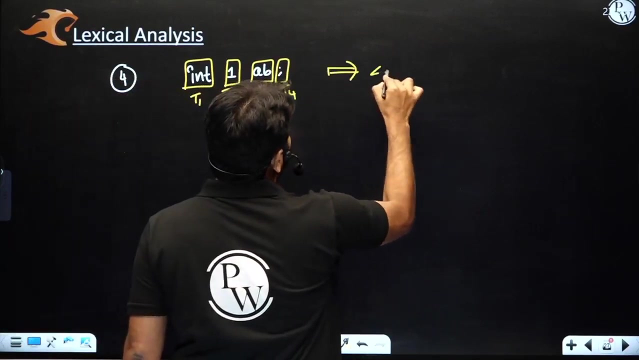 it groups. now int is token one, one is, oh, one, space. i told you space is going to separate the tokens at any cost. so one, it's constant. now a, b, it looks: identifier, semicolon, special symbol, punctuation. now it's going to be four tokens. no lexical error, but there is a compilation error. 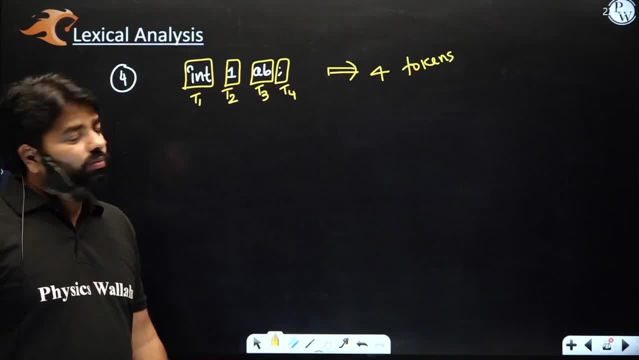 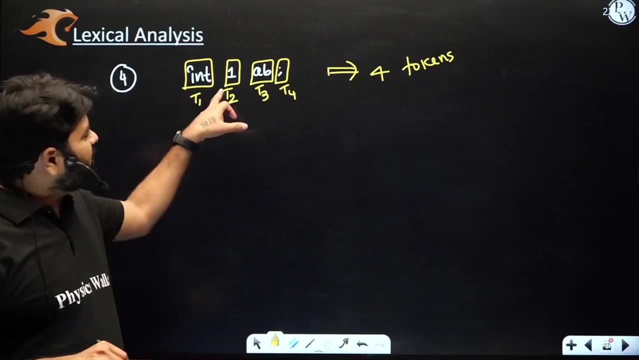 what compilation error syntax, why after int you are writing one. one actually represent what you can't stand there. so this is not going to be updated just after integer keyword or float keyword. so already the grammar has rules. this one should never come there. one is not going to come there. so here the syntax error present. 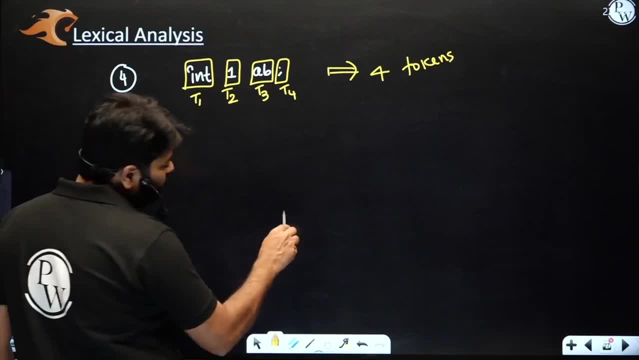 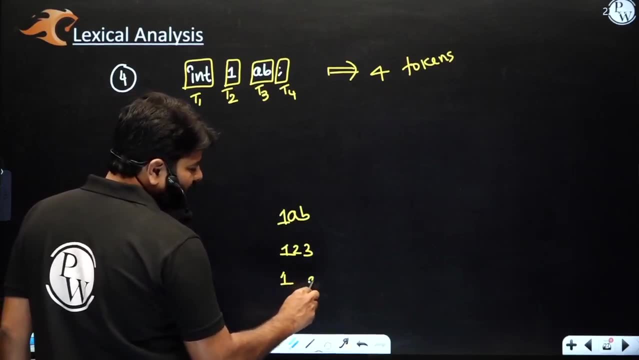 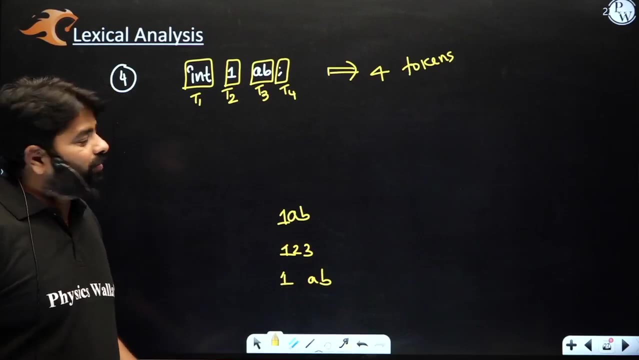 but not lexical error. previously you have seen, when you write one- a- b error. when you write one, two, three- no error. when you write one space a- b- no error, because this are actually not contexto errors. going to look at what i am doing, not who is there before and after. that's what the lexical job right? 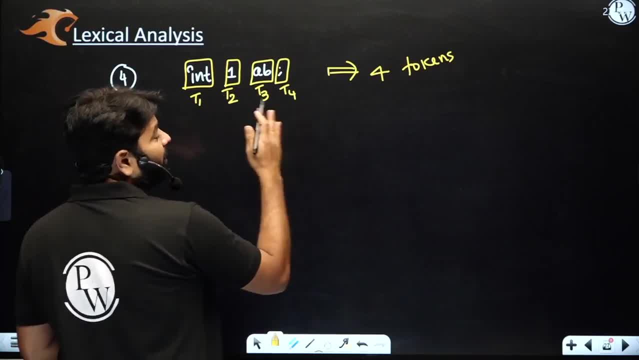 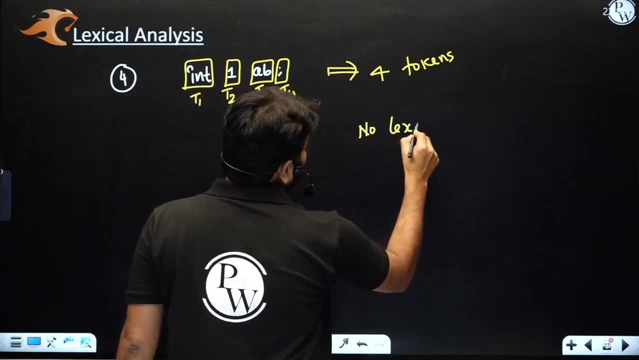 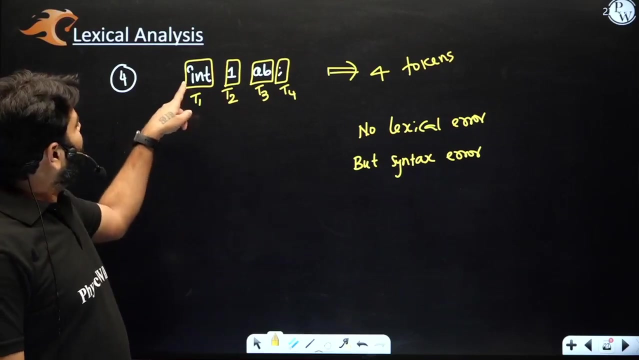 so this is going to be no error. because of the space it's going to assume two different tokens. but there is here syntax error, but not lexical error. but what do you have? but syntax error exists. why syntax error? you should go a compiler and check the grammar and after then can you produce. 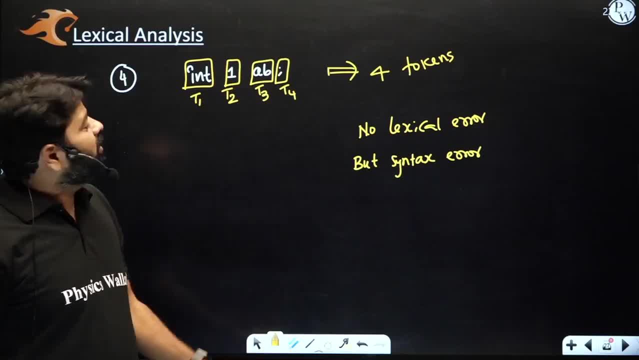 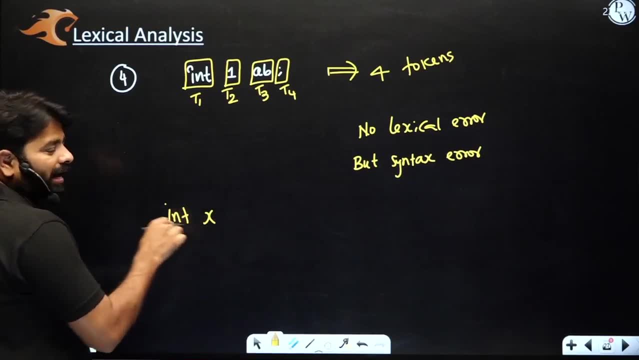 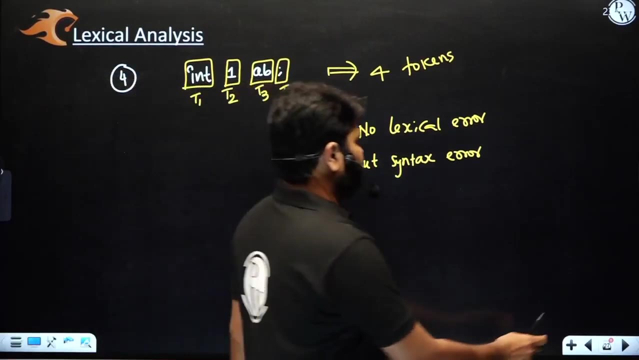 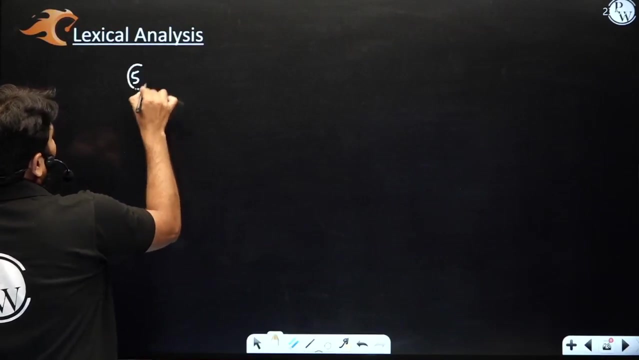 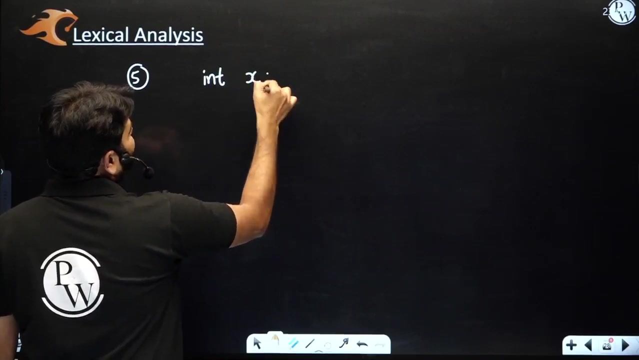 a number or a constant, not possible. that's why it's going to always. you have seen right int x int temp. you need some variable name there, identifier, there, clear this point. fifth example now. sometimes you write the comments right inch x semicolon. you write some comments here. 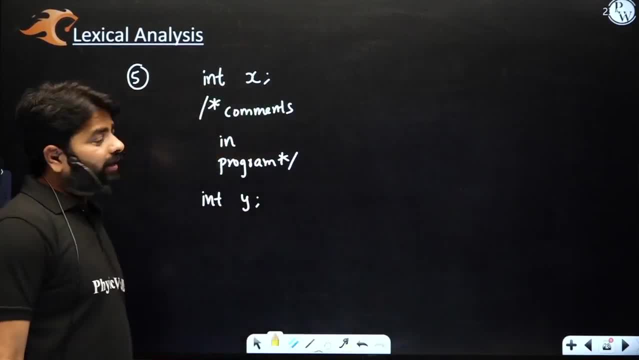 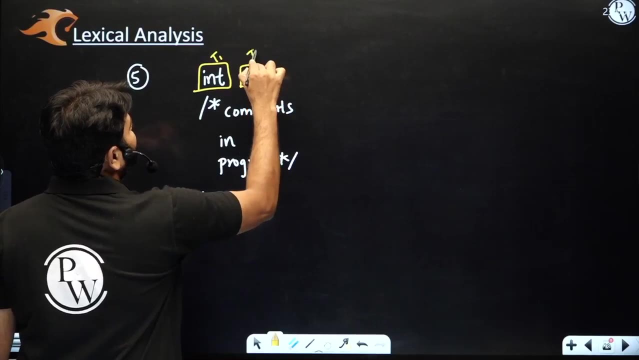 okay, what happens now? i told you that, uh, the comments are identified by the lexical analyzer and also ignored, because it's not going to be considered as a token. what it does is it's going to be producing token one for this, token 2 as an identifier, token 3 as a punctuation. 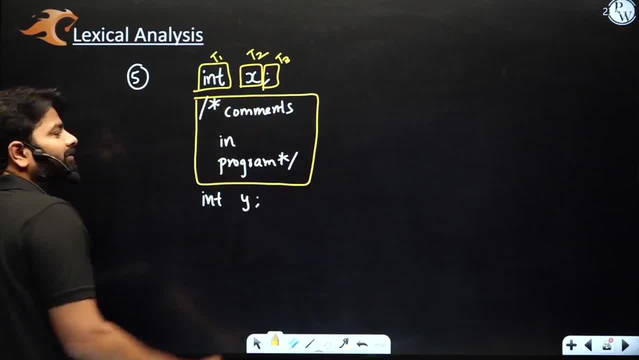 and this thing, whatever you see here, how it's going to be identified, how it's going to be identified, how it's going to be identified, this comment is going to be identified, identified with the pattern. you see this pattern: right slash star. it's called as a begin. it will. 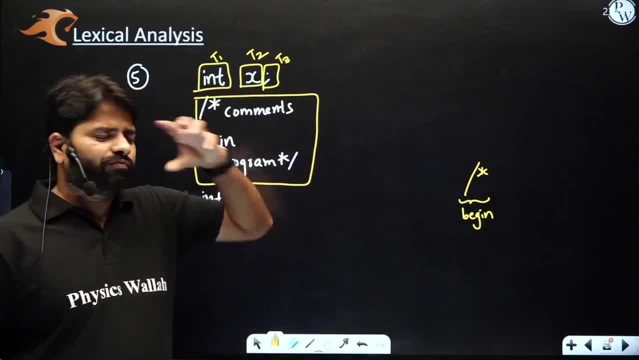 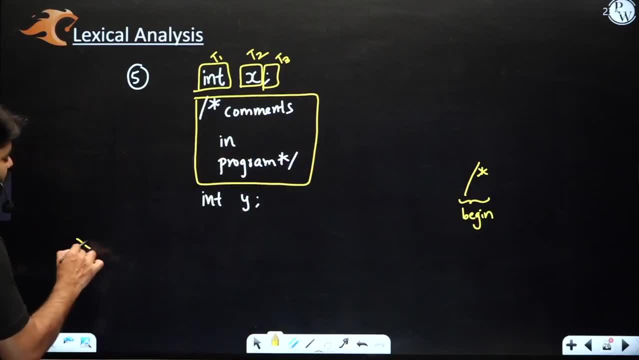 not look for end at all without have a begin. this is very, very important. it's begin occurred, then only it will look for end directly. end happens without begin, it will not consider as a talk comment. it assumes, like you know, you are writing multiplication or division some. 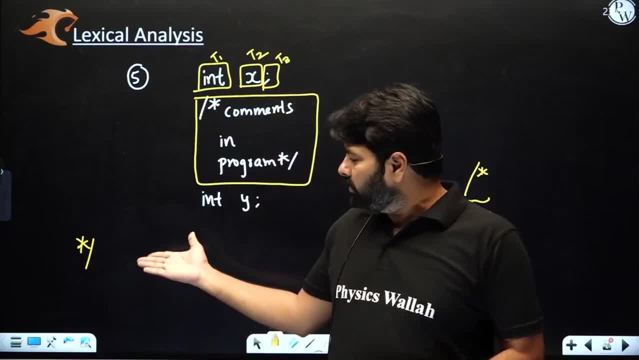 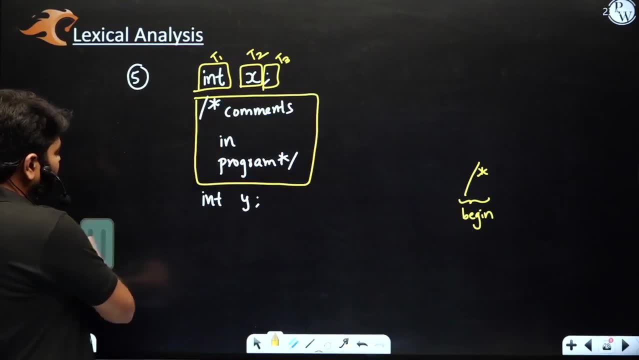 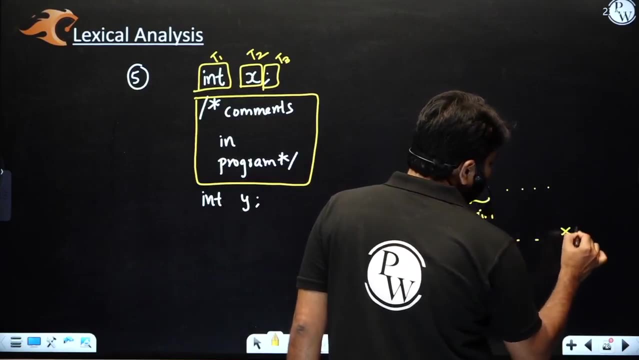 operators you might be writing, so it's not going to understand this. uh uh, it's not a pattern at all. right, without a begin end. it will not understand because the pattern will have the begin and end rules. now this begin and then it has to end somewhere with a star and slash. this is what. 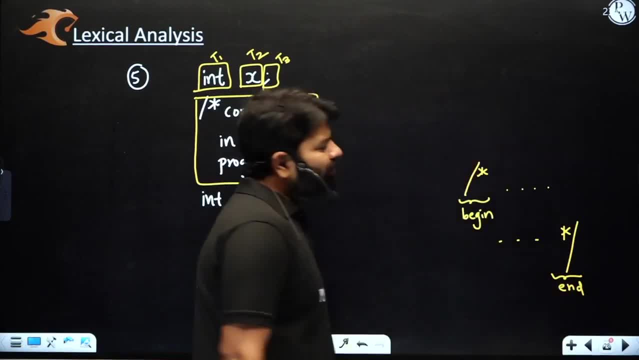 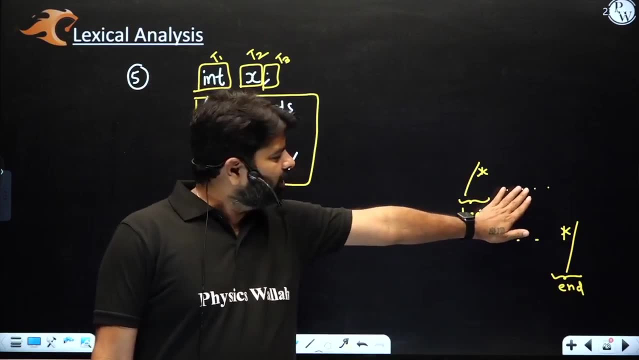 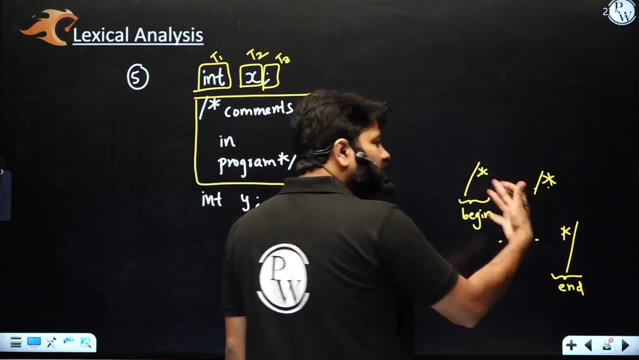 end rule in between: doesn't matter what you write before star slash. if you don't have star slash here anywhere, it will simply assume comments right. even you write one more star slash, doesn't matter. it just consider as a part of the comment, because this is already begin. 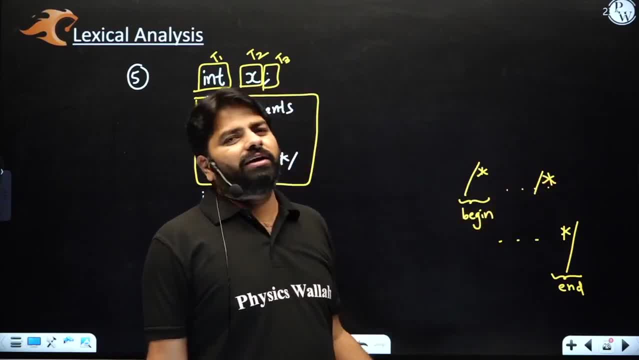 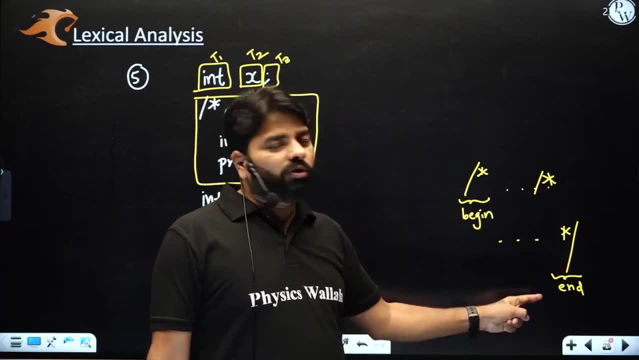 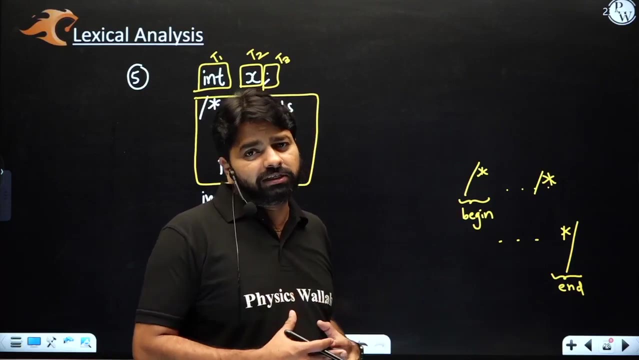 happen, it will only look for end. now, if you give again, begin it it will not care. it will only care where is the end. so remember what is happening, begin and then only look for end. if begin not happens, then it will never look for end. so begin is the very, very important sequence. now it's a 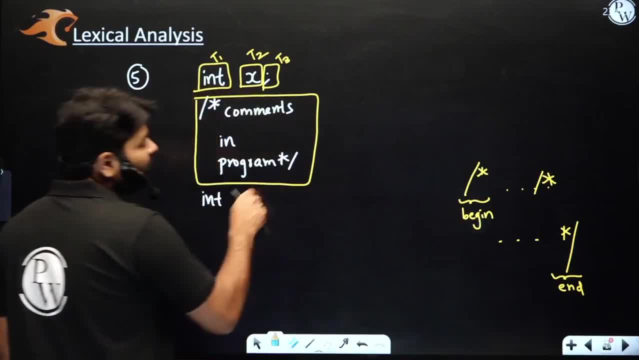 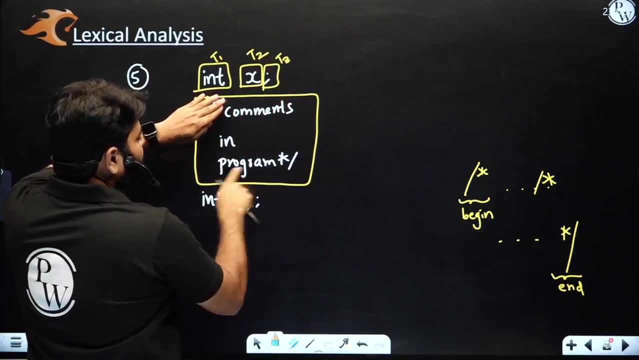 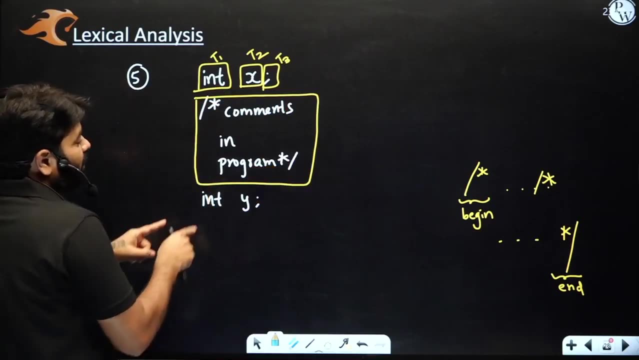 begin happened here. that is the only reason it's looking for end. if this is not going to happen, it will not look. it will start here. okay, comments. identifier in identifier program identifier: star operator, slash operator. it will do some other some way, right, so be careful here. this is happened. 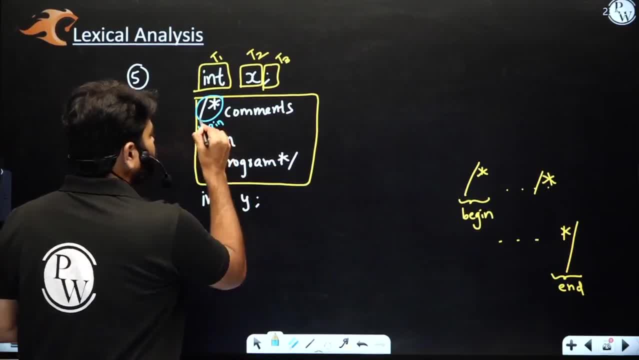 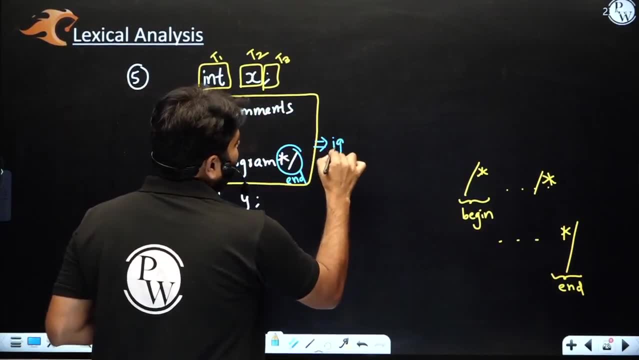 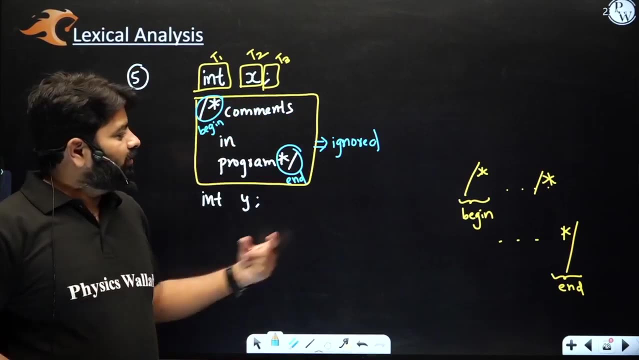 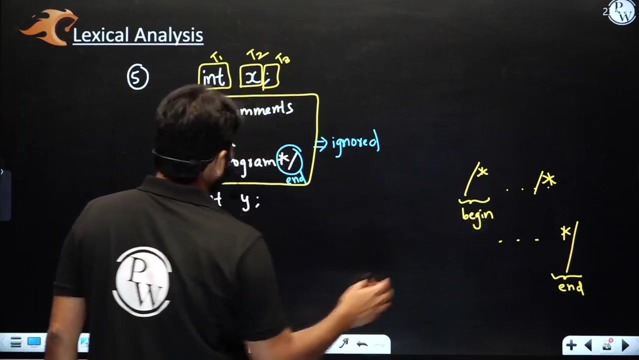 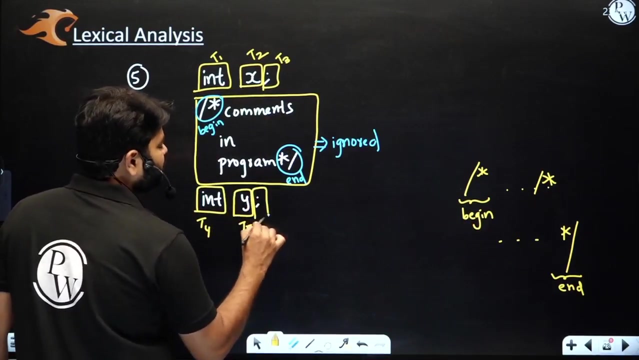 so it's a begin rule of the comment. so it's look for end here, end rule for the comment. so whole thing is ignored, simply ignored or deleted from the program because the valid comment. so it's identified with this rule. that is the reason it's ignored and later whatever is after is another token: t4, t5, t6. how many tokens? 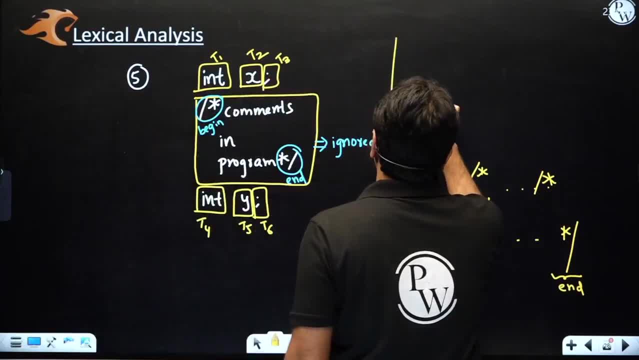 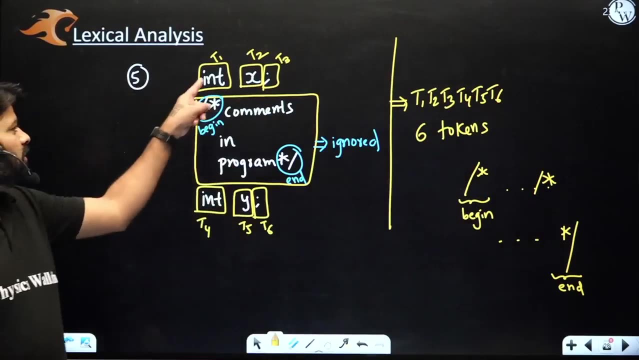 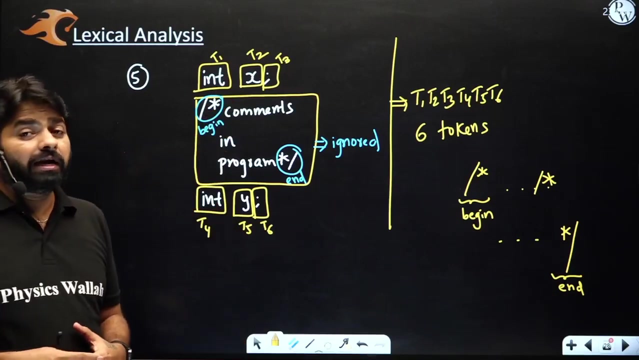 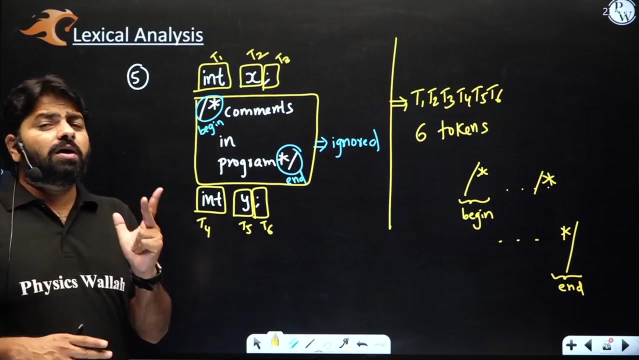 it is produced. it's produced something like t1, t2, t3, t4, t5, t6. total six tokens stand in the program, among them two keywords to identifiers, because keywords identifiers are, uh, the easy way to recognize rather than operators and other special symbols. okay, and constants are also easy. so keywords, identifiers, constants are pretty easy. 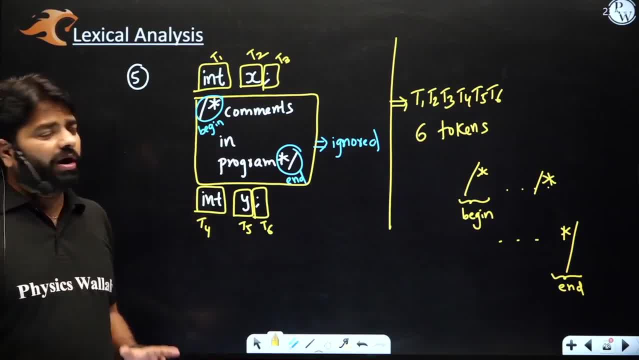 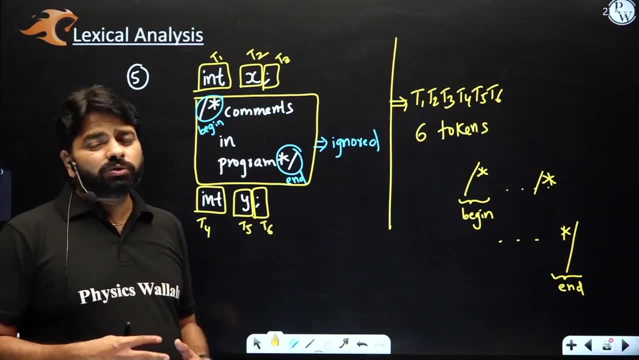 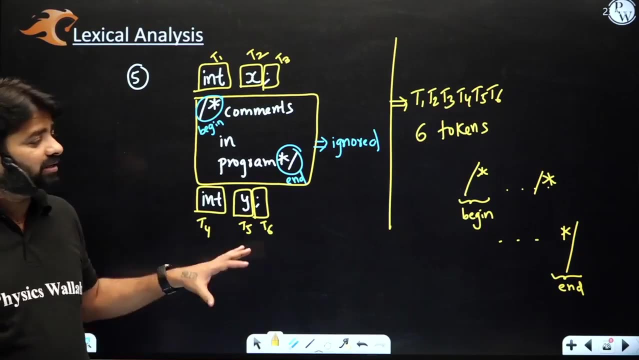 than operators and punctuations. why, uh, they are not easy? because sometimes you don't understand the operator or punctuation. okay, like you know, if i say open panthers, closed panthers, that comes under panthers and really difficult to uh understand. is it one token or two tokens? that's why some things uh better not to discuss about them here. 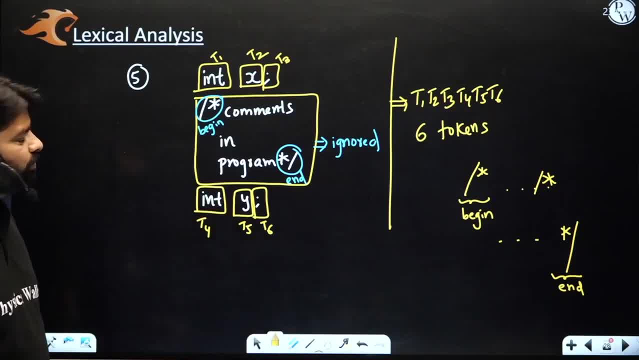 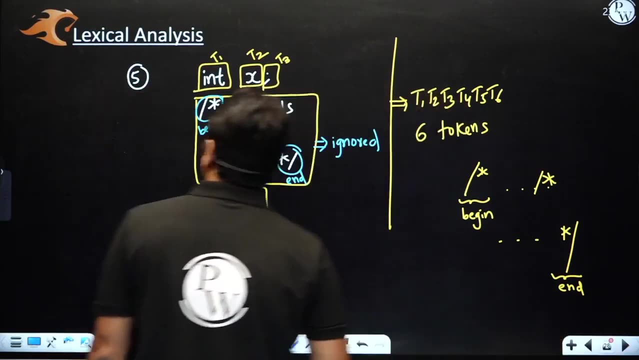 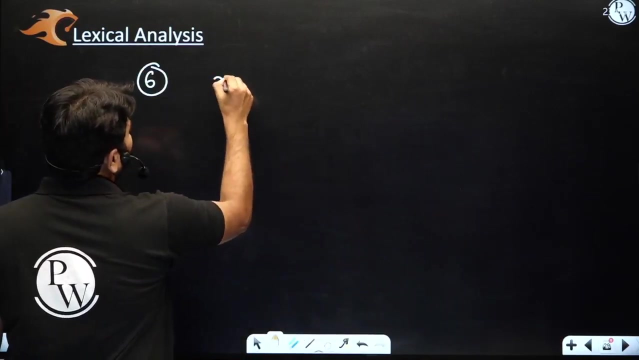 okay, this is about the fifth one. now let's move to the another example. do you have any error here? no error at all. no error at all. right, there's no error in this. it's compilation successful. will will be successful. no doubt. the sixth one, when i'm writing something like in the program: don't worry, main, i have not written. 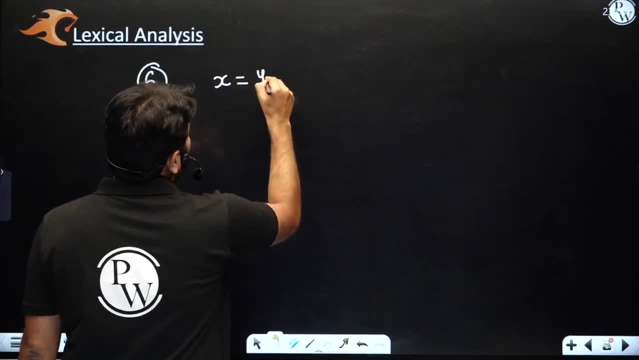 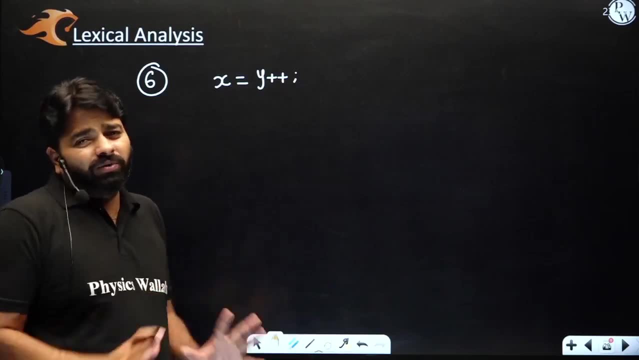 but still understand. x is equal. somebody written y plus plus semicolon, don't try to understand the meanings. also, don't say that x is not declared, y is not declared, so we don't care. now, who is going to care that if you have written this code within the main, within the main? 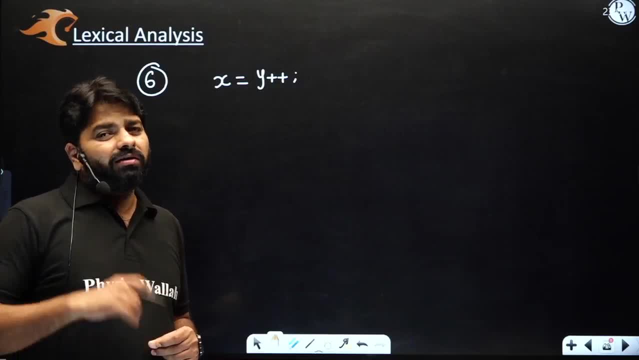 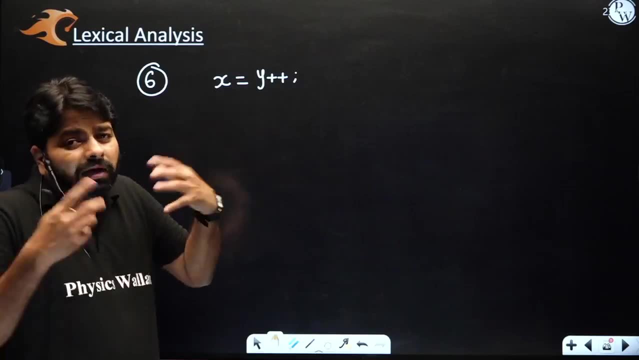 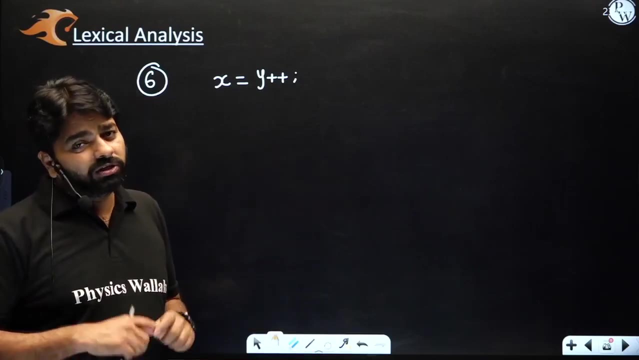 is going to care that x is not declared, y is not declared. the semantic analysis then, the syntax is correct, lexical is correct, but semantically x and y don't have the types, because symbol table it is going to look at, it's going to trying to store the types but you don't have the types it's going to. 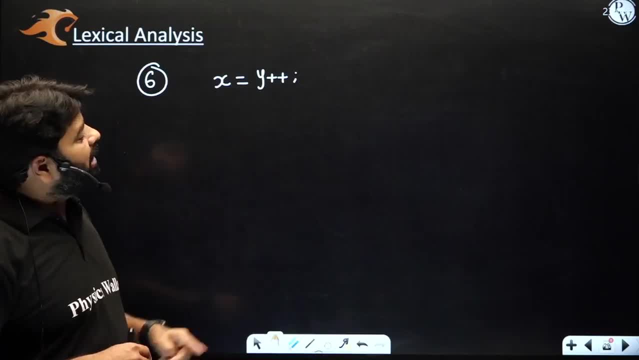 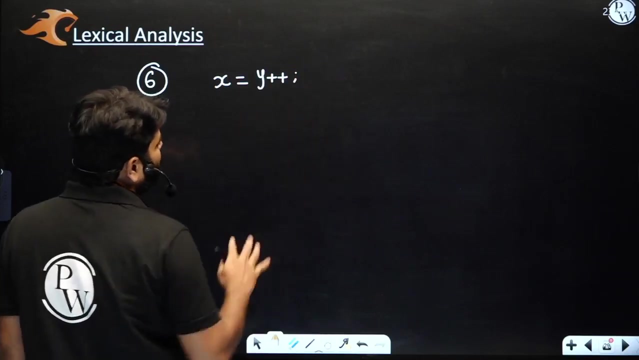 generate the semantic error. semantic error: this one is lexically correct, syntax is correct, but semantic is wrong. okay, so semantic analysis produces uh error where the type mismatch happened to lx and l value and r value. okay, fine, what happens now? how many tokens you have? how many tokens you have? 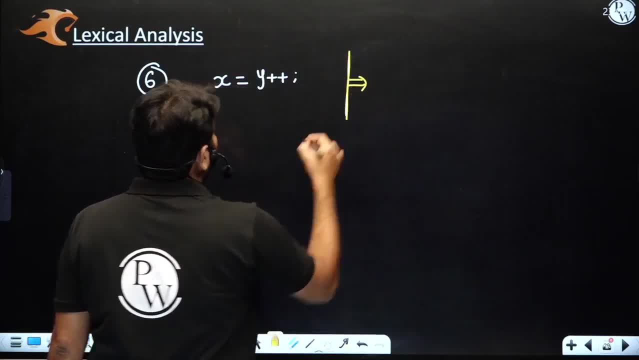 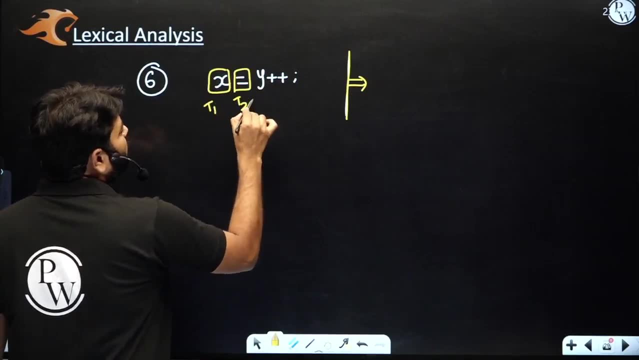 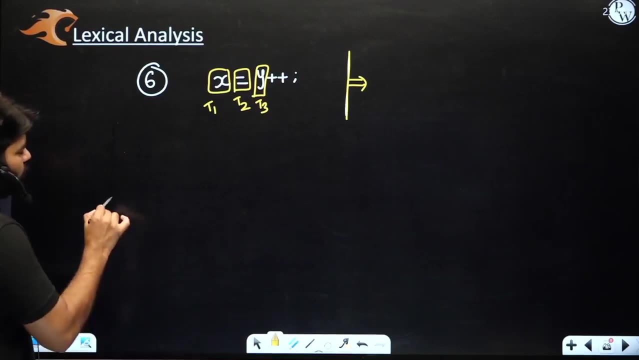 the first one, x token. one equal operator, y is identifier. now, double plus: is one token or two tokens? i told you the longest prefix rule. right, it starts from here. it will take first plus it's token. but you can't decide now because you need to scan further: longest and double plus. 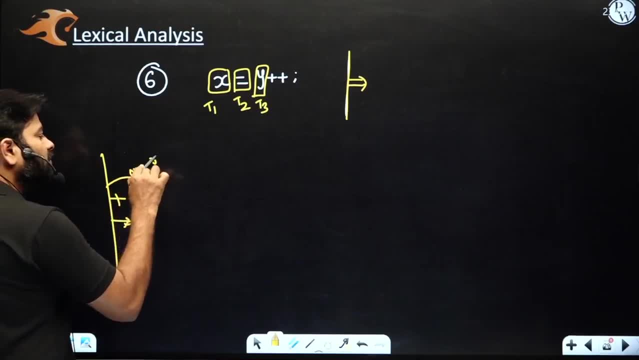 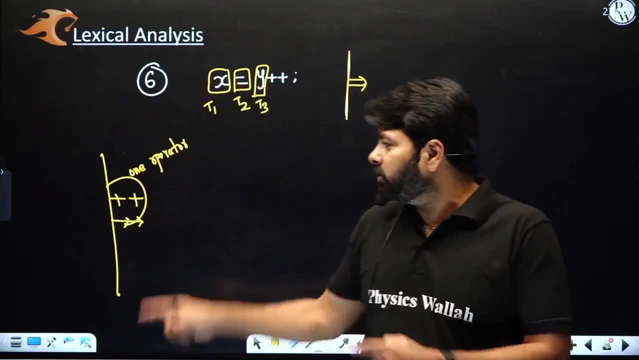 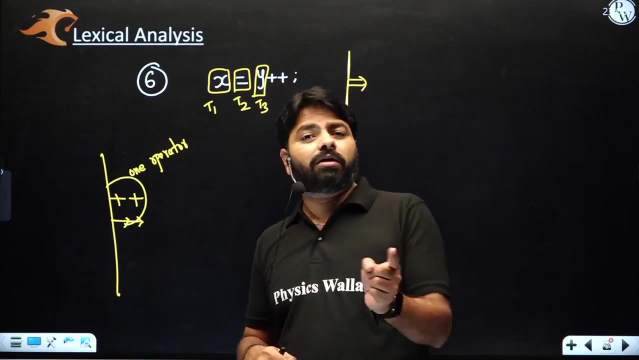 is also one operator, yes or no. even it may be. it may be two character, double character operator, but it is single operator, right? you can't assume it is two operators. it is a one increment operator. it's when you look at here. it's a post increment operator, not operators. okay, so one operator. so. 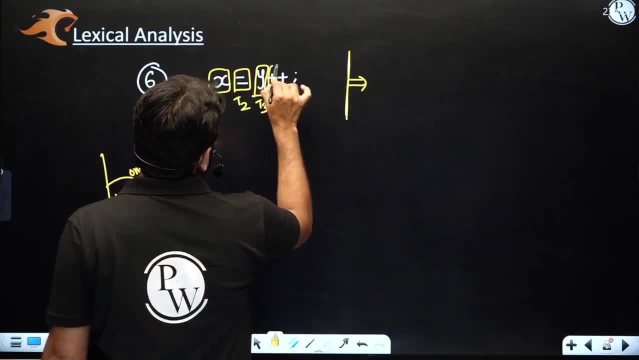 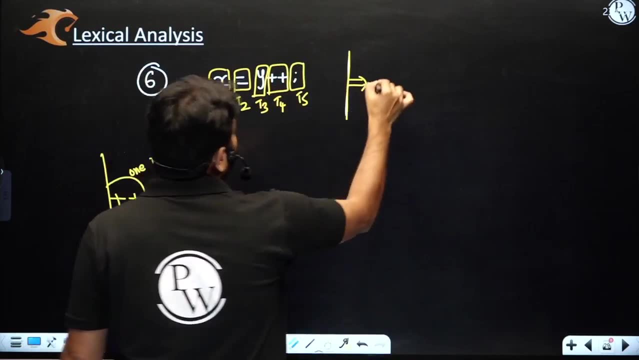 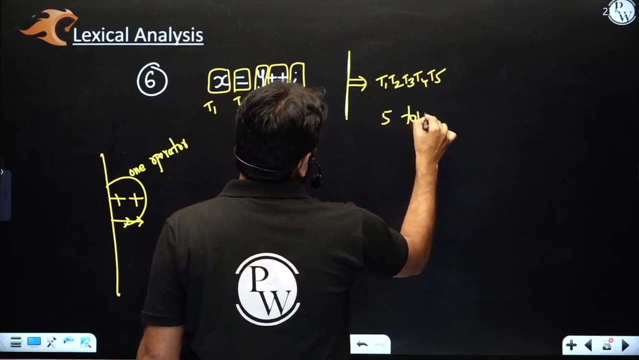 it's a one token here, so this one is considered as one token, which is t4, and increment operator that two. it's a one token total. you will be seeing five tokens in a sequence, the total five tokens, right? you should know how to do that. longest prefix match longest. 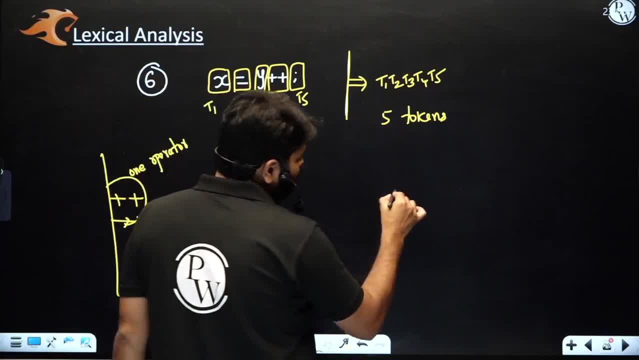 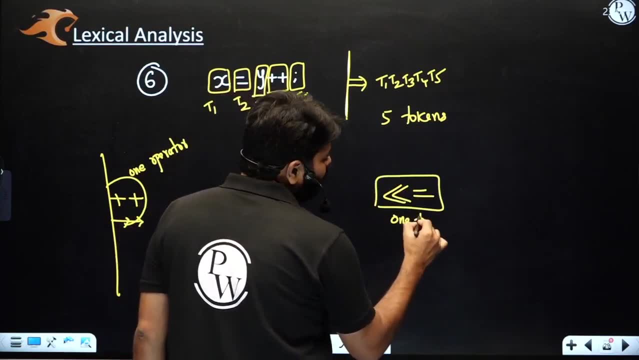 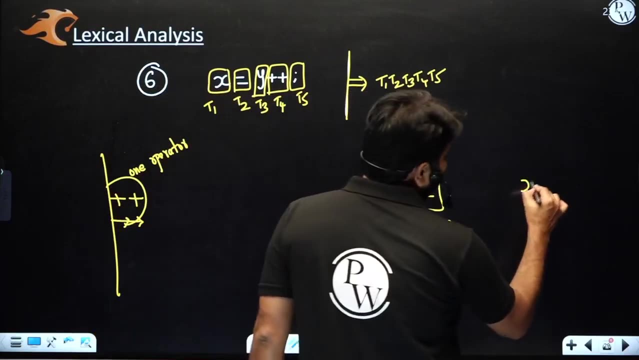 prefix match. i'll give some instances like left shift. after that you see: equal, it's just one token. it's just one token why? because when you see the assignment along with other additional operators, this is going to perform something like that: right x, left shift, equal to y is nothing, but x is equal. 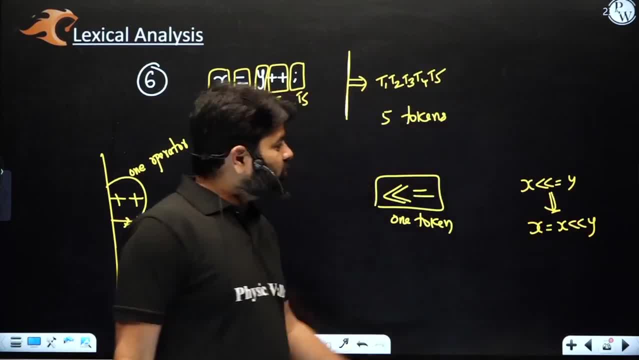 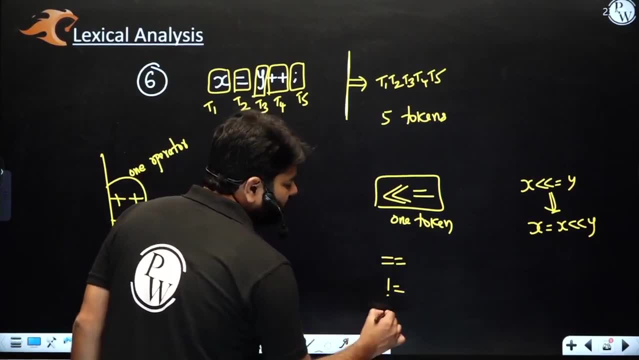 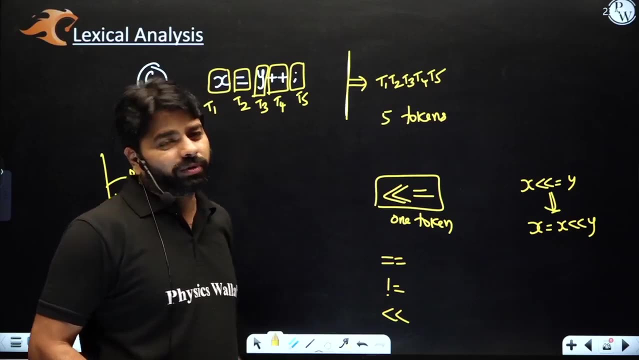 x, left shift, y, the meaning of this line, right. so this is going to be considered as one token, not only this, when you see double equal, or when you see not equal, or when you see left shift, left shift. after that equal is there again. this group, three characters is the single token, right, it's a single operator. also, what else you have like. 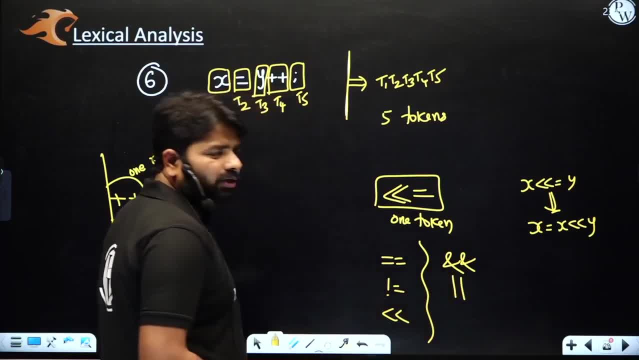 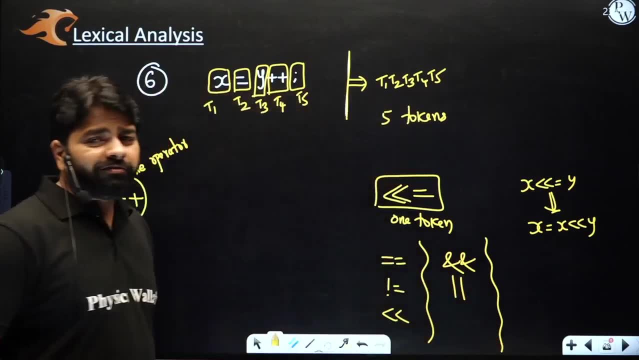 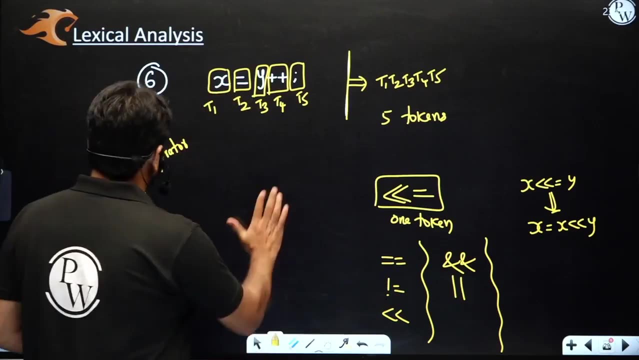 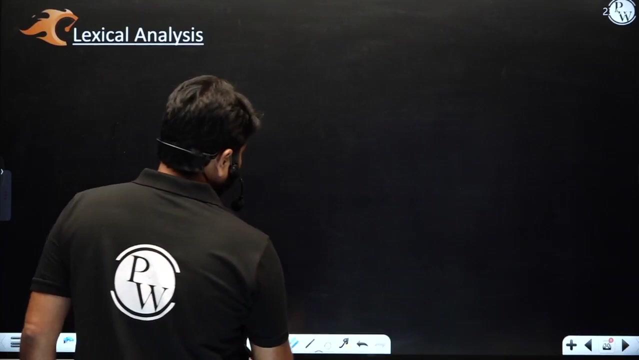 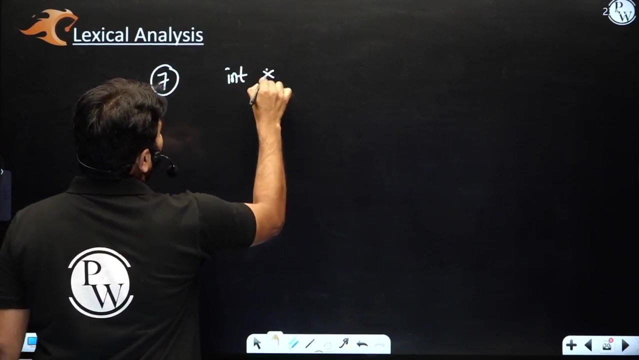 logical and logical r looks like there are two characters. but don't assume two tokens, it's, they are single tokens. okay, what else? if you have seen uh many things and you may do some mistakes here, uh, let me introduce that to seventh example int. very interesting example: star, star. let's start triple. you know, pointer, we say that 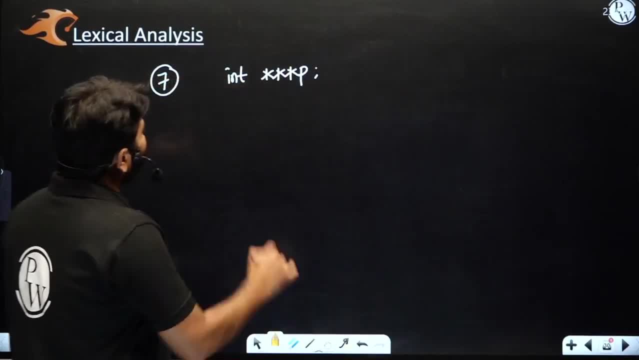 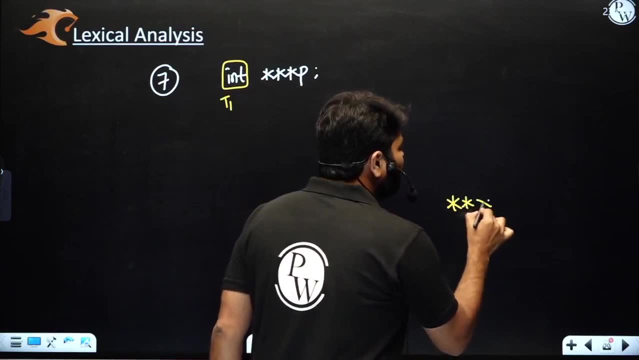 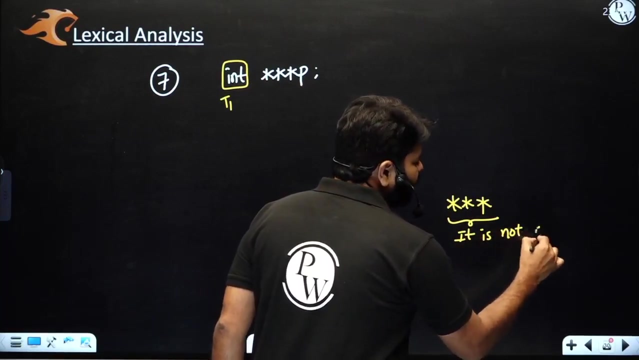 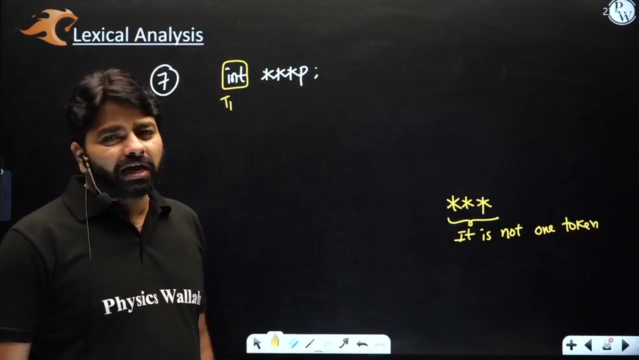 how you do. the iter int is one token, fine, that star, star, star. people might assume it is the one token. wrong, it's not one token. it is not one token. why you might be saying triple pointer doesn't mean that it is a single operator, the triple star. if 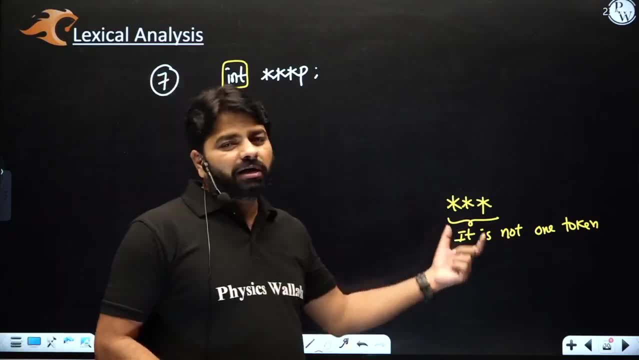 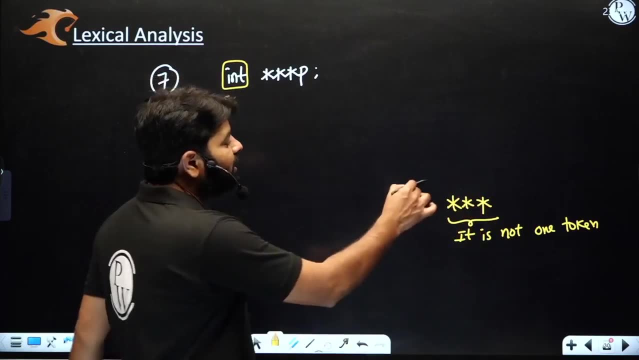 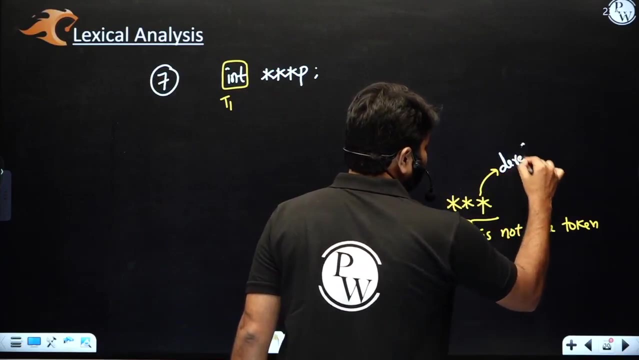 you look at your operator presence table, when triple star comes, it follows right to left, right to left and the four star is going to be having highest presidents. this star is one operator, another is using a three times. when you have this triple star p, what happens? it's going to be. 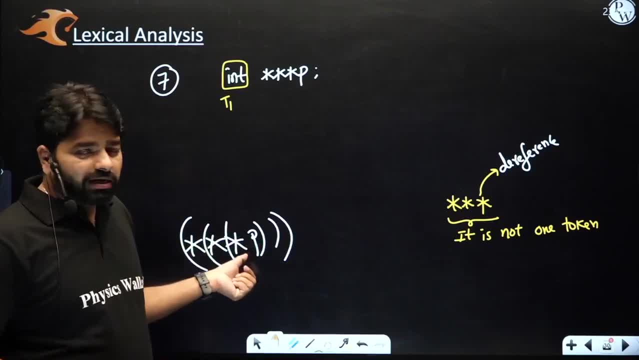 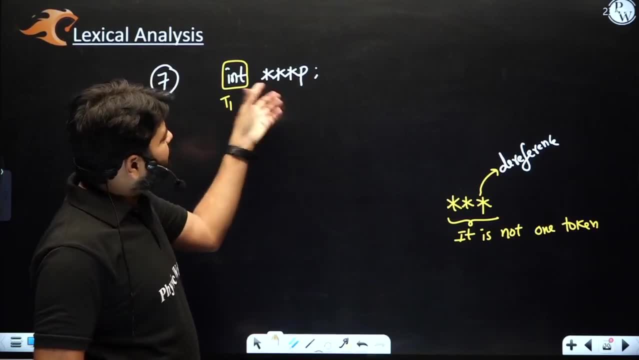 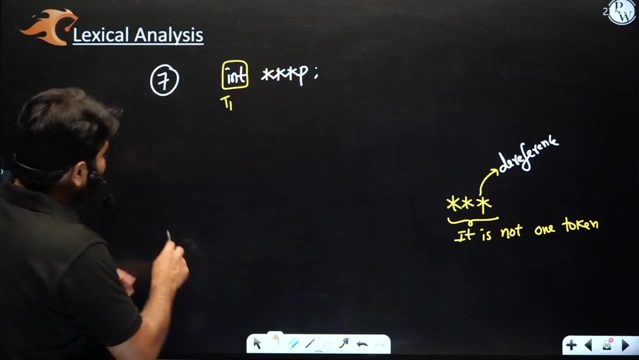 d reference operator and that is used three times. when you have this triple star p, what happens? it's going to be assigned like that, it's going to understand this way, a thing or some particular layout, but what is it? it's actually when you write something, this: 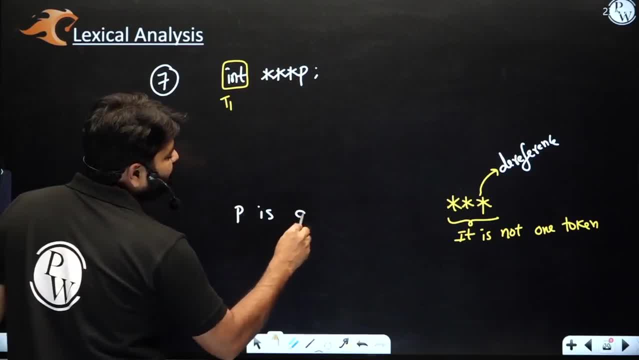 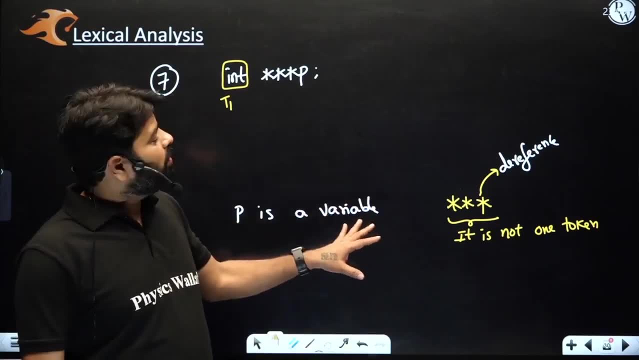 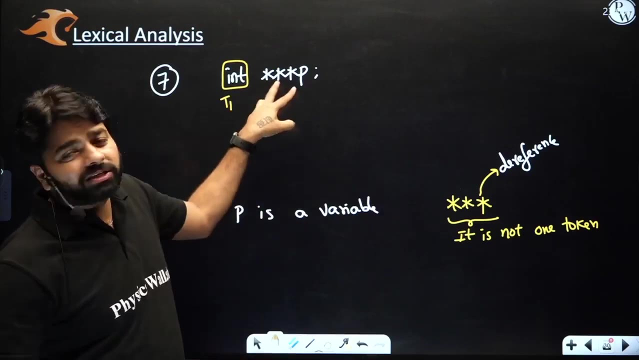 the p is a variable. what is it? p is a variable. which variable, pointer, variable? p is a variable, and that's going to point integer, that's going to pointer, to pointer, to integer, pointer. the three pointers are there here. so p is actually a variable. the other three stars are going to tell. 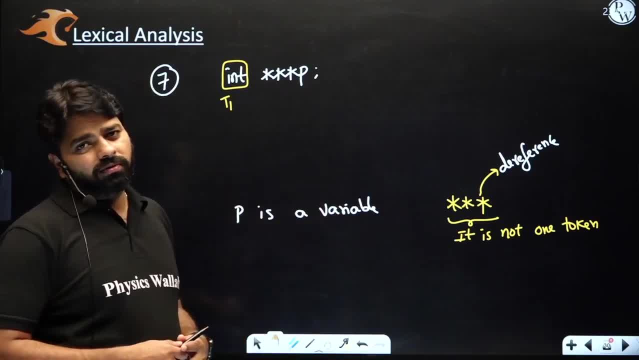 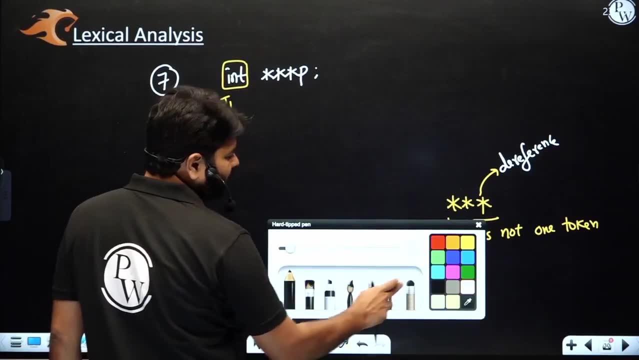 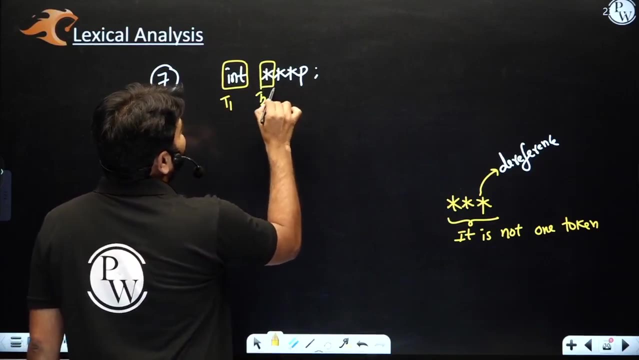 that how many levels you need to reference a d reference. you can say so now here. what happens? that's what i said: the we do some mistakes. one of the mistake might happen here. actually, it should be like t2, this one is t3 and this one is t4. 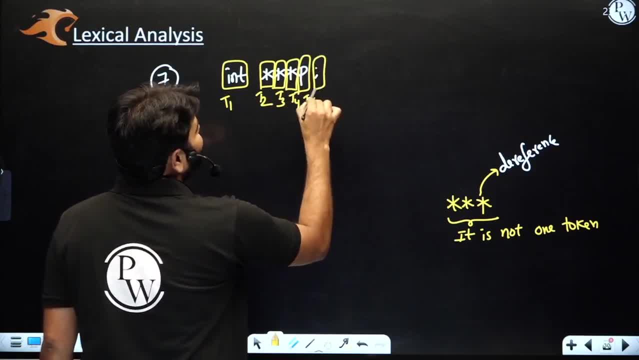 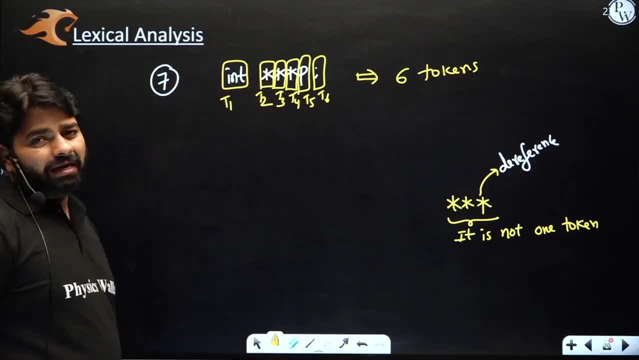 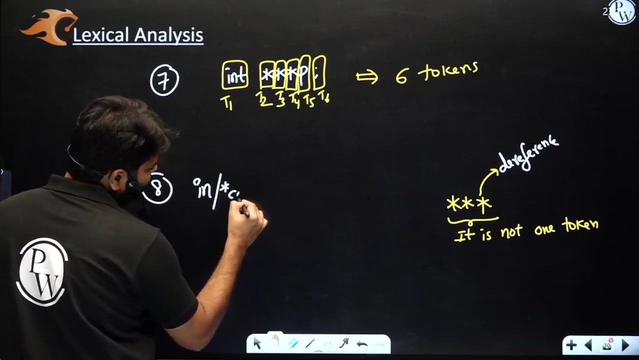 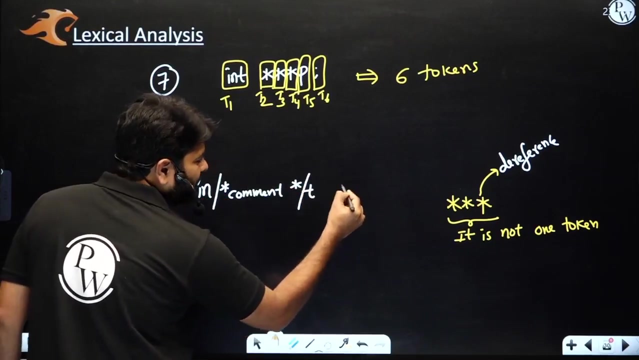 and this one is t5 and t6. so total you have here six token and no lexical error. no lexical error. and next, example 81, the sometimes we may write in and keep some comment here. very famous example, star slash. and you write without any space here t and x, after in you write a comment. it will work. 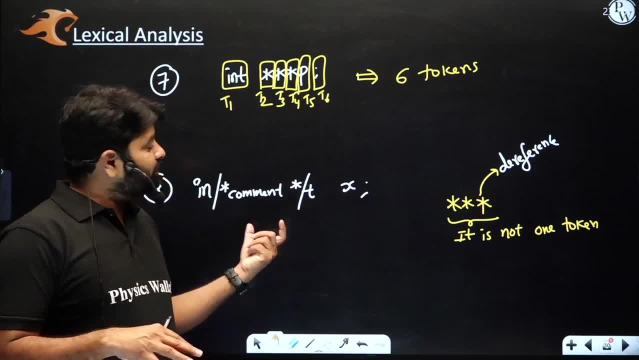 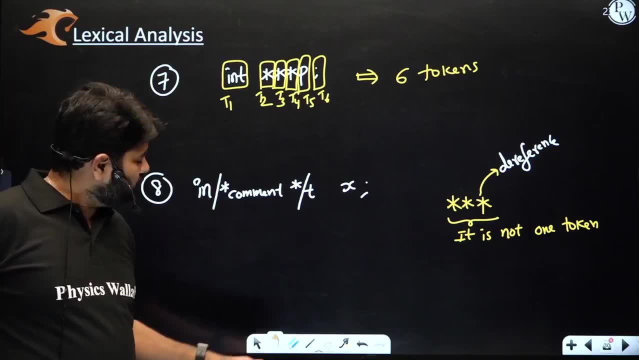 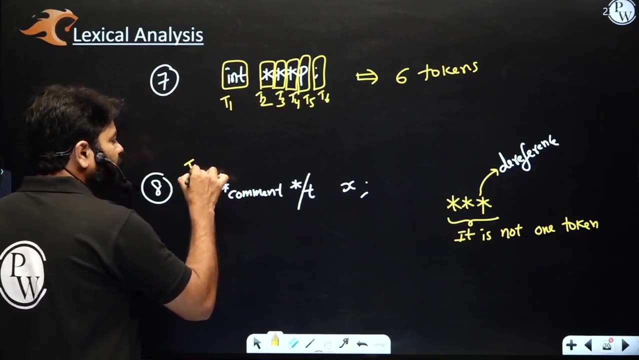 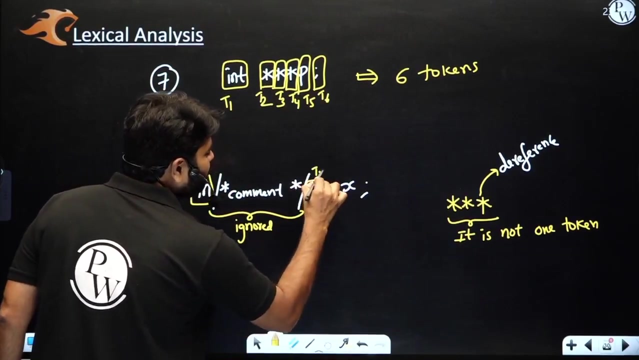 what you, however, you know you may predict as per your understanding, it works properly. but here your prediction may go wrong, why you might be assuming int is a one token. no, int is not going to be a one token here. this in is actually one token and this is ignored by lexical analyzer. and t is another token. it is. 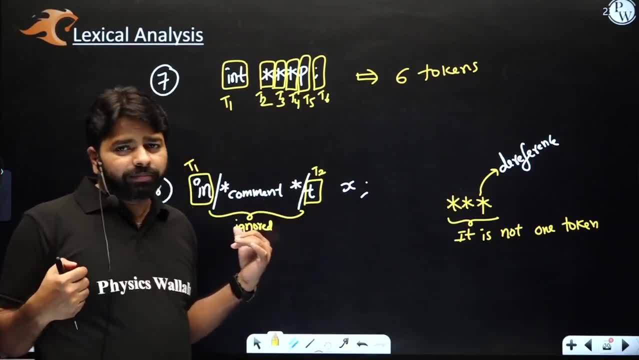 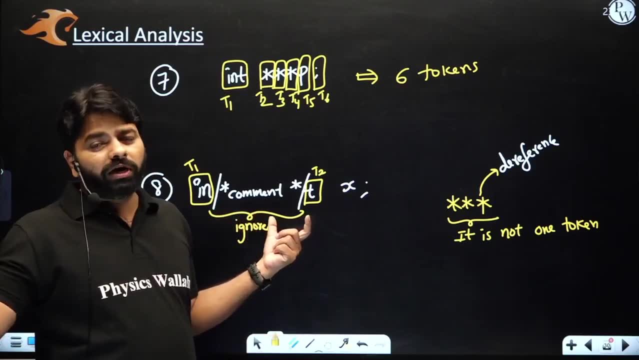 not going to have a much memory to remember all these three. whenever something is recognized, you got something to detect. now i want to start another rule. then previous one is separated. it can't remember this one, so it will throw is the token and will start identifying the comment. 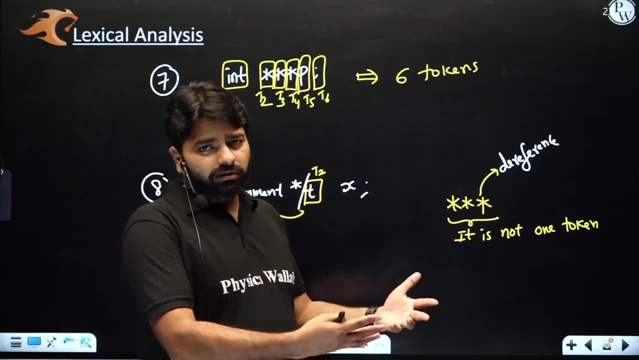 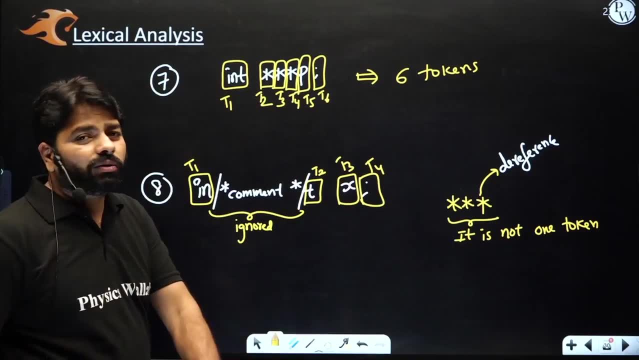 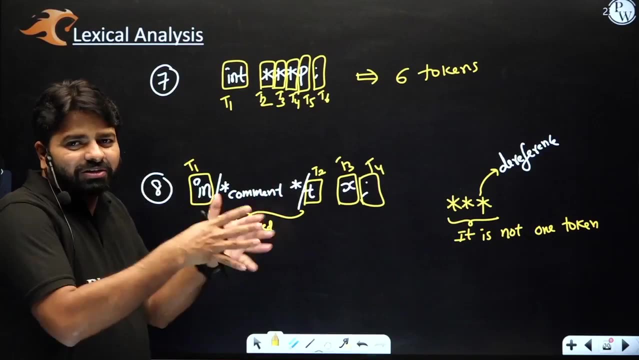 once it is over, then it will ignore. it will start another token. once it is over, it will start another token like this: so do not assume that you can include the comment anywhere, but not like this within the in between the you know keyword. so don't do that. it's going to separate the keyword. 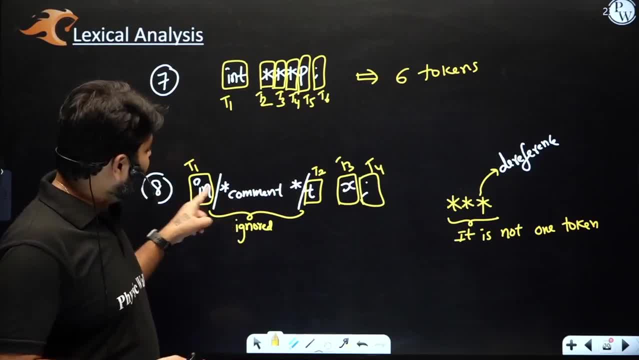 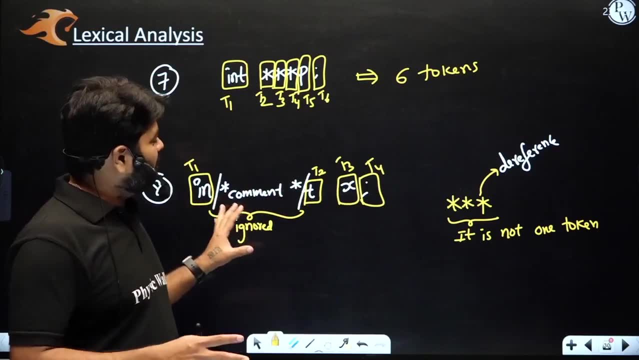 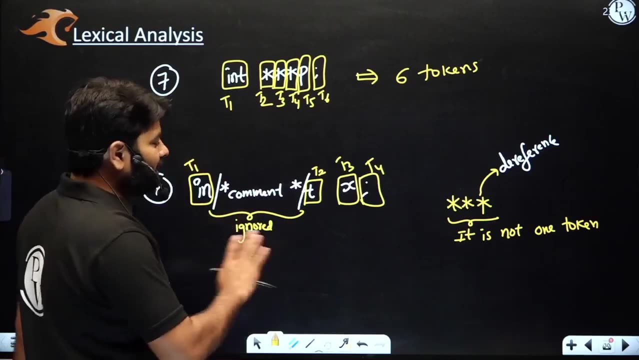 now this two will act as two different identifiers: id 1, id 2, id 3- semicolon. of course, even it may be the syntax, it is the syntax error. it might be the syntax error, but it might be, and, but not the lexical error. fine, it's not a lexical error, that's sure, but check whether it is syntax error. 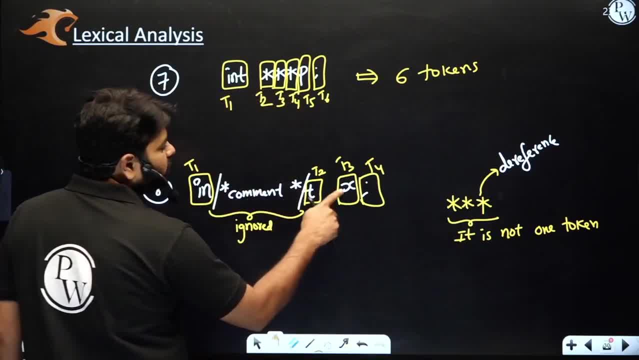 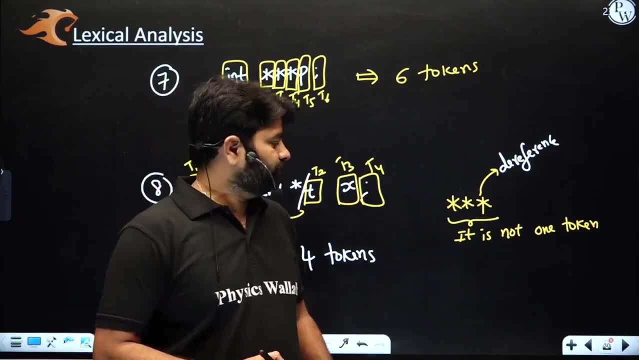 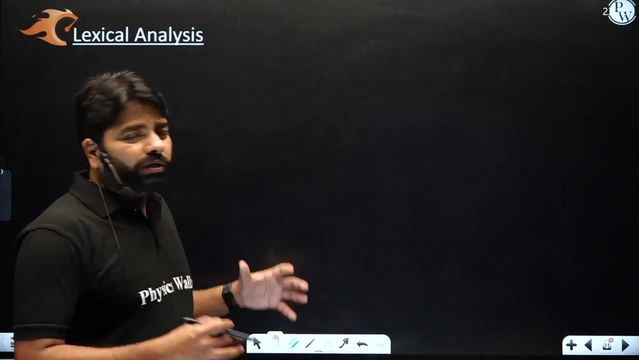 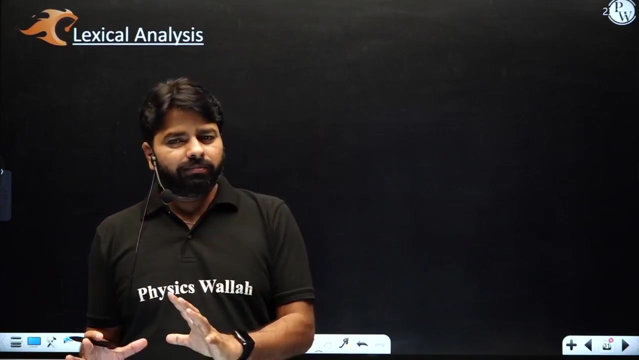 or not. how many tokens? one, two, three, four. so four tokens will be produced. okay, now what we have understood, how to recognize the tokens in the. while recognizing tokens, do not forget comments may come, spaces may come. ignore them, but it's the job of lexical analysis to 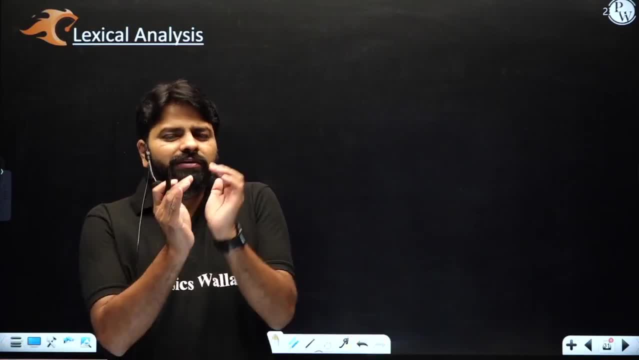 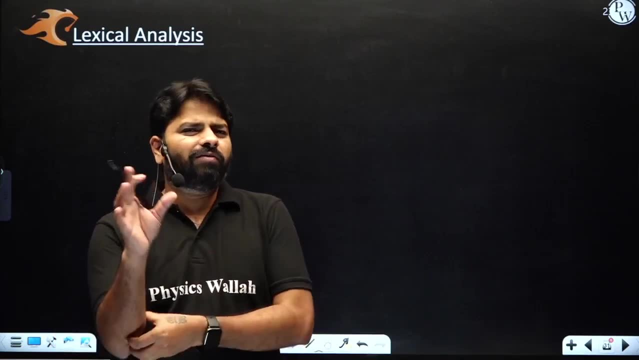 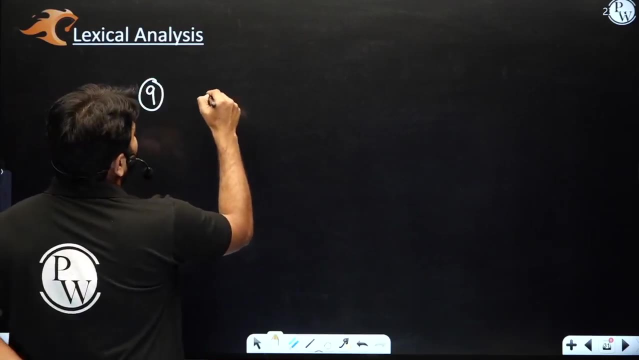 identify. and whenever you see lexical error, like something which is started with digit but after that you see some alphabet letters, then it will produce an error. okay, this is one kind of lexical error. what is another kind of lexical error? in case, if you want to see another kind of lexical error, somehow you did like this, you know. 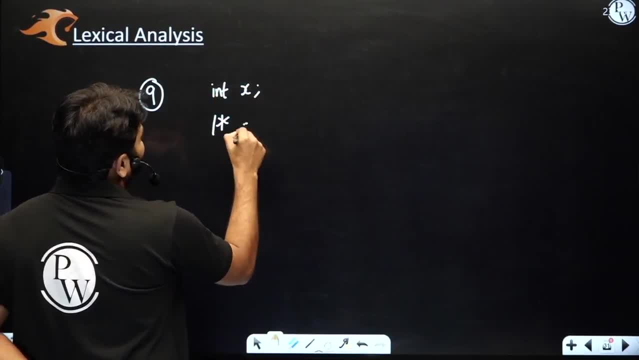 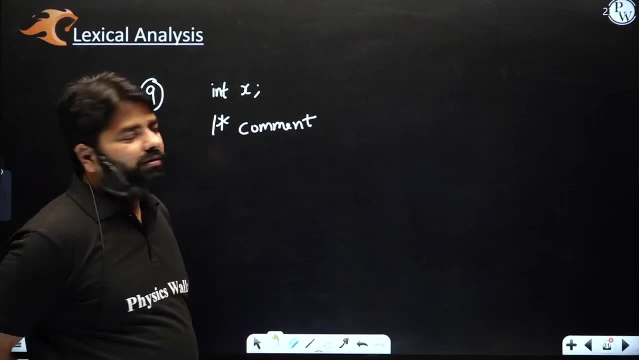 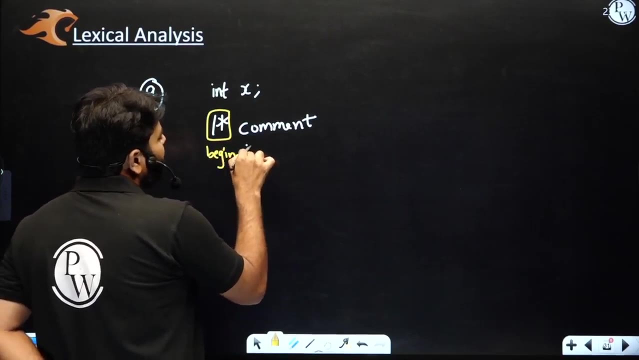 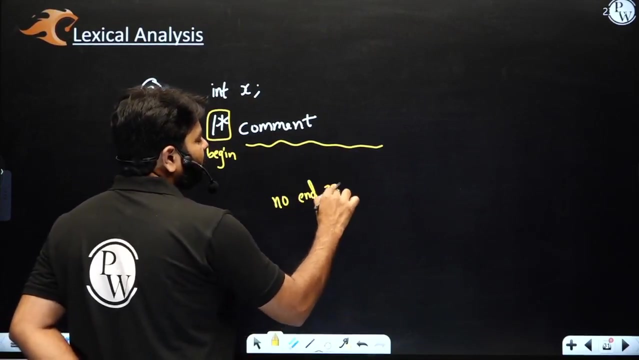 int x. you started the comment. it started but you did not end anywhere. then what happened? the lexical analyzer is trying to look for the end rule. it's begin right now it's trying to look for the end. where is that end not happened? so no end pattern for the comment. no end. right, that end is not happened. no end of comment. 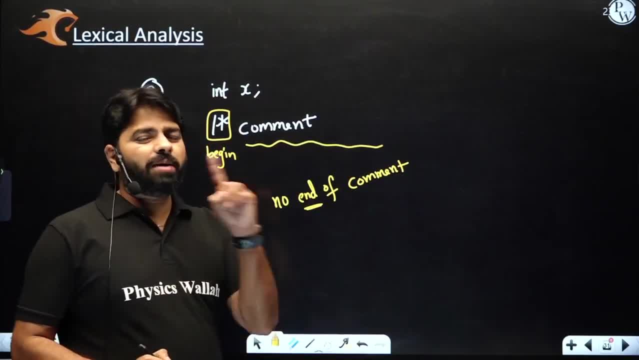 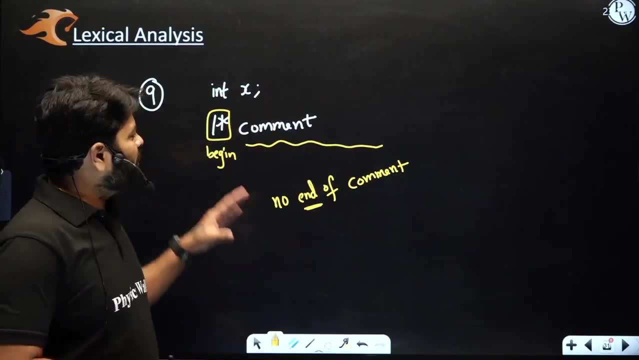 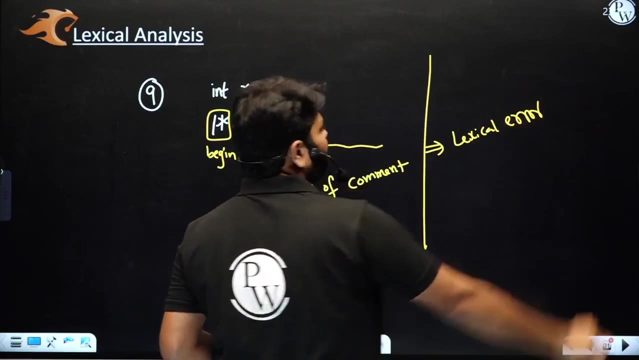 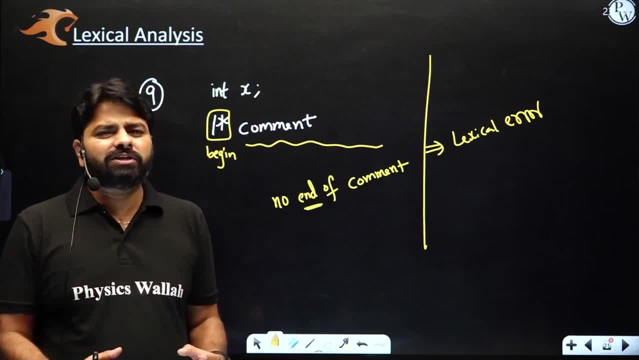 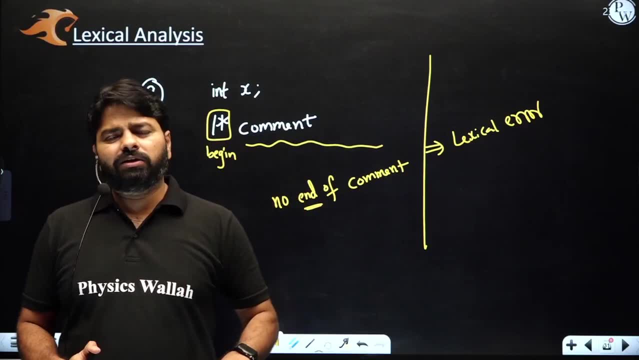 but for the exam point of view you have very, very easy questions. hardly you see five questions in throughout 30 years of the gate. you see just five questions from the lexical analysis. so you just learn the concepts and have the basics. like finite parameter is used in this, our regular expression. 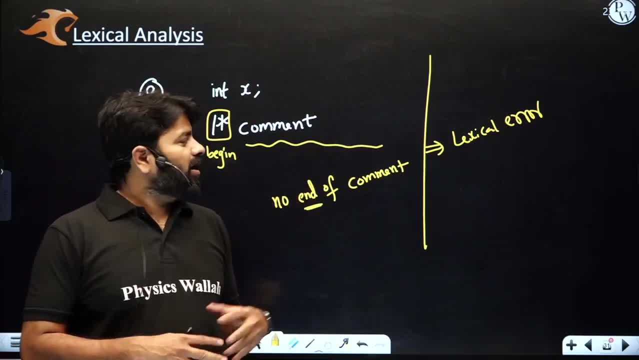 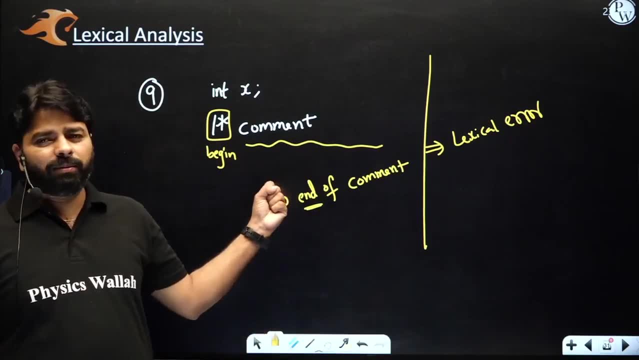 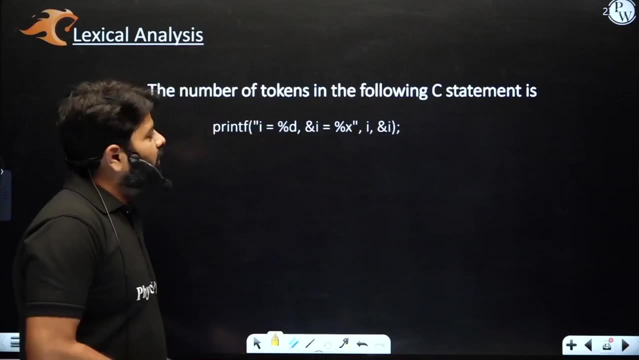 is used to design the finite parameter and how to recognize the tokens. what are the lexical errors, what type of tokens you have that would be sufficient, and what is the symbol table, what it stores? fine, you want to practice some of the gate previews. you have very simple questions, but do not. 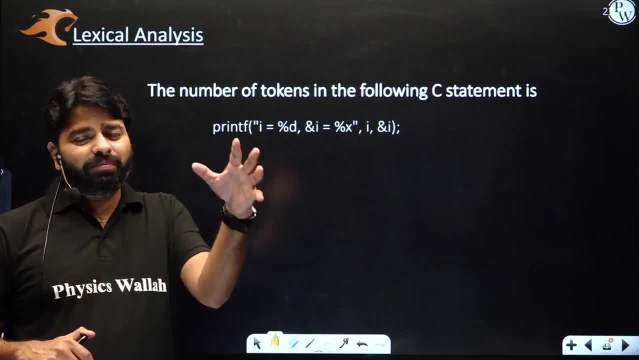 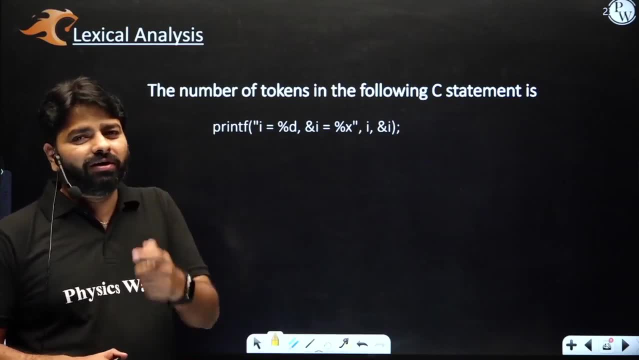 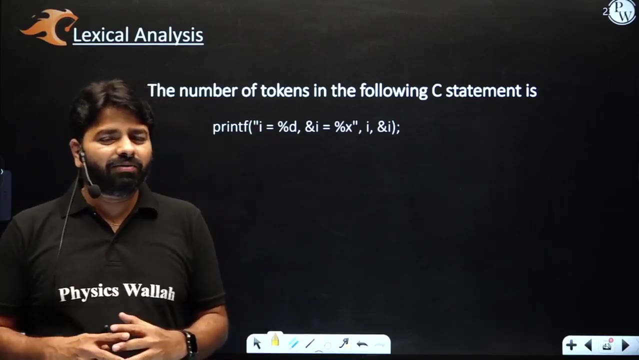 practice the fortran or you know some other programs you know before few years, before, i think, 15 years. you have other programming language in the gate exam like fortran. so they were, uh, they were asked one question: uh, find out number of tokens in fortran statement? we don't need that, okay, don't. 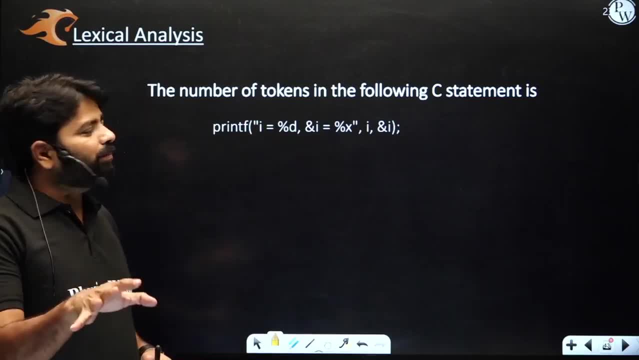 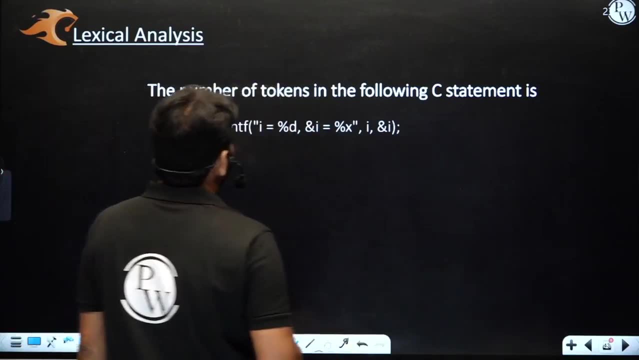 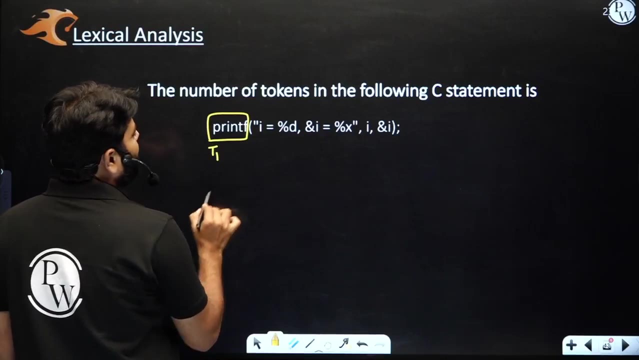 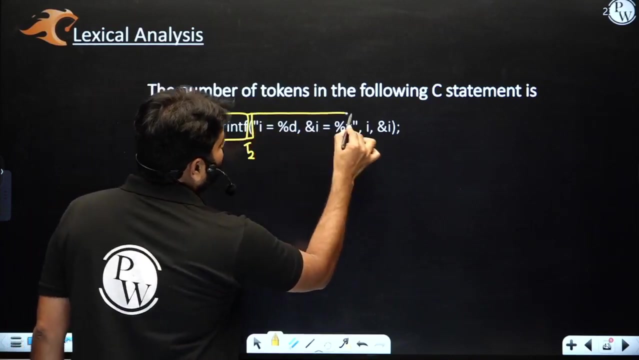 practice now it's to find the number of tokens in the following c statements, because, as we have today, the c in the syllabus, now how do you find a very simple printf is one token, okay, so t1, and then we have the open parenthesis t2, and then you have this all. 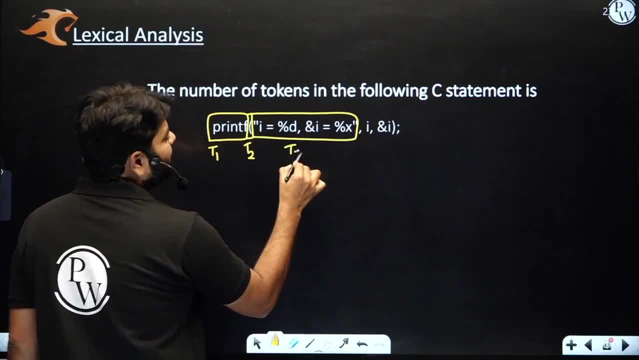 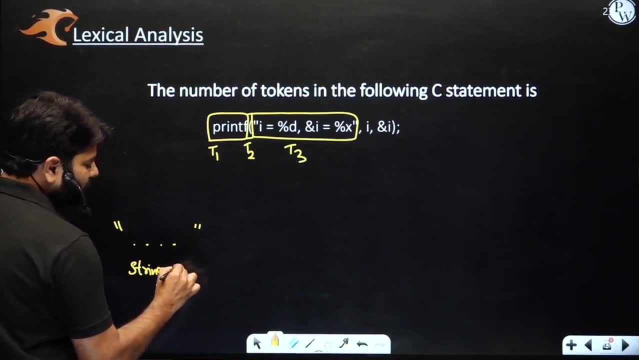 so ilose不同 ant responso. but if you think about it now, there are several ways: from y- usually open parenthesis- to ordnance p, sugar, great, exactly. so this is its הצ. Proper thing is considered as the one because it's considered as the spring. anything you mention in the double code is called as just bring. 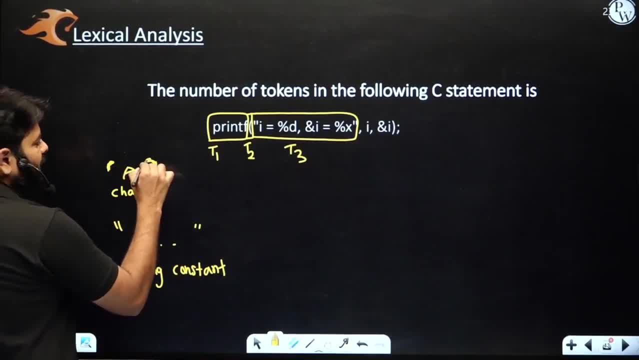 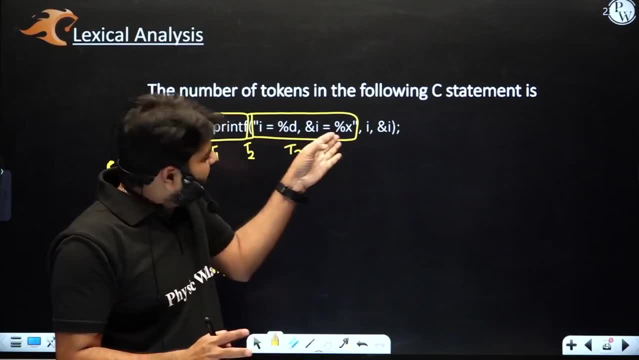 constant, one token only. okay, remember this, and not only this. if you cover in single- uh no, like this, it's just called as a character constant. if you specify anything in single code, the single code all together, even you have a lot of things inside, but just consider as one token and then comma. you. 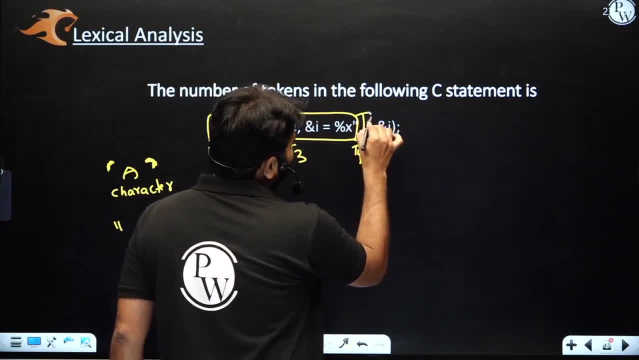 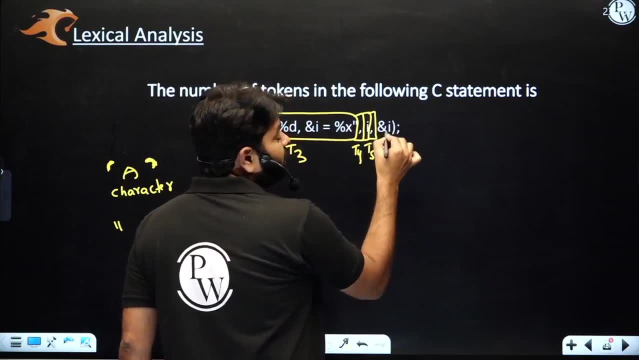 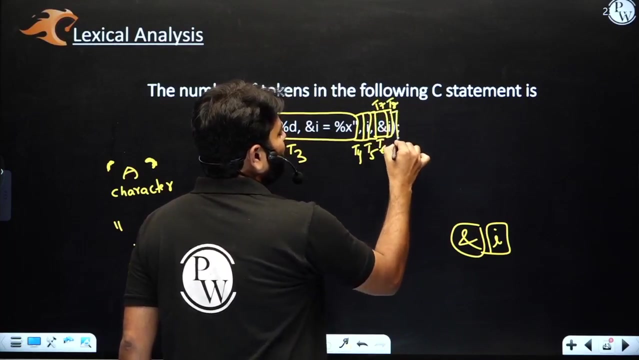 have here. so it's t4 and you have i it's t5 and then comma it's a t6 and here ampersand i. ampersand is an operator, i is identifier, so both are two different tokens here. okay, i'll just keep here t7 and then i it's th, then closed parenthesis t9 and semicolon t10 and come here: you don't have. 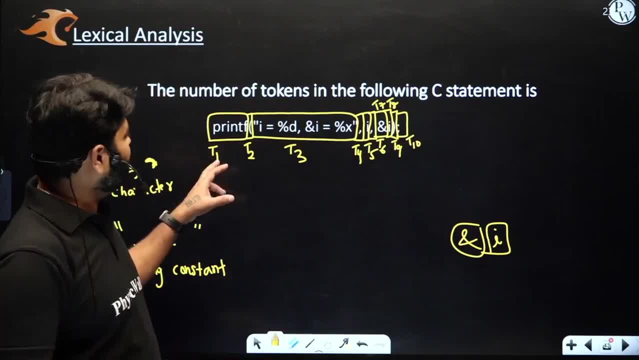 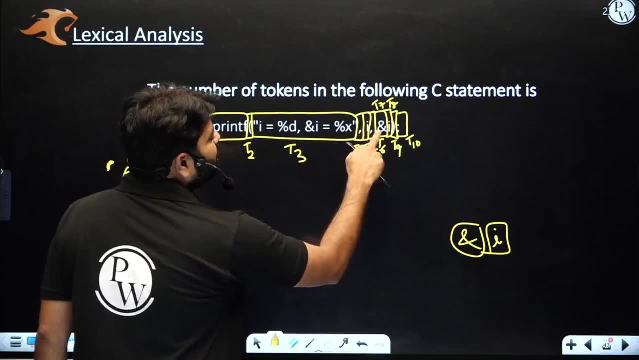 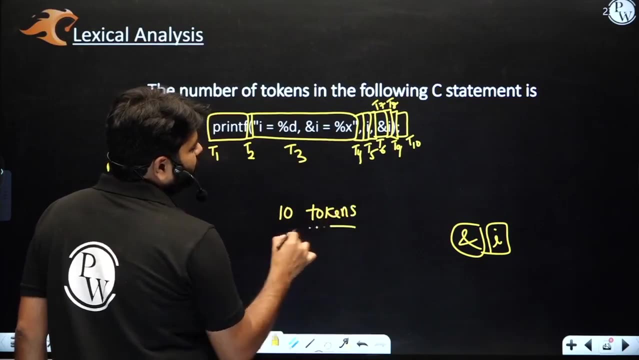 anything right. total how many tokens you have. just scratch it if i count. anything is wrong: one, two, three, four, five, six, seven, eight, nine, ten. the total you have ten tokens. in case, if you have any syntax mistake in this line, just ignore it, because we are not looking. 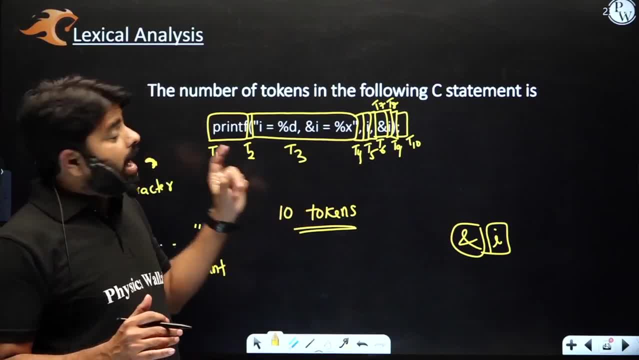 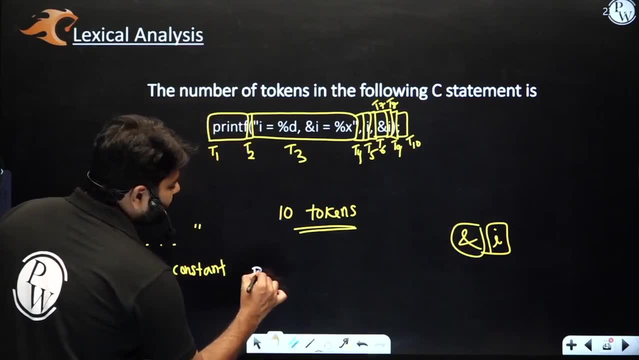 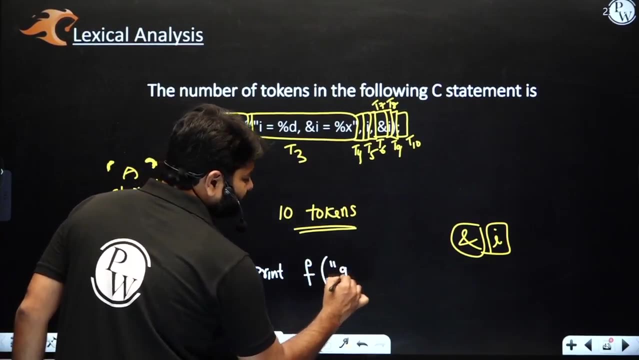 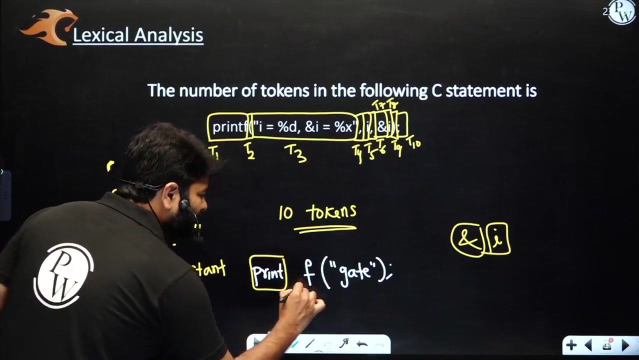 for the syntax. we are only trying to group the tokens in case in future they will gently ask a question. i'll just mention that too, after print, in case you see the space. then you have something like this: right then, what do you do? you just consider: print is identifier and f is another. 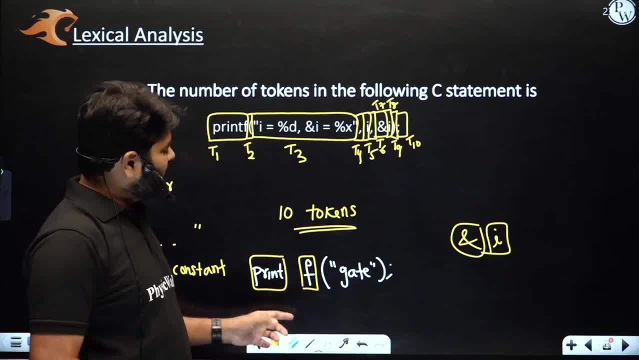 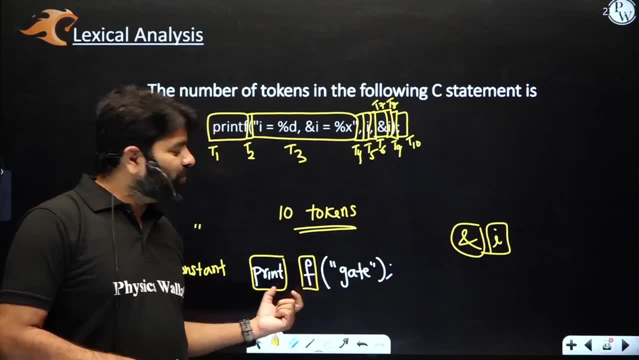 thing. you just consider print is identifier and f is another thing. you just consider print is identifier and f is another identifier. you just count here two, not one. okay, don't assume that they have done mistake in the gate question. no, they might be asking intentionally: how do you count the token? so here, printf is the. 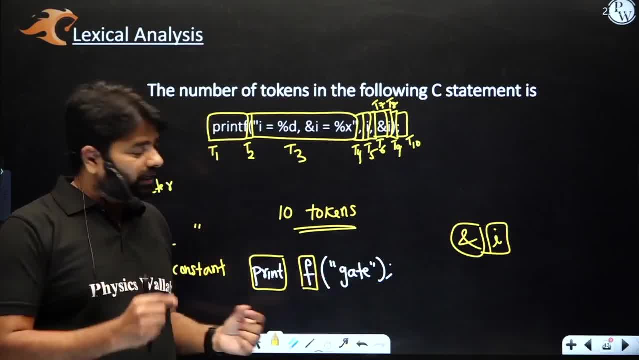 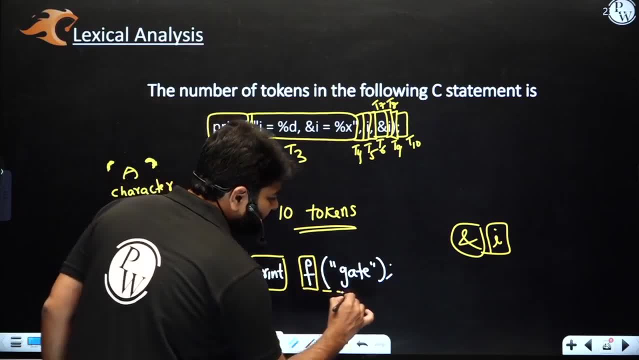 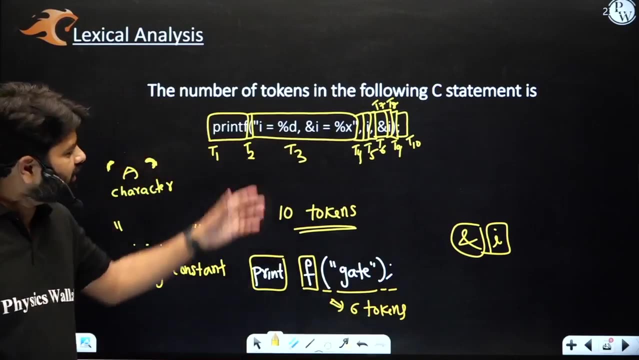 one token, but here print f two different tokens, because space will separate the tokens. okay, remember this point. one, two and you have a three, four, five, six. here you have six tokens, just variation. when you have already one question, then you should expect some other question with a little bit variation. 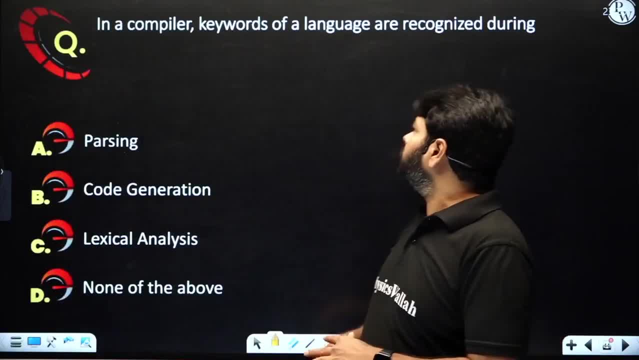 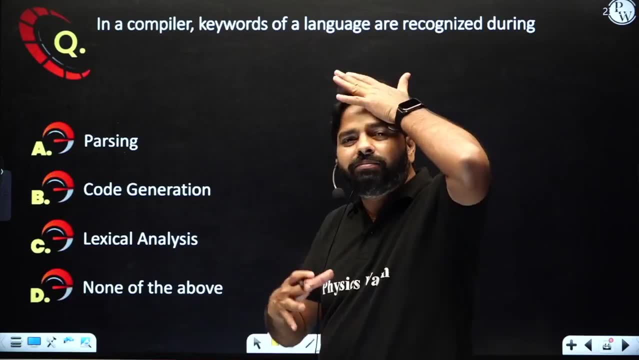 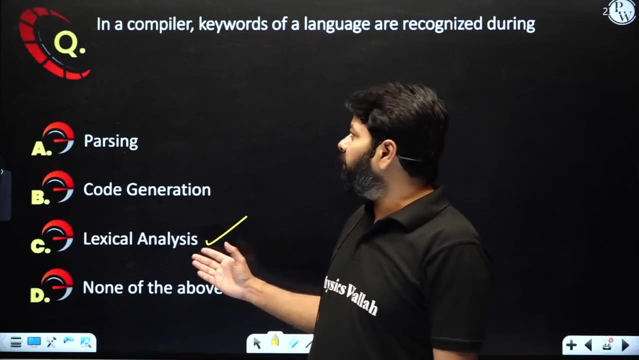 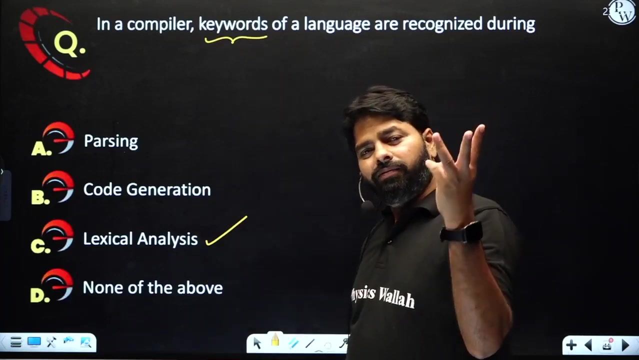 in a compiler, keywords of a language are recognized, during which phase- very simple, right in passing, you do uh generating pass tree by looking at the syntax right. but here lexical analysis is the right option. this phase only will recognize the key words of a language, not only keywords. any kind of token right like uh identifier operator. 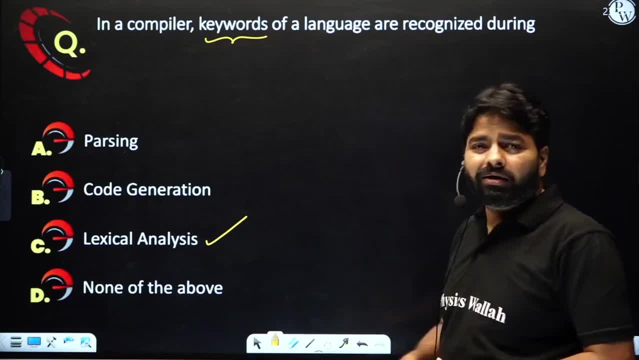 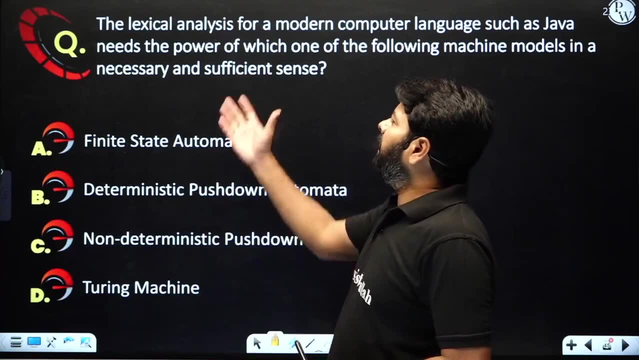 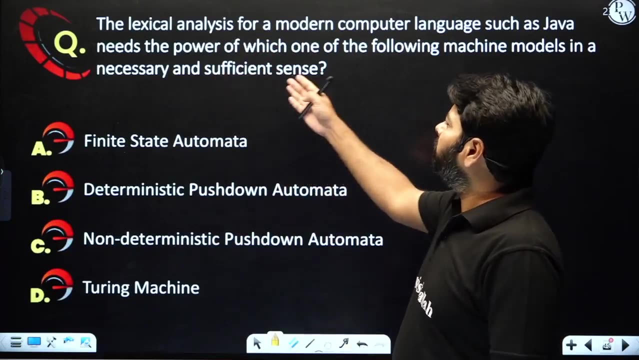 constants, punctuations, all done, uh, recognized by lexical analyzer. fine, the lex analysis for a modern computer language such as java. you know you may use c or something like that, needs the power of which one of the following machine models is: are in your necessary, and you may use c or something like that needs the power of which one of the following machine models is: are in your necessary and are in your necessary and. 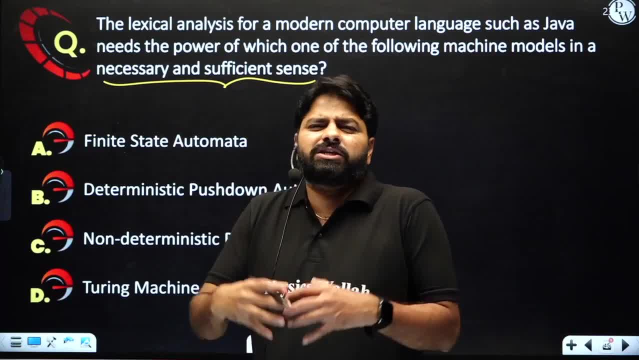 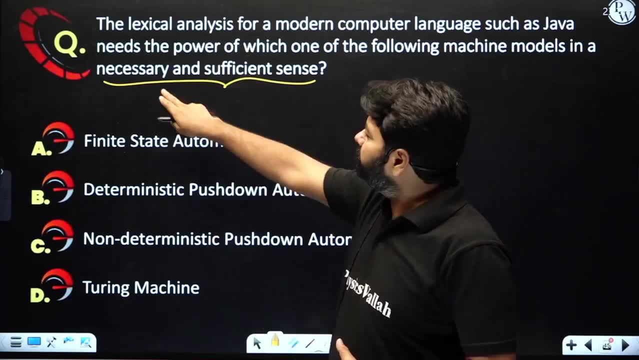 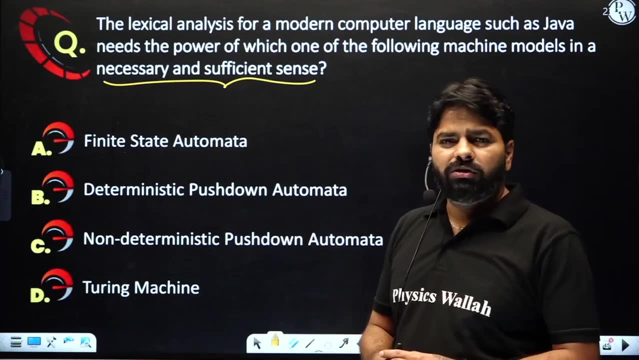 a sufficient sense. necessary and sufficient means a split form and that's enough, basically. okay, actually, if i don't have a sufficient word here, if they ask only necessary, right, you all are necessary here. if you ask me, you know, anybody can be used, but necessary and sufficient. 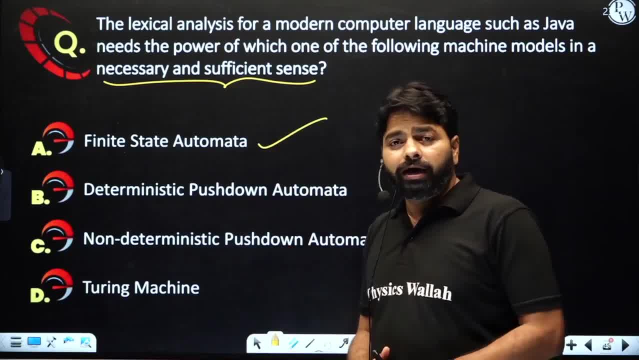 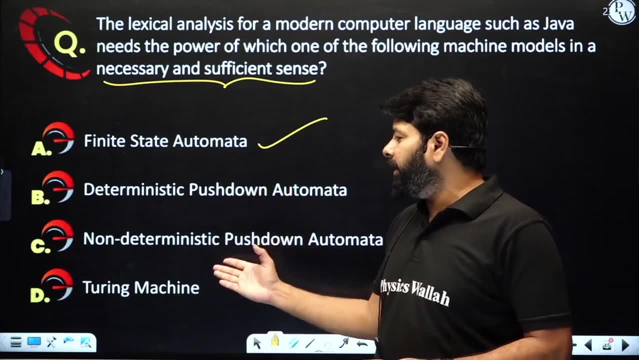 the finite state. automata here looks like all are correct, because if final data can do, then others can do because they are more powerful machines in theory of competition- deterministic vda, non-deterministic vda, turing machine- these three are powerful than finite parameter, if finite. 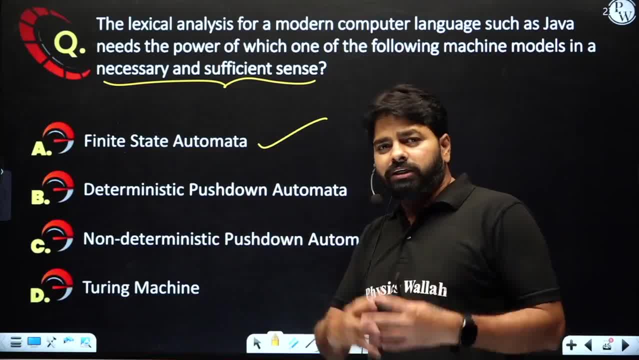 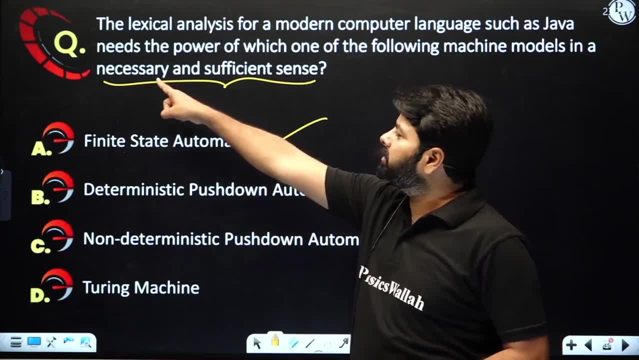 parameter can do. these three can do finite matter. able to design. you can use for designing lexical analysis. it means all that they can be used, okay, but when the word is necessary and sufficient, then this would be sufficient. you don't need these three just to implement the lexical analyzer or 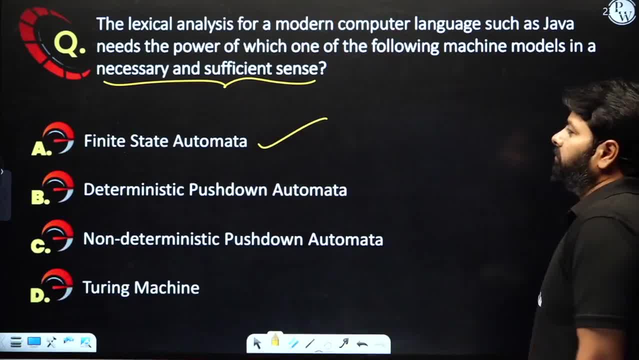 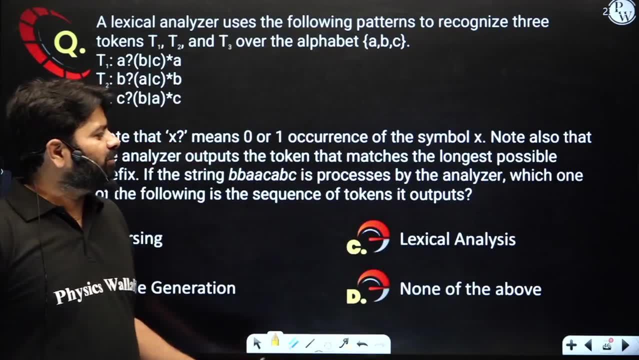 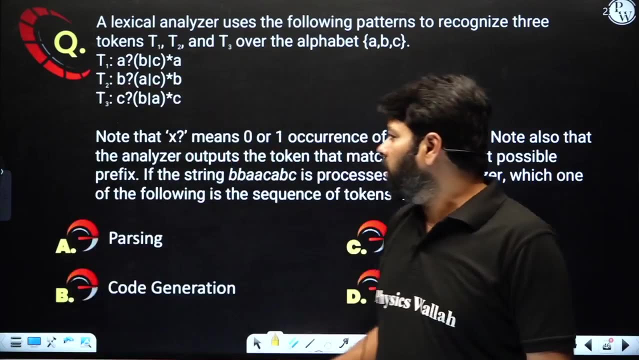 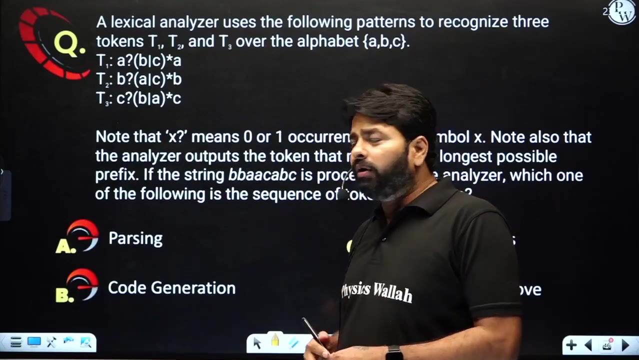 just to design lexical analyzer. so this is one of the uh interesting and time taking of question. but once you know the concept that i have already discussed, you can easily do it right. use the longest prefix rule and read each and every statement, what they have mentioned and you need to follow their definition right. what you, what you learn and 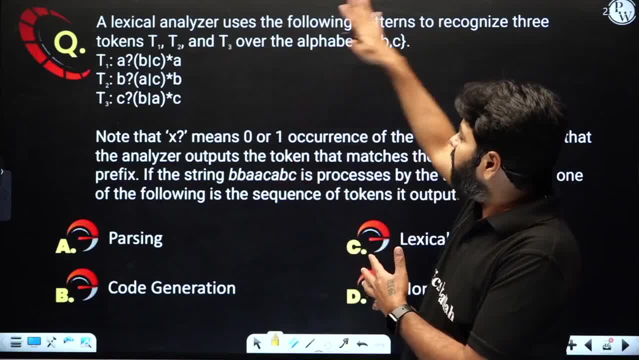 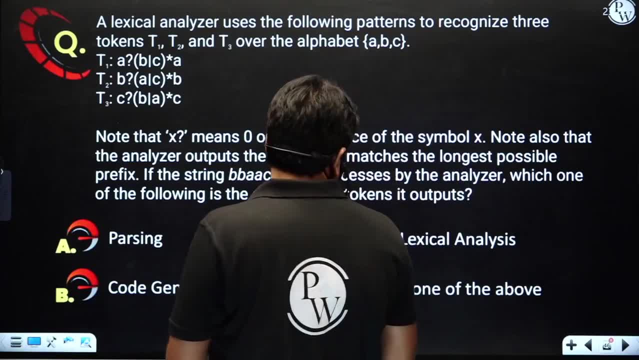 what you study might be different from this question, but this question, everything is given. it might take two to five minutes, but you should spend the time, okay, so let me start doing it. what are the options we have here? uh, um, um, um. i'm very sorry for the options, but 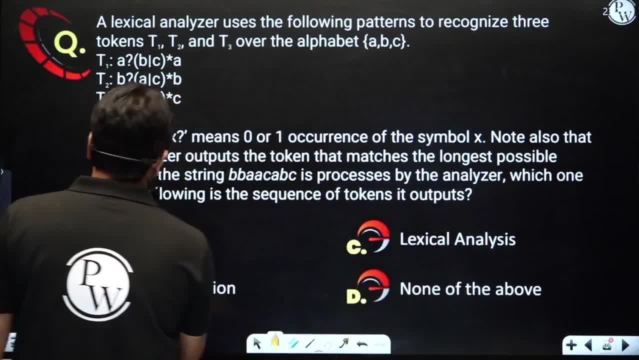 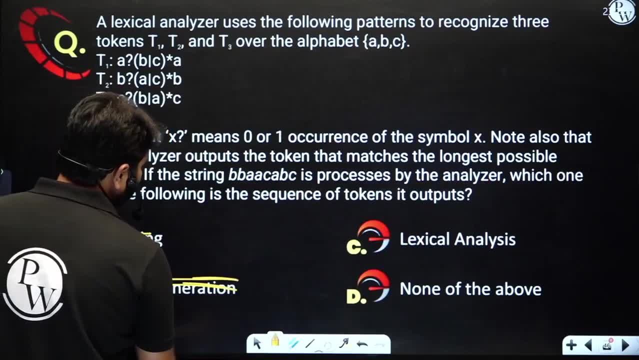 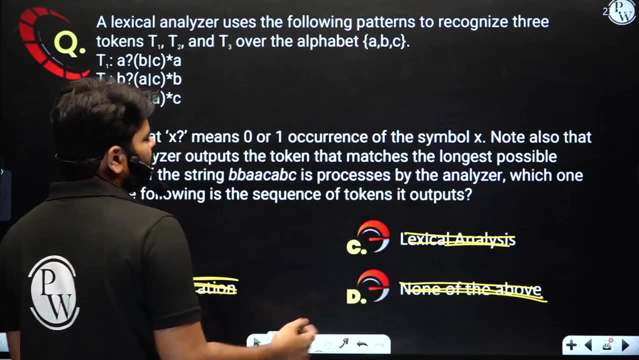 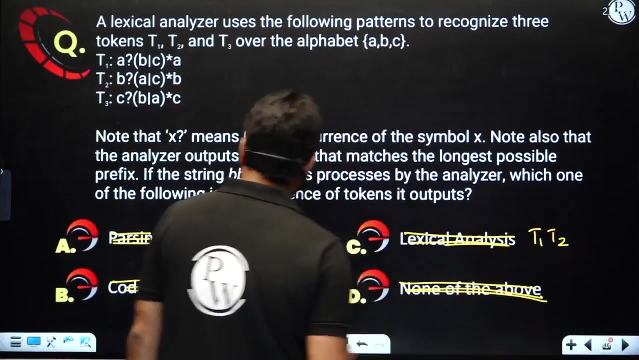 okay, the question is about uh. which one of the following is the sequence of tokens? right here you should have the sequence of tokens and we'll find the sequence of tokens here. okay, they might give some of the sequence like uh, t1, t1 or t1, t2, t1. 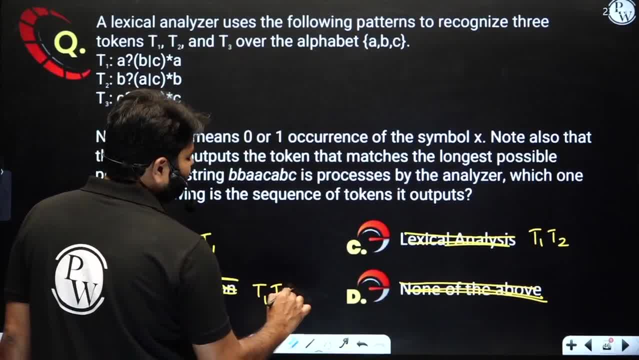 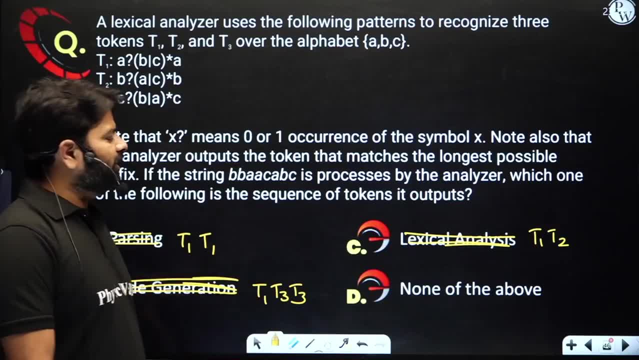 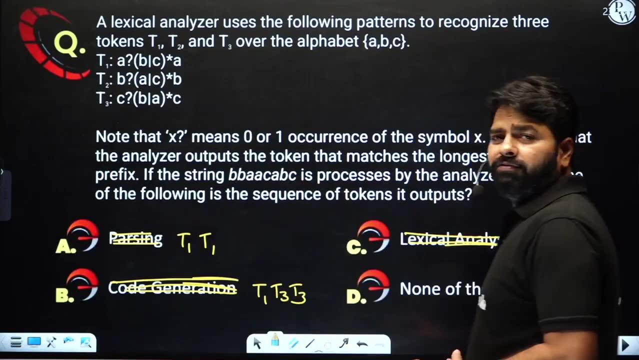 uh, something like that: three, three, three, three or none of this. it could be none of this. actually, options are different. uh, you can look at a gateway q question now. how do you, how do you, analyze this data? read the question carefully, as i told. everything is mentioned. that means you need. 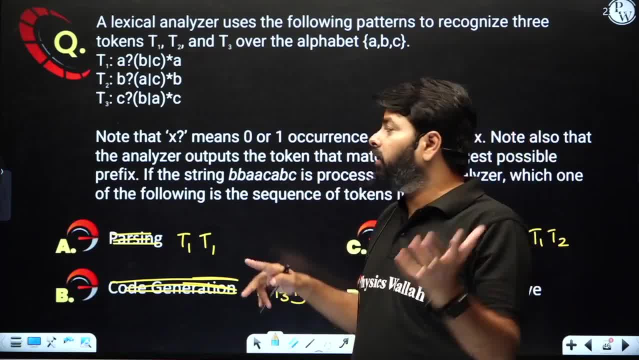 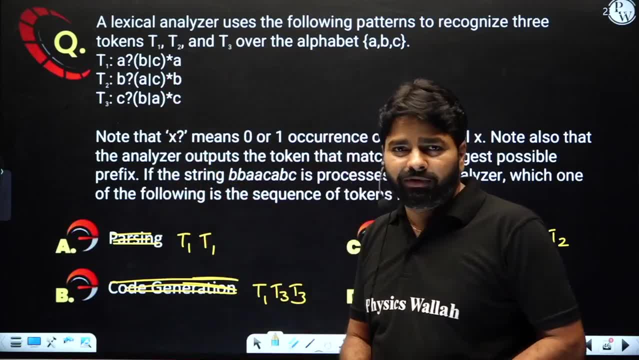 to focus on the data, not on your knowledge. your knowledge, we will apply it, but don't bring your knowledge directly without reading the data, because you did not aware that what you are doing is not question mark. what is the meaning of it? because i never read- uh, even in compiler, somewhere, except 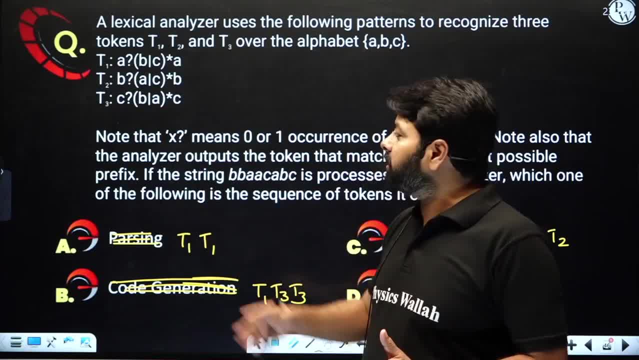 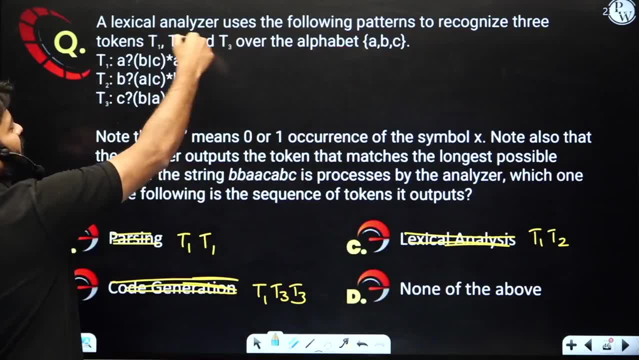 in regular expressions: right. if you want to implement lexical analyzer, you will see this code, but while preparing the gate, you don't. now, a lexical analyzer uses the following pattern to recognize the three tokens c1, t2, t3. right, so there are three tokens i used to represent. 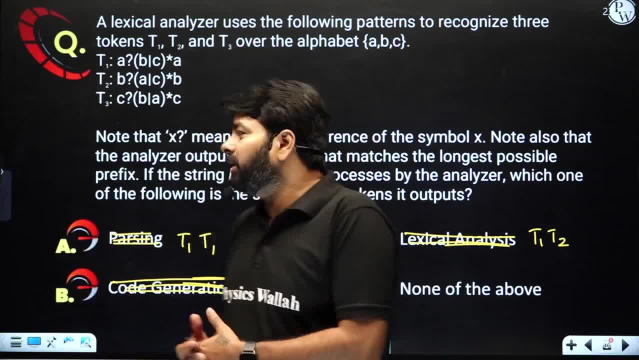 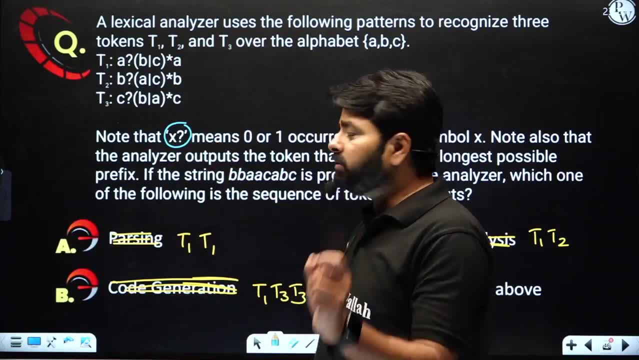 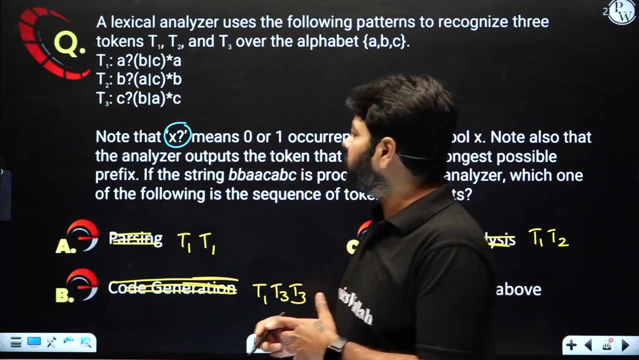 always right: t1, t2, t3, t4, because that is how we understand the code. now they have given some you know pattern, don't worry about it. they have mentioned the x followed by the question mark represent means 0 or 1.. if you study theory of computation, 0 or 1 occurrences of x means here: 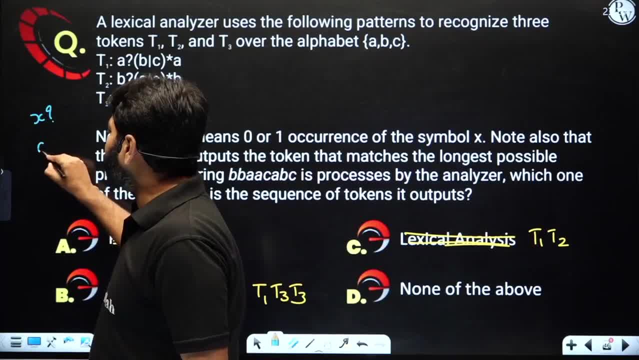 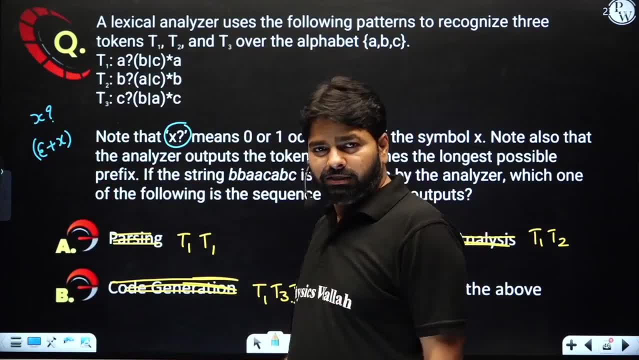 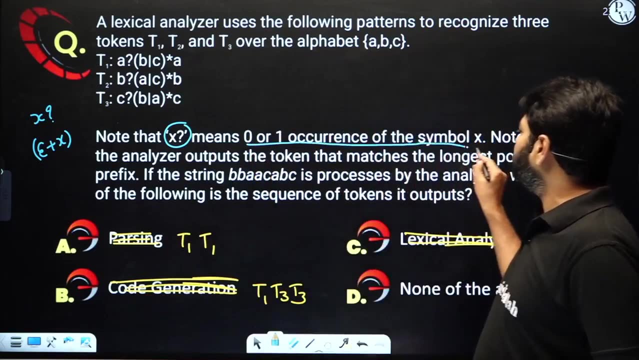 the x question mark means it's just like epsilon or x, only that's the meaning. epsilon means 0 occurrences, x means 1 occurrences. if you want two occurrences, double x, x followed by x- this clearly mentioned 0 or 1 occurrences of the symbol x- then whenever you see that this one, you can simply say: 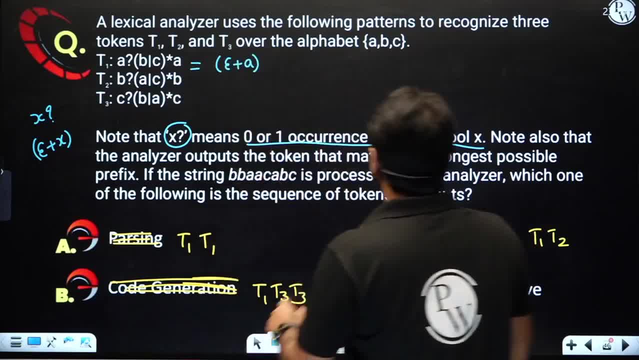 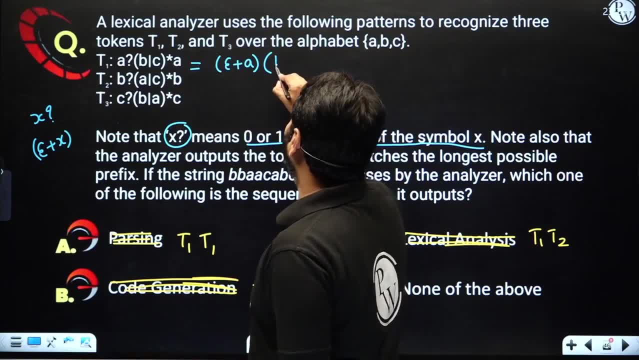 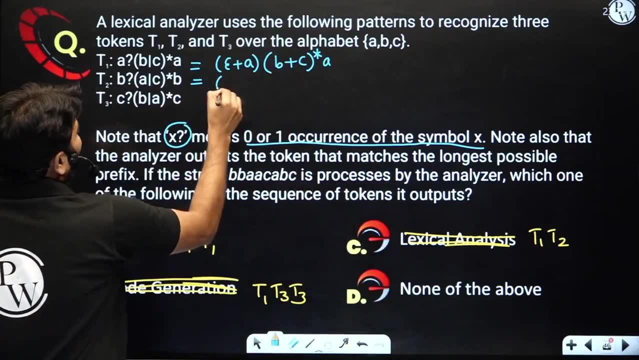 epsilon or a and r is the dimension anywhere not required because this slash represent- uh, it's a bar- represent the b plus the r, only star a. now you got to know what is that question mark represent. right, you can write everywhere: epsilon plus b a r c, whole star b and then epsilon r c. 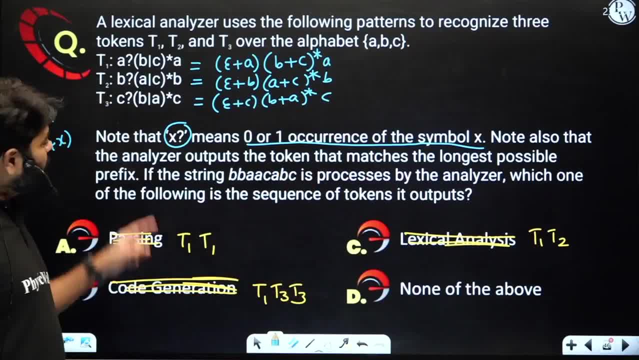 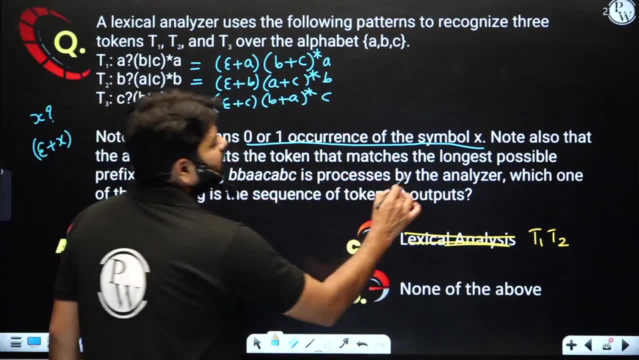 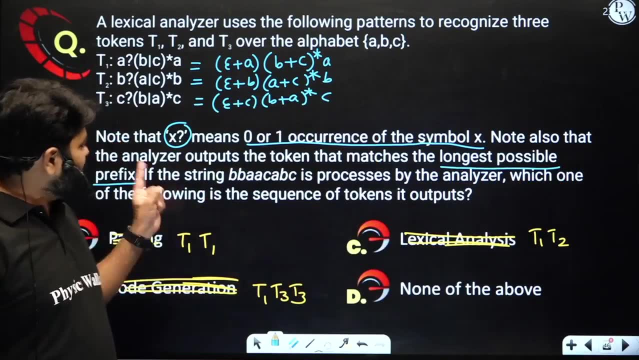 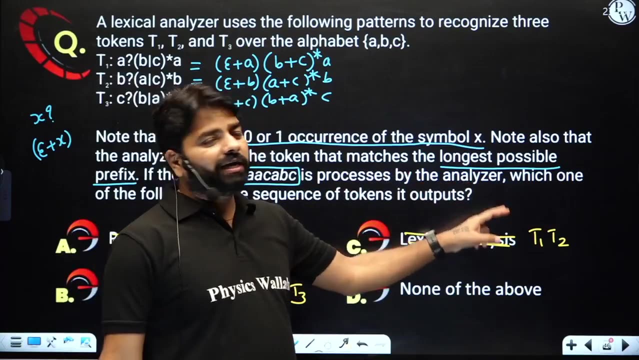 b plus a whole star c. this is how you got to know what is this? uh, question mark representation. note also that the analyzer outputs the token that matches the longest possible prefix, and you need to look at always longest possible prefix. we'll see that again. the string is clearly mentioned here, whatever it is, and is processed by the analyzer, which. 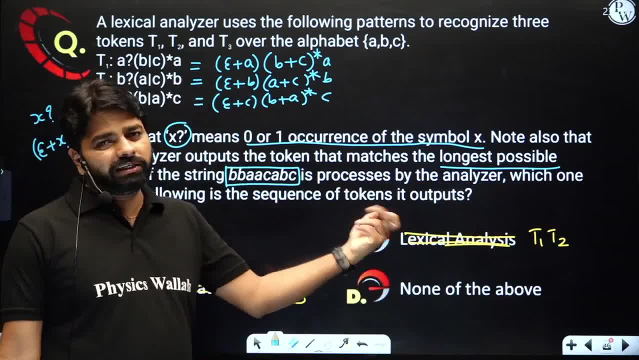 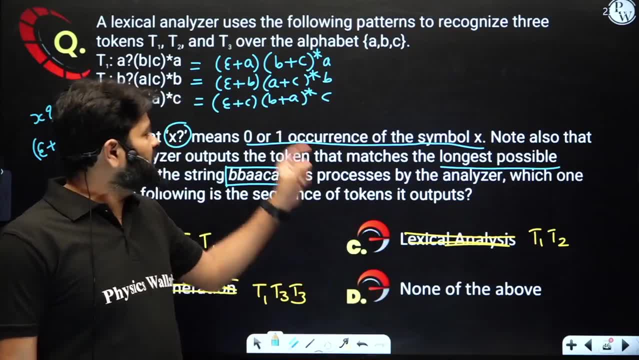 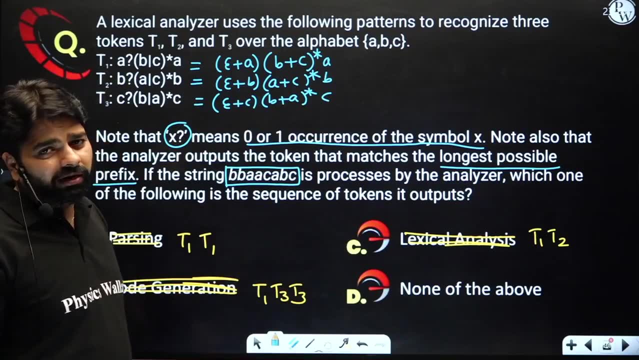 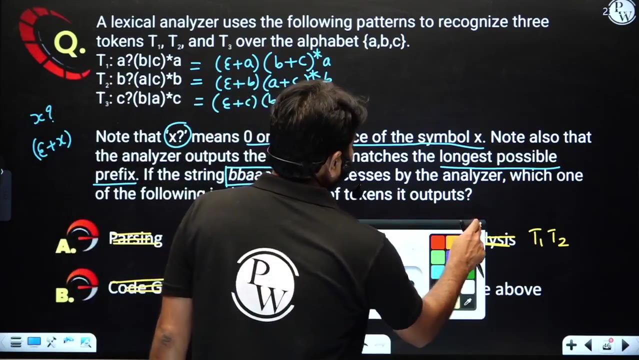 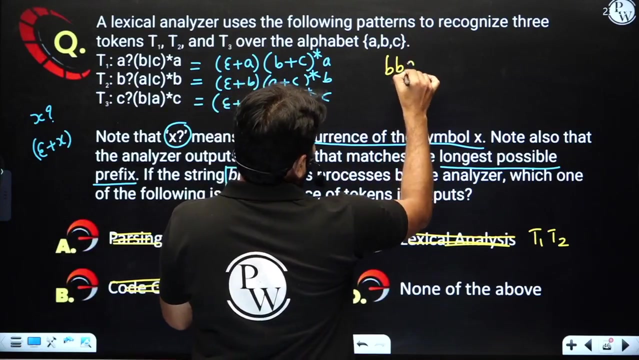 one of the following is sequence of tokens, its output. so there are some options and definitely one of the options only correct because you are following longest prefix match. okay, if you have more than one option also, we will see it, that's, you know. anyhow, should not be when you implement a compiler. now, this is the key point for you. i'm just writing here b, b, a. i need. 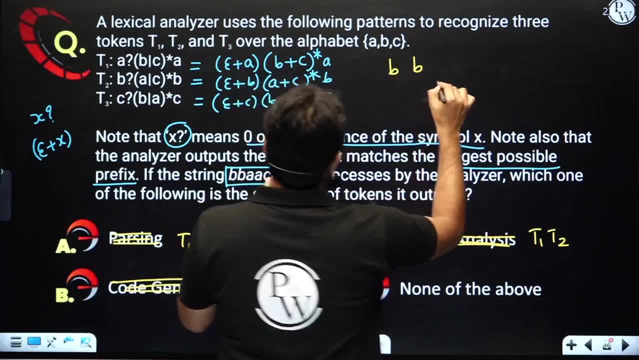 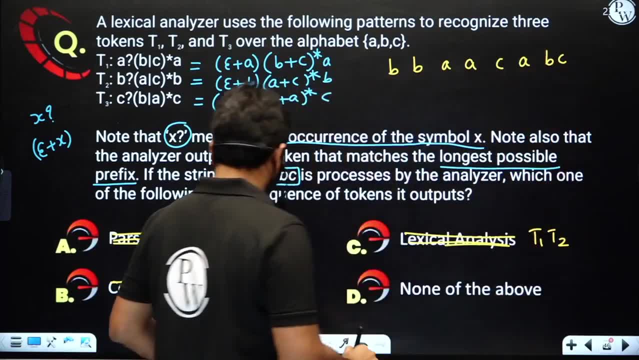 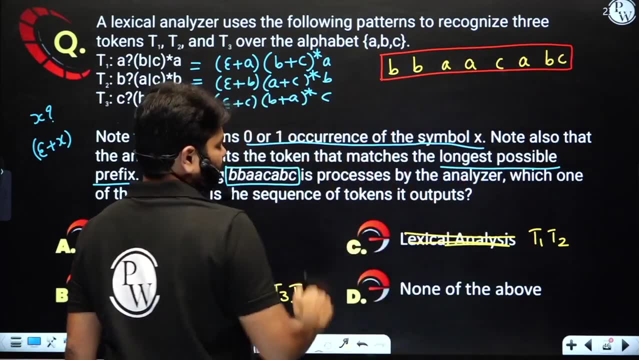 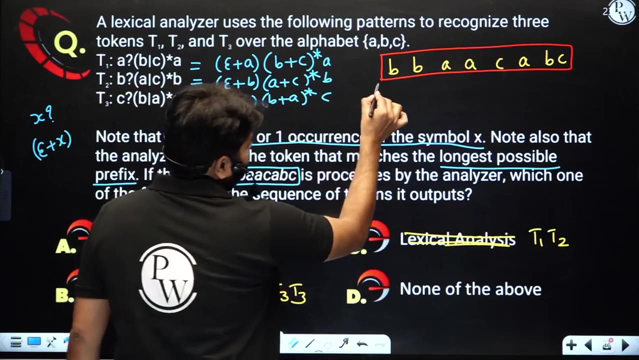 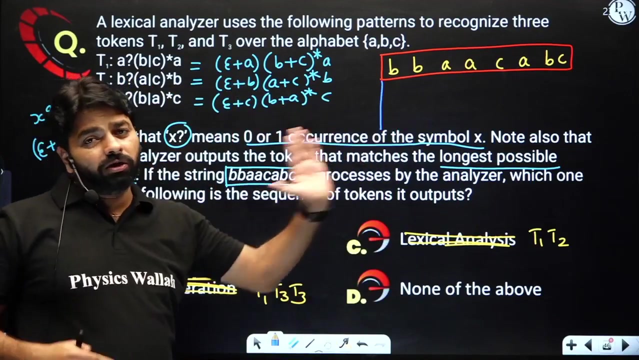 spaces also b, p, a, a and c, a, b, c. this is your input or this is your program. you can assume that is your program. you can assume that is your program. sorry, how many tokens are there? three tokens, anybody can match right, but who will be matching the longest preference? now you need to focus. 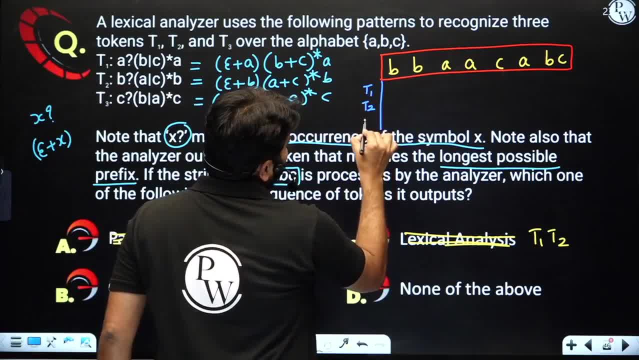 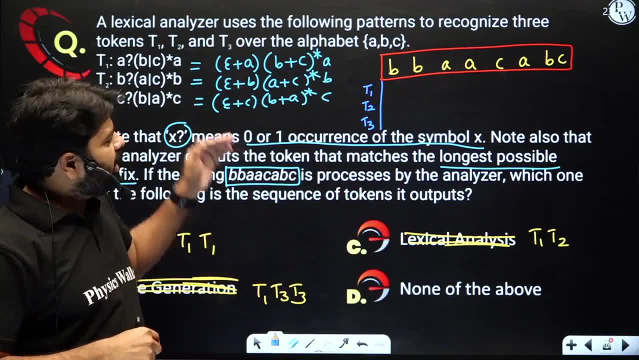 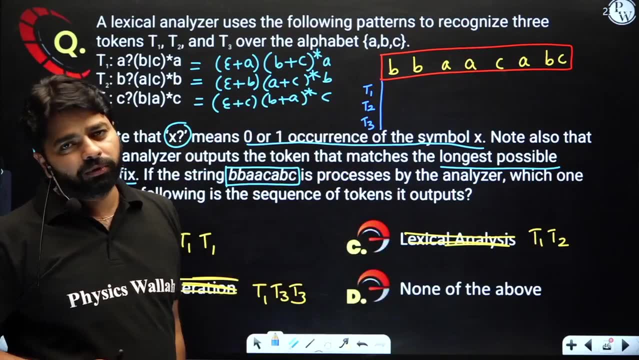 on three things: t1, t2, t3. you don't know exactly who is going to be the longest, but you need to look at who is going to generate the longest one. if any of these three is producing all our entire sequence, then that is only the possible token. produced right, but we don't. 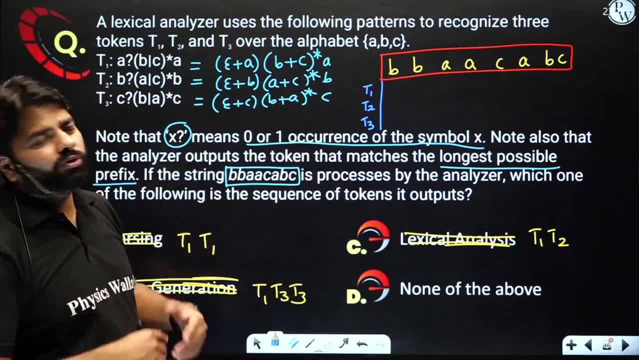 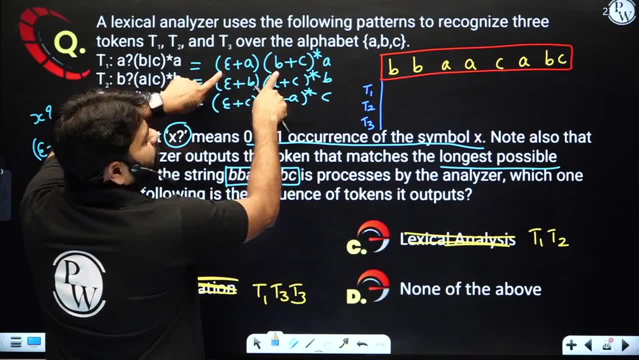 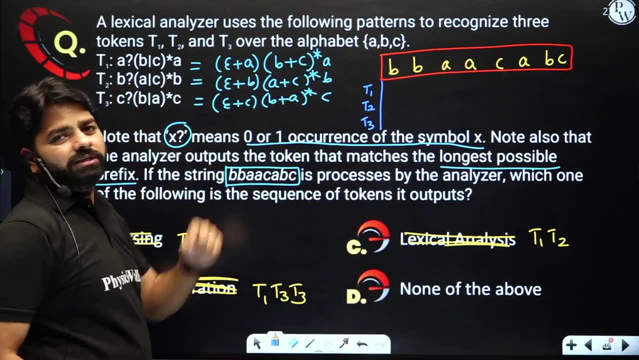 know right. let's try t1- how long it can produce this string as a prefix. now let's try b. can you produce epsilon b? yes, you can produce, they can be. can i produce s, b, b. can i produce this a? yes, but this a i can't produce with this. i can do here b. 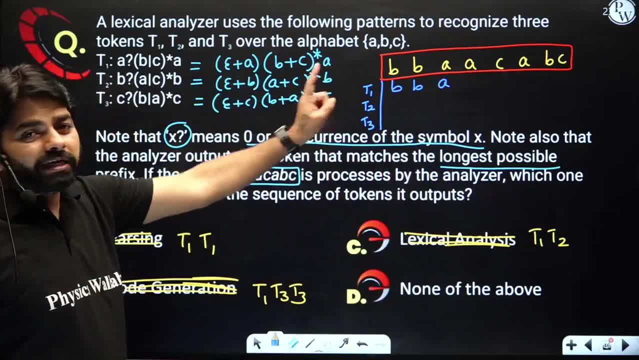 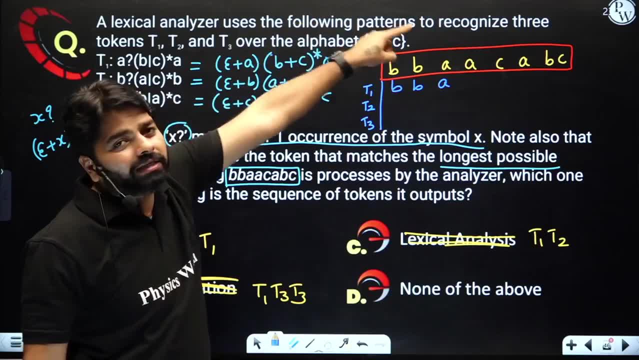 b a up to here, only see that second icon. i can produce two b's from here because of star is there. i can repeat twice. then, once i go to this, a other a i can't produce from this option. okay, so b b a. that's all. right. now let's try b b a now. let's try b b a, that's. 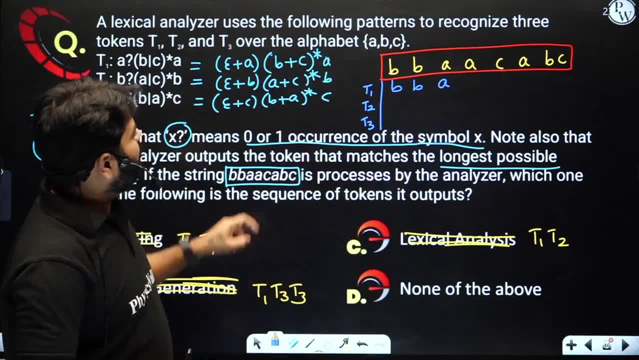 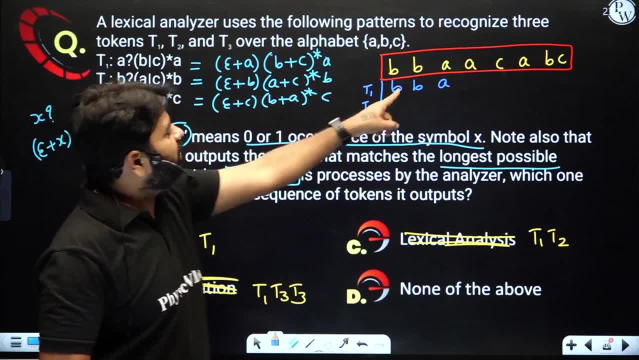 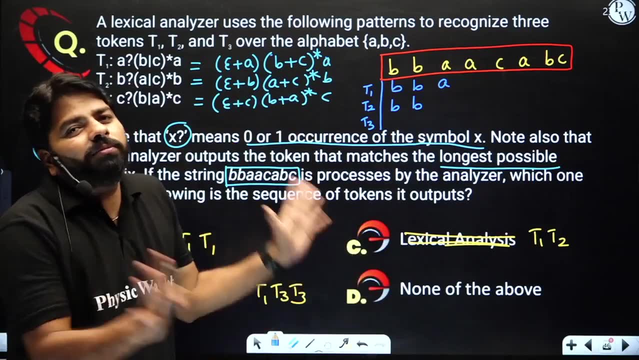 the longest that t1 can produce and t2 now, uh, b, i can produce here another b. if i want to produce i have to go here. if i go here i can't come back. so b, b, that's the longest one i can produce with the t2. that's t2, definitely not going to be the first token, because t1. 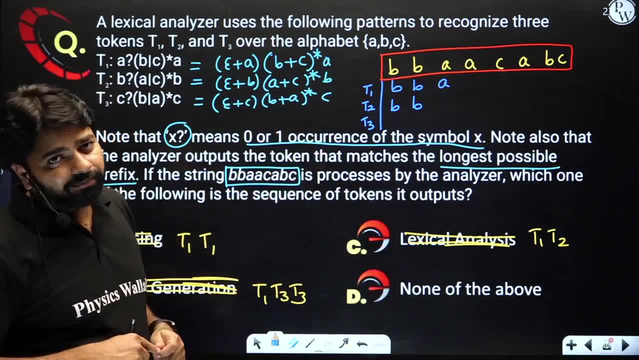 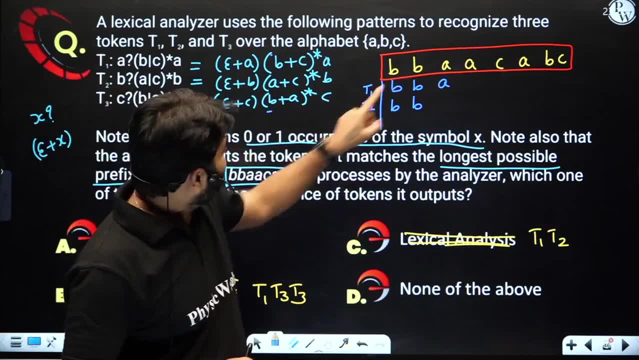 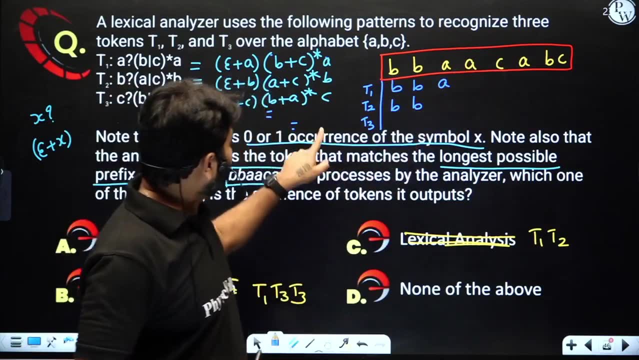 already showing the longest. okay, now let's go to t3. go to t3. b i can produce. i can put epsilon here. i can take b here and another b i can take from here. only a i can take from here, a i can take from here and c i can take from here. 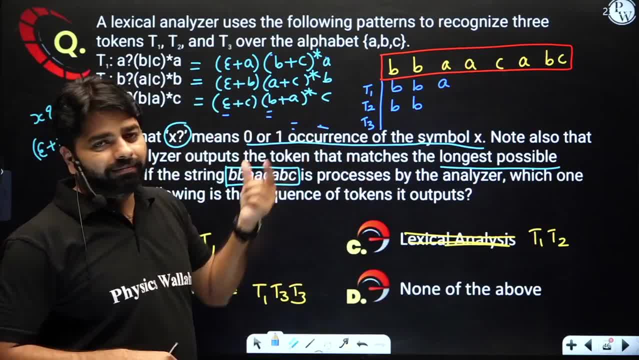 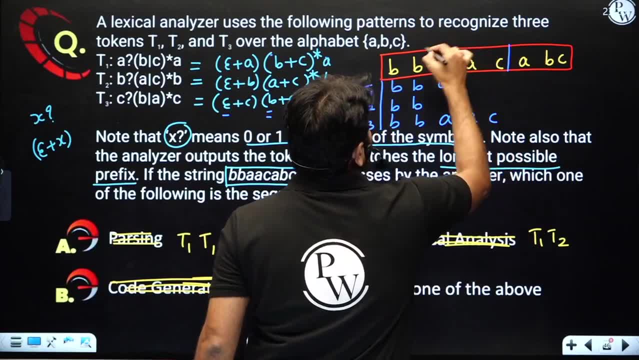 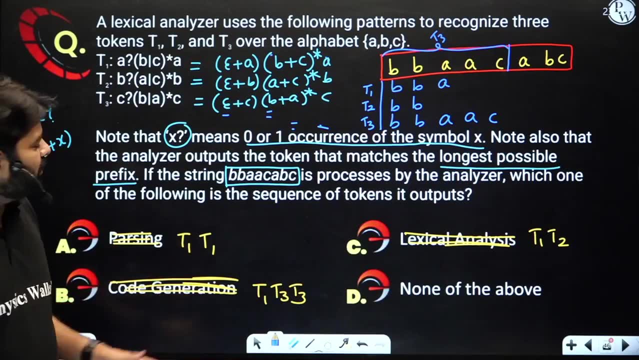 see that epsilon b, b, a, a, c i can produce up to here, that means till this point. till this point we have just t3. first token is produced. looks like, when you look at the option, nobody matching because in the exam they started with t3 somehow here, okay, the first option. 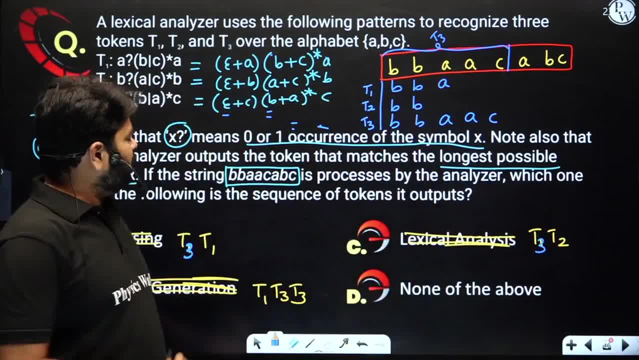 they have taken up to here, but now they are not matching. no one is matching they have. they have taken only a from here, only a i can take from here and c i can take from here. can t3? okay? so then you had a confusion. which option is? because many options are having the 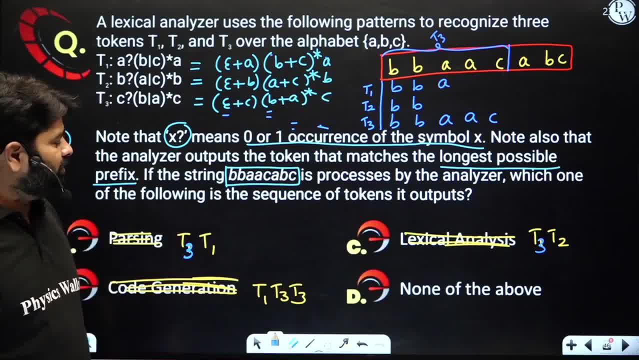 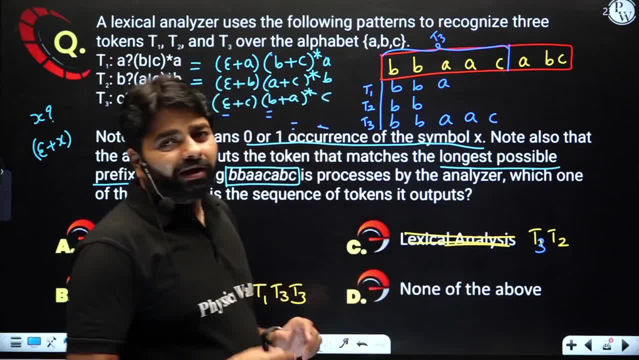 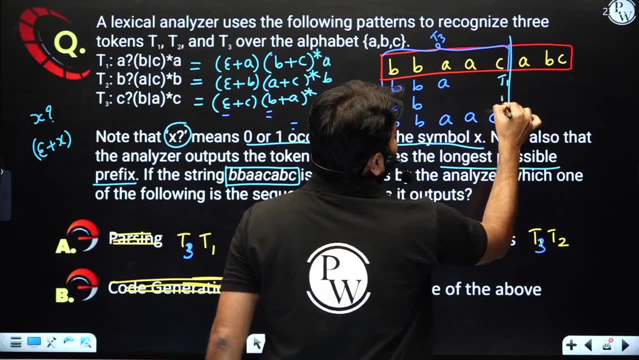 first token is t3. so that's the problem in the gate exam. okay, anyhow, don't look at these options right now and now let's move to the next remaining again. it will start again. it will start now. look for a t1, t2, t3- who is going to be the longest one, right? that is very important. 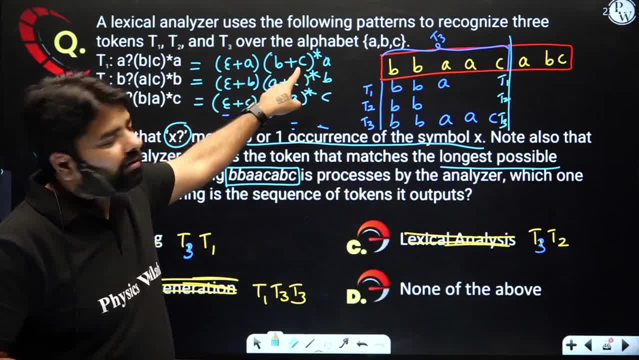 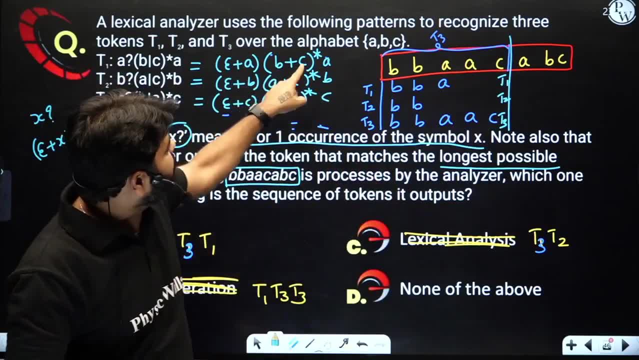 a b c. can i have here a b c? i can, but i should end with a. i'm not proper if i i can't generate a b c. i can generate a b c a. see that that a b c, even though i have till here, but i am not. 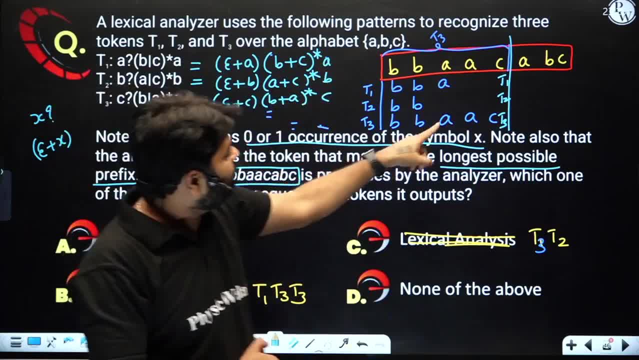 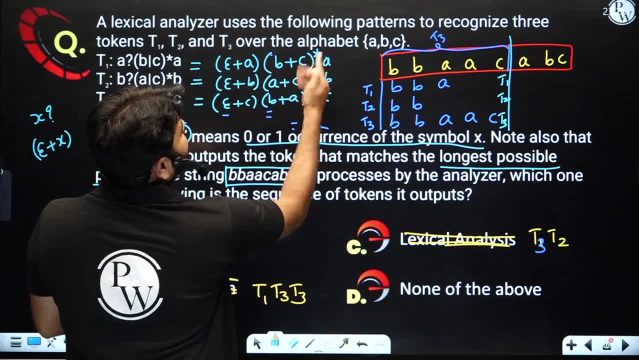 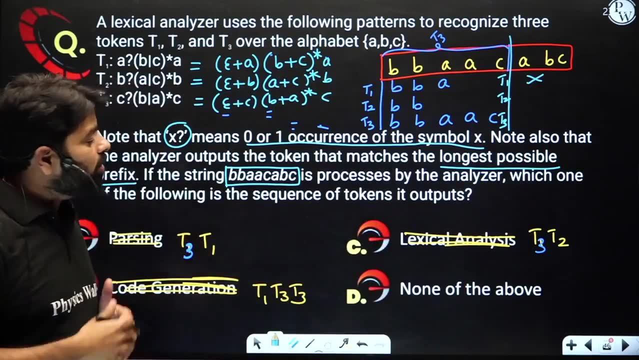 complete, because this a need to be there. see, if you look at here, i stopped here because that t1 was ending with a. but now this one, i can generate what a, b, c, till here, but without ending with a, t1 is not correct. you, so t1 can't generate at all. a, b, c is not possible. what is possible? a, b, c, a is possible, but i don't. 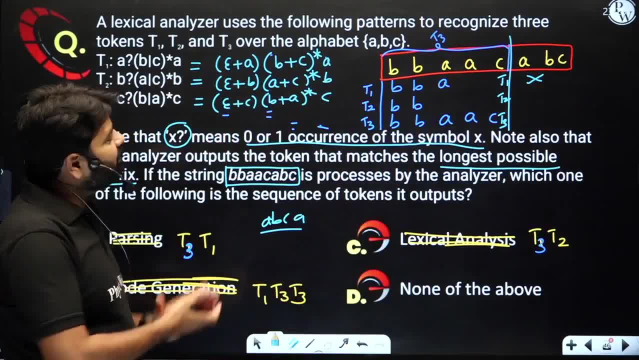 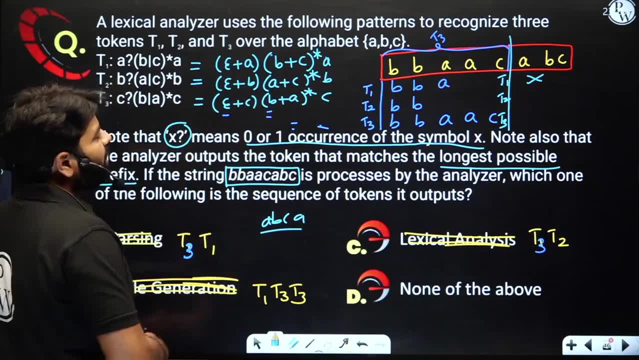 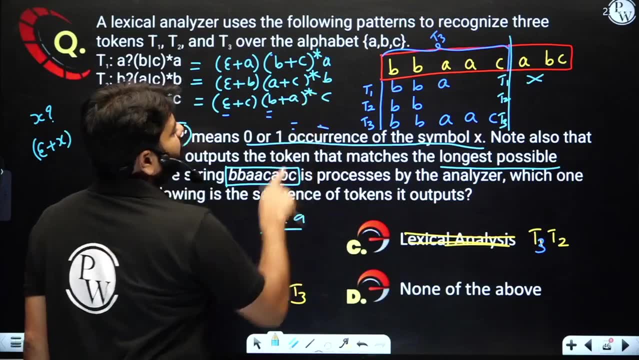 have a there right now, so i can't generate a b c with this expression. right, it can't generate a b c. what can generate a b c a? remember that part of the string only it can generate. that doesn't mean that whole t1. okay, next one, epsilon a b. but that can generate a b but not a b c. so this one i can. 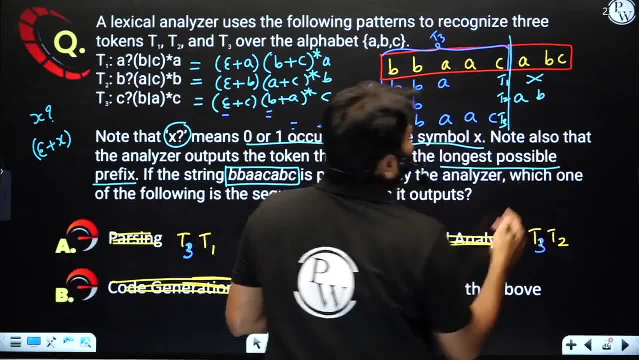 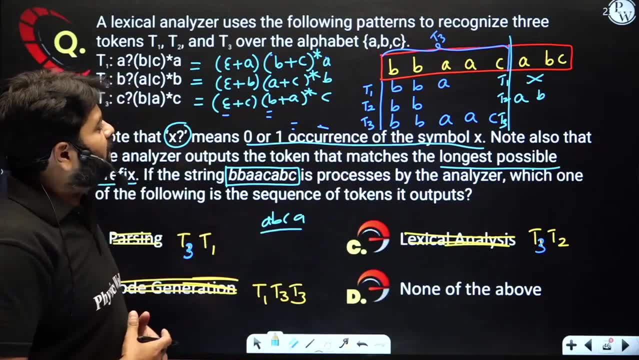 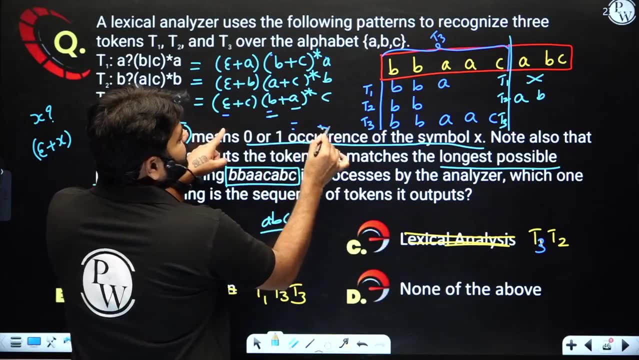 generate a, b, a. it's okay, may be correct or may not be correct, because after that, if t3 can't do it, i will take t2, because that is the longest now t3, a, if epsilon, i take here a, b, then c, that's now complete t3. 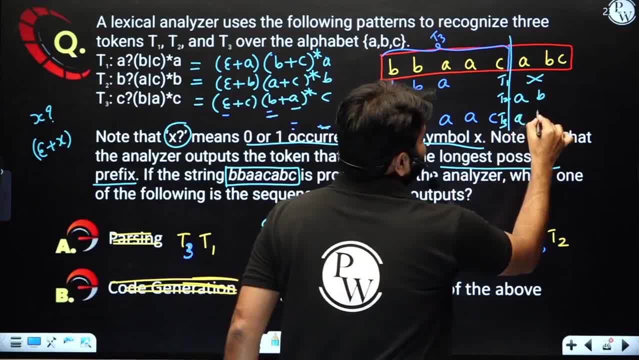 a, b. i'm properly ending with c. also this a, b, c i can generate. so now this is also t3. so one of the option you will see: t3, t3. that's going to be the right one. so now this is also t3. so one of the. 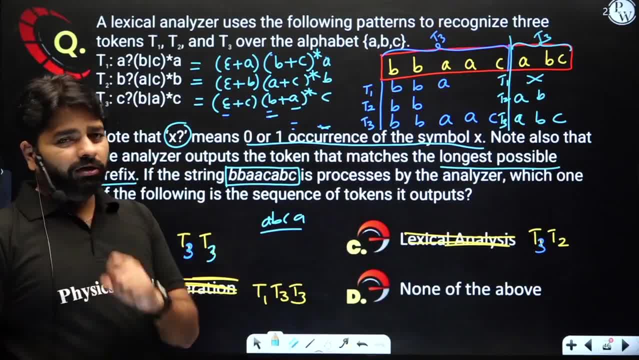 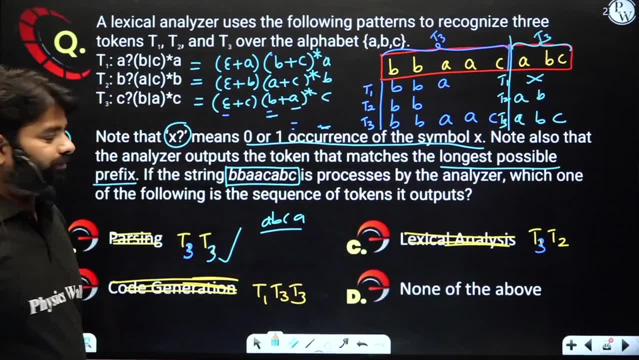 option, you will see: t3, t3. that's going to be the right one. so now this is also t3. so one of the option- t3, t3, now t3, t3- is the right answer. that's all you need to do, if you can do it properly. how to start and? 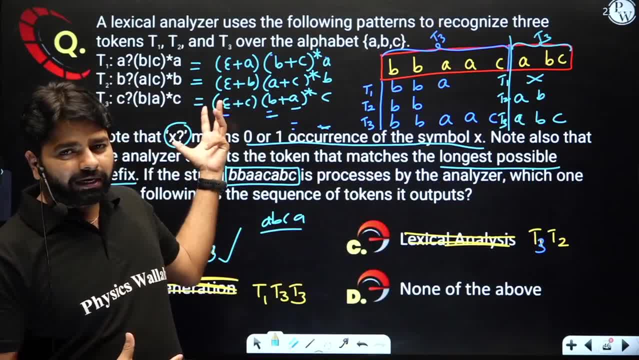 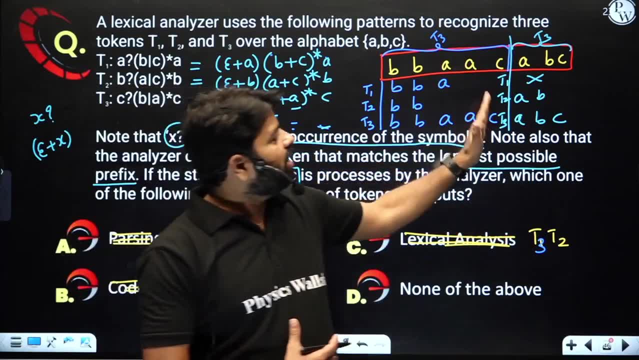 what is the longest prefix match? i have three rules, three patterns. then which one is going to match longest, then that will be considered as a token till that point. after, again, all the tokens you are trying to match, who will match next? okay, the answer is t3. t3 is going to be the 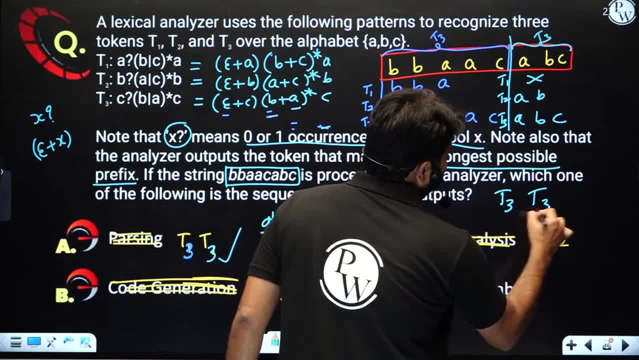 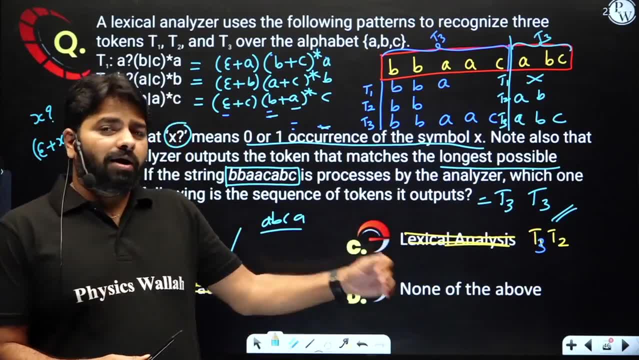 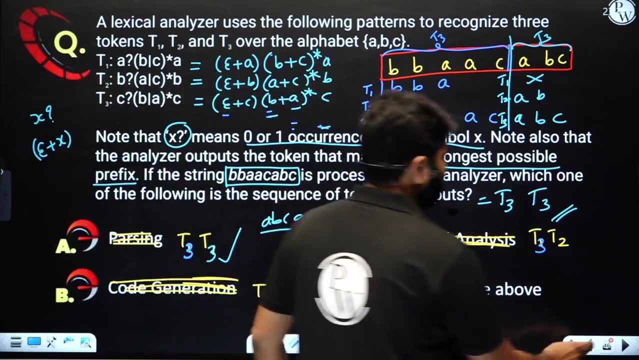 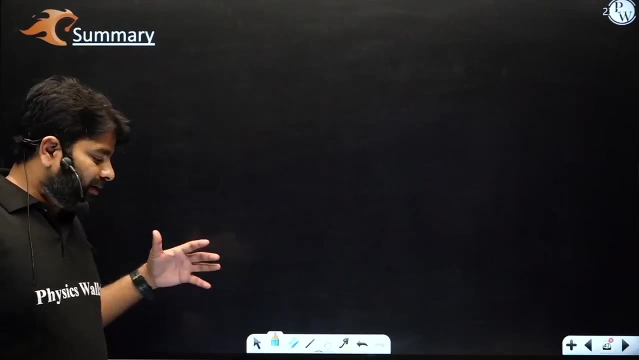 right option for this: t3, t3. fine, sometimes they may ask how many tokens are produced in the sequence of tokens: t3 followed by t3. that's it. so if overall, in overall, in this introduction as well as we compiled in, let's write analysis. it's very easy. it's very easy for. 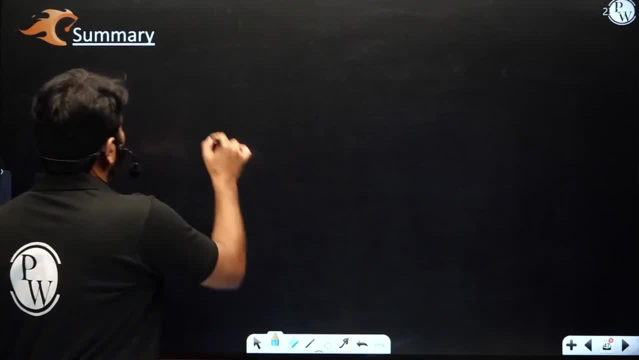 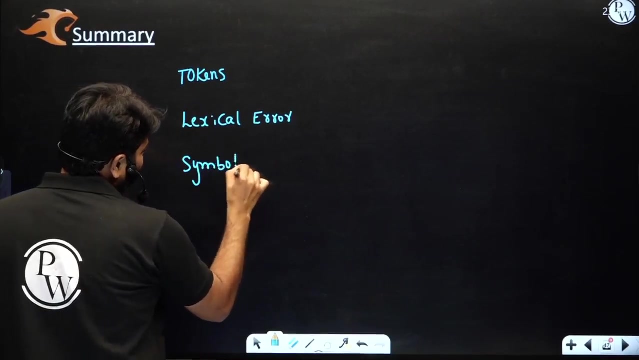 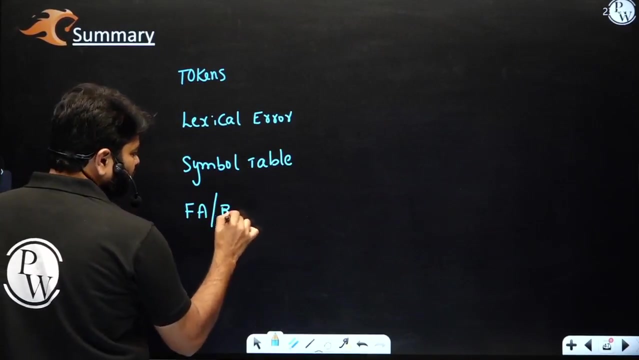 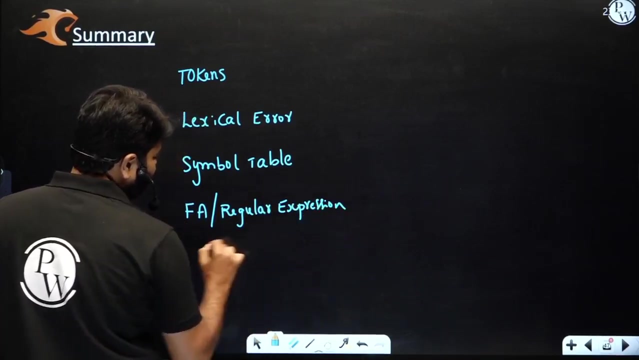 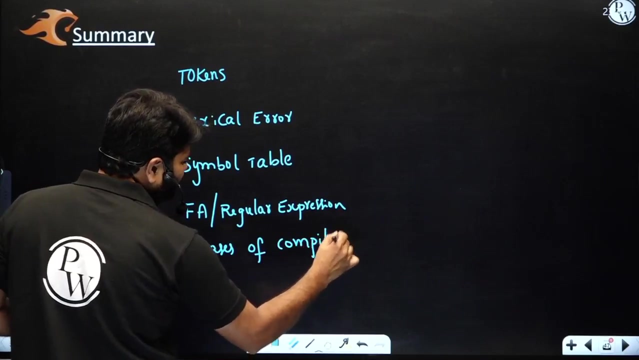 that is just. you know how many types of tokens. tokens focus on this. the whole lecture analysis will become easy. and then, what is lexical error and what is symbol table and finite automata, regular expression used to design lexical analyzer. phases of compiler five, six, seven, and you should know how to use these words. basically looks like six words, but